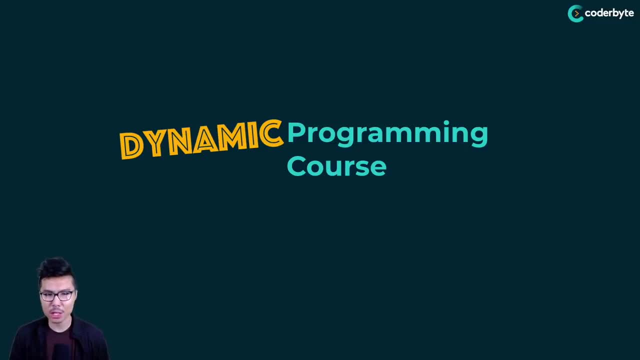 and algorithm interviews. you definitely need to know dynamic programming, So I hope to give you all the background knowledge you need to really crush those types of problems. Now, that being said, what problems are we going to solve throughout the course? Here are a few examples. So one question I can ask you is to calculate the 40th number of 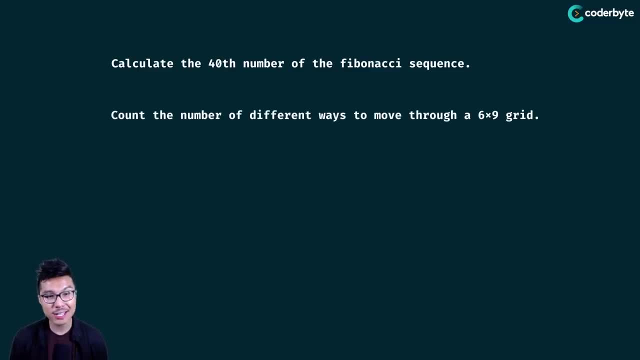 the Fibonacci sequence seems like a very easy problem. can also ask you to count the number of different ways to move through a six by nine grid, Or something like that. You can also ask you to count the number of different ways to move through a six by nine grid, Or something like that. You can also ask you to count the number. 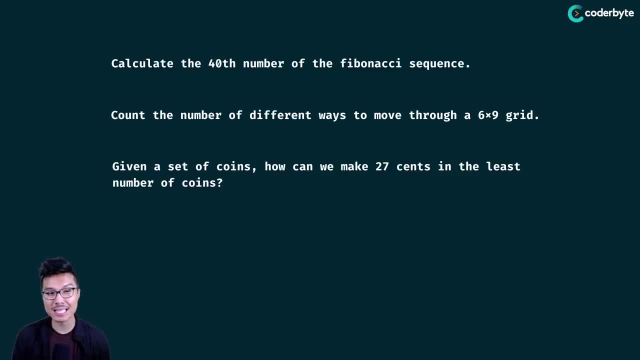 of different ways to move through a six by nine grid Or something like that. You can also ask you to count the number of different ways to move through a six by nine grid, Or something different like: given a set of coins, how can we make 27 cents in the least number of coins? 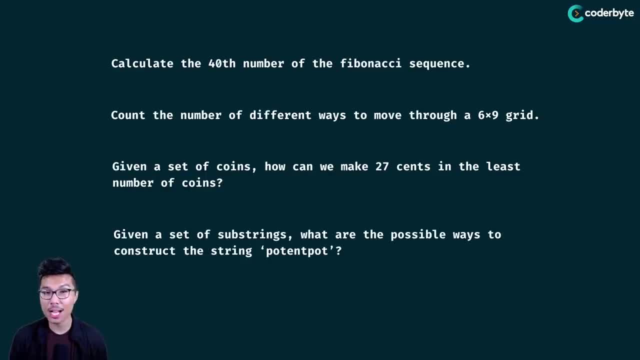 A final example would: be: given a set of substrings, what are the possible ways to construct the string potent pot? And all of these questions really fall under the umbrella of dynamic programming, And this is really why I think the topic has such a bad reputation for being. 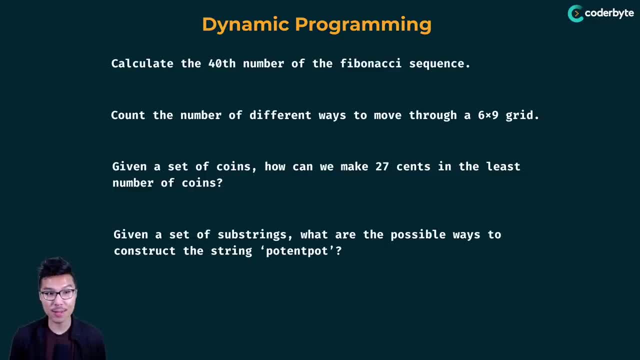 very difficult Because the problems range so much. right, It looks like these problems are totally different And there may not be any underlying mechanic that we can use to tackle all of them, But the short answer is: we really can if we have the correct way. 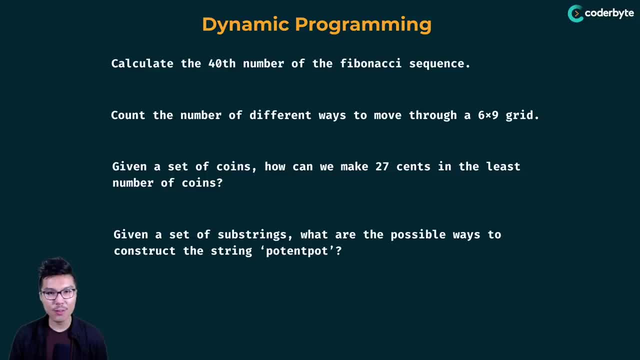 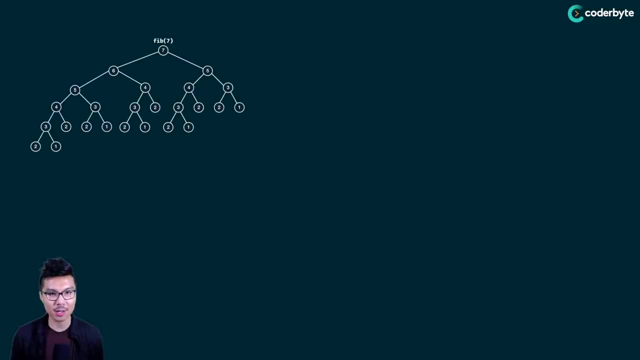 of thinking about these problems. That being said, let's go over the overall format of this course And this course. I think our key to victory is going to be to really visualize all of these algorithms right. So we're going to spend a lot of time drawing things on the 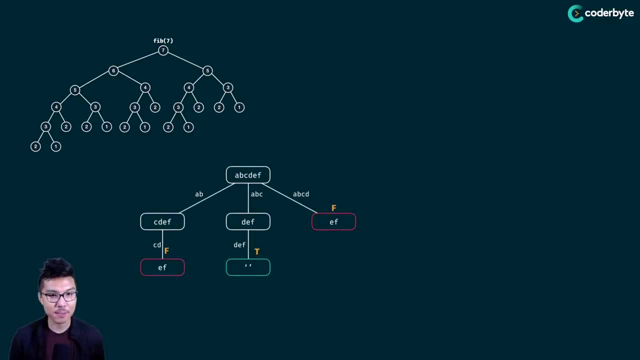 whiteboard as well as visualizing things with animations. To me, all the heavy lifting on an algorithm interview is really done when you come up with that picture right, When you describe that process and then translating it into some code is really the most important. 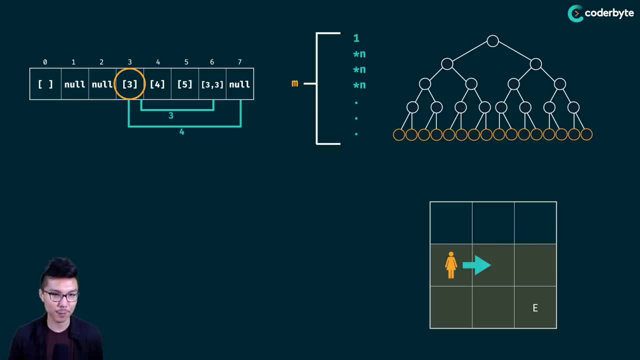 part right. The hard part is designing the algorithm in the first place, right? So we're going to draw a lot of things to make sure we understand the structure of the problem as well as coming up with a solution, And then, once, we're really happy with that pen. 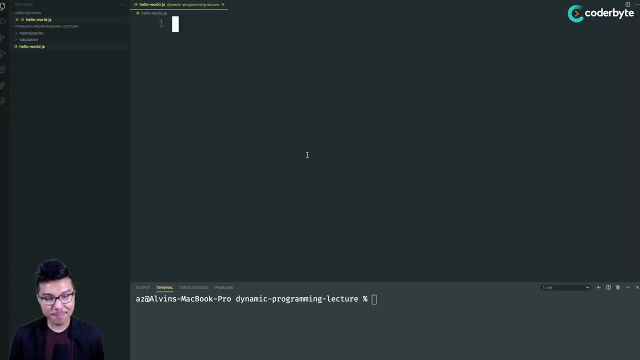 and paper process, then we'll hop into my editor and we'll solve it in some code. we'll probably have to go back and forth until we end up with an algorithm that runs in an efficient amount of time, right? So it goes without saying we're also going to analyze the time. 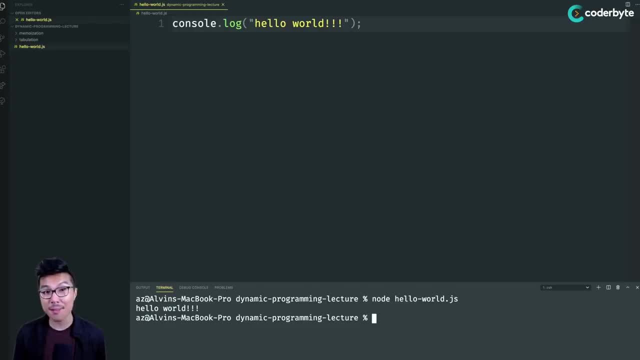 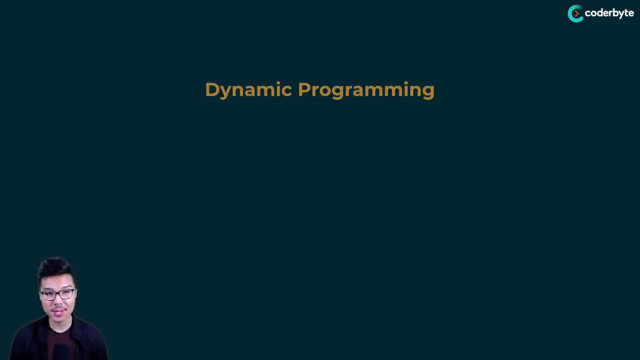 and space complexity of all of our solutions. I'll be writing my code in JavaScript and you'll find it very easy to translate our solutions into the language of your choice. So in this course on dynamic programming, we're going to divide the material into two main 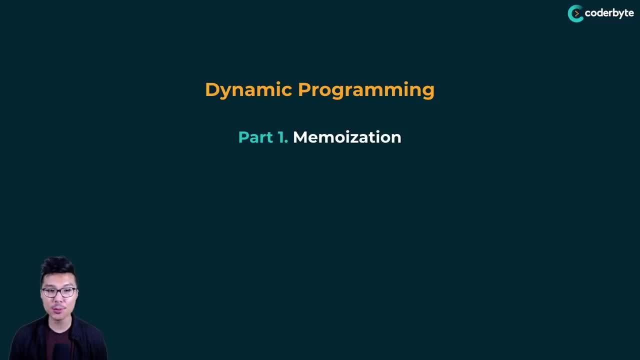 parts. Part one is going to be about memo ization and then part two is going to be about tabulation. And don't sweat it if you have no idea what those two terms refer to. don't worry, we'll reach all of that material step by step together. I think you're going. 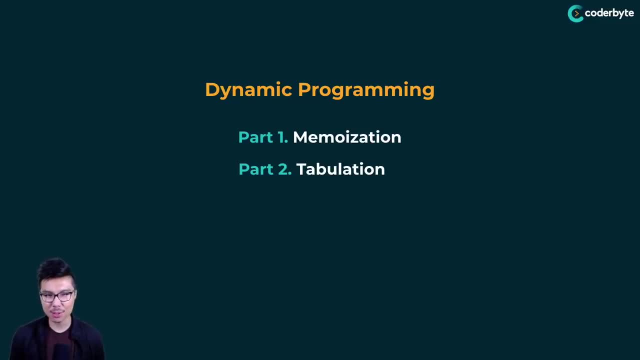 to realize if we actually learn these things in a very logical progression. we're almost like discovering these algorithms, And I don't just have to tell us what the algorithms are, what the rhythms are. So, in terms of prerequisites, I won't assume you know anything about dynamic. 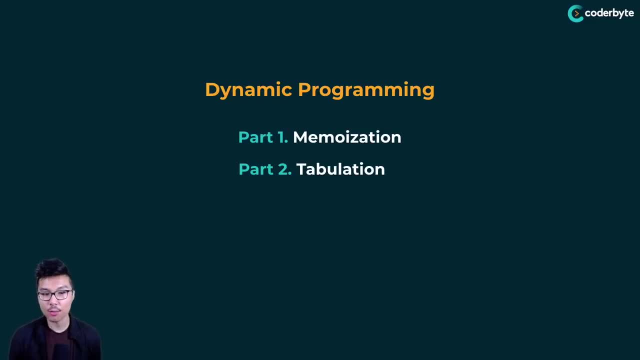 programming. But I will assume that you understand a little basic recursion as well as some basics of complexity analysis, right? So you're sort of familiar with big O notation And I'm sure that we'll be able to review some of that notation as we move along. So I think 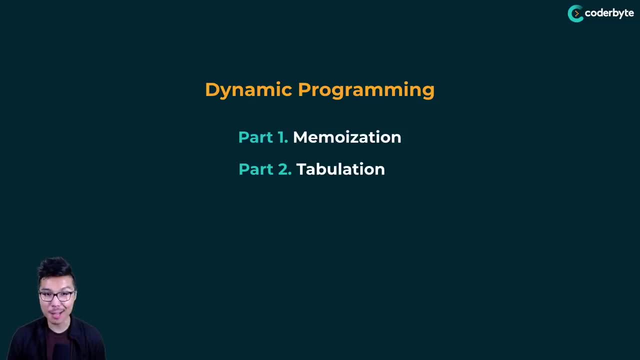 with all that out of the way and no further ado, let's hop into the course. All right, so where should we start? Well, I want us to really ease into this new topic, And so what we'll do is we'll start by attacking a problem that you've probably seen in the past, that is, I want. 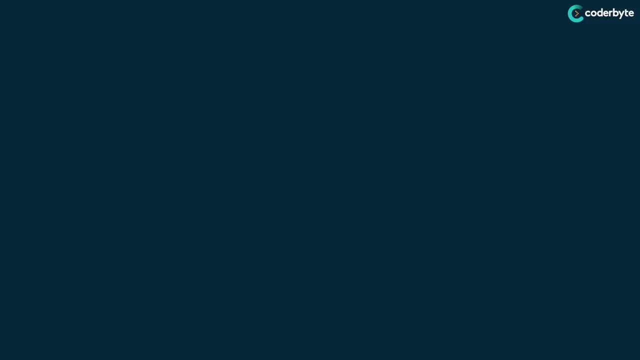 to solve a Fibonacci problem, And so for us, we'll have a particular phrasing of the Fibonacci problem. what I want to do is write a function fib of n that takes in a number as an argument, and I need to return the nth number of the Fibonacci sequence And just to review how. 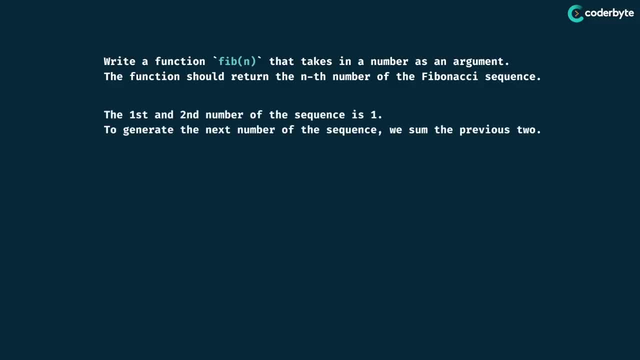 does the sequence work? Well, the first and second number of the sequence is just one, And then, at any point in time, to generate the next number of the sequence, we can just sum the previous two. So, for example, these are the first few numbers of the Fibonacci. 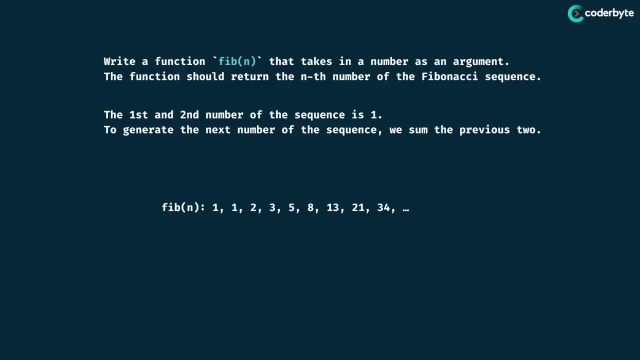 sequence right. It starts one, then the second, and then the third, and then the fourth, and so on. What I'm saying is your number needs to take in like a position of the sequence. In other words, if I asked you for the seventh Fibonacci number, you need to return the answer. 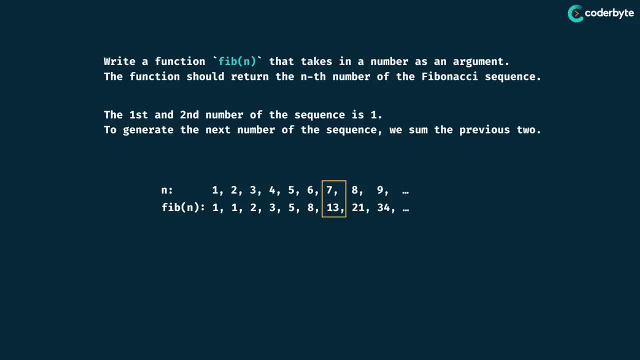 13,. right, Because the seventh Fibonacci number is 13.. And how do we actually calculate that 13?? Well, logically, it's just a sum of the previous two elements. that is, five plus eight gives me the 13.. So very, very classic function here. And to really get us going, for what? 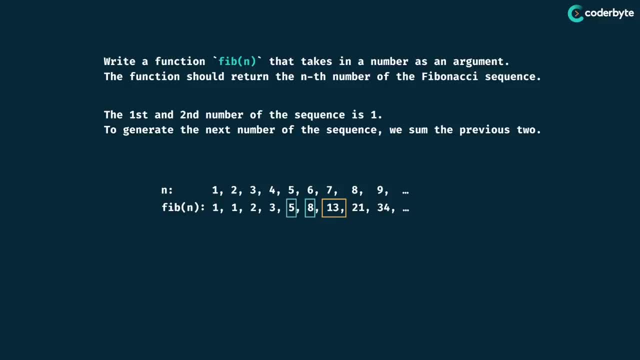 we do later on in the lesson. I'm going to require us to solve this one problem And we're going to solve this one recursively. right, it's really going to be at the heart of a topic for today, So why don't we kick things off by quickly implementing the classic? 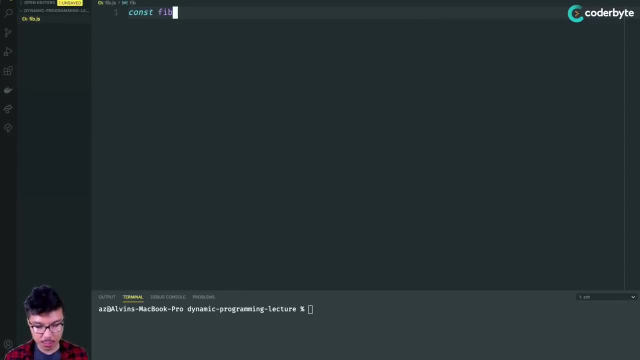 recursive implementation of a Fibonacci function. probably written this function a few times in your programming career, usually one of the earliest examples of recursion that we face. So we'll just lay out the classic implementation here. So I want to take in a number, n and 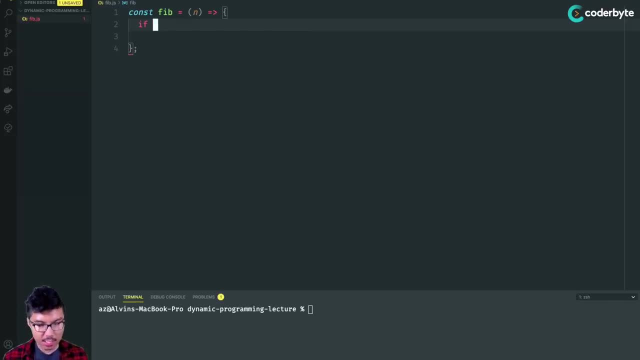 I want to return the nth number of the Fibonacci sequence. Like we expect, the base case is just about: you know the first two numbers of the sequence. In other words, if I'm given some n, that's going to be the first two numbers of the sequence. So what I want to do is I'm going to 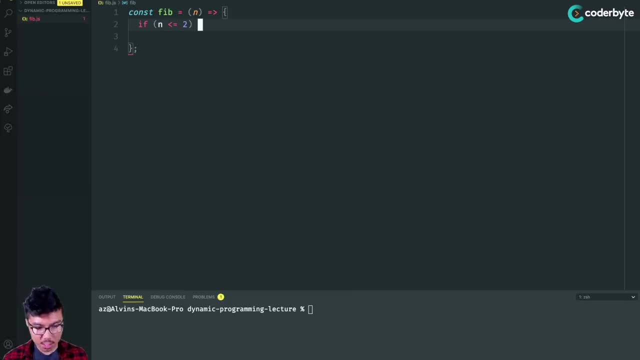 take some n that's less than or equal to two, then what I should do is just return one- And I'm writing this because, hey, the first two numbers of the Fibonacci sequence are exactly one. But in the recursive case in general, what I can do is just return the. 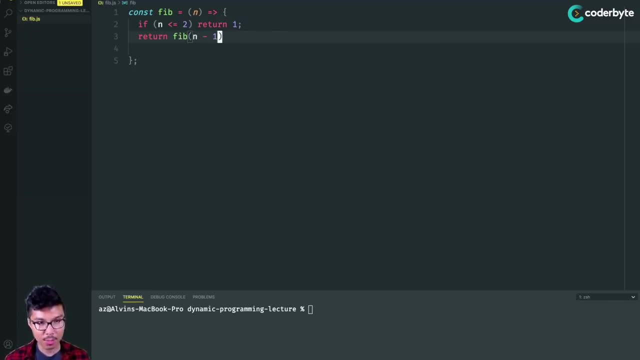 sum of the Fibonacci number right before the one I'm asking for, as well as the Fibonacci number two before the one I'm asking for. right Again, the kind of baked in recursive nature of Fibonacci is to calculate some Fibonacci number, you can take the sum of the previous. 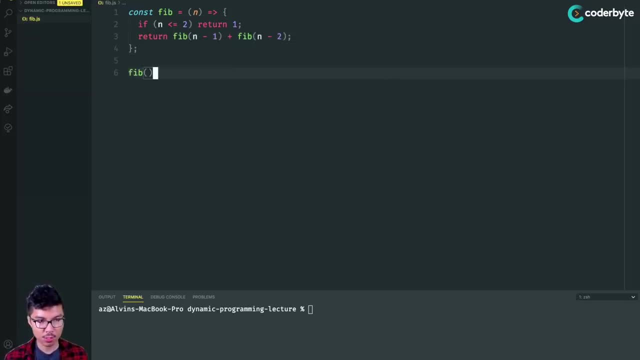 two numbers in the sequence right Now, of course, we should test our code for some correctness. what I'll do is call a few examples of this Fib function. So I'll try Fib of six, seven and eight, And I should 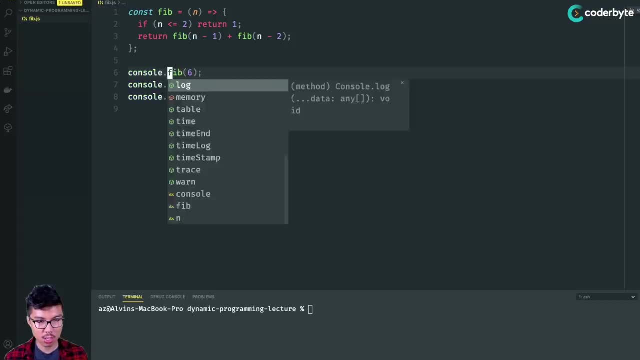 get the answers of eight, 13 and 21, respectively right, So let's give this a go. I'll run this in some JavaScript. There we have it right: eight, 13 and 21.. So this is a very, very. 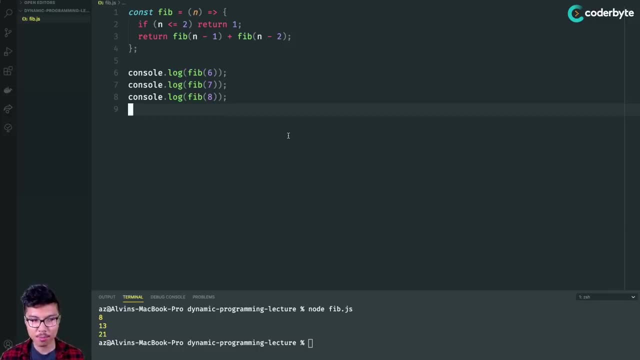 classic implementation of Fibonacci. You've probably seen this many times before and we did solve it recursively. And really what I want to do is give some larger number, you know, to this Fib function. So what if I asked for, let's say, I don't know- the 50th Fibonacci? 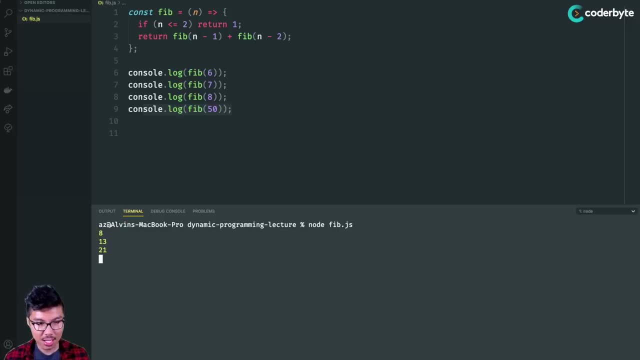 number seems like something reasonable to ask for. So if I give this code a shot, looks like the first three calls to Fibonacci do work fine. right, I get eight, 13 and 21.. But the fourth call is actually still running right. my program actually hasn't finished. 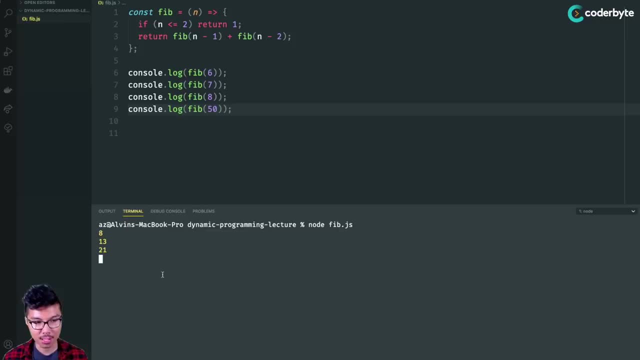 And this is a big issue with this type of implementation with Fibonacci. So obviously this Fibonacci function needs some work. Let's go ahead and head to the drawing board, Alright? so it's apparent that our Fibonacci number is still running, So let's go ahead and head. 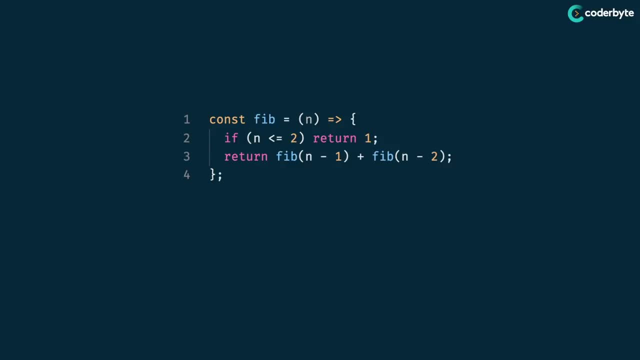 to the drawing board. Alright, so let's go ahead and head to the drawing board. Let's go ahead and head to the drawing board. Alright. so at the end of the drawing board we'll see that a Fib function is correct in that it returns a proper result. However, if we 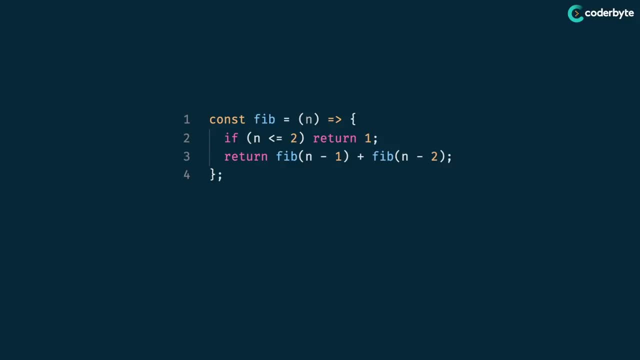 give it a large enough value of n. it's pretty slow. That is our function- has correctness but lack some efficiency In the long run. we definitely want to improve this implementation of a recursive Fibonacci, But to do that it's really important that we identify exactly. 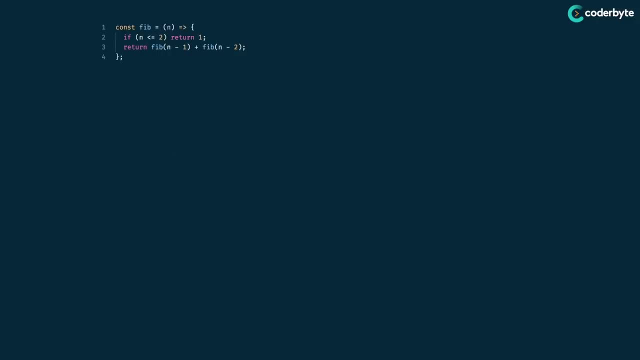 where there's even room for improvement, And to do that, I think we should draw some things. This is something I think students actually need to work on. Students have this habit of trying to like picture everything in their mind, And that works for some easier problems. 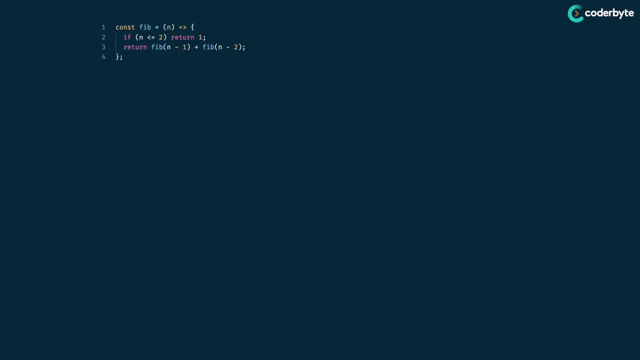 However, when we want it to work, we can't do that. We can't just go ahead and draw, tackle more complex problems if we just try to capture all this information just mentally, without drawing it on like pen and paper or marker and whiteboard or chalk and chalkboard. 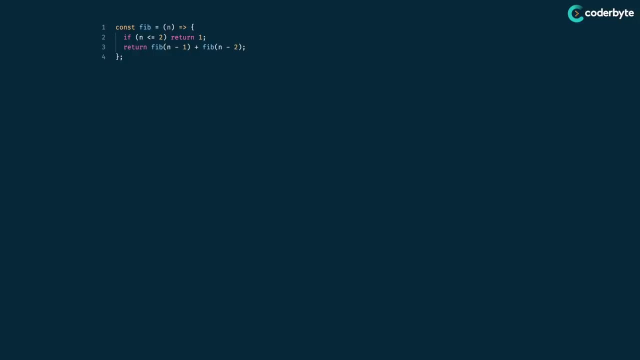 you're going to really lose track of the finer details in these structures. So I want us to be very, very methodical And we're going to draw really how you should visualize a problem like Fibonacci. And so over to my drawing. let's say that I wanted to trace through what happens when 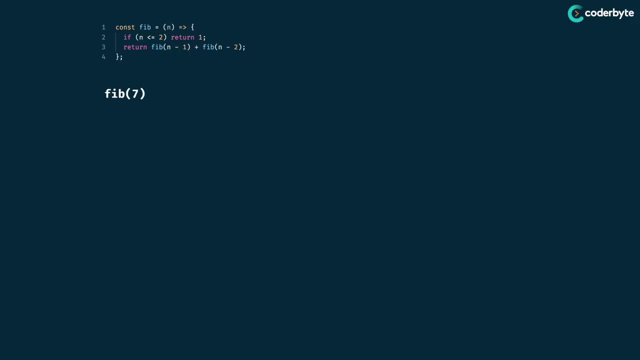 we call fib with the number seven, that is, I'm asking for the seventh number in the Fibonacci sequence. I know that in the long run I should get back a 13,. right, 13 is the seventh number in the sequence, So I'll keep that goal in mind. But over to my drawing. let's say I called fib of 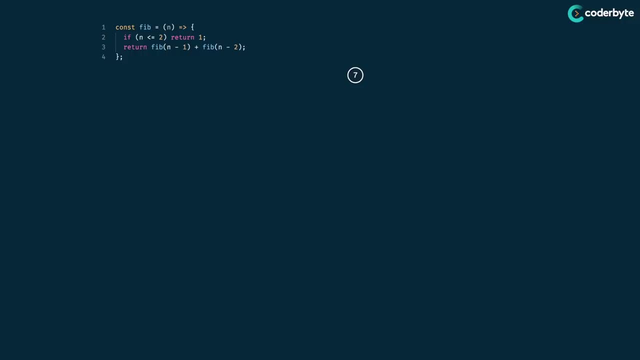 seven. I'll denote that by really drawing just a circle with my value for n inside. So if I think about this call to fib of seven, what is it going to do? Well, I know that seven is not the base case, right? Seven is not less than or equal to two. So this call is going to branch out into: 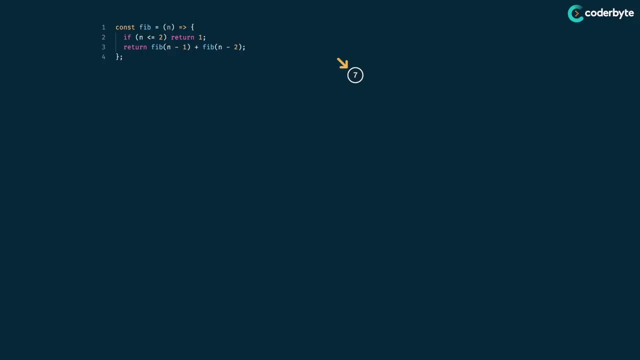 some more recursive calls, In particular on its left hand side. I'm going to call n minus one, which is going to be n minus one. So I'm going to call n minus one, which is going to be n minus seven. So I'm going to call n minus one, which is going to be n minus one. So I'm going to call n minus one. 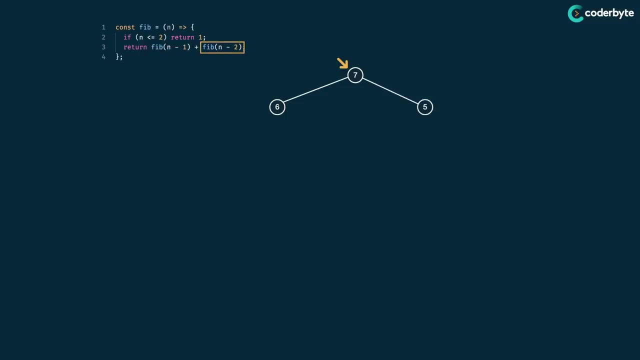 which is six. on its right hand side I'm going to do n minus two, which is five, And at this point I carry over the same logic for the other nodes of the structure right. If I look at the sixth node, if I'm rooted right there, then that will have a left child of minus one, So five it will. 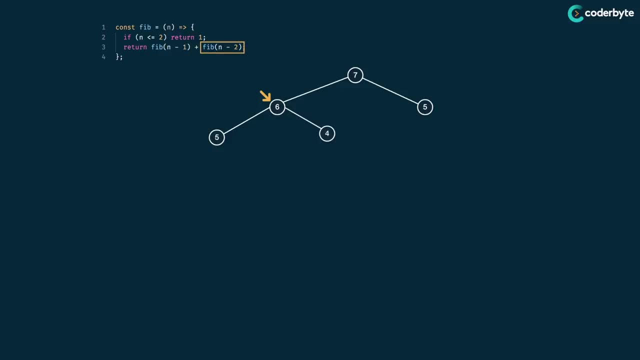 also have a right child of minus two, So four. you can start to see a pattern where really this recursive structure just visualizes as a tree, which is really neat. If I hop over to this five node, it too will have some children right, Minus one on its left, minus two on its right, And we 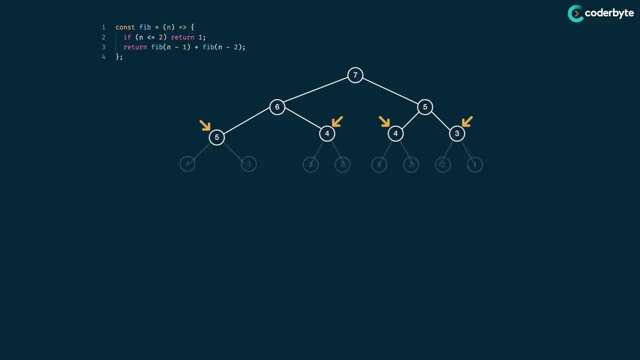 will actually just have a child of minus two on its right And we will actually just have a child, just continue this process for most of these nodes. But let's say we pause right here. So you'll notice that these nodes that I have pointed to in red, they're actually the base case, right For 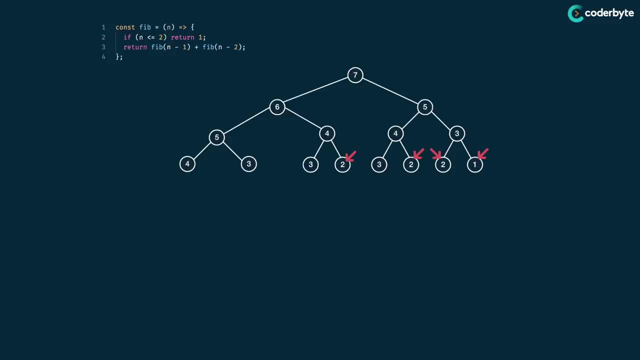 those nodes I have values of two or one And I know that those function calls will return immediately. More importantly, that means they don't branch into any further calls. So I don't want to start fleshing out the tree of those nodes. Instead, I'll look at things that are not 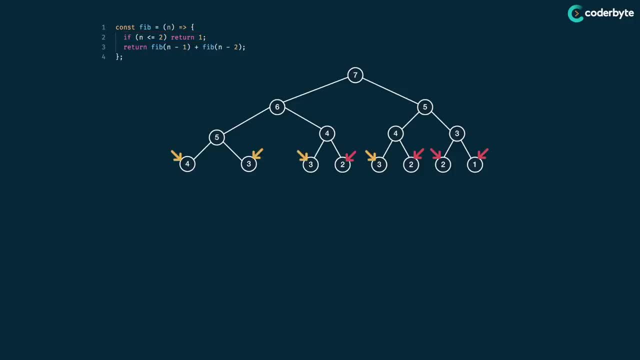 the base case, right, That is, these nodes in yellow. So I'll continue to flesh out this tree But not branch out further for the base cases. So at this point I built out my entire tree and I stopped fleshing out the tree whenever we had a. 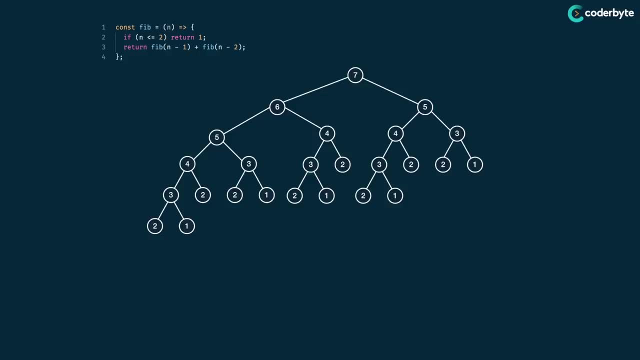 base case scenario. So this is actually the full recursive tree. Remember that the numbers inside of the nodes here represent the end that we passed in. That being said, if we have this visualization, how does this tree really calculate? the Fibonacci answer: right, So let's start to break it down. 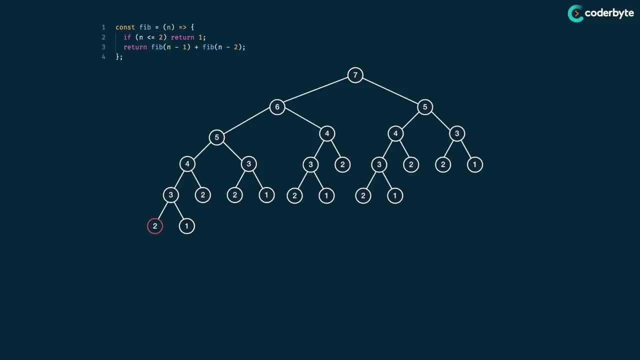 over here. Let's say, I looked at some node, in particular this base case node, which is a node of 12 k. right, I know that this node is a base case, So it's going to return the value of one according to my base case. 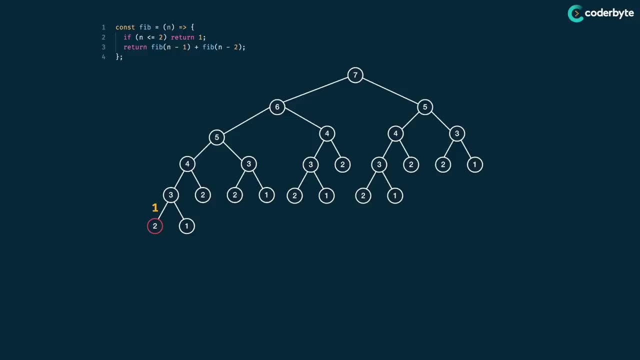 when we say return, that really just means return to your caller right, return to your parent. So this node of two is going to return one to its parent of three. In the same way, this node on this side of one is also a base case. it two will return one, both of those values that are. 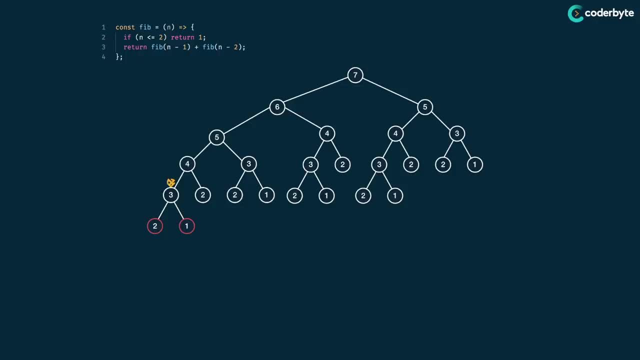 returning. they go back to the parent of three and three is actually going to add those two values up. one plus one is two And this makes a lot of sense because we know we can prove two. we can prove two actually needs, so we are going to be able toiciaq ability. 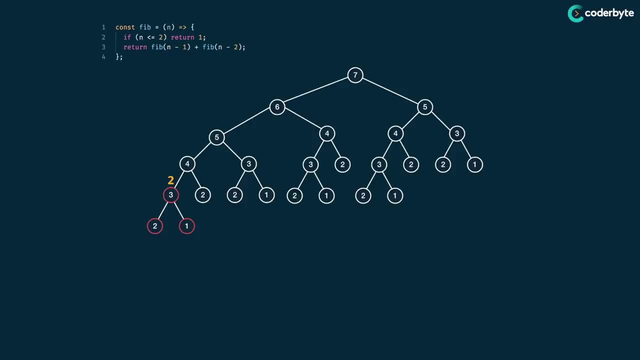 which means that we can have two values, because two is also a base case. At this point, it's going to turn one, which is 2, and 3 adds 2,. we know that the third Fibonacci number is two. So we can continue this process. I'll get this. 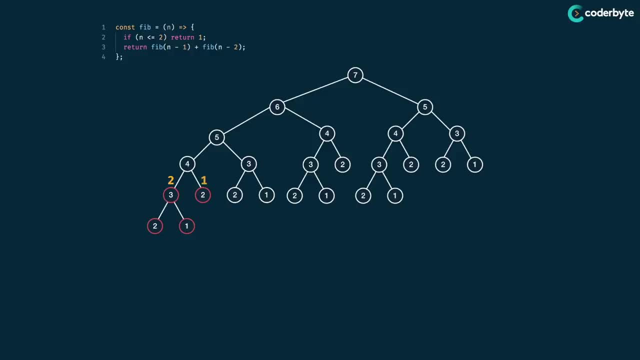 node over here. This is also a base case, So it returns one. And now the parent node of four is going to sum up both of its children values. two plus one is three, And that makes sense in itself because the fourth Fibonacci number is three. So you probably get the picture. Now let's speed. 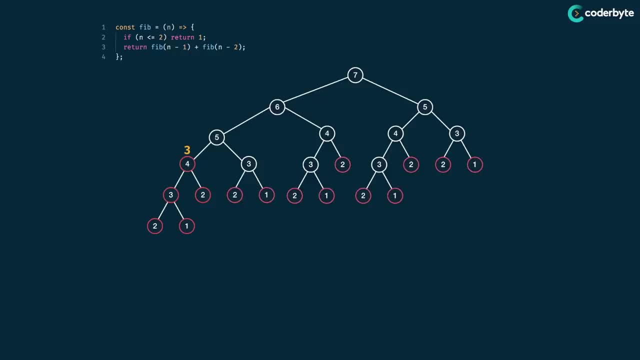 things up For all of these base cases. I know that they're going to return one to their parent And for all parent nodes that have both of their children ready, that is, both of their children returned. they're just going to add up those values And this process just continues all the 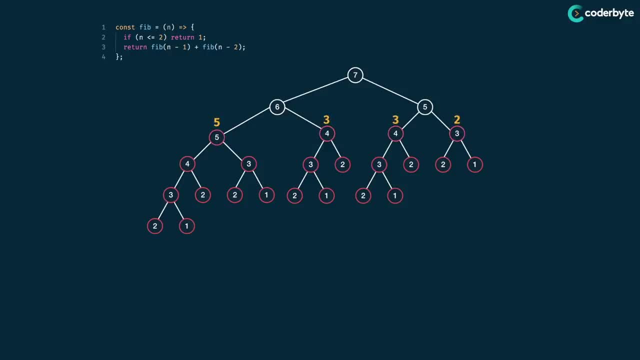 way up the tree right. just adding our left and right children to get the answer that we should return The very top of our tree, at the root of our tree, we get the final result of 13,, which makes a lot of sense because at the start we said that, hey, the seventh Fibonacci number is: 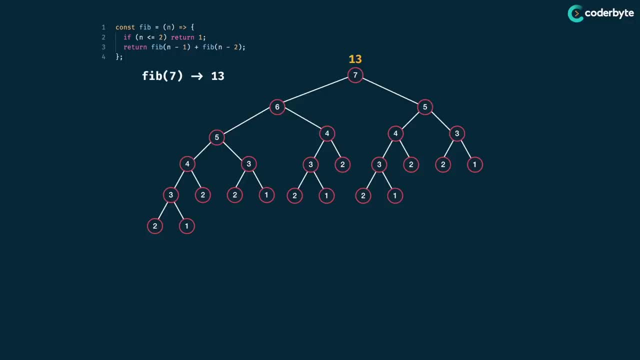 indeed 13.. So, now that we have a robust understanding of how to visualize this fib function, what do we actually know about it? Well, first of all, we know that the first Fibonacci number is going to be two to the n in time complexity, And that is the case. However, 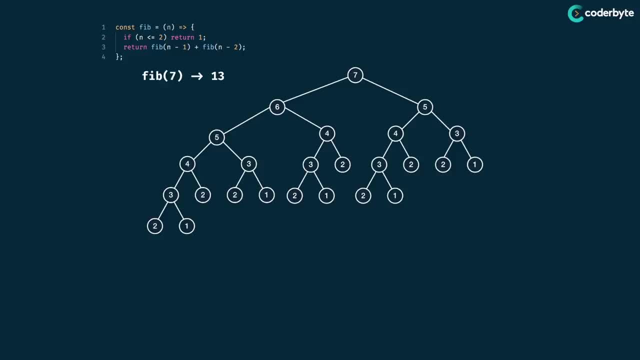 do you really understand the reason why? So hidden in this picture is the reason why Fibonacci, for us, is going to be two to the n in terms of its time complexity. However, something that's kind of unfortunate about this drawing is it's asymmetric, And that's, I think, a big reason why students 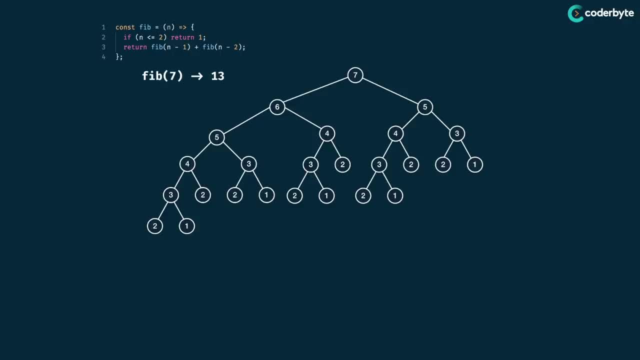 have a really hard time convincing themselves that a function like this has a two to the n power: time complexity. So here's what we'll do. why don't we warm up and kind of go through some basic understanding of time complexity? And I promise we'll answer that Fibonacci question. So let's do. 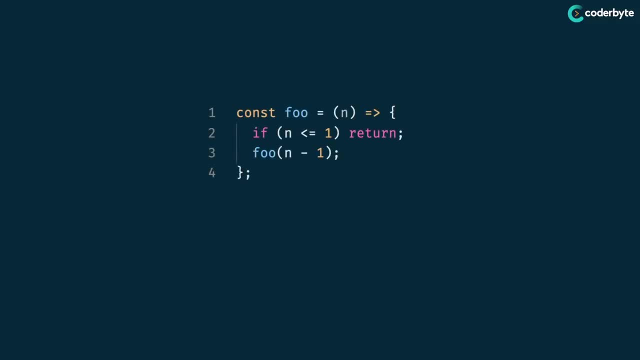 a little warm up. let's say that I gave you this foo function. notice that it's different from our fib function. right, It's similar in that recursive. this function is kind of arbitrary. it actually doesn't calculate or solve any particular problem. So if I wanted to visualize how this foo 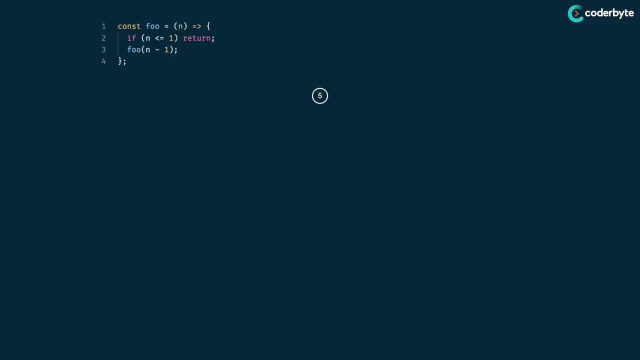 function behaves. let's draw it out. Let's say I initially call it the top level foo of five. I know five is not a base case. So it's going to call upon n minus one, or it's going to call upon four, four calls three, three calls two, two calls one, And then here we've actually bottomed. 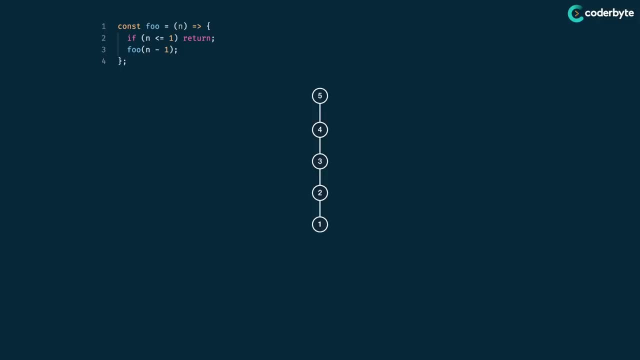 out at a base case. If I look at the number of calls I made, I basically made exactly five function calls, which makes sense because, in terms of our base case, we stop once we hit a number less than or equal to one And in every recursive step we just subtract one from our 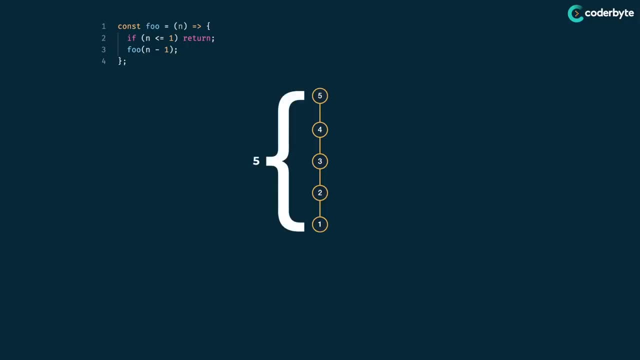 current value of n. So overall I have five calls here. But if I generalize that for any arbitrary function, I know that in the long run I'm going to have about n different function calls recursively And so for that reason the time complexity of this is really just O of n time. 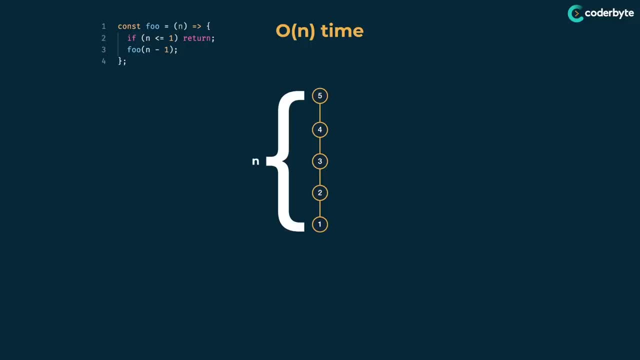 right, I have to evaluate O of n different function calls. And while we're at it, why don't we take a look at the space complexity? Well, you may have heard in the past that when we analyze the space complexity of our recursive functions, we should include 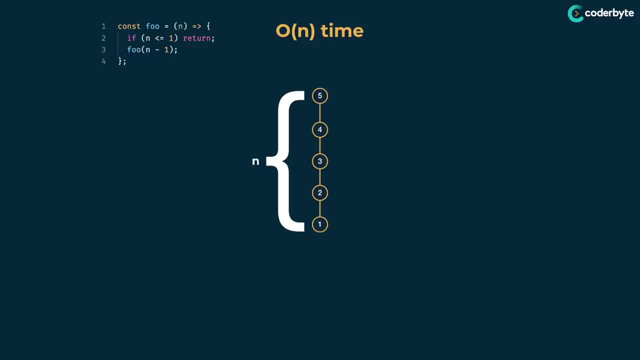 any of the additional stack space that our function calls take up right When we make a recursive call, we add that to the call stack and those must be tracked by our computer And then a different function calls added to the stack Before we hit our base case. 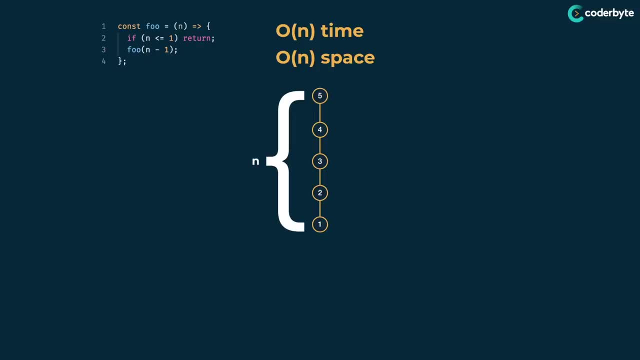 you can see that the space complexity of this code is also O of n space. So overall, we're looking at O of n time and O of n space for this foo function. Pretty straightforward stuff, right? Let's look at another, more involved function. So let's say: I gave you now this: 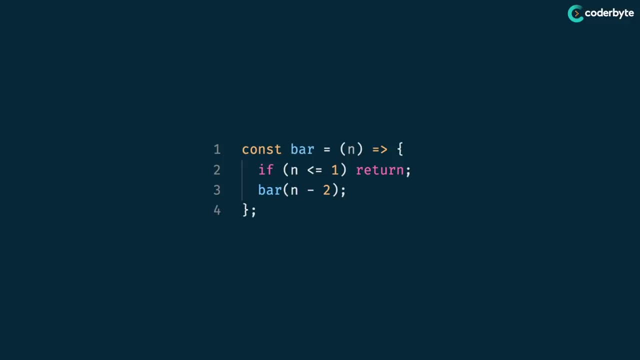 bar function. It's another arbitrary function. It's very, very similar to foo, which you should notice is the only difference is, when we make our recursive call, we do an n minus two instead of an n minus one. So how does that actually change? 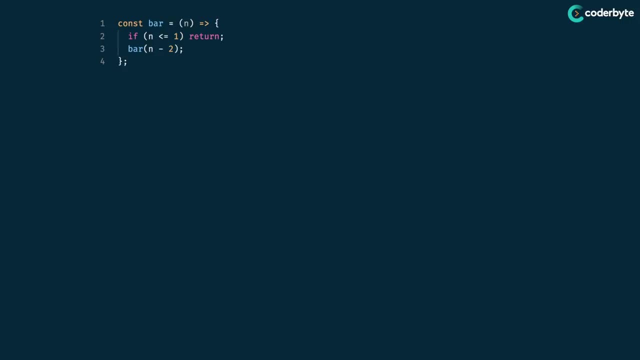 the time complexity of this function. So let's say I wanted to trace through this and I made a top level call to bar of six. I know six is going to call upon four, four is going to call upon two, two calls zero and zero actually hits a base case. 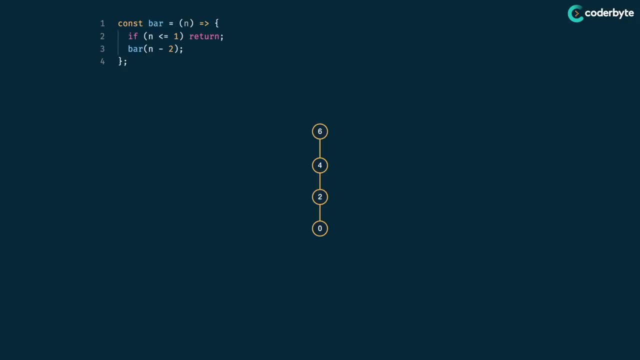 So this is very similar to our last example, except we kind of see that from one call to the next we kind of take a bigger step in time, right, And so in a way we can say that we're moving twice as far upon every recursive call, And this would actually half the number of 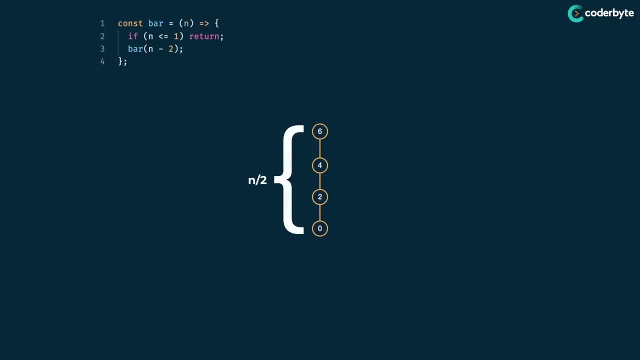 recursive calls we need overall. So I guess we might be tempted to say that the time complexity of this function is very similar to the number of recursive calls we need. overall complexity of this one is n over two time. But a keen observer would note that according to our 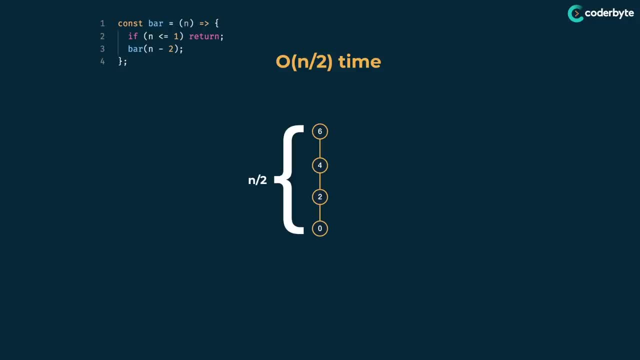 big O. you know, understanding, we can remove any multiplicative constants when we have a time complexity. So n over two is the same as one half times n. So this simplifies nicely. it's just an O of n time complexity. Using the same exact argument, we can also say that the space complexity 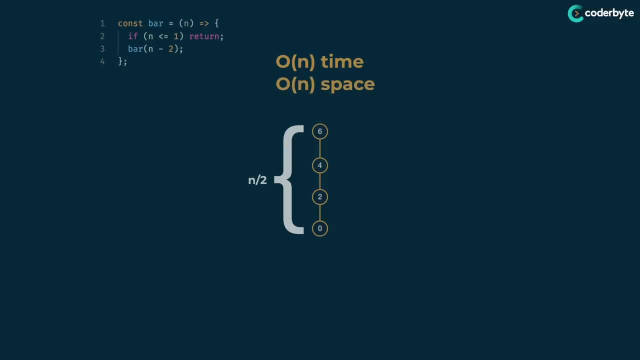 from the stack is also O of n space. Alright, so let's take a lay of the land. I showed you two functions that are very similar. they really only differed in how they made their recursive calls right. one did minus one, the other did minus two. But in the grand scheme of things, 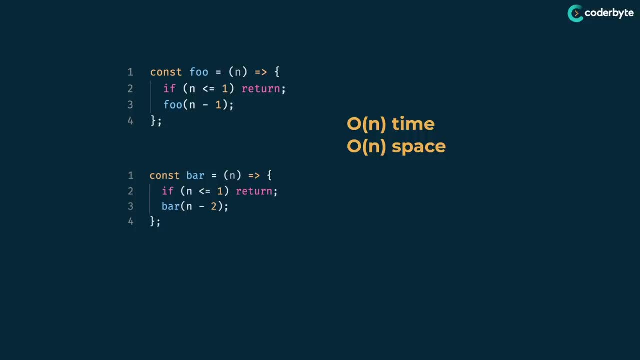 we saw that they had an identical complexity class. right, we have O of n time and O of n space for both of these functions. So after these two examples, you may be able to see the reason I wanted to bring them up right? maybe you're actually ready to make the logical leap and make 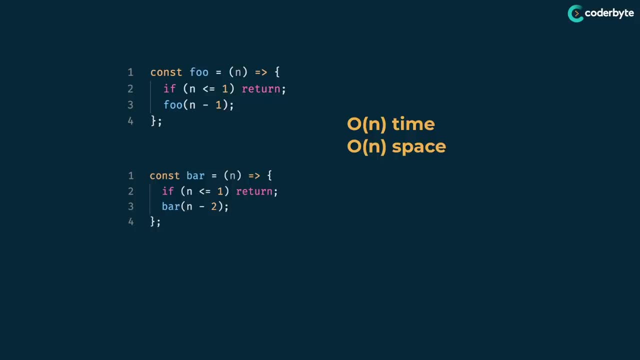 some conclusion about our classic Fibonacci recursive function. That being said, I don't want to skip any steps. I want to be super methodical. I think if we pay the cost of understanding fib right now- and I mean truly and like absolutely understanding fib, it's really 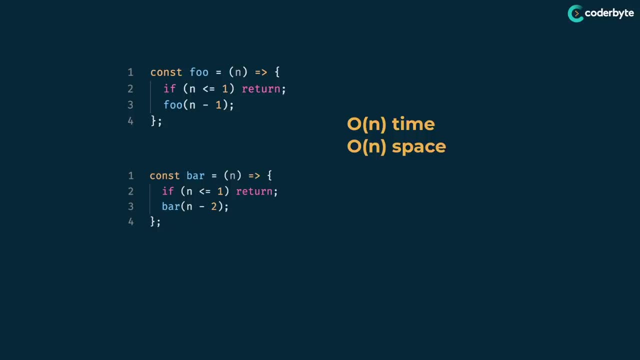 going to pay off later on in the lesson when I slam you with some much harder problems. So let's be nice and methodical over here. Let's take a look at some other functions. Let's say I gave you this dib function, now very particular name, right, Pay it no mind. What do we notice about? 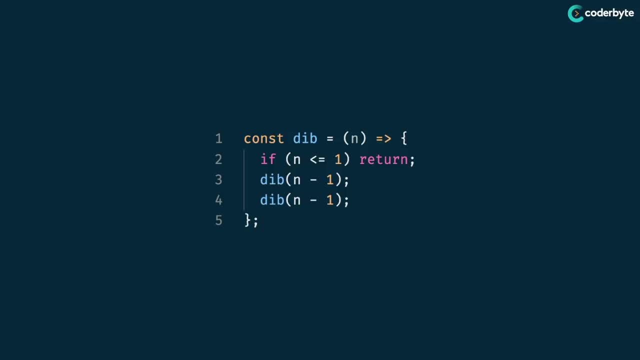 this dib function Well. it has two recursive calls now right inside of every single call And they both do an n minus one. how should we visualize this one? Well, it's kind of similar to, I guess, our initial fib drawing in shape where, if we start with some initial call, let's say five. 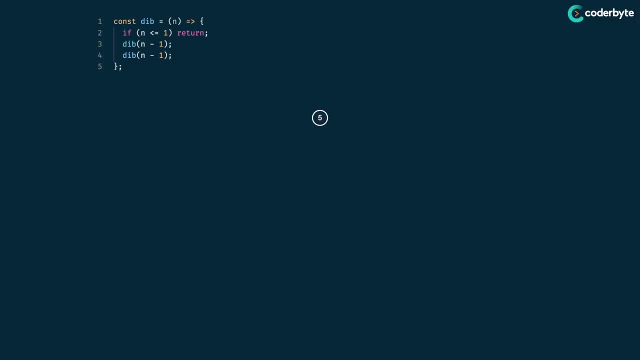 five is going to branch to exactly two children. right is not yet the base case And for this did function. it does a minus one on its left and also it's a right child right. So the next level is just for next levels, just threes. 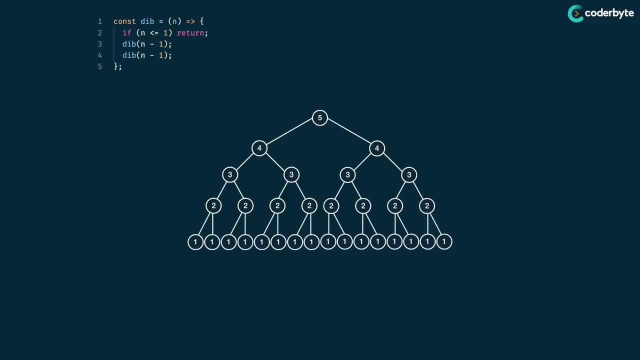 then twos, then just ones, which would actually hit our base case over here. This is a really nice and like beautifully symmetric tree, right? Okay, so this is the visualization for our dib function, But what does it tell us about the time complexity of it? 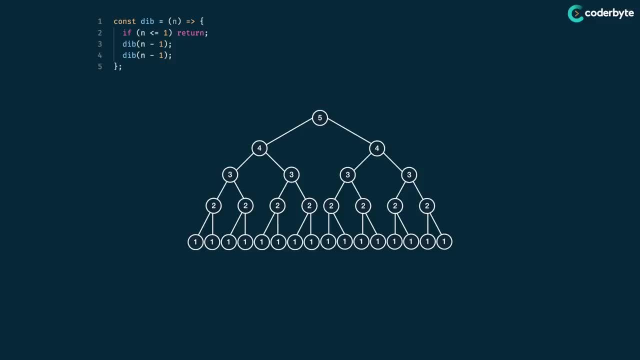 Something you'll hear me say a lot in this lesson is when we tackle a quote, unquote- new problem or new pattern, we're really trying to do is just leverage our past experience, Right. So when I look at this tree structure, I'm trying to notice anything familiar, right Is? 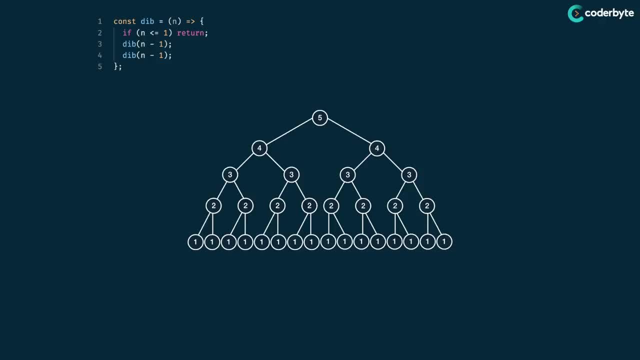 there some strand over here that I can grasp at to really feel comfortable and kind of extend my previous learnings right. Where can I find our base inside of this drawing Boop right here? So if I look at this path I have highlighted in yellow, it's really just the path starting at the 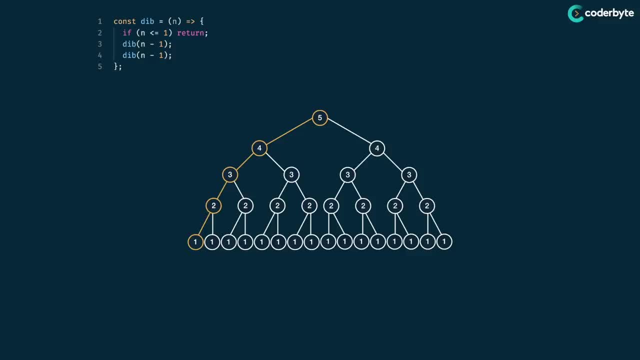 root node going down to some base case. here I just designated the leftmost path And what's really nice about this structure is just referring to the nodes in yellow. it's all linear structure that we saw before. right, If I start at the root, it just goes 54321. And so I know that in. 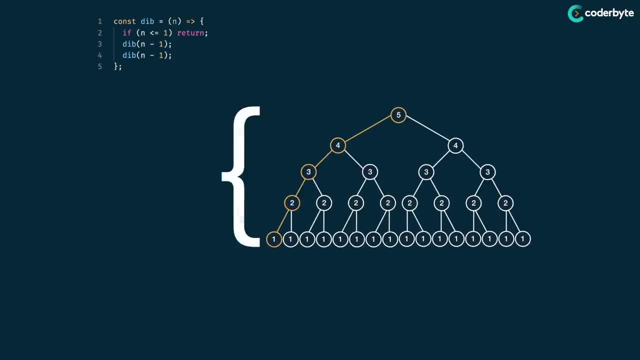 general, based on my initial input of n. like the length of this path, that is, a number of nodes highlighted in yellow, is going to be about n different nodes, If I kind of adapt that language, for, like the tree, I can also say that the height of this tree is n, So the height of a tree is 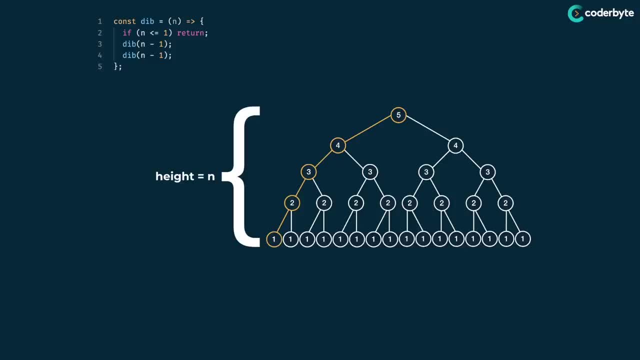 really just the distance from the root node all the way to the farthest leaf. In this case, that just means the distance from our top level, called no five, all the way down to a base Case which is going to be exactly five here. something you may also hear in passing is: we can. 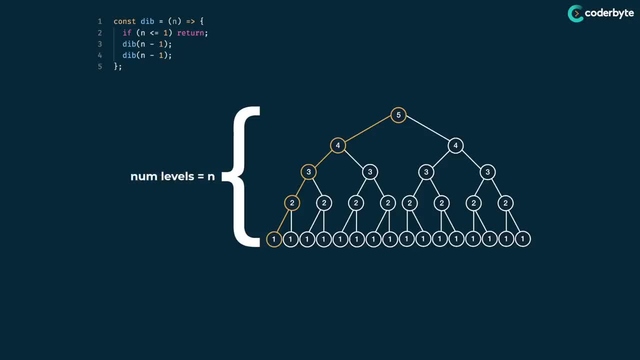 say that the number of levels in this tree is also n. this term is pretty straightforward, right When we say the number of levels. a level is just a collection of nodes that are the same distance away from the root. So for example, here in yellow I have highlighted level zero. 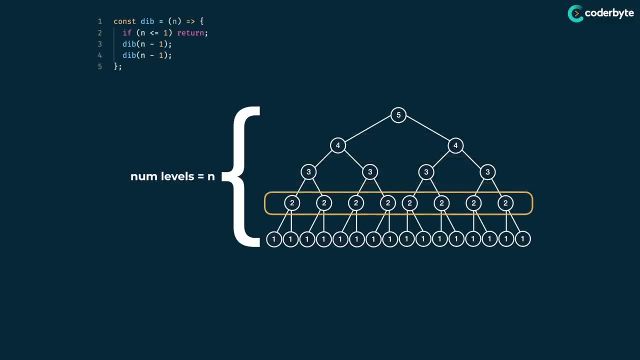 this is level one, this is level two, this is level three and so on. But if I rewind things a bit, I look at the very, very top level. there's one node here. on the next level, there's two. 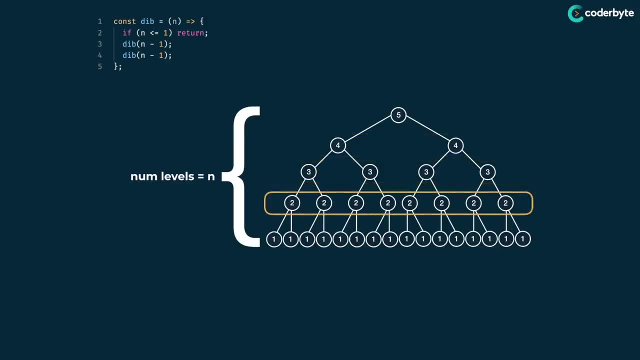 nodes On the next level there's four nodes, then eight nodes, then 16 nodes. see the pattern. So let's try to generalize that. So I know, no matter what, whenever we call some top level argument for dib, we know that we're going to have one node at the top level. But to get the number 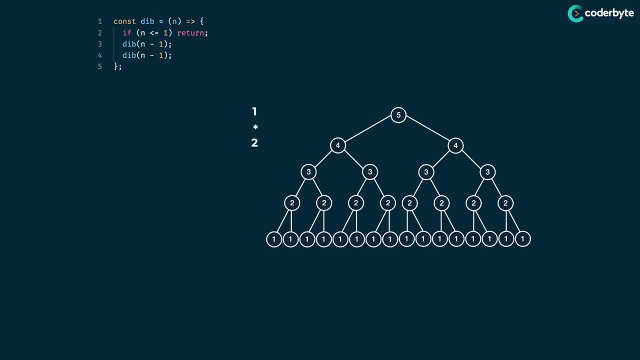 of nodes on the next level, I'll just multiply that by two, And the level after that would also multiply by two, and multiply two again for the levels after that, And I do this a total of n different times, right, Because I know that the 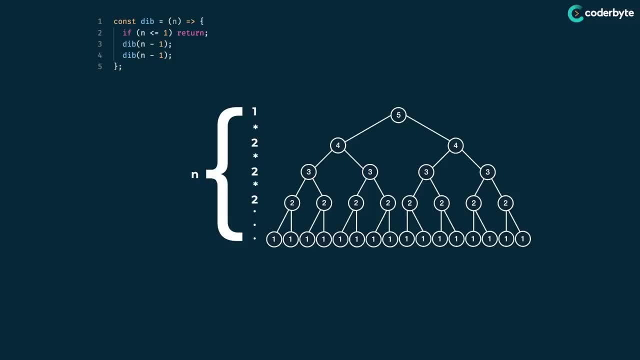 height of the tree or the number of levels in this tree is exactly n, And so what conclusion can we make over here? we're basically saying that to get the total number of nodes or the total number of calls a recursive function would make you would just take the number two and multiply. 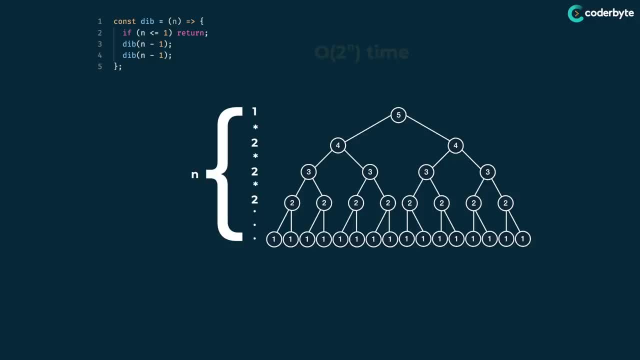 it by itself about n times over, And that is really the definition of an exponent right. This is the same as two to the nth power, And so we can say that this tree structure, this recursive function, has a two to the n time complexity, Awesome. So we identified: 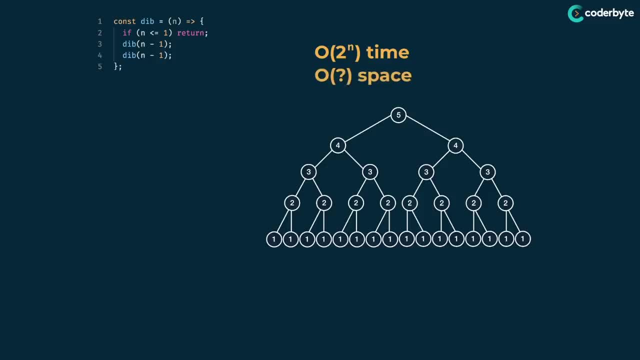 this div function is having a two to the n time complexity. But what do we know about the space complexity over here? I think a common mistake I've seen people make is kind of automatically assume that the space complexity of a recursive function will be the same as the time complexity. 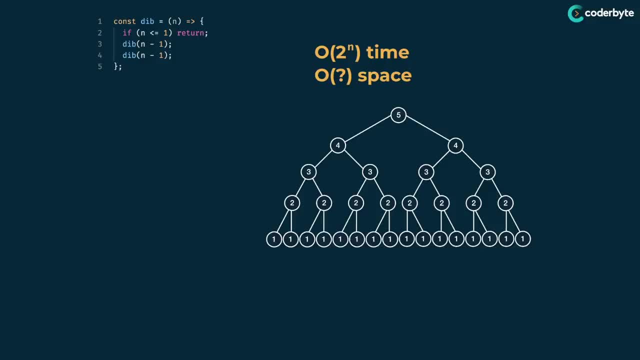 And that might be a reasonable trap to fall into, because we know that in the long run we're gonna have to evaluate two to the n function calls, And so I guess that means we have to put two to the n function calls on the stack. But there's actually some nuance to this. 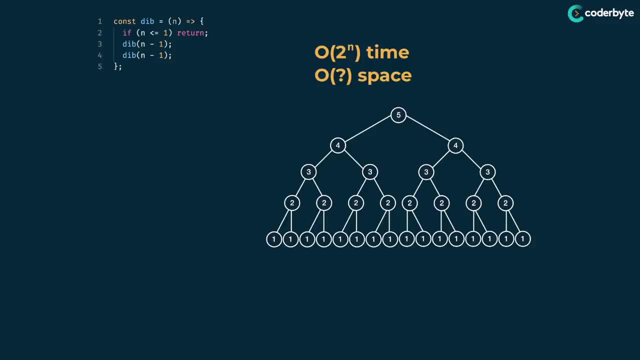 the type complexity of this is not the same as its space complexity. So let's jump in. We made our top level call to div of five. we know that that is added to the stack. in the same way, five calls four, So it's added to the stack. we add a stack frame for every call that we make. 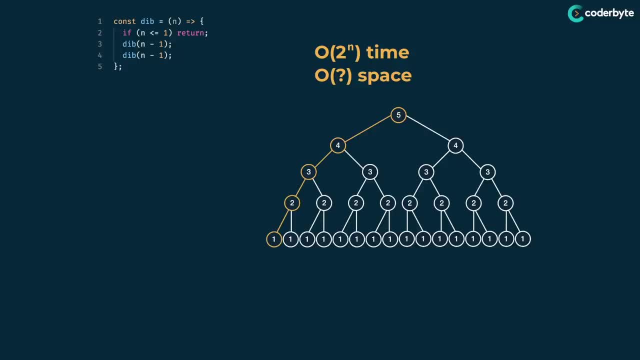 down until just the base case, right. So at this point I reached a scenario where I have a base case and I'd have about five stack frames on my call stack And the important insight is when we actually hit this base case that I've highlighted the left one over here- it actually will return. 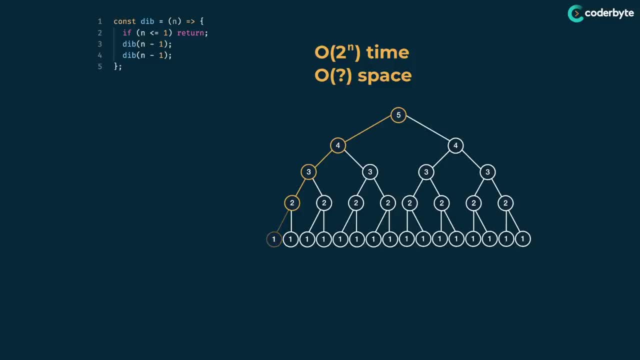 when something returns. when a function returns, its stack frame is actually removed or popped from the stack, And at this point, only after the function returns, its stack frame is actually removed or popped from the stack, And at this point, only after the function returns its stack. 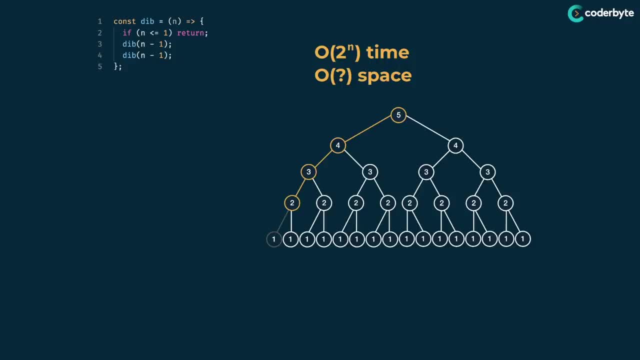 frame is actually removed or popped from the stack, And at this point, only after I have returned from that left one, would I actually add the right one to the stack to be explored. And this process continues. Notice that any point in time, the most number of stack frames that we use up. 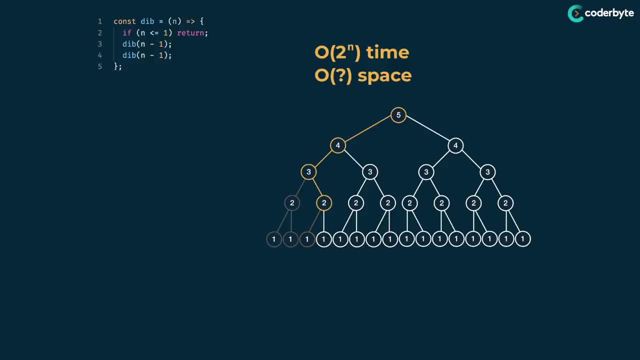 it's exactly five, right? it's not as if we throw all of these function calls on the stack at once Because we have such a nice tree visual. we know that the number of stack frames that we're ever going to use is really just the height of the tree, right? So the height of the trees. 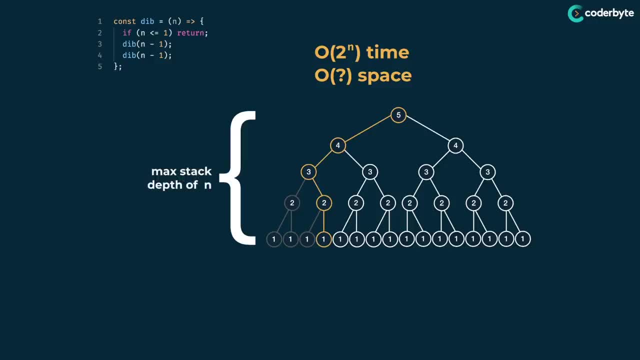 and, like we said before, it means our maximal stack depth is also n. So we have n space complexity coming from the call stack. So, overall for a dip function, we're looking at two to the n time complexity, but only in n space complexity. Alright, so let's look. 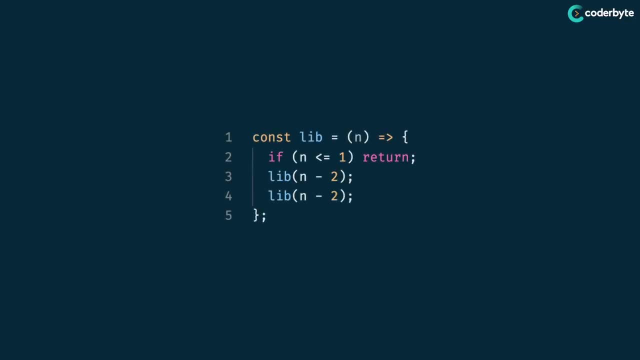 at one more function, Say. I gave you this very similar lib function. Notice that in its recursive calls it does an n minus two. So by now you should be able to visualize what a structure like this would look like. Say we initially called lib with a value of eight, what would? 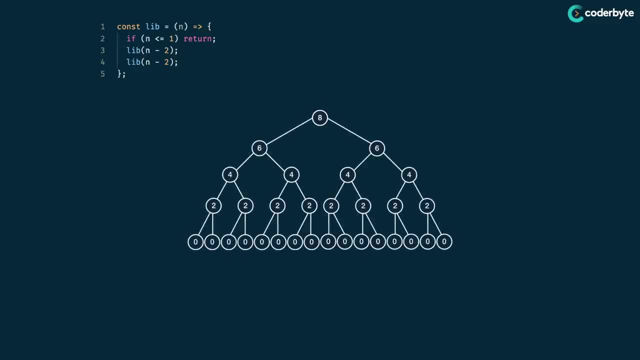 the full tree look like. Well, it would just look like this. Notice that it's still a tree right where every node branches to two children, But this time we go by twos right. So if I look for some familiar ground here, I noticed that from one node to the next, I do a minus two And this: 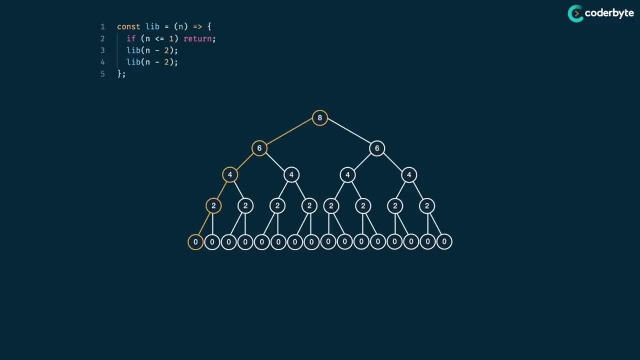 occurs all the way down to a base case. So we already know that. hey, we can identify this tree as having a height of about n over two. So I guess that means that the time complexity is going to be two to the n over two power, right, Because from one level of the tree to the next we double the 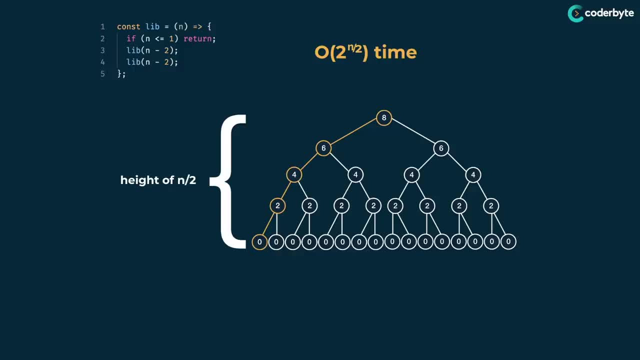 number of nodes. So that's that two times two times two. repeating pattern for the number of levels and levels is n over two, right? However, we can actually simplify this time complexity. you can take that n over two in the exponent and simplify that to just an n. So overall we're looking at a. 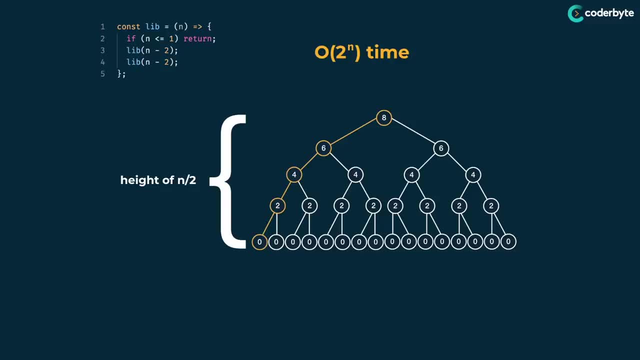 two to the n time complexity And using our same arguments from last time, we know that the space complexity for this from the stack is also going to be n over two, which simplifies nicely to n space complexity. So we see that overall for our lib function we're looking at a two to the n time. 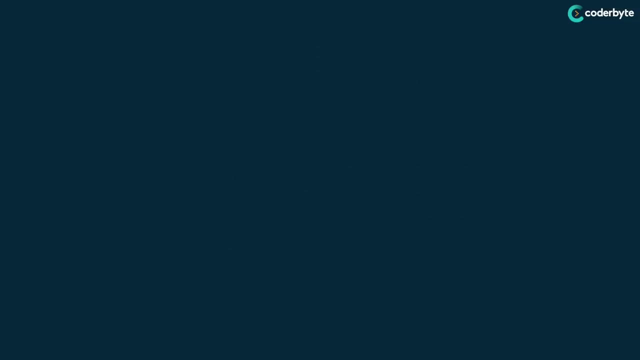 but n space complexity Alright. so now it's time to look at the big picture. We looked at two toy functions of dib and lib And we saw that they only differed in how they made their recursive calls right. did did a minus one and lib did a minus two. And we saw that, despite their differences, 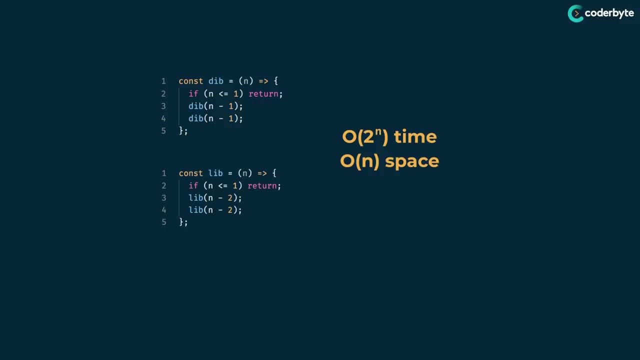 both functions had an exponential two to the n time complexity and a linear n space complexity. That being said, where does our original Fibonacci function fit in this picture? Well, you can imagine that kind of falls right in between. we know that for our fib function. 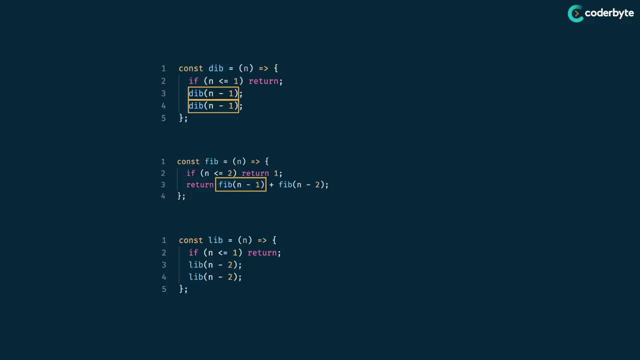 it has two recursive calls for the first recursive column makes it does n minus one, like dib did, But its second recursive call this n minus two, like lib. So in a sense it's kind of like smack in the middle, right, If you. let me abuse the notation a little bit and just talking. 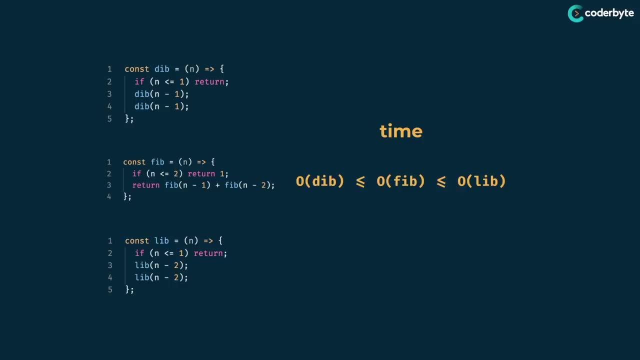 about the time complexity. we can kind of say that the complexity of fib is somewhere between dib and lib. But we've already plugged in some values, right? you know that. hey, the lower bound, that is dib, has two to the n, and the upper bound, that is lib, has two to the n as well. So that means 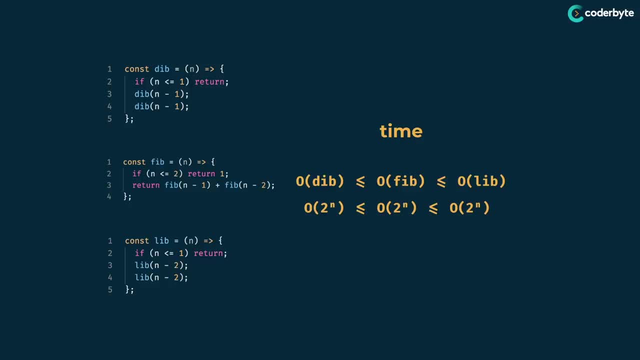 that our fib function must have exactly a two to the n time complexity as well, right? All three of these functions have an exponential two to the n time complexity. So that means that our fib function must have exactly a two to the n time complexity as well, right? All three of these functions have an 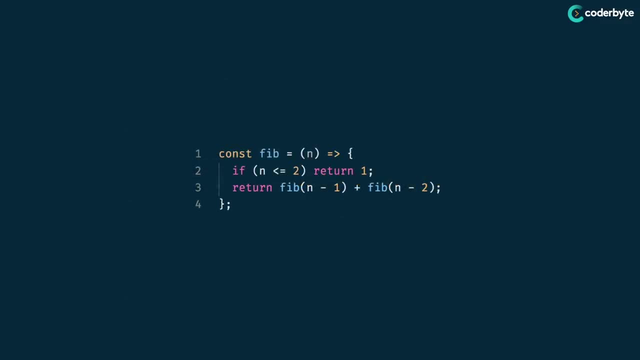 exponential time complexity- Awesome. So that was a really complete analysis of why we have this fib function. It's evident that it has a two to the n time complexity and an n space complexity. Right now, the bottleneck that we're experiencing is, of course, the time complexity right. 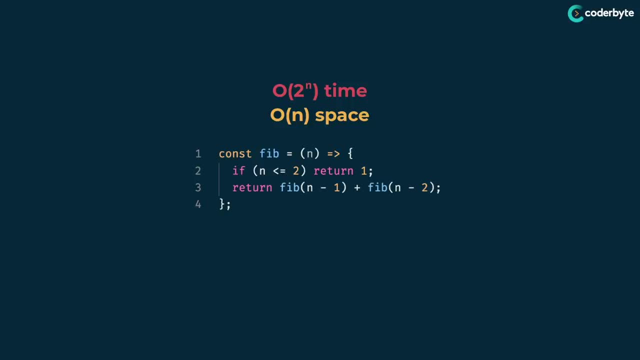 two to the n overall is not a desirable complexity, But we really have a nice feel for what this really implies. So let's take a look at this two to the n. So what's the implication of this? Well, you could kind of imagine that. hey, if I asked for the 50th Fibonacci number. 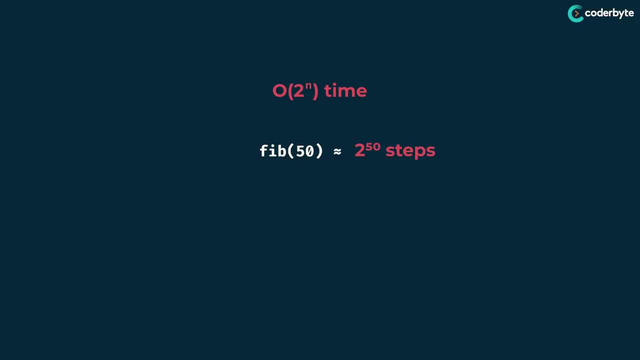 that would take, you know, roughly two to the 50th power number of steps, And so if you punch this exponent into a calculator, you're going to end up with a result like this: This is roughly a 16 digit number, So you should have a vibe, for you know this being a very, very, very large. 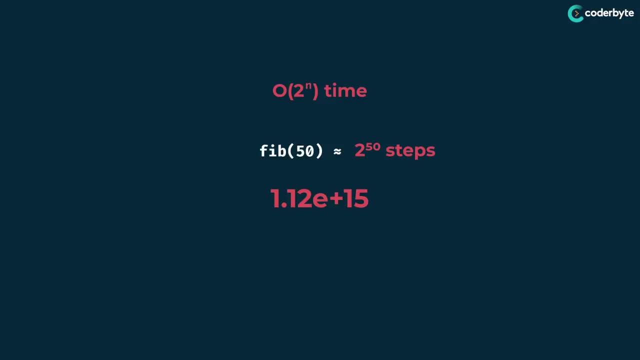 quantity, But I think that you know to really understand the gravity of what we're really saying here. if we expand this number, that quantity is exactly this. That's over one quadrillion, or 125 trillion, which is a lot of times more than a quadrillion. 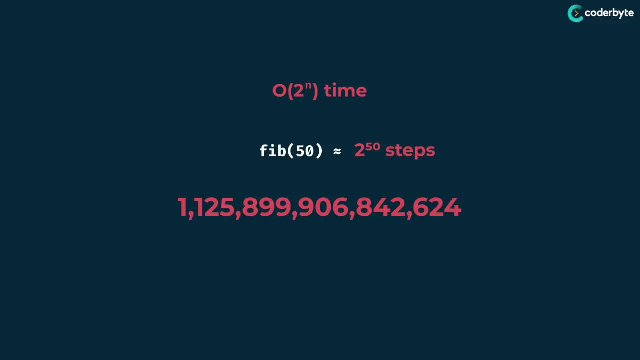 Which is really really interesting, right, Because we just asked our Fibonacci function for just, you know, something relatively modest, right, the 50th Fibonacci number, and it's going to take quite literally a quadrillion steps to do that. And, of course, 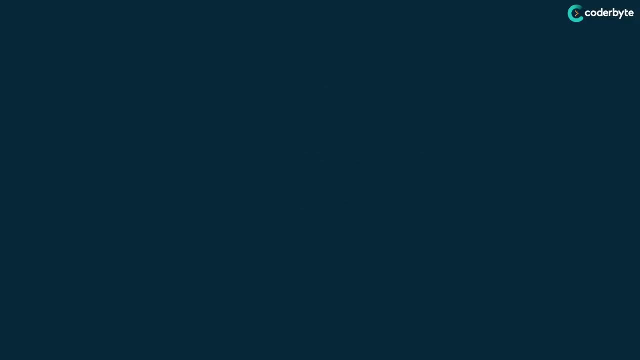 we can probably do better, So let's work on making this faster. So if I recognize that the bottleneck for this fib function is the tab complexity, I know that that comes from the number of recursive calls that I make. So what I want to do is look for any patterns that I see in the 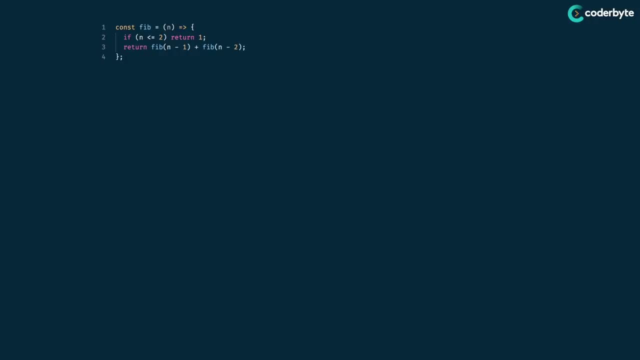 recursive nature of this problem. Let's see a quick snapshot of what the recursion for fib of seven would look like. We know that it looks like this tree, just like we saw before. So take a moment, look at this tree. do you notice any interesting patterns within it? Well, one thing. 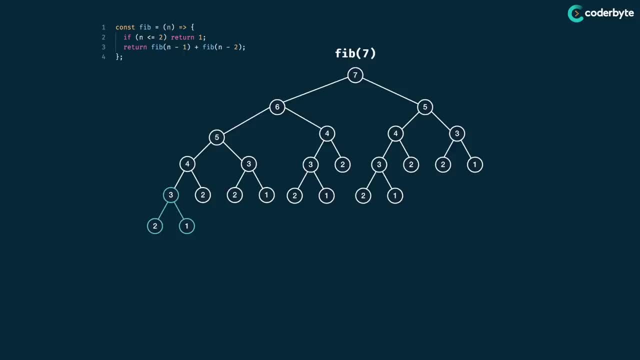 that I notice is I can see this subtree rooted at three there. I have two on the left and one on the right And if I look at that subtree I can actually see it in many different places. in this tree right, The subtree rooted at three appears in a bunch of different places. 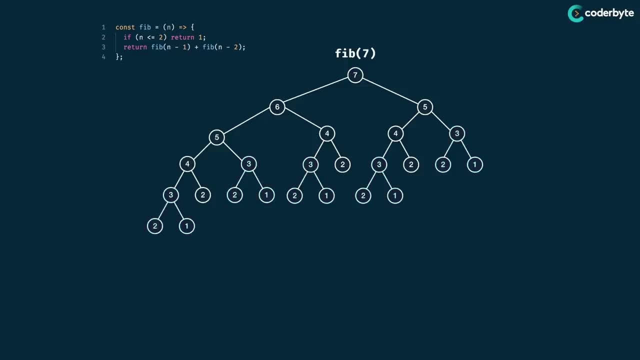 it's very duplicate. In a similar way I can look at other sub trees. let's say I root myself at four. I can see that duplicate for subtree all over the place And it's even carries over for larger values of n, like fib of five. So I see that this tree has a lot of duplicate sub trees right And 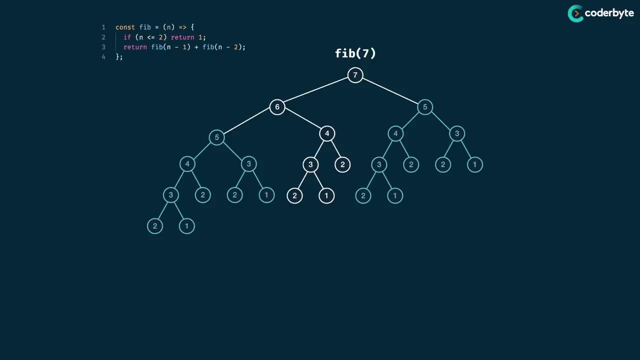 I want to now draw the connection between you know this diagram and what happens in my code. I know that if I root myself at any of these sub trees of five, I know that each sub tree is trying to answer the question: hey, what's the fifth Fibonacci number? I know that the fifth Fibonacci 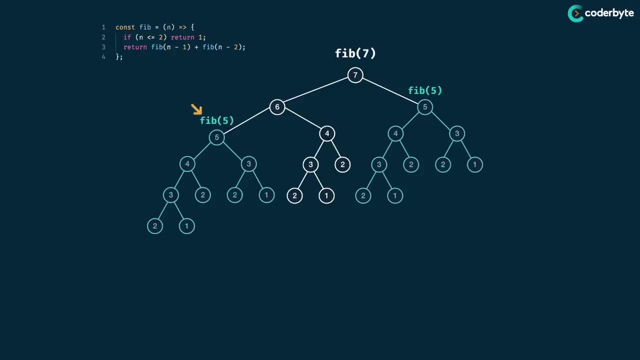 number never changes, right? If I calculate it once on the left hand side, then the answer I should get back on the right hand side- is that the fifth Fibonacci number never changes. right hand side shouldn't differ at all, And so what I want to do is possibly reuse these calculations. 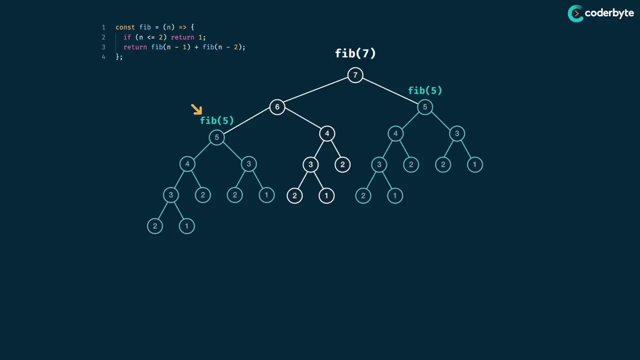 right If I calculate the fifth Fibonacci number over here. that should just store that because later on it might be useful we'll need to recalculate it over here. that would basically get rid of a lot of the tree. I wouldn't have to travel down this entire recursive tree rooted at 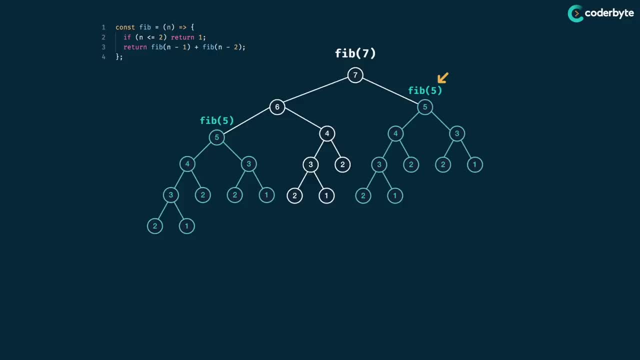 five: This pattern of overlapping sub problems is known as dynamic programming, And so, for us, dynamic program is going to be any instance where we have some larger problem- in this case Fibonacci- and we can decompose it into smaller instances of the same problem. But we also have an 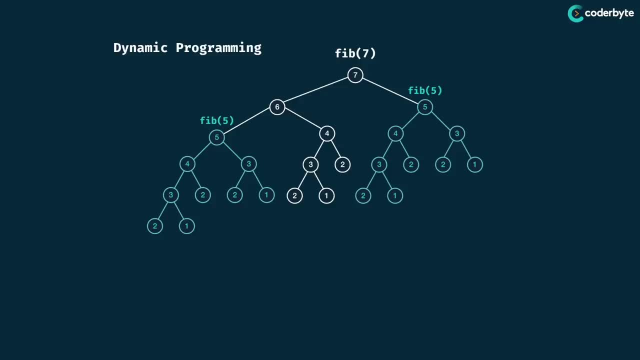 overlapping structure. So for us, right now, I see that I have to calculate, let's say, Fib of five twice over to calculate the larger Fib of seven. solution- And something we're going to be doing a lot in this lesson- is really trying to visualize problems in terms of, like their recursive nature. 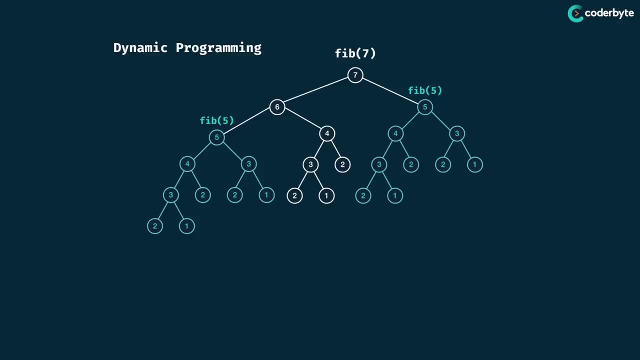 So we're going to be drawing a lot of trees And what I'm always going to do is try to really recognize, hey, what pattern in this tree is duplicate? right, If I do some duplicate work, if I do some duplicate drawing, that I know I can optimize it out later on. But that being said, 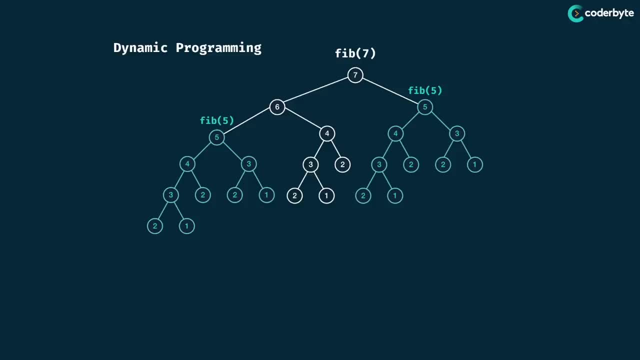 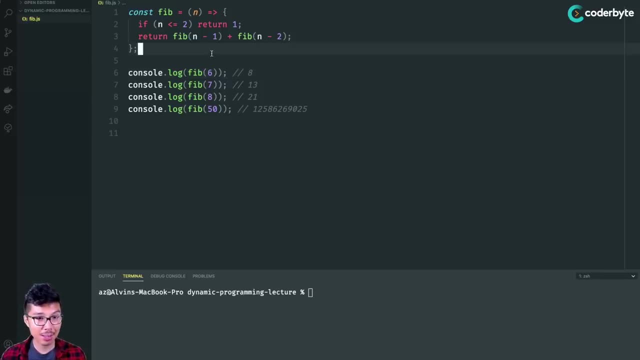 let's go ahead and get to the punchline on this fib function and work on optimizing this solution All right. now that we discussed a plan, I think we're ready to actually implement some code that will actually carry that plan out. Here I have our classic Fibonacci implementation. This was the one 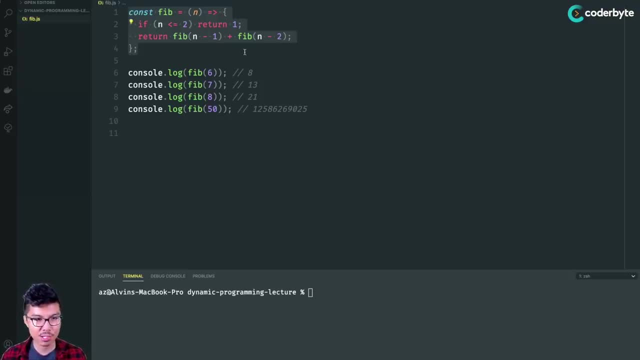 that we ran earlier And it's definitely too slow. right has an exponential time complexity. So now that overall what I want to do is kind of capture a duplicate sub problems, I want to store any problems that I get. That way, if I have to recalculate those sub problems later on, I can. 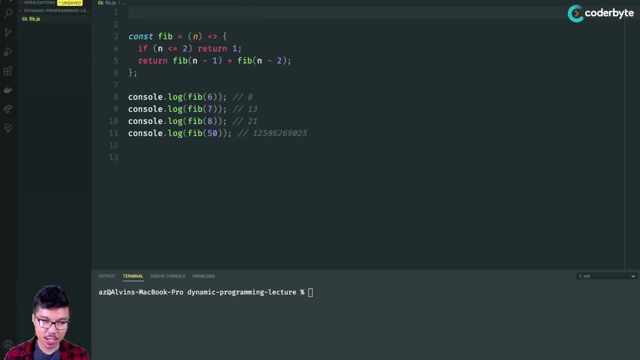 just use my stored data, And so the trick here- it's a very common programming pattern. we're going to implement some memoization. Memoization is actually one of the overarching strategies we can use to solve any dynamic programming problems, And so just looking at the name, like why is it? 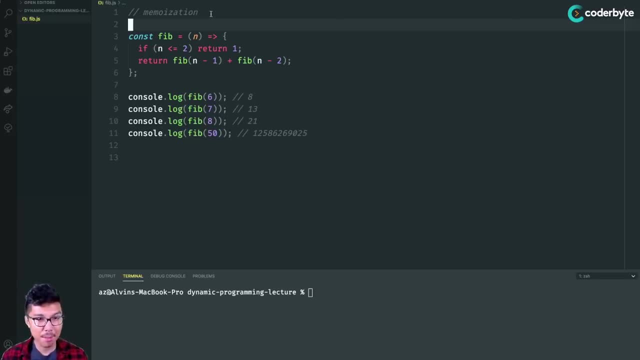 called memoization. Well, just refers to like memo, right? So if I have like a memo and, let's say, like real life, it's really just like a reminder for myself. So, using memoization, I'm looking to do is store some duplicate sub problems. 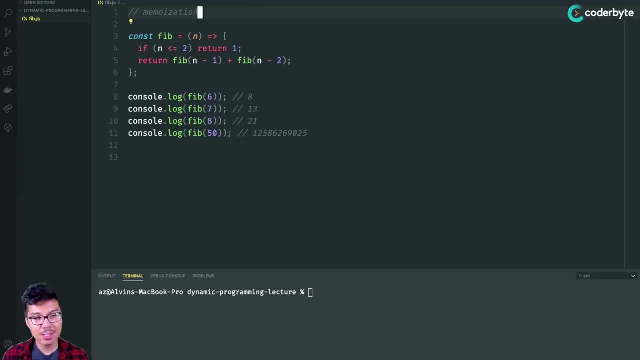 That way I can just get those results later on. I think a really neat way to implement memoization in JavaScript as well as many languages, is to use some sort of a fast access data structure, usually be like your hash map equivalent in the programming language of your choice. For us, 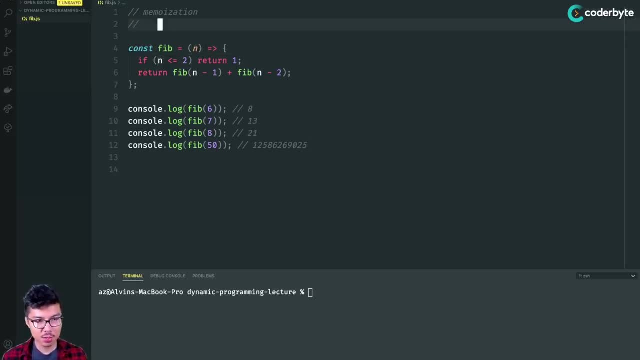 that'll be a JavaScript object, And so our plan is to use some JavaScript object. And so what do I want the keys to be? So the keys in the object are going to be the argument to our function, right, And then the value will be. 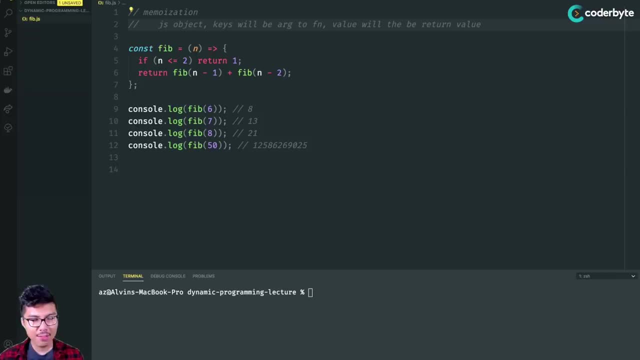 the return value. That way I have a nice mapping for a argument to the function- that is, a function call, as well as its return value, right? And so what I can do for my existing fib function is I kind of just bake in some optional arguments. So my favorite strategies to do this can assign a 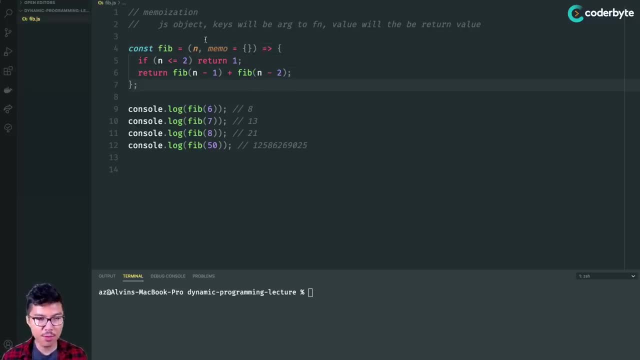 memo to be an empty object. So if you're unfamiliar with this syntax in JavaScript, it's pretty useful. What I'm saying is, if I were to call our fib function and not pass in a second argument, by default it's going to be the return value, And so what I'm going to do is I'm going to. 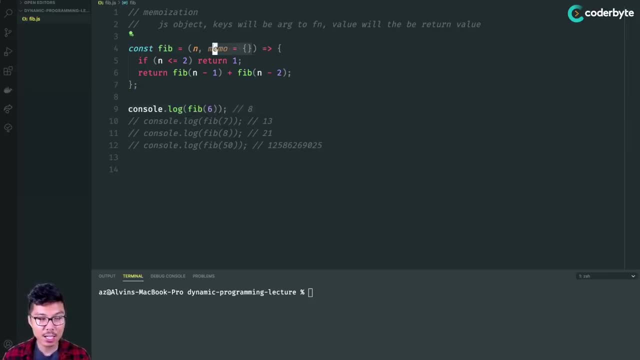 default, it will create this memo as containing a new JavaScript object. that is empty, of course, right, So it's going to be useful. that way, whoever is actually testing my code doesn't have to deal with setting up any memo object, And so we'll prefer this strategy over here. 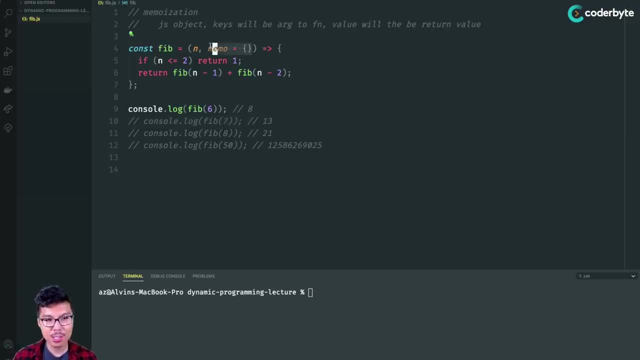 And what I want to do is treat it as if that. hey, this memo is going to store n as the key, and values are going to be just the return values for this function. So you're going to see us doing a lot in this. lesson is at the start. we're going to first check. 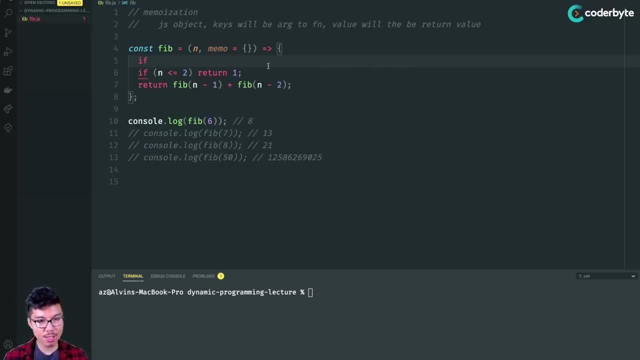 okay, is there an existing argument in our memo? So let's say that we're somewhere in the middle of our recursion. the first thing I should do is kind of add an additional base case and say, hey, is my current argument n inside of the memo? And if it is, then I can just get the stored value. 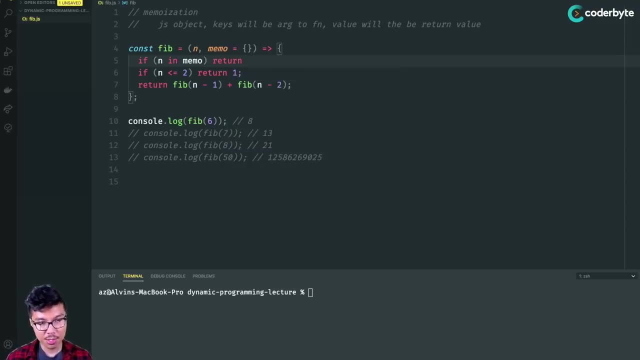 from that memo And I'm done. So I'm gonna do an early return here. I'm going to return the value that corresponds to that memos key, right? I'm just using the original argument n as a key in my memo And this condition is really just some classic JavaScript syntax. I'm just checking if 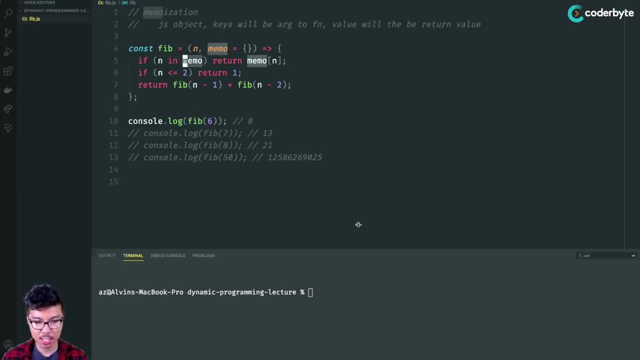 key is inside of a JavaScript object. So really quick, maybe just to warm us up. maybe you haven't seen that syntax before. So let's say I had some object and had some properties inside, maybe had a name of Alvin- that's me- then it had a favorite color of like. 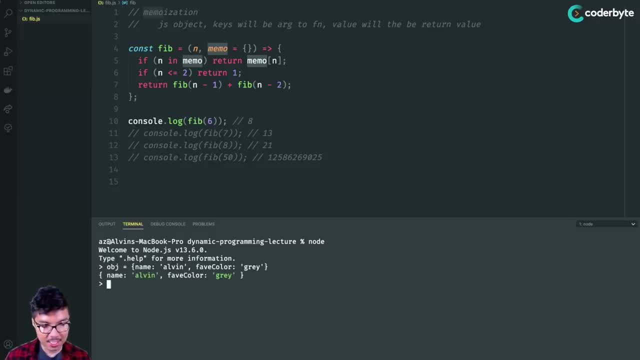 gray, And what I can do is check for an existence of a key in that object. So JavaScript, keys are mostly strings, right? So I can check. hey, his name in the object, that's true. the fav color in the object- make sure I spell right, that is also true. I can check for a key. 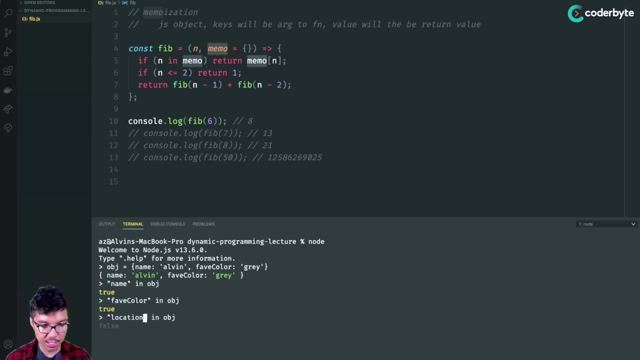 that's not there, like I don't know, is location in the object. that is false, And so here I'm just using that same pattern, but for n right, which is going to be a number. technically it'd be. 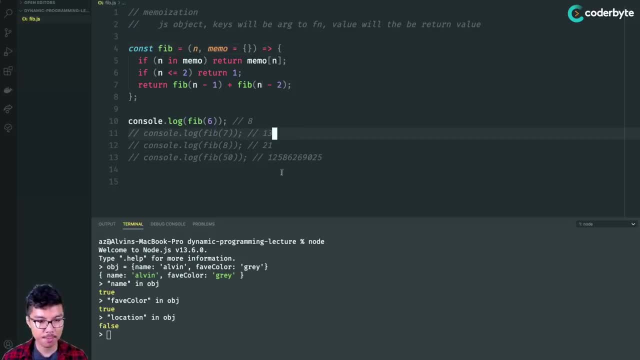 converted into a string key, which would still totally work here. Awesome, So I have my memo fetching logic right. I check, hey, is this argument in the memo? But if it's not, I'm gonna have to actually manually do the calculation, which is okay, because I know I need to do a. 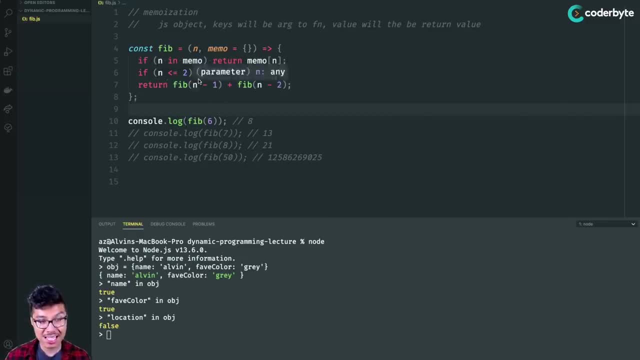 subtree, at least once. So what I'll do is I'm going to take the exact return value, right. So this is my return value In the original brute force. what I want to do is actually just store that entire result inside of my memo, And the key is, of course, n right, the key you use. 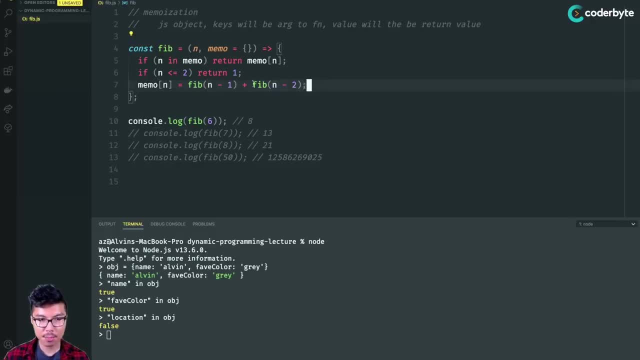 to access is always just what your argument is, And I want to complete the original return So you can just go ahead and return what I just put in that memo. So I'm not going to go ahead and return what I just put in that memo. So I'm not going to. 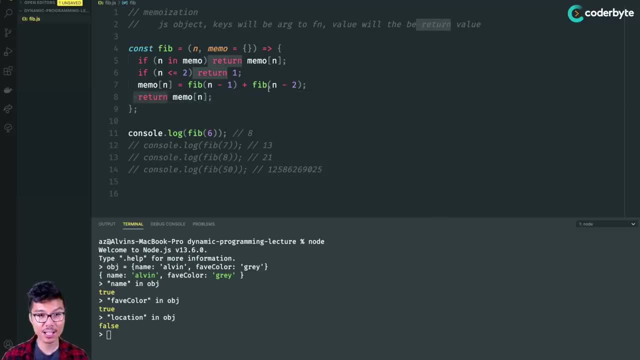 really changing any return values, where I'm returning exactly the expression that I returned before, But now I'm actually also saving that value inside of the memo object And what I want to do is make sure that all of these recursive function calls are accessing the same memo. 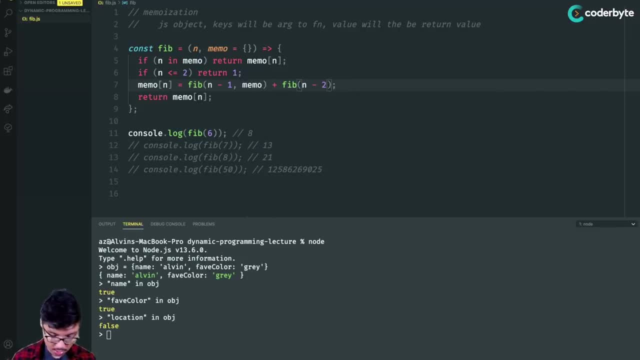 So what I'll do is I'll pass in that object to both of these calls. A really important pattern here is: I know that I only receive a new top level memo object whenever I make a top level call. that's a fib right, Because I'm not passing in a. 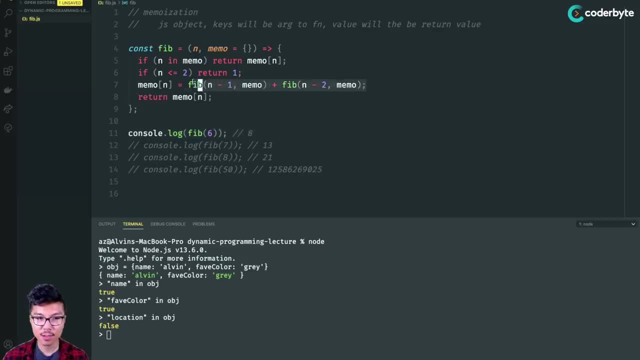 second argument over here. However, if I look at my recursive calls, I do pass in explicit second arguments And so they're actually going to receive the same memo object And it would be like pass by reference right, Because when you pass a JavaScript object to a function, 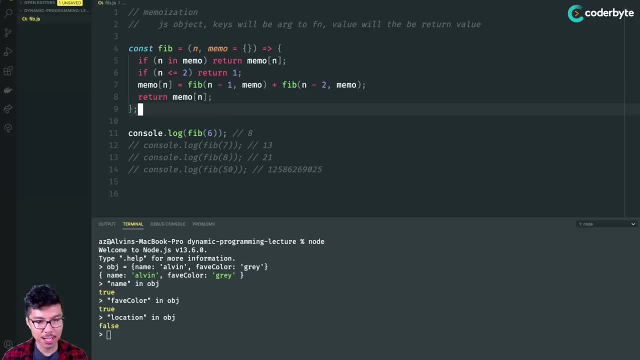 you actually receive kind of that exact object, right, You don't receive a copy of it, which is really neat. So basically I'm giving my function calls a way to sort of communicate to each other. they all have some sort of global information to reference across other recursive trees. 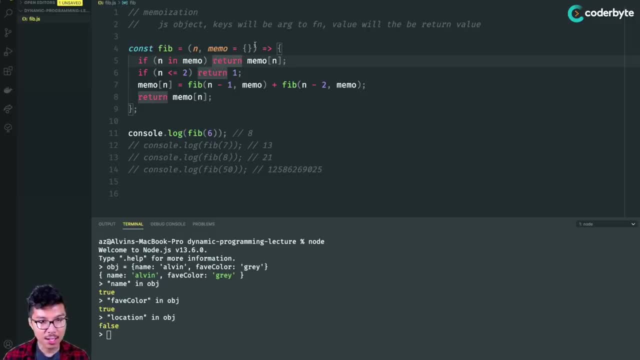 So this code is looking good Again. I just want to emphasize: I only added a new argument over here. I added a new base case on line five, then I added my memo storing logic on line seven, But I didn't change any of the functional logic here. Let's go ahead and run these test cases And we'll. 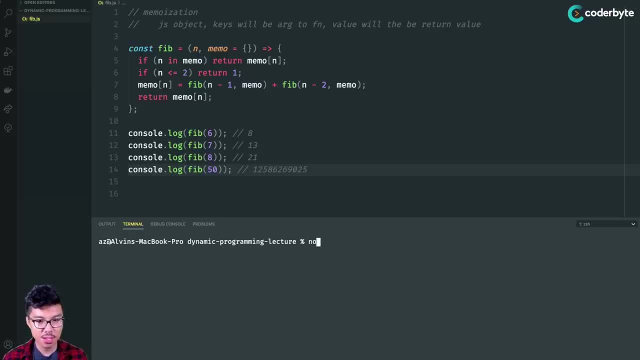 see how our code is doing now. So, moment of truth, I'm going to run this file And notice how blazing fast our program was. I still get the results of 813 and 21. And the 50th Fibonacci number is indeed. 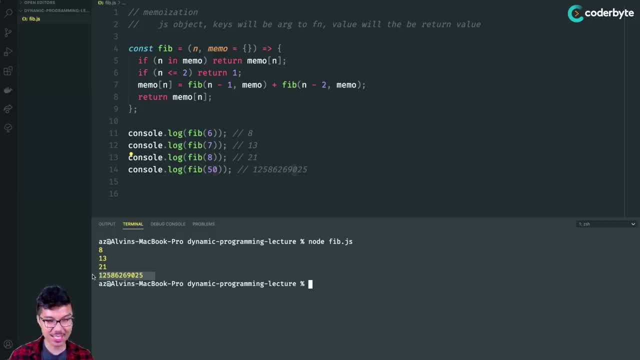 this very large number And it basically executed almost instantly. So let's go ahead and head back to the drawing board and really understand. you know what happens when we execute this sort of code. Alright, so it looks like we implemented the improved version of Fibonacci by memorizing it. 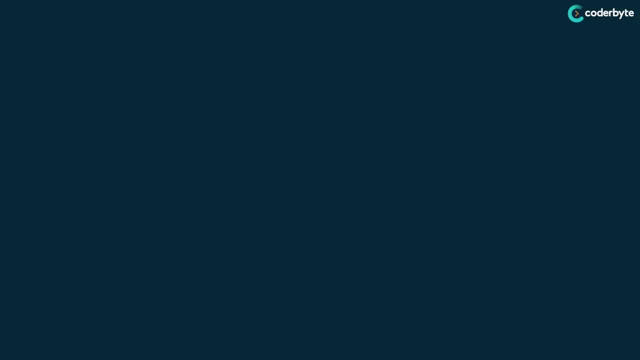 And it's clear, by running the program, that we definitely had an impact on the time complexity. However, I really want us to understand, you know, how the structure of the recursion tree changes once we implemented this memoized version of the code. So let's say I want to step through an 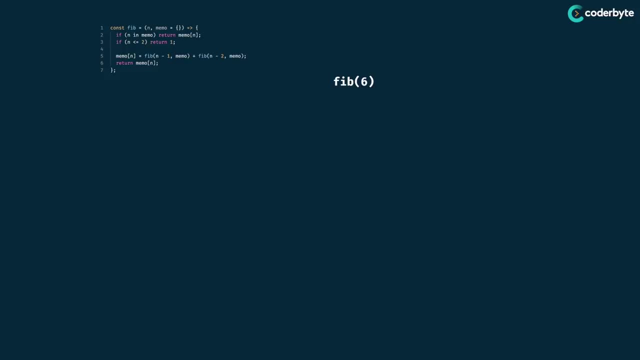 Fibonacci, And let's say I pass in a number six. So really what I'm looking for here is to get back eight, because the sixth number of the Fibonacci sequence is indeed eight. So we know that we're going to have a tree that looks like this right, This is a tree that would really be the full. 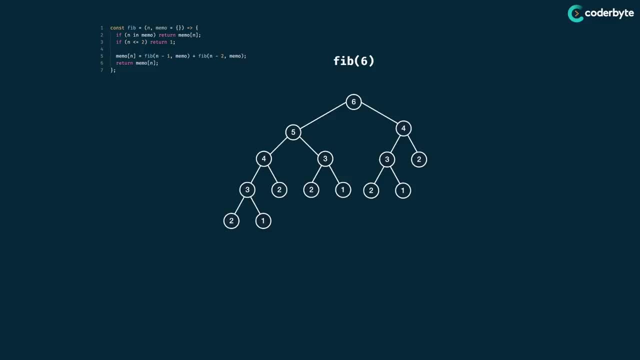 recursive nature. So this is how the tree would look like if I did not optimize it. And what impact do we have by actually adding this memo object right? so let's start tracing through this. I know that when I call them of six at the top level, important thing to know is I'm not going to pass in some memo object. So by default, I'm going to pass in some memo object. So by default, I'm going to pass in some memo object. So by default, I'm going to pass in some memo object. So 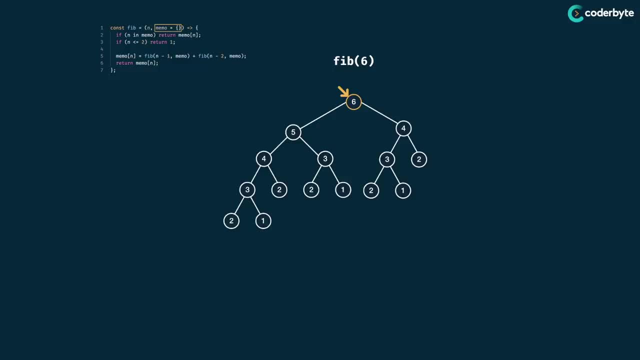 my code says it will initialize it to an empty object, And the really important aspect of this is I'm going to create a new object just for the top level call, But then that same object is going to be passed down to my recursive calls- right, noticing line five. And so I'm going to travel. 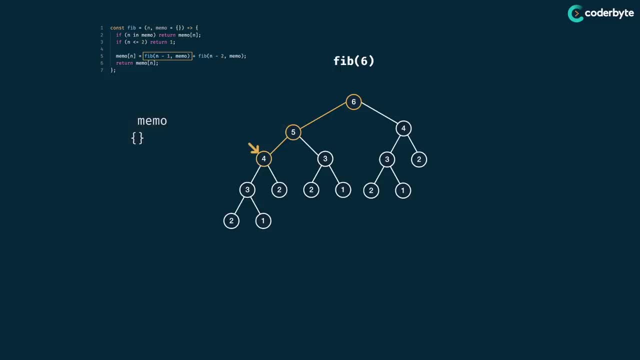 down my left hand path, right: six calls, 55 calls for, four calls three and three calls two, And right now I've hit a base case. So I know that this node of two is going to return one. So that's kind of business as usual, right? In the same way, now I need to evaluate this other node. 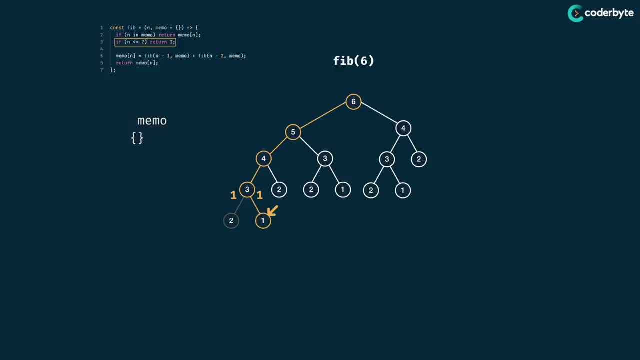 this other node of one, which is also base case, it also returns one, And at this point my parent of three is actually ready to compute the sum of its children, right? So one plus one just gives me two. So I just add up those values And now three is returning to. however, looking at line five of 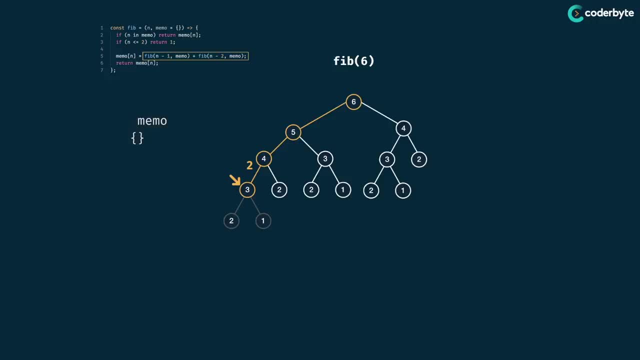 my code. not only is this node going to return to to its parent, it's also going to store it in the memo object, right? So the key insight is: at this point I would add a key to my memo of three. 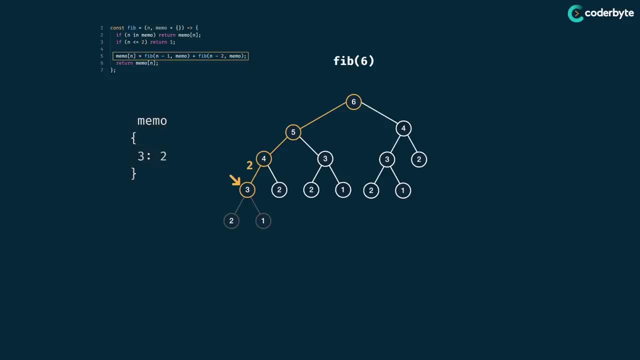 whose value is two. basically, in my memo I kind of read as if I'm saying: hey, the third Fibonacci number is two. right, That in itself is logical, So I can just continue this pattern. right Now I start to evaluate what happens when I'm at this node of two, which is also base case. it returns: 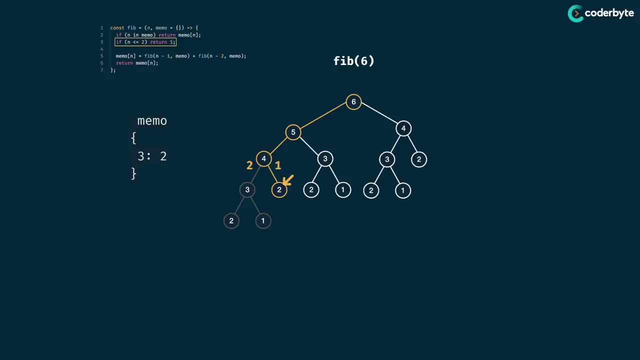 one. Now my call to four. is ready to compute, right, it's going to take the sum of its both children, So it's going to do two plus one gives me three. But of course it's also going to store that inside of the memo, right, it's going to cache that result not to be used later on. 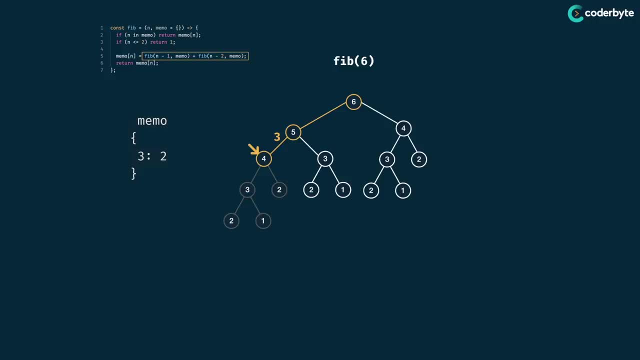 So that means I make the n my key and I make the return value the value right. So I'm going to have four points to three inside of my memo object. And now here's the beauty of this memo eyes solution. At this point I need to compute what happens for fib of three. However, this is 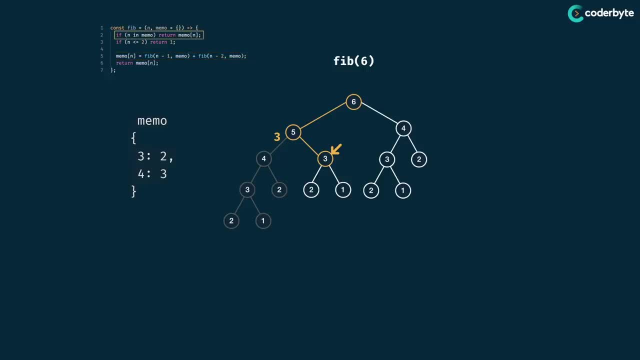 actually going to hit one of the new base cases. I added: right, I know that three is in the memo object looking at line two of my code: right, It's in the memo object And so I just immediately return the store value. And so this call to fib of three is just going to return the stored value of two. And if 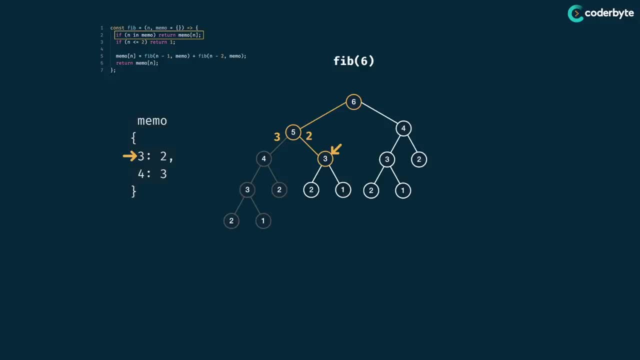 I do that I won't have to travel down the full, you know recursive subtree rooted at three right. I don't need to travel to these nodes at all, So I already used some stored value in my memo. At this point, five is ready to return right. five will take the sum of both of its. 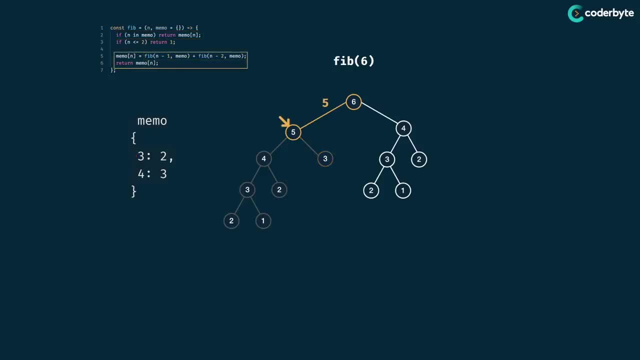 children. three plus two is five and it's going to store that in the memo right. the fifth Fibonacci number happens to be five And now the same thing happens for six is right child. So I have to evaluate this node now. So what is the fourth Fibonacci number up that's actually stored? 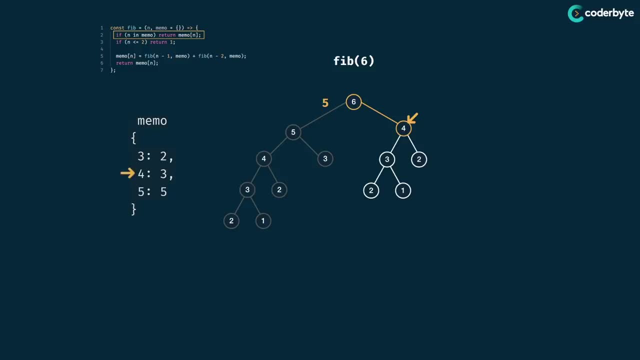 directly inside of my memo. So this actually early returns the stored value of three right And again, the key insight is it will return that stored memo value without having to travel through that full subtree. And at this point I can return for fib of six. so I do five plus three that. 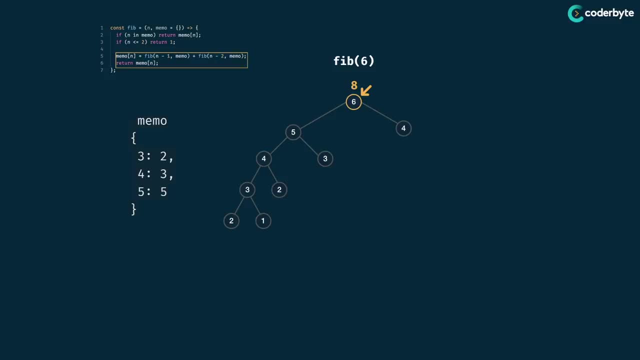 gives me eight. this would actually technically be stored in my memo as well. So I have the six Fibonacci number as eight. And there we have it right: the answer is eight. So it's evident that by memoizing our Fibonacci function we definitely cut down on the 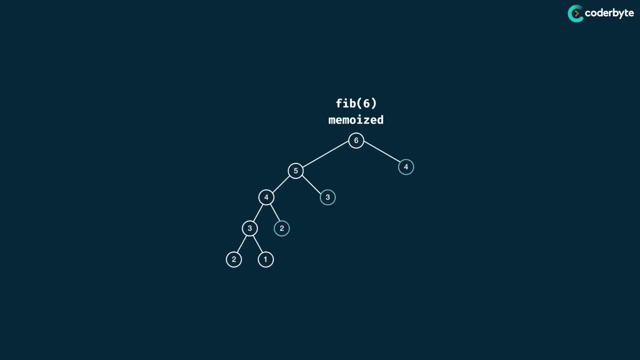 number of recursive calls. we wanted to visualize that we ended up with this kind of structure. Here in a light blue I have a circle: the nodes that we technically didn't need to do, the full recursion at right. So these nodes of two, three and four for the small example of my initial Fib. 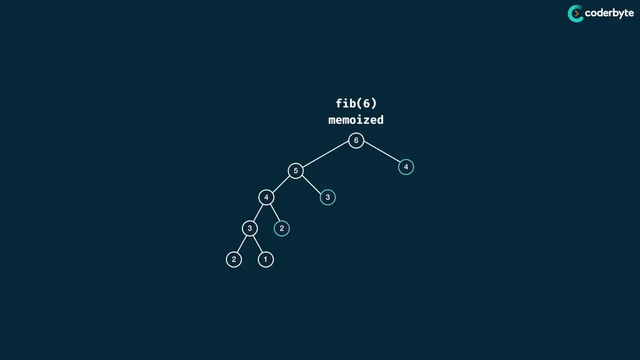 of six, I was able to kind of fetch a value from my memo and kind of forego traveling down the recursive subtree. So what do we actually know about the time complexity of this function? now, Well, I think it's really important that we always 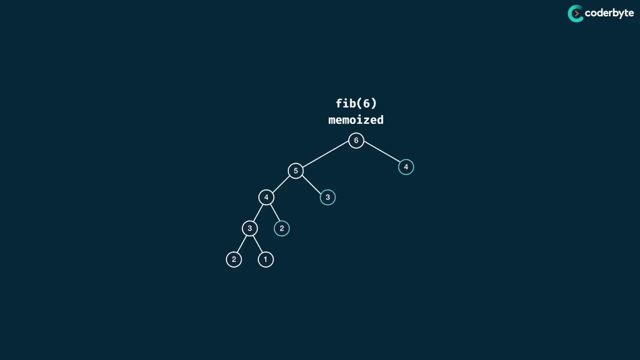 try to generalize things. So we just stepped through a relatively small example of fib of six. But how does this sort of scale? So this is the same tree, let's say? I kind of tidy it up a little bit. So I know that in general fib of six kind of has this structure. So I want you to take a. 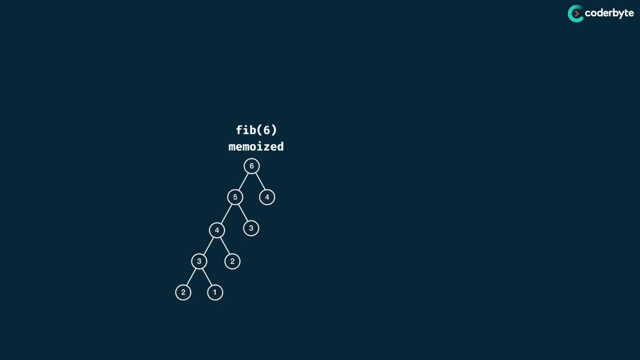 moment. look at this And in your brain picture what fib of six is going to look like, So you can see what fib of seven would look like. If I memoize fib of seven, what would it- sub trees- look like? Well, it really just looked like this. Notice, if I root myself at the seven node, it's left. 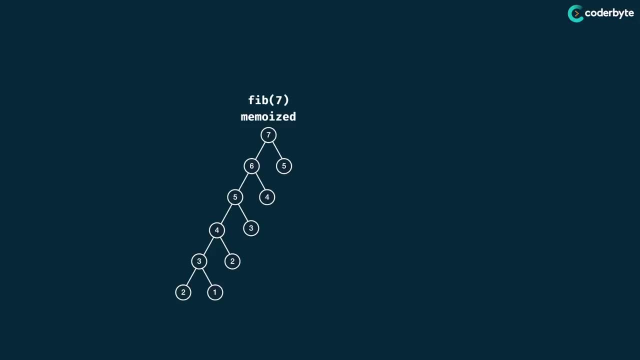 child is still six right minus one and it's right child still five minus two. So this still obeys the laws of Fibonacci. If I asked for fib of eight memoized, the structure would be like this And nine would look like this: See, the pattern looks like at this point. we're just growing this like. 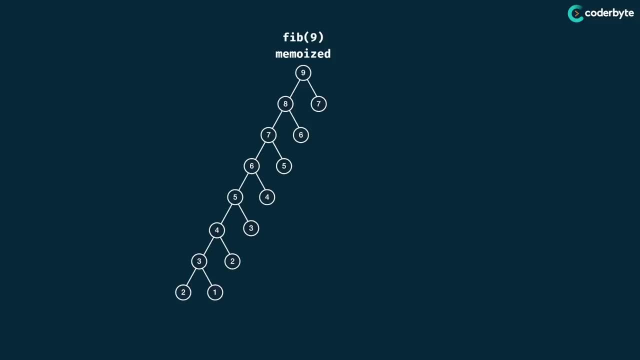 memoized chain in a linear kind of way. We're not convinced by you know that, just like structural argument. Let's say we were a little more methodical. We know that in this drawing there is some common ground right Again, like I, 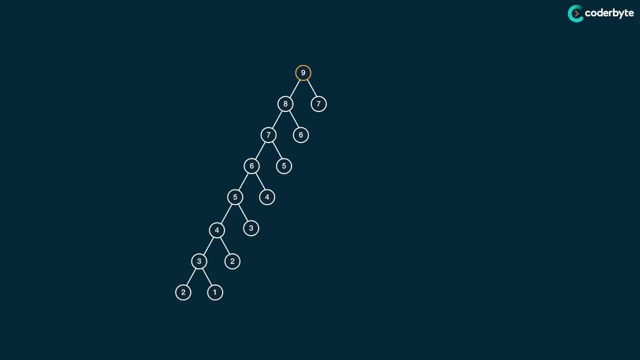 always say, when you tackle these new problems or new patterns, try to find some familiar territory, right. Where can I recognize stuff I've seen previously? So I look at this chain. I go nine, eight, seven, six, five, four, three, two right. So this goes all the way down in a very 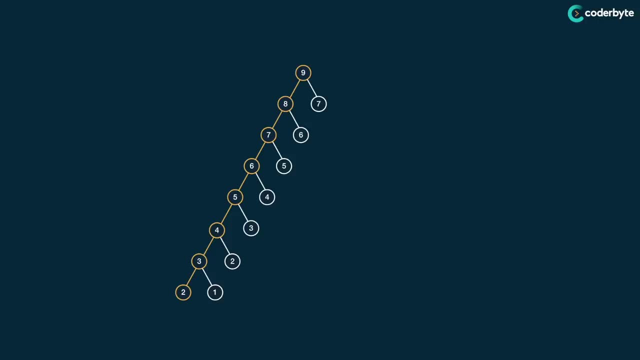 very, very linear fashion right, Just counting down. So I know that if I just look at this, I'm going to see that this highlighted chain in yellow that's definitely just n nodes right Where n is my initial top level call. So I know that what I have highlighted in yellow is just a. 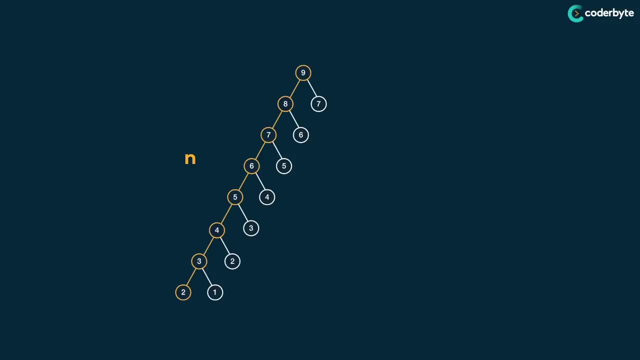 linear chain. right, They're exactly n nodes, But I haven't accounted for everything in this picture right. Some of the nodes are still in white, meaning I need to kind of work them into my description of what the shape of this tree is. Well, I know that each of those white nodes is 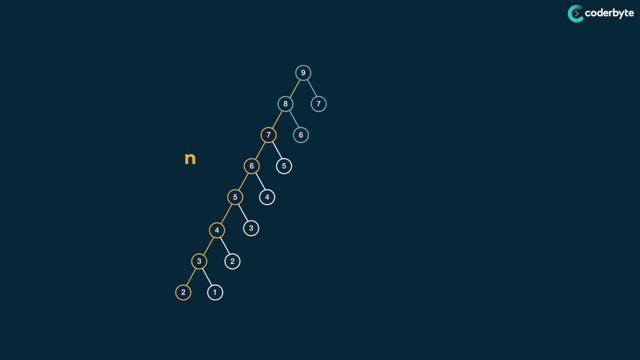 actually connected to some of the nodes I've colored in yellow. They're kind of paired off in a way. right For every node in my yellow chain it has exactly kind of one partner node, one right-hand node on its right-hand edge, And overall if I have n pairs that means I have two n things. 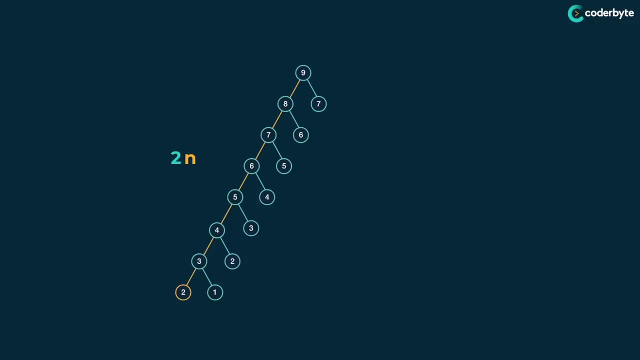 overall. right, There are two things in a pair. So overall the number of nodes is roughly two n, And I know that that can actually be simplified right. The time complexity here would be two n, which just simplifies to n time complexity, And using the same arguments we did for our 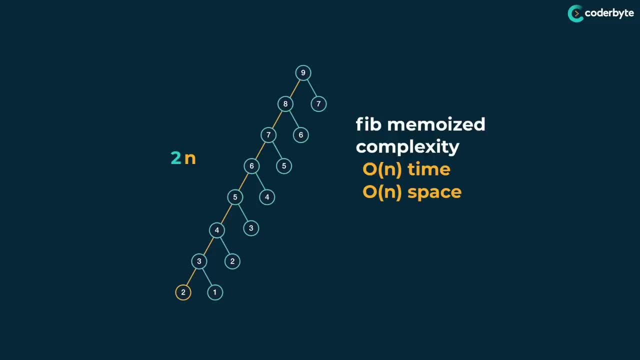 space complexity. we know that the space is going to be n as well, And this is pretty powerful stuff. By memorizing our fib function, we brought it down from an exponential time complexity to just a linear time complexity. Pretty cool stuff, right? All right, I think we're ready to. 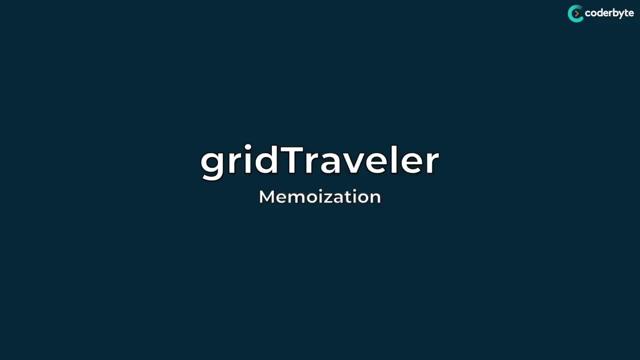 graduate from Fibonacci And what we'll do is work on a more involved problem. This one has more of a narrative to it. So say that you're a traveler on a two-dimensional grid. You begin in the top left corner and your goal is to travel to the bottom right corner of that grid, And the rule is you can. 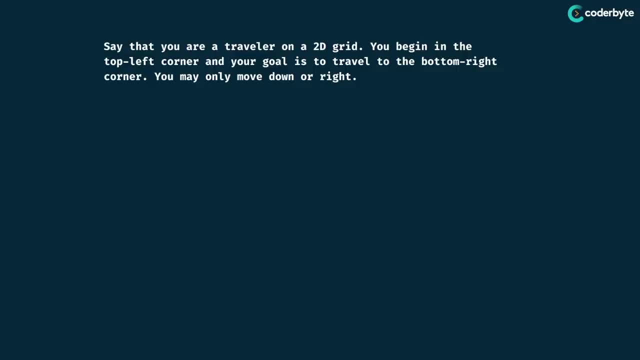 only move down or to the right. That means you can't move up or to the left, and you definitely can't move diagonal. That being said, in how many ways can you travel to the goal? That is, how many ways can you travel to the bottom right? 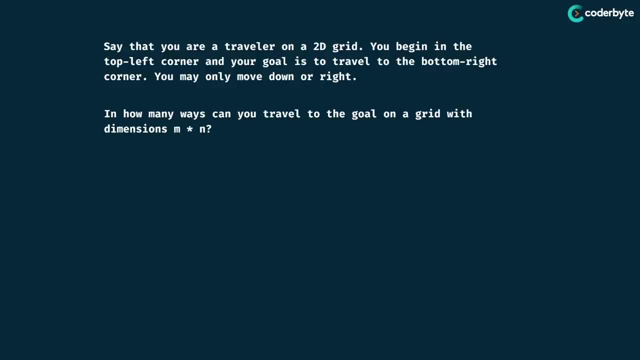 If you had a grid of dimensions m by n. So the first thing I recognize here is: looks like the grid may be a rectangle, not necessarily a square right, And overall what we want to do is implement a function that calculates this. That is, our function needs to take in the dimensions of the. 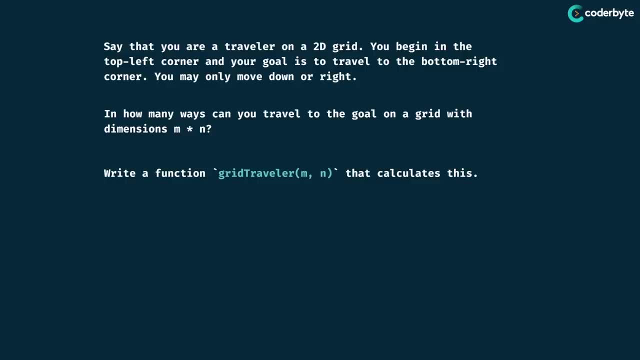 grid. And so before we hop into sketching a strategy for this one, I think it's really important that we make sure that we actually understand what this question is asking. So let's say they ask us to calculate grid traveler of 2,3.. That means they're asking us: in how many ways can you travel from the? 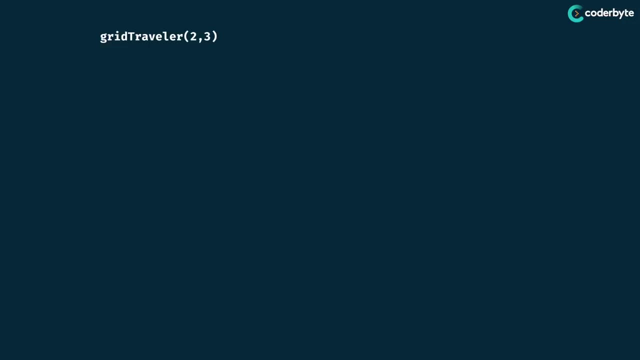 left to the bottom right of a two by three grid. I will tell you right now that the answer here should be three, right? So there are three ways to do that And, in particular, you can imagine that we had, you know, a two by three grid, So that means two rows as well as three columns, And we 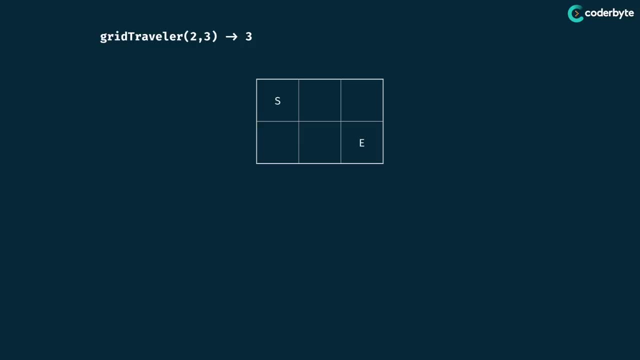 start in the top left and our end goal is in the bottom right. And so why do we say that there are three ways to get from the top left to the bottom right? Well, they told us in the problem that we can only either take a right move or a down move. So one of the ways would be going right, right. 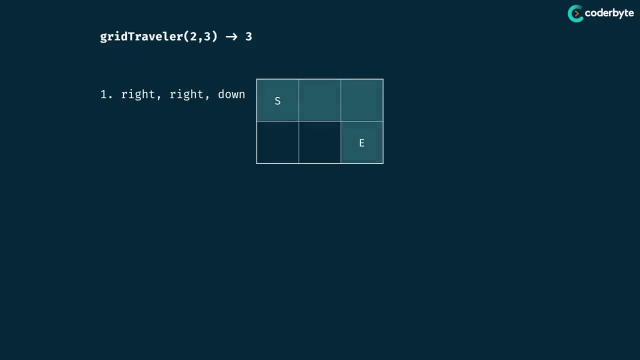 down right. That would bring us from the start to the end, And it would kind of look like this. In a similar way, another path we can take is doing a right down right. it would kind of look like this, And the only other way would be going a down right. 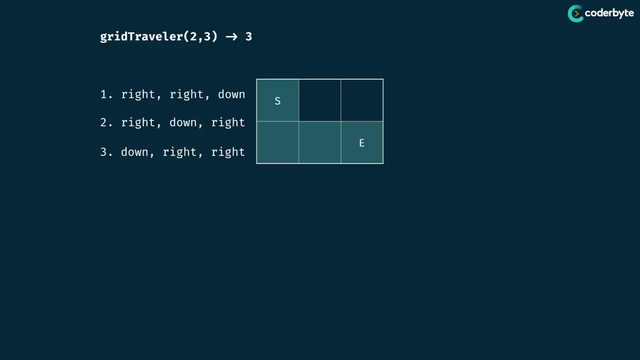 right, which would look like this path, And that's why we say there are only three unique ways to travel, not through a two by three grid, Alright, so that was just one example of how we might call grid traveler. I think what's really important to notice is try to also frame the problem as if you 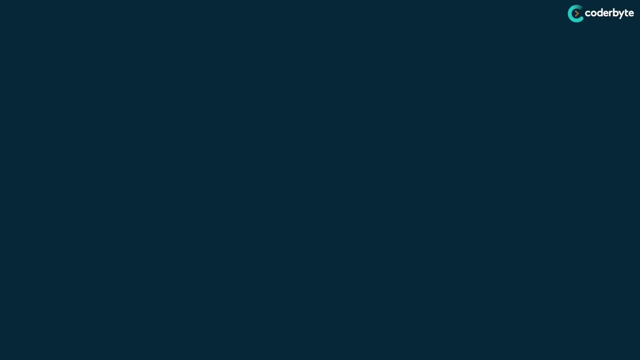 were given some relatively small inputs. So I think they're really important cases. but it's really important to think about is what happens if they give us like basically the smallest valid grid we could have, that is, a one by one grid. This one is kind of trivially simple. 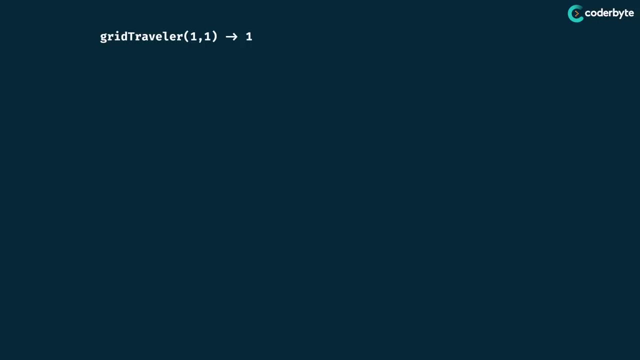 right. A one by one grid only has one unique way to travel from the start to the end, And it's kind of concise in that if you had a one by one grid, there's really only one position right. So that means that the start is really the same as the end And kind of you already have the problem. 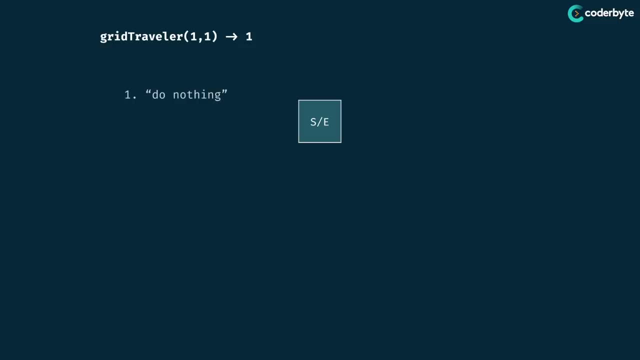 solved out the gate, because to travel from the start to the end you kind of just do nothing Right. So the logic here is: in a one by one grid, there's only one way to travel from the start to the end. you're kind of already there, So you don't need to take any moves. Something else we might think: 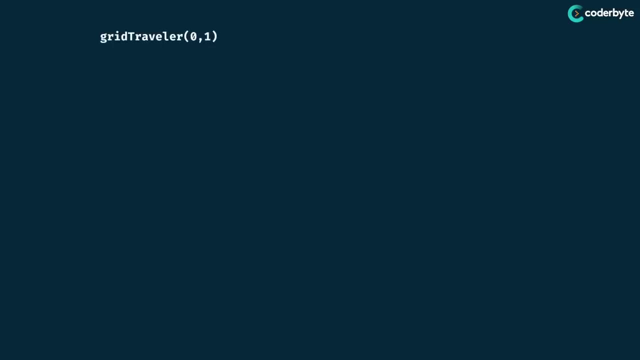 about is what happens when one of our dimensions is zero. So let's say, someone asked us to calculate grid traveler of zero comma one. This is a kind of strange question to ask, Because, for one, if there are zero rows and one column, that kind of means that the the grid is empty. So I would 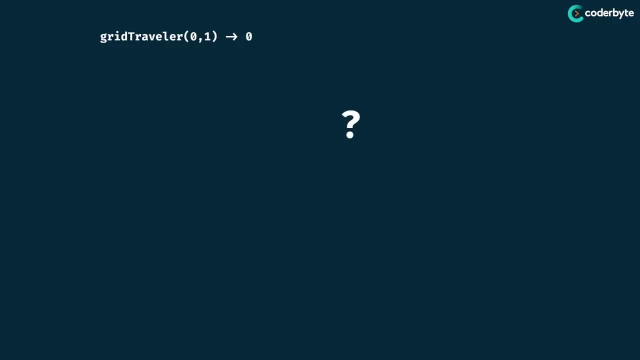 consider that as there being zero ways to travel through that grid, because the grid is sort of invalid In a way. in a similar way, if I asked you for traveling through a one by zero grid, there's still no grid to be found here, right? So it should also return zero. And likewise, when either of the dimensions 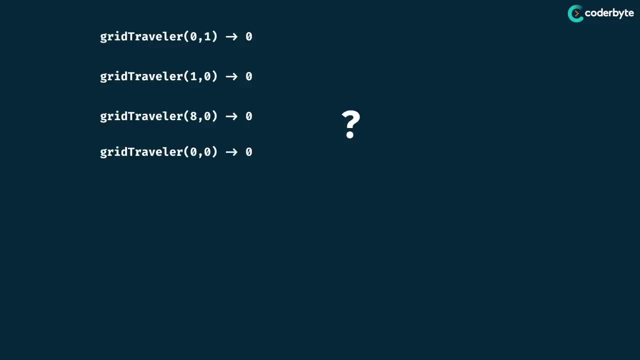 is zero. the answer should just be zero, right? If one of your dimensions is empty, then there really is no grid. So maybe you're catching on into why I brought up those trivially small grid examples, right? Those kind of sound like base cases which we can use to reconstruct a larger answer. But 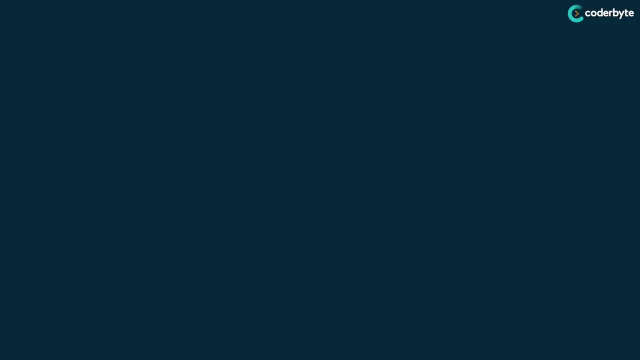 let's stay grounded and look at another grid. So let's say, I asked you to calculate grid traveler of three comma three, right? So I want the answer for a three by three grid. Well, how can we reason that one out At this point? what I'm looking to do is sort of frame the problem in a way where I can decrease. 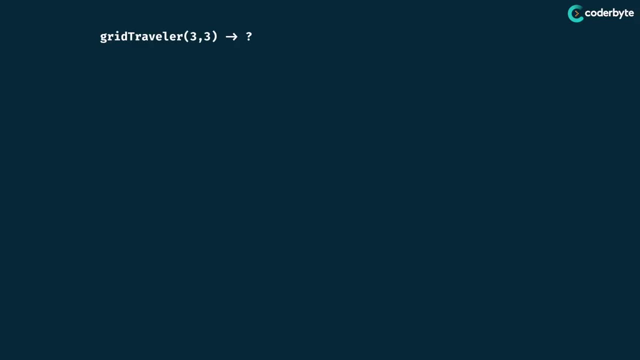 the problem size, usually by mutating the arguments to my function call. So let's imagine this three by three grid: As always, I want to move from the top left to the bottom right. So I begin at this position. let's say: And so I know that overall I have this top level problem of saying, well, I'm 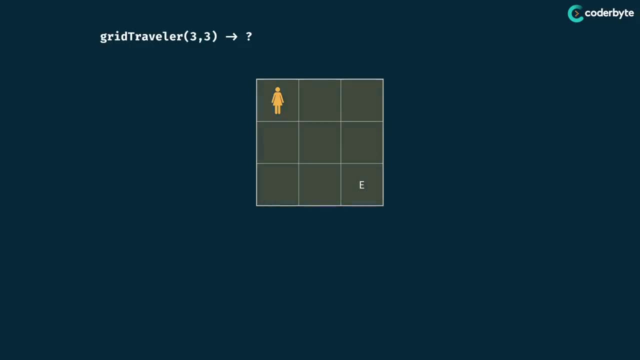 going to move from the top left to the bottom right. So if I move from the top left to the bottom right, I can just move one way or the other. And I can move into the bottom right. And let's say I move to the bottom left, I can move to the bottom right, And if I move to the bottom I can move to. 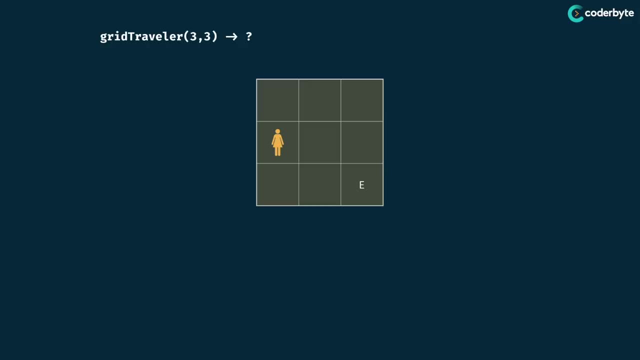 the bottom right. So that's basically saying, how many ways can I travel through this entire three by three grid? Let's say I took one of the moves right. I can move either right or downward. Let's say I made the decision to move downward. Well, if I move downward, then I would appear here now. I. 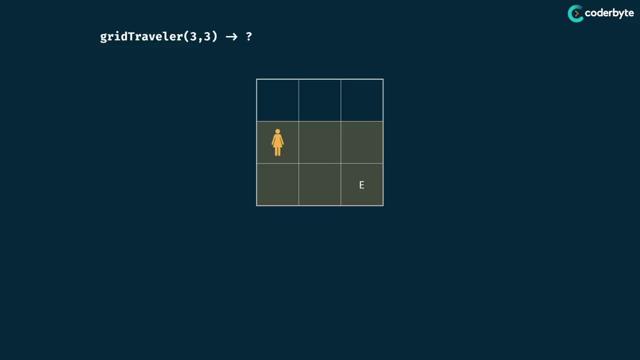 grid where now I'm really trying to answer the question: hey, in how many ways can I travel through this two by three grid? And this is a really important way that we're shrinking the problem size right. I had a three by three grid initially. now I have. 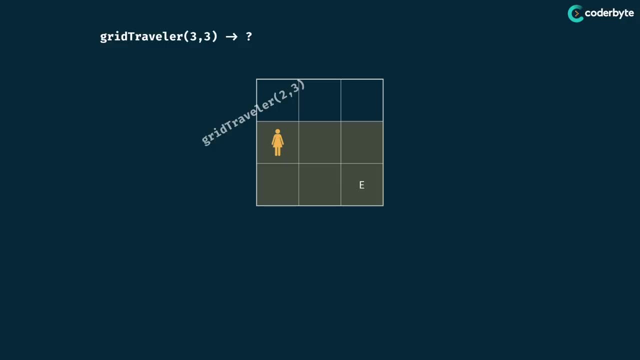 a two by three grid And this is really like the relative grid from my current position, will say spanning all the way to the end position. So if you look at this coordinate of like two comma three that technically that is like not the coordinate of the person. 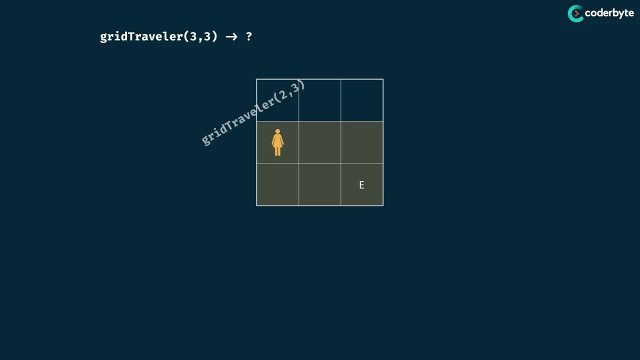 within the larger grid. this is really the size of the rectangle that the person is trying to cover now, right? So in a similar way, let's say that, hey, I wanted to move to the right now. well, that would also shrink the grid along a different dimension, So I'd appear. 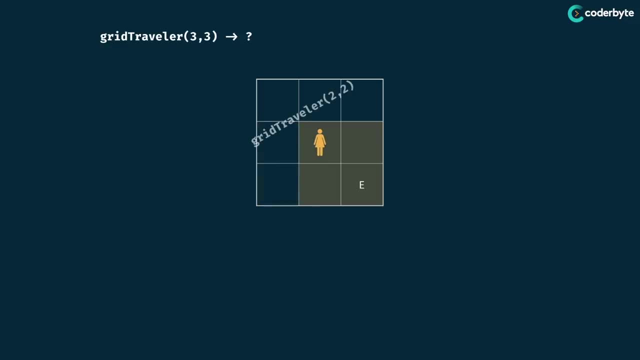 over here And now I have a two by two grid that I'm trying to solve And if I keep following this pattern, we're going to keep shrinking on the problem size over here. Now I'm asking for a grid traveler of one by two And finally, if I take a right move over here, I'm asking: 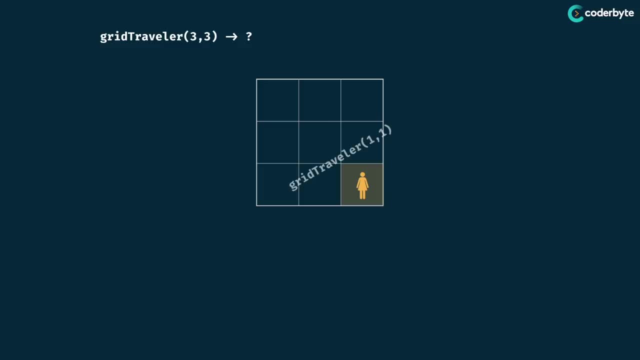 for grid traveler of one by one, Which I know is one of those sort of base case scenarios that I had previously. So that's going to be really useful when we actually implement this in some code. And so the key insight here is when we make a move through the grid, that is, when we go right or downward. 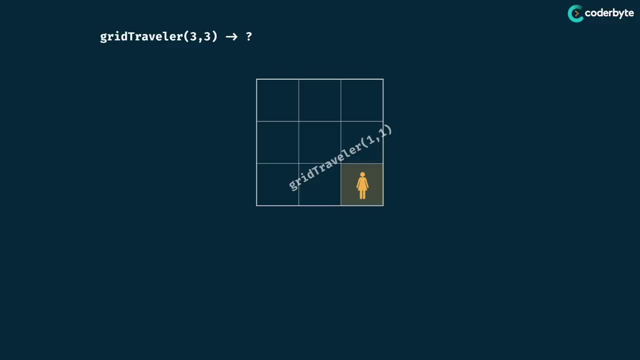 or basically shrinking the effective size of the playable area. right, our grid gets smaller along one of its dimensions- Awesome, So I think now we're able to see that, hey, this grid traveler problem definitely has some overlapping sub problems, right? Well, 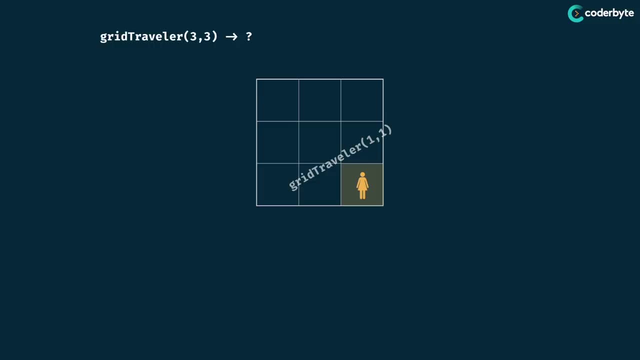 let's say I tried to take more of like a programmatic approach, something that will be doing a ton like basically for every problem in this lesson is, whenever we have a problem that we kind of know is going to be recursive, the move is to really structure it like a tree, right? 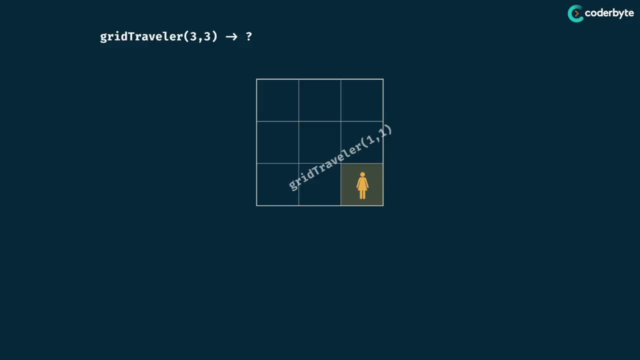 I want to really visualize this because I know that if I had a tree structure on pen and paper, I can implement that with just some recursive code using some JavaScript right. So let's say that I wanted to take more of a tree based visual understanding. 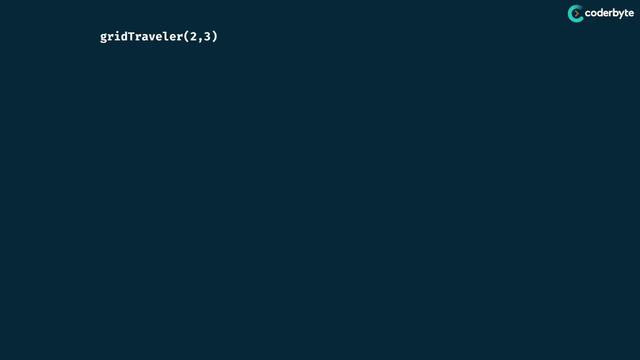 now a grid traveler of two comma three. So I know that usually the way we do this is we encode nodes of the tree Using the arguments to this function. right Now I have two arguments: or I have the number of rows and number of columns, Whereas before, for something simple like Fibonacci, I only 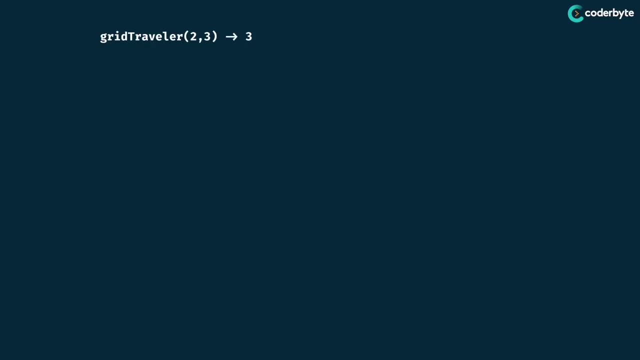 had a single argument. So in the long run I know that the answer I should get back is three. So we'll just keep that goal in mind. But let's start to flesh out this diagram. So I'm going to start with that top level call of two comma three. And now I think about 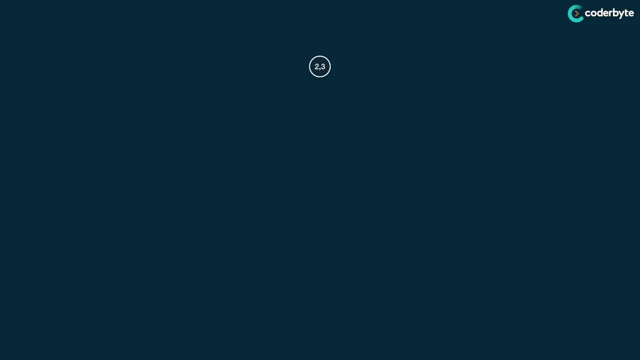 how this node can transition to other nodes, right? How does the state of my game actually change? Well, I know there are really two options I can take. right, you can either have one child going downward or another child going rightward, right? Those are the two options based on. 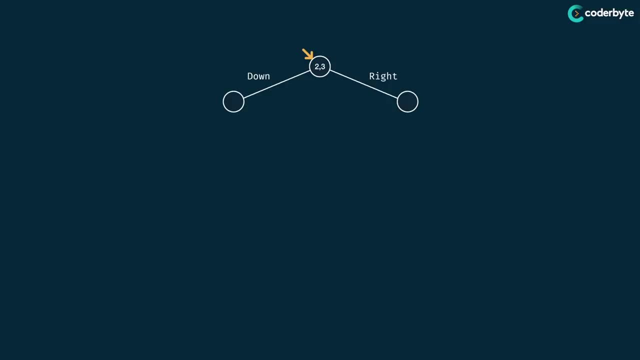 the gameplay here. And so if I go down, how does that change the number I put in the node, That is, how does it change the dimensions of the playable grid area? Well, if I go downward, then I'm reducing the number of rows by one, So that means my left child is just one comma. 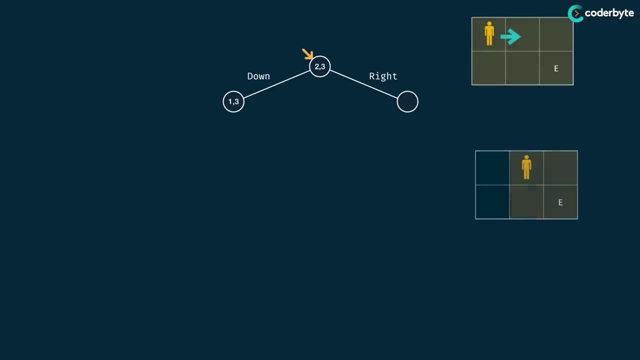 three. Now, if I had moved to the right, that would mean I'm reducing the number of columns by one. So my right child is just two comma two. Notice that from here to child, all I'm doing is reducing one of the dimensions by one. right That. 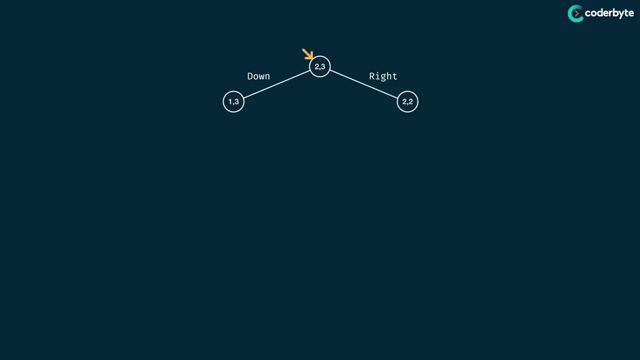 means you're either going downward or going to the right, And I can just carry over this pattern recursively, right? So let's say I'm fleshing out this node Now. if I'm at one comma three, then it's children would be just 03 and 12.. In a similar way, if I root myself, 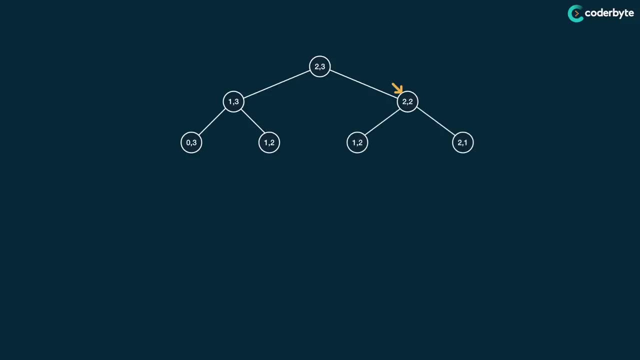 at two two, then I have children of one two and two one. But now let's notice something important Here. I've kind of spotted a node where I have zero comma three. Remember what we trace through in terms of the visual drawing. What is this node trying to answer? Well, let's 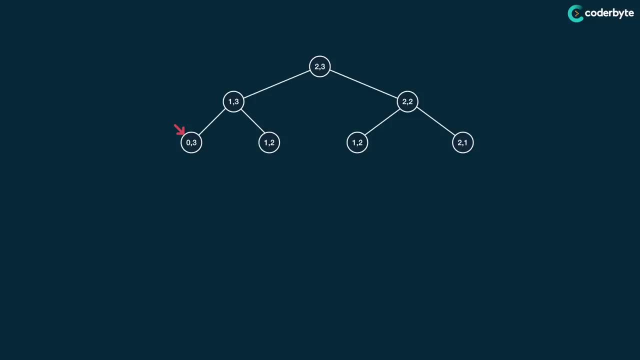 notice saying in how many ways can you travel through a zero by three grid, but if you have zero rows and there's really no grid to be dealt with. And so I think for this node of zero, comma three, or really any node that contains a zero, we don't need to actually 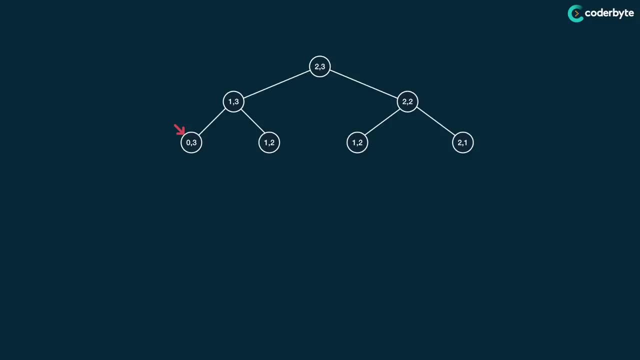 flesh out its children. So instead I'll work on recursively drawing out these other nodes, So we'll carry over this pattern. At this point we've actually hit, I think, all of our base scenarios right. So if I look at these nodes that have one comma, one that was exactly. 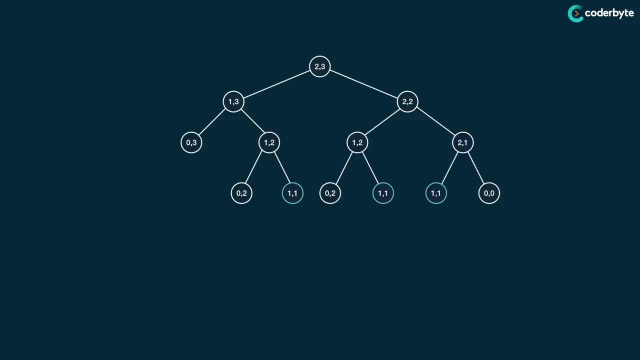 like the affirmative base case, meaning that I know trivially I can solve the one by one grid. In other words, these function calls are going to return one right in a one by one grid. there's exactly one way to travel from start to end, right? you kind of just? 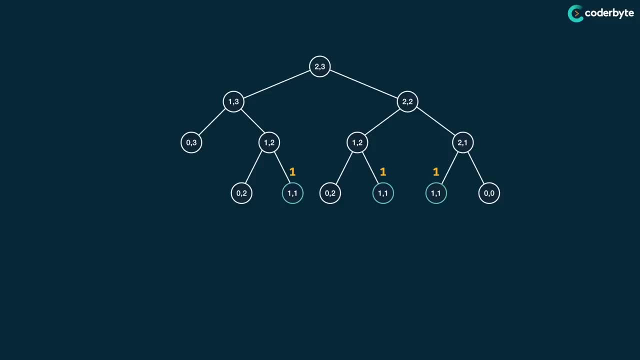 do nothing. And, on the flip side of that, for all those nodes that contain a zero, they're also a base case, but they're kind of like the negative base case, meaning that they're. there is no way to actually travel from start to end. So, for all of these nodes containing 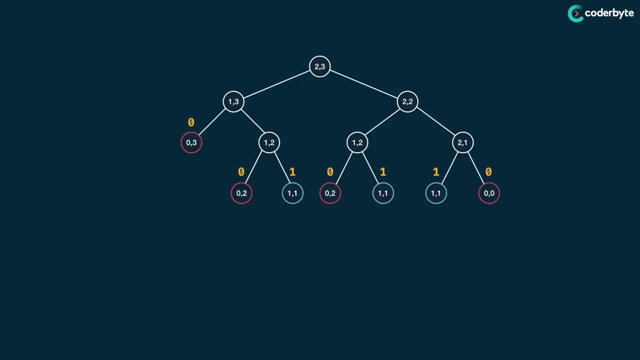 zero. they should return zero to their parent, right? there are zero ways to travel through that grid At this point. I just sum up these values at the parent node, right. so I just lift these and then I add them together And if I look at what these things are saying, 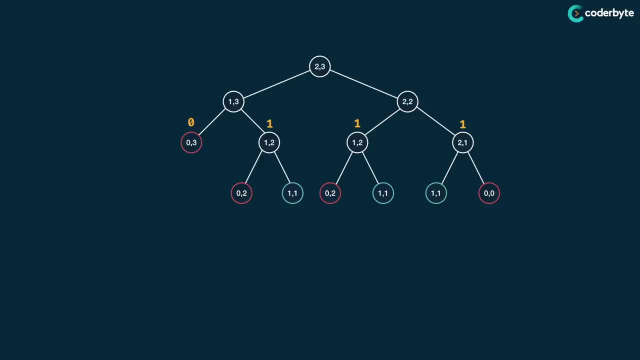 right, if I look at like the node one comma two above, it is one meaning. there is one way to travel through a one by two grid. right, you kind of just move rightward And so I carry this pattern over. I keep adding the children. 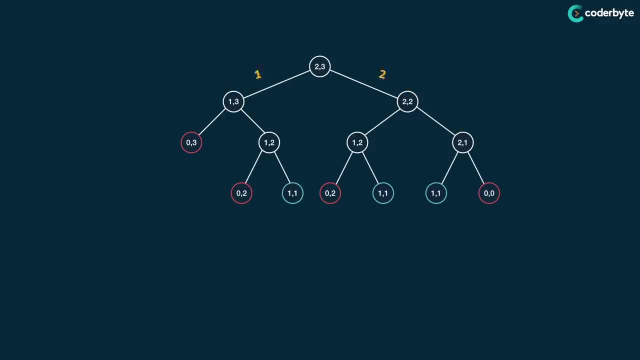 nodes at their parents And this carries up all the way to the root node And what do I know? there are three ways to travel through a two by three grid. So, although there's like a narrative and there's some, you know, cute story behind this problem, it's really just 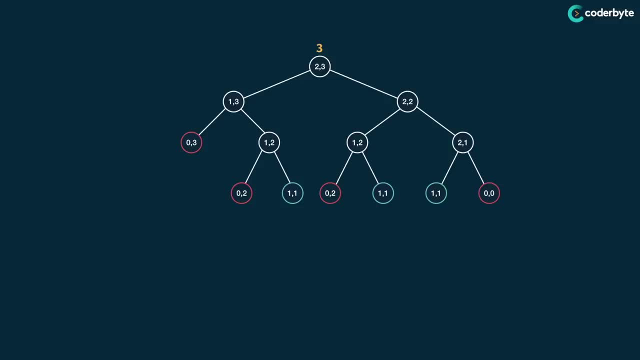 a spinoff of Fibonacci, And that's going to be the case with many of these dynamic programming problems. So we've confirmed that there are three ways to travel through a two by three grid, And there's also some other information encoded in this tree. I know that whenever 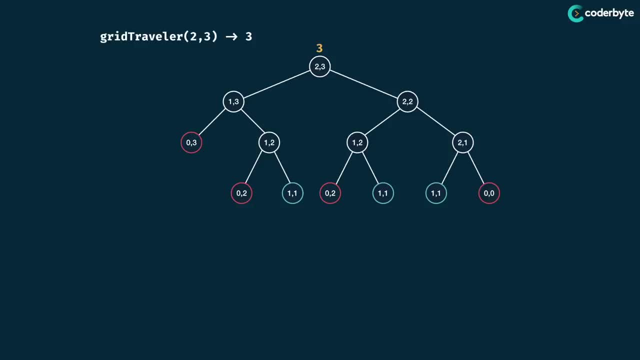 I took, like, a left hand edge in this tree- едь tree- that represented the choice of going downward, And whenever I took a right hand edge in this tree, that represented the decision of moving rightward. And so, if I have that pattern in mind, that not only have I been able to count the number of ways that I can 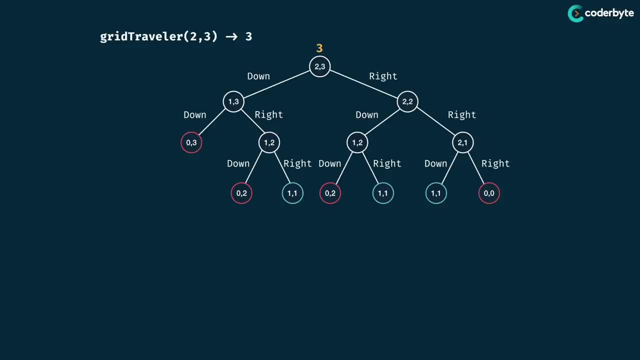 win the game, but I also know exactly which combination of moves lead to a solution. One of the ways to win this game is to go down, right, right, Another way is to go right down, right, And the final way is to go right right down, So we can glean a lot of information. 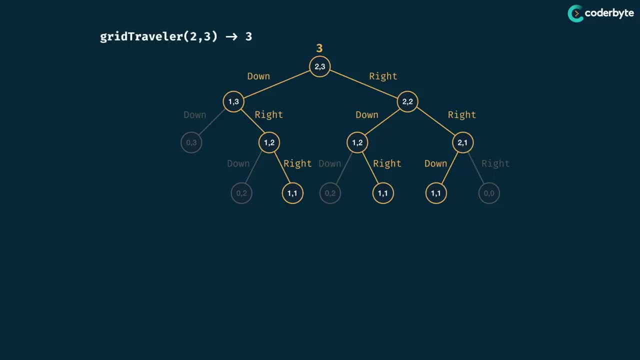 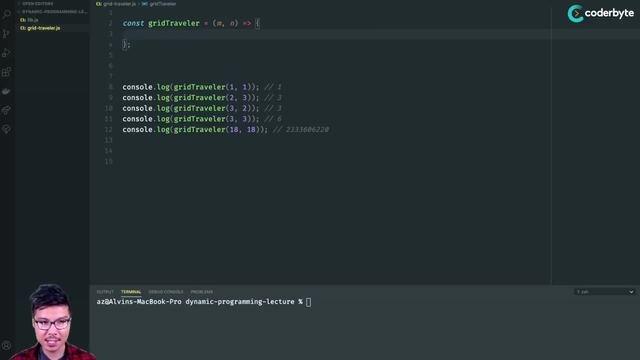 just from the same tree structure, Cool. So I think that's enough drawing for now. Let's go ahead and implement this in some code. All right, programmers, here we are back in my text editor. let's go ahead and implement this grid traveler function. So we want to go with that recursive strategy. So I'll start. 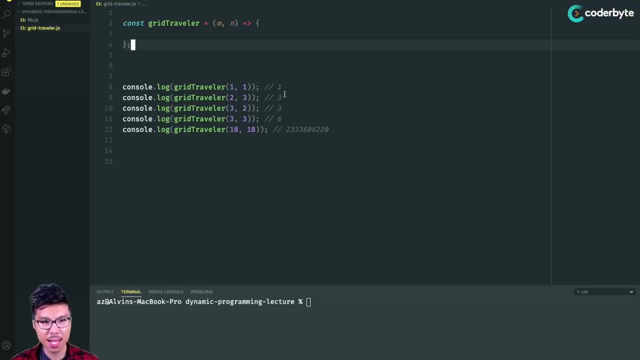 by just laying down my base cases. I already referred to the fact that, hey, one of our base cases is we have a one by one grid. just go ahead and return zero, right? So that's really easy to do. So I'll check. hey, if m is one and n is one, then the answer is just trivially one. 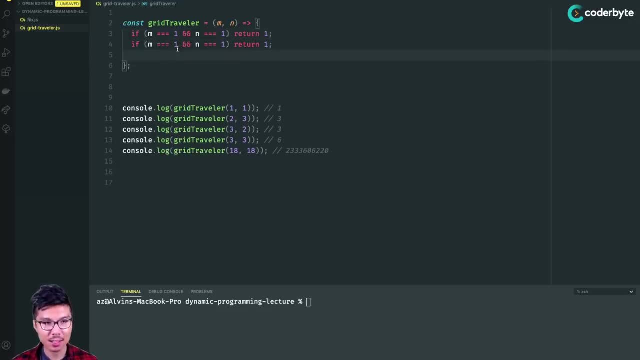 right. Then along with that, I also have the base case when I had like an invalid grid. That means if either of my dimensions is zero, so I'm using an or here. right? If either dimension is zero, then your grid is empty, which means there's definitely no way to travel. 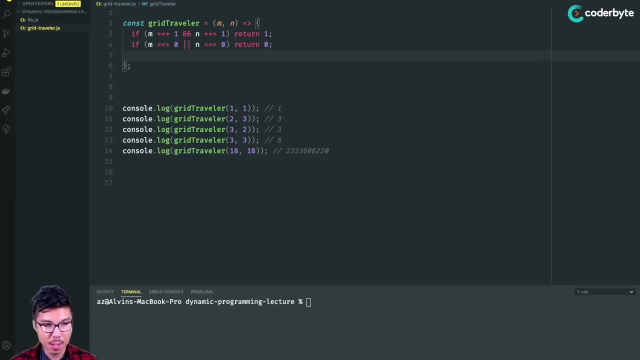 from top left to bottom right of that grid. Cool, Then my recursive scenario is very straightforward. all I need to do is get the sum between me going a downward and me going rightward, right. So if I go down, remember m is the number of rows. if I go down, then I'm decreasing the number of rows effective. 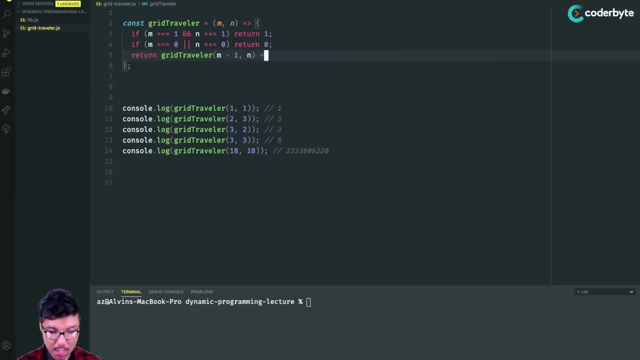 rows, that is by one, but I keep the same number of columns And then, in a very symmetric way, if I move to the right, that means I still have the same number of rows. So I keep him, but I decrease n right I have one less column. So this code is looking pretty sharp really. 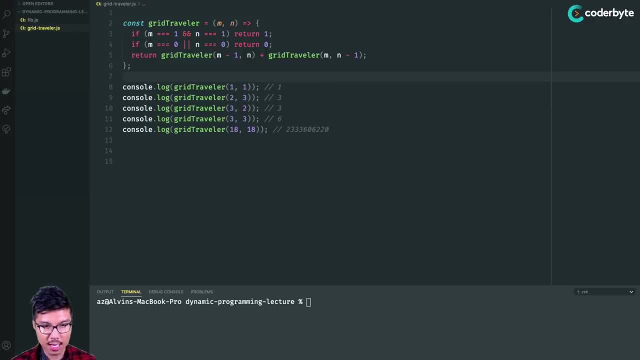 just some reminiscent Fibonacci style code. Let's go ahead and give this a run. So I'm running a few examples over here And these are the expected results In some comments. go ahead and bang this one out. Great traveler, Cool. So I get the first four results: 1336. 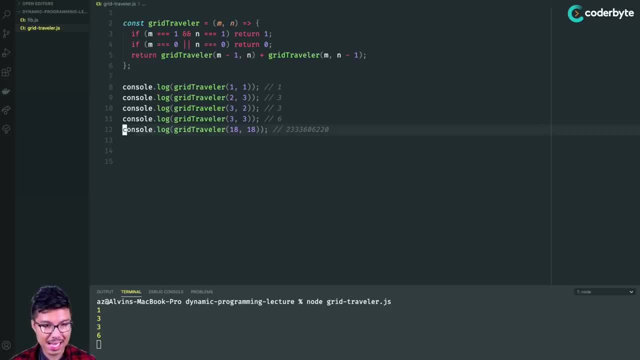 looks like it's working just like a charm. However, for this last example of an 18 by 18 grid, it looks like my programs hanging right now. It's actually a little too slow to calculate an 18 by 18 grid, So you probably see where this one's heading. Let's go ahead. 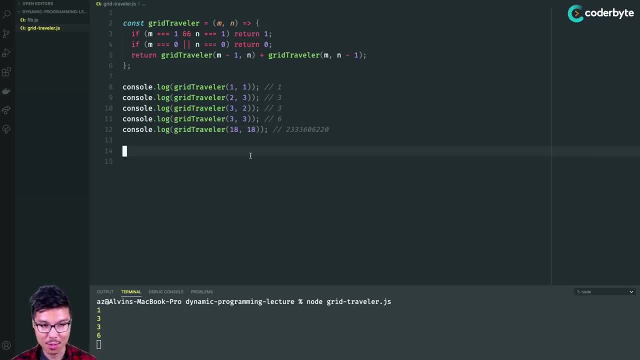 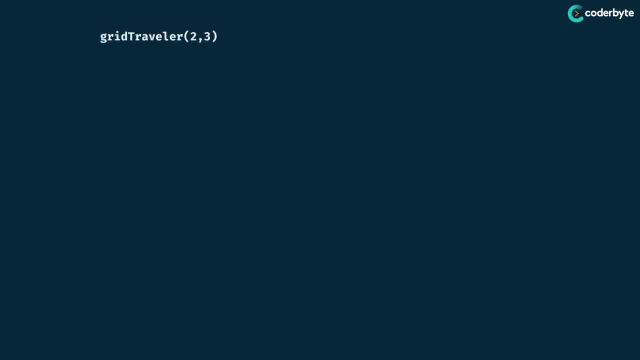 back to the drawing board and really understand a why this code is fairly slow. All right, so here we are back in the drawing board because it looks like we hit a wall when it came to our recursive implementation of grid traveler. That being said, I think implementing the brute force solution here is actually a really 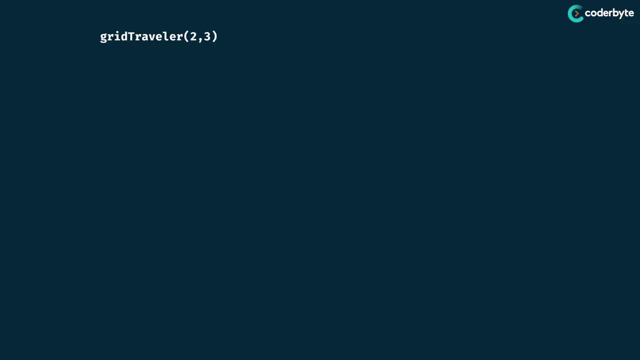 logical first step, And now we can just focus in on where there is room for improvement. So our first question is: you know what is the actual time complexity of this implementation? Well, I know what I call a grid traveler of two, three. the full tree would explore is 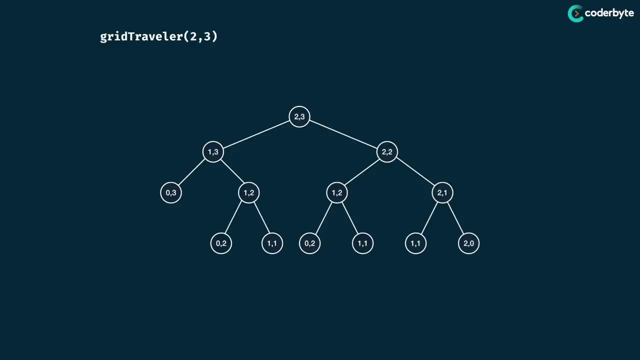 this right And, like we said in our Fibonacci, to understand the time complexity here it's really about to understand the number of function calls we make, which is really the number of nodes in this tree, And of course I want to generalize my understanding for any large inputs. So I know that this tree sort of looks. 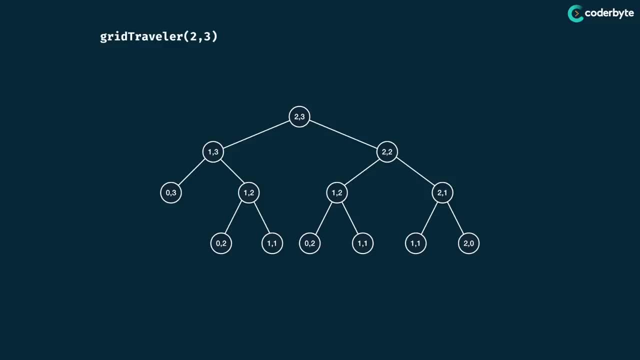 you know, binary in a way, meaning that a node can branch to up to two children, which makes sense because, from one position of the grid, I have two choices to make: right, I either go down or I go to the right. But that being said, I need to realize what the 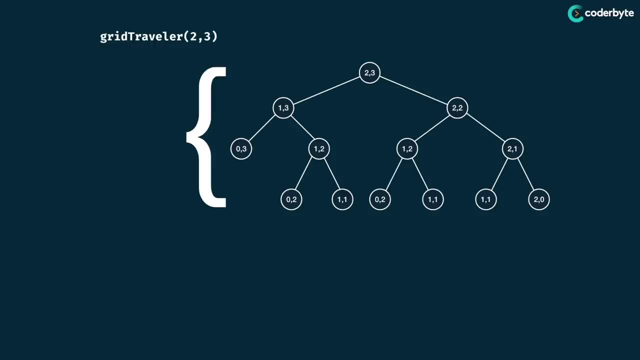 height of this tree is. And this one's pretty interesting because out the gate, we actually have two input arguments to our function. I'm given two numbers, m and n, And since this function contains two inputs, it should be the case that our 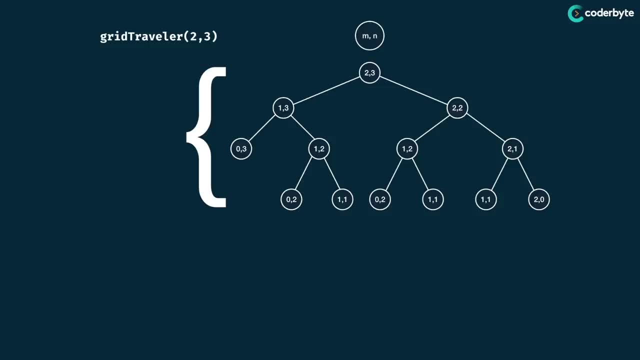 final complexity analysis actually describes it in terms of those two number inputs. So what I'll do is try to recognize the height of the street And so I'll just choose some path from the root to the leaf And kind of in the recursive sense that means I take. 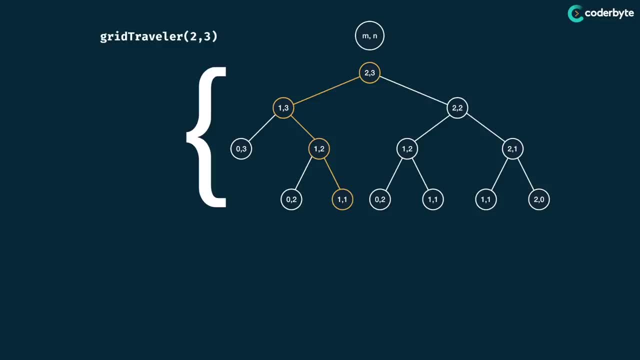 some path from my top level call all the way down to the base case, and preferably the farthest base case. So I know my base cases are either when one of my arguments turns to zero or when both of my arguments turned to one, And I think in general the farther base case would be. 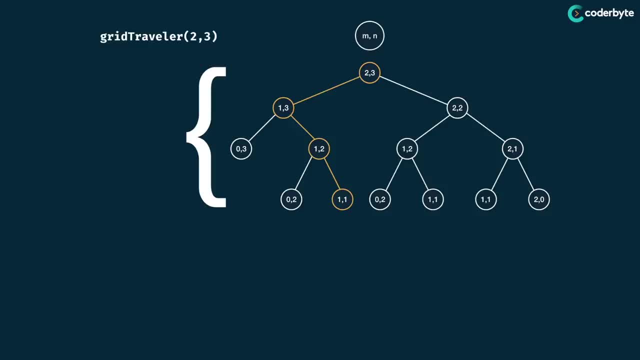 a scenario where both of my arguments are one. So here I have a path highlighted that ends in a one one, And in general I know, from one node to the next, what I do is either decrease the M by one or I decrease the N by one. it's never the case that I can decrease. 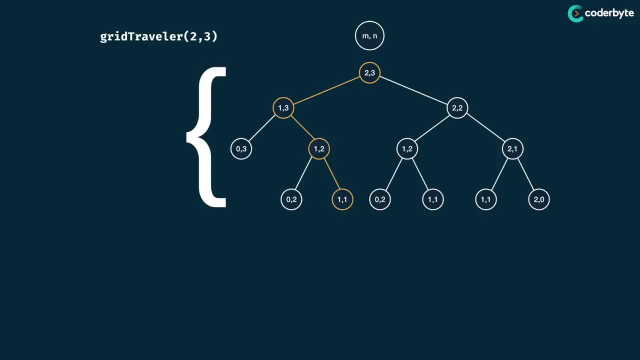 both of the numbers by one, because that would kind of entail that you're moving down the line, And so I'm going to go ahead and do that, And then I'm going to go ahead and do that, And then I'm going to go ahead and do that, And then I'm going to go ahead and do that. So I'm going to go ahead and do that, And then I'm going to go ahead and do that. And again, I think, in general, the farther the base case, the farther the path is going to go. But in general, no matter what you do, it's going to end up with a path with 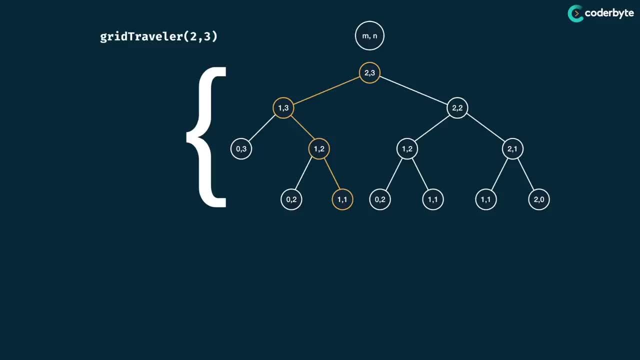 one of at least one point one, But in general, the farther the path you take is going to end up with one point, three points one. So if I don't have that path, I'm going to kind of go ahead and take the path that goes diagonally across the grid, which is not allowed in the gameplay. So 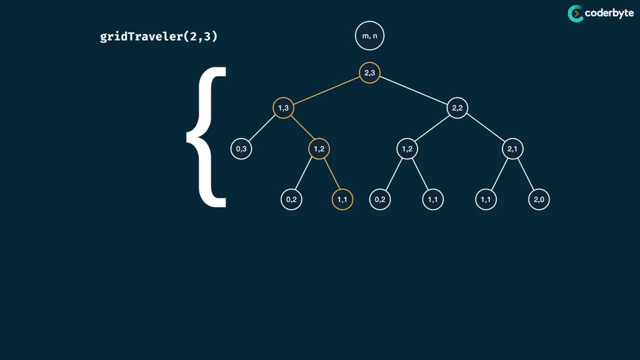 if I can either subtract one from M or subtract one from n, then overall a path from my initial input down to a space like 11 is going to have a distance of n plus m. you basically have to subtract, you know, n and m from your initial node to reach that bottom level. 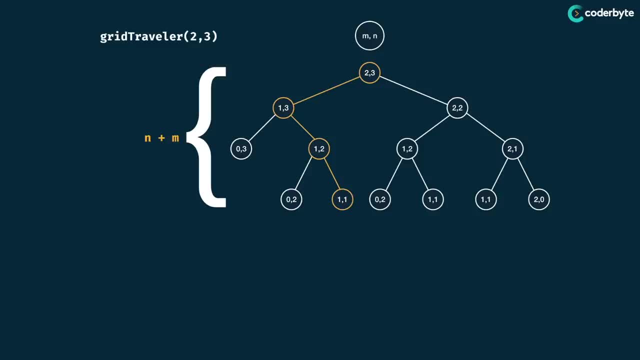 of one comma one. So that kind of tells me the number of levels in this tree, right using the same arguments as before. And it's still the case that most of this tree is going to be binary, meaning that a node branches to two children, And so I have that two times. 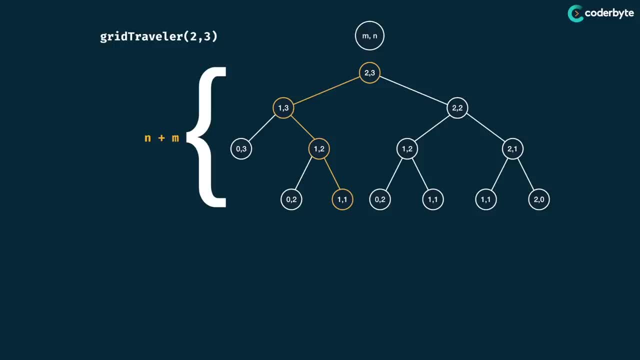 two times two pattern for the number of levels in this tree. we're saying that they're n plus m levels, So really the time complexity is two to the n plus m power. right, so still some sort of exponential. Now it's just sort of the multi variable exponential, because 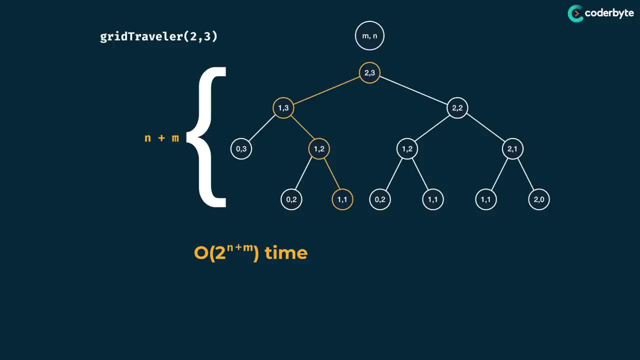 I have two variables of m and n. And likewise for the space complexity. we know the space complexity in general for recursive code is just going to be the height of the tree. the height of the tree gives us the maximal stack depth of the recursion. In this case it'll. 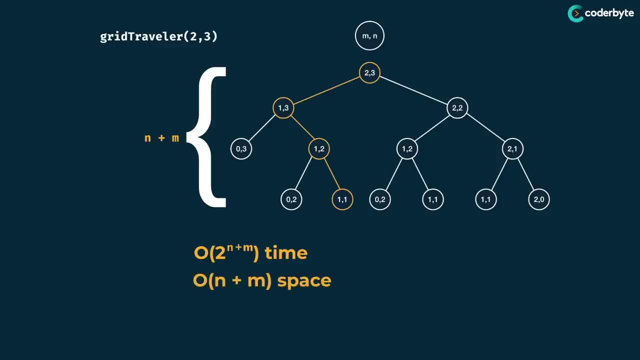 just be the number of levels still, which is n plus m. Cool. So obviously the limiting factor here seems to be that time complexity of two to the n plus m time. Alright, so you probably anticipated the time complexity of this one being exponential. That being said, 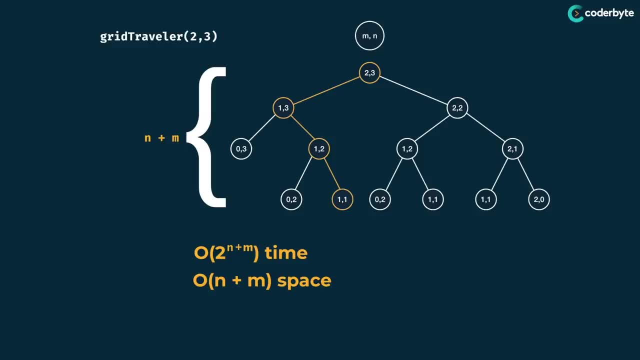 I think it's really important to still have a nice argument to you know, say what the time complexity is. That way you can get a massive buy in from your interviewer, right. So don't skip these steps of trying to draw it out. 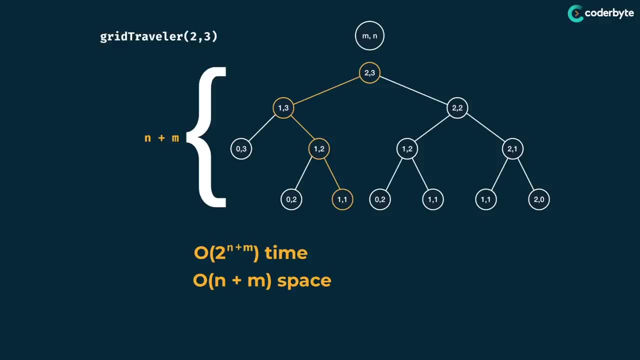 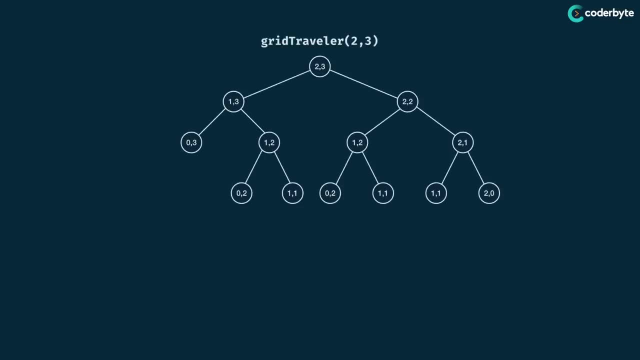 and actually defend here, reason for why the time complexity is exponential. But let's try to improve this now. Is there any room to actually improve the runtime of this function? Well, here's that same drawing right, just sort of cleaned up. So I have grid traveler. 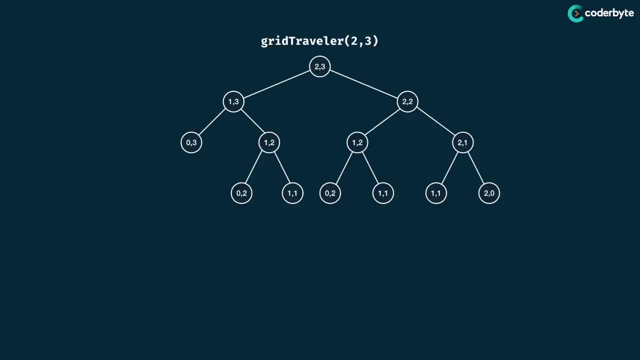 of two comma three, and this would be the full tree, And we sort of already know. now that I have this recursive tree structure, what I could possibly do is notice any duplicate work, right, Is there some work I can prevent myself from doing here? So take a moment. 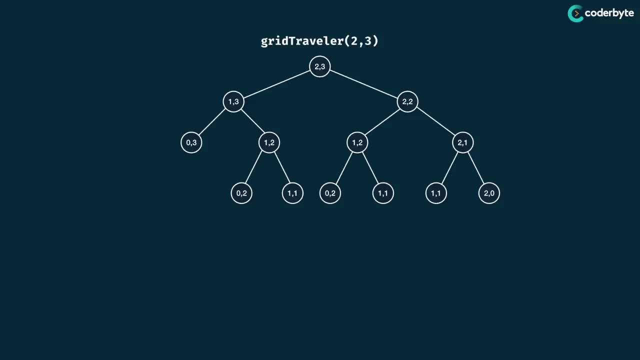 and really remind yourself of the actions we took in the Fibonacci problem and see if there's any patterns in this tree. Probably from the gate you notice that I have some duplicate sub trees. right, I have one comma two, So in these the two highlighted sub trees. 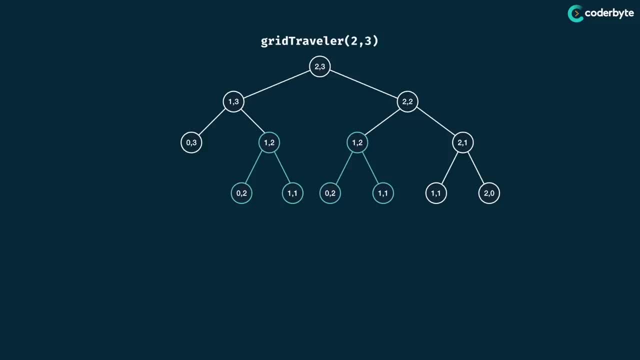 in blue. that's sort of asking the question: hey, what is the total number of ways I can travel through a one by two grid? That being said, I think there's even more sub trees that correspond to that particular problem. What if you look at this far right subtree? 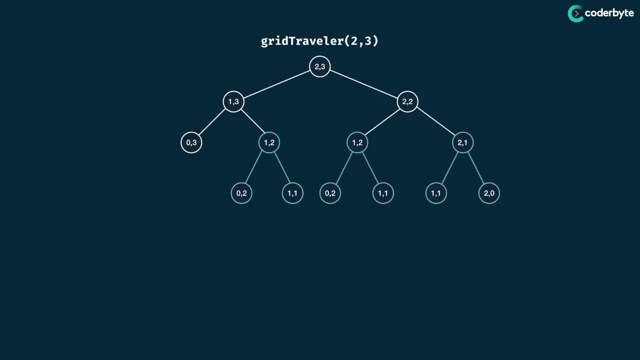 of two comma one. if you really really think about it, asking the number of ways to travel through a one by two grid is the same as the number of ways to travel through a two by one grid. you're just flipping the rows in the columns, but the total number of ways 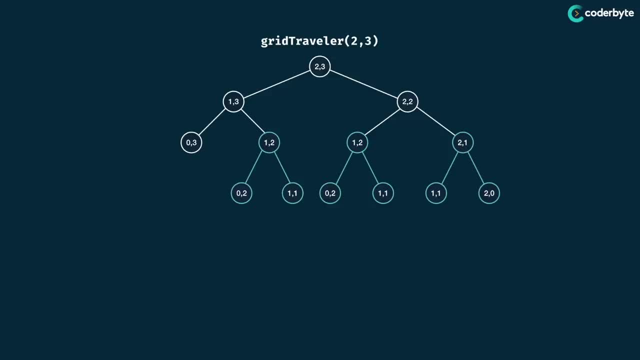 should be exactly the same. So that's actually a pretty interesting way you can optimize the solution. So I can still memorize it. That is, I have these duplicate sub problems. but possibly a really cool insight we can make in this problem is you can also sort. 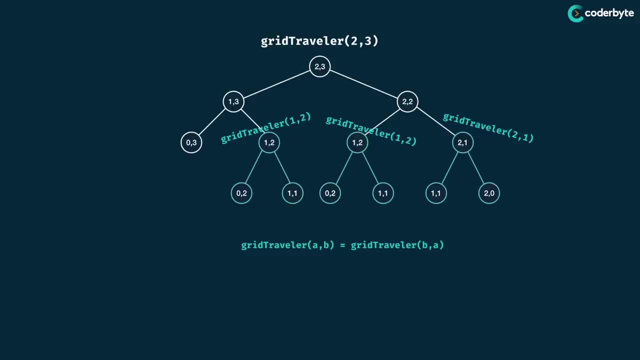 of flip the arguments. In other words, if someone asked you for grid traveler of a comma B, then that would be the same answer for a grid traveler of B comma a right. the order of the arguments technically doesn't matter here, And so we can totally encode that in. 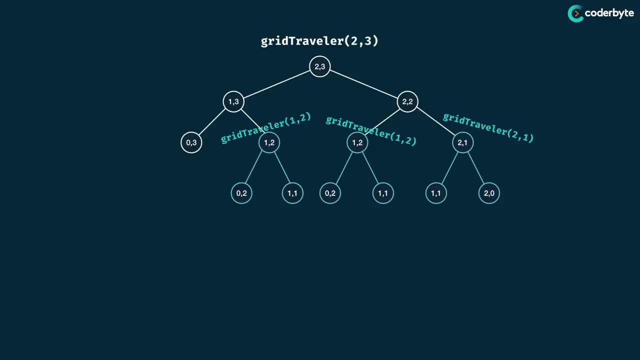 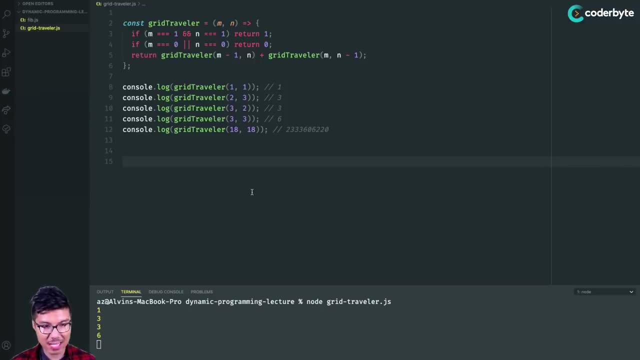 our memo object. That being said, punchline here is we better memo wise, this one, So I think let's hop to it. All right, here we are back in my text editor And hopefully that diagram of how we can improve the time complexity for this one makes some sense. Let me go ahead. 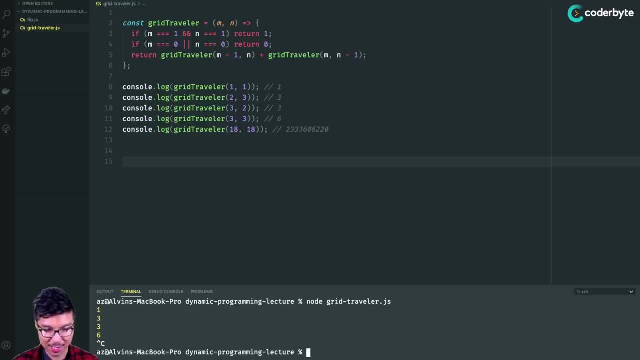 and kill this program still running, And my computer's fan is actually going crazy now is running the entire time. Let's go ahead and memo wise this one. So the beauty of you know, solving these dynamic programming like problems is if we have the initial strategy. 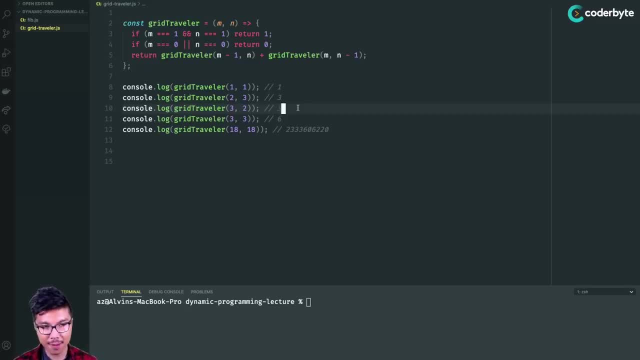 of implementing like the brute force recursion, and we wrote like a very well formed recursion, meaning that I actually use return values And I reconstruct the sub solutions all the way up to the tippy top, Because I have a really nice recursion here. memoization is a very like formulaic pattern, So it's going. 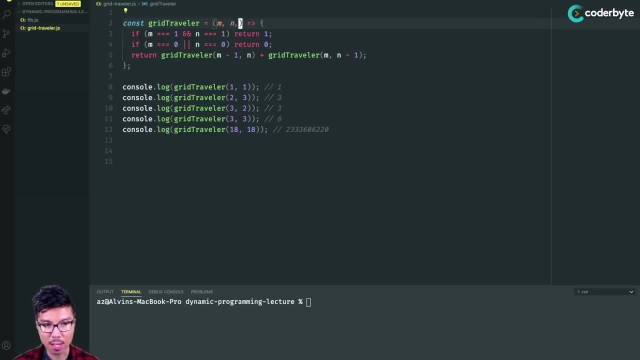 to be almost the same strategy we did of Fibonacci and even other problems that we do in this lesson. So we're going to bake in my default memo as an empty object And then along with that I'm going to add my memo checking logic. So I know over here in general, I need to. 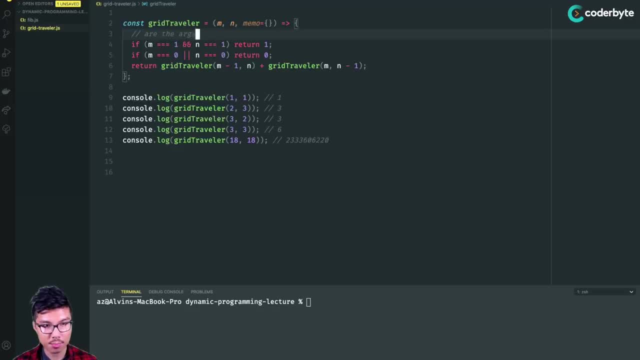 check. hey are the arguments in the memo right? I need to key into my memo object using all of the arguments. Now I have two arguments And since I have two arguments and since both of the arguments combined sort of dictate the output, I need a key that. 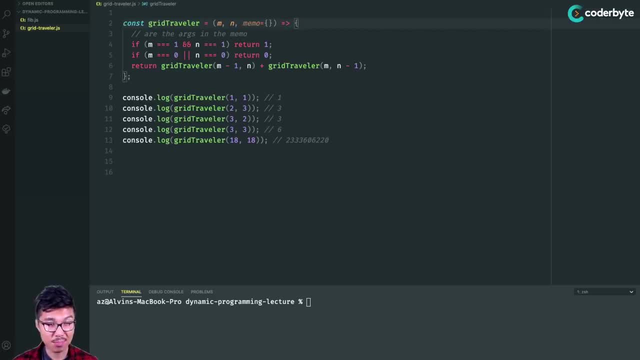 sort of contains both of those. in JavaScript, the keys are either strings or symbols. So for us right now, really, strings is the most irrelevant one. So what I'll do is I'll concatenate both of these integers together. That way I have a 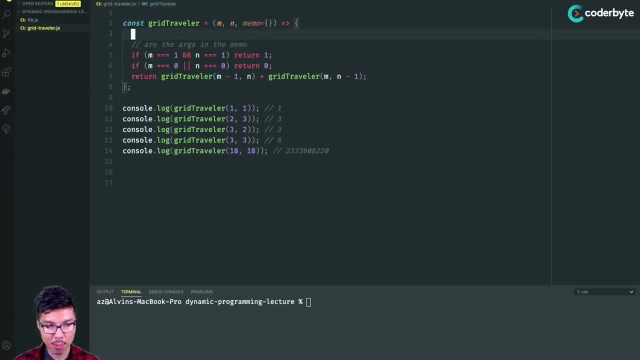 string which I can key into the object with, And what I'll definitely want to do is also maybe separate them with a comma. let's say so. I'll say let key equals m plus a comma plus n, And the reason that you'd probably want, like some sort of separator between these. 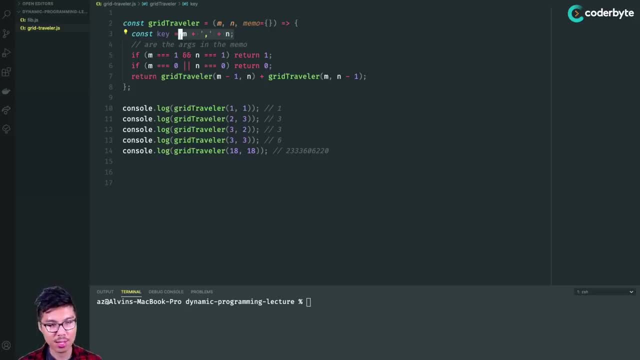 two arguments in your key is to make sure the numbers don't get misinterpreted. So I've actually ran into this issue in the past. Can you imagine like if I had a scenario where, let's say m was 42. And then we'll say n was the number three? So what? I don't want to. 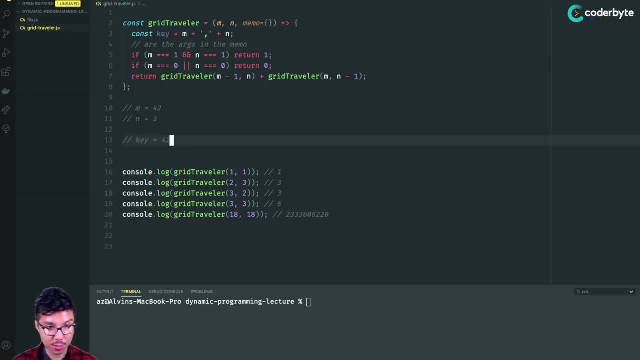 do is just make my key something like 423.. Because this isn't going to uniquely identify the exact input argument. right? Because if this was just my key, then I guess I have the same key for a totally separate set of arguments. If I gave you four and 23,, right? 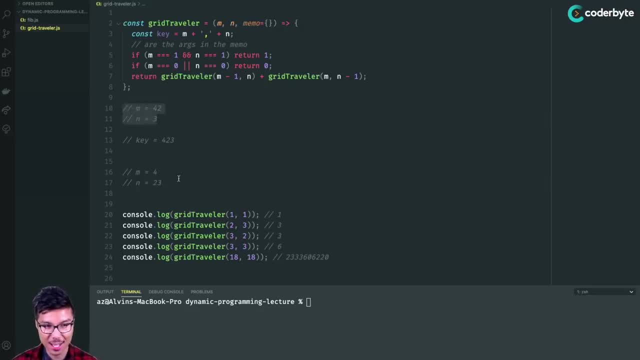 both of these combinations of very different arguments would lead to the same key. they would collide the same key. So instead I'll prefer to put a comma between them right now. I know, know without a doubt, that this key corresponds to four comma 23,. right, So that's why I put a. 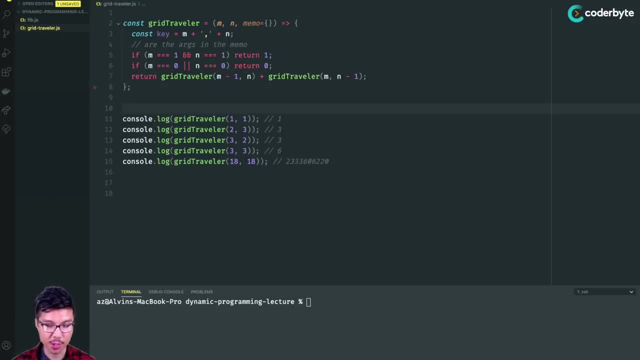 separator between them And, depending on the language that you know you're choosing for interviews, you can find a very similar construct. Cool, So now I'll go ahead and check. hey, if my key is in the memo, then I have the result cache already, So I could just return that cache. 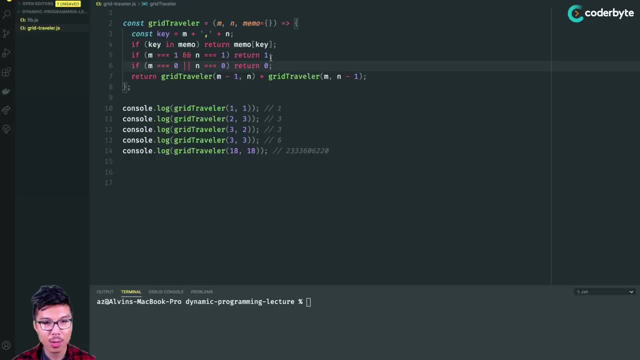 value. So return memo at key And then what I want to do is look for my old return value, right? So here's where I actually do the manual recursive calculation. Before I return that, I want to store it in my memo using the same key and then return that thing I just put in the memo. just completing. 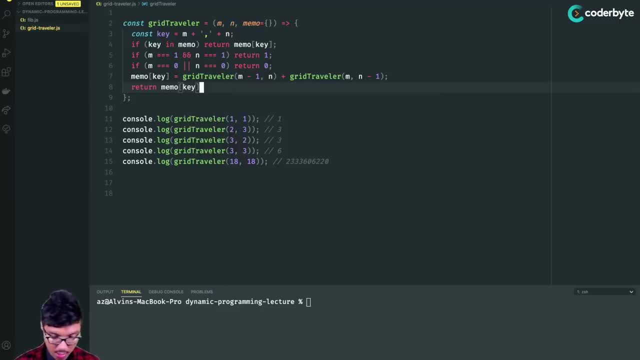 the old return logic, Cool. So you've seen this pattern before. I just want to emphasize a few things. Now it's the second time we're seeing it. memoization, for me at least, is a very, very formulaic thing, right? So I always take the exact expression that I returned previously. 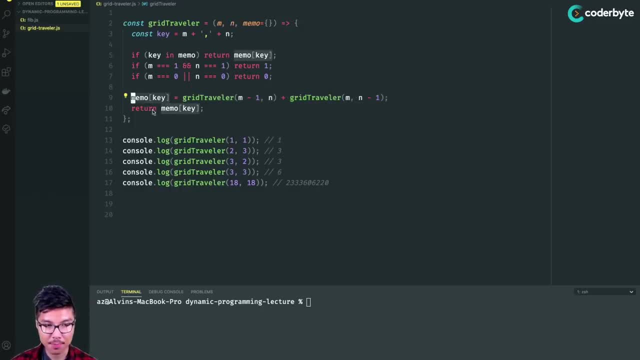 and I put that entire thing in the memo. object: Right: Notice that my key encodes the arguments for this function: right, m and n. something that I've seen students do in the past is do like very heavy handed logic where they try to you know. 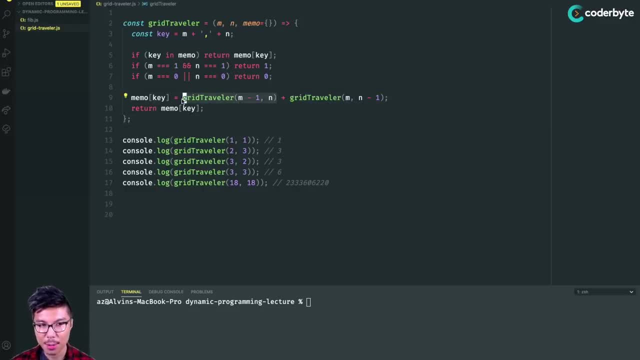 check if the child call is in the memo. In other words, don't write any preemptive logic where you check: hey, if you know m minus one comma n. so if you like, concatenate those two things together, don't check, if like your child's key. 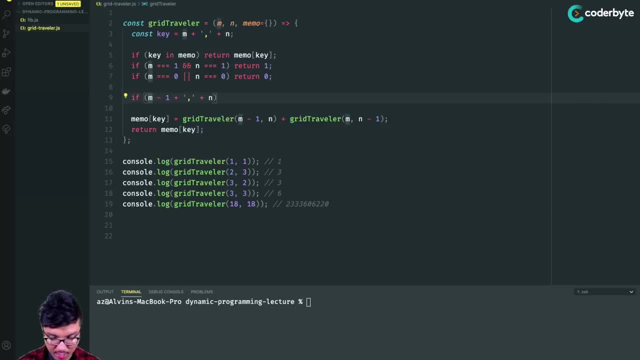 is in the memo, right? So imagine like: this is my key right now. Right, Don't check if that is in the memo. When you write logic like that, it ends up being very, very duplicate and a little harder to debug, right? Instead of writing your function as if it's, you know reasoning for its children. 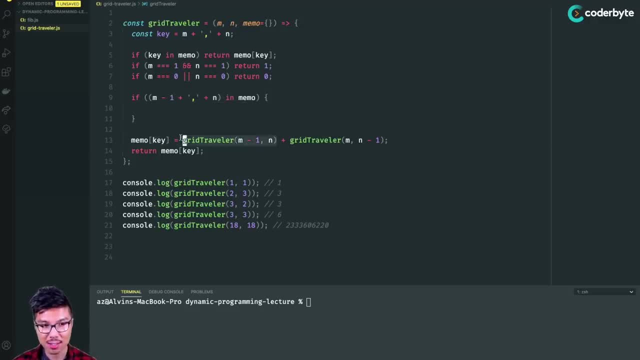 calls. you know that once you actually evaluate those child calls, they're going to cache themselves, right? They're eventually going to check this if statement anyway, right? So don't do any of like the look before you leap logic. just make the request and then you're good to go. 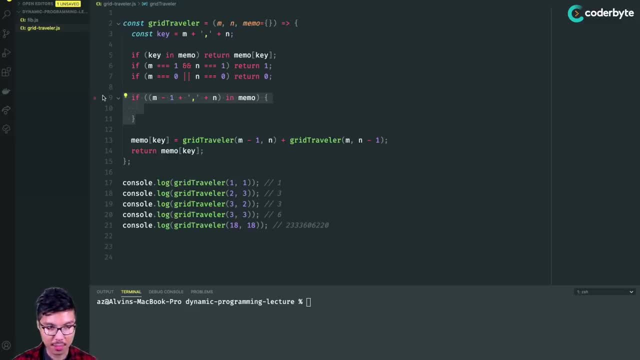 So let's go ahead and run this code, So I'll give this a shot. grid traveler, I still have that 18 by 18 grid, which took way too long last time didn't actually finish while I was waiting. Looks like I'm still hanging here because I'm actually missing a little bit in my code, So take a moment. 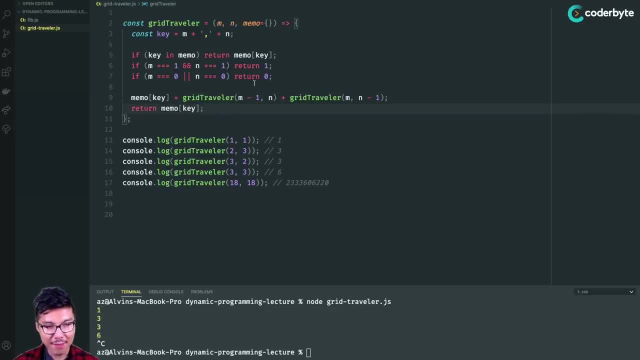 see if you can spot it. I forgot one really important thing. So I have the logic of checking if my key exists in the memo And I also have the logic of checking if my key exists in the memo. So if I'm storing something in my memo if the key doesn't exist. but what I failed to do was 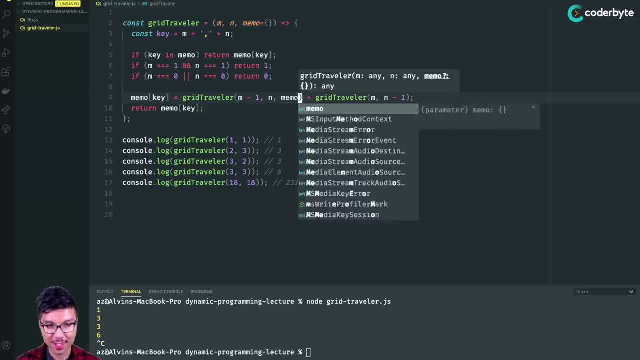 actually pass down the memo. object to all of the recursive calls. I want to pass it down over here. Remember the trick is only top level. when someone calls like two comma three for grid traveler, then we're going to initialize a brand new empty object which will be shared for the rest of the 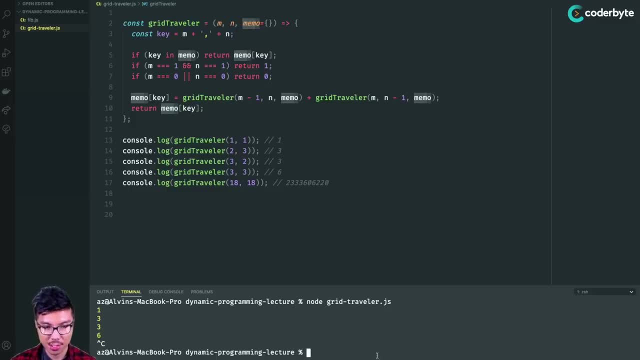 recursion, because it's passed down by reference at this point, So that's a common mistake. Let's go ahead and run this now. Nice, And there we have it. Look how quick our last execution was over here, And that is the expected answer for an 18 by 18 grid. Cool, So here's what. 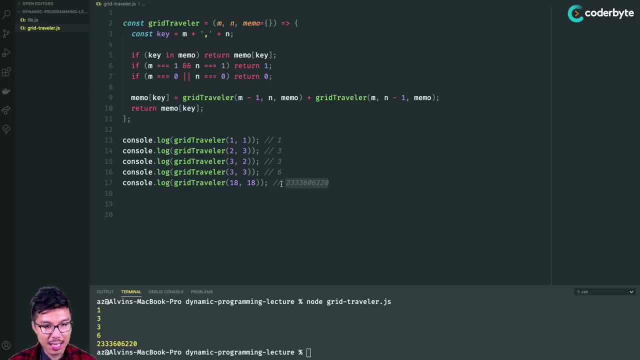 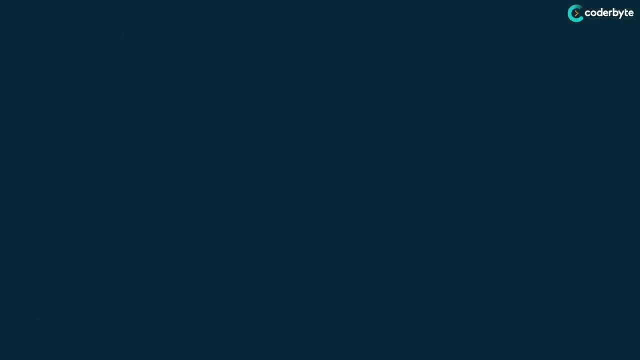 we'll do. It's evident that we definitely sped up the execution of this one. Let's head back the drawing board to wrap up this problem and really see how we cut down the complexity here. All right, so it looks like we definitely improved the runtime of our function, But I want to really 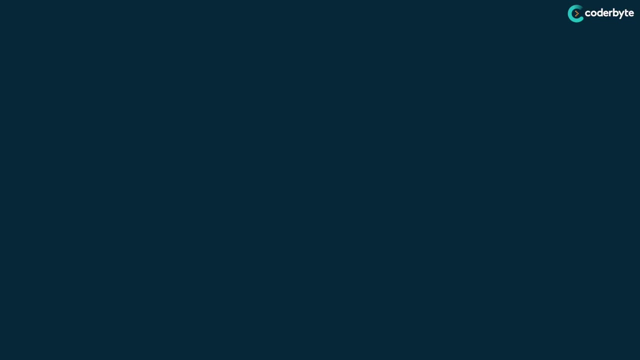 understand. you know what the big O complexity of our improved function is now So sort of a way we can structurally argue for what the new time complexity is Is to think about. you know what are the values of the nodes that we'll actually have to travel? 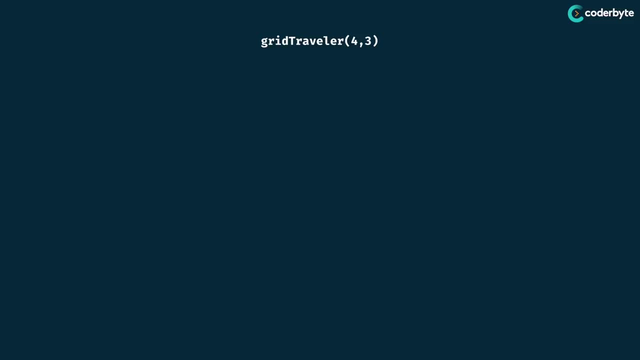 through. So let's say I looked at this example. I wanted to find the number of ways to travel through a four by three grid. I know in general there'd be a top level node of, of course, four comma three, But in general that refers to m n right. So I'm trying to think in a very general. 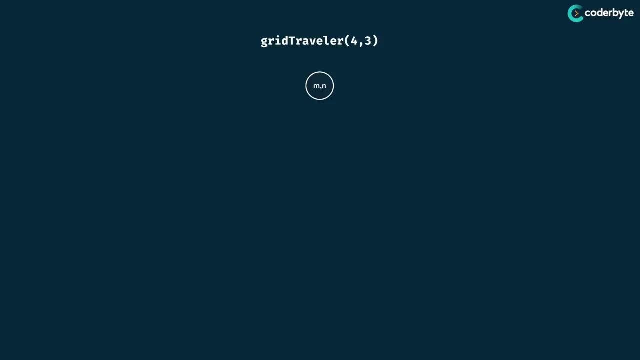 way right now, And so I know, when it comes to the other nodes of this tree, they're all going to sort of at most be four comma three, but then probably be less than that. right. They have like a range of values for the nodes. It's not as if to 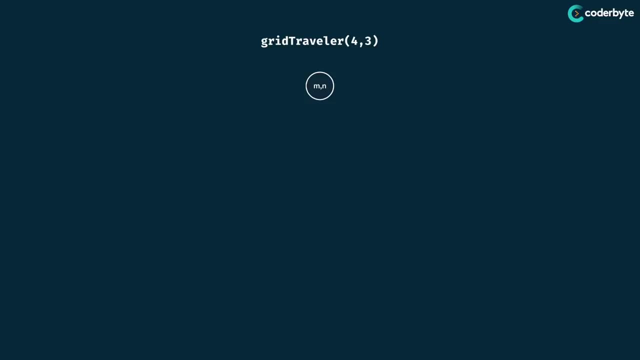 solve grid traveler for three, I would have to solve five, three, right, that would be a larger grid, But that doesn't make sense here, right, I'm shrinking the sub problems only in this rendition of grid traveler, And so if I think about some possible values here, I know that if m is four, 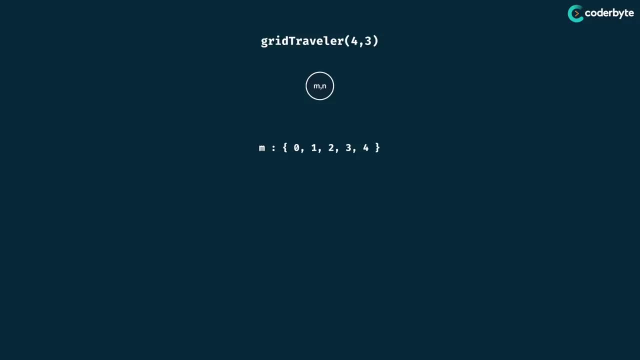 top level, then all of the values for m in the rest of the tree would be from zero all the way up to and including four. right, it's never going to be bigger than four. And a similar way of thinking. since n is three here, the only possible values for n and the rest of my tree are zero through. 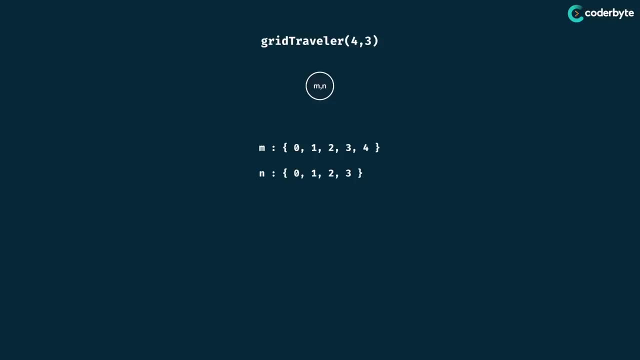 three right. So roughly. you know we're a little off by one here because I have to include zero, because we know that that's a base case in our rendition of this problem. But that being said, they're roughly m choices for the first number in the node and n choices for the second number in. 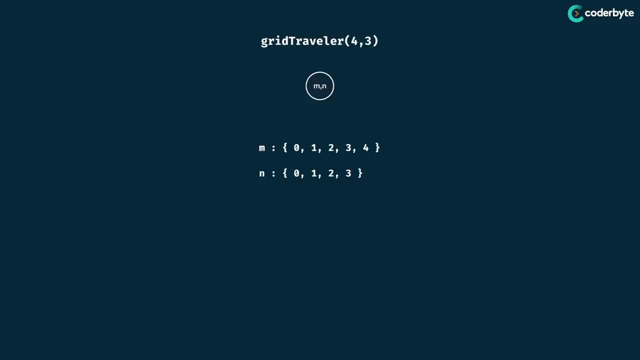 the node, And along with that, we know that we're not going to have to travel through many duplicate sub trees, because we memo wise them away, And so I think what I can say here is the total number of nodes you can possibly have. 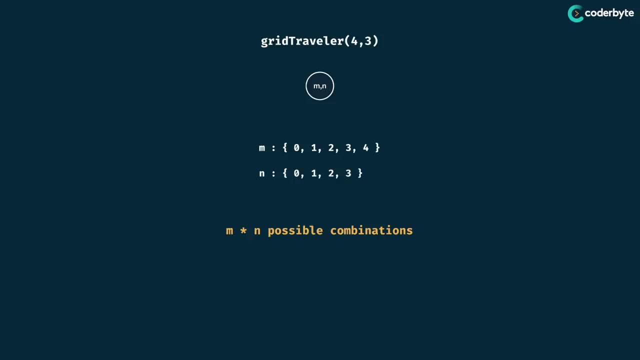 Is m times n and that'd be the number of like distinct nodes, right, Because I have m choices for the first number in the node and n choices for the second number And I know that I'm going to really minimize any duplicate exploration through the memo object. So they really the implication. 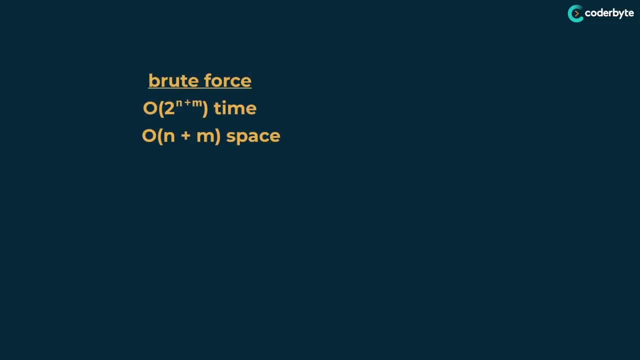 here is. we started out with our brute force recursive implementation, which looked like it was exponential in the time right. it was two to the n plus m time- And then, by memoizing this function, we were able to bring it down to an m times n time. complexity, which is much. 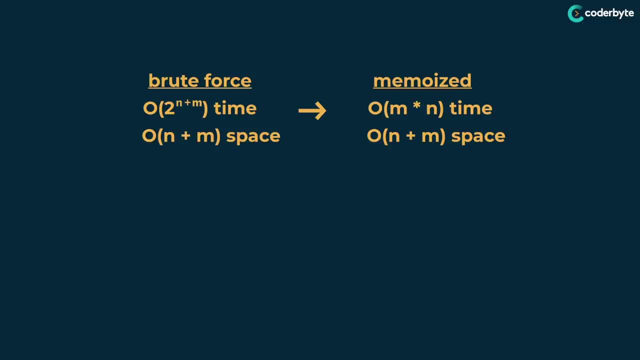 much faster. notice that the space complexity stays here, which is really fine, because n plus m is some sort of a multi linear function, Cool. So there we have our nice optimal solution for this grid traveler problem. So key thing I want you to take away from this one is: although the initial 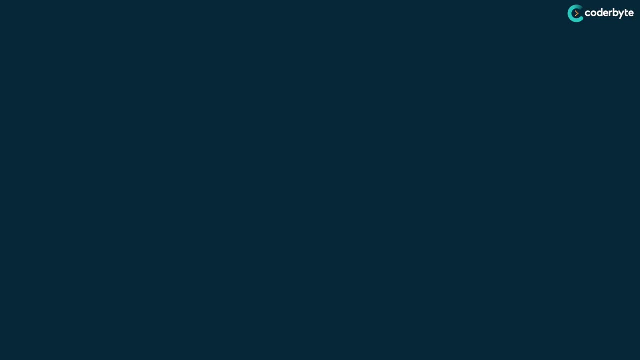 narrative in the problem made it seem, you know, pretty specific and pretty different from a previous dynamic programming problem like Fibonacci. it was really the same sort of story, the most important thing, that we're going to sort of leverage throughout this lesson, and we leverage. 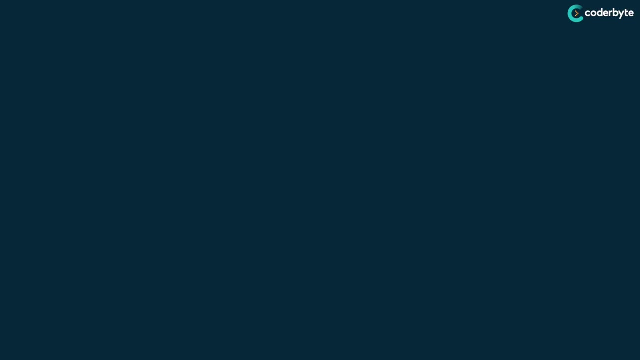 it in a lot of different ways. So the idea is: try to think about your recursive functions in terms of a tree. right, I get the most information out of the tree And then from there I can use that tree to not only implement a brute force, but to also recognize hey. 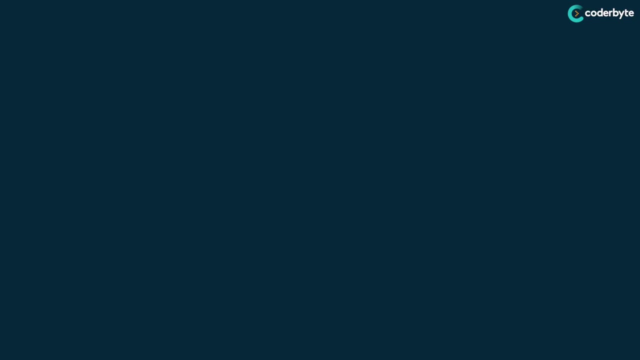 we're going to optimize this brute force. that way, you can reach for the optimal solution. Alright, so we've gone over two different problems together And hopefully we're starting to notice how we tackled them in similar ways. I think it's about time we give ourselves. 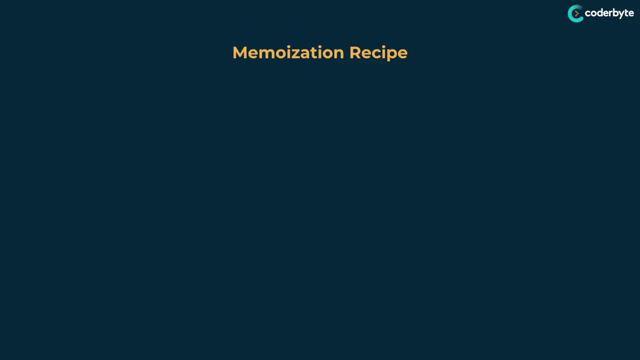 some guidelines for solving dynamic programming problems using a memo ization strategy- And we'll call this our memo ization recipe- And there are a few different ways you can go about learning this topic of memo ization And you might have different recommendations. 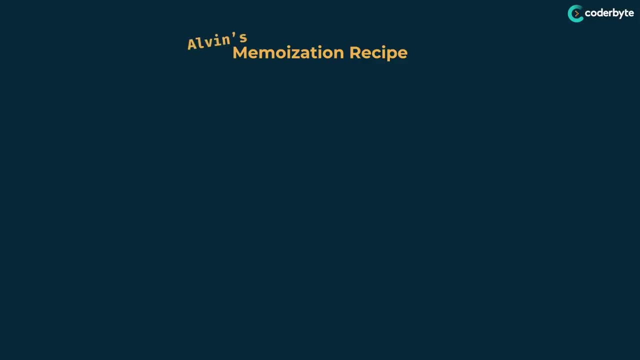 This is just my particular recommendation. So I think the most important thing to establish, if you want to, you know, solve some dynamic programming problem using memo ization, is to stick to two like high level steps. we definitely need to at first just have a solution. 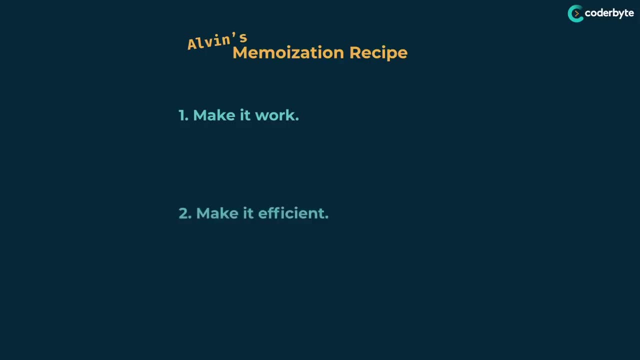 that's recursive. So just make it work. could be slow, that's okay, And then after that we make it efficient. I think this is where a lot of students sort of try to take the take on too much at once. they try to just solve it quickly all in one, go right To. 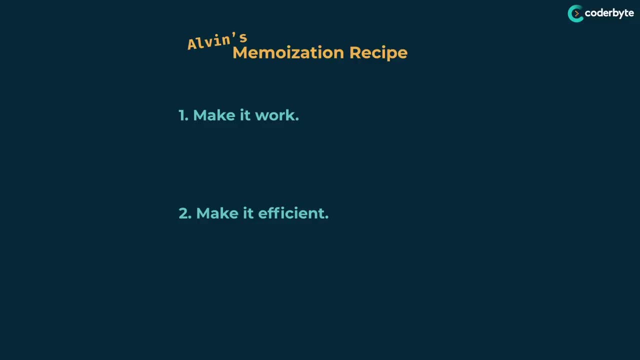 me it should be a very separate process, right? First I look for correctness in my solution And then, once I have correctness, then I look for efficiency in my solution. So when we go through step one, if I just want to get a working solution, then I have. 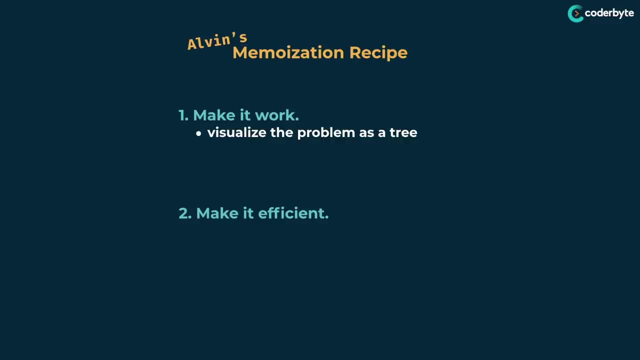 to start visualizing these problems as trees In dynamic programming problems. the gist of them are that we have some large problem that I can break down into smaller instances of the same problem. So when I visualize it as a tree, what I'm looking to do is figure out: all right in 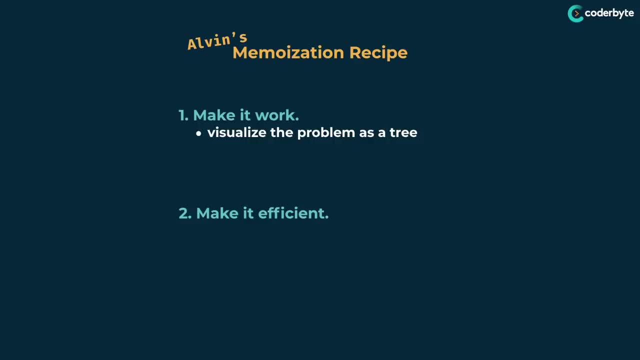 the nodes of the tree that should represent a problem And when I draw an edge between nodes, that should be shrinking the size of the problem. And depending on you know how your problem is stated, you'll have to figure out that logic, right, In the case of our. 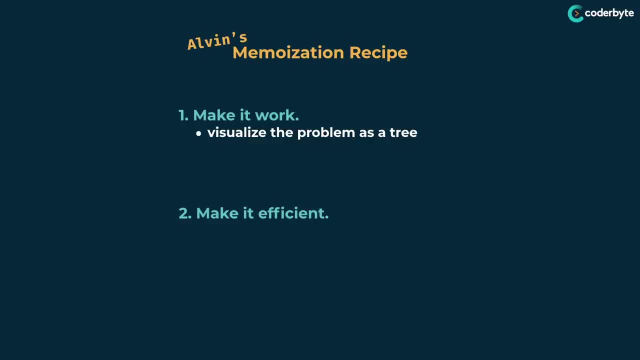 Fibonacci, it was as simple as we know: we can decrement our values of n. But in the case of our grid traveler, what we had to do was travel rightward or downward, And in the case of Fibonacci, it was as simple as we know: we can decrement our values of n. 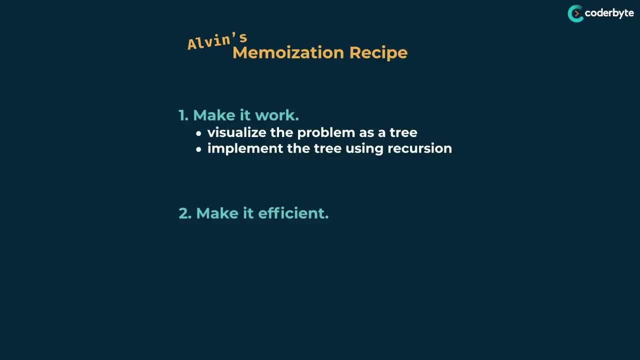 And once we do that, you want to implement that tree using recursion. What's great about a tree is it's already a recursive structure, right? So how do you start to translate that kind of tree visualization to some recursive code? Well, you think about the leaves of 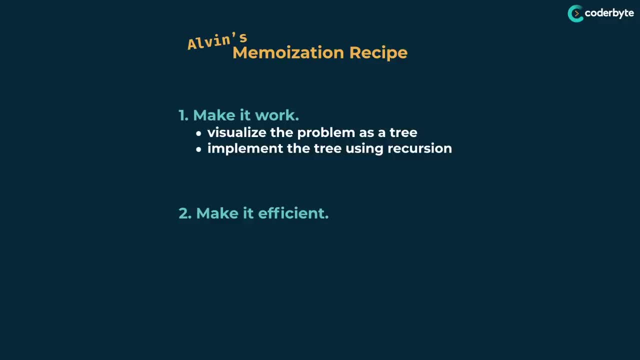 that tree as your base case. right Lately for us it's been about some small numbers, right, So like a grid of size one, or it could also be in the case of Fibonacci- just our initial seed values of n equals one and n equals two. Now, once you have that baseline, 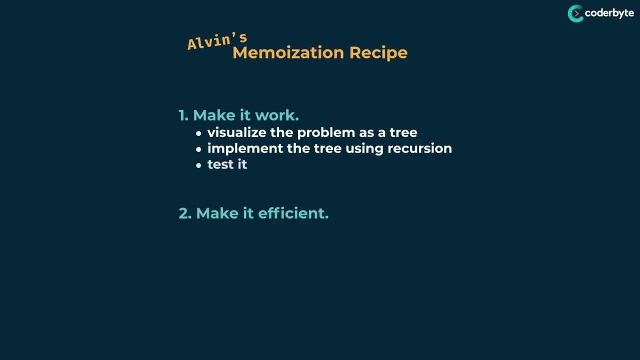 that baseline recursion. that's going to be your brute force solution, And so you'll want to test it. To me, this testing step is really important, right? So if you pass inputs into your brute force recursion, it should give correct answers, although possibly for large. 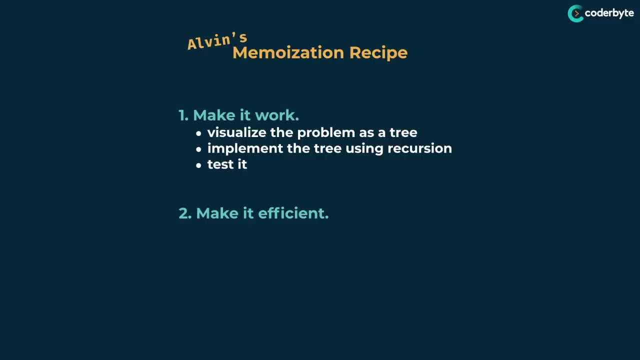 inputs, it may take a long time, right. To me, there's a big difference between code that is slow and code that is wrong, right? So here we should give back valid results, although maybe our code is a little slow. Now, once we have our working brute force, solution, making it efficient. using memoization, we're going to be able to do a lot of things that we don't want to do. So we're going to be able to do a lot of things that we don't want to make. awesome when we're starting to build workingстран And ourômultession. 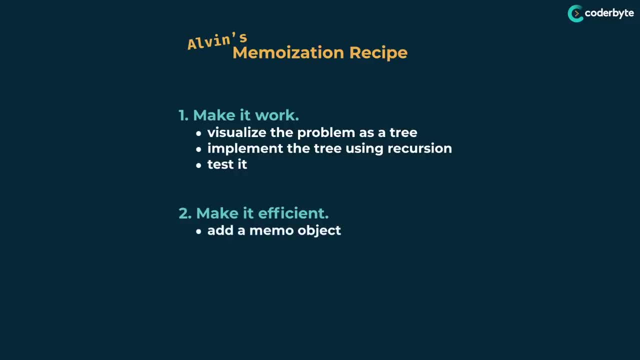 is a very, very canned scenario. All we do is start by adding a memo object into the mix. So this memo object needs to have keys which represent arguments to our function And the values of that object to represent the return values for those function calls. 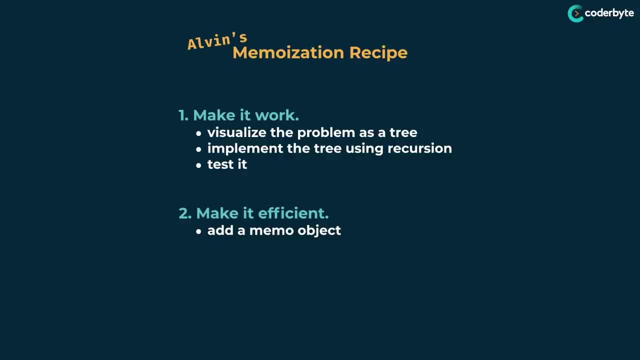 We know that in our functions a unique set of arguments should give me a particular results or just having that sort of mapping inside of an object. You need to make sure that this object is shared among all of your recursive calls. one way you can do that is to pass them along as arguments, And lately I've been doing. 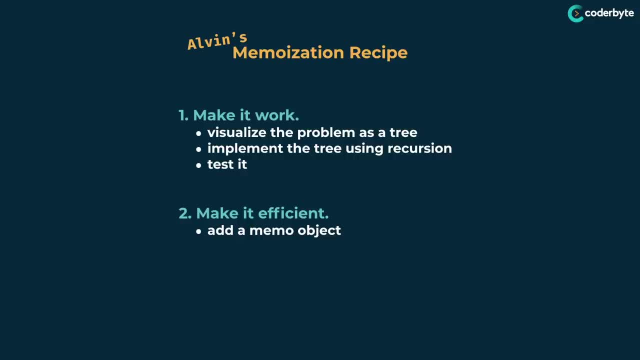 that by giving myself a default empty object at the top of each of my recursive calls right through my top level call. Once we do that, we need to add a new base case into our code. So I'm not going to remove any of the old base cases from my brute force solution to. 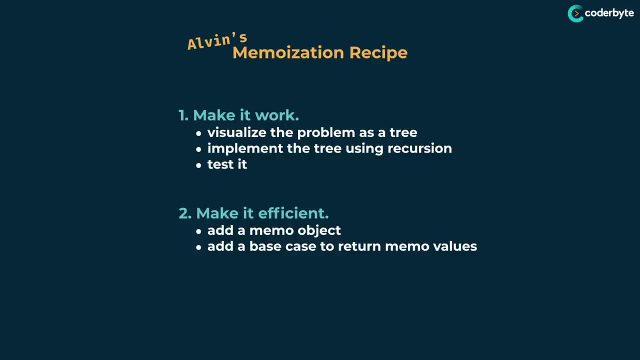 me. I'm just adding a new base case that captures the memo. In other words, if my arguments are in the memo object as a key, then I'll return the stored value. I refer to that as like my memo fetching logic right, looking up some stored value in my memo And beyond. 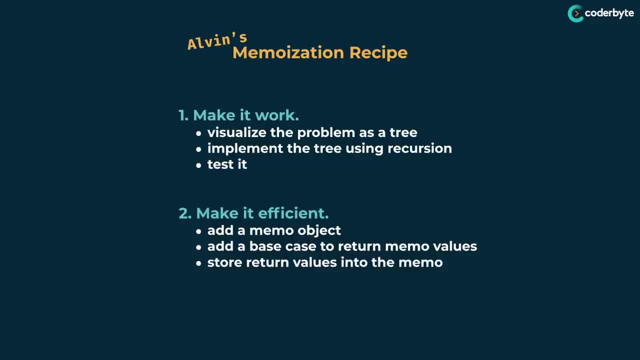 that the only thing we need to do is implement our memo storing logic, And it's as simple as going to exactly where we had our return values in our function And then we just make sure that we add those return values into our memo object before returning, right. So 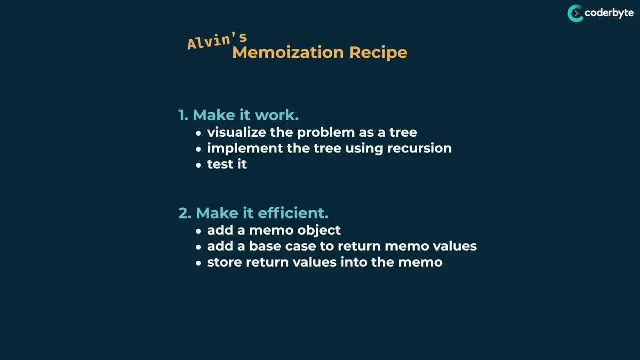 I always look to the exact return expression And just write some code around it, right, storing that result into another memo object before I return it right. Step two is actually very, very easy to implement, meaning it's very easy to memoize a brute force solution. it's really coming up with the brute force. 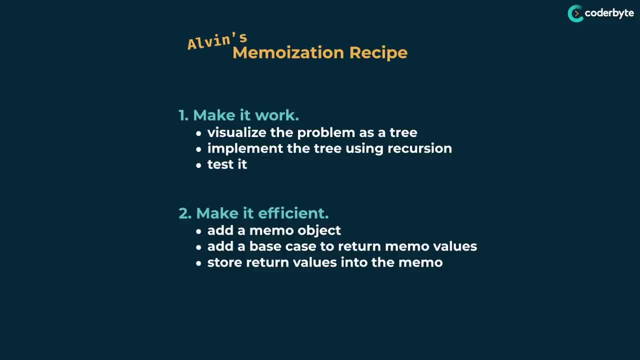 in the first place, that kind of feels more difficult. So as you're learning and practicing memo ization for these dynamic programming problems, I highly highly recommend you stay very methodical and follow these steps right. Don't try to efficiently implement an algorithm from the get go. get a brute force working solution. 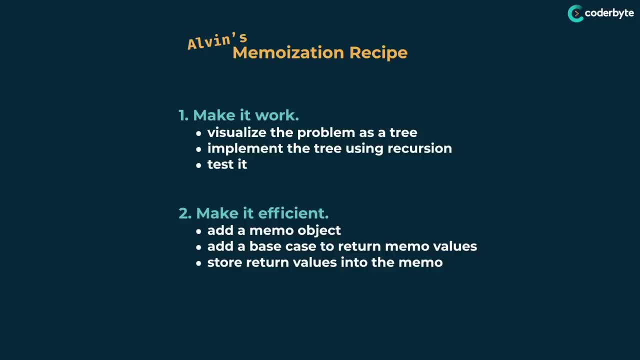 with recursion and then implement it using memo ization afterwards. right, And as you get more practice with this technique, soon you'll be able to do everything all in one swoop, But I don't recommend that until you've definitely finished this course. So we'll. 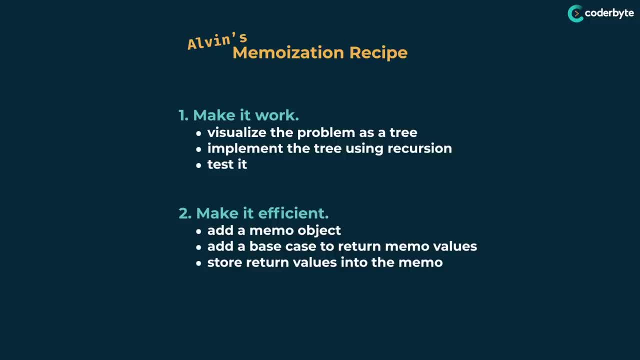 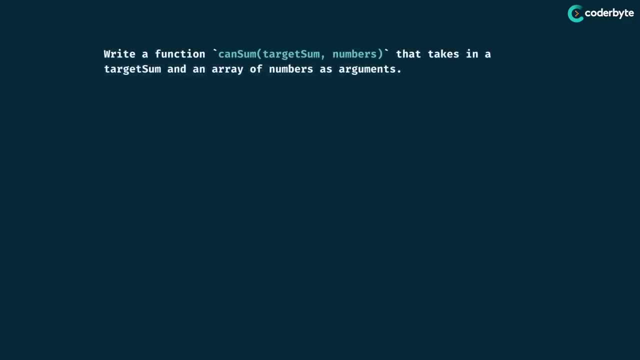 be sure to follow these rules for our following problems. Alright, so I think it's time to increase the difficulty and work on another dynamic programming problem. So let's go on the scale. While we're at this, let's continue with the next case. right? So we've been testing. 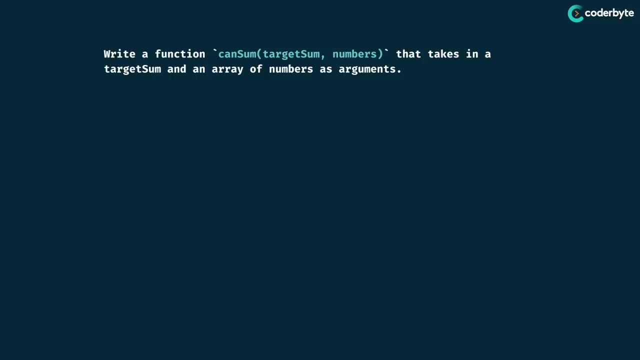 out this and we've been using other logic that we're using for this case, but we're going to try and solve this problem with someuranjs. So let's wait here. It's just to see if we can do this. So let's start with our first thing. I'm going to call this exercise. we're going to do an array of array of numbers And as we're used to doing array of numbers, you can see, here I've already set up a function and it's going to set up an array of numbers. here, What I need to do is take in a target, some as an argument, as well as an array of. 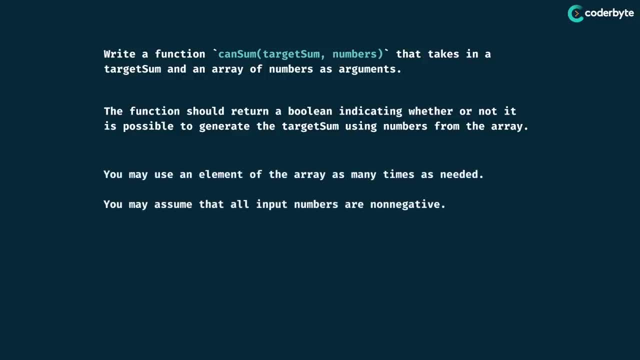 numbers. my function needs to return a boolean- So true or false- indicating whether or not it is possible to generate the target some using some numbers from the array Along. Along with that, we have some constraints here. we can totally use an element of the. 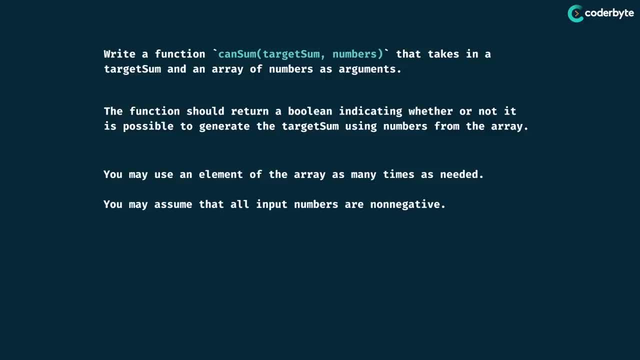 array as many times as we want, And we can also assume that all input numbers, so the target sum as well as the numbers of the array, are non negative. So let's try to understand what this question is asking. Let's say, I gave you this example case So it looks like. 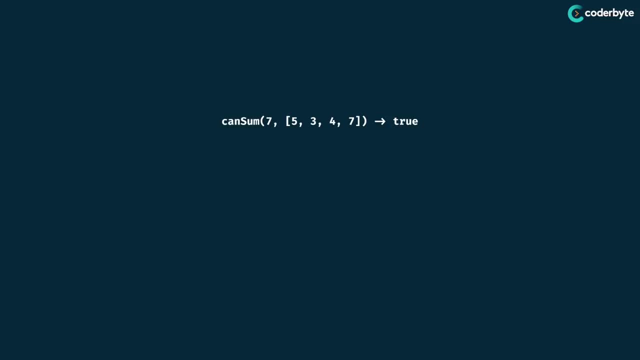 our target sum is seven and the array of numbers is 534 and seven. Here the response should be true, because it is possible to generate seven by adding some amounts of numbers from the array. One way you can generate seven is by just doing three plus four. Another. 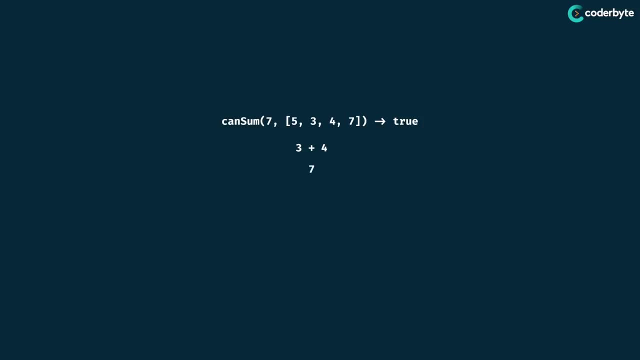 way would actually be to just take the lone seven, because seven is actually a member of the array. So it's definitely possible to generate seven using you know some amounts of numbers from the array. So that's why we return true. Let's say I gave you another. 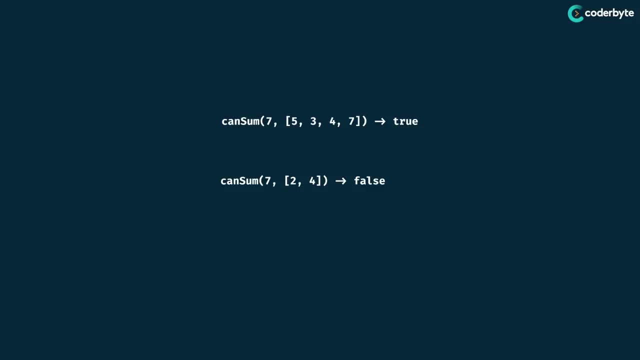 example, let's say I gave you a target sum of seven again, but I gave you a different array of just two and four. this is actually going to return false, because there is no possible way that combinations of two and four can actually sum to seven. 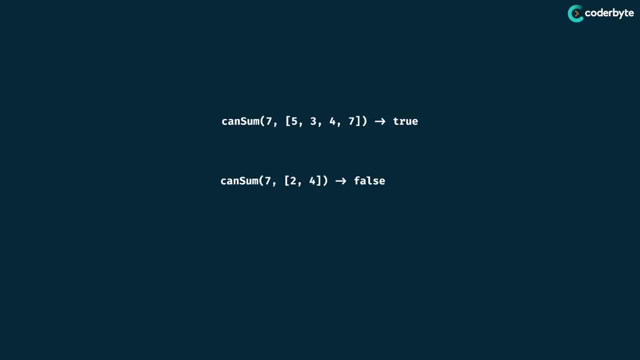 Cool. So that's really what the question is asking. Now let's try to think about how we can frame this problem of recursively right. Hopefully you've already gathered in your mind: if we have a smaller amount of target sum, then they'll tend to be a smaller or easier problem. 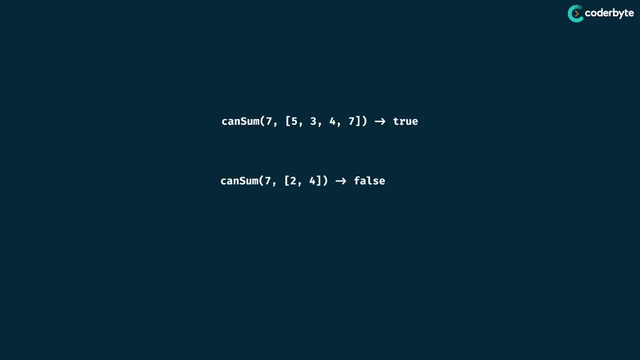 than a larger number for target sum. Alright, so let's start to think about the recursive structure. for the first example. we know in the long run we should be able to derive the answer true from this drawing that we make. So, like we always say, we should encode the arguments to our 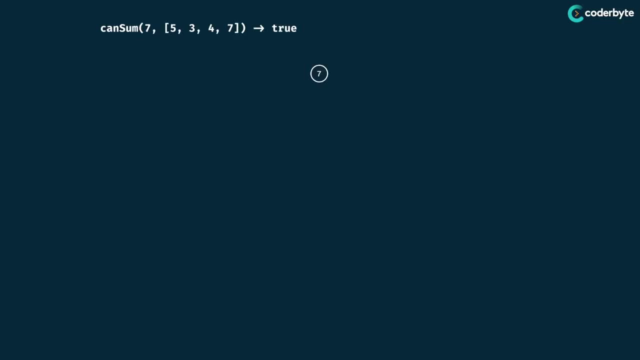 function into the nodes of our drawing. That being said, since in the problem they told us that we can reuse an element of the numbers array as many times as we need, I'm just going to omit that from the node drunk is basically every node or every function call is going to receive the 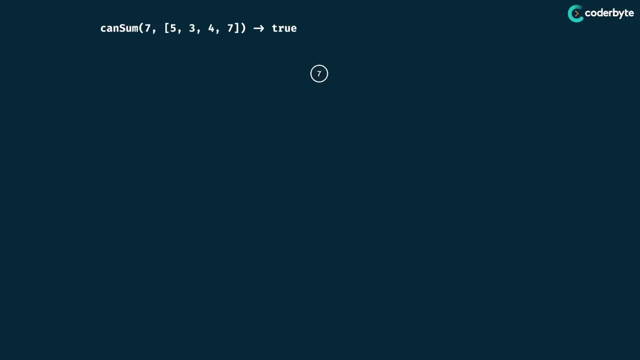 same array. So I'll just list the target sum in every node. So I start with seven and I have to think about how I can transition to other nodes. right, How can I shrink the size of this problem? Well, I know that I only have, you know, four options I can take, right, have an option. 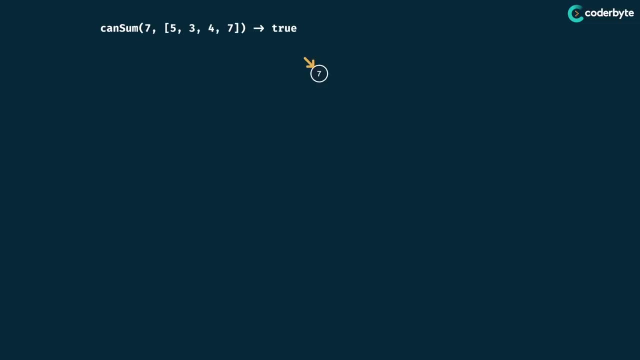 for every element of the array. So basically, if I'm at this seven node top level, I can branch to some children And sort of. the rule for my transition is you can either take a five, take a three, take a four or take a seven. And if I actually take, you know those elements as a 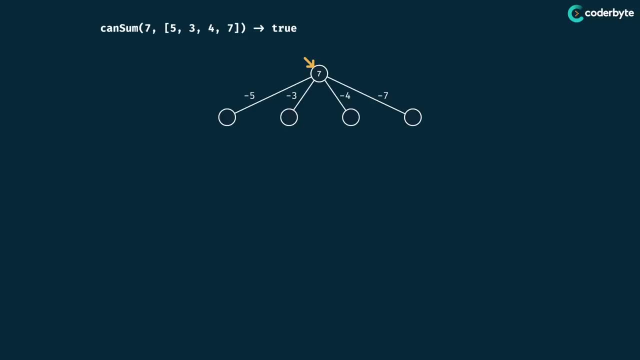 choice. they are going to decrease my current target sum. In other words, seven minus five is two, seven minus three is four, seven minus four is three And, of course, seven minus seven is zero. So notice, we have a very particular rule. 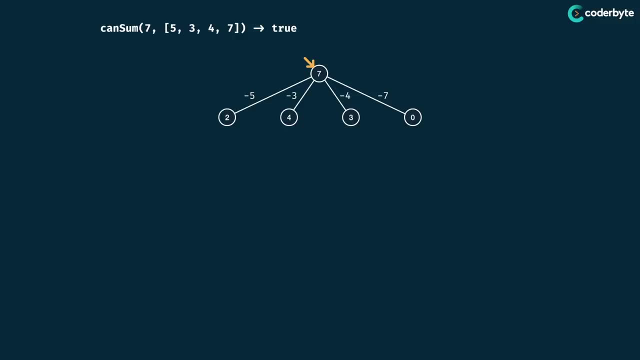 from traveling from a parent node to some child. I can just carry over this pattern. However, we have to watch out, right? So let's say I tried to flesh out this node where my target sum is two. if I look at the options, I have right. I still have the options of five, three, four and seven. 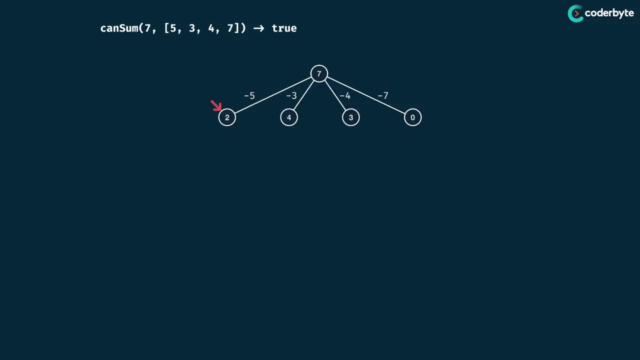 However, none of them are really compatible with this target sum of two. right, what I don't want to do is take any of these choices, because that would kind of give me a negative target sum. So I can't really flesh out this node two anymore, That is, there are no valid options for this node. 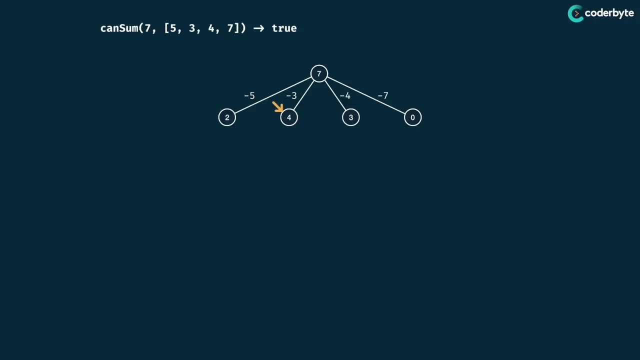 However, some of these other nodes, like this for a, do have valid options. So what I can do is take a three or take a four, and of course, I get a one and zero respectively, And I'll also do this for the three over here. right For this three node. 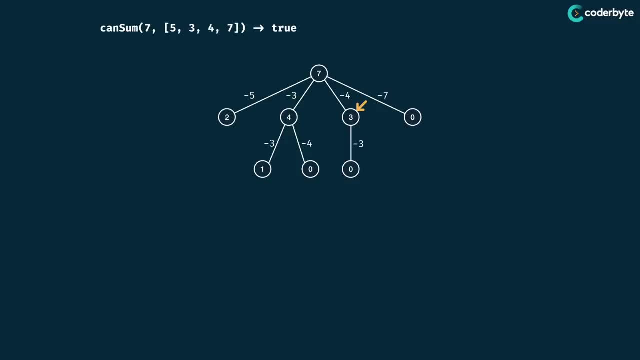 I can only take a minus three as a choice. Cool, If I look at all of the nodes that I have now I like the the leaf level. it looks like they all sort of bottom out at a base case, that is, there is no further choices we can take. And I also noticed that some of my nodes I have a 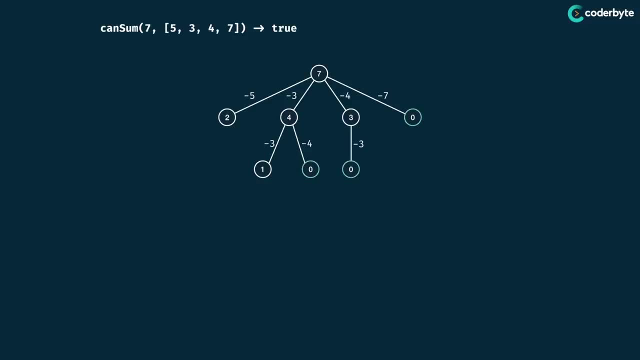 zero in them. If I look at the nodes that have a zero in them, they actually are a really nice base case because I basically have found that I can generate the original target sum right. A way you can kind of understand the base case when the target sum is zero is: 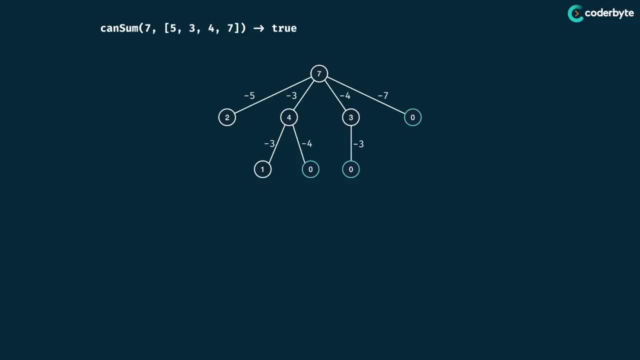 you can always generate a sum of zero by taking no elements from the array right. So these zero nodes are trivially solved And to me they should return a true backup to their parent right And sort of on the flip side for all of my nodes that. 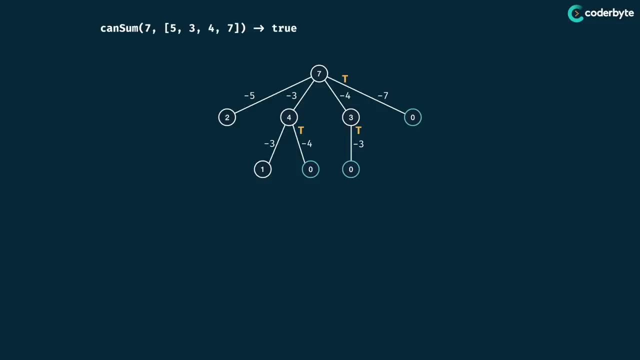 are not zero and they also can't break down into any further nodes. those return false right, Because I kind of have a leftover And I know there are no possible options I can take to reduce that further. So all of these other nodes should return false to their parent. 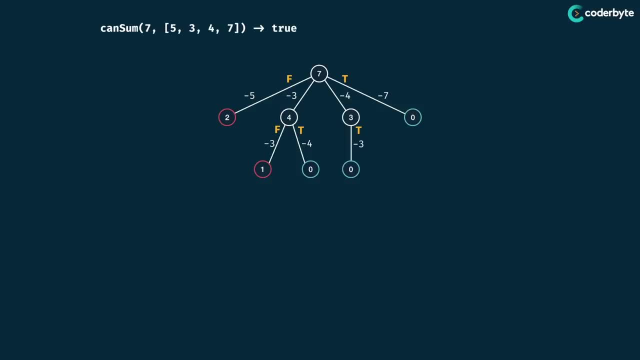 And remember what this question is asking. right, It's really asking: hey, is it possible at all to generate the original target sum? And so the logic is: when these values, these Boolean values, return to their parent, the parent should just check if at least one of them is true, And if at 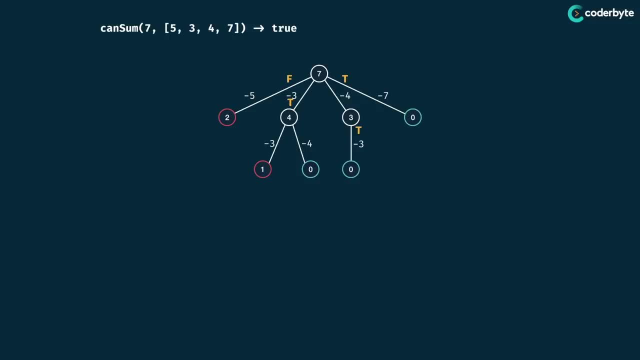 least one of them is true, then that parent should also return true, If I look at this, for node have a true above it, and that sort of answers the question. hey, can I generate a sum of four using elements of the array? and you totally can, because if you look at the elements of the array, 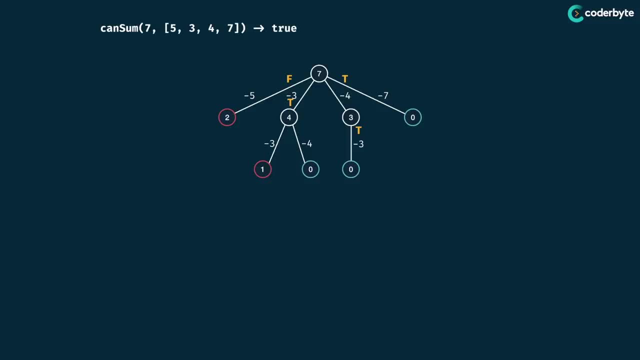 there is exactly one for, so I could just take that into my sum. So I'll be sure to bubble up, you know, all these Boolean values to their parent And again, the parent will just make sure that at least one of the values it gets back is true. 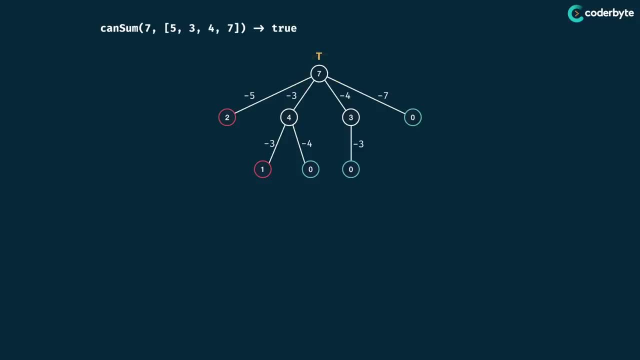 And so if at least one of them is true, then the parent itself will also return true. So very reminiscent of some like Fibonacci bubbling up pattern as well as our grid traveler, except now we're kind of adapting this for some Boolean data, but it's really the same structural understanding. 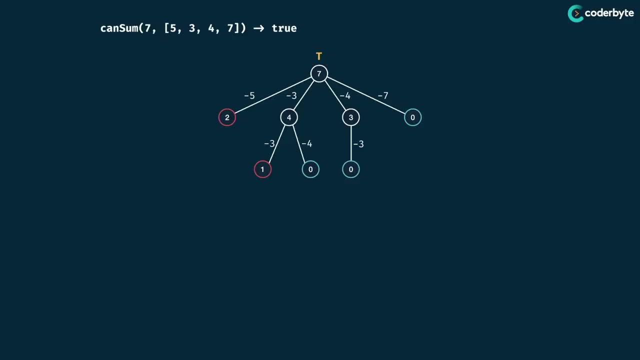 I have Cool. So that was an example where we said, true, right, there is a way to generate the sum. But let's look at another example. right, How do we know the flip side? So if we have this example, right, seven and an array of two, four, it's going to be true. So if we have this example, right seven and an array of two, four, it's going to be true. So if we have this example, right seven and an. 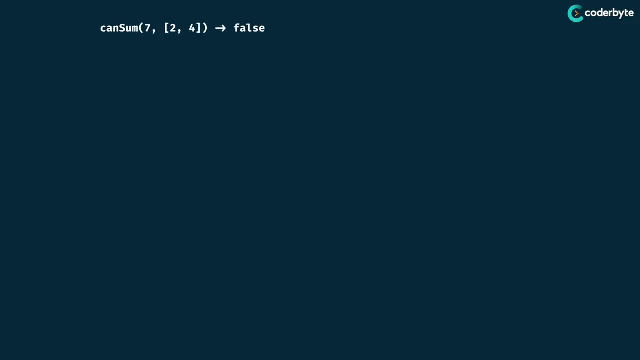 array of two four, it's going to be true. So if we have this example right- seven- and an array of two- four, in the long run that's going to return false right. there's no possible way you can generate. 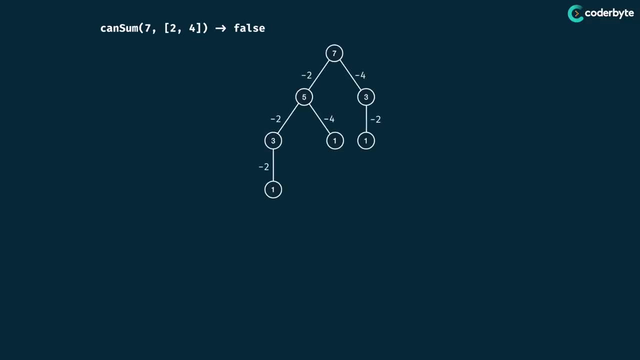 that target sum of seven. So the tree for this example would look like this. So this is a full tree. notice that all of the leaves get as low as one, but they can't be broken down any further. Like we just said in our last sketch, all of these ones, since they can't be broken down any. 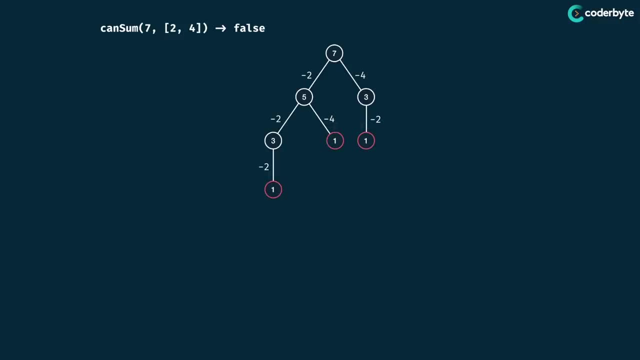 further and they haven't reached a zero, they're going to return a false up to the parent And I know that if I bubble up all of these false values, of course a top level call will also return false Right. So it looks like a key insight we have for this problem is if we find at least you know. 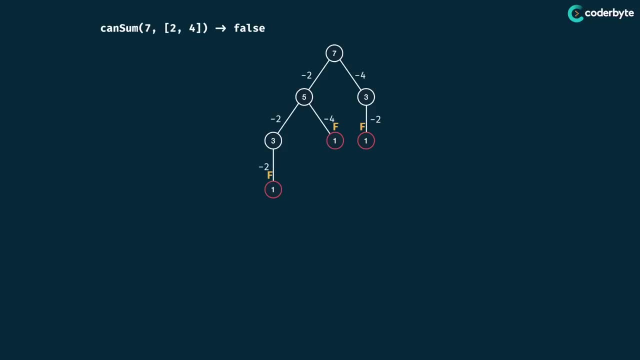 one base case that returns true. I know that I can sort of stop early and just return true all the way up to my parent, because they're not really asking, like, how many ways can you generate the target sum? They're just asking, hey, yes or no, can you generate the target sum at all? 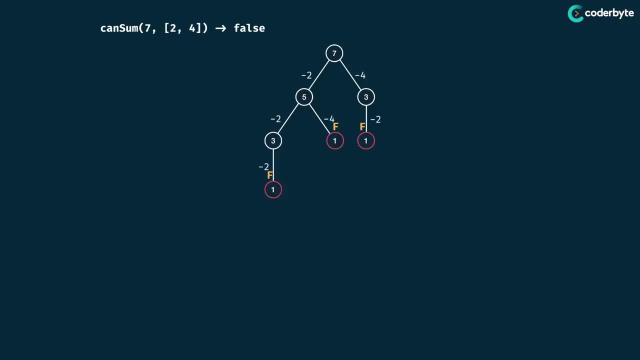 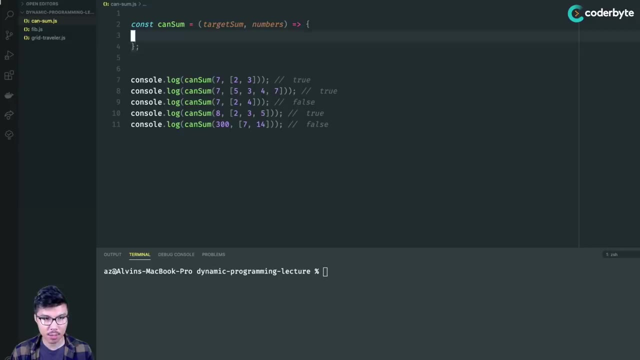 so that's going to be a really nice way to implement this code. I think we're ready to jump right into the code, So let's do it. Okay, so let's go ahead and implement this. can some function? So, since we're going to solve it recursively, I think a good starting place. 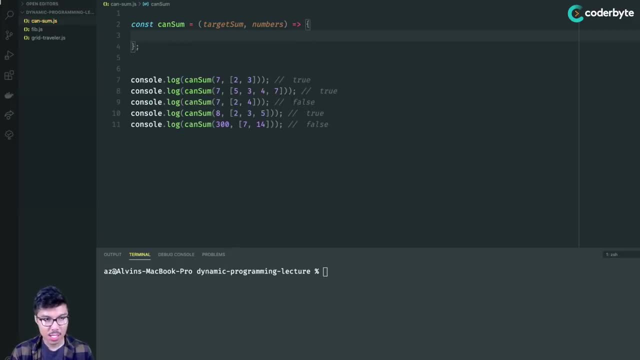 as always, is to maybe handle some of the base cases. So when we drew out the tree, I noticed that one of our base cases was when the target sum reaches the value zero. right, If our target sum is zero, then we have like basically trivially solve the problem, because 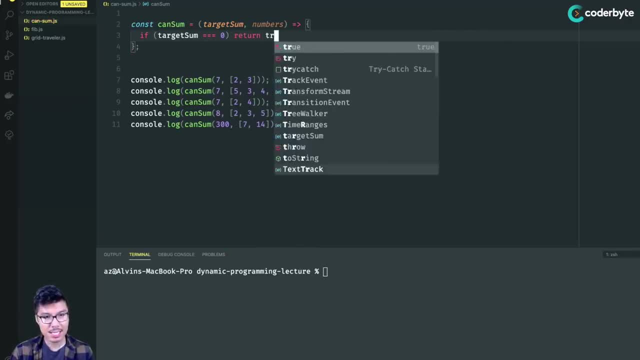 you can definitely always generate the target sum of zero by taking no numbers from the array, right? So I'm going to return, true, if ever I reach a zero. But apart from that, I think let's go ahead and do that. So let's go ahead and do that. So let's go ahead and do that, So let's go. 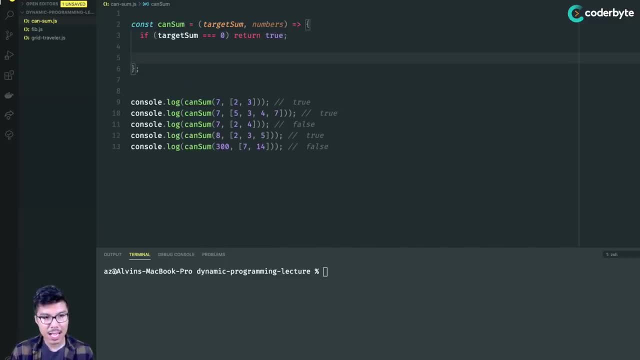 ahead and work on the recursive scenario. So I know that I need to establish some logic where I make a recursive call or a branch for every element of the numbers array. So what I'll do is I'll iterate through that array of numbers. So I'll use some for let of syntax. we'll say let. 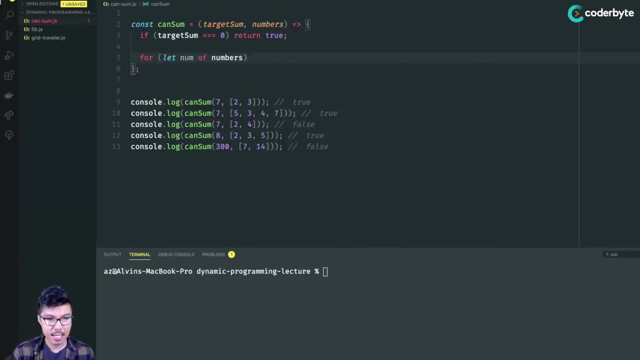 num of the numbers array. So if you're unfamiliar with the syntax, all it does is iterate through every element of the array. So, for example, let's say I just called the first example for can sum of seven and an array of two, three. 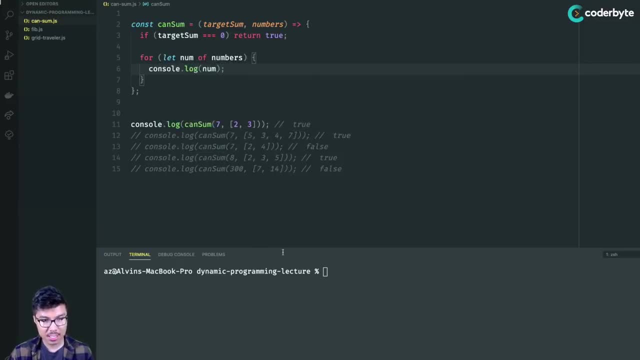 if I just console dot log the num, I'm just going to see the elements printed out of two, three, right? So I'll give this a quick spot check. Nice, So just iterating through every number of the array. no tricks here. But now that I have that number, I need the branching logic. 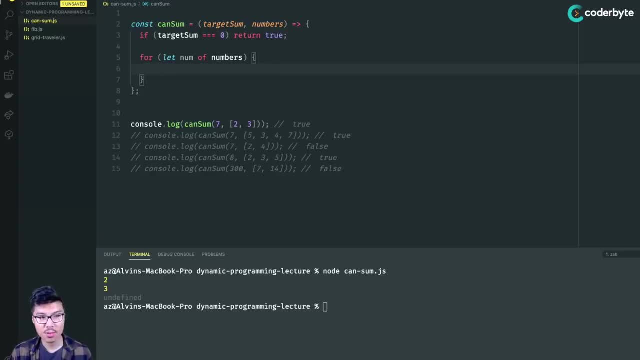 So remember the logic we use for transitioning from one node of the tree to the next. what we did was subtract our current choice of number from the target sum and they basically gave us, like the new target sum. So I'm going to express that. maybe some 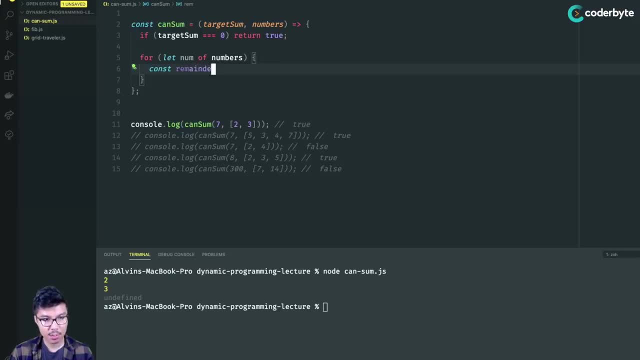 variables. So I'll say: all right, I'm going to generate the remainder by calculating the difference between the target sum and the number, right? So I'm just subtracting the number from my target sum. that gives me my new remainder, which becomes a target sum, right? So at this point I think I need to call recursively. 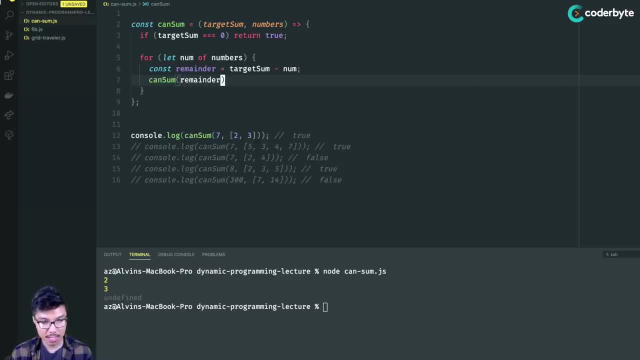 on can sum of. I'll pass in this remaining quantity. it doesn't need a second argument. still, I'm still going to pass in the same exact numbers array. So I'll still pass in numbers unchanged. I think that you know the fact that we pass. 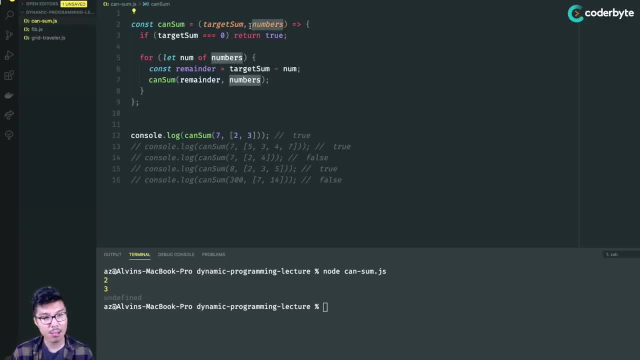 in the same exact numbers are right. it's pretty consistent with the way they stated the problem, because we can totally reuse the numbers of the array as many times as we like- Cool. So now that I'm using our function again, I'm making the recursive call. I want to think about. 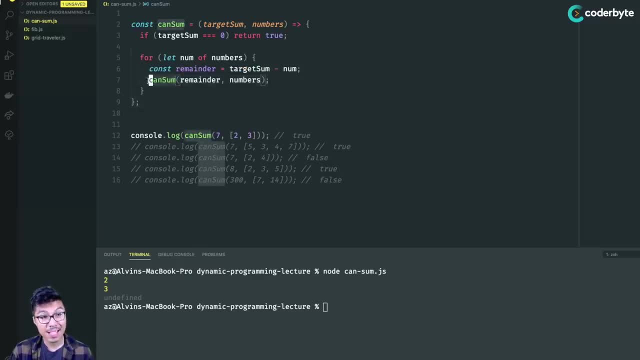 what this call will return. I know at any point in time my can sum function is going to return Boolean, And what's great about Boolean data is there's only two possibilities, right, It's either true or false. So I think, based on what we said about the tree was, if this call, if that, 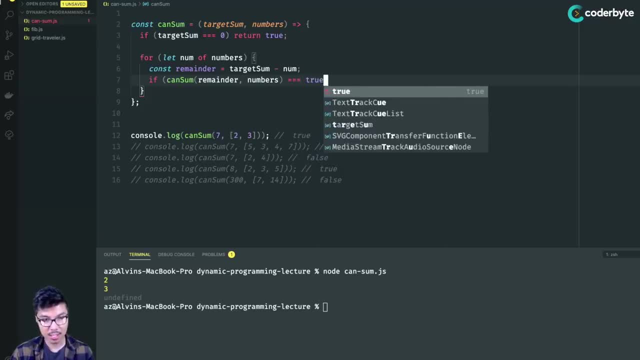 returns true, then I can just ultimately respond with a true right now. So we'll write it like this. So this is saying: alright, if we figure out that it is possible to generate the remainder using numbers of the array, then I can return true for this larger problem of target sum. 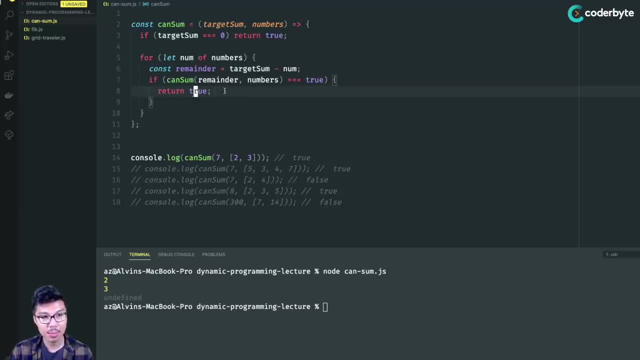 Right. So if I find at least one way that works out, then I'm going to do an early return true. And the really important pattern here is we don't want to write the else, then return false. Instead, we'll want to return false after the for loop. So here's the reason. 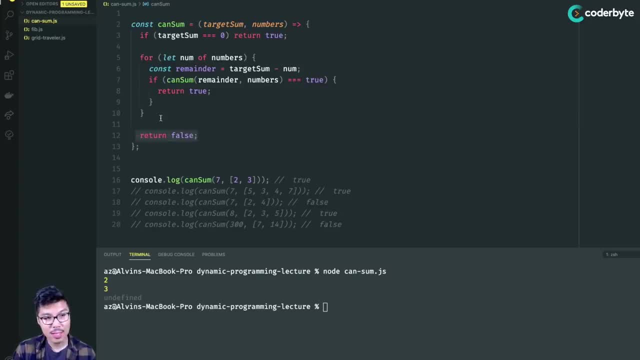 why we want to return false after the for loop. I only know that after I attempted. you know all possibilities and I found that none of them worked out. can I actually say that it is impossible to generate the target sum right? so I need to make sure that this for loop tries. 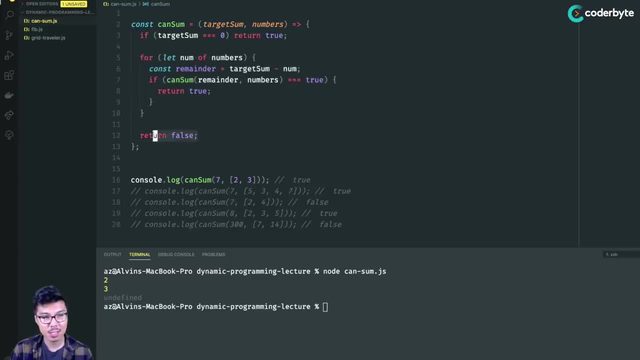 all possibilities of number Before I can say false, the target sum cannot be generated. That being said, there's one thing we should add to our code. So if you look at line six right, I'm subtracting our choice of num from the target sum, And that means that sometimes the 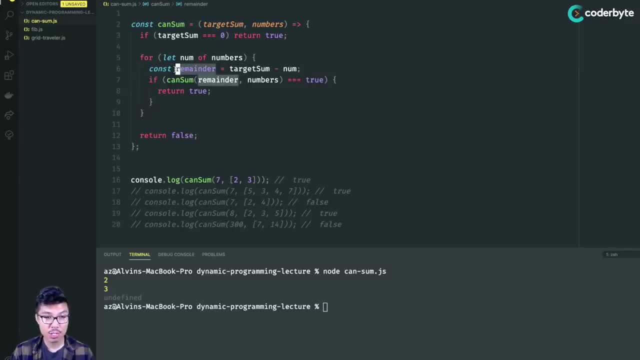 remainder might become negative. So, remembering our tree structure, we made sure to sort of return a false whenever we had some node that didn't do any branching To kind of account for that I can kind of bake that into another base case, But this time make sure it doesn't return true. 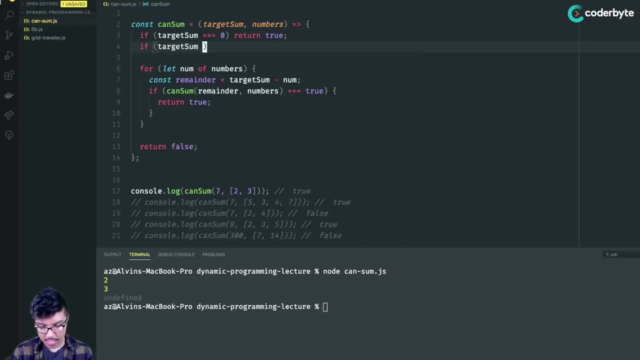 So I'll say: you know, if my target sum is negative, so if it's less than zero, then you've gone too far and you can just return false. Here it's safe to just automatically return false if your target sum 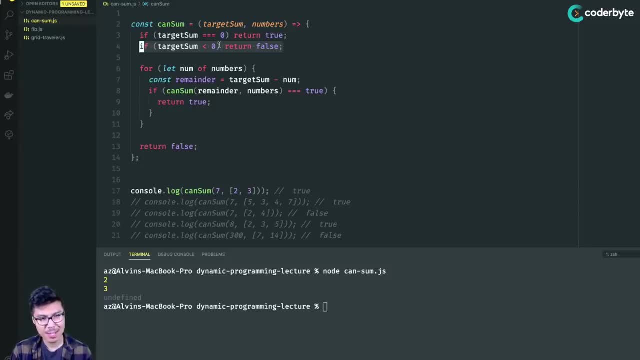 hits something less than zero because you've gone too far And there's really nothing else you can add from the numbers array to ever fix that negative target sum. Remember they told us in the problem that your numbers are always going to, provided as positive numbers or just zero, right? 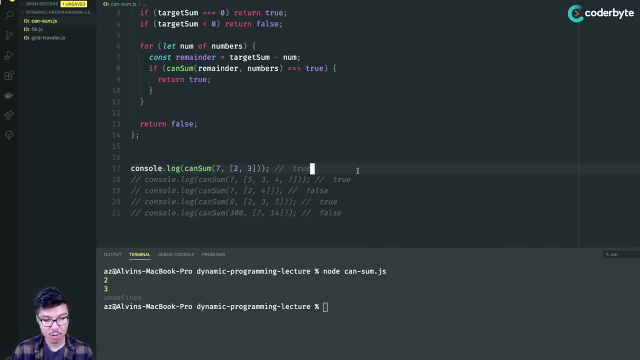 So let's go ahead and give this a go. So I'll try all of these examples And we'll see what we get. So I expect a true, true, false, true, false, Cool. So it's like a few of them are working right. It looks like the first four are working. 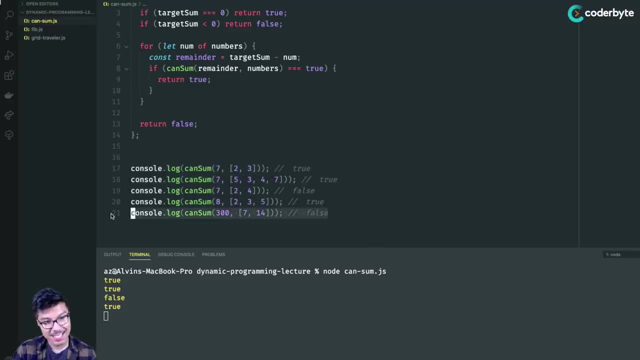 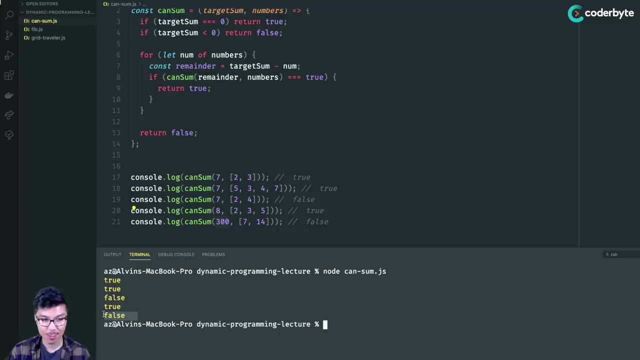 totally fine. But looks like on that last example my program is still running And, if you notice, I chose a pretty large value for M, So kind of like we expect. this solution has correctness, but it possibly lacks some efficiency. it looks like it just finished. it definitely took way. 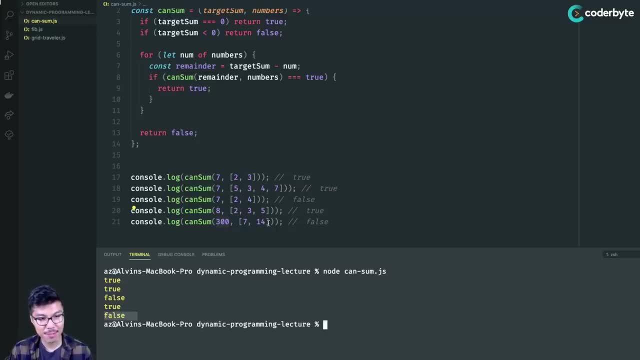 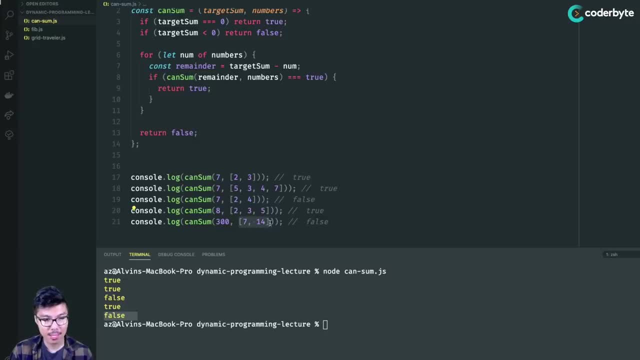 Because, for one, the length of the array is pretty short. I only gave two elements here, But it seems like this number as a target sum really affected the runtime. So what we'll do? let's head back to the drawing board and talk about the complexity of this baseline solution. 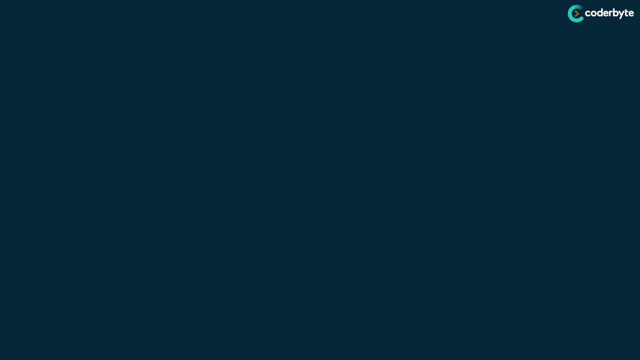 Alright, so we implemented the brute force for our can sum, But obviously now we want to make it a little faster. But before we kind of just jump into memoizing the solution, let's at least describe the complexity of our current brute force. So let's try to visualize this example. So I have a target sum of eight And my choices for 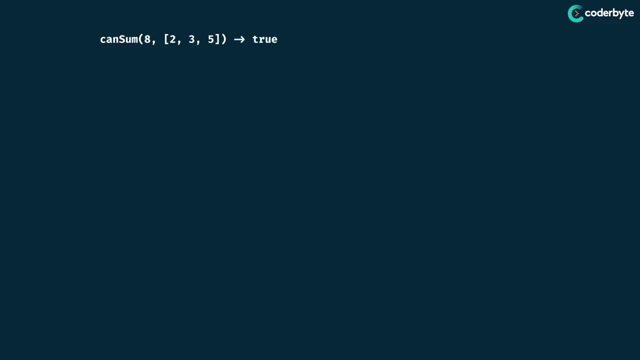 my numbers are two, three and five. In the long run, this should return true. The visual for the full tree would look something like this: Notice that it's a fairly large tree for some relatively small inputs. right, I only have a target sum of eight and only three choices, So let's try. 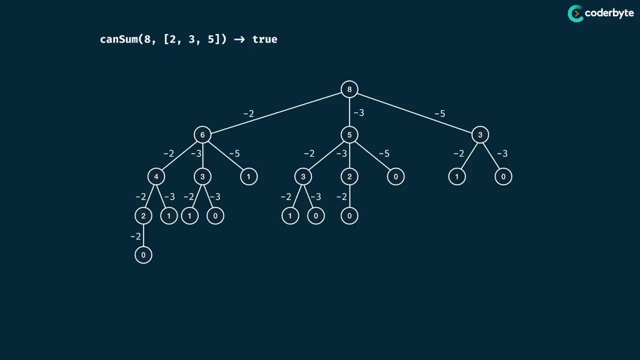 to describe the complexity of this, I'll sort of generalize the shape of it, get rid of those numbers. So this is the overall shape of the tree And I know I want to describe my complexity in terms of the size of the tree. but I'm going to go ahead and describe the size of the tree. So I'm 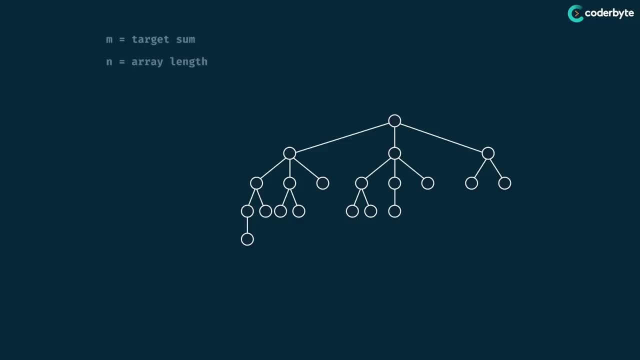 going to go ahead and describe my complexity in terms of the input to my function. This function has two inputs, though. right, I'll say that m is the size of the target sum and n is the length of the array I'm given. I know that both of these arguments definitely have an effect on the 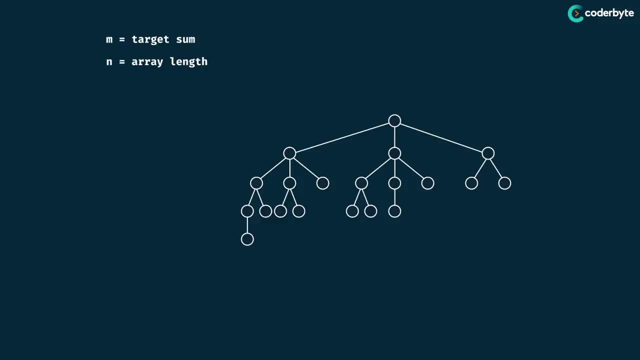 dimensions of this tree. So, like we did in all of our other examples, I'll start by maybe analyzing the height of this tree. That is what would be the maximal distance from the top level call to a base case Or, in the structure of the tree, What is the maximal distance from the root of the tree to the 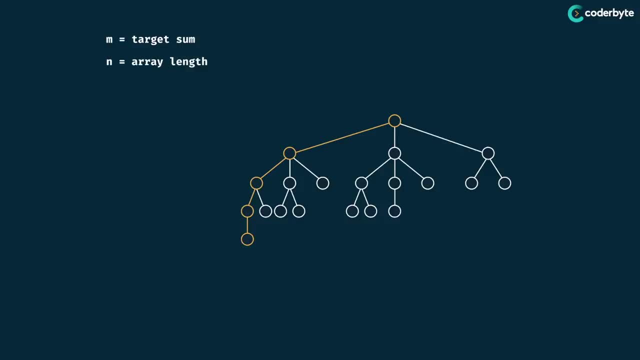 farthest leaf. So if you sort of imagine that we have m as the root of the tree, imagine that along the left hand path we just did a minus one all the way down right. So we kept taking a minus one right In. 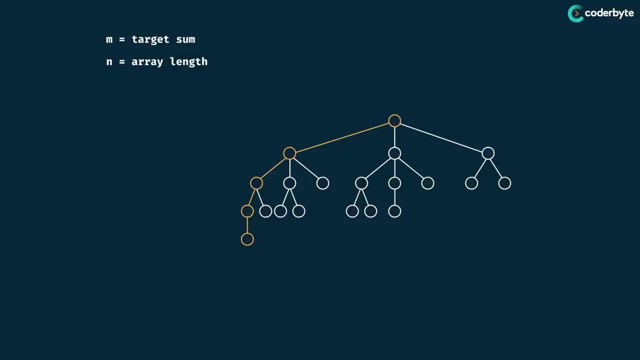 the worst case, maybe there's a minus one present in our numbers array. In the worst case, the distance from the root to a base case would be exactly m, because you have to subtract one m times right. So I can basically say that the height of this tree is m, And kind of like we. 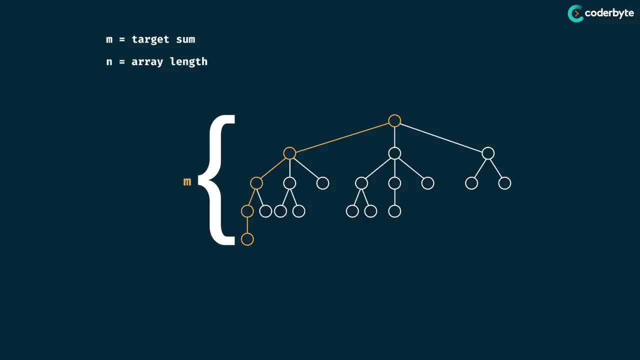 said under other problems. that means that the number of levels is m Right. So now that I've identified the height of this tree, the move is now to identify the branching factor. that is, how does the number of nodes change from one level to the next? 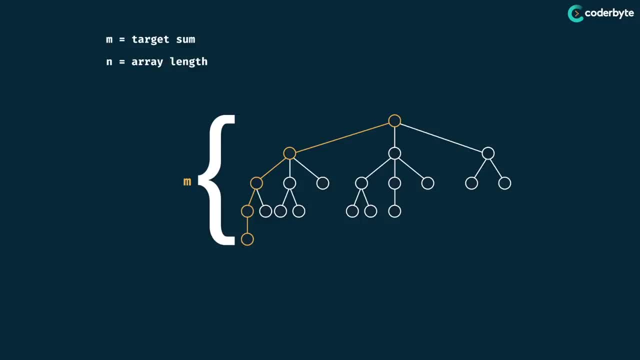 Remember that initially we described this particular tree example as having numbers array length of three And you'll notice that the maximal branching factor is exactly three, or in general n right, because n is the length of the array. So, for example, if I had three numbers in the array, then a node would have at most three. 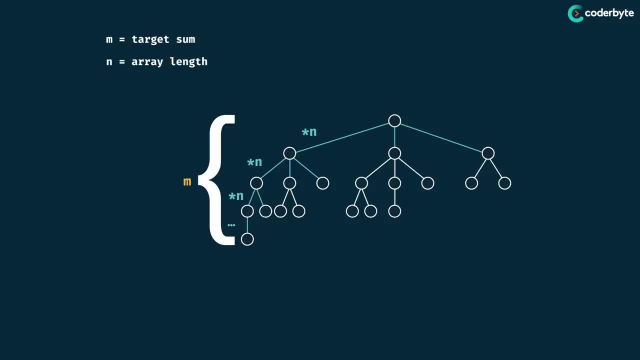 three children. right, because you have three options to take. we've seen this pattern before. I have m levels and from one level to the next, I would multiply the number of nodes by n, right? this is the same thing as saying, hey, we take n and multiply it by itself, m times And this: 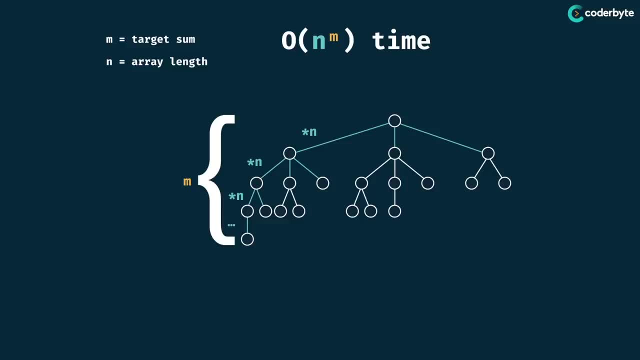 would definitely give us an exponential complexity right, in particular n to the m time complexity And, like we always say, another great thing about this type of diagram is we can also derive the space complexity right. So what would be the space used by the call stack? 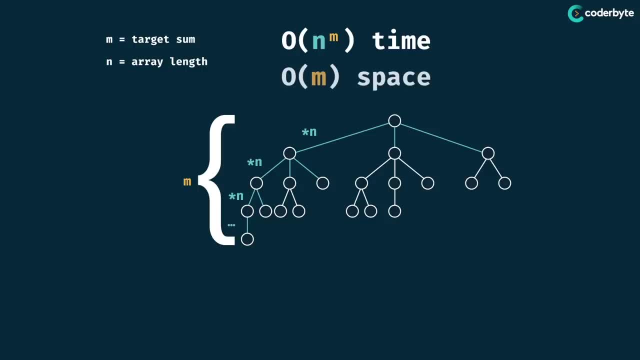 really just be the height of the tree, which we already described as m. So, overall, our brute force is looking at an n to the m- time complexity and m- space complexity. So now that we actually have, you know, those concrete numbers for complexity, let's go ahead and focus on how. 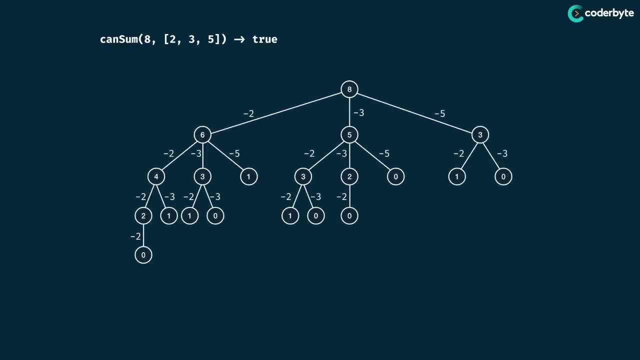 you can truly improve this. So here's again the drawing for this particular example. it's a fairly large one And typically you know when you're trying to notice where there is room to be optimized. you might have to give yourself a sufficiently large example to see. 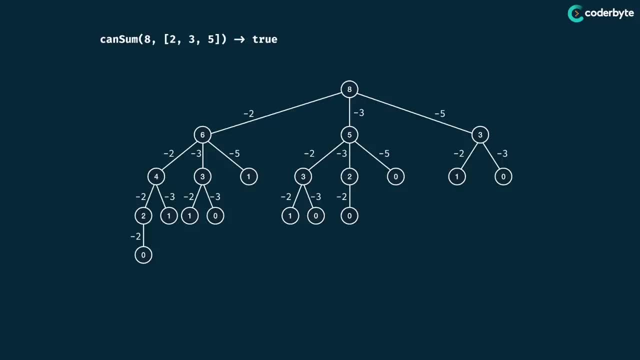 of these scenarios. So in this example I do have overlapping sub problems And in the context of my tree that means I have duplicate sub trees. So I can look at, possibly, this subtree rooted at three. notice that the root of that subtree is trying to answer the question. hey, can I generate? 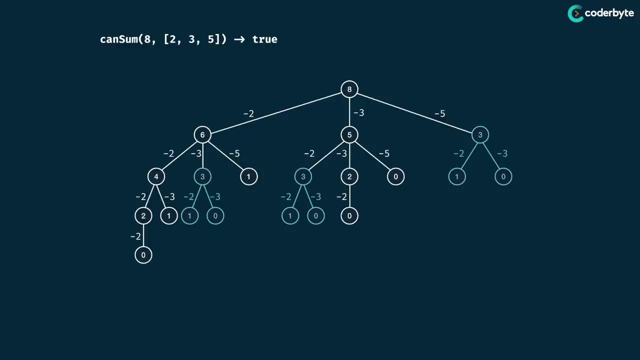 a target sum of three using the array. And, of course, once you find that answer, that answer is never going to change for your target sum of three, right? So I know that all three of these sub trees are trying to ask the same problem. 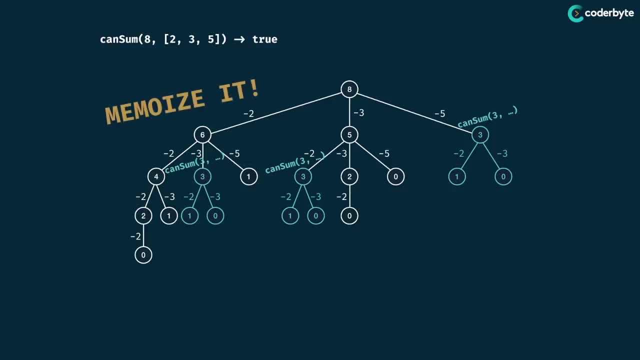 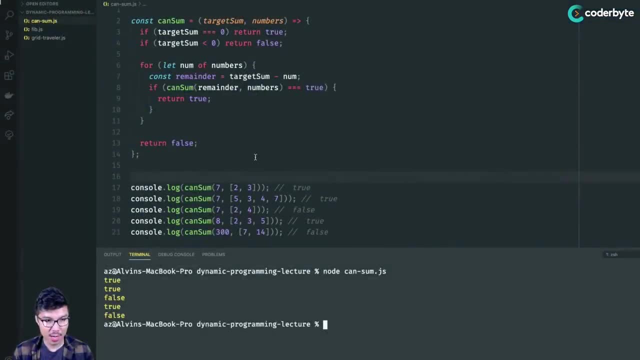 So what I'll do is I'll just cache those results in my memo object, like we always do. So let's go ahead and work on that. All right, welcome back to my code editor. And same stuff different day. let's go ahead and memoize this. can some function right Once we've 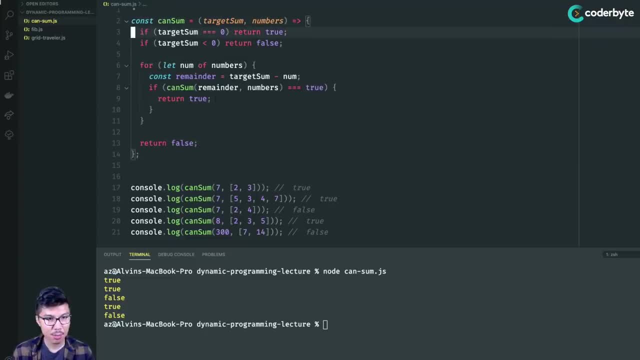 established the brute force through the recursion, then memoization is pretty formulaic, right? All right, so we'll start by just baking in our memo object, like we usually do. So if someone calls our function without a third argument, that is, you know, like a top level call. 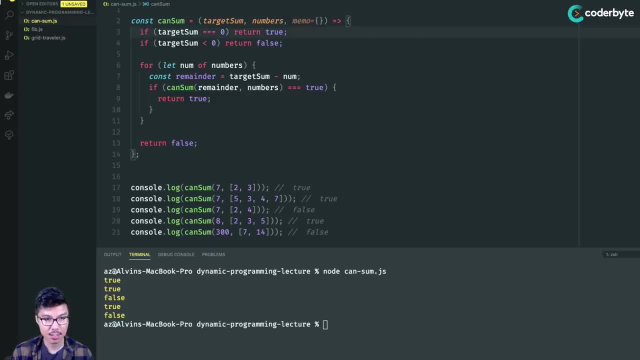 we'll be sure to give them a new object And I'll, before I forget, be sure to pass down this memo object. So I'm going to make sure that every top level call in its recursive tree shares the same memo object. But now I need to figure out what I- what should I- use to key into. 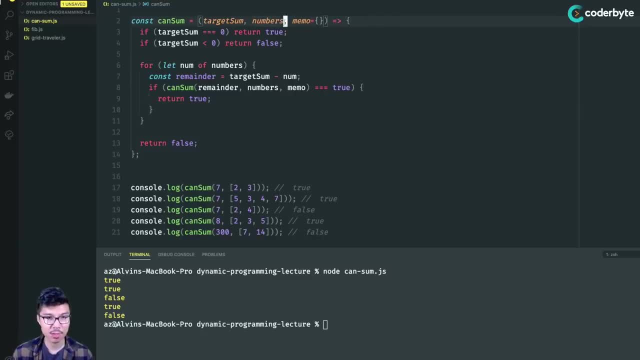 the memo object. So here I have, you know, two arguments of my original function. I have targets, some numbers. what I want to do is try to notice, you know, which of these arguments is actually going to directly impact the return value. So I know that. 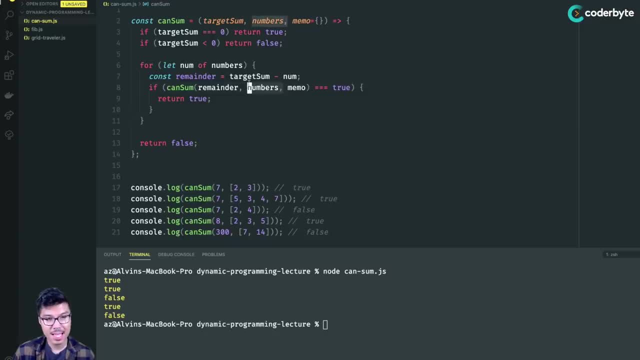 let's say I want to do the recursive calls like this call over here. the numbers argument doesn't change And so if it doesn't change then right now it doesn't really affect the return value. So I'd be okay to just use the target sum as the key into this memo. So we'll go ahead and 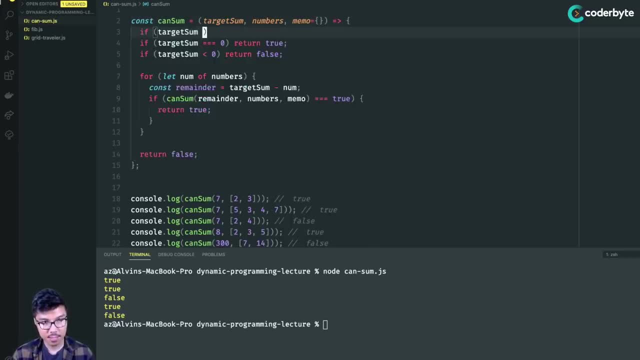 do that, So I'll check. if my target sum is in the memo, then I've seen that sub problem before. so I can just return the stored value. Cool, And now I have my- you know- memo fetching logic. But now I need to actually store things in the memo, And the trick is: 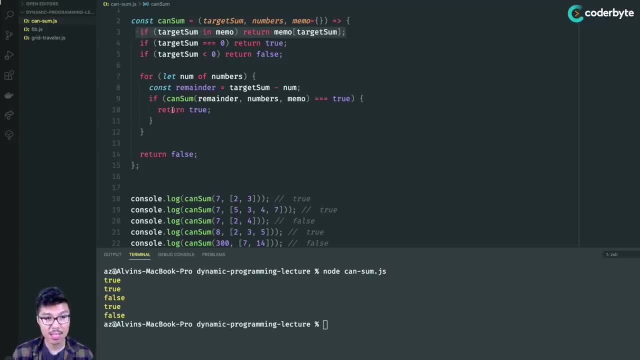 what I want to do is look at all of the return values that were not base cases and I need to now store them in my memo. So I have two return values here, right, these two lines, lines 10 and 14. And so I need to store data into the memo for both of those lines. It's as simple as quite. 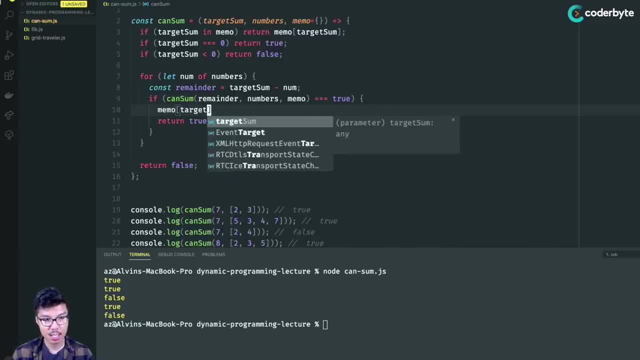 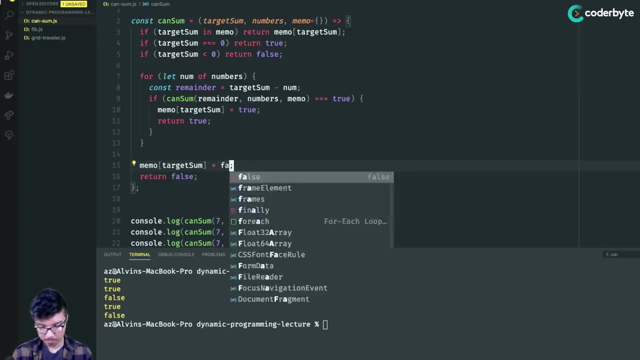 literally going into your memo using your key, so target some, then assigning the value you just returned. So I'll just write it like this And this is going to be sort of a hard and fast rule you can always use for a memoizing a brute force recursive function, right? So I'm just going to take exactly. 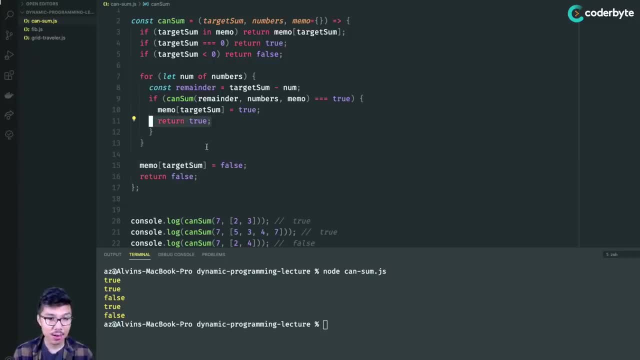 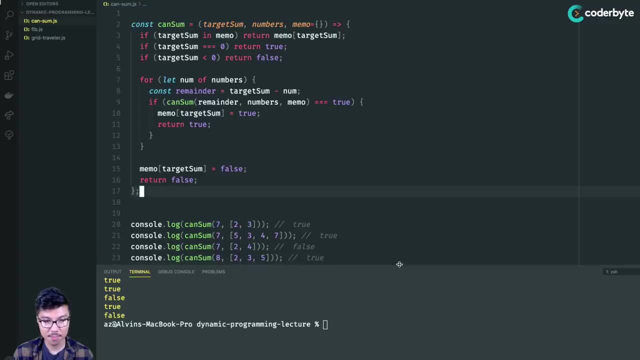 the lines or the expressions that I returned in the recursive scenarios and now just store them in the memo. Cool, So let's go ahead and give this a shot. This code is looking pretty good And remember before, this last call with an input of target sum 300 took noticeably long. 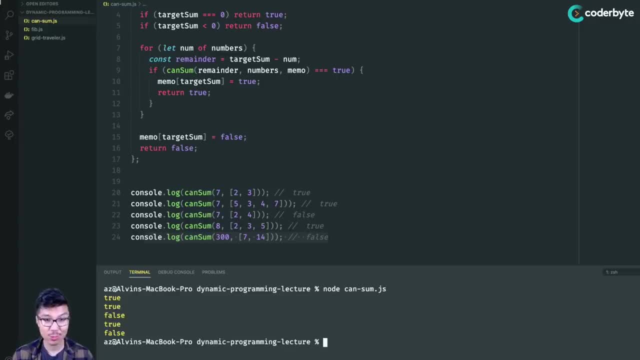 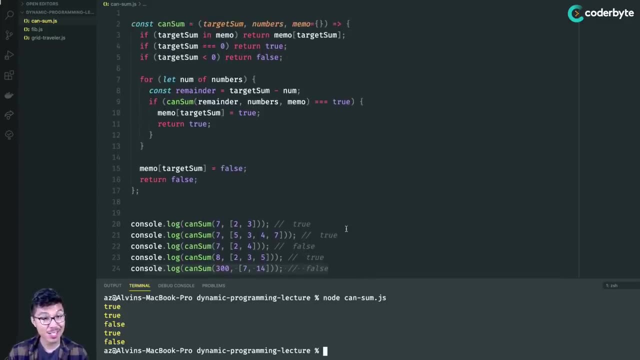 but I think now when I give this a shot right, it finishes really quick. So this is going to be a nice optimized solution for can some really most of the work of this problem was done in the brute force And then afterwards it's really just a minor adjustment. 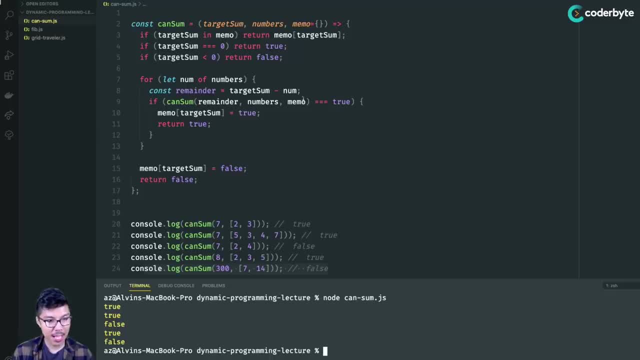 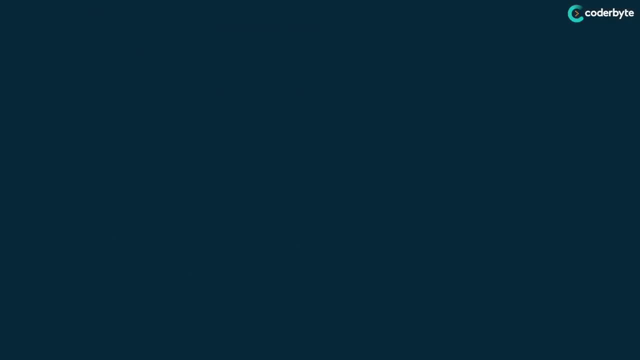 to make it efficient. So to wrap up this problem, let's go ahead back to the drawing board and talk about the improved complexity. So we definitely memorize the heck out of that code, But let's recap by just understanding what the new complexity is. So again, we're saying that n 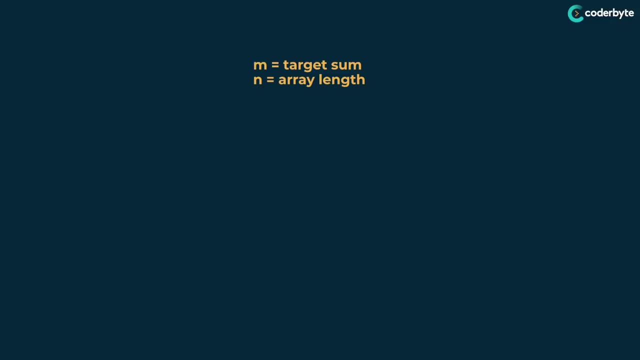 m is the target sum and n is the length of the array. Initially we said that our brute force solution had an n to the m time complexity which is exponential, And actually once we memorized it we really cut down on that complexity. we brought it down to an m times. 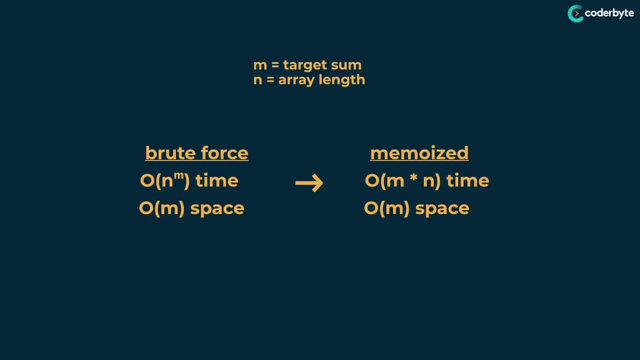 n time complexity. And so here we say that the memoized complexity is now m times n because of the memo object right. we know that the value of the nodes in the tree are just going to be values up to m right. there are m different possible values that we can have in a node. 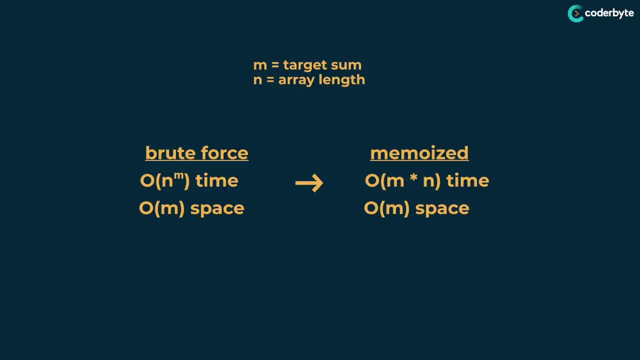 However, now since we are able to cache values or cache results inside of the memo object, I'm never going to have to re explore a subtree before m. That being said, I still have to branch n times for each of those nodes right. So overall I have m times n nodes, So hopefully that can some problem made some. 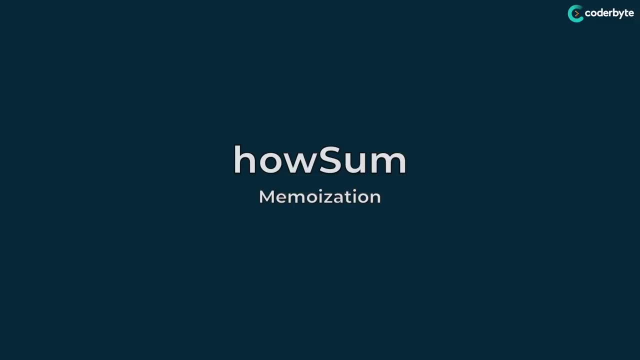 sense, because we want to do now is actually carry over a lot of that knowledge to solve this new house some problem. So this problem is very similar. it still asks us to take in some target sum and an array of numbers, But this time around what we want to do is return an array containing a combination that adds up to: 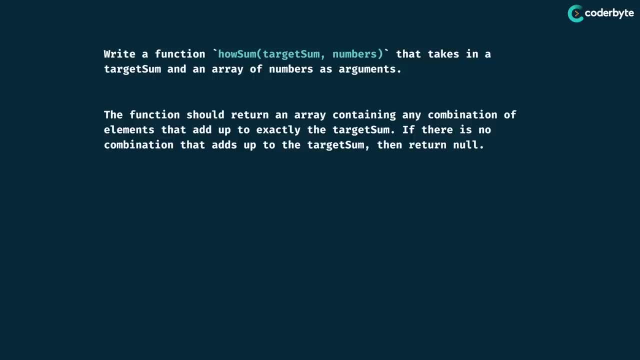 exactly the target sum, And if there's not any combination that actually leads to the target sum, then I should just return null Along with that. if there are many possible combinations that can reach the target sum, then I can return any of those. So you're probably already recognizing. 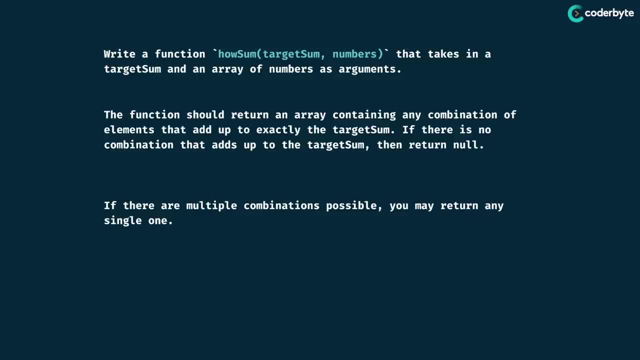 that this house some problem is very similar in logical structure to the can some problem, right? Instead of returning a Boolean, instead now I want to return exactly the combination of elements of the numbers array that leads to my target sum, So it's a little more involved. That being said, 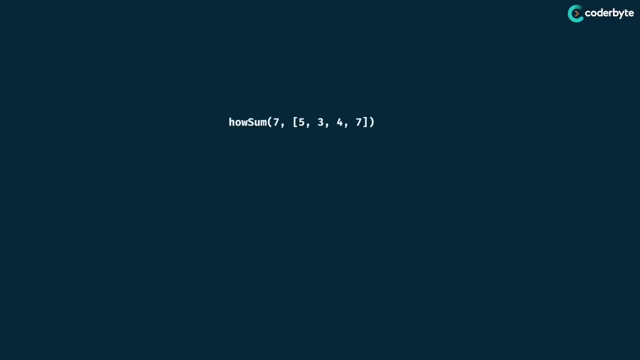 let's take a look at some examples to make sure we're on the same page. So let's say, someone asked us to calculate how some and our target was seven, and our array of numbers are 534 and seven. So there are actually a few different combinations that can give you your target sum of seven. 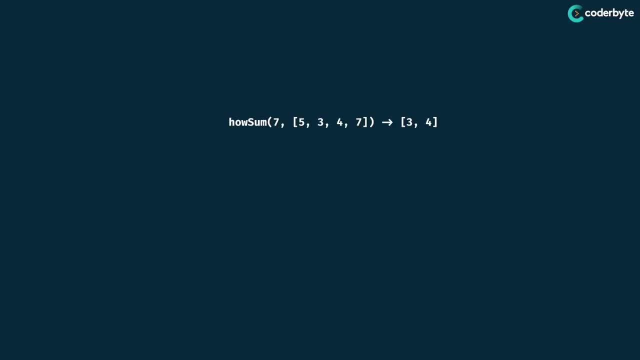 one way would be to take three plus four. that's one possible answer. Another possible answer would just be returning an array of seven. So no matter which combination array you return, it'll be the same. Let's say, I gave you another example where your target sum was eight and your choice. 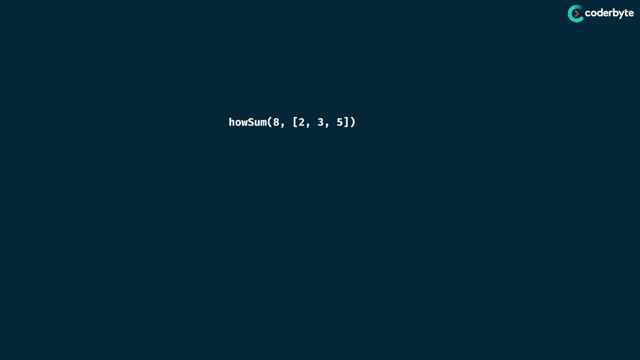 of numbers were two, three and five. one possible solution for a combination is two plus two plus two plus two, right? So I returned that in an array. Another combination would be just three plus five. notice that, no matter what, we're always looking to get back in array if it is. 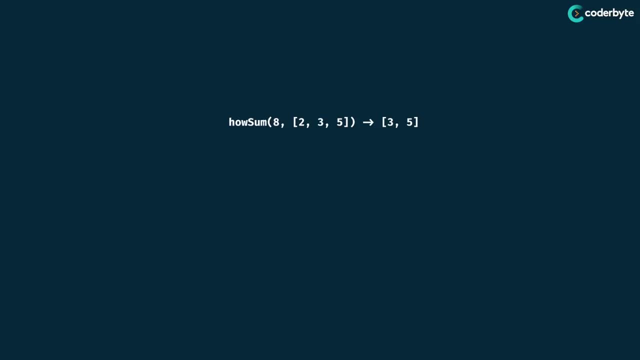 possible that our target sum can be generated. But let's look at the flip side. Let's say that we were given this input, So I have a target sum of seven and my array of numbers is just two and three. First thing we notice is it is not possible to actually generate the target sum of seven. 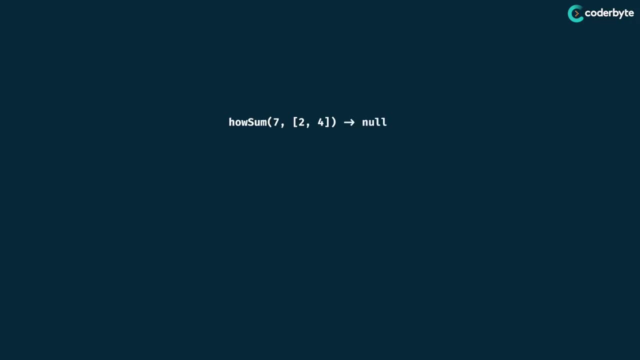 Like they said in the problem, in this scenario, what you want to do is return gnome sort of symbolize that, hey, it's not possible to generate any combination that leads to the target sum. Alright. I think it's important that we think 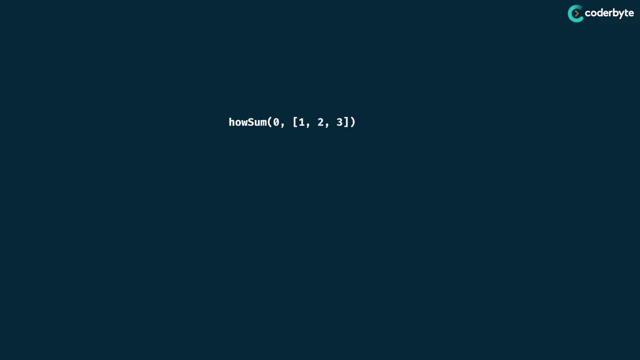 about one more scenario. So let's say that I was given a target sum of zero and we were given really any array of numbers. In this case I just gave us one, two and three. we already know that in our previous problem we had to return a Boolean result. we use the target sum of zero as a base. 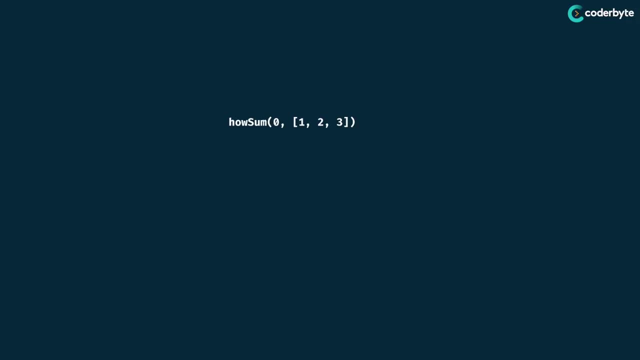 and so what I want to think about now is: how is the target sum of zero just trivially solved? Well, if I want to know the combination that sums to zero, then that's really just the empty combination, right? So I think the logical result here is to return an empty array when your target 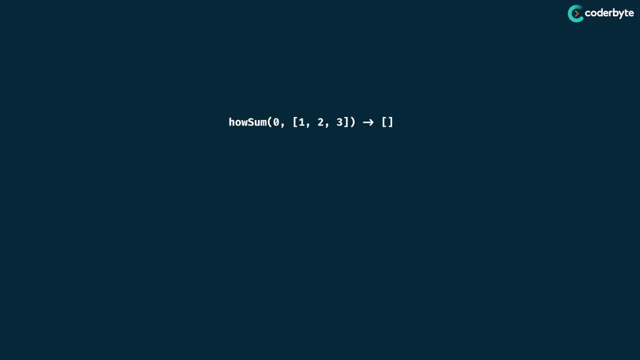 sum is zero. remember that an array represents a combination, And if I have an empty array, that means I take no elements into my combination. right? If I summed up all the elements in that empty array, it would indeed have a sum of zero. So that's going to be a really important facet. 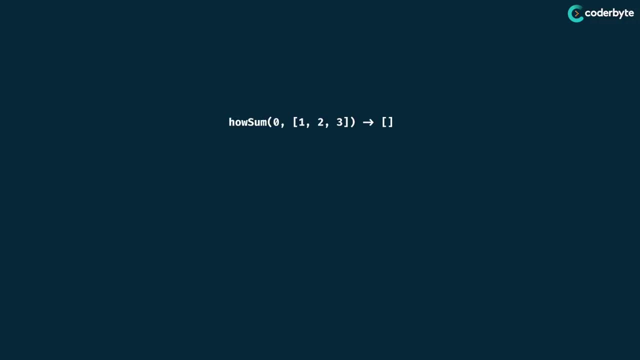 that we need to encode into our logical tree that we draw next, as well as our code, right? So let's take a look at how we can structure the tree and try to take a step toward a really understanding how we could implement it in some code. So let's say we're stepping through this. 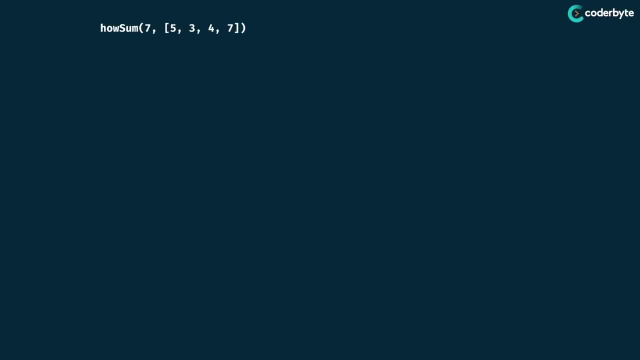 particular example of target sum of seven, as well as an array of 534 and seven. So the full tree- in really the same tree that we drew last time- will look something like this From the get go. I see that I have some scenarios or some nodes where I reach zero, which means that it's 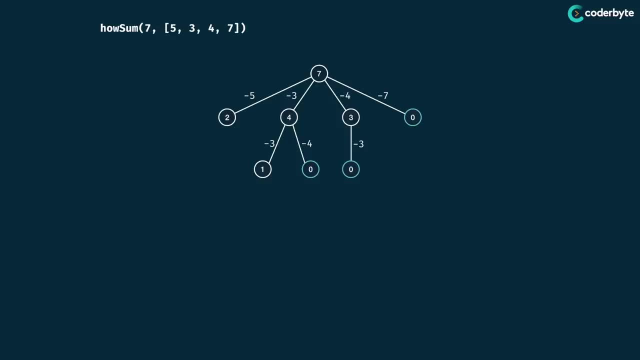 definitely possible to generate some of these elements, So let's take a look at how we can generate the target sum. That being said, how can I get back a valid result, right? so I need to return an array, So we sort of reframe this problem in that, all right, all of these base cases that 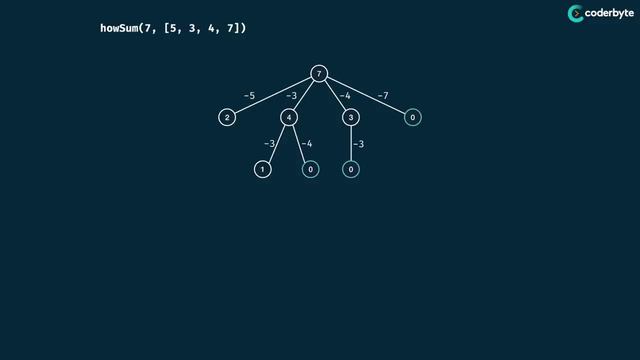 have a target sum of zero, they are trivially solved because their combination would just be the empty array, right? So for now I'll just kind of trace through how one of these base cases will return. So I know that this particular zero is going to return an empty array And, like we, 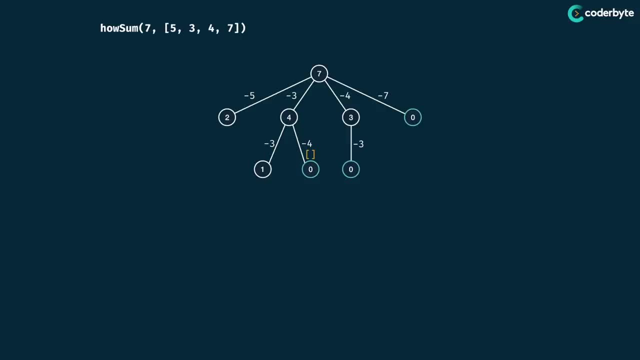 always say when it returns, it's really returning that information to its parent, right? So this array sort of bubbles up to its parent. And now what I want to do is actually manipulate this return value. I want to add something to it. So I want to really put the number that brought me. 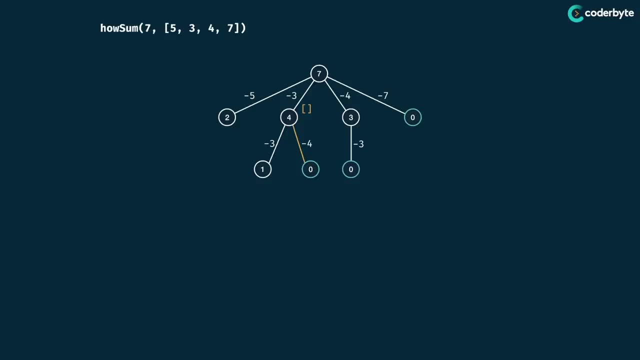 to that zero in the first place, And that would really be the choice of four. So notice, along the edge, I have them labeled with a minus four, meaning that, hey, I took a choice of four And I want to actually add that choice into the current array. So I'll just really push it into the array. 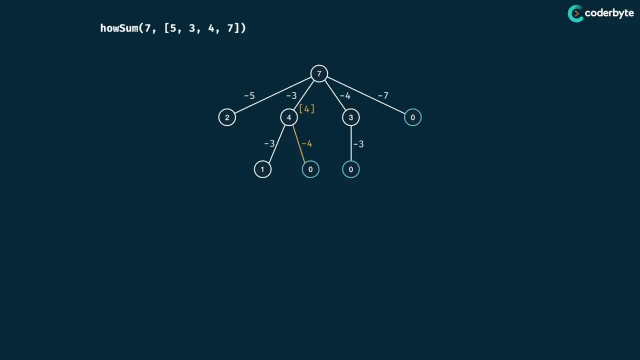 Of course, I actually don't need a negative sign. that was just for the sake of understanding the math here. But now that my call to how some of four is returning an array of four, that array bubbles up to its parent And of course now I need to push that edge that I took, which would be that 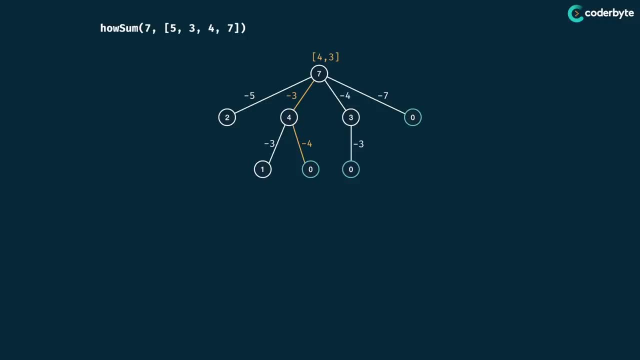 three. So now that three gets pushed to the array as well, And if I look at what I'm seeing right now, it looks like above the seven we have an array of 43, which makes sense because you can totally generate a target sum of seven by doing four plus three. Awesome. So four comma three. 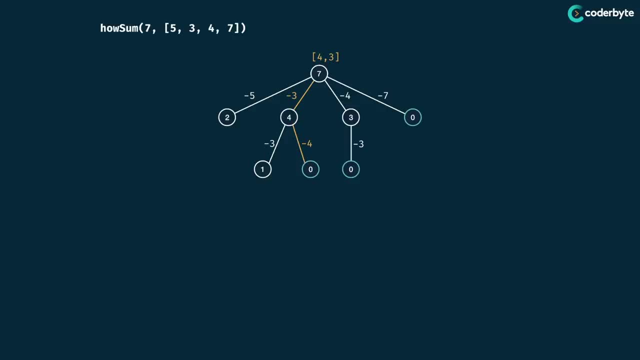 would be a valid answer in this particular problem. But, like they said, you could return really any valid combination if one exists. So let's say we were chased through this far right base case. we know that this zero is going to return an empty array. 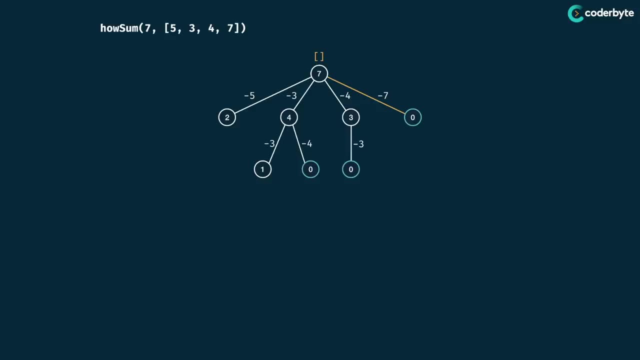 that empty array will be returned to the parent. But we also have to add the value according to the edge right. So I would put a seven in this array And that makes sense because I could generate the target sum of seven by just summing up a lone seven. So that's still good to go. 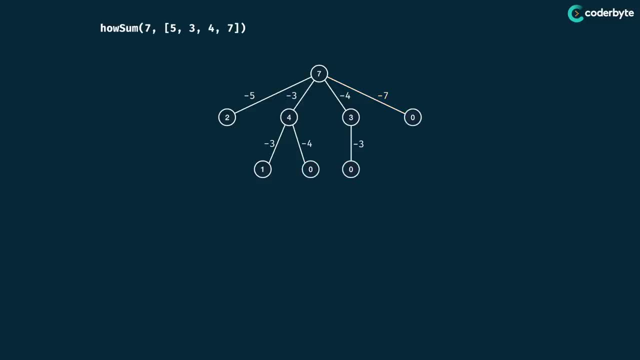 So I'm feeling pretty good about how we can return a valid combination, if one exists. But let's say there are some options that we take that don't work out. So, for example, let's say we explored this node first, right, this was the first base case we hit And, logically, 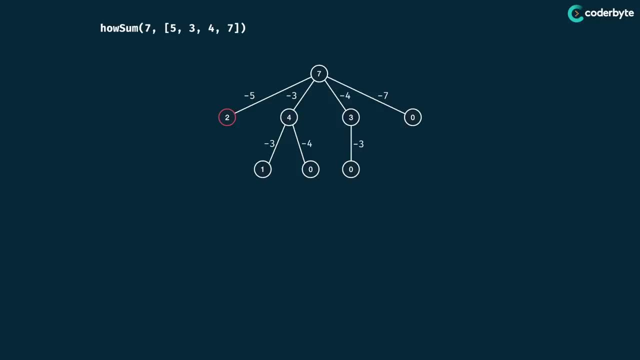 in the space of our code. it really would be right. So I know that this node can't really branch out any further, So it's sort of a dead end. This is a node that should return null, meaning that, hey, there is no way I can generate a target sum of two. 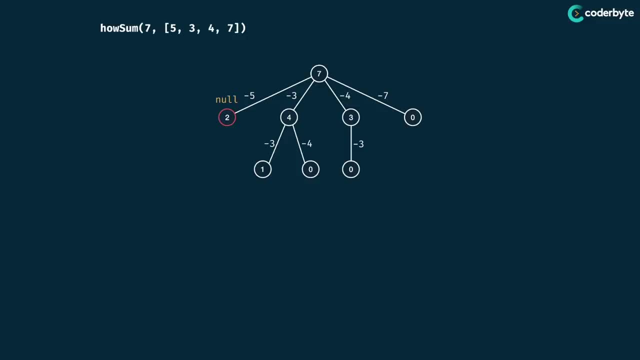 using elements in the array, or if you look at the elements of the array, they're all too big right. So I know that this base case is going to return null, But along with that, if you look at the next base case we would hit, it would be this one, which also returns null. And if you look at 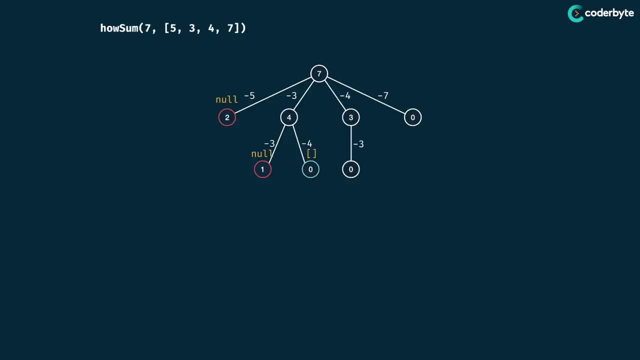 the next base case to the right that is actually an affirmative one- that should return an empty array. So it's kind of reason out how these return values should be considered at their parents. So I know that both of these values, but to the left of the node four would return right. so it 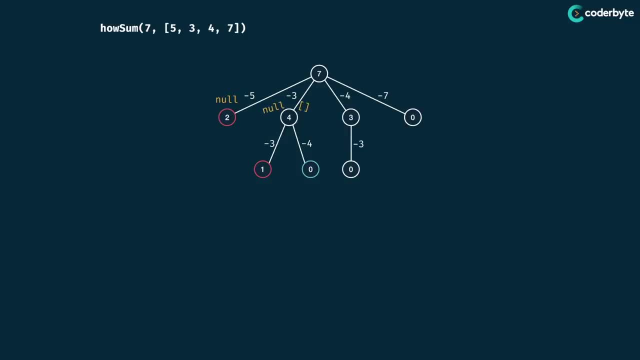 kind of bubbles up a little bit. But for the array on the right hand side I would also have to push the edge that I took a four in this scenario. So now I'm sort of comparing, you know, the null in this four. 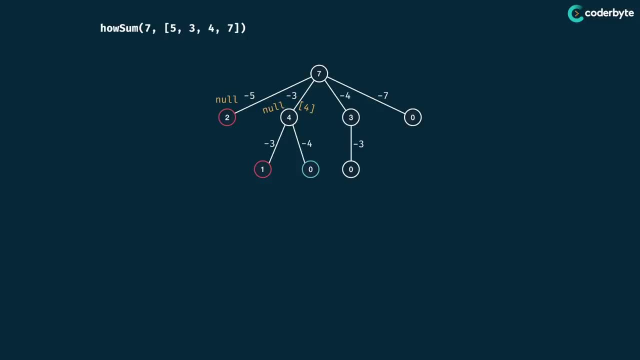 or really I'm comparing all of the branches that I take from a node And if at least one of the branches gives me back an array, that I know that it's possible, right. So basically, in this scenario the array of four actually wins out over the null, right I know it's possible to. 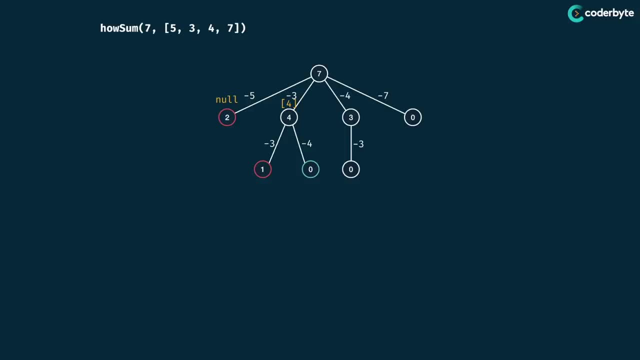 generate a four, and I'll just continue this process. right Now, I can return these two values to its parent, So once I'm considering them at seven in the same way, I would have to add the edge I took, which would be a three, on this array And then from there. 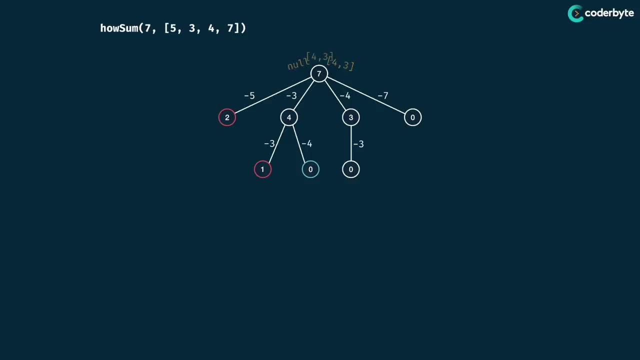 I know the array would always override the null right, so I could just ultimately return this four comma three, And a really nice pattern in this code is as soon as we find a winning path through the tree, or that is, we find a combination that creates the target sum. 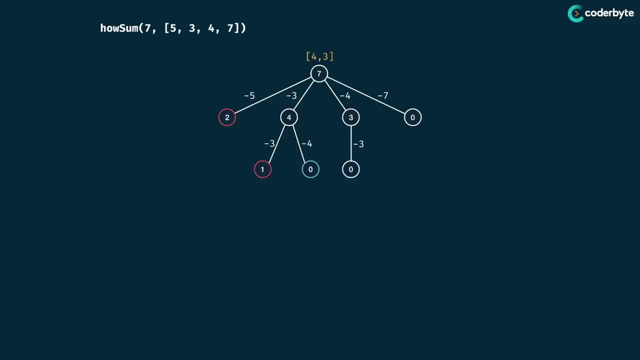 we can actually return early because we don't need to really travel through the rest of this tree. we don't need to explore any other options because they're happy with at least one combination: right, Awesome, So again to recap, the punchline is for this tree. I have the information for a. 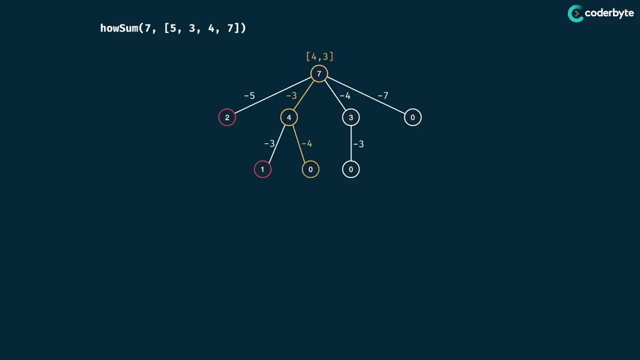 combination encoded as a path through edges of this tree right. So if I look at this path I have highlighted in yellow, I see that I took a three, followed by four and that eventually led to a zero. So I know that one valid combination would be four comma three. All right at this point. 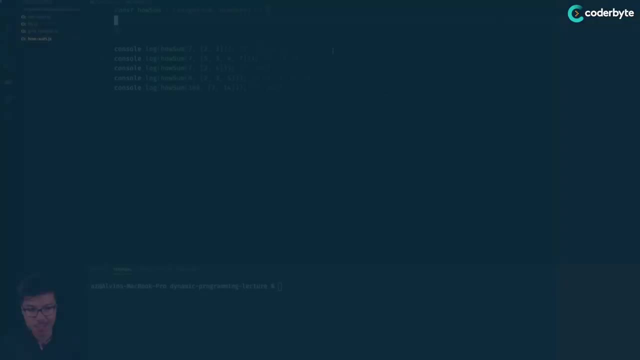 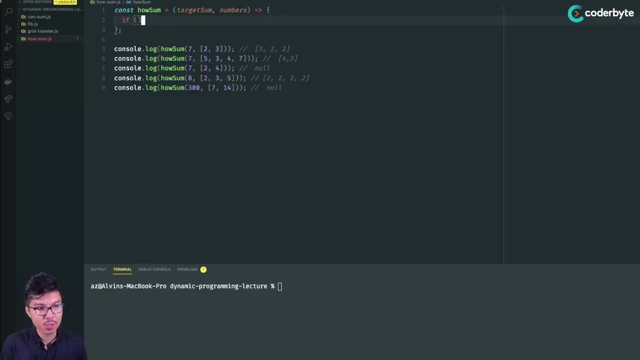 I'm feeling pretty good. Let's go ahead and work on the code for this now. All right, here we are back in my code editor. let's work on solving the house- some implementation. So the code is going to be pretty similar to the can- some problem. That's the really the whole. 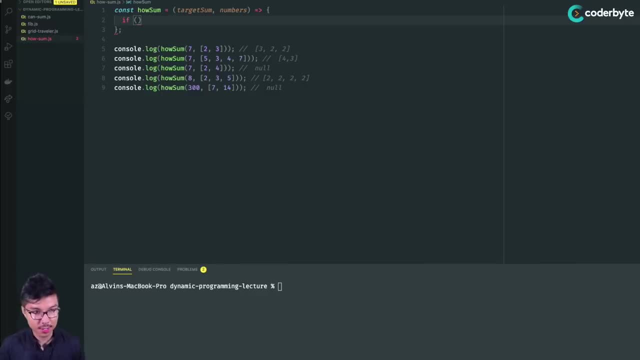 point. we're just kind of going to finesse the return data over here, So we're gonna have a very similar base case, like we said in the tree diagram, whenever we have a target sum that's zero. we have trivially solved the problem because I could just return an empty array. 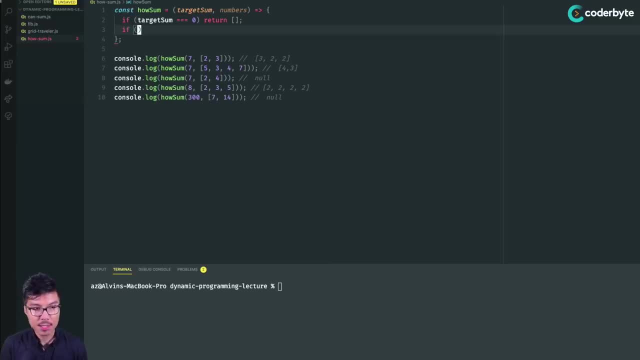 In a similar way. what we can do is also have a separate base case. if our target sum ever reaches a negative quantity, then I'll just return null. That's because it's never possible to generate a negative target sum, right? Remember, in this problem the array is going to be negative. 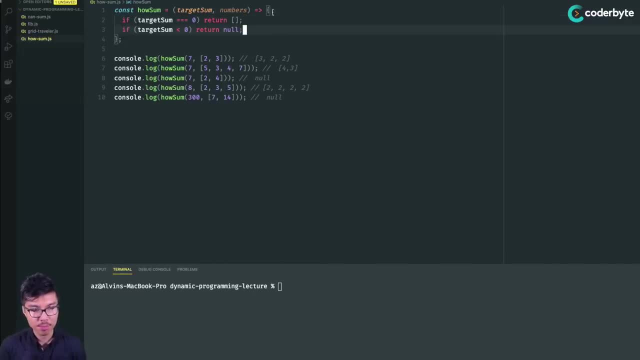 but the array of numbers is only going to be positive ones. Cool, we ended up writing very similar base cases for our last problem, Except now, instead of returning true, we return an empty array, And instead of returning false, we return no. Nice, So let's go ahead and get the branching. 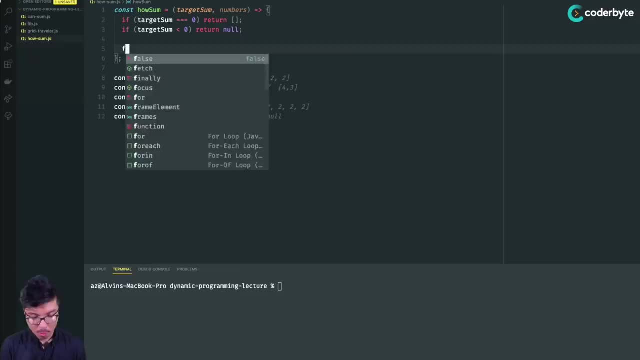 logic, right? How do I want to make my recursive calls? Well, I'm going to need to make a recursive call for every element of the numbers array. So I'll say: let's numb of numbers, So I'm just iterating through every number of this array And I'll go ahead and do the same thing for the 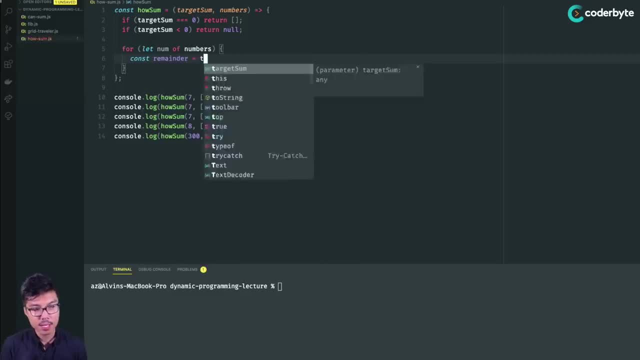 same logic as last time. So I'll subtract the number from my target sum. that would give me my remainder. right, So remainder equals target sum minus my number. Cool, So this remainder is now what I want to find the combination for, right? So here I would make my recursive call. 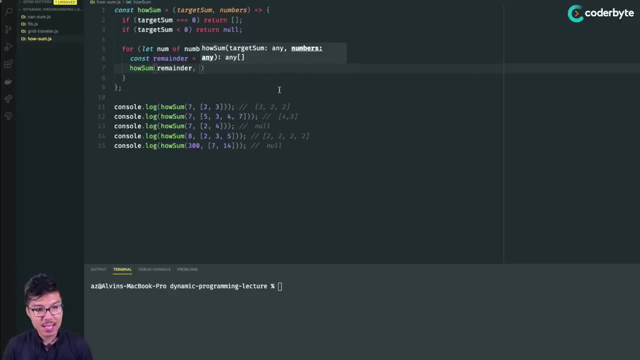 So how? some pass in the remainder and the second argument will stay exactly the same. I'm going to pass along the same exact numbers array. I don't need to remove anything from the numbers array because they tell us in the problem that we can reuse the elements however we see. 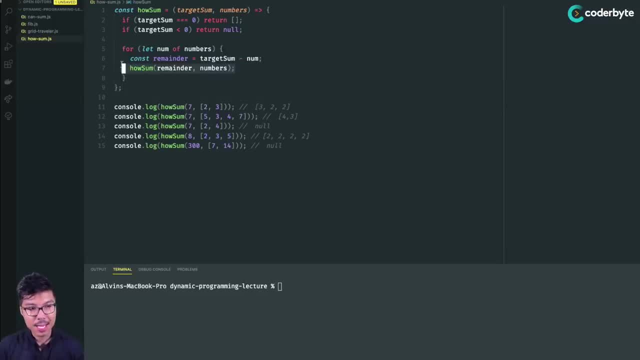 fit right, Cool. So now I need to really think about what type, how some returns. So this problem is interesting because we basically have two different types. right, we could get back in array of some elements if it is possible to generate the remainder, or we can get back null when it's. 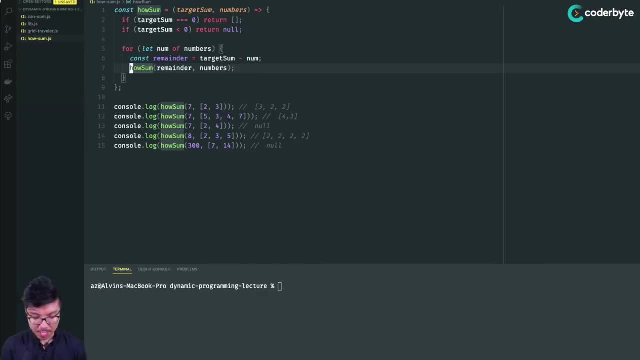 not possible to generate the remainder? I think no matter what I get back, I'm just going to save it into a variable. So I'll say cons, So this is the result for the remainder. I'll call it remainder result. Cool. So I know that in the context of like you know, like you know like. 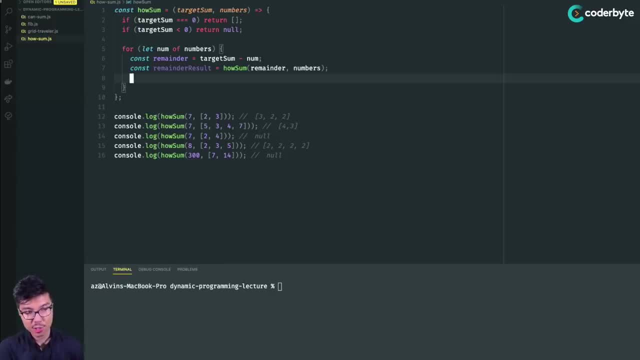 in the context of like how I thought about this logic in terms of the tree. I wanted to basically do an early return if I found a valid combination, And so I'll go ahead and check, you know, if the remainder result is not null. So the implication if I enter this if statement. 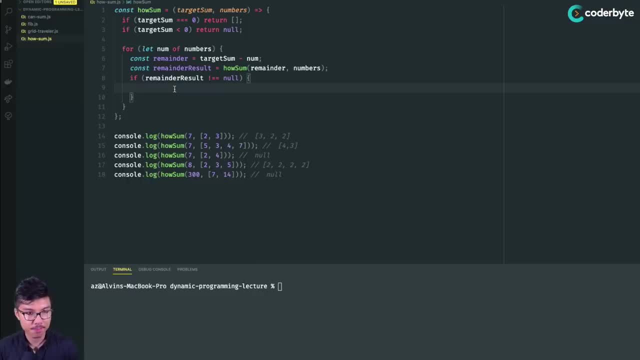 that means that it is possible to generate the remainder, And so what I can do is just return early, and I can return a basically almost the same remainder results, So the same array expression. However, I need to make sure I include the element that I took recall from. 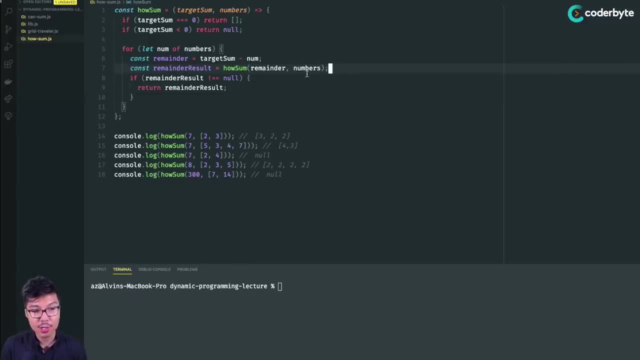 the diagram. whenever we had a recursive call that returned an array, the parent had to also add the number that it took to transition to that recursive call in the first place, Right? So in the context of the tree, I had to put the labels of the edges into the array. here that means I. 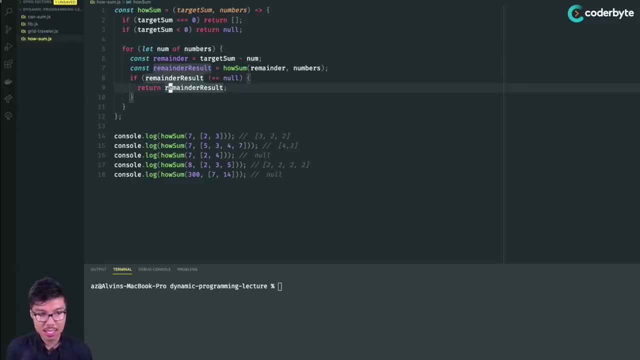 have to put the num into this array. So some syntax I can use for that is to use some spread operator So I can copy all the elements of the array. I can copy all of the elements of the remainder results into this new array, But I'll also add on the number I just took right. 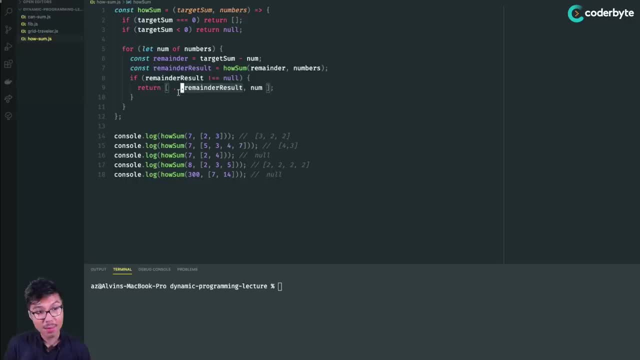 So all I'm doing in this return line is I'm returning basically the same array that I get back from my recursive call, with the number added to the end of it. Let's say you're unfamiliar with the syntax. I can preview it really quick. It's pretty neat. Let's hop into the node. 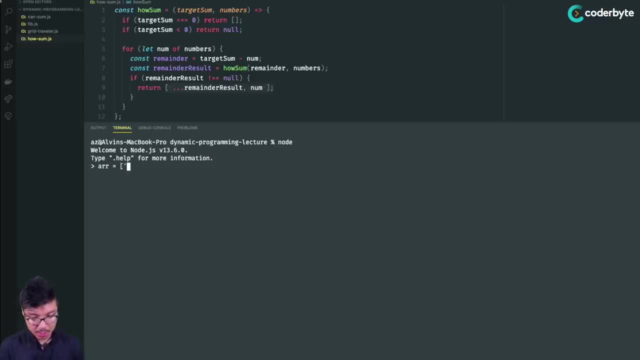 REPL. So let's, I had some array. I'll say it was this array of just ABC, sort of an isolated example. you can use the spread operator, which is the three dots here, to like unpack an array And you can sort of say, like new array equals bracket. So this gives me a new 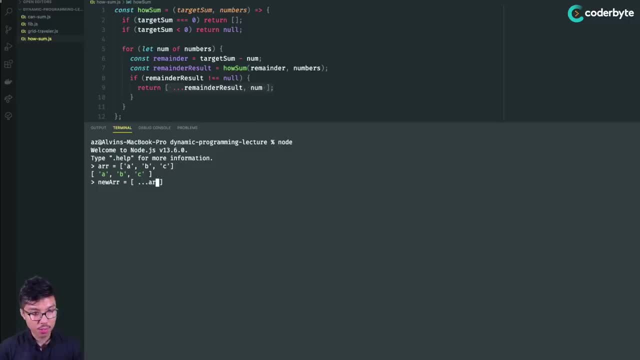 literal array And I can spread out the elements of the old are right. So if I do that, the new array just has all of those same elements. if I capitalize that properly, Cool, We can extend that syntax right. So I still have that array of ABC. Let's say I had another. 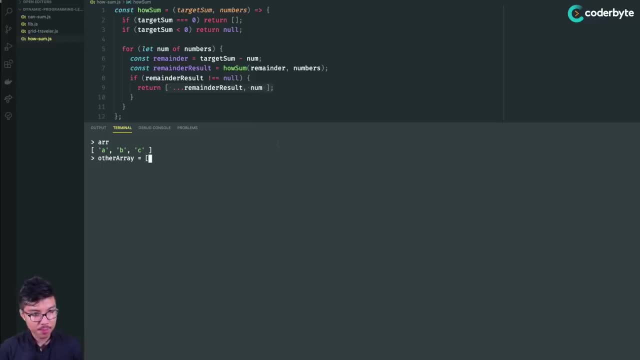 variable. we'll call it other R array. what I can do is create a new literal array, copy all the elements from our using the spread operator, And then I can comma separate any additional things I want to add while I'm here. So let's say I added a Z. So if I look at my other array now, it contains: 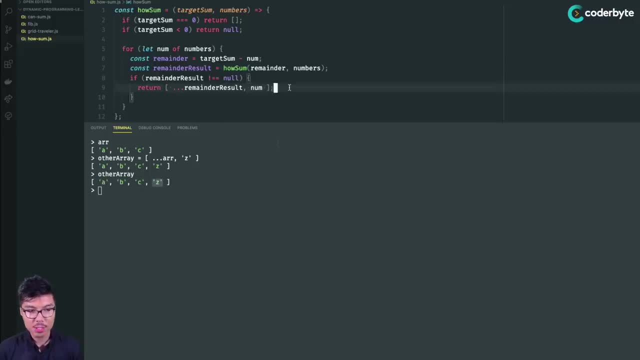 ABC and also this new element Z. So it's all I'm doing on this line, right? I'm returning the same combination that my recursive call gives back, with the number that I took added to the end of it. Cool, So what's really? 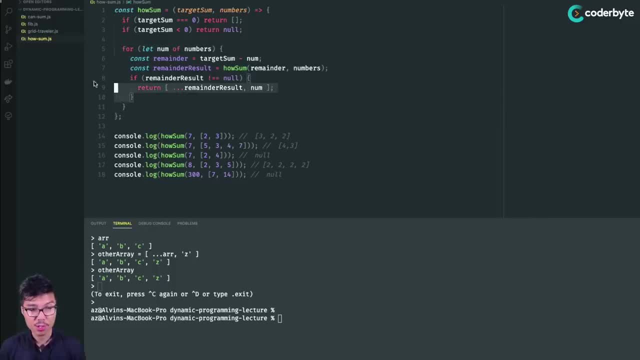 nice about this code is it's very reminiscent to our previous code because we have an early return. So if I find at least one way to generate the target sum, I could just go ahead and return that first way that I found right. they say we can return any valid combination. 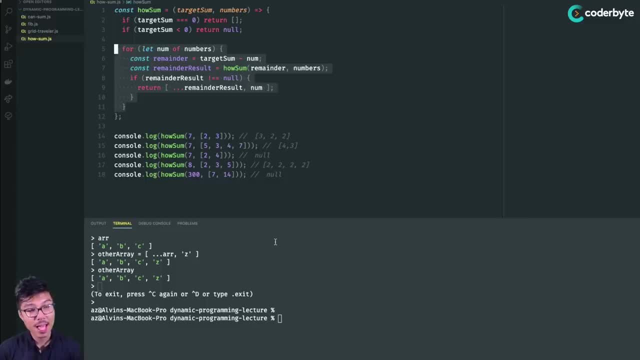 here. But let's say this: for loop finished and we never found a valid way to generate the target sum. Then after the for loop, you can just return No, because it's not possible not to generate the target sum. apparently Cool. So this code is looking pretty good, I think. 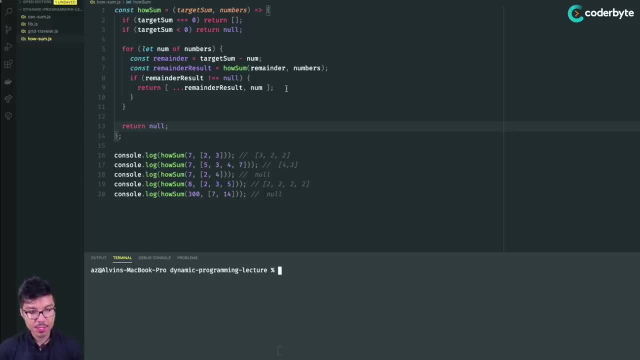 let's, let's give it a shot. goes without saying. sometimes the remainder right will become negative, But we already handled that with this nice base case, right, So let's test this code. So I already have some example outputs over here, So it looks like our first. 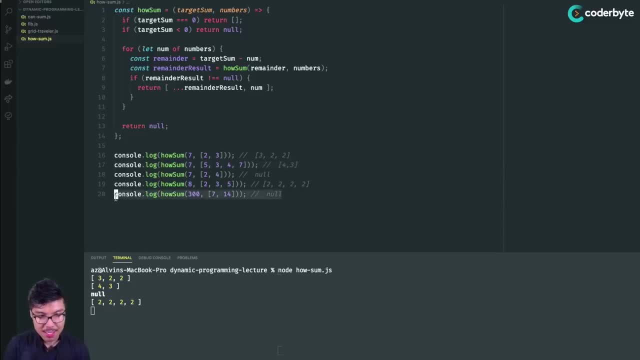 few examples are working. Obviously, our last one seems to take quite a long time, So I'll just kill this program early. But before we talk about how to optimize for this larger example over here, we'll get these other examples. What I can see is this array of 322 does add to seven, So that's looking good. 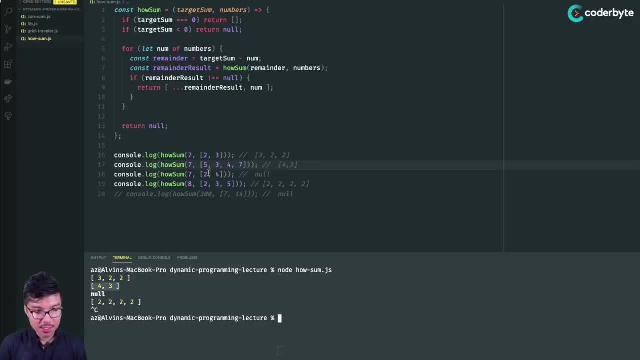 This array of four, three also adds to seven, So that's good. We already saw that. this example of seven and two, four, that's your return. No, because it's not possible to generate that sum And it looks like the array for the eight example is also good to go, So notice. 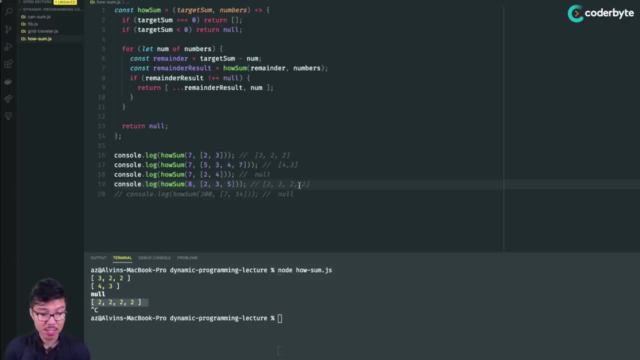 here. there are also some other arrays that we could have returned and it would still be considered valid output. the exact combinations that we get back are really just dictated by the order that we happen to iterate in the array. So, for example, let's say I: 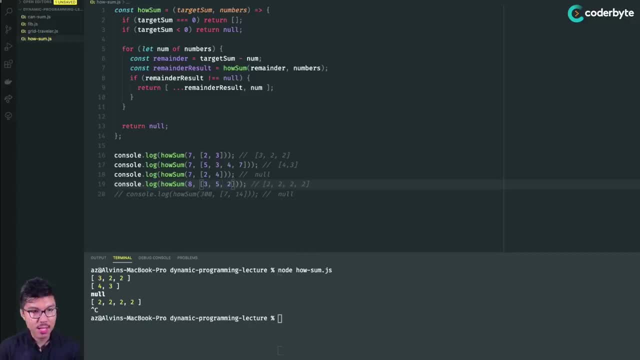 switch things around here like I did. 352, it's really the same array, just in a different order. we'll probably get a different answer for that particular one, right? So I'll run this now. notice, I get 233.. But either case, that still sums to eight, So we're totally. 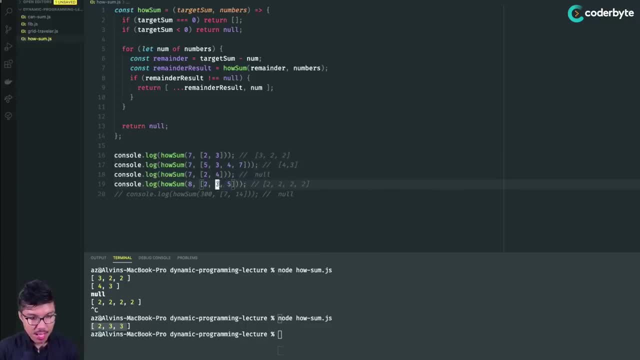 good to go. Awesome, They bring this back to the original code And, yeah, it seems that now the limiting factor seems to be the speed of our solution. right, We've been here before, And so let's go ahead and talk about the complexity of it. So we know that the time complexity- 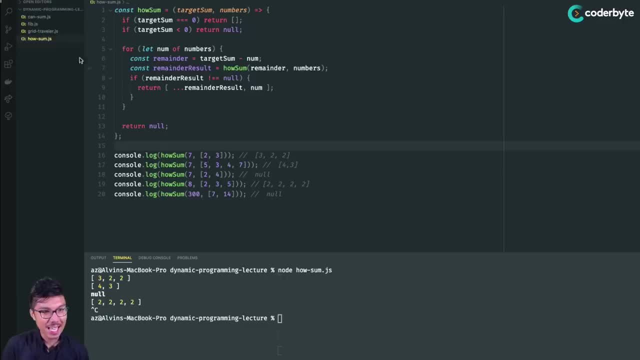 for this is almost identical to what we did in the can some problem, which is conveniently over here, but sort of refresh. By now you recognize that all right. the time complexity should be described in terms of like the recursive tree. So let's lay down a little foundation. 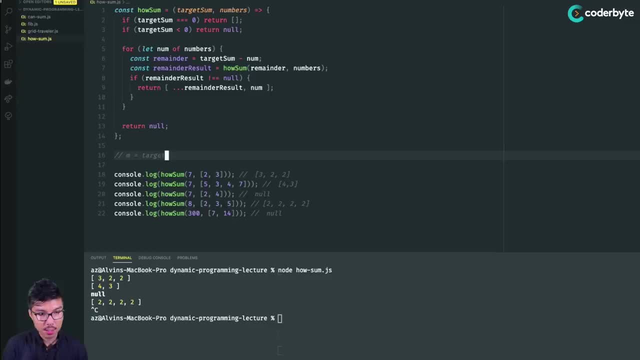 And we already know that m we're going to call the target sum, And let's also say that n is the numbers dot length, Cool. And so if I think about the number of recursive calls that I'm going to make, it's really 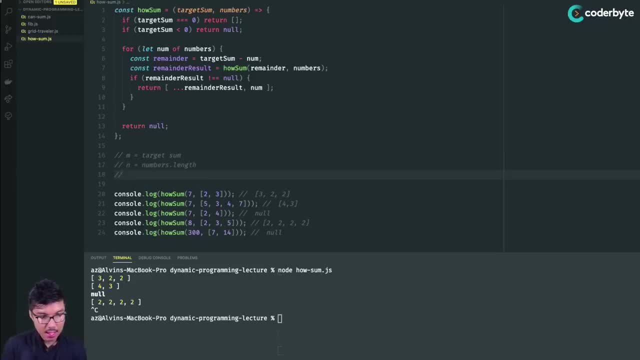 the same as last time, right? So I'm going to say that, hey, the time of this function seems to be, Oh, and I have an exponential. the base of the exponent is the branching factor, which is the length of the array, And then the depth of the tree would be the. 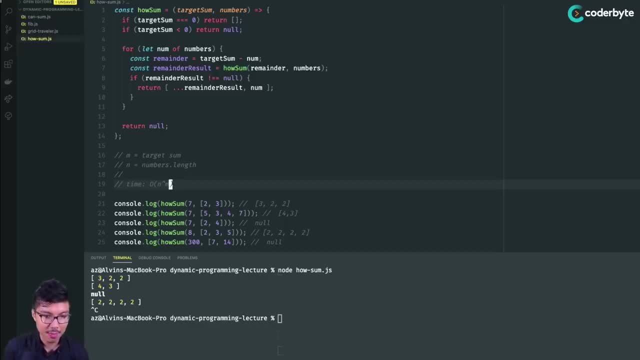 exponent, which is just m. right. So this was the same time complexity as last time for a brute force right, m to the m power. However, it looks like it's going to be the same time complexity as last time for a brute force right, It's m to the m power. However, 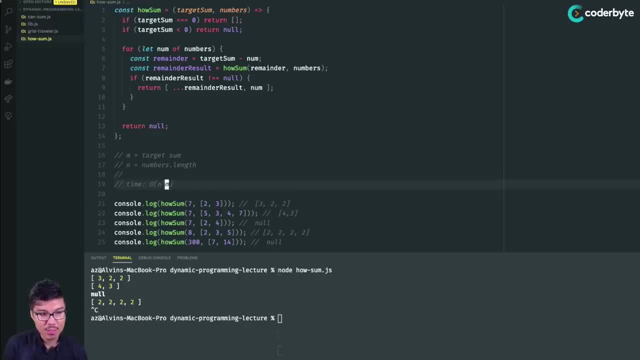 it looks like it's going to be the same time complexity as last time for a brute force, So it looks like we have some additional time that we consume in this function, really coming from this expression, right? So if I look at line nine, in particular this line, 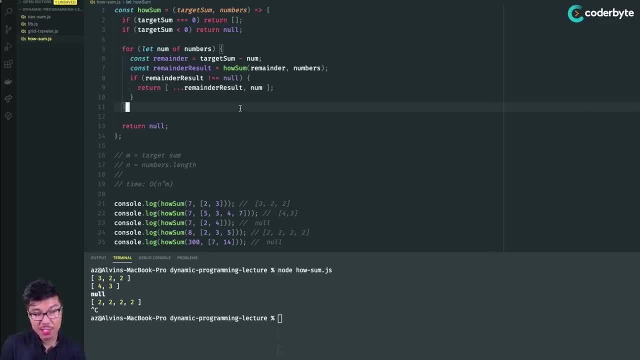 creates a copy of an array. So that will actually take sort of a linear number of steps to copy over every element of an array, right? So I will have to consider the cost of this operation. it's sort of under the hood like iterates through the remainder result, And I know that. 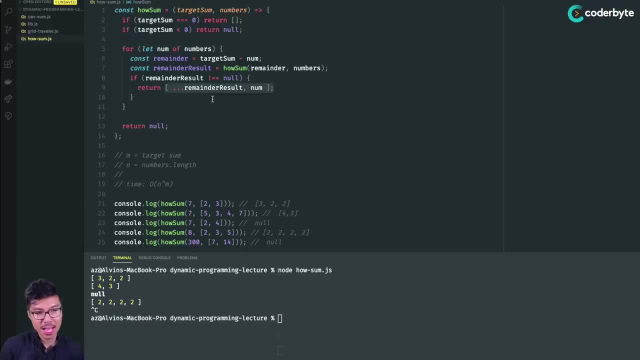 the maximal length of the remainder result is going to be m times m And that's going to be the maximum length of the remainder result I can get back will be, at most, m right, Remember that remainder result in the worst case is going to be an array the longest. 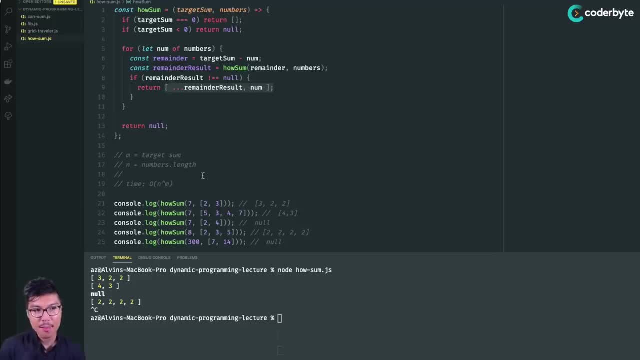 that array could be is exactly the target sum, right? Imagine that we had the most simple you know sort of combination to generate the target sum, if it was just a bunch of ones, right? my target sum was 50. And I had an array filled with one that I can just. 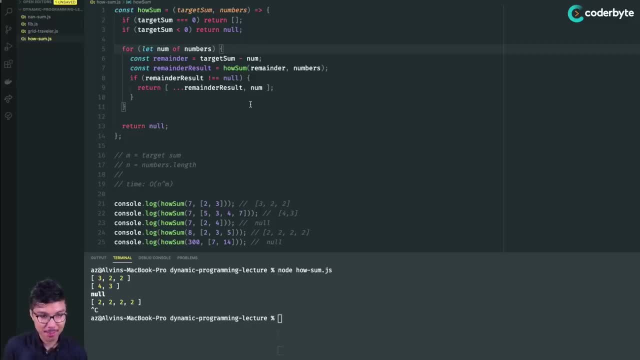 do one plus one plus one plus 150 times to generate the target sum. So in the worst case, this copying operation will take m steps, and I need to do that for every recursive call, And so if I have this many number of recursive calls in addition to that, I do. 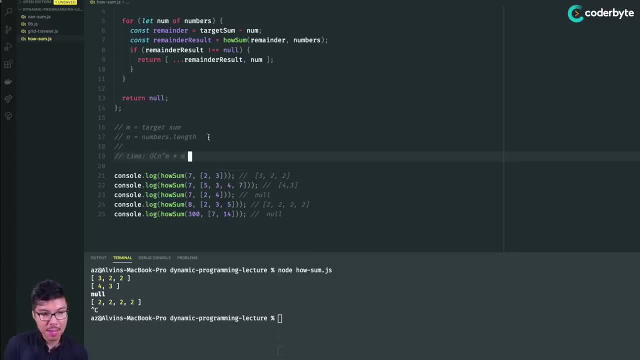 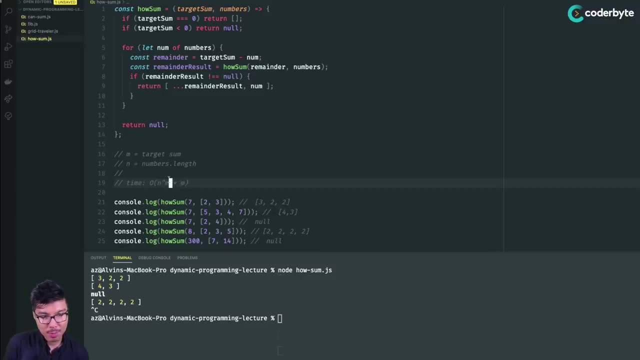 an M operation. you just multiply that m right? So the time complexity for this brute force so far is n to the m power times, m. Really the thing we want to optimize the way is this exponential part right? So I really want to focus in on that. But while 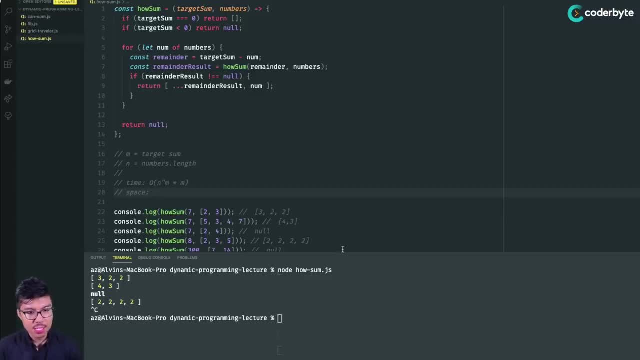 we're here, let's go ahead and talk about the space of this brute force. So the space, the few things to consider, the terms of the stack space. it's going to be the same as last time, So it's going to be O of M, But think about any other space I use up, I guess. 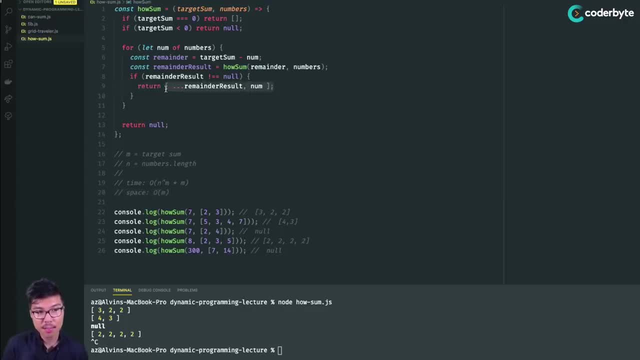 you could also consider the array that you return back. However, we know that we're going to return back like the first array that we find all the way back up to the top level call, And the combined length of all of those arrays that we return is really just going. 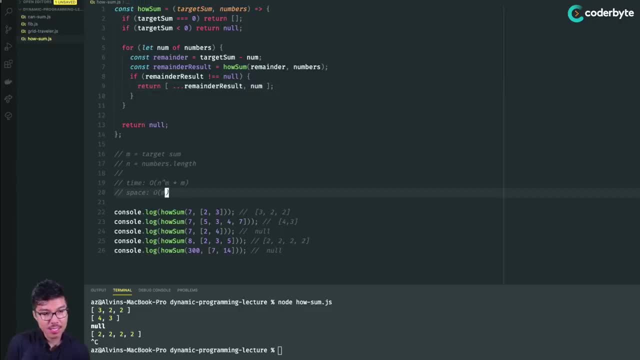 to be, in worst case, m right. So I would still say that the space complexity, which, for this function, is just m right, now Cool. Obviously, let's work on optimizing this time complexity. So this was the brute force. So brute force, and you guessed it, and there, 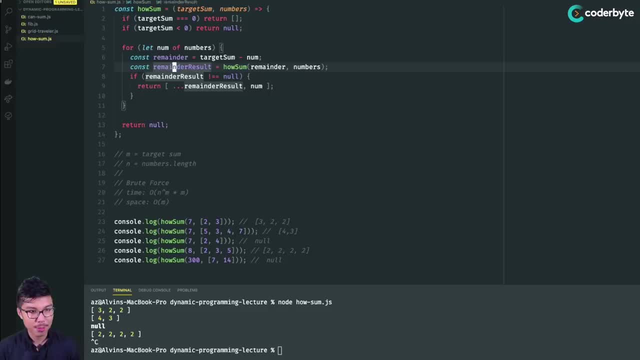 is definitely some duplicate sub problems in this brute force, So we'll just memorize it away. So very formulaic stuff. Most of the work is always the brute force. So I'll start with my empty memo object And, like we always say, we'll use the target sum as 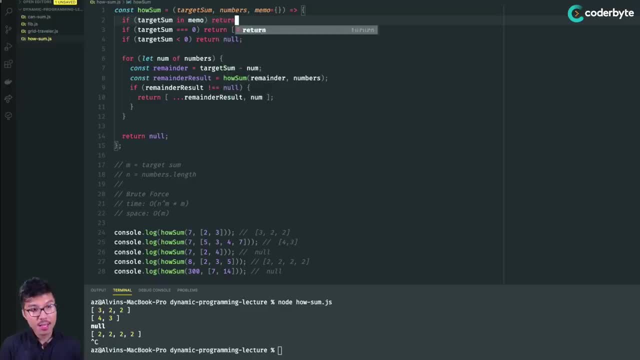 our key Before that is, if it's in the memo, then I'll return what I have stored in the memo And at this point what I want to do is make sure I pass along the same memo. object to all of the recursive calls. that way they can benefit from any information or any sub problems. 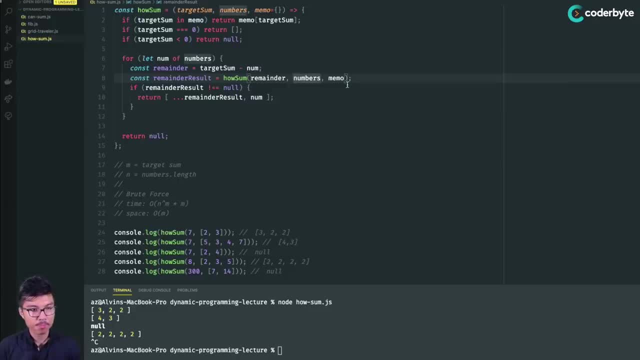 that I worked on over here right in this stack frame. Cool, At this point I need to make sure that I take all of the return lines that I had before and I store them in the memo right? So the trick here is I can say memo. 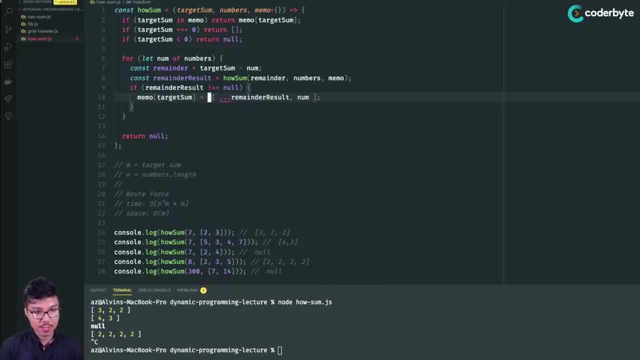 of target sum. I'm going to save that array. So notice that now the values in the array, or sorry, the values in the memo object, are going to be arrays, because that's the return value of this. it's either going to be an array or null, right? So I'm just going to 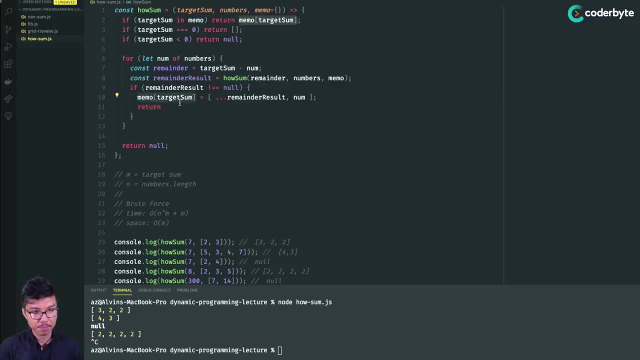 complete this return value by returning what I just put in the memo. And in a similar way, I also want to memorize this late return, So it will also be memo of target. sum equals null. Cool, So with that change right, it's very, very straightforward change. Let's see how. 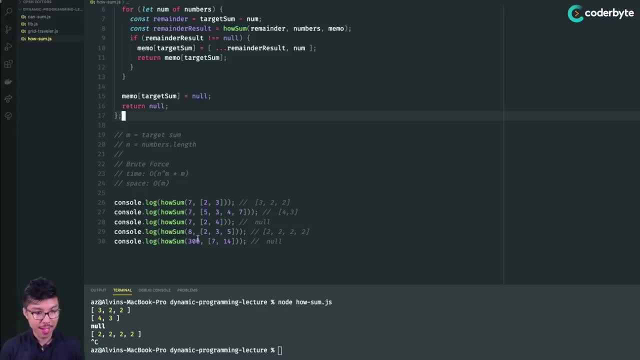 this does. Now I know that for this last example of how some 300, it is not possible to generate the sum of 300 using just sevens and 14s, So I should get a null for that one. So let's give that a shot. Nice, And there we have a really quick running a null of that. 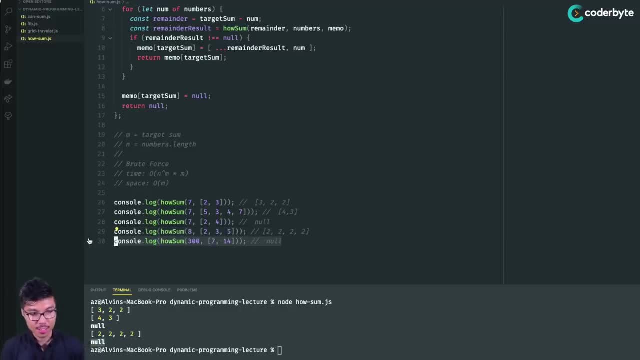 very last example. So we definitely had an effect on the runtime here. Let's talk about how we changed the complexity of this code. So that was a brute force. Let's talk about the memoized version. So what's good with the time over here. So we know that in terms. 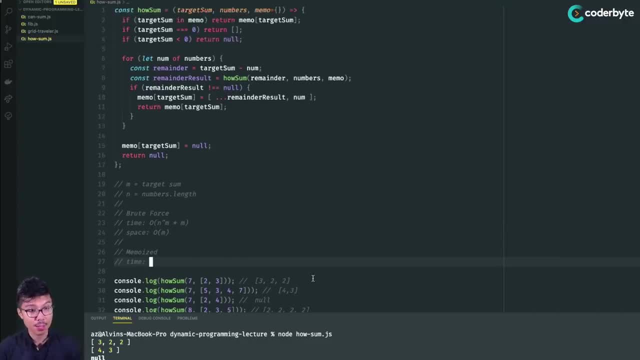 of the time complexity from the number of recursive calls that we make. it's the same story as our last problem. right, We just have to consider any other time operations, which would still be this array copying. So, but in just terms of the recursive calls that. 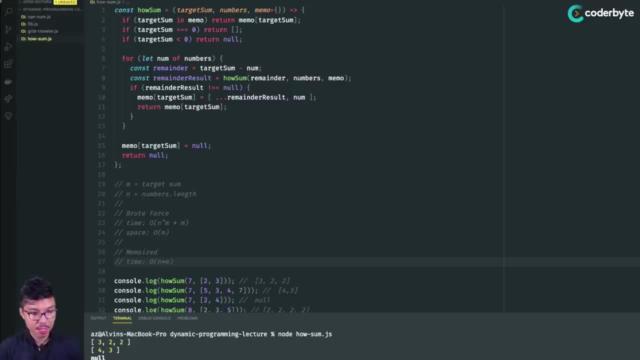 we make. it's going to be n times m Our recursive calls And then in each recursive call I need to do this copying pattern right, copying over the contents of an array, and the array will be, at most, m elements long. 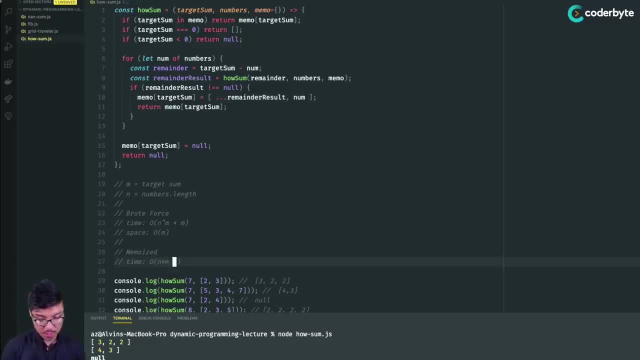 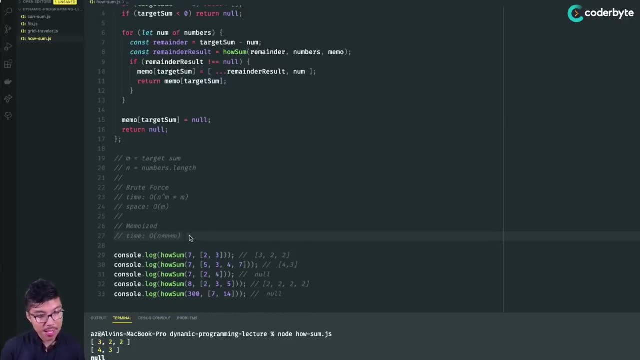 right. So if I have this many recursive calls and each recursive call needs to make an m length operation, that I just multiply by another m term. So right now this looks like n times m times m, which is the same as n times m squared. And now let's talk about 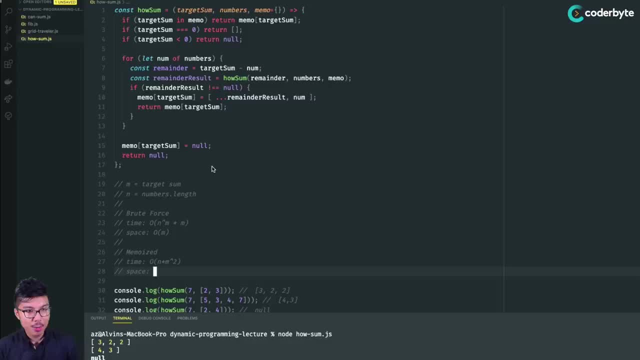 the space complexity. So the space complexity will be at least as big as our brute force. So it's going to be at least O of m. But now we have to consider all the space we use up in the memo object. So I think about the keys of this memo object. the keys are just going to be all unique values. 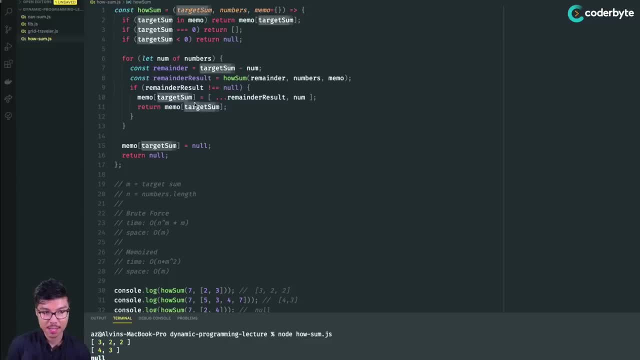 of target sum: right, Because I just literally use target sum as a key on all these lines, right. But then I have to think about the value, right? the values are going to be pretty chunky now because of sometimes a value. 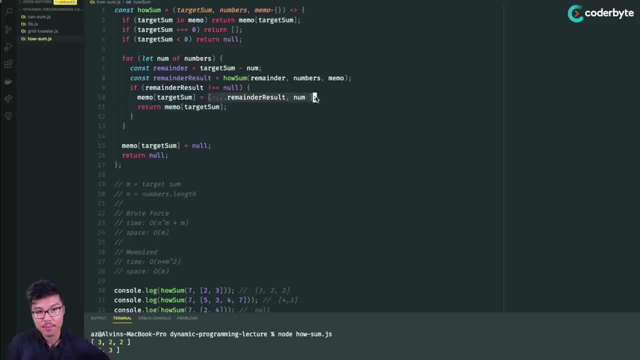 But in the object is going to be an array And I already said that the maximal length of any of these arrays that I return is going to be of length m right. So to me it's now the case that your space complexity comes from mostly your memo object, which is going 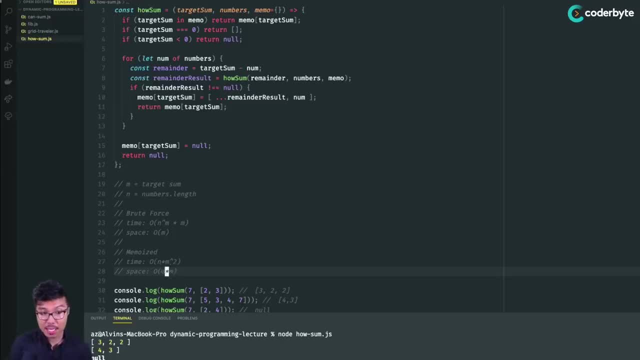 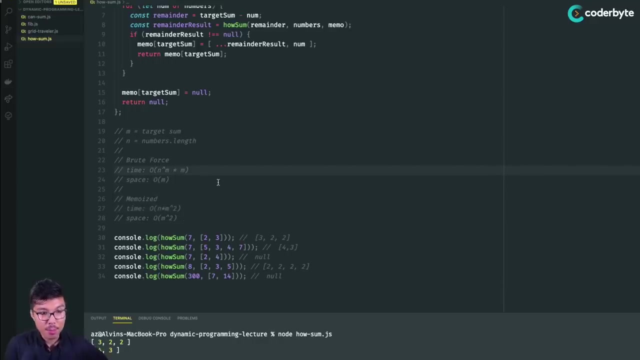 to be of size m times m, right, because you have m keys And each key has a value which is, at worst, going to be an array of m elements. So it's m times m, which is m squared, Cool. Well, notice that we definitely cut down on the brute force implementation, especially. 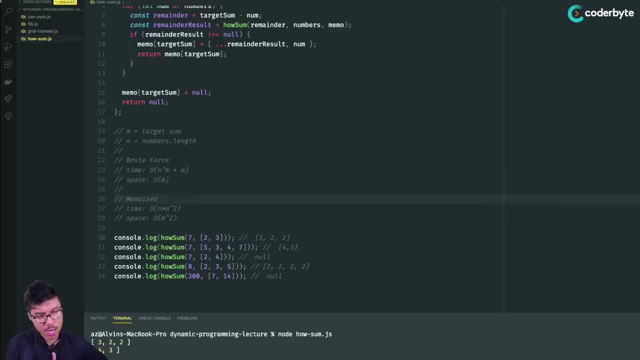 in terms of the time complexity. obviously there's a little trade off that we made here, But now we're able to run our house some function in a reasonable amount of time. So to wrap up this problem, let's go ahead and hop back into the drawing board. Alright, now that. 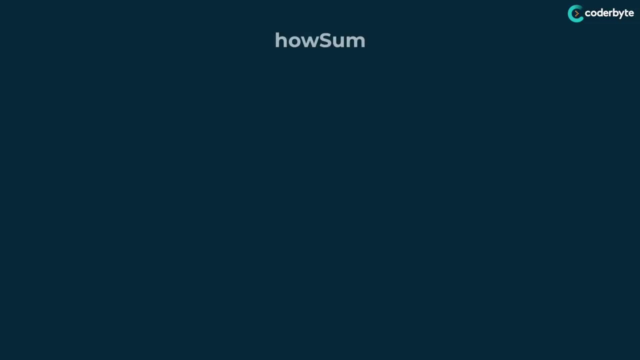 we coded the How some problem. let's wrap it up by actually analyzing the complexity of it. So recall that for our How some problem we have multiple arguments right, So I need to describe them. So I'll say that M is my target sum. 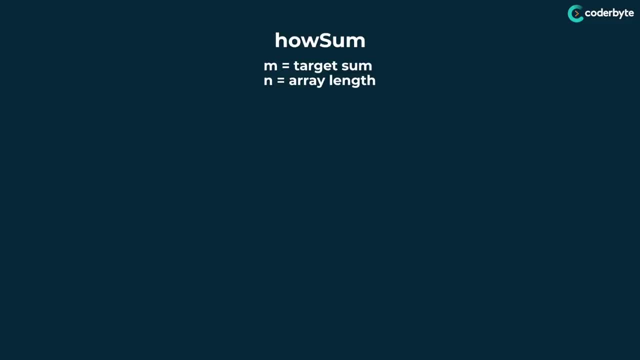 and n is the length of the array. Remember that the array contains the choices we can take And our baseline solution, that is, our brute force. recursion had an exponential time complexity right. it was kind of in the form of n to the m, power times, m And after we. 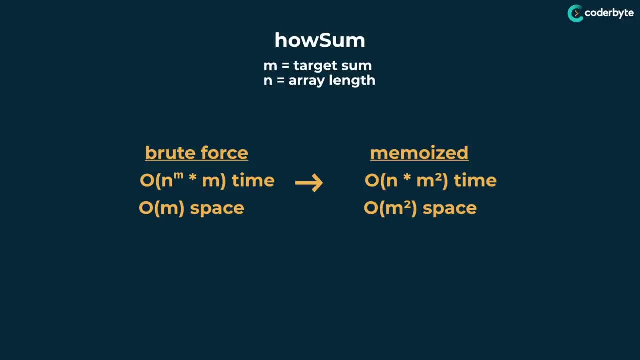 actually optimize it. using the memo ization strategy we actually reduced it from exponential down to a polynomial time complexity. In particular, our new time complexity was n times m squared. So really important fact about our memoized time complexity is it is no longer exponential. 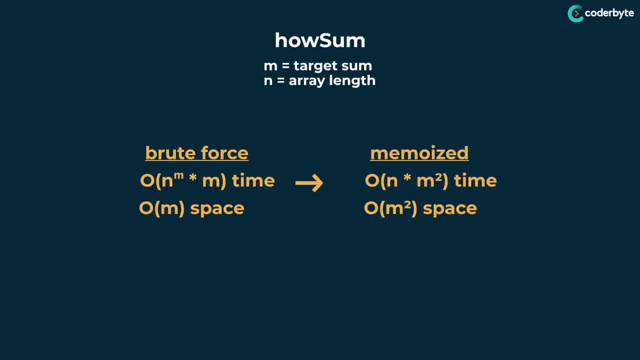 Please recall that when we have m squared, that is not exponential because the exponent is a constant number. Cool, If I look at the the space complexity. for this I had to actually pay a little more cost in terms of the space because of the memoized object, But that space 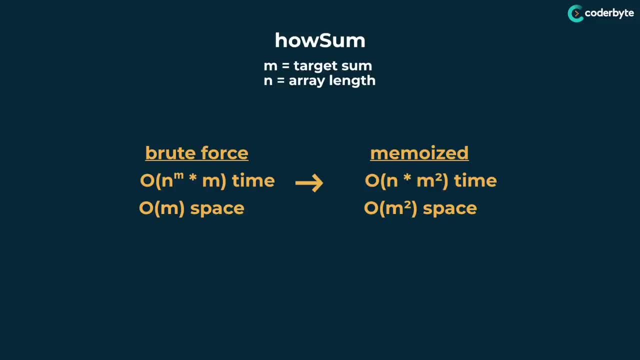 complexity we use up is still not exponential right, still a polynomial or quadratic complexity. So I'm still satisfied with it overall. So we definitely prefer this memoized complexity over the brute force. Alright, that was the how, some problem, but now let's go over one more variation of it, And this problem I'll still give you. 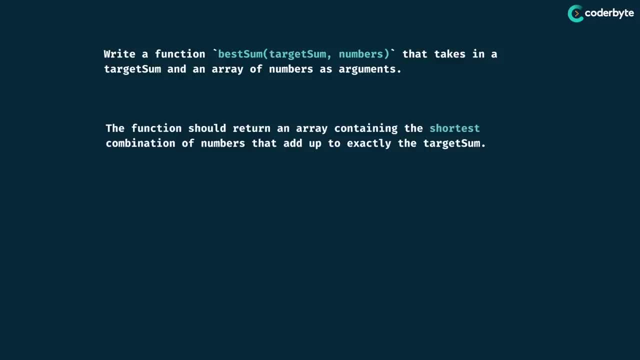 a target sum as well as an array of numbers to choose from, But this time what you want to do is return an array containing the shortest combination of numbers that adds up to the target sum. Along with that, if there's any ties for the shortest combination, you can. 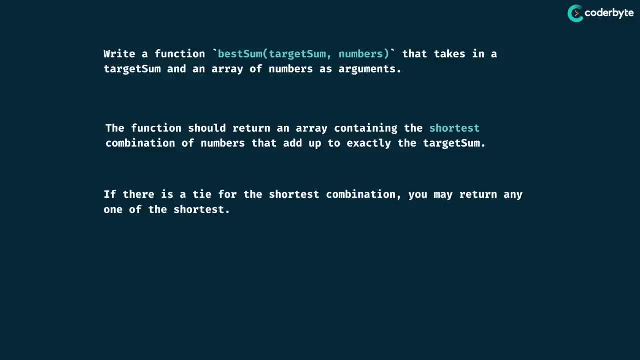 return any of those shortest ones. So from this description you probably recognize that this is similar to our last two problems. But now they're asking for a little bit of an optimization, right? So I want the shortest sum, So that means an array containing the least amount of numbers, but it still. 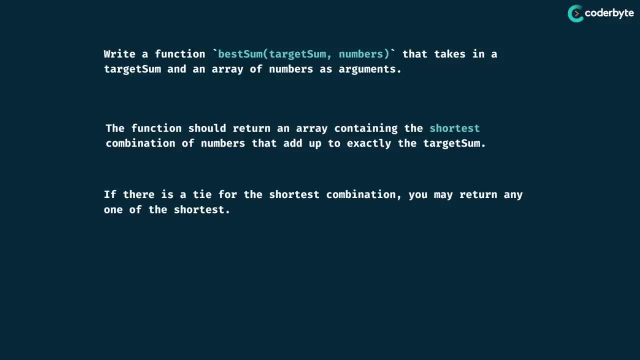 adds up to the target sum. So we're really just going to add on top of our previous understanding. Let's take a look at a few examples. So let's say I gave you this example, So here my target is seven and the numbers I choose from are 534 and seven. So there are a few different. 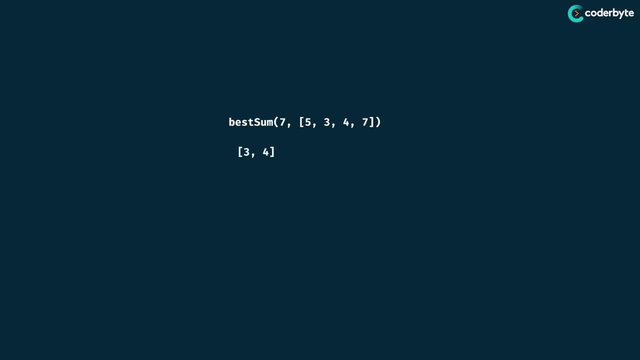 ways you can generate your target of seven. one way would be to do three plus four. that's one combination. But another way would be just take the seven, because notice that seven is actually a member of the array. And here I want to. 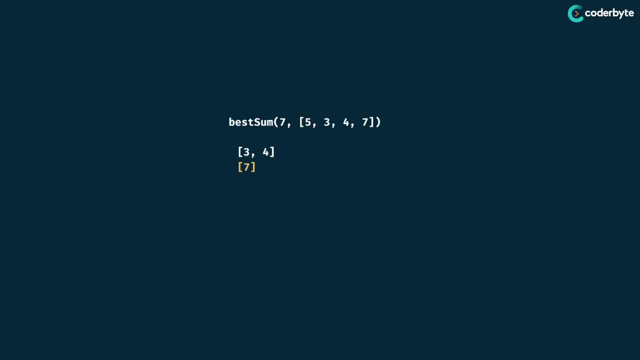 choose the smallest array, which would be just the lone seven. So that would be the expected result for this one. In a similar way, let's say I gave you a target sum of eight and your choice of numbers were two, three and five. there are plenty of ways. 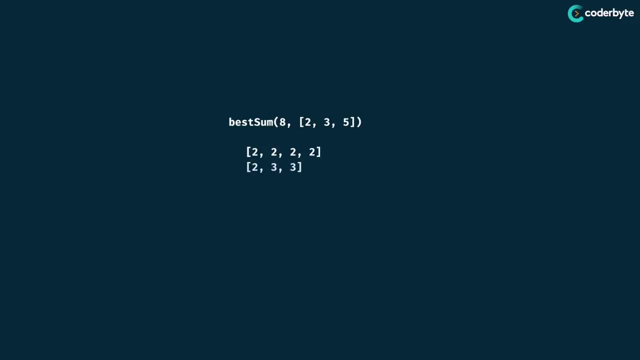 to generate eight. you can do two plus two plus two plus two, or you can do two plus three plus three, or you can just do a three plus five, And here I want to return always the shortest combination, which would be the three plus five. So that will be the result. 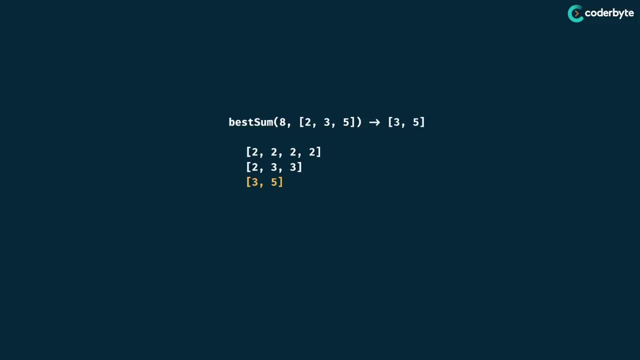 over here. Cool, So we definitely have some awareness that. alright, this problem is similar structure to our previous one, where I need to sort of generate a way to make the target sum, But now I want to really specify the shortest array, right? So let's try to visualize. 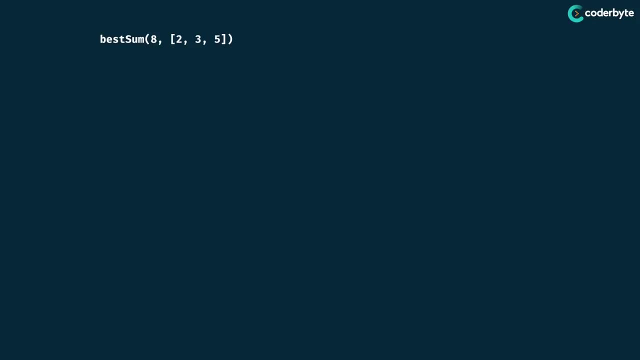 this as a tree, like always. let's say, we're stepping through this example with the target sum of eight, So we know that the full tree would look like this, And we've seen this tree before, But now what we're trying to do is come up with a different process for 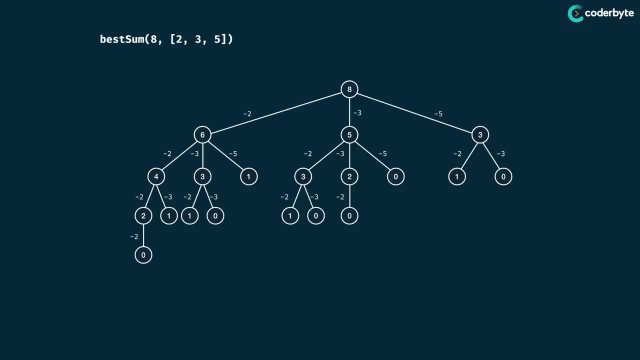 the value you return right No longer going to be valid. to just return the first way that I find to generate the target sum. Now I want the best way, So let's start coming up with the strategy for this. At this point, we know that we can definitely implement some logic in our code where we 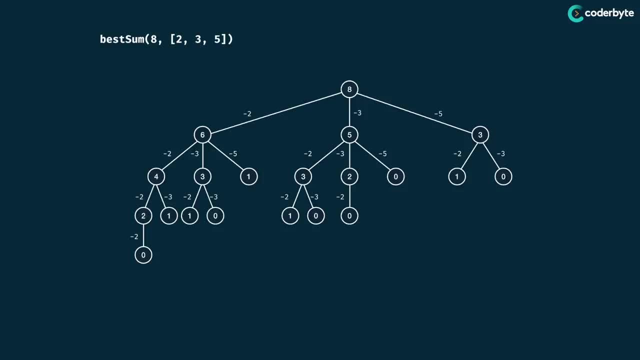 return an array up our recursive calls. we did that in the last problem, So here we'll sort of use some abstraction to assume some return values. So let's say that I'm breaking this problem down. my top level problem asked me what's the best way to generate eight. 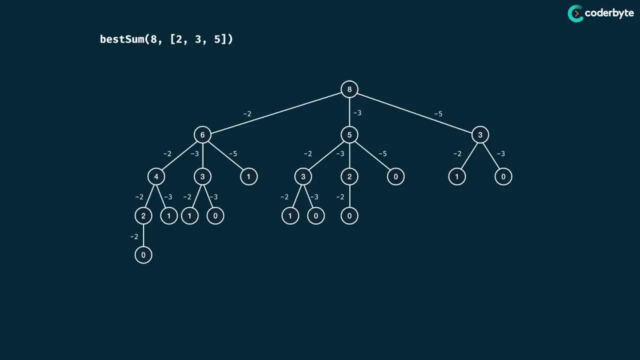 But I see that along that path I have to find the sub solution for the best way to generate six. So let's say we're rooted at the subtree And we know that there are a few ways we can make six right. If I look at this subtree, rooted at six, there are 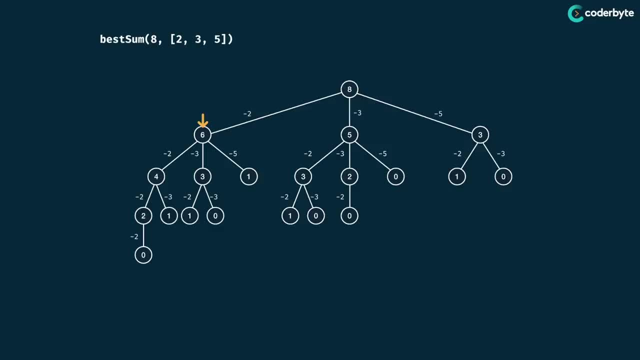 two zero base cases. you know downward right. So if I look at the first one, I look at this path, I know that my subtree over here we'll be able to know that. all right, one way to generate six would be two plus two plus two, right? we kind of implemented that logic in. 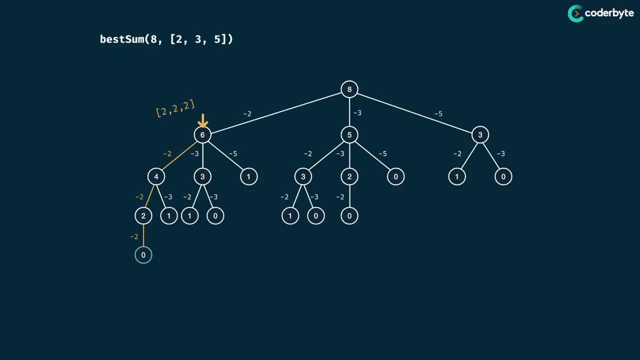 the last problem. But now what I also want to do is consider any other paths in case they end up being shorter. So let's say I want to generate six. I want to generate six here, obviously I know that this path of 33, or to return upward, And now I have to. 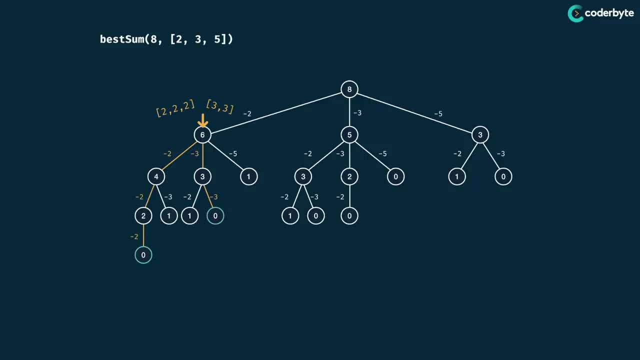 kind of make the decision, you know, between these two options for generating six, I should just prefer the shorter one. So that means it's sort of 222 versus 33.. And obviously the 33 wins because the array length is shorter. And if I pause right here and I look at what, 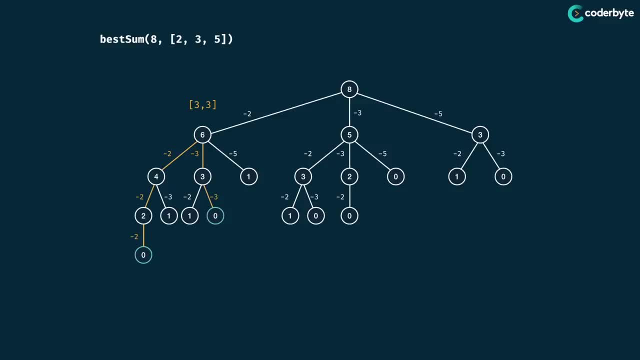 the diagram is saying, it does make sense that above the six we have three comma three, because that is the shortest way we can ever make a six right, just three plus three. But now I can return this subarray to my parent. But if I do that, I should also include 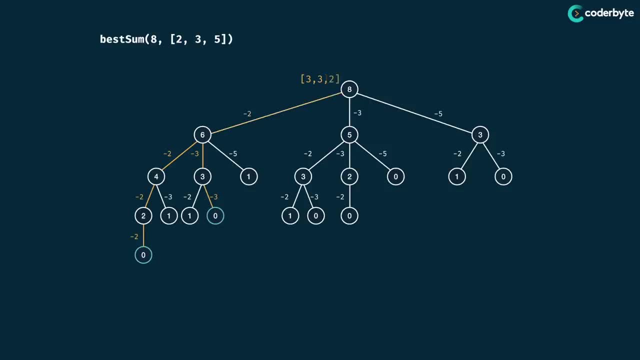 the value of the edge along that path, right. So I also included the two over here. Now this makes sense, because one way I can generate eight is three plus three plus two. right, But we know that's not the optimal way. Let's say we step through this a little further. 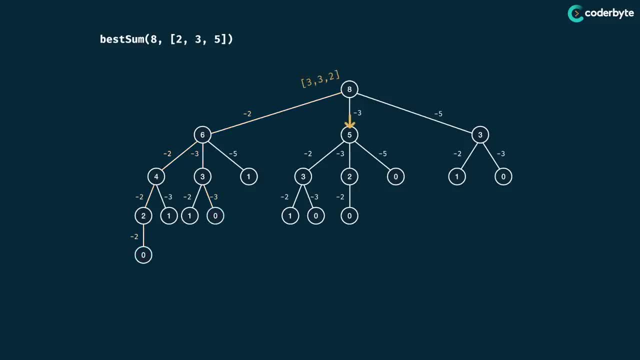 Let's say we took the same sort of process for this other child of five. So I know that to generate five there are three options according to the subtree right, Because I see different leaves that have zero inside of them, And so I know that for these paths, 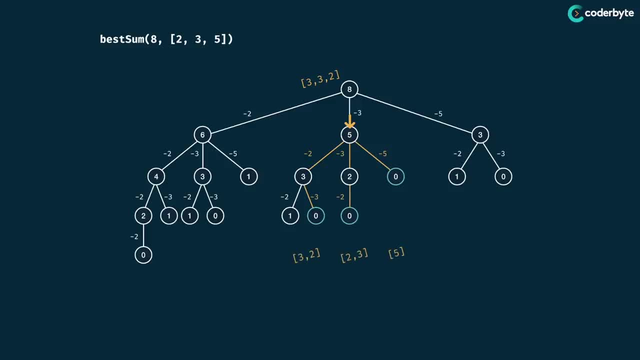 they would work out to their own subarrays. And here I really just want to choose the shortest one, right? So obviously the lone five wins out over here. So that'd be returned all the way up to that five node, But then that five node will return it to its parent. 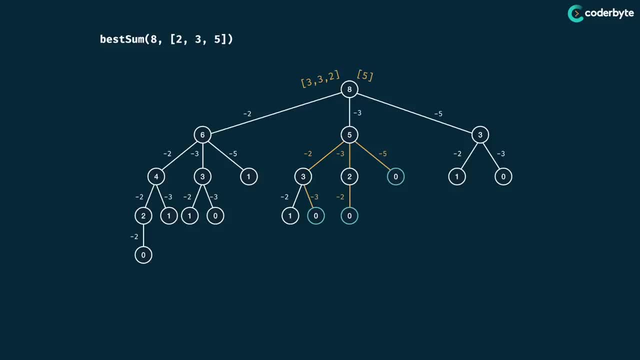 Then of course, I need to include the edge that connects the eight to the five, right. How did I transition to that five in the first place? So I go ahead and just add it in. And now the root node Over here has a decision to make. which one does it prefer between 332 or 53?? It'll just. 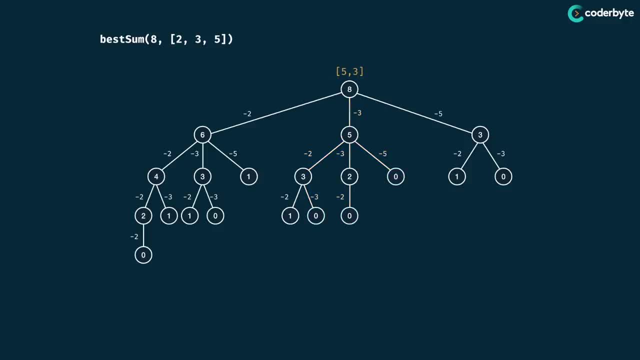 choose the shorter one, So the 53 should win out over here And I just need to continue this process for any other branches in my tree, right? I can't return early and this type of problem because I need to find the optimal way and I can't be sure until I've 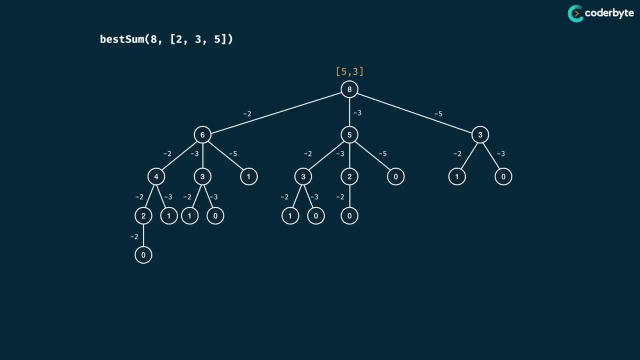 tried every possibility. Cool. So it looks like our overall logic is we want to explore and find any ways to generate our target Some, but then when we find a way that shorter than our currently tracked way, we can just replace it. I'll continue that process through the entire tree If I check every possibility. 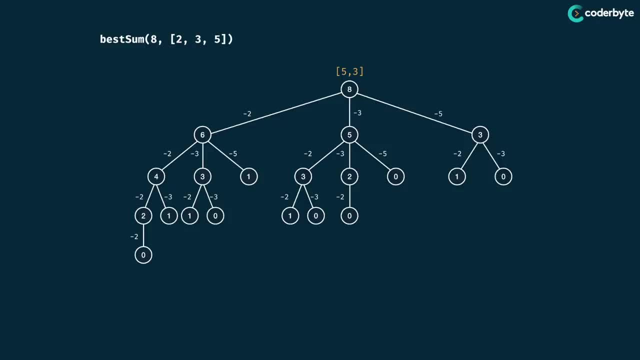 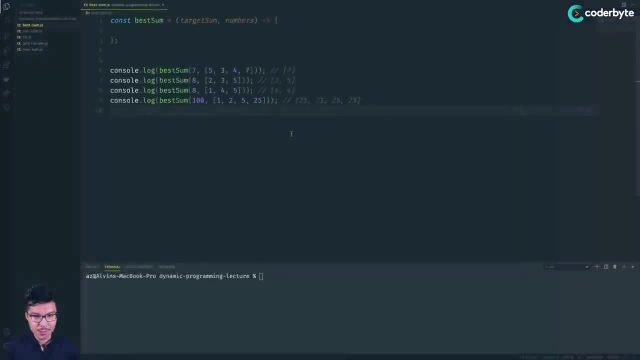 and keep replacing what I consider the shortest. by the end of us exploring every branch, we would have the absolute shortest. All right, I think we're ready to hop into the code. All right, programmers, welcome back to my text editor. Let's work on coding this one. 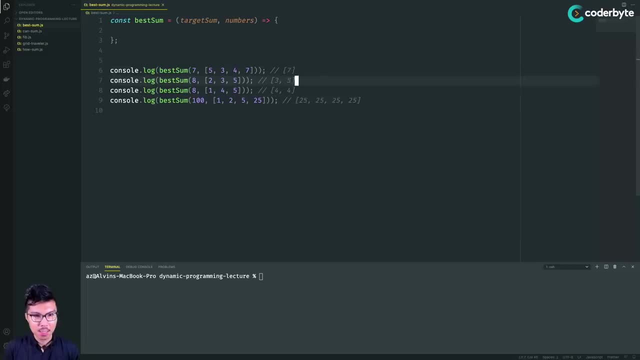 out. So here I have some initial examples that we'll use to test our best sum function. I noticed, for this last one right, I give my initial target sum of 100.. And the best way to do that is obviously just take a bunch of 25 right for 25.. And what I also want to bring our attention to is this third: 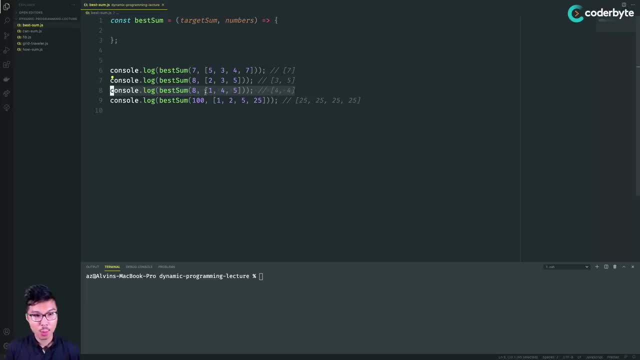 example over here. So my target sum is eight and my choice of numbers are one, four and five. The optimal answer here is four and four. right, That is the shortest way to generate eight. A common mistake I see a lot of students make is sort of assume that the best way to 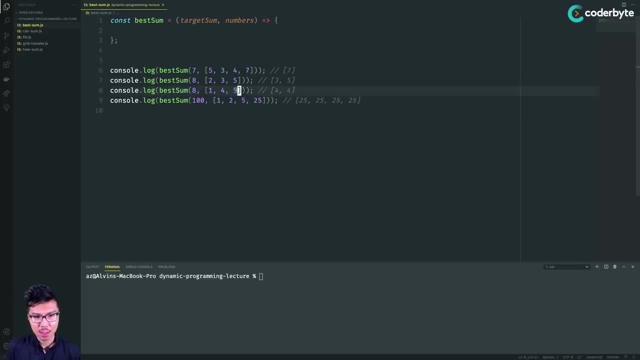 generate the target sum always involves taking the largest choice of number as many times as we can right. That is not true. If you took a five, a one, two, three and a three in your your sum, then you would have to take three ones. 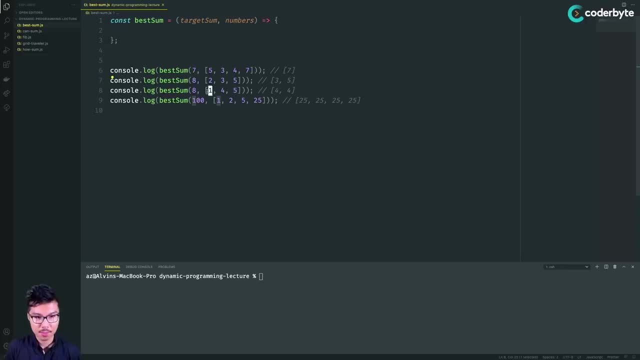 in the long run, which is not going to work out to the shortest answer right. So it's not the case that just taking the biggest choice of number always yields the target sum in the shortest amounts of numbers overall. so don't fall into that trap, which means 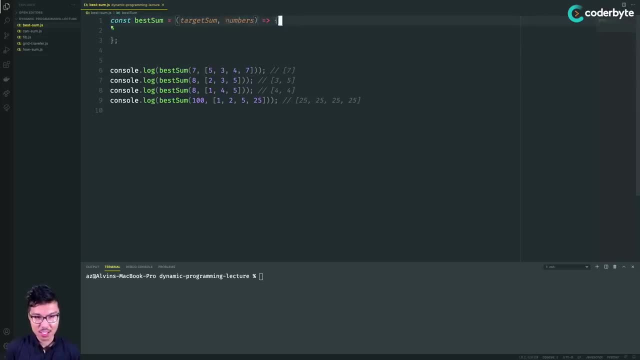 that we have to do the full tree exploration right, we have to do an exhaustive sort of search using our recursive code. So let's start with that base case, like we always do. So we're in this a few times, but still right here. So if the target sum is zero, then I 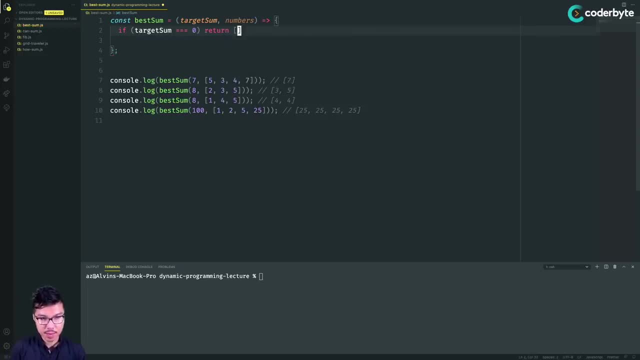 have trivially solved the problem, So I can just return an empty array. right, That is the exact single combination and the shortest combination that can generate the target. So cool. Along with that, let's handle that scenario if our target sum goes too far downward, so if it's less than 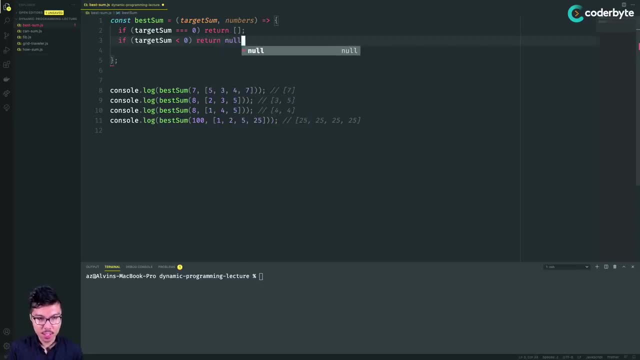 zero. so if the target sum is less than zero, I'll just return null, meaning that's not possible to generate that target sum. And now we'll use our branching logic. So I'm going to iterate through all choice of numbers. So I'll say: for, let's numb in numbers, And like we always do, I'll go ahead. 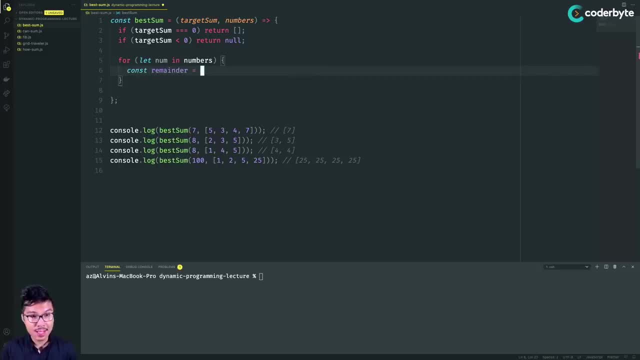 and create my remainder, which I know would be the difference between my target sum and that choice of number. Alright, so what I'm doing is I'm choosing the number and that decreases my target sum. At this point I would make my recursive call right with that remainder passing in the same. 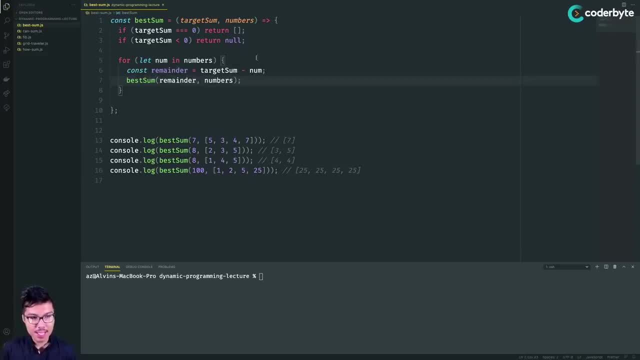 numbers array. But now I have to do some thinking. I know that, alright, best sum is either going to return to me a combination or an array, Or it's going to return null. So I'm gonna have to kind of differentiate between the two. So over. 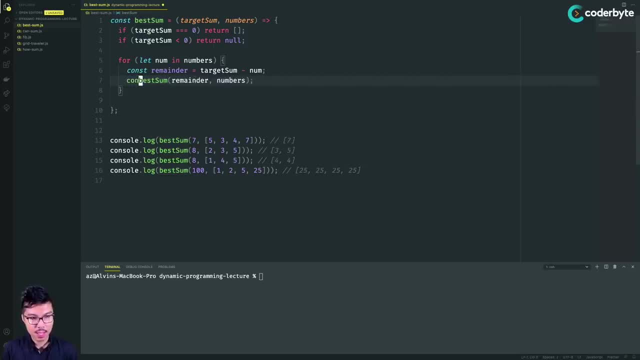 here. maybe I'll just save this. as a result, I'll call this my remainder, let's say combination, And if this remainder combination is not null, then I can do some other logic right? So I'll say: if the remainder combination is not equal to null, then do stuff. So if I enter this, if statement, 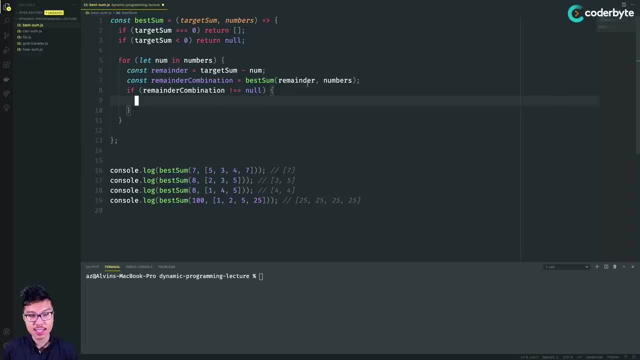 then that means it is possible to generate the remainder. And exactly what remainder combination is is an array containing the shortest way I can generate the remainder. Cool, So if I enter this if statement, then I also have a way to generate the full target. So right, I can just take the remainder combination. 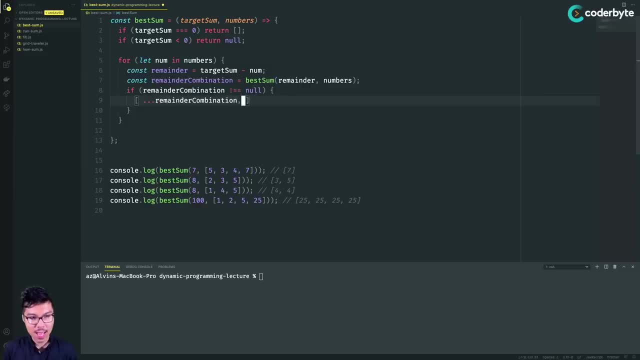 copy the elements over from it, like we did last time, and also add on the choice of number I just took right. So this would be now a complete combination for target sum. So I'll just save that as a regular combination. Cool, So so far. this is very reminiscent to our last one And we need to. 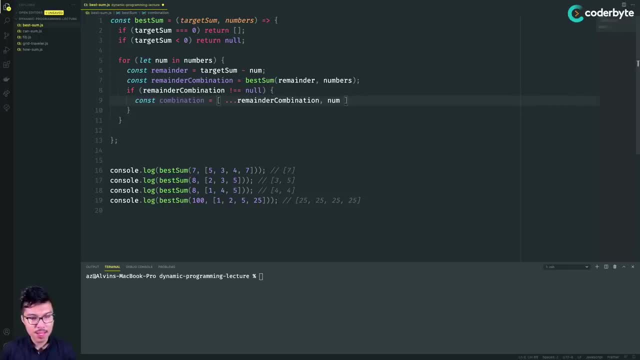 work in some more logic relevant for this problem. That is a very, very important characteristic that we need to implement. in the tree was I need to sort of choose the shortest combination, right? So I'm going to need to work in that logic. So here's what we can do. I know that I need to. 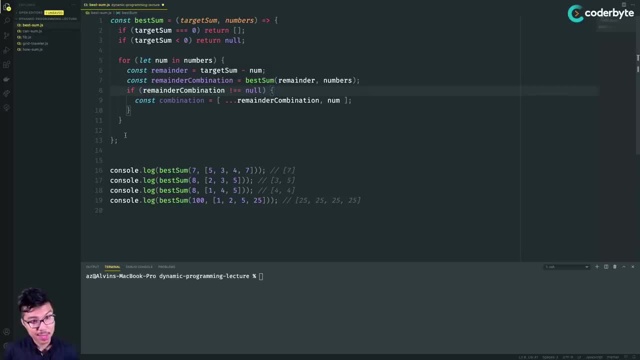 compare basically all of my branches together, all of my recursive calls together, and pick out the shortest combination. So I know that this for loop is the piece of code that sort of iterates and attempts all of my branches, And so outside of the for loop I'm going to need some outer variable. 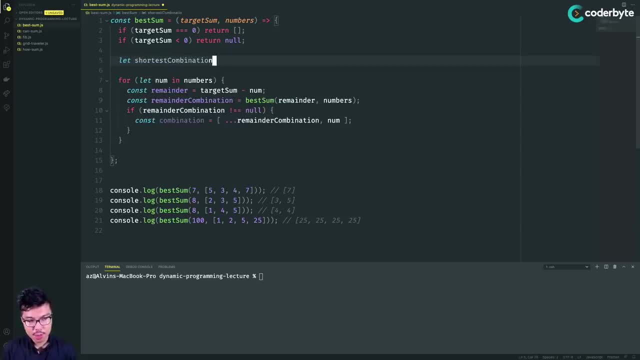 I'll call it my shortest combination And over time I'll just keep updating this variable if I find a combination shorter than my current shortest combination, right? So I'm going to initialize this to null, And the reason is: imagine that we set up this shortest combination variables. 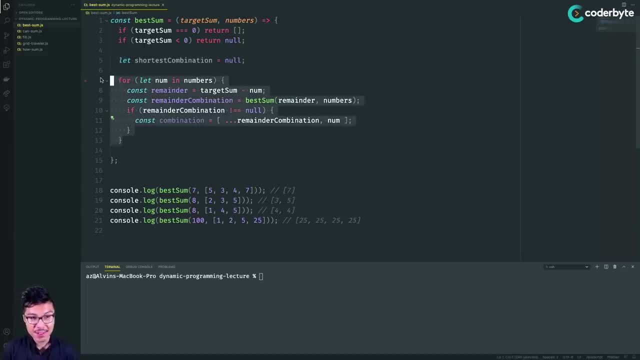 and then we iterate through the for loop and there isn't even any way to generate the target sum. So this for loop finishes and shortest combination would still be null, And that'd be great to return right. Because in this problem they said, if it's still not possible to generate 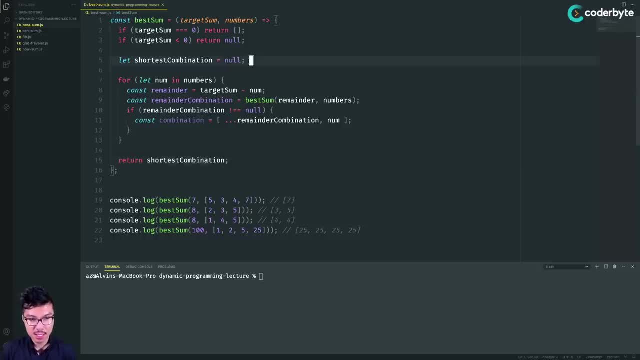 the target sum at all, you should still return null. So this is a good initial default value for shortest combination. But now I need to do my update logic. So here, on line 11, I've actually created a combination that gives me the target sum. 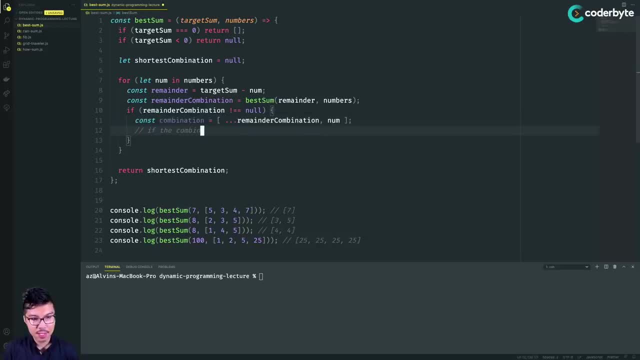 But now I need to check right. So I'll say: if the combination is shorter then the current shortest, then I need to update it. So it's translate that into some code. just use an if statement And I'll start by checking if the 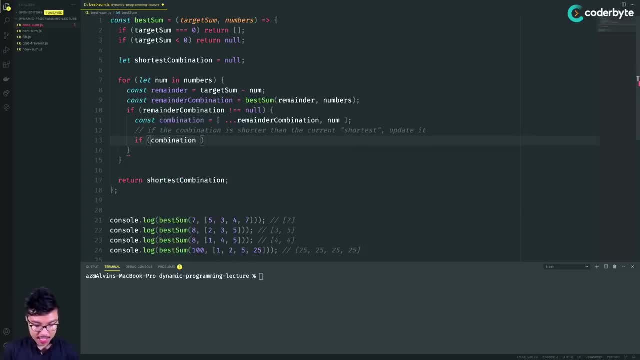 combination that I currently have, which is an array- right, I check if that is less than in length, then the shortest combination variable- And really it looks like shortest combination- starts as null. So I need to fix this code up a little bit, But if I update it with a valid 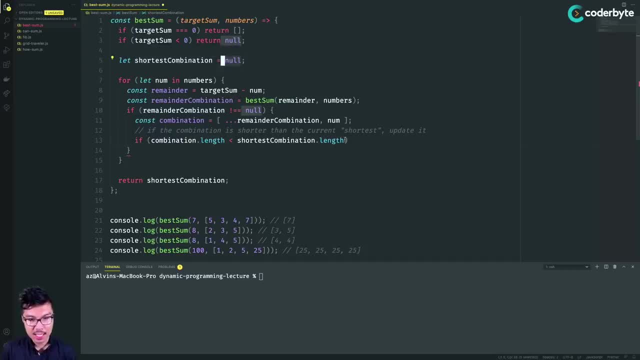 combination, then it's going to be an array, right. So I'm really checking the length of the arrays here. So what I want to do is assign my shortest combination with the combination that is now shorter. good, So this means the shorter combination wins out and gets to stay right, If I 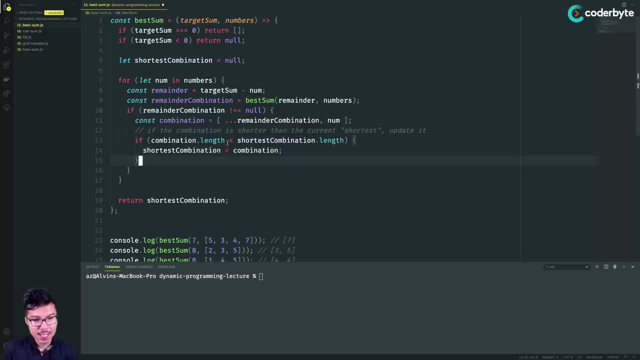 look at this code. it needs a little bit of work Because the first time I find some combination I know that I'd be comparing that array length to to null dot length. right, Because shortest combination starts as null and I can't do null. 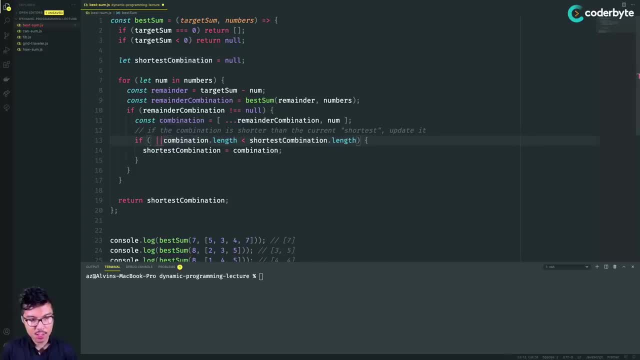 dot length in JavaScript. So I'll need to like a nice or clause here. So I'll say: if it is the case that your shortest combination is equal to null, then you can go ahead and replace it. Cool, So this sort of check over here is going to make sure that I automatically replace. 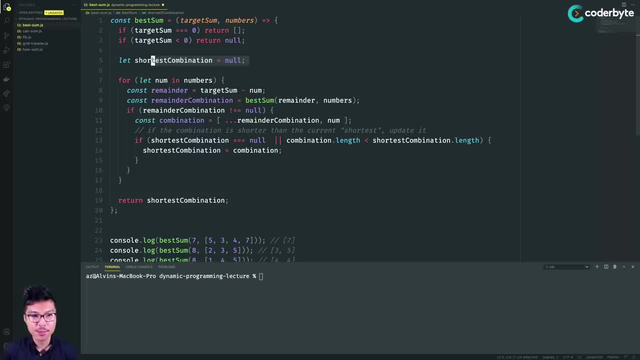 this null value with the first valid combination. Even if right now it may not be the shortest right. Later I'll compare that combination I have stored to some possibly shorter combinations. Cool, So this code is looking pretty good. Let's go ahead and give it. 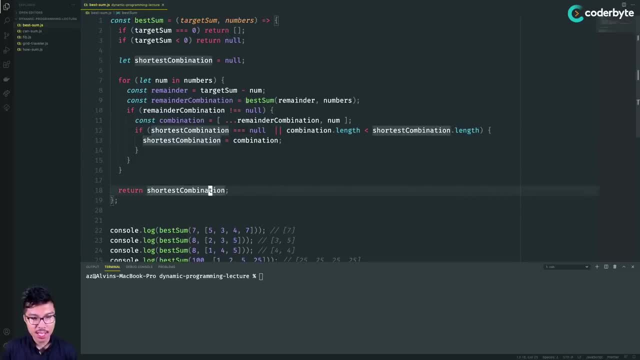 a little test run. Nice notice that on occasions where we call best sum with a remainder, that is negative because, remember, sometimes we subtract a num that is maybe too large. that's okay, because that will actually bottom out at a base case and return null. 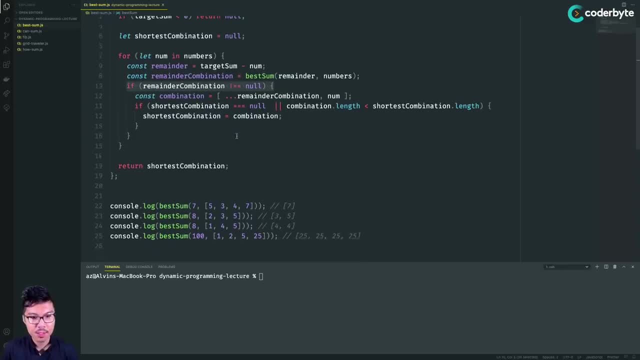 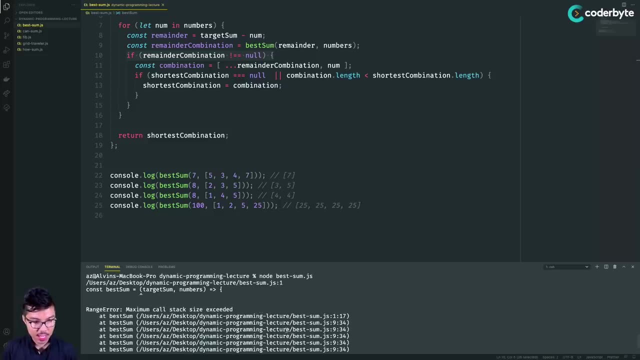 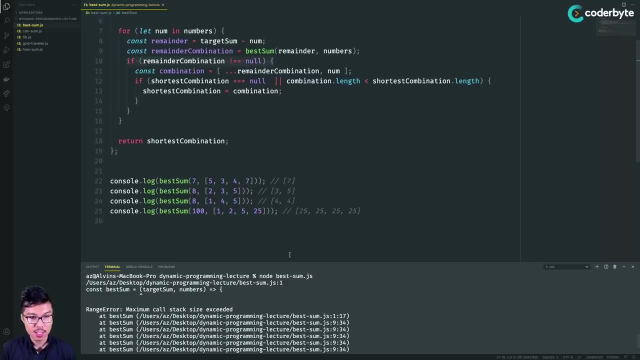 which we sort of check for explicitly in this if statement. Cool, So let's give this code a run. So node best sum. So I get an error over here looks like I get maximum call stack size exceeded, which means that we didn't really hit our base case. So there's some work to be done here. So 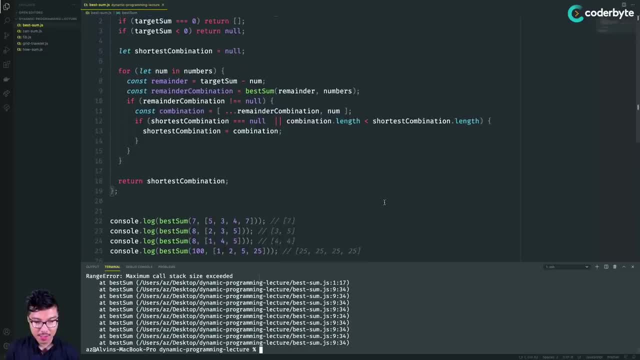 let's take a look at this code. So if I take a look at this code, it's a very, very small typo. it's kind of unfortunate that it breaks the entire code, But it's really. I messed up when I iterated. 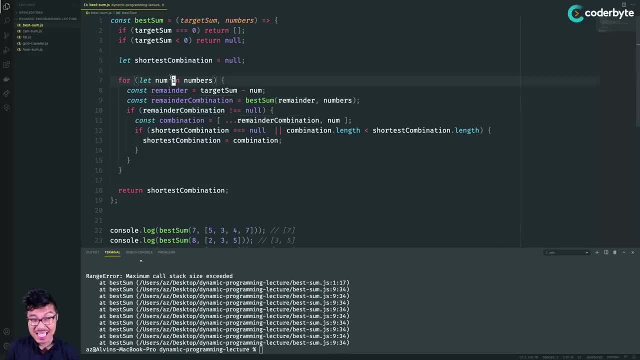 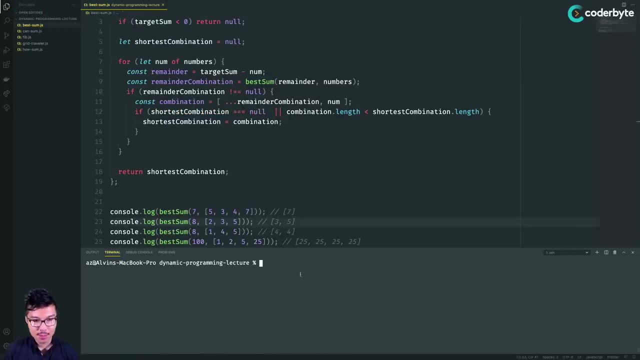 in the for loop over here. So here I wrote for letting them in numbers that would actually give them the indices of the array, So that'd be like 0123.. Whereas I want the elements of the array right. So instead of in any of over here. so that's on me. So with that small change, let's. 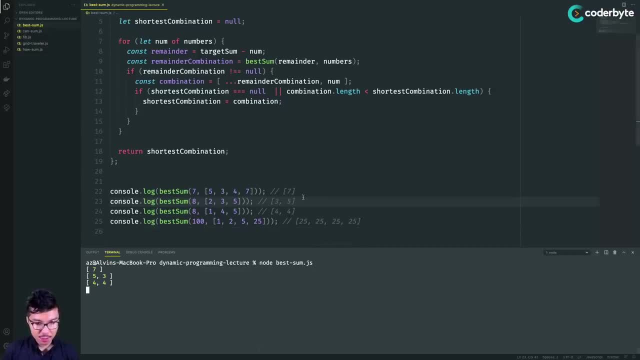 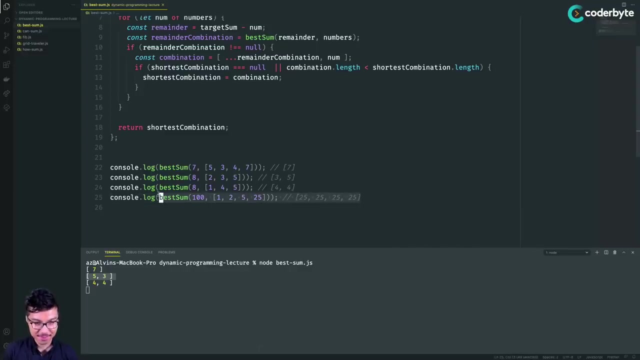 give it a run now. Yeah, it looks like we're passing these first three examples. we have 735 and four. four- notice that the order among the elements in the combination doesn't really matter too much, But looks like we're definitely a little too slow on this last example over here. 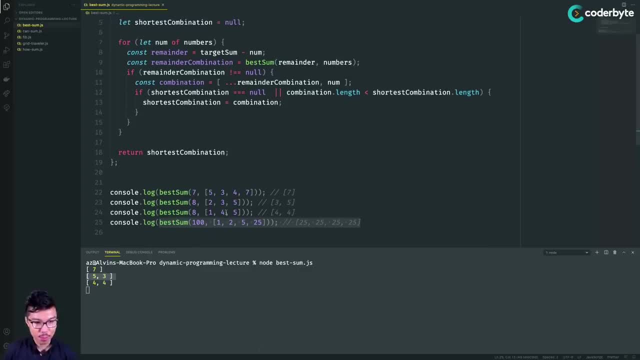 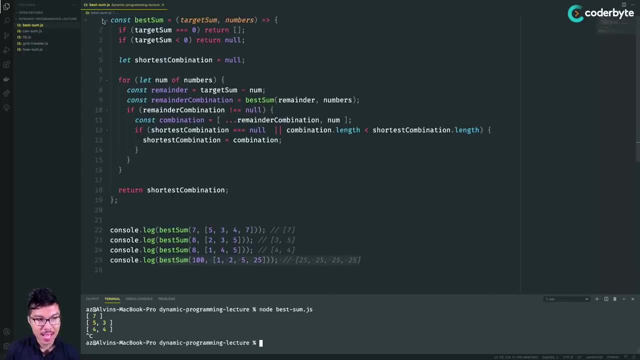 we know the move is to memorize this because we have the brute force recursion. But before we do that, let's just talk about the complexity of this. So this code is going to be very similar in complexity to our last. how some function. we sort of compare the two. it's. 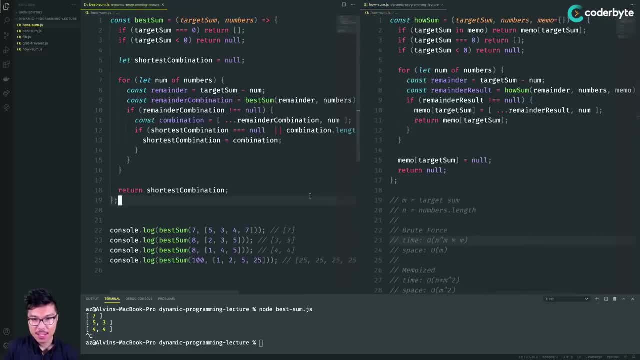 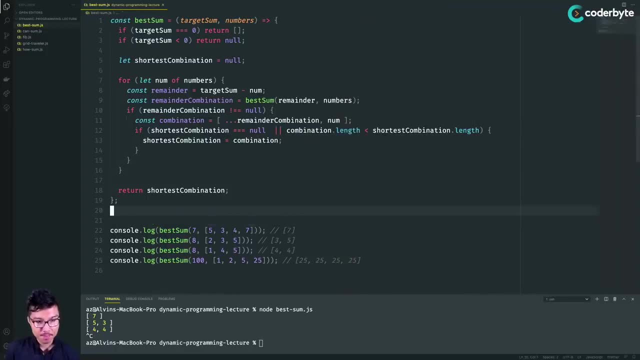 almost the same code, right? If I do these side by side, right? these two functions look very, very similar. So we know in the long run we probably have the same, or close to the same, complexity. Let's be methodical. So we know that over here we always like 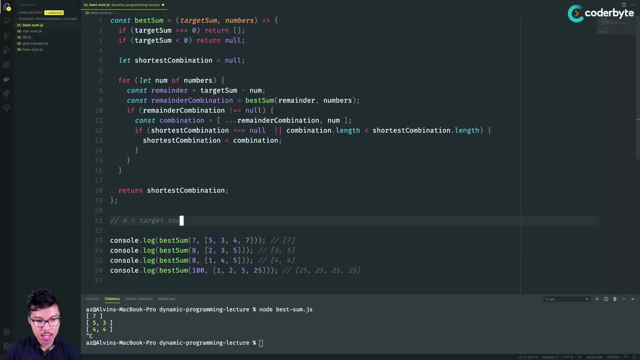 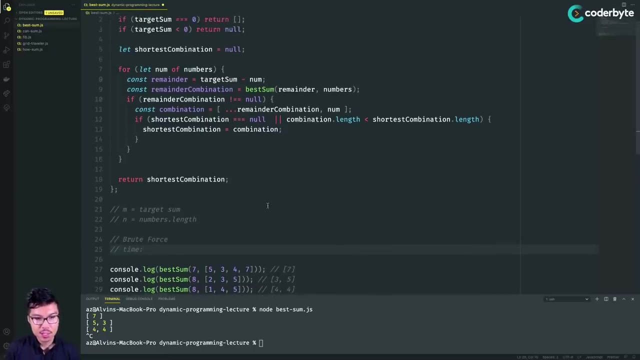 to say that m is the target sum, And we'll also go ahead and say that n is the numbers dot length. So we just did the brute force, And our brute force should be the same story as last time. So talk about the time. So the time of the brute force is going to be some. 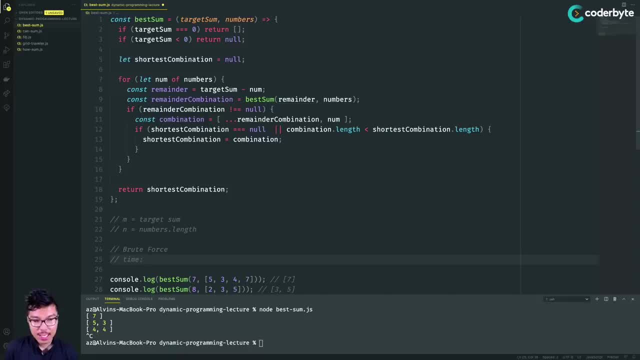 sort of exponential right. If you remember that tree drawing in general, the exponential number of nodes in a tree will be the branching factor to the height power. So now that the branching factor here is n right, I branch for every choice of number. 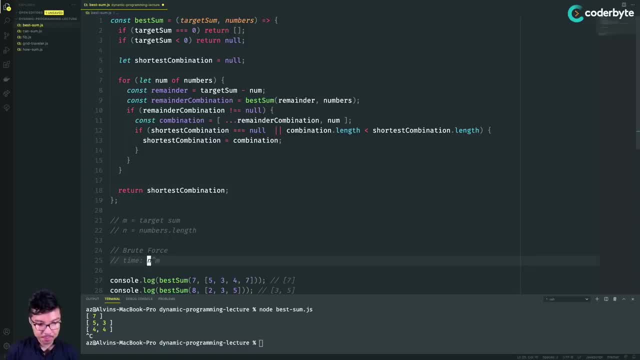 And then the height of the tree would just be the target sum. So that's n to the m. But along with that we also have some additional operations, right, If I look at this for loop. so this for loop gives me the branching factor right, But then I also do this operation on. 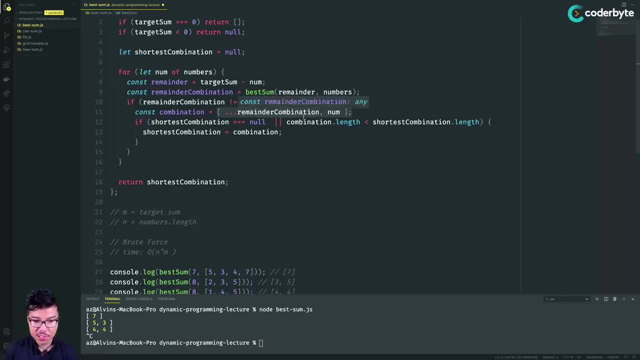 line 11,, which is copying over the array of remainder combination, And that array, in the worst case, will be of length m. right, the largest sort of array of length m. Now, this just sort of a combination, give me back, is a combination that is just filled with a bunch. 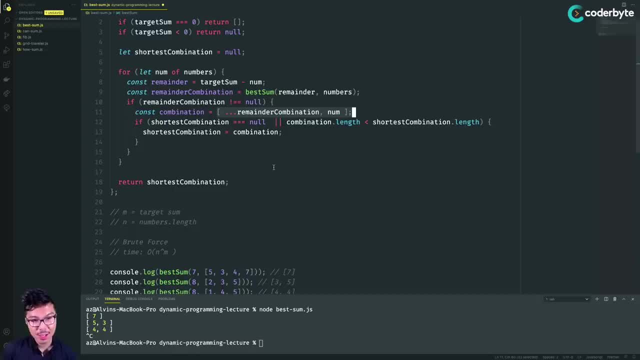 of ones right? If my target sum was 50, the longest combination possible would be a bunch of one, So 50 ones in an array. So what I'll do is I'll say that for each of these n to the m power calls, you also have to do a linear operation in M right. So, like before it's. 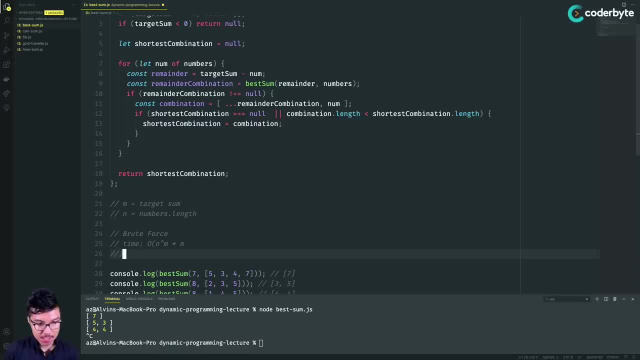 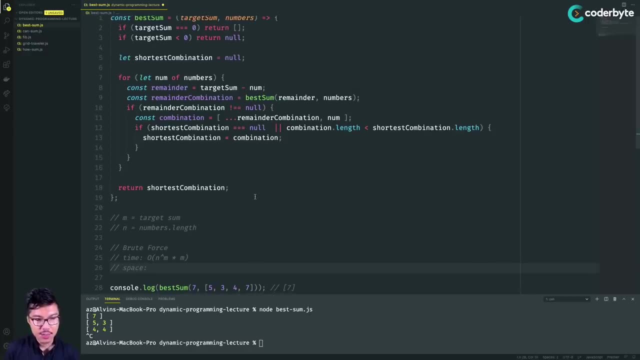 n to the m times, m Cool. And then the space complexity is a sort of interesting in this one because we're maintaining some values. So look at this. So if I talk about the space complexity just from the stack space, it would just be the heights of, like, the recursion. 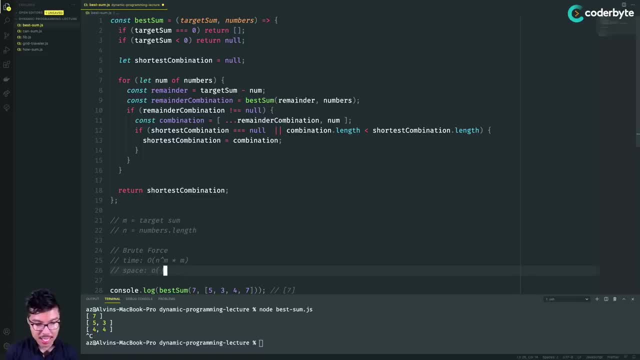 In other words, it would be m over here, right? So I know it's going to be at least m, So I'll jot that down. But then we have also like this variable on line five, right? So I know that over time I'm going to be storing an array inside of this variable And this: 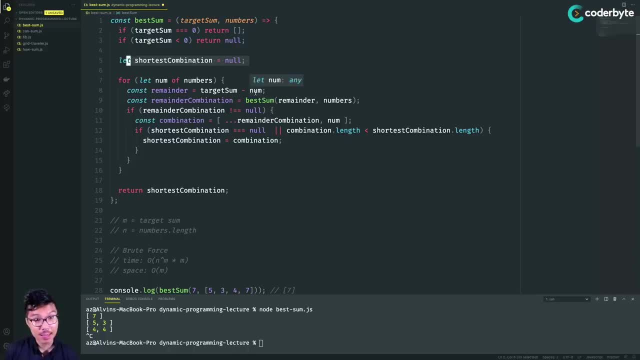 array is going to be, in the worst case, m in length, right? So what I'm saying is I'm going to be storing an array inside of this variable, And this I'm saying is every recursive call would have to have its own shortest combination. 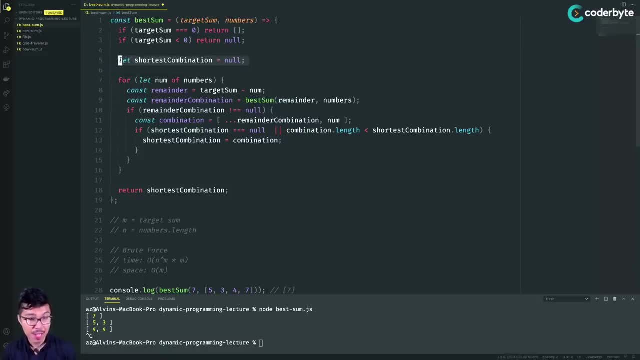 variable right. If the shortest combination variable is going to be an array of length m, that means I have an array of length m for every recursive call right before I bought them out at like my final base case, And so I'll say that the space complexity here is 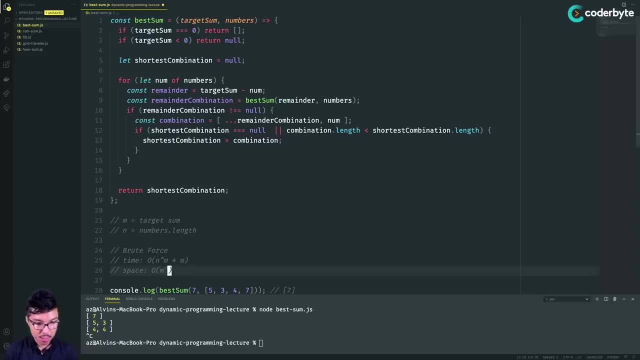 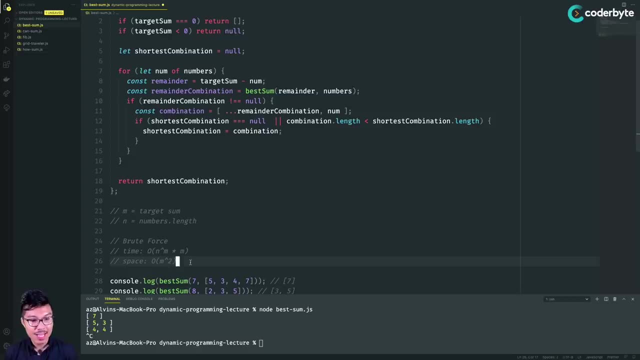 m times m, which we know is the same thing as m squared right And sort of. the reasoning is: your maximal stack depth is still m, like last time. However, now, in each of those stack frames you need to store. 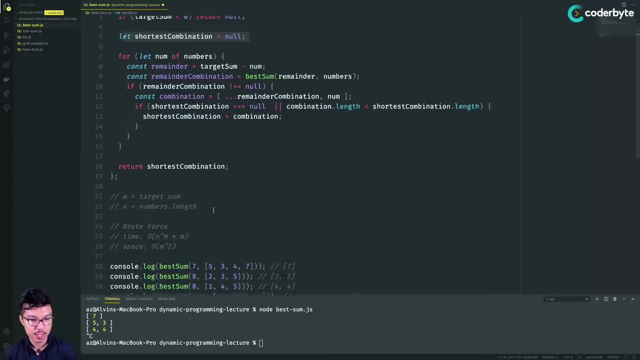 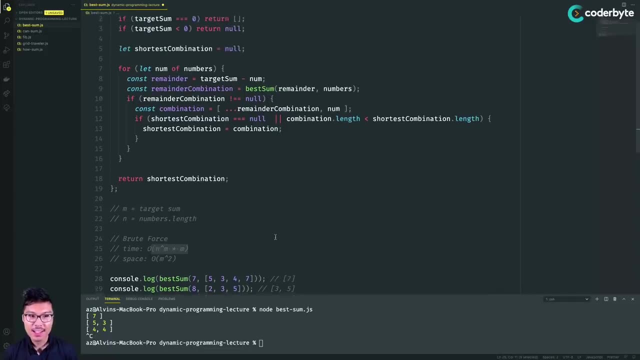 In array right as you recurse, Nice. So really, the limiting factor for us right now is going to be the time, complexity, which is exponential. And so, like we always say, let's go ahead and memo eyes this. So memo ization pretty trivial right now. right, You've done it many. 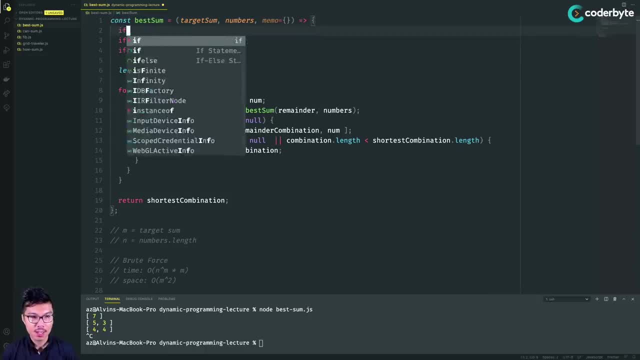 times. So I'll just bake in my initially empty memo object And I'll check. you know, if my target sum is in the memo, then I should actually return the stored value. So return memo at target sum. So now that I have my memo checking logic, what I also want to do is add the memo storing. 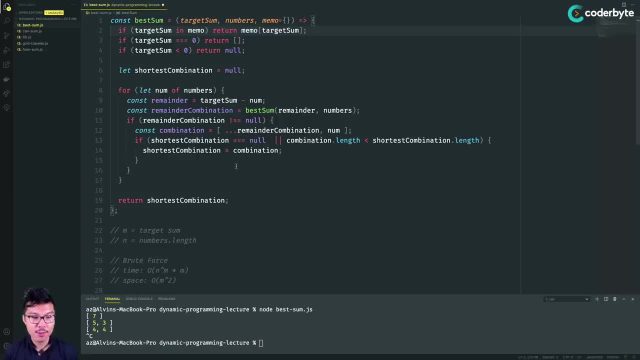 logic right, So I need to just go to my return value and store it in the memo before I return it. Notice that the return value- right now it's no longer inside of the for loop. right in the last problem that was in the for loop because I can return early, But this time 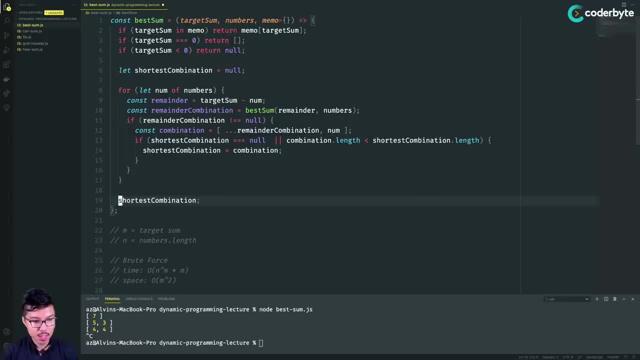 we're going to return at the very end, So I'll replace it over here. So I'll say for here, the memo at target sum should be stored with the shortest combination. I can still return the shortest combination. And before I forget, let me go ahead and pass down the. 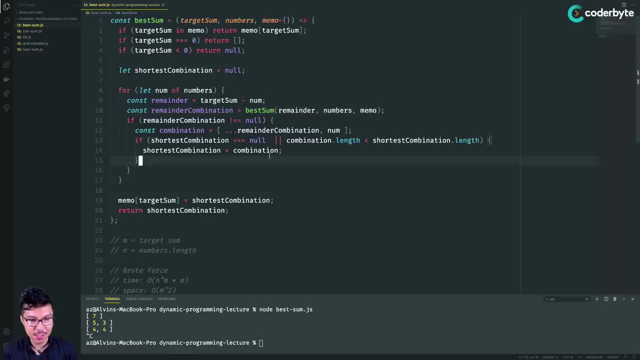 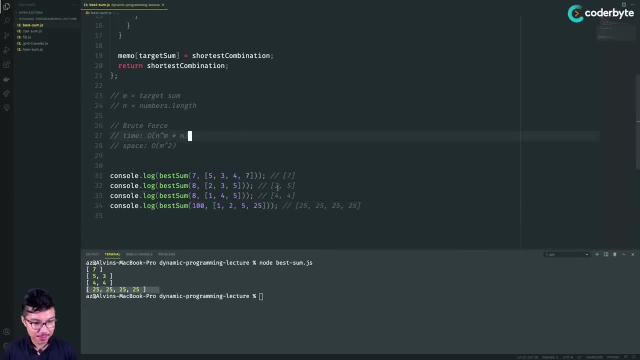 same memo. object by reference. Alright, nothing too much to that. Let's go ahead and try this last example. Now Give it a shot. Awesome, And there we have it. We have 425.. In this last example- and that is the best way to generate 100- is pretty evident that we cut. 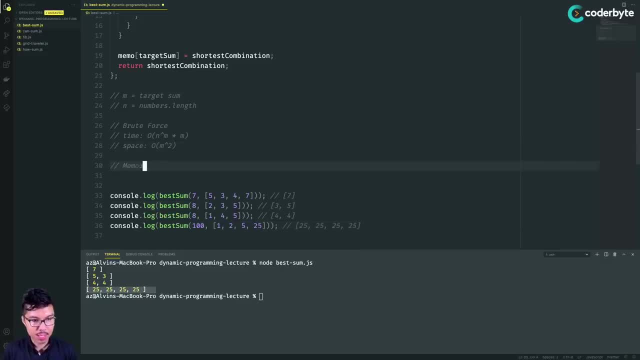 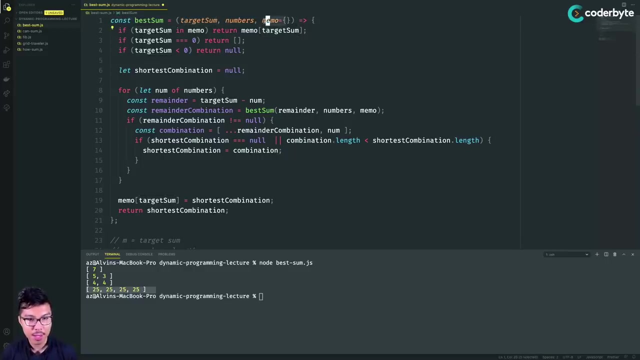 down on the runtime. So let's talk about the memo eyes, complexity And wise, and so the table Time is obviously much faster, should not be exponential, But if I take a lay of the land, I know that now every target sum is going to be a key of the memo object And target. 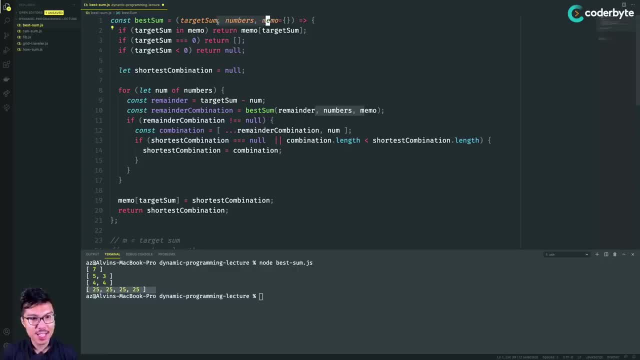 sum is really just a number, right? So if my target sum is 50, then I basically have 50 different keys I can ever store in the memo object. So if I have m different keys in my memo object, I know that I won't be exploring any full. 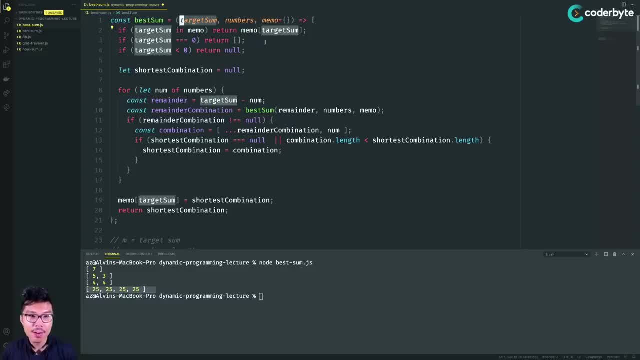 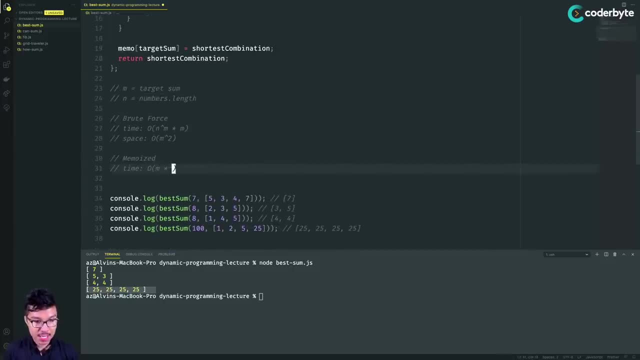 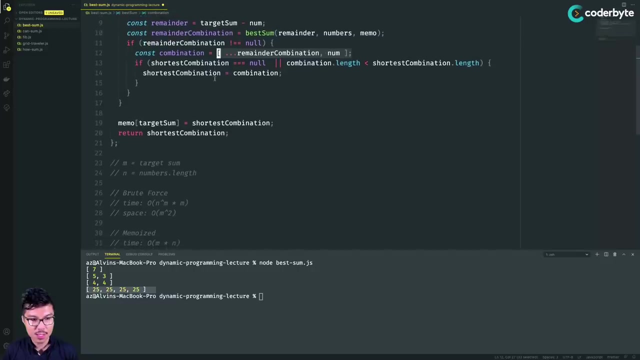 duplicate sub trees for each of those keys. However, I will still have to branch for a number in the array Right. So overall I'm looking at in m times n. So so far I have m times n, But I have some additional work from this array right. So notice that the 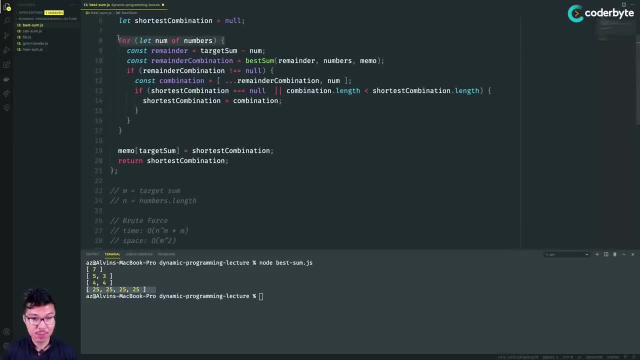 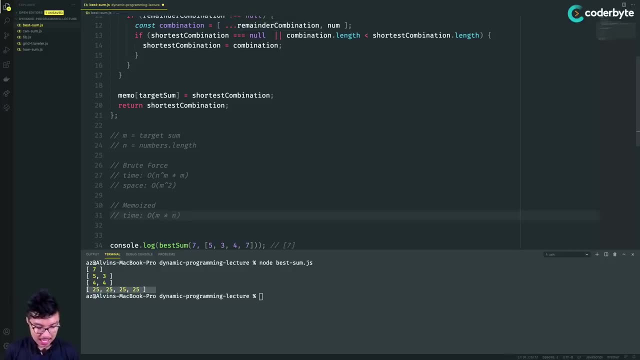 n over here. that comes from this for loop- I'm iterating through numbers. But then the additional m comes from copying over this array, which would be linear. So it would be m times n times m, And I can just kind of squish these two M's together So it kind 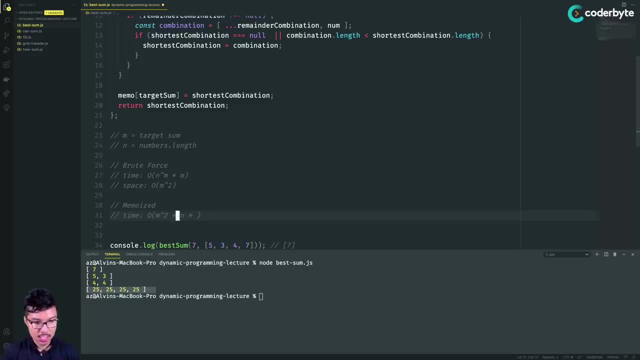 of boils down to M squared times n, which is really the same thing as last time, And our space complexity would also be the same as it was last time, which was just m squared, mostly coming from the memo right, And the logic is: your memo keys have m possibilities, But for each of 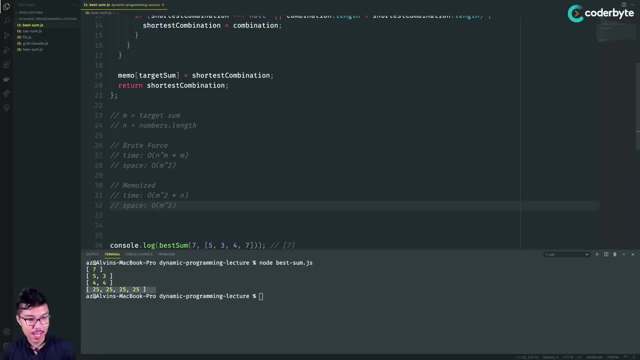 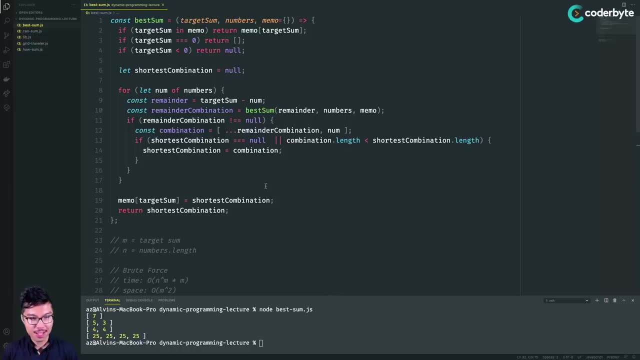 those keys. their value can be an array of length, m, right, so just m times m or m squared, Awesome. So looking at this code, you're probably, you know- feeling that, oh my gosh, like this best sum problem. 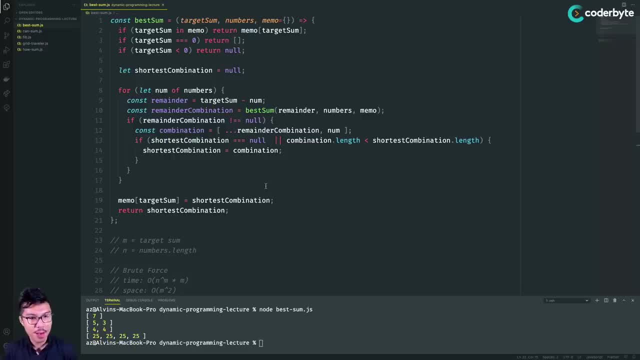 It's pretty complex And I think it, you know, to be honest, it is. However, what I really want us to focus in on is this: like progression we took right. I think that everyone could tackle this best sum problem if they warmed up and really understood simpler problems. 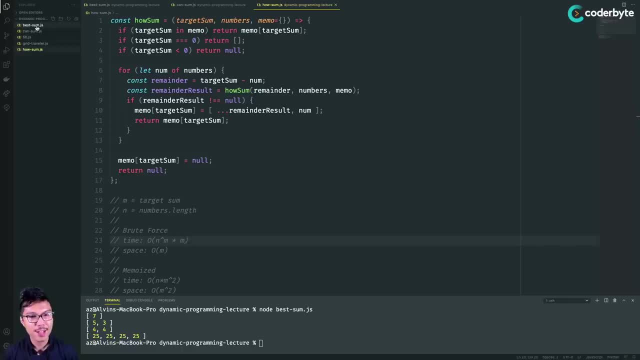 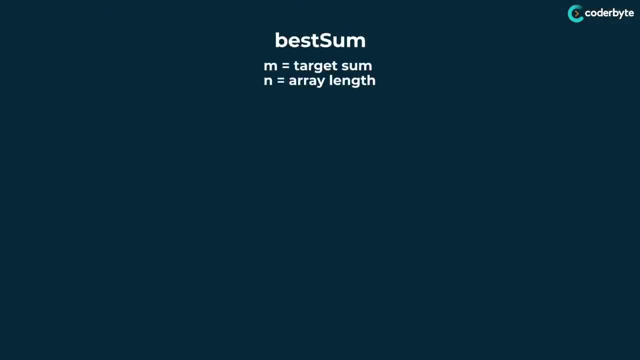 like can sum and how some right, the code is very, very similar. So to wrap things up, let's do some closing words on the drawing board. So in this best sum problem- right, we had two inputs. we had m as our target sum. I also say that n is the length of the. 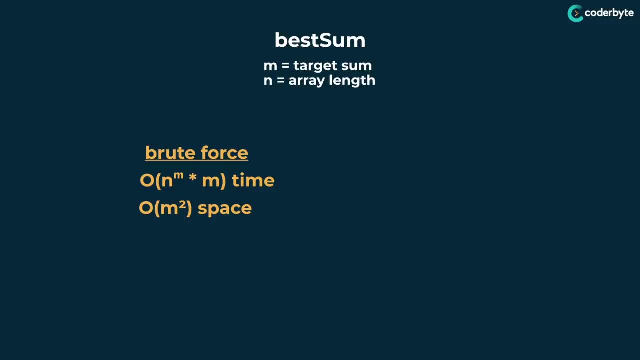 array. So the root force that we initially implemented, with just some recursion, was exponential in time And after we optimize it we brought it down to just a polynomial time complexity And notice that between our brute force and our memoized solution they actually have. 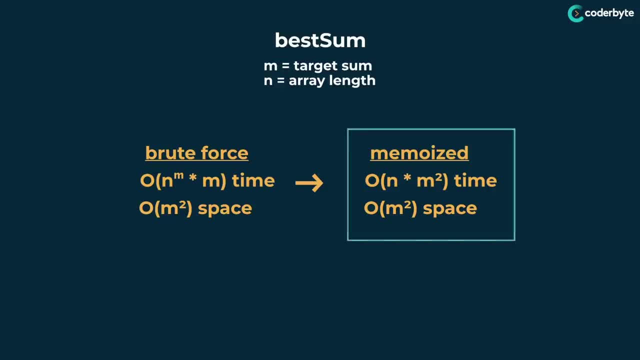 the same space complexity. So we definitely prefer this memoized version. So I hope you enjoyed this series of problems, That is, we worked on the Kan sum, How some and best some problems they all had the common frame of us having some targets on that we need to. 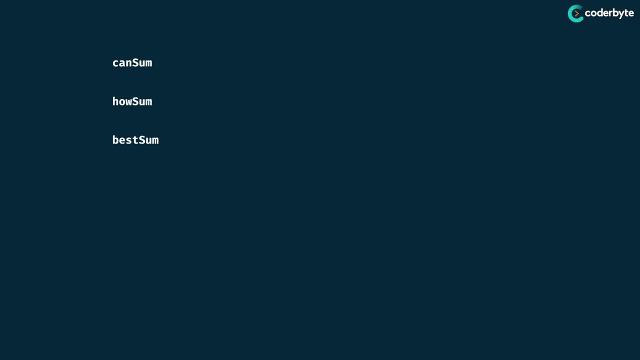 generate with some options given in an array of 10.. So let's go ahead and take a look at options given in an array. In particular, if you look at the can sum problem, it asks us with that task of generating target sum. can you do it? So, yes or no, the house and 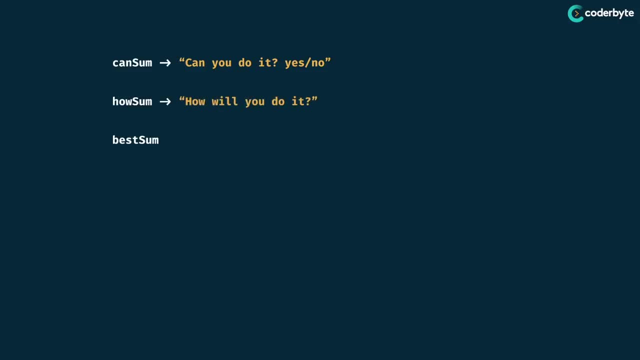 problem asks us: how will you do it? So what are the exact combination of elements that you'll use? And finally, the best sum was the hardest version And it asked what is the best way to do it in terms of the least number of elements of the array. So there, 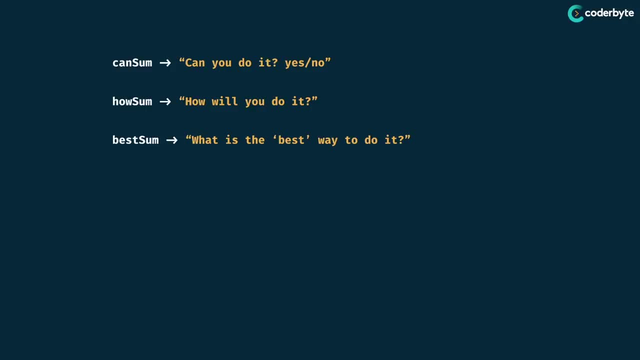 definitely is a logical progression to these problems And in particular they kind of capture a different variation of a dynamic programming problem. For our can some problem, right, we had to return Boolean there. That's a type of decision problem, right, Yes, or? 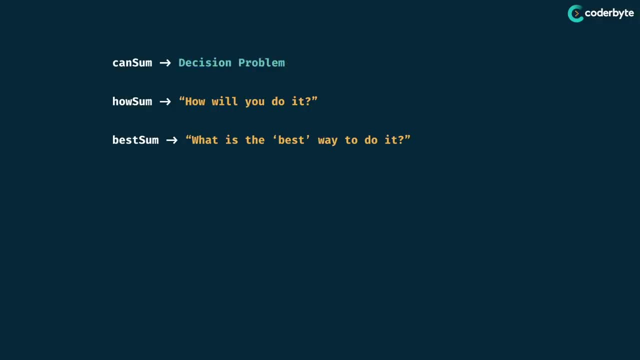 no, can you accomplish this task? Is it possible? Along with that, the house and problem was a combinatoric problem, right? We want to know the exact combination that works out And the best. some problem was a variation of an optimization problem, right? I want. 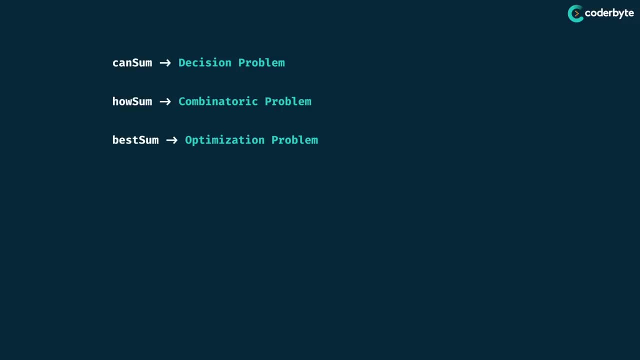 the shortest way to generate the target. So we saw that these three problem types definitely have some common ground, but they also have some nuance, depending on exactly the question we're asking. So we saw that these three problem types definitely have some common ground, but they also have some nuance, depending on exactly the question. 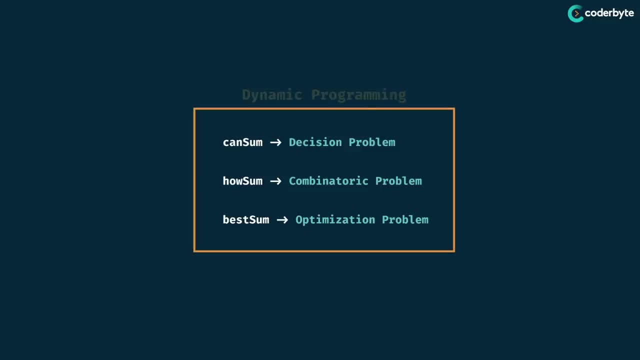 we're trying to answer, And these all fall under the umbrella of a dynamic programming. That being said, dynamic programming problems aren't just limited to number inputs. All right, I think it's time to work on a another prompt. Let's say: I gave you this what I 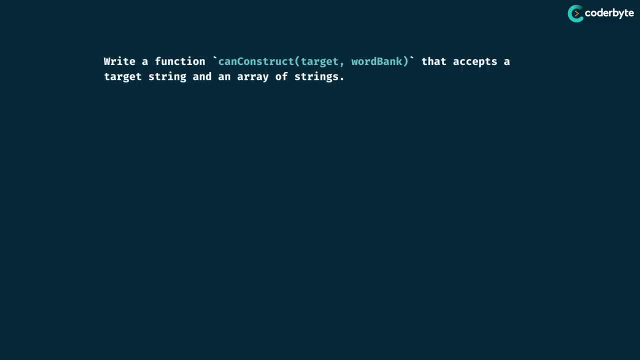 want to do is write a function called can construct that takes in some target string as well as an array of words in a word bank. My goal is to return a Boolean indicating whether or not I can make the target by concatenating together elements of the word bank And along. 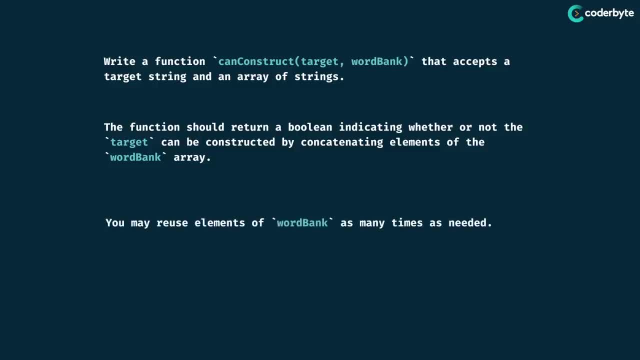 with that, we can reuse as many elements as the word bank as we see fit. All right, notice that in this problem we're looking for a Boolean response to start right. So just yes or no. is it possible to generate the target? So? 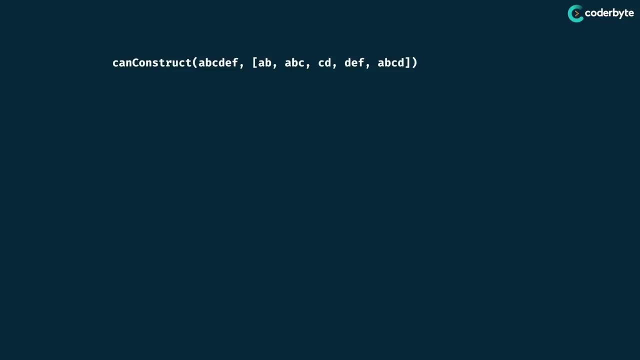 let's take a look at an example here. Let's say I gave you this, So my target is ABCDEF And I have a nice long array of some words And so basically asking: can you construct ABCDEF using elements of the array? So if I kind of take a look at the array there, 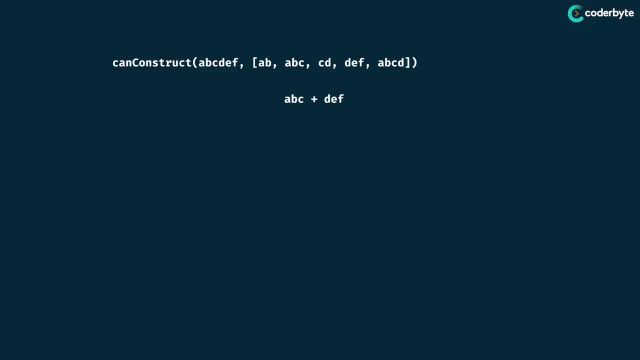 is exactly just one way to generate the target string, which would just be ABC plus DEF. So the answer here is true, because there is at least one way to make the target right. Let's take a look at the opposite example. So let's say I had this: 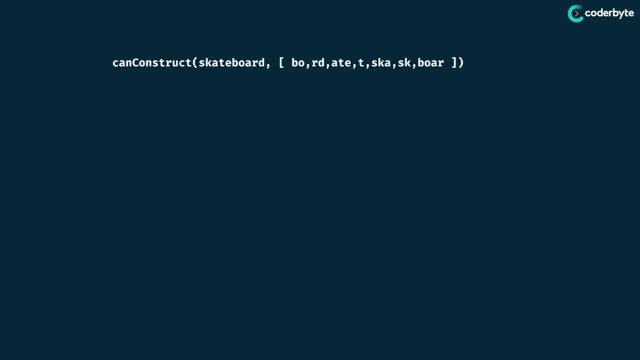 word of skateboard, And I gave you all of these words in an array. So take a moment to kind of look this one over And you tell me right: Is it possible to generate skateboard here? And the answer here is no, right. It is not possible to generate skateboard using. 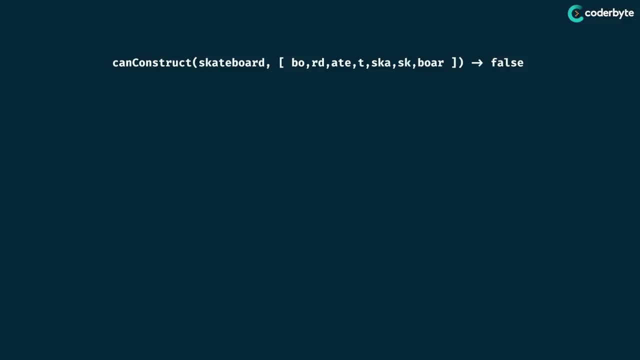 this array of words, So we should return false. We get pretty close to making skateboard, but we can never build the full string right. So here are a few ways that we can attempt, but they don't work out in the long run, right. 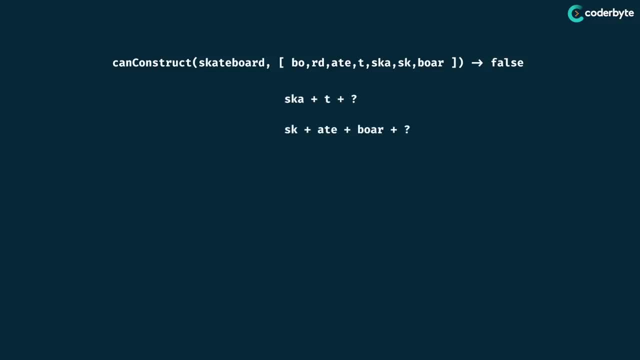 This is one series we can take, but we kind of get stuck as well as this and also this way, right Point being, there are zero ways we can ever generate skateboard, So we should return false over here, Awesome. So I think let's look at one more example. we sure already 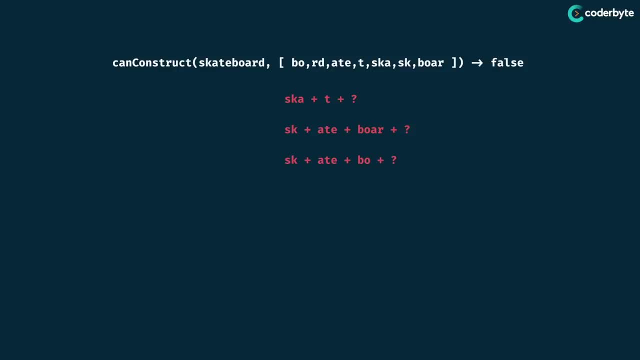 have the vibe that in general, it's easier to create a shorter string than a longer string. right, You're probably going to need to use more elements, So if I have that kind of framing in mind, then I know that possibly the easiest string to create would be the empty string. 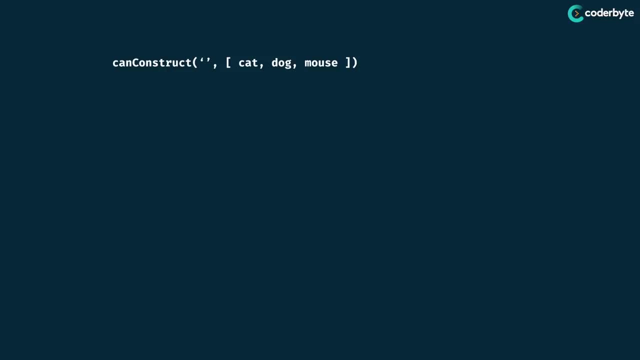 Right. So let's say your target was the empty string and I gave you, you know, some kind of random array of words. really, the array of words doesn't really matter here. I think no matter what they should return true, Because to generate the empty string, you can just. 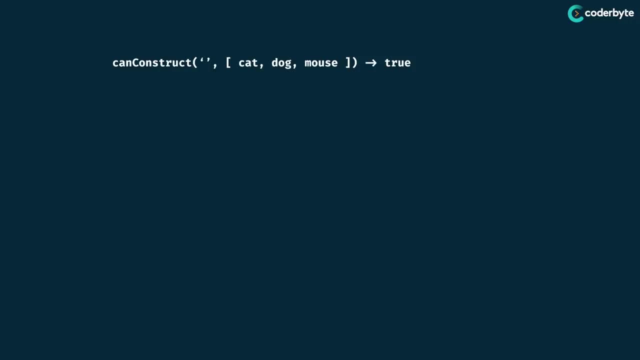 take no zero elements from the array, And that kind of line of thinking is going to help us really start to solve this problem. So we'll kind of take this example in stride. what we want to do is return true if our target is empty, and that takes place no matter what array of words were given. right, Cool. 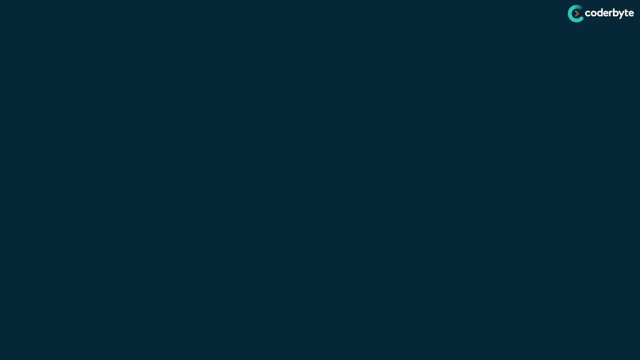 more or less. that kind of sounds like a base case, right. But let's go ahead and start to kind of define some process we can take to explore all of the options, right? So I want to really visualize this in a well ordered way, And that really means a tree, right? 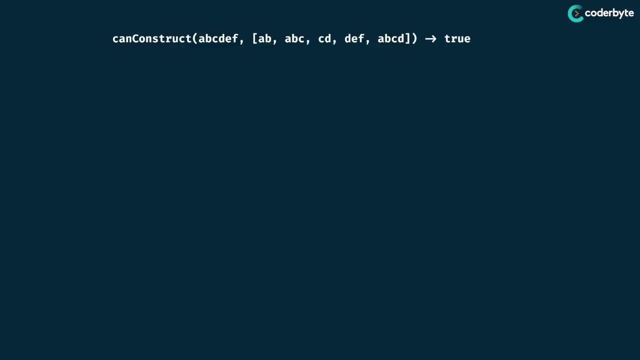 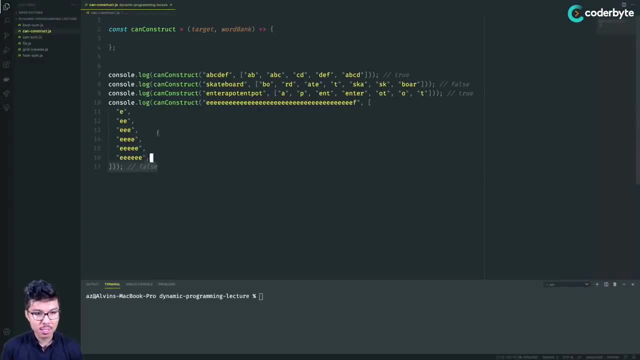 So let's say we're going to use a tree, right? So let's say we're going to use a tree, right? All right, let's go ahead and code this one up. So here I have some initial examples we can use to test our code for correctness. Looking at the last example over here, it's: 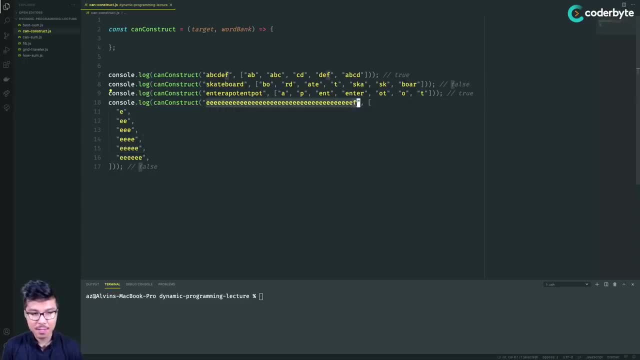 a fairly long one and notice that the target incident F, whereas no words of the word bank have an f in it. So we know that that should result in a false. So let's go ahead and lay down the base case for this. So, like we said, a reasonable base case is to check if your 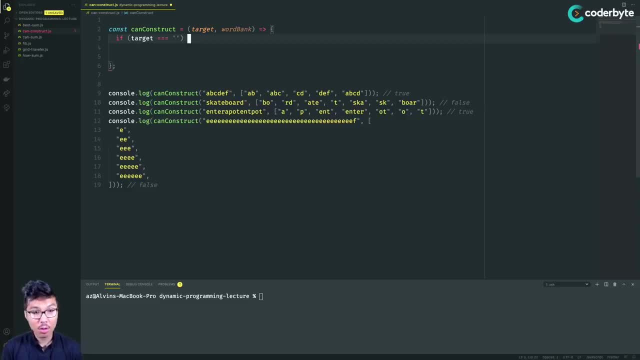 target is empty, right, If you have the empty string, then you can already configure your target to And check out by click and go. Not because that wasn't a activation like: construct the empty string by taking no words from the word bank, So you just return true. 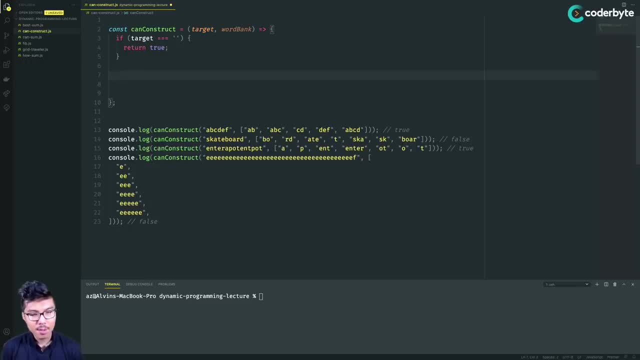 over here And now. I need to make my recursive call in a way where my target string gets progressively smaller and smaller toward this empty string, And so I know that, based on the tree I drew, I need to make a choice based on the words in the word bank. So I'm going. 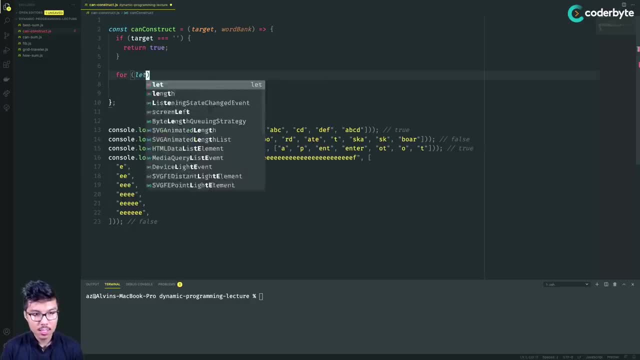 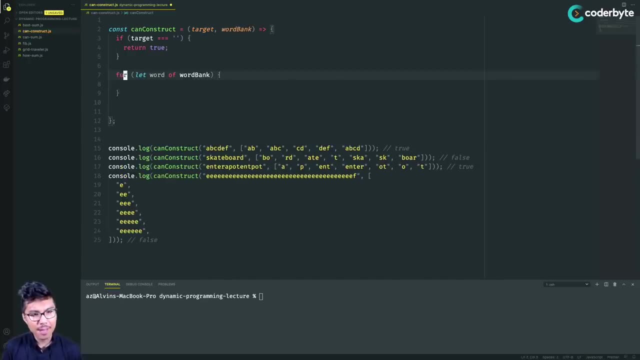 to iterate through all of the words. So I'll say for let word of word bank. So I'm entering through every element of the word bank And now that I have the word element, I have to think about when it's okay to make the recursive call using that word. And we spoke about this. 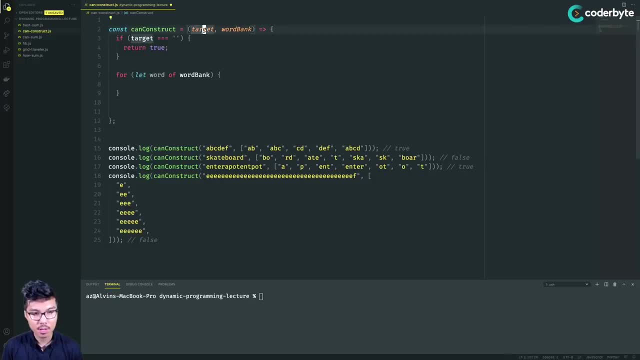 we pointed out that we need to make sure that the word is a prefix of the target. So I can do that. I can just check if the target dot index of word equals zero. So index of will just give me the index where I can find some substring inside of a large string And I 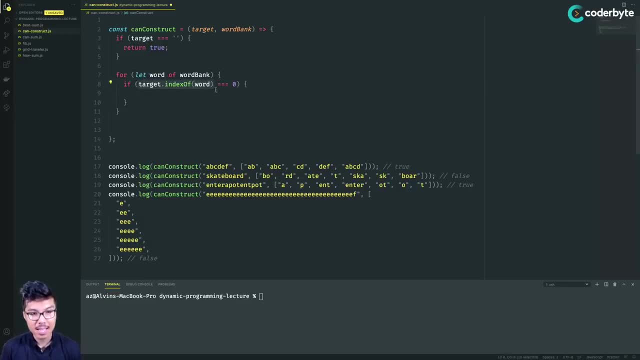 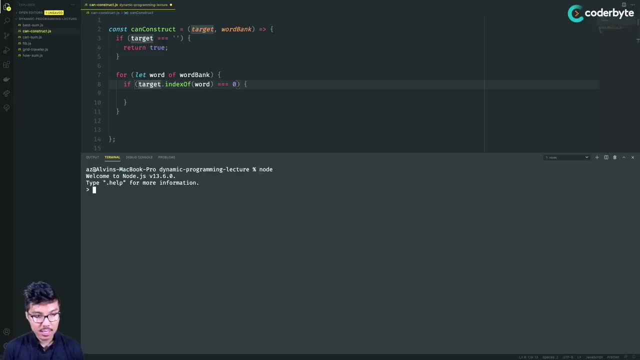 can check if the index I get back is zero. that means that the word starts at index zero of the target. So if you're unfamiliar with this method in JavaScript, really quick let's say I did potato dot index of pot. that will tell me the index where I can find it. 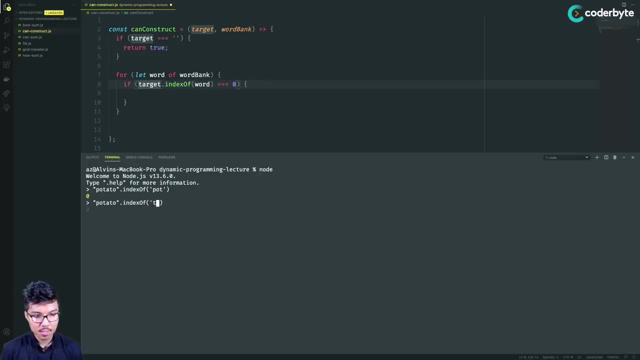 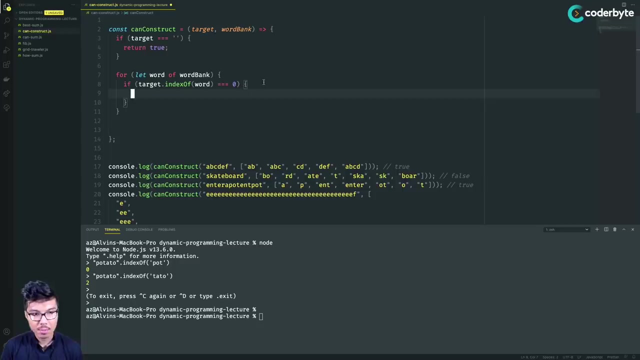 which happens to be at index zero. But if I looked for Tato, I would get the index of the T, the first he, rather in potato. So this is a really nice way I can use to check if some substring is a prefix of another string, right, the index should be zero within it. So we interpret. 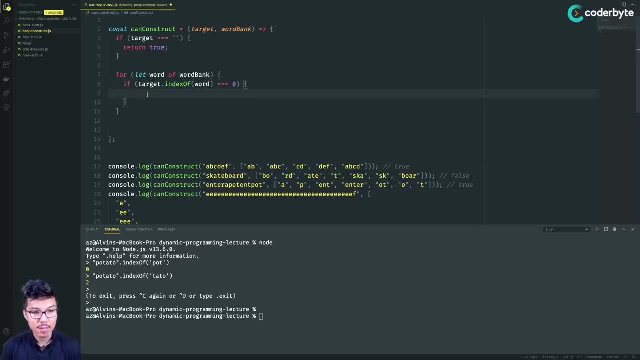 this: if statement is: if I have a prefix, then I can sort of use it to shrink the target. So I'll create another variable here. I'll call it like the suffix, So that's like the string after I remove the prefix. what I can do is slice my target strings. I do target. 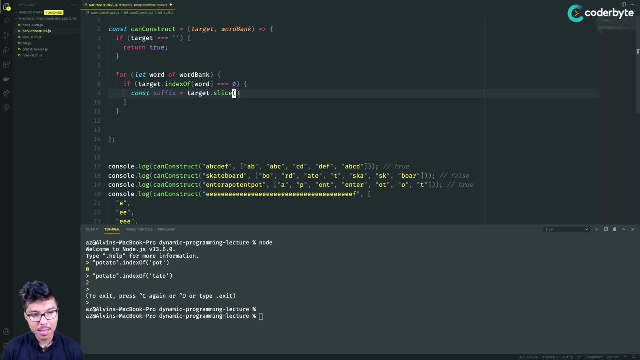 dot slice And what I want to do is start picking up characters After the length of the words. I can say word dot length over here. So let's kind of reason out what this logic is doing. So we'll trace through this. let's say that I don't know my word, so I'll open up the node: repl. let's. 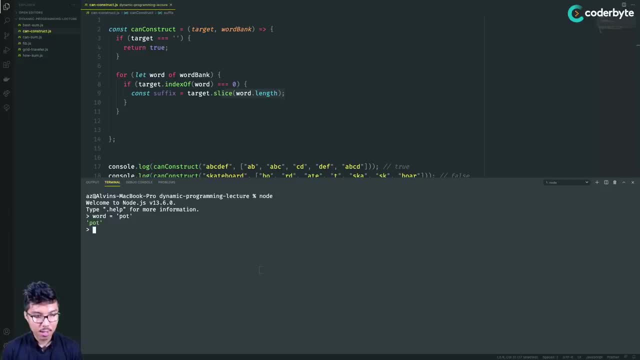 say my word was the string pots, And we'll also say that my current target is potato. So I know when I do target dot index of word that is going to give back zero. So this if statement would be true. And then what I do is target dot index of word. dot index of. 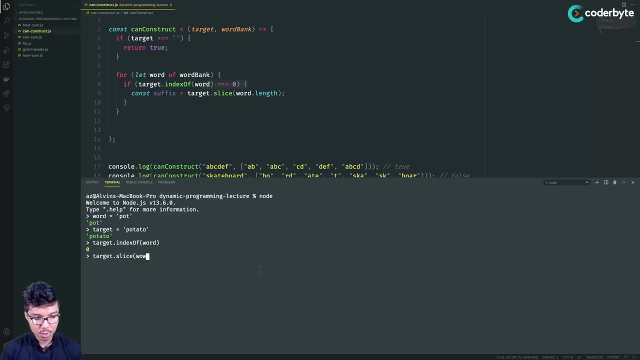 target dot slice of word dot length. So word dot length is just the length of the prefix I took right. so it would be three over here. But if I do target that slice starting at index three, that would give me everything after the prefix right. So I basically have removed pots and got. 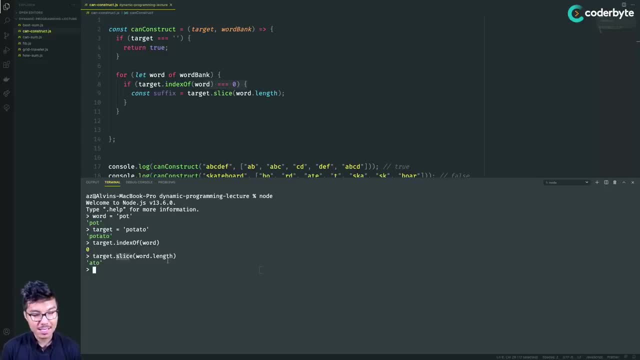 a toe, Cool. So when you use slice, if you pass in a single argument, that's going to be the starting position of where you start grabbing characters and you'll go all the way through the end. Cool, And that's the logic I definitely want here. So back to the code, Now that I have the suffix. 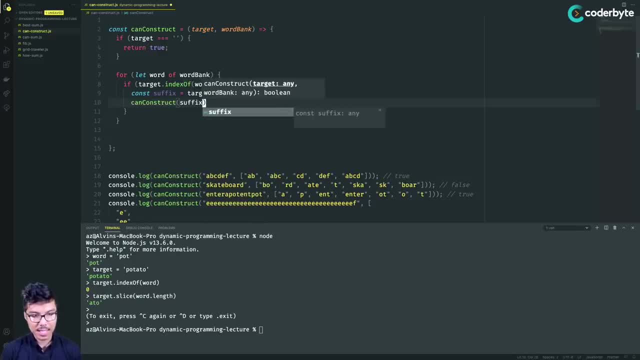 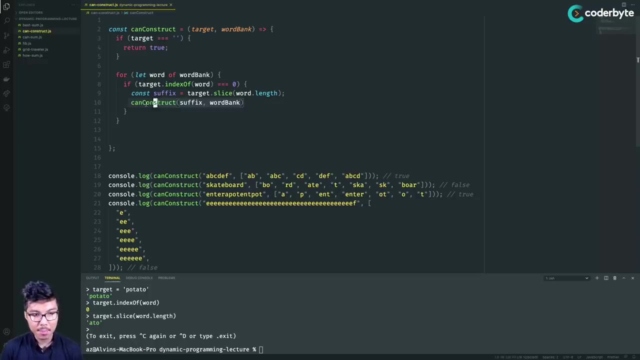 I want to make my recursive call on that suffix, So basically asking: Hey, is it possible, Can I construct the suffix now and I'll pass along the same choice of word: bank, Nice. So here's where I should think recursively. So I'm focused in on what type of data do I get back from? can construct I? 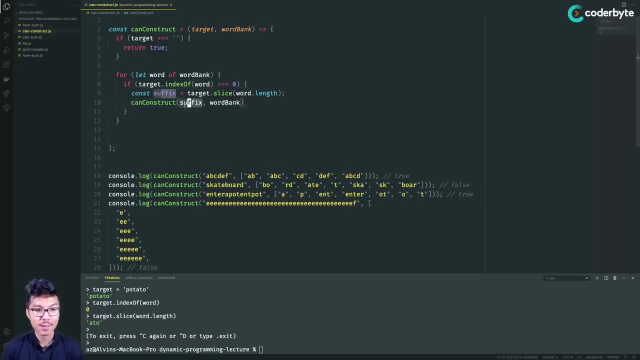 know I get back a Boolean right, true or false. it tells me whether or not the suffix can be made And I want to check out if this call returns true. maybe I'll be explicit here. So if the recursive call is true, 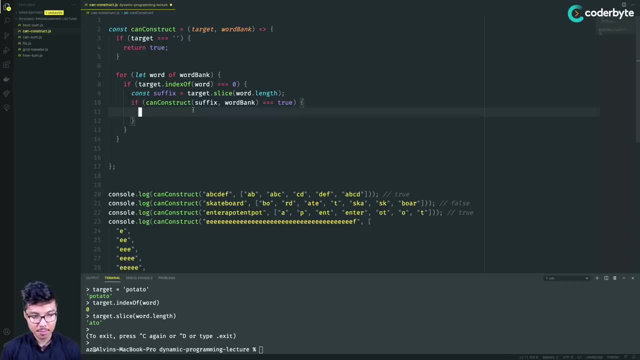 then I know that the original target can also be made. So what I'll do is return true early here. Cool, I know that if the suffix could be made- and the word that I use to generate the suffix is also in the word bank- then the entire target must also be able to be made. Nice, So here I have my nice. 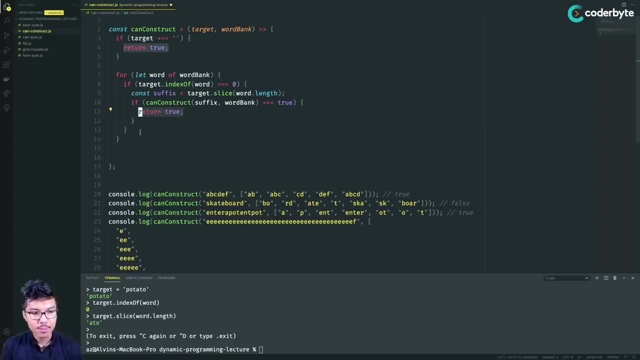 early return: true. And like you expect, where should I return false? it should be after the for loop right. only after I've tried every possible choice of the word and none of them worked out, then can I say no, the target cannot be created, So I want to do a late return false over here. 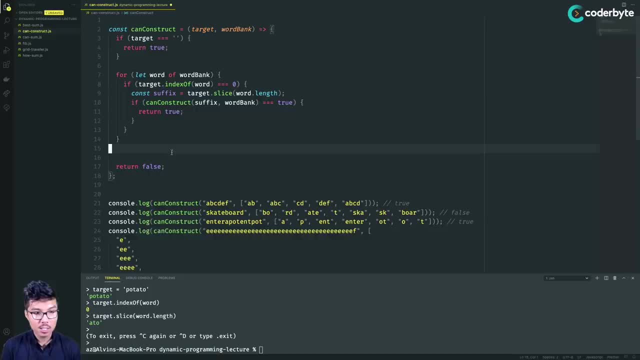 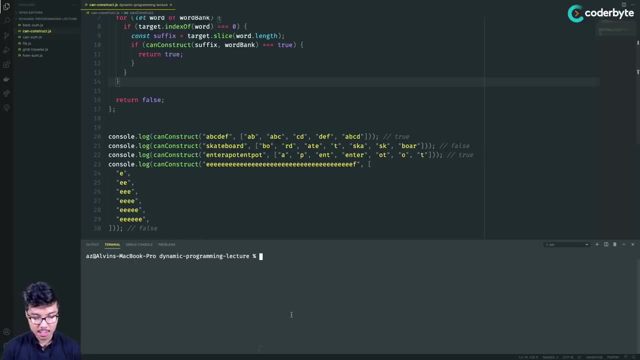 So this code is looking pretty sharp. I think let's go ahead and test these examples. So I should get true, false, true and then false for the last one. Give this a go. So I get true, false, true And it looks like the last example over here. 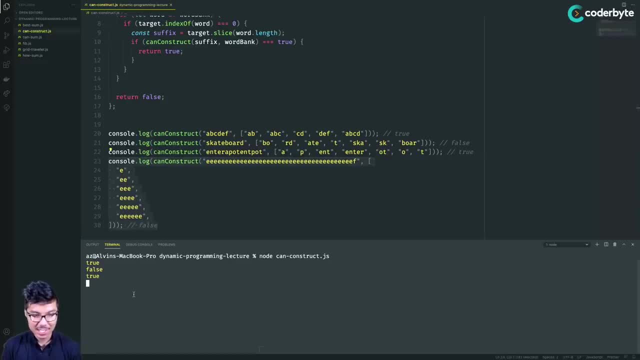 is taking quite some time to finish. So I think our code has correctness, But it's not efficient enough to you know reasonably run this last example. So I'm going to kill this program. If you take a look at the example, I pass it for this last one. 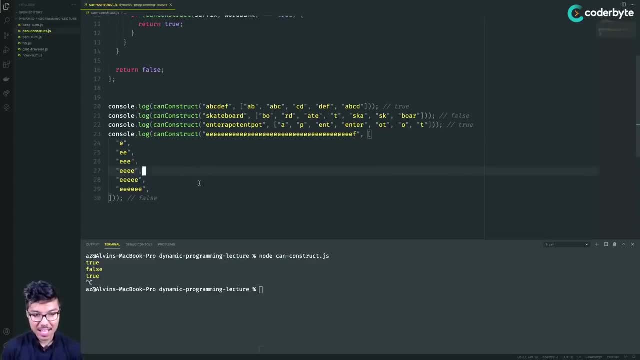 it does sort of describe the worst case here. For one, we know that the answer is going to be false, So you will have to do a full exploration of the tree, meaning you can't do any early return. trues right And because of, like the length of the string and also the length of the word bank. 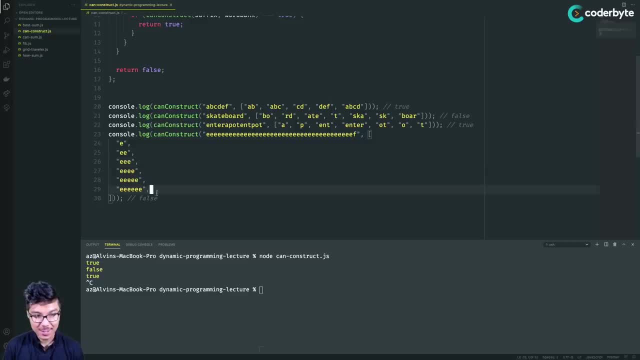 I have a very big tree right. Notice that there's going to be a lot of prefixes that work here, right? Every element of this array is actually a prefix that could be found over here, And that happens again and again. So tell you what? let's go ahead to the drawing board And we'll try to. 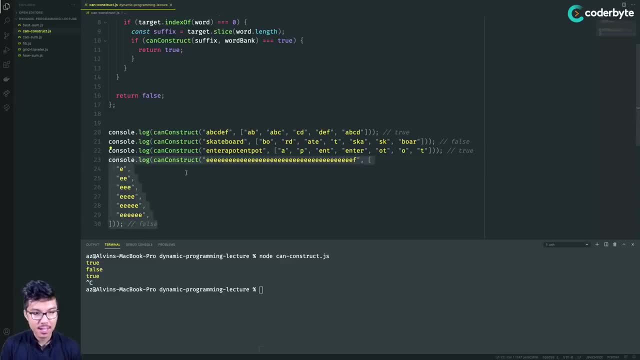 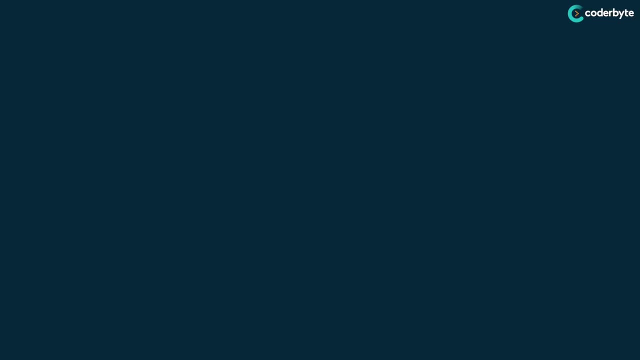 visualize what the exact complexity of this function is. All right, implemented looks like the brute force for this solution. Let's talk about how we might want to optimize it, And I think any conversation of optimization should begin with actually understanding what the current complexity is. So let's say I gave us this kind of large example. 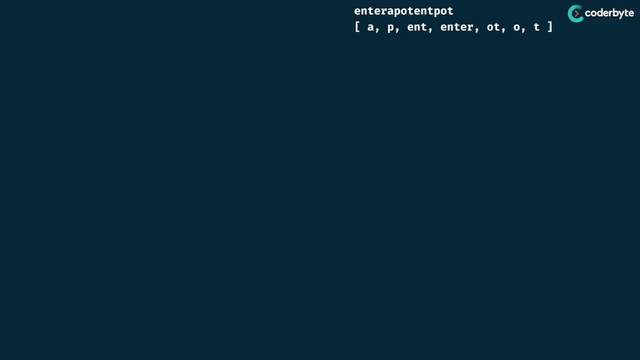 to sort of visualize with. So my target string is: enter a potent pot, And I gave you a pretty diverse array of words in the word bank, So I'll just go ahead and kind of give us the full tree and what it would look like would be this pretty long tree, right? So I follow the same logic that we did in. 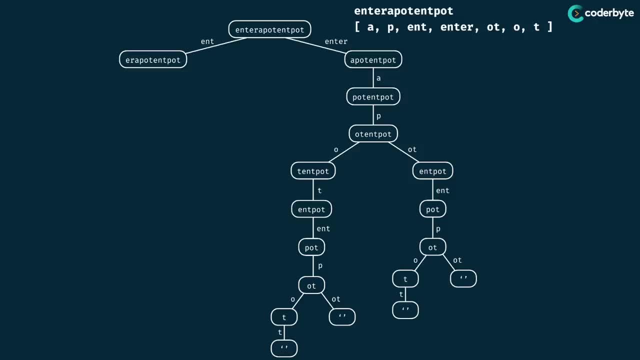 our earlier example. So let's go ahead and give us a pretty long tree, Right? so I follow the same logic that we did in our earlier example. Notice a few things: There are some occasions where I transition using a single character prefix, which is totally fine, And that kind of tends to feel. 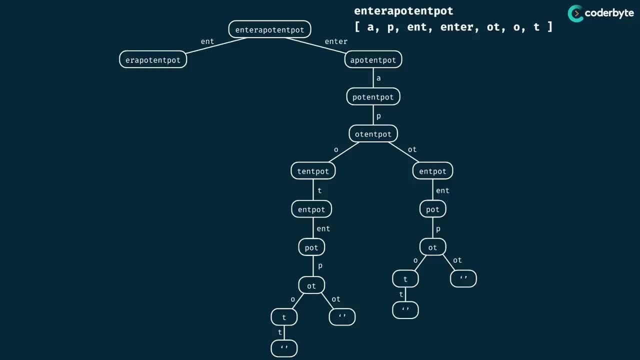 like the worst case scenario. right, If you take single characters out of your target string over time, then you're going to have a very, very tall tree height or you're gonna have to take many, many steps. So that kind of reminds us of a worst case scenario, like we saw when we ran the code. 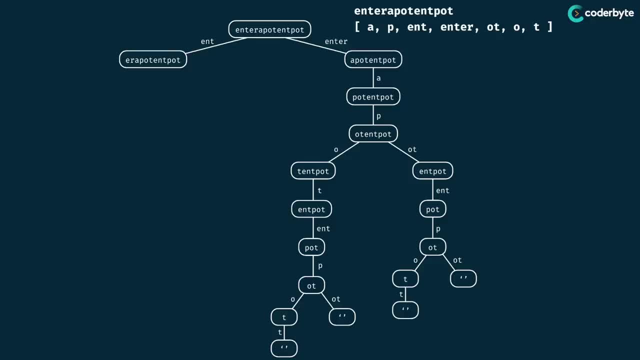 But that being said, we want to generalize this understanding right for basically some generic size of our input. So let's say we kind of just looked at this tree in terms of its overall shape and then we'll kind of generalize it. So to me this tree has 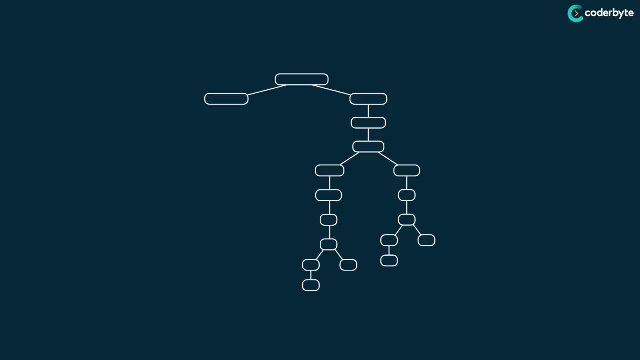 this sort of basic structure. And let me start by defining the terms I'll use to describe the complexity, right? So I'll say that m is the target string length and n is the number of words in the word bang, right? So I'm really trying to use a different variable for each of. 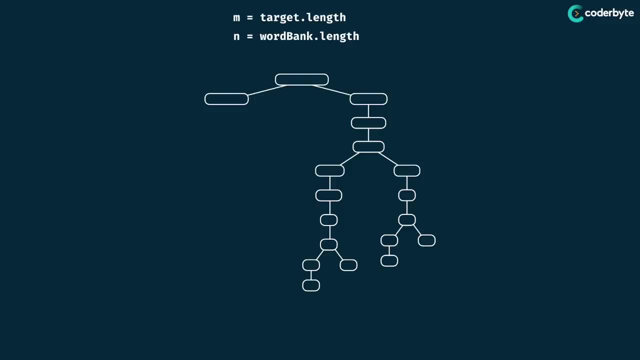 my inputs because I have the vibe that both of them contribute to my complexity, possibly in different ways. So you've seen, you know us analyze trees before in terms of like their structure right we're visualizing is the call tree. I know that the time complexity would 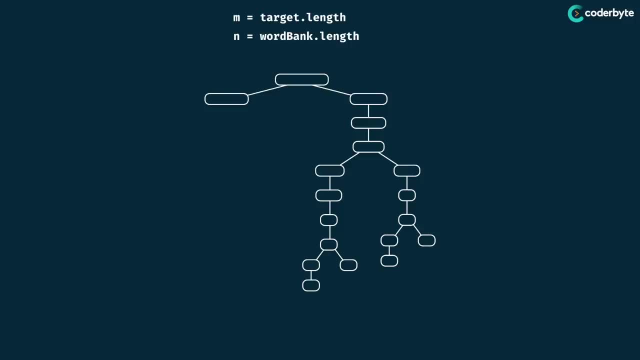 be the number of nodes in the call tree, right. And so let's start with some familiar territory. I kind of already know that I need to realize the height of this tree. the height of this tree is going to be m, right, remember that m is our target string. And so imagine, in the worst case: 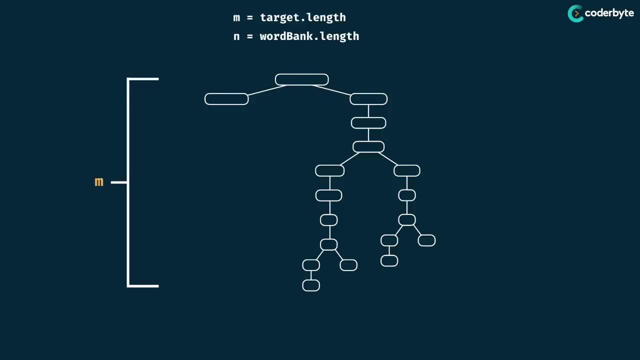 that we took, or we had to take, a bunch of single character choice of words to construct our target string. That means that the number of things I would have to take all the way from the root to a base case or the root to the leaf, 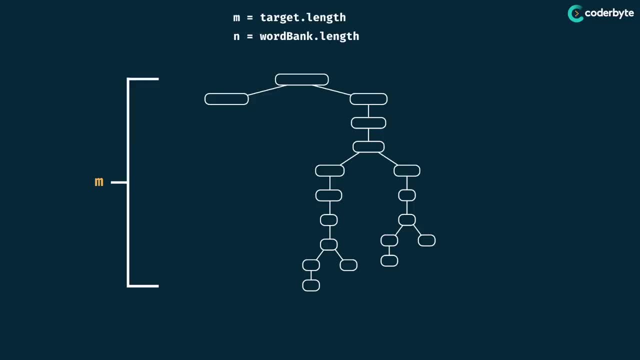 would be exactly m right if I had to take a bunch of single characters. so we can be confident that the height of this tree would be m. So I talked about the height. now I need to realize the branching factor, that is, from one level of the tree to the next. how does the number of nodes 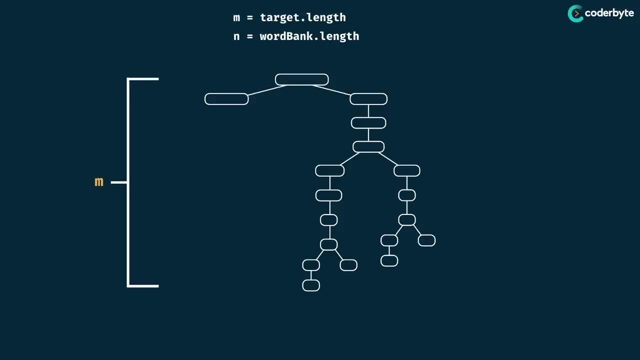 change in the worst case. Well, I know that the branching factor is dictated by how many words I have in the word bank, And so that would be some relation on n. So I know at the root level I have about one node, But then in the worst case, to get to the next level, I will multiply by n. 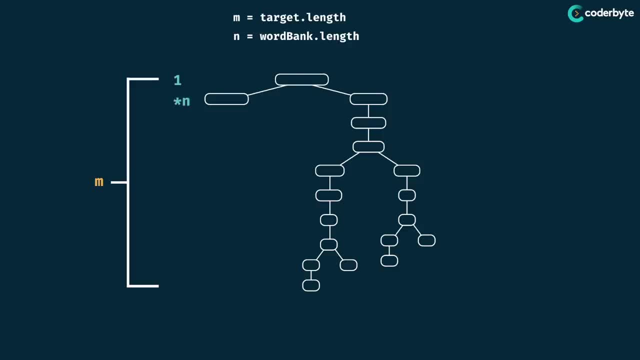 right. imagine that basically almost every element of the word bank was a matching prefix, right? So you multiply by n And let's say that, carried over further, let's say almost every word of the word bank was still a prefix of those resulting nodes. I would keep multiplying by n And I would do this. 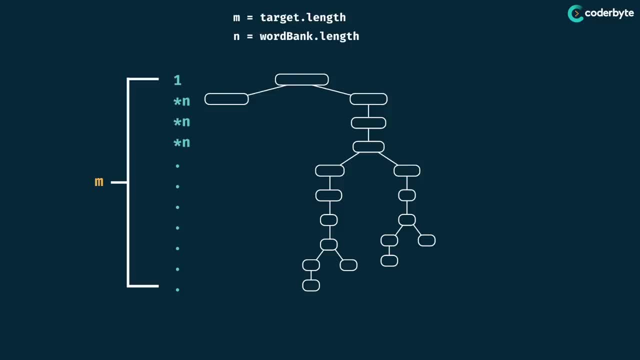 overall m times right, So we already know that this is going to be exponential. I need to multiply n by itself m times over, And so this would give me an n to the m time complexity In general. if you visualize your recursion using a nice call tree like this, then the overall time complexity 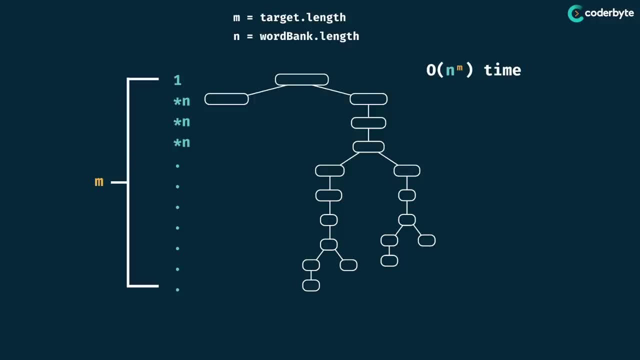 is going to be the branching factor to the height power. So we have a branching factor of n and a height of m. That being said, this will just really consider the number of calls that we make. I want to be super sure and make sure we didn't do any other kind of performance or costly operations. 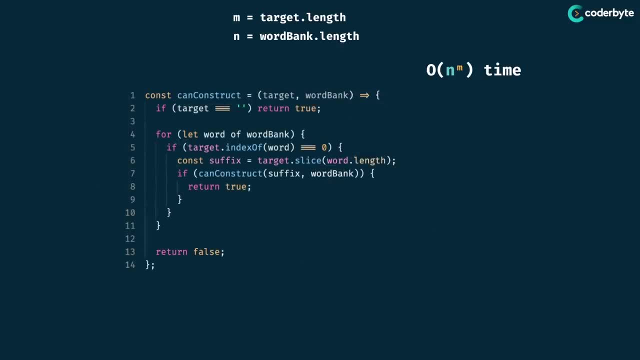 inside of our code. So here's our code, same code as we did before. If you look at this code, some things I need to consider are probably line six, right? If I look at line six, that was where I did a target dot slice. So that's like copying over a part of the target string And to do that 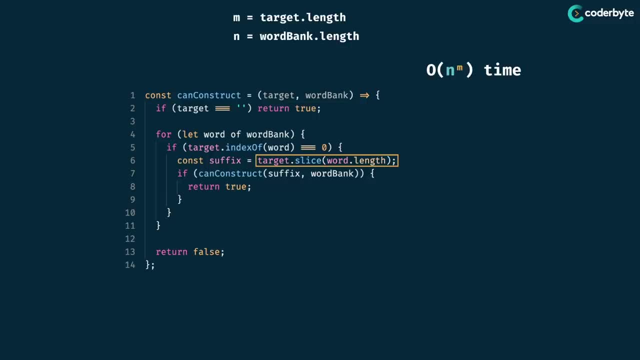 operation, I would actually have to iterate through the target string, Right, So that would actually contribute to my complexity here. So, in the worst case, what would I be slicing? Well, if I'm slicing the target string, that would have like a maximal length of m right And 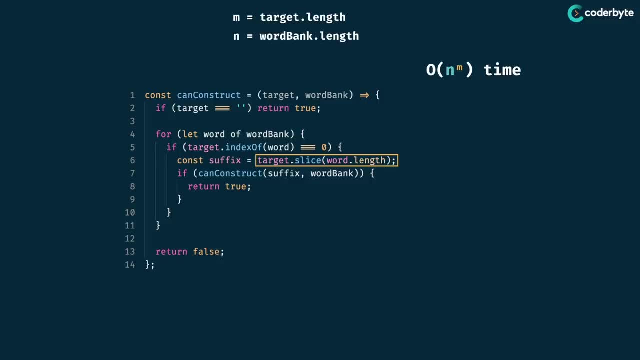 so in every call to can construct I'm going to have to do an additional m operation. If I have n to the m calls, then I can just multiply an additional m over here. Alright, so I added some additional term into our complexity. just multiplying by m. Cool, And so overall. 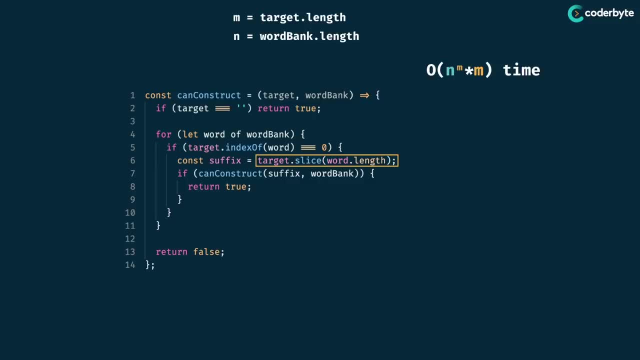 if you look at that time complexity, it was already exponential, So that multiplication by m doesn't really make it that much slower. It's really the end to the M that makes it unbearably slow in the first place. So that was the time complexity. Now let's look at the space complexity. 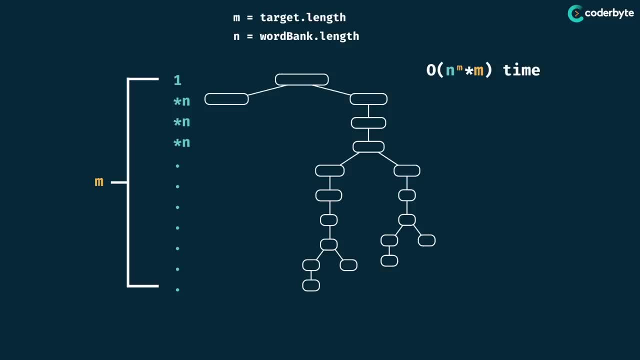 So if we just refer to the space complexity due to the call stack, it looks like it's going to be the height of this tree, right? Like we always say, the height of the tree would mean the maximum number of stack frames you would need on the call stack before we bought them out at the base case. 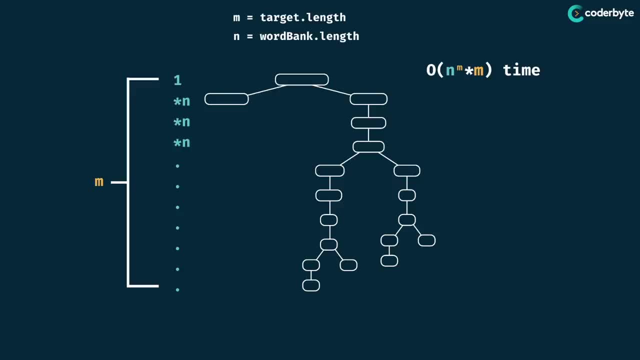 right, Because when we were turned from a call we would actually remove something from the call stack, right? The height of this tree is definitely just M, So we'll say the space from the call stack is just O of M. But again, we should also, you know, look at our code and see if we. 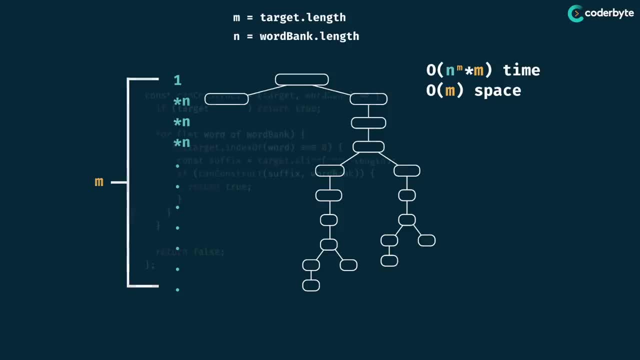 created any other like growing structures. So if I look at the code right now, I see that online six kind of talking about that slice statement again. the slice returns you a new string, right, And that new string is going to tend to be of length m. So on every call to can construct I'm creating. 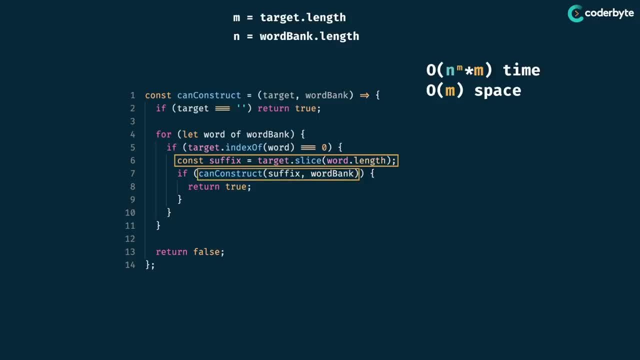 a new string. I actually need to maintain it through the recursion right Because I actually slice before I return out on line eight. So because of that I know that each of my M stack frames will have to store a string of length m. So that just means m times m in my space- complexity. 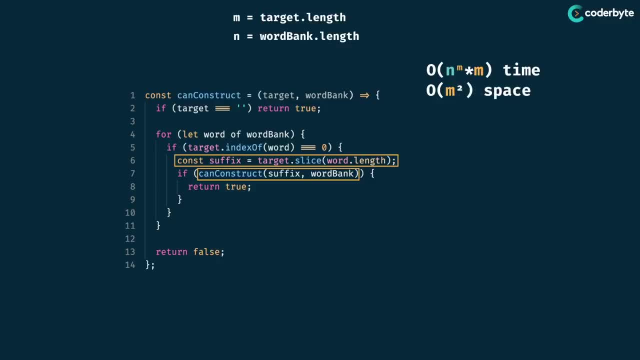 which is really just m squared Cool, which isn't too bad of really a space complexity overall, Alright. so it looks like our final complexity for our brute force solution is exponential in time And it looks like quadratic in space. So obviously let's work on improving the time complexity over here. 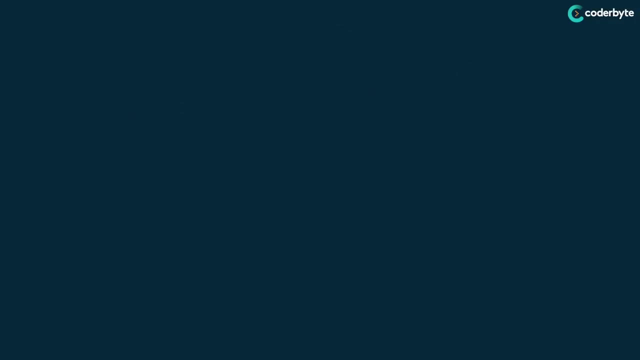 And so hopefully you're seeing where this is heading. Let's say we jumped back into my enter, a potent pot example. So this was a huge tree. take a moment, look at this tree And where can we actually optimize some work away? 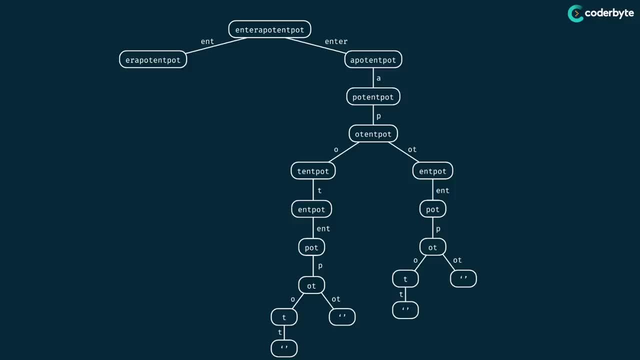 So we're trying to do is notice any overlapping sub problems And in the context of our tree, that means I'm looking for any duplicate sub trees. And I see duplicate sub trees right here. Right, They follow the same structure all the way down, even to their base cases. So if I look at 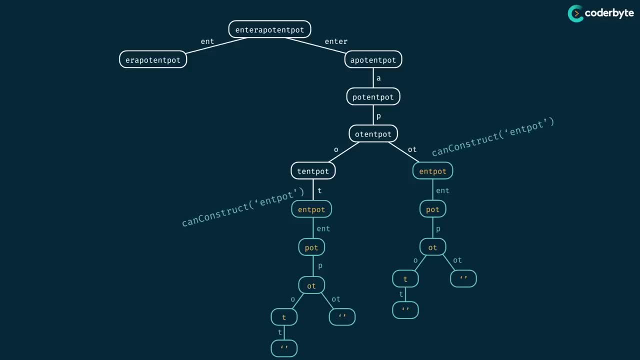 these sub trees. they're really trying to solve the same problem, right? That is, they're both trying to figure out: can we construct the string and to pot? right? And if I solve it once on the left hand side, the answer is going to be the same on the right hand side, So I can just store that. 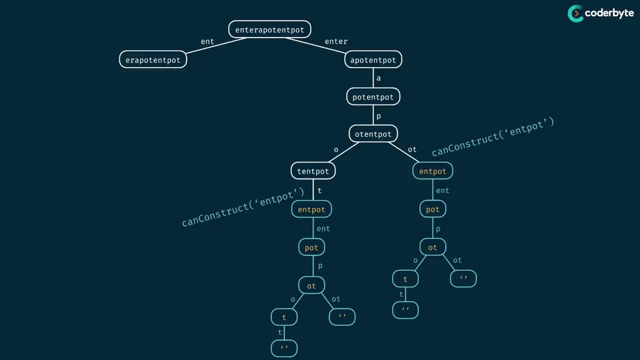 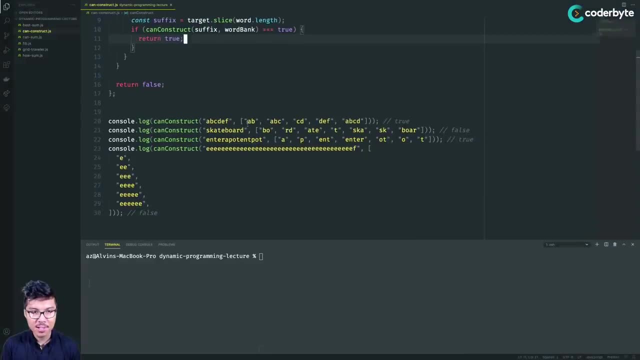 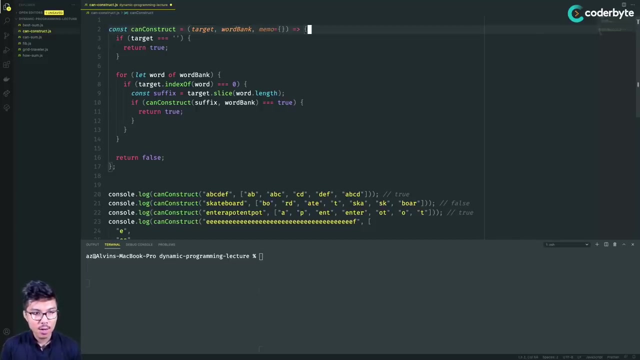 information in a memo right. So the trick is here to, of course, memoize it using our classic strategy. So let's hop to it. All right, here we are back in my code editor. Let's go ahead and just memoize this one. So I'll create my memo object, And here I'll prefer to use the target as the key. 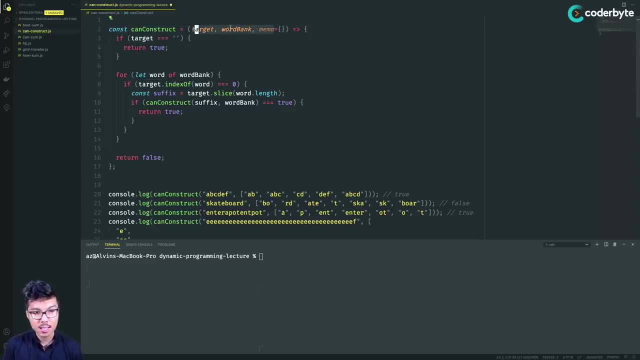 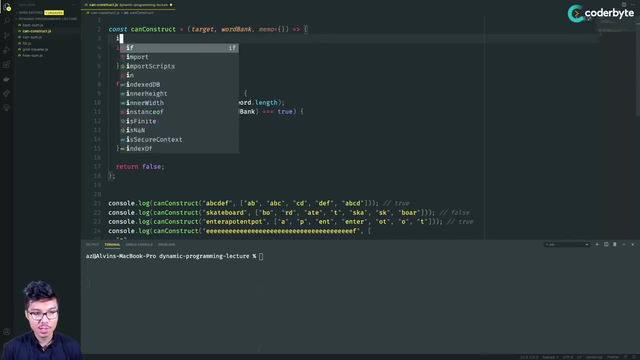 to my memo. I know from one call to the next the word bank doesn't change right, So I don't need to actually make it a part of the key for my memo object. So I'll just check, Hey, if my target is in. 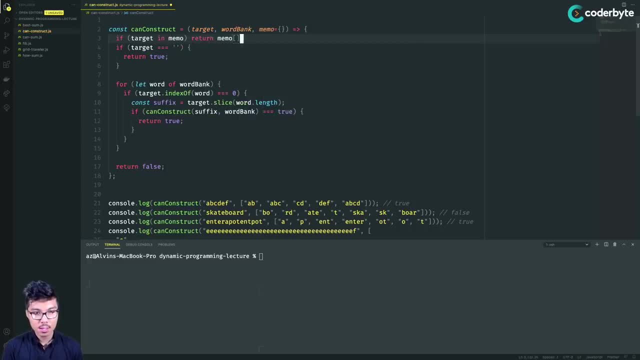 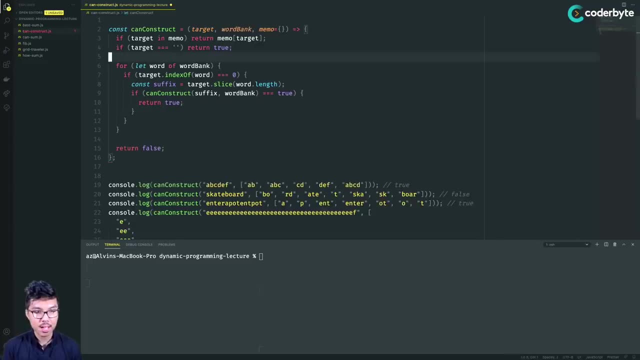 the memo, then what I'll do is return the stored value of that target. Cool, While I'm here, let me squish this down to a one liner. So I have the memo checking logic. Now I need to make sure I pass down that memo to all of my recursive calls, And then I need to actually store data in the 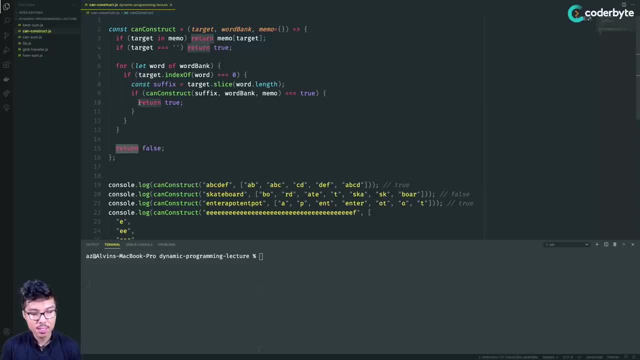 memo And the rule is, wherever you have your recursive returns now, you should also store that return value in your memo before you actually complete the return right. So for both of these lines I'll make sure I store them in the memo. So I'll say: memo at target equals that. then I 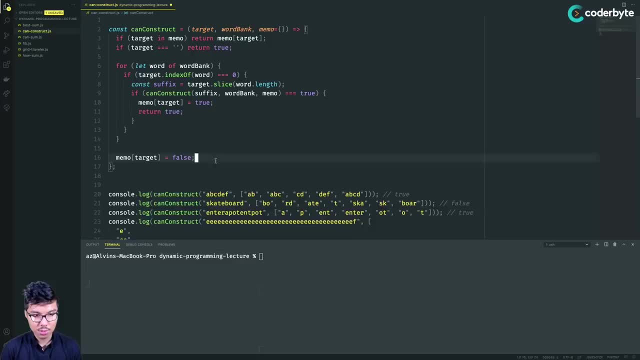 still want to return That same value. So return true and return false. over here Again. notice that I'm using my exact argument: targets right. I don't need to write any memo ization logic about the suffix right. Imagine if we made the call to can construct. suffix becomes that frames target. So the memo ization. 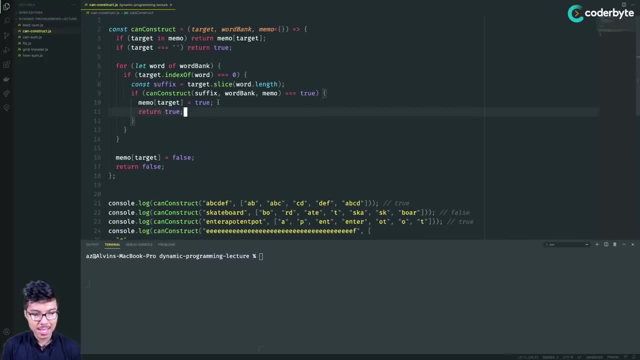 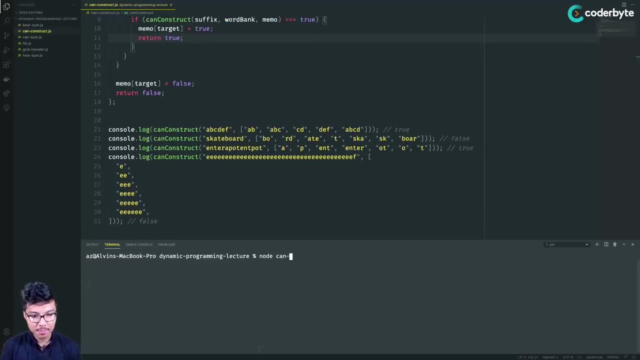 would still work properly, right. So that looks pretty good And it wasn't that much code, right. memo ization is always this slightly extra layer we add on top of our brute force solution. So let's try this now. can construct Nice. And there we have that last example finishing. 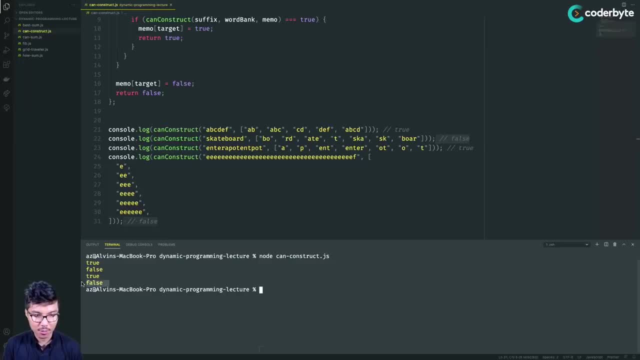 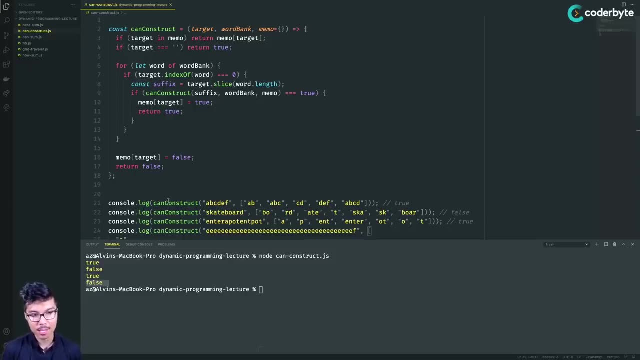 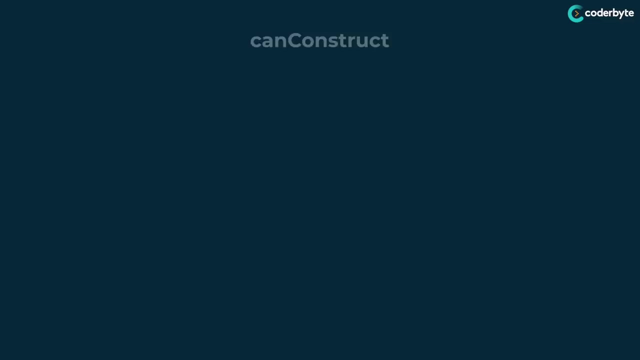 fairly quickly, or we do get the correct answer of false over here. All right, so here's what we'll do: We're going to head back to the drawing board And, of course, we'll come up with the final complexity analysis for this function. Some classic memo ization, right, Let's take. 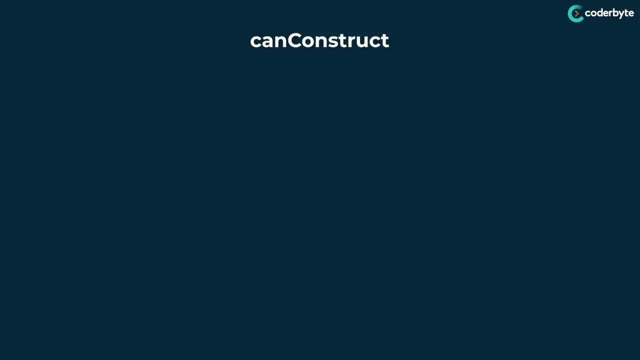 a lay of the land over here. So we wrapped up this can construct problem. let's describe its final optimized complexity. So again, like before, we'll say m is the target length and n is the number of words in the word bank. Our original brute force had an exponential time complexity ray and that was n to the m times. 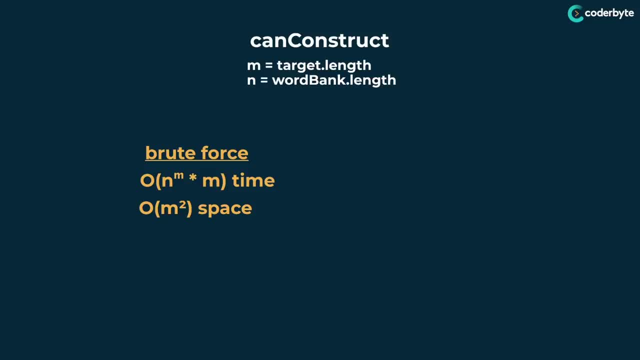 m And when we memory was our solution, we actually improved it from exponential. So now the time complexity of our solution is an M times m squared right, And the reasoning is now we don't have to fully explore any duplicate subtree Every time we run into it. 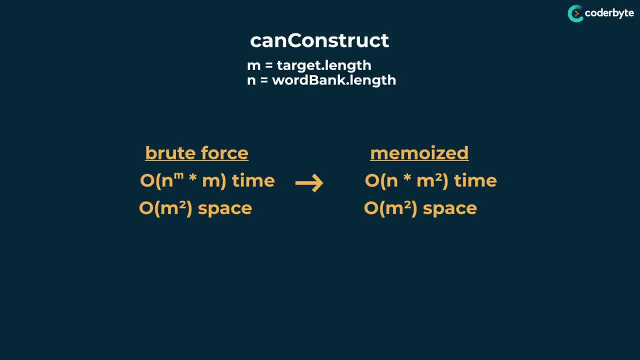 Instead we just store the results and then memory and we can just kind of short circuit and fetch memo. Notice that I have an M squared in the memoized type complexity. that second M really comes from the fact that we still have to do the slice. we still have to pay for that cost. 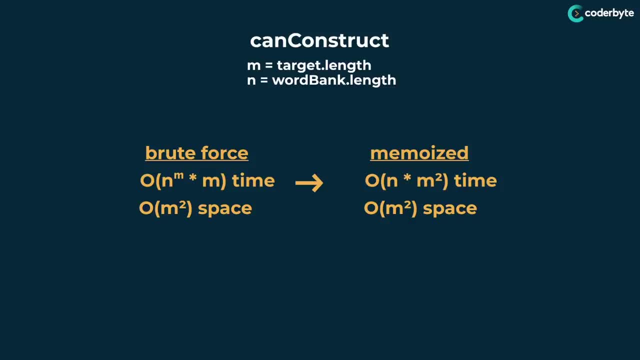 So, although we added an additional object in our memoized solution, our space complexity would remain in the polynomial class. So overall we definitely prefer this second solution because we remove some exponential- you know- complexity. So now is reasonable to actually run this in an amount of time. I think that wraps up this. can't construct problem. 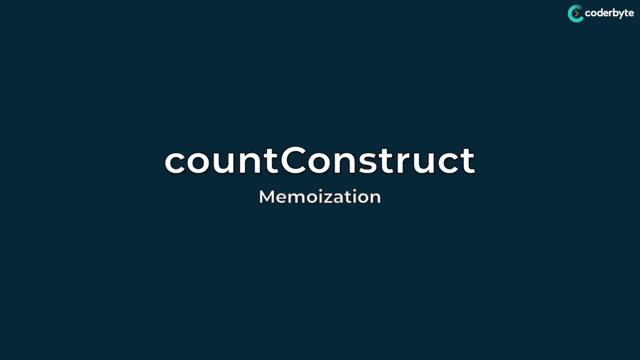 Now let's work on the counting version of this problem. In particular, I want to work on count construct, So we have the same setup here. I want to take in still a target string and also an array of words in a word bank, But this time I want to return a number. I want to return the total number. 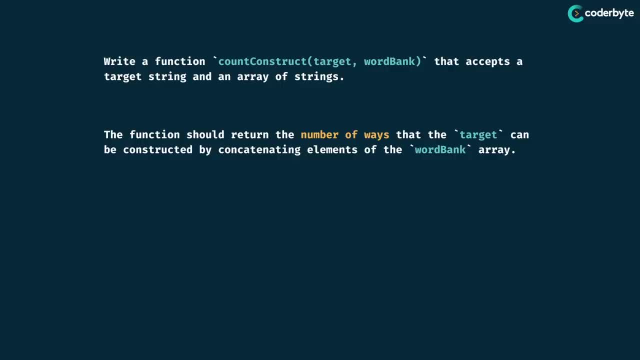 of ways that the target can be made using words of the word bank And, like before, we can reuse elements of the word bank as many times as we want. So notice that this question asks us to do something slightly different. We don't want just true or false. if it's possible, we want the exact. 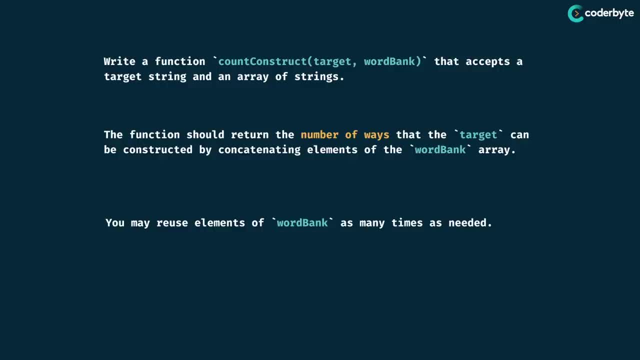 number of ways that we want to use the target string. So let's do that. So notice that, this ways that we could construct the target string. So let's take a look at some examples And also, you know, take a high level view of the strategy here. So let's say: I gave you. 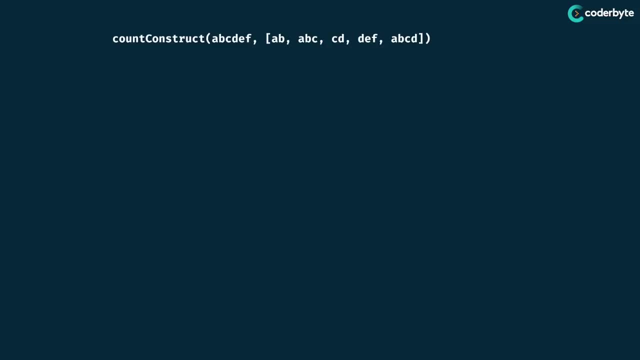 this string of ABCDF And this array of words, this particular example we saw before and it is possible, And there's actually one exact way we can generate ABCDF, So we can construct the tree in the same way we did before and we end up with this, However, this time around. 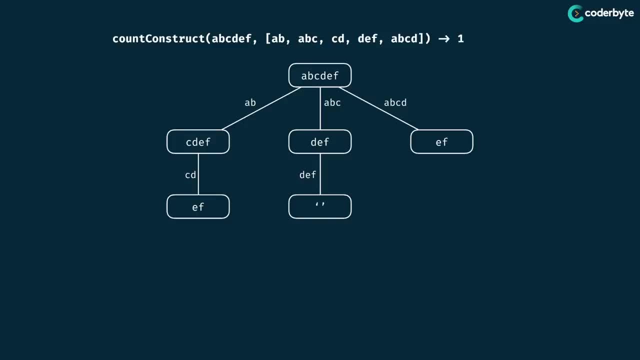 we want to choose a different value to return for our base cases, as well as changing the logic for reconstructing our sub solutions. right And so, if I look at the base cases here, I want to kind of just adapt the return value for this new type of data that I need. 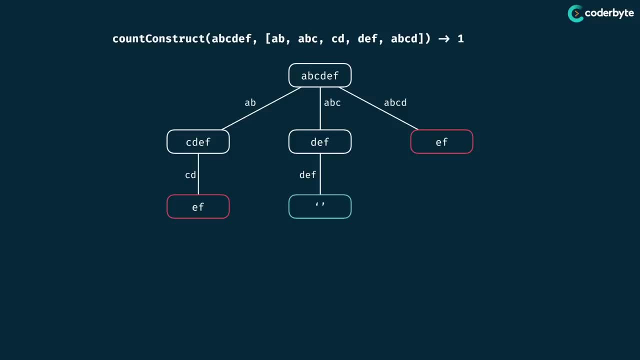 to return, which is number. So I think the move is for these scenarios where we can't break down our current target any further. that's your return. zero right EF can't be broken down because it doesn't have any more matching prefixes from the array, So that 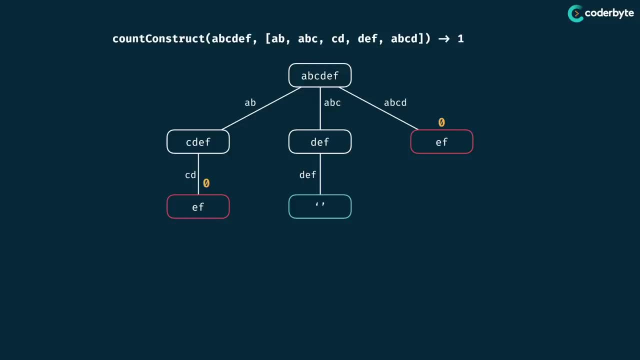 means there are zero ways to break down EF, And so we should return zero And those sort of scenarios. And then when we have the empty string, we know it was successful. So we could always, you know, create the empty string, And so that should return one. And we've seen. 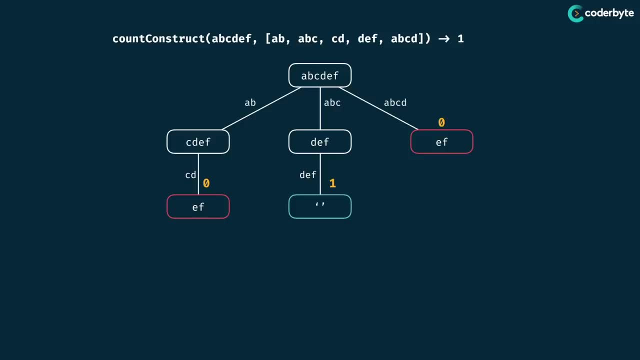 this logic before in problems like Fibonacci, as well as our grid traveler problem. we just want to bubble up these values to their parents and make sure every parent will add up all the numbers that come back from their children. So it just bubbles up like this And top level. 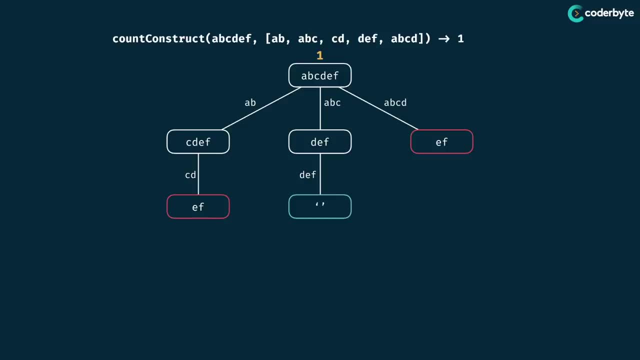 we do zero plus one plus zero, which means that we can generate ABCDF in exactly one way And the way that actually is symbolized inside the tree. it's exactly the path from this root node all the way down to that lone base case that returned an empty string right. 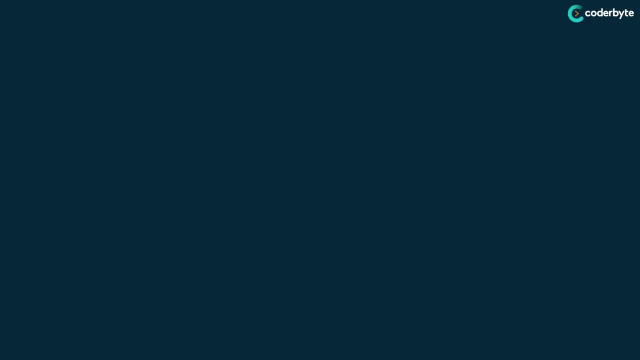 ABC plus D, F. Let's take a look at another example. So here I have the target string, purple, and I have some other characters and words inside of the array, So take a moment to look at the input here and predict what number this should return. 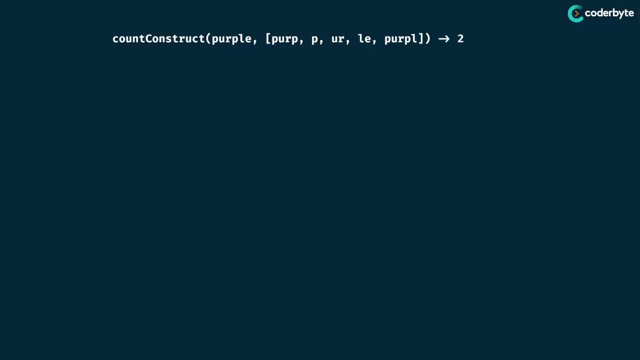 So the answer here is two right. there are two ways to create purple. So if we construct the tree, we know we start with the initial node of purple. then we have about three prefixes that match here And those yield some children. we can follow the same pattern recursively. 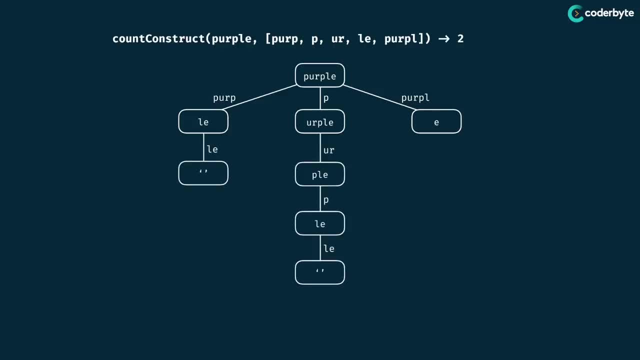 down the tree, So the full tree really looks like this. notice that I have two base cases that actually end up as the empty string, So I know those are going to turn one out to their parent. And on the right hand side I have a lone e that can't be broken down. 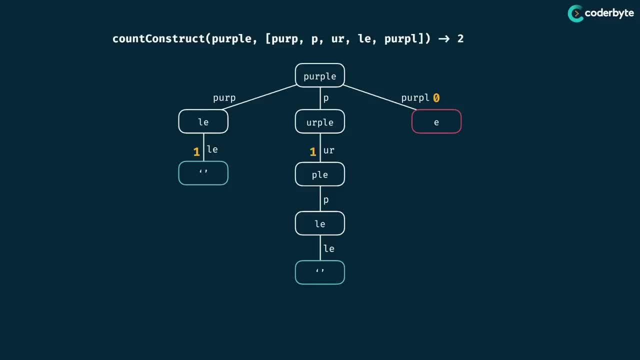 further. that returns zero And, like always, right. I just bubble up these values until at the parent. I actually do one plus one plus zero, which gives me two right. there are two distinct ways to create purple using this choice of word bank. All right, I think. 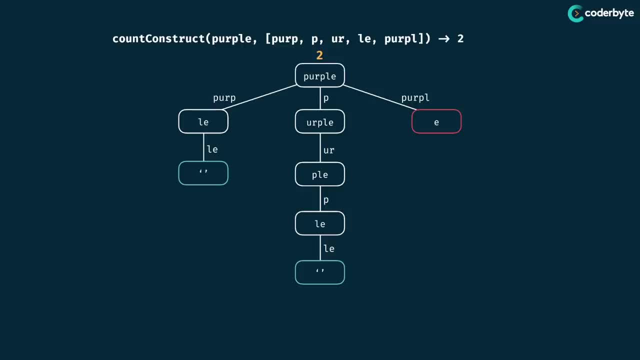 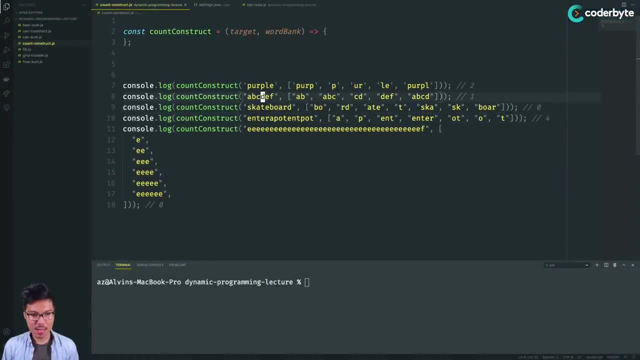 I'm feeling pretty good about jumping to the code for this one. It's really just a small variation of the last problem we did, So let's hop right in. All right programmers, back in the code editor. let's go ahead and bang this one out. So I already have some examples. 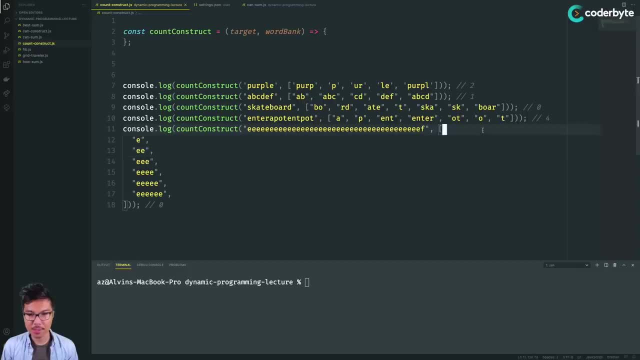 that show us what numbers we should return for this count construct right. So I have some examples here. Notice I even have that big example with our large input, So we know that that will probably need to be optimized. Let's lay the foundation with the brute force. 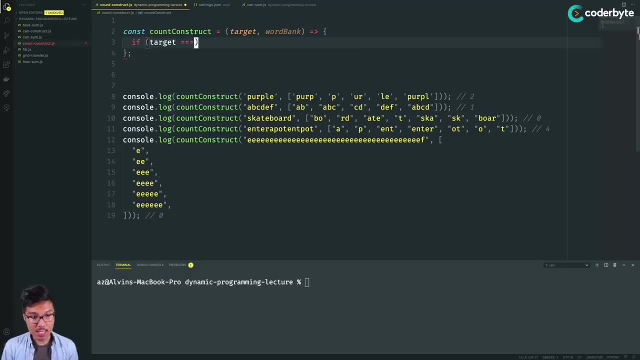 So we'll start with the same base case as always, right? So if the target is the empty string, then we have trivially solved the problem, meaning that there is definitely one way to generate the empty string. right? just take no elements from your word bank. 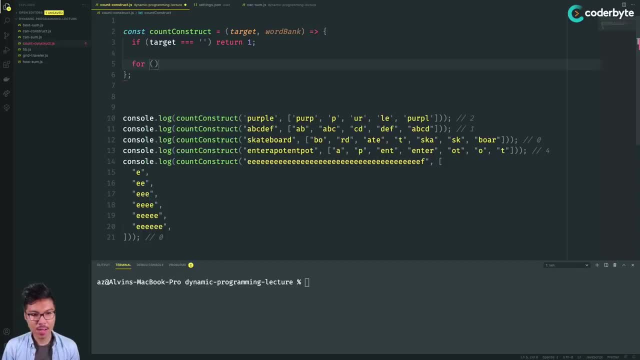 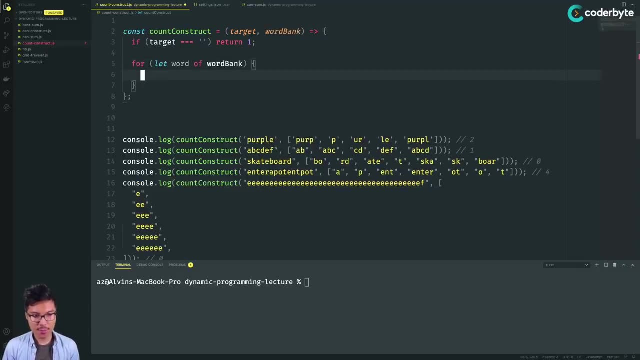 Along with that, I need to make my recursive call. So the usual structure, right? I want to iterate through every choice of words. So for let word of word bank, and then for every word of that word bank, I need to check if it's a prefix. So we've done this before. 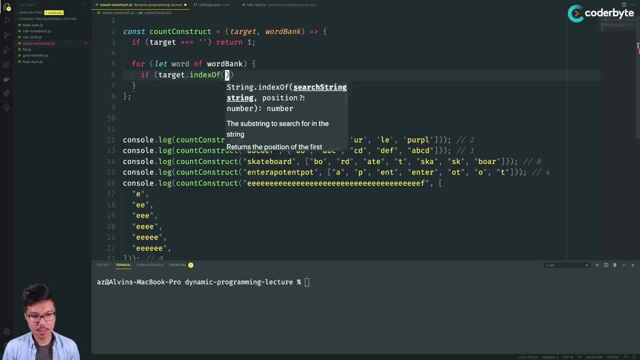 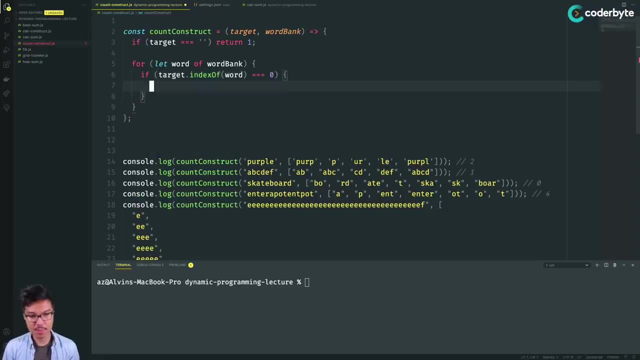 if the target dot index of word bank, or rather index of word, if that is equal to zero, then it must be a prefix. And if it's a prefix and I can go ahead and take, like the rest of the word, or that is the suffix, and call recursively on it, So I'll do this in line. 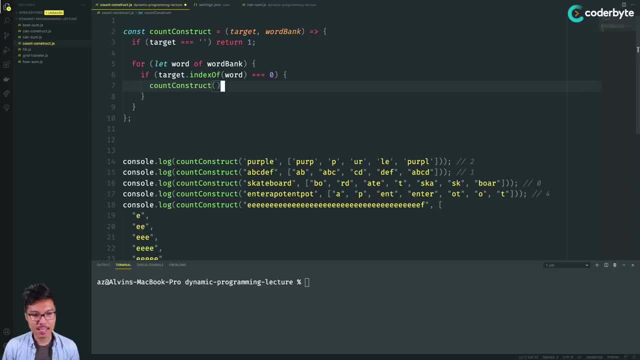 now say count, construct, and I'm going to pass in the rest of the word, which would be target dot slice, then I'll slice starting at word dot length. So this means that the slice contains everything after the word or everything after the prefix, And so I'll also. 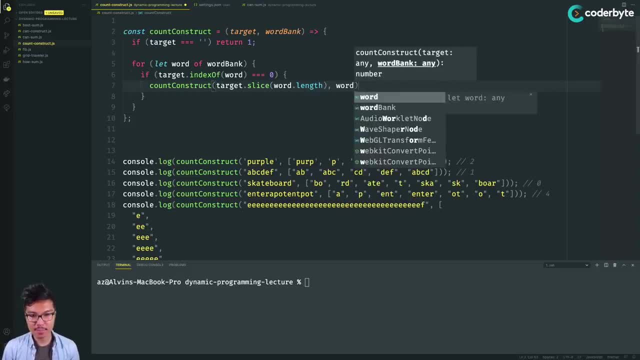 be sure to pass into the second argument the same word: bank Nice. And now I need to think about what count, construct returns. So it's returning a number, now, right. So in particular, this will be the we'll say num ways And I'll say num ways for the rest. 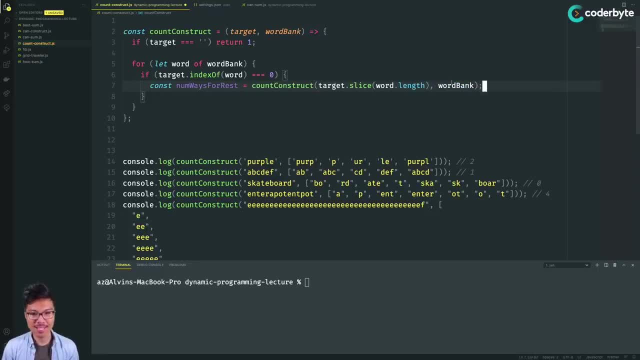 maybe a little wordy of a variable name, but I think it does describe how exactly what this returns here, right? So this is a number of ways that we can generate the suffix or, like the rest of the target. What I want to do is keep a running total. So, outside this, 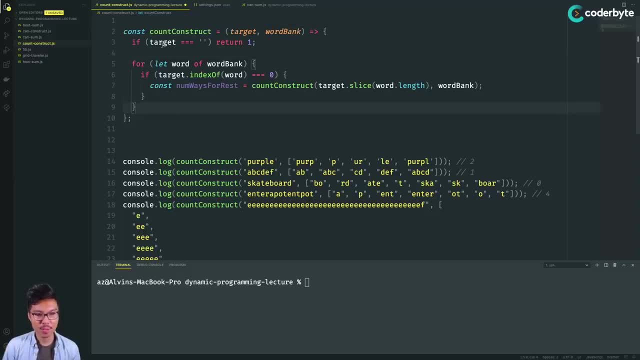 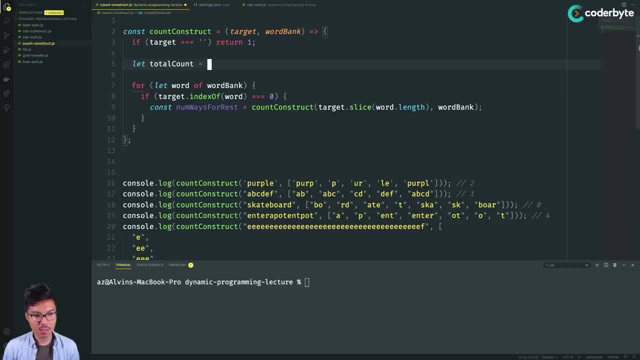 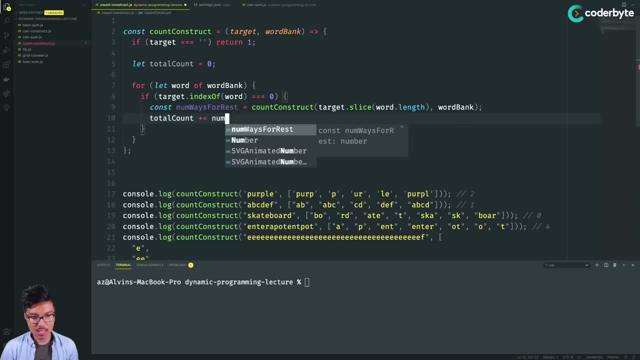 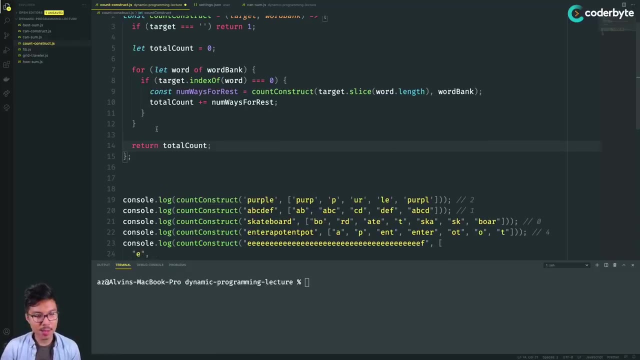 as total count plus equals the number of ways to generate the rest of the string right after I have removed the word And after I take the total through the entire for loop, that I can just return the total count. Something really great about this, this programming pattern is, let's say, that none of 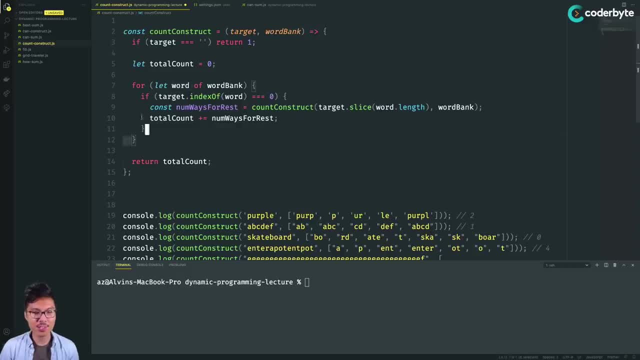 the choice of words were a valid prefix. So that means I finished this for loop And this if statement is never true, If this if statement is never true, that I never add anything into the total count. So if I return total count afterwards, I return a still zero, which makes sense because 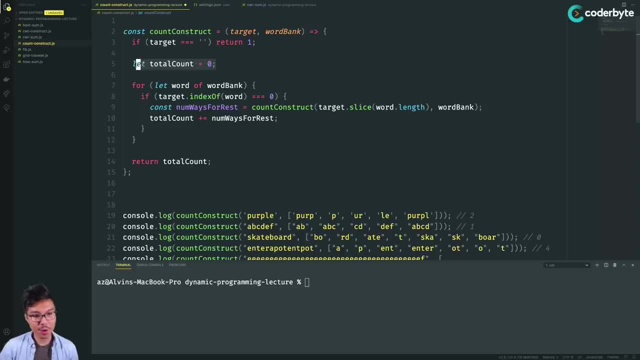 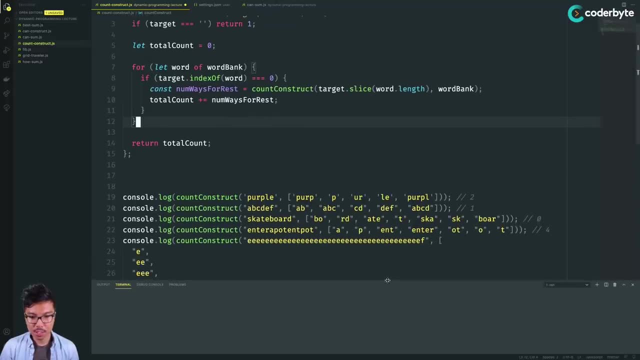 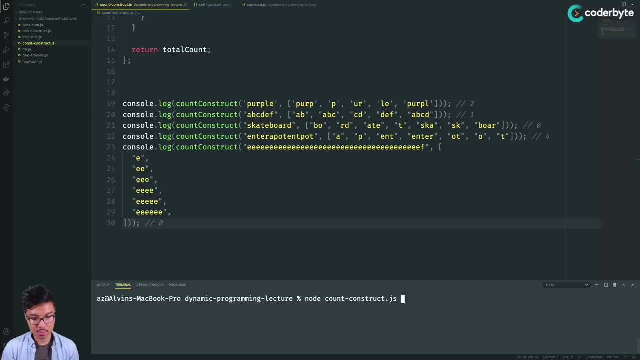 apparently there are zero ways to make the target right, have no initial step to take in the word bank, So let's go ahead and test this one out. So looks like we should get 2104.. And then also a zero at the end. Let's give that a go. So 2104.. And it looks like the last example is just a little. 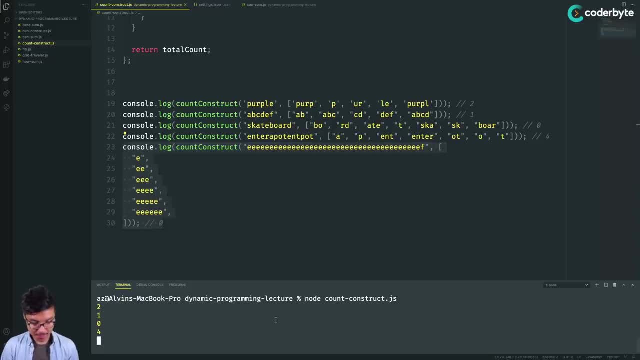 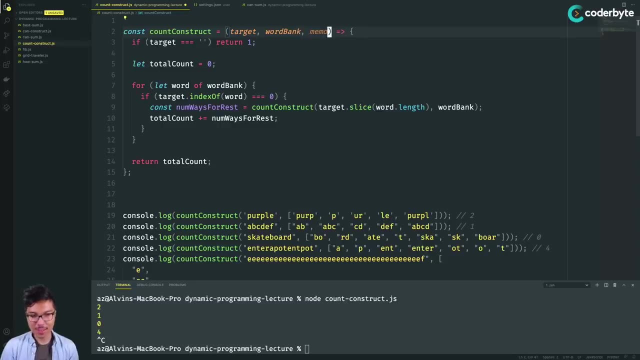 slow for us, So you already know where this one is heading and we tell the program: let's just go ahead and just memoize this one off the bat, right? Hopefully, I think through all these examples, you're feeling really good. 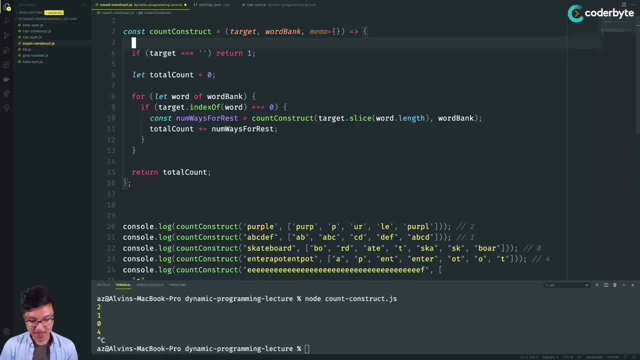 good about memoization And it's a pattern that we basically have drilled into our minds already. So if the target is in the memo and just return the stored value memo at target, and then I'll need to adjust my return value right, So where I return over here is 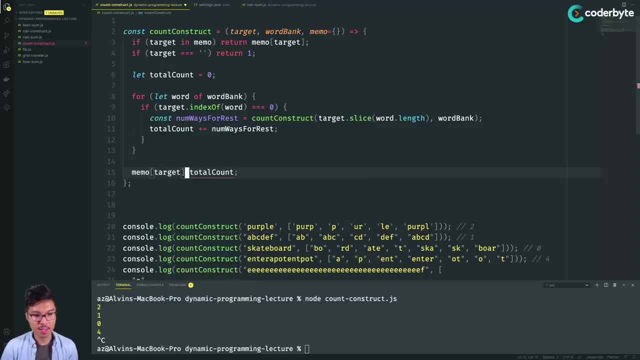 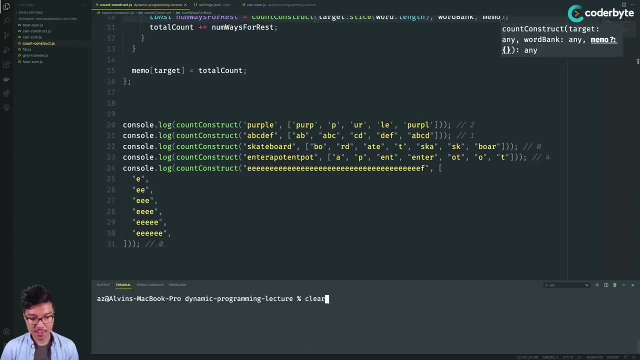 I'll store that total count as the value corresponds to the target, And let's not forget to also pass in the memo to our recursive calls. right, So memo goes right here. Nice, So let's give that a run Again. I expect a zero for that last answer, right, So looks like I have a error over here, And of. 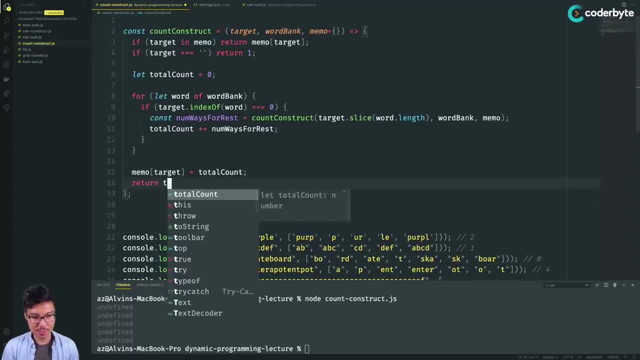 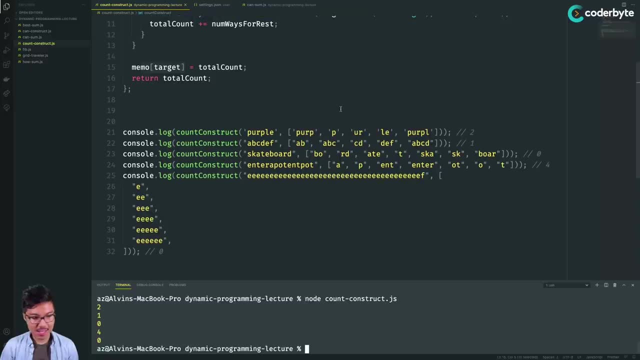 course I forgot to actually replace my return value, So I can still return the total counts And in addition to that, I'm actually adding it into my memo. So let's try that now. Yeah, and these answers look correct. right, I get zero for the last one. notice that the last one is not. 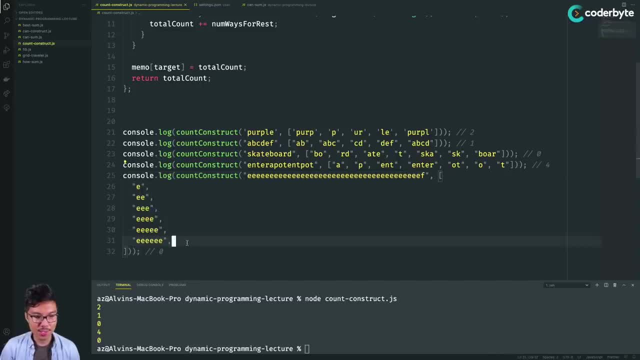 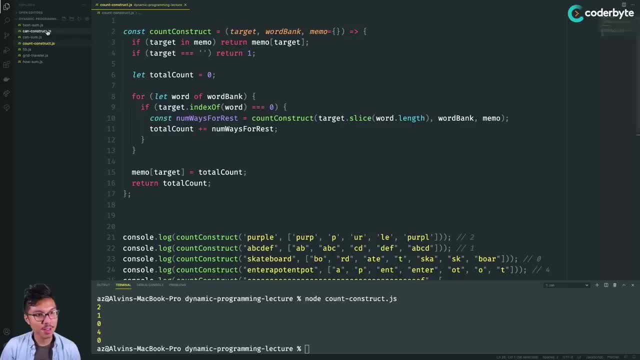 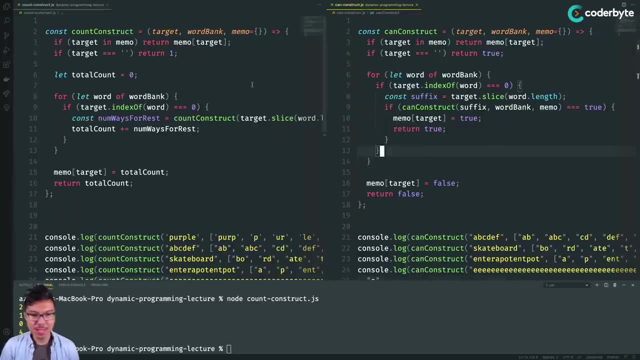 pretty simple code. It's a pretty simple code. It's a pretty similar to our previous problem of can construct. if I kind of split these, can construct basically has the same shape. Really, the only difference is this number of variable that I add into and, of course, the return. 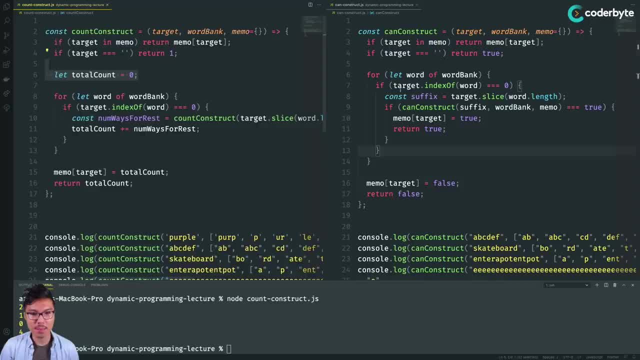 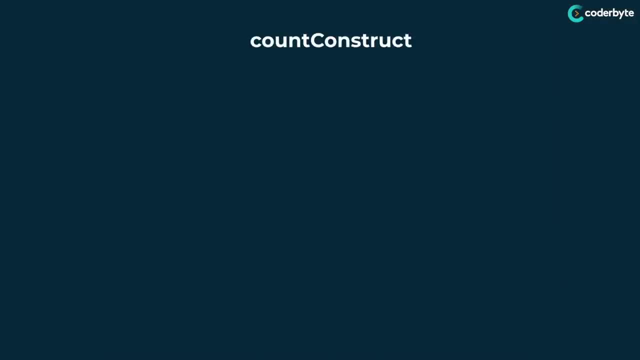 values. So we do expect the complexities to be the same for these two functions. Let's wrap this one up on the drawing board. Let's look at the complexity of this. As always for this count construct problem, our M is going to be the length of the target string and our n is going to be the 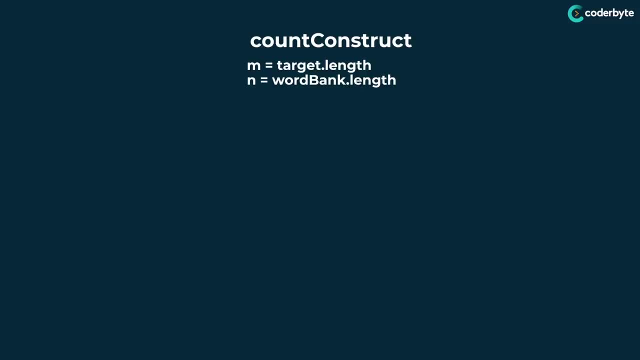 length of the array- right, So that means the number of elements in that array. our brute force is the same as it was in the can construct problem, right. So it's still exponential And using memoization we just brought that down from an exponential to a polynomial time complexity. 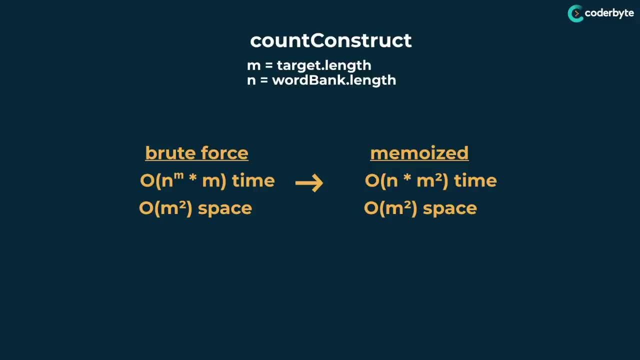 and the space complexity remained the same. Really, there is no additional cost that we pay in our implementation for this counting version of the problem, right? The only difference is now we're maintaining a number that we just add to, you know, on every iteration of that for loop. 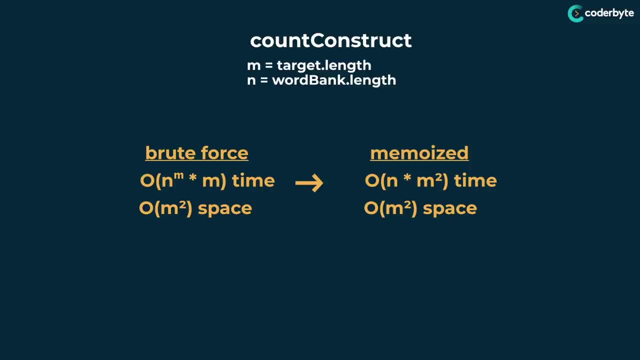 but that doesn't really affect the runtime or the space complexity at all. So I think this wraps up this count construct problem. Now I want to do one more variation of this string problem. So what I want to do is write a function called all construct that has the same setup right. So I'm going to 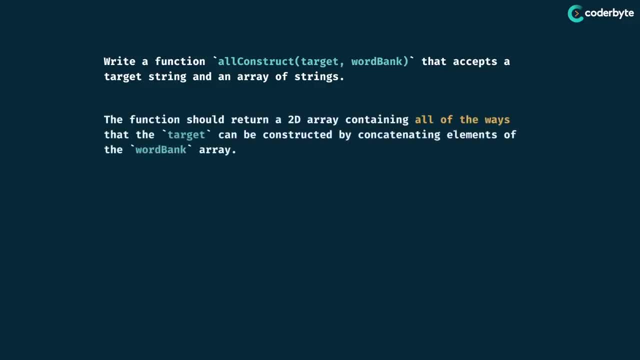 take in a target string as well as an array of words in a word bank, But this time what I want to do is return all of the ways that the target can be constructed by concatenating elements inside of that word bank, And that means I should return a two dimensional array, a single element. 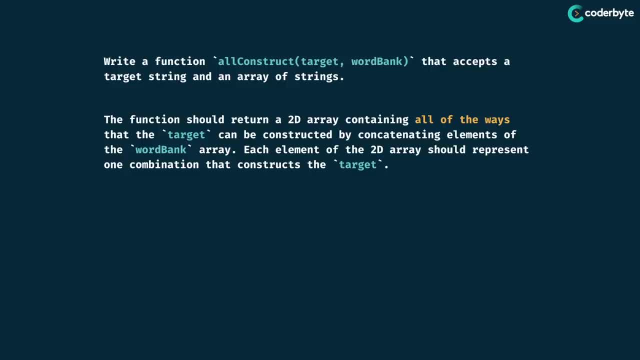 of that 2d array is going to represent one of the combinations that can construct the target right, And I want to return all of the ways within a 2d array. And, as always, we can reuse elements of the word bank as many times as we need. So let's make sure we understand this question by 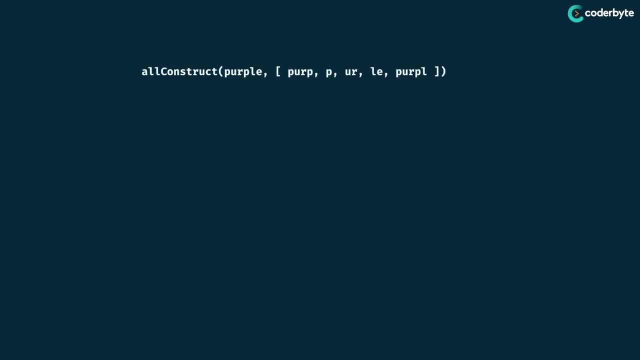 looking at some examples in their output. So here's an example using purple, and it's the one we've seen before in the last problem. In the last problem I had us return two because there were two ways to create purple. But now I don't want the number, I want the exact ways that actually 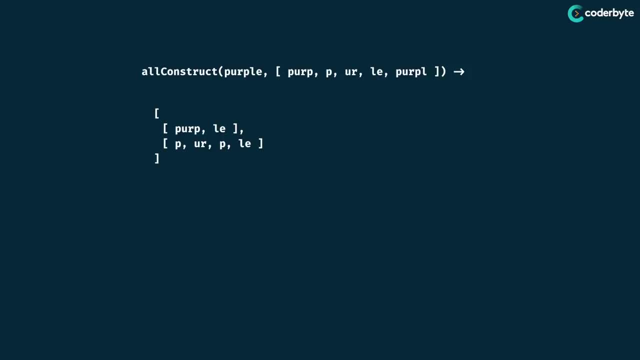 create purple. That means you need to return a two dimensional array of words, And that means you need to return a two dimensional array of words. And that means you need to return a two dimensional array of words, And that means you need to return a two dimensional array, The outer array or the. 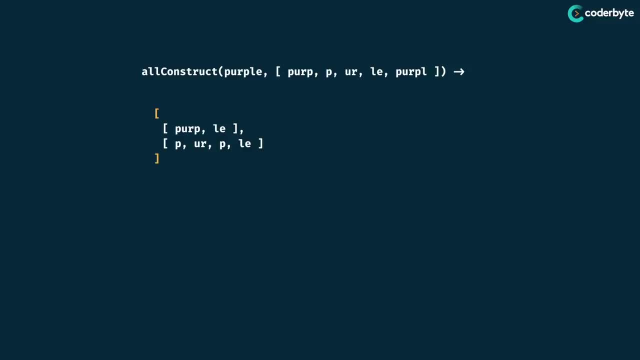 outer set of brackets represents the collection of all combinations, whereas a set of inner brackets or a sub array represents one of the combinations that creates purple. Let's take a look at another example. Let's say I gave you ABCDEF And I gave you this long array of word. 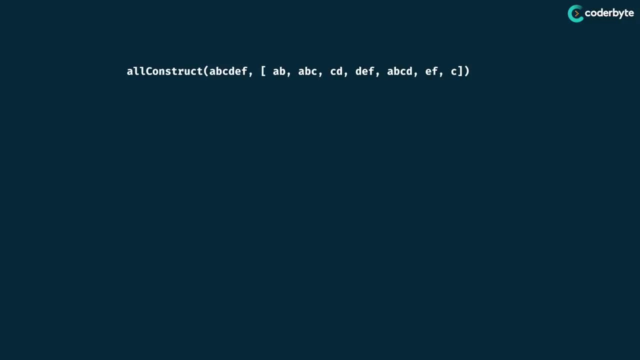 bank. notice that I actually added some elements inside of this word bank array. it's a little more complex than our previous examples. Because of this, there are actually many ways you can create ABCDEF, And this contains all of them, right? So there are four ways that you can create ABCDEF. 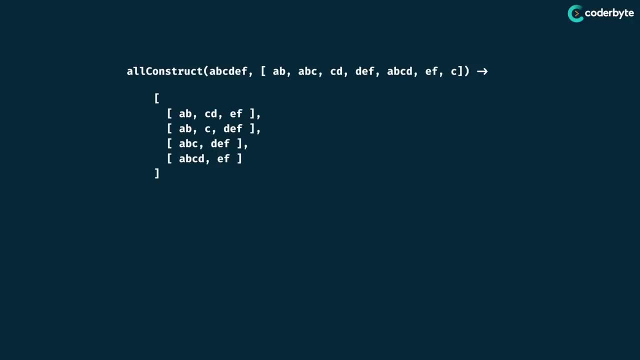 So there are four ways to create our target string. And again it noticed that each sub array represents one of those combinations of words in the word bank that creates the target. Cool, So now that we kind of understand like the shape of this problem in terms of the data we 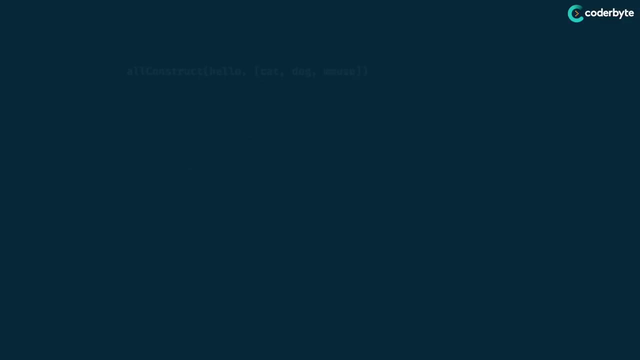 should return. let's take a look at some base scenarios. So let's say I gave you this example right, so I have the target of Hello and my words in the word bank are just cat, dog and mouse. Obviously, you know that is not possible to generate Hello. So there are really is your ways. 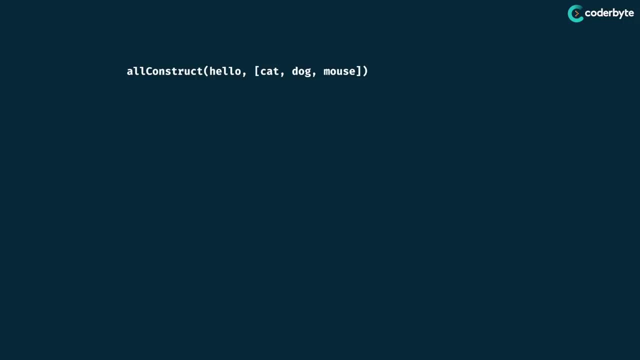 to create this. how should we actually return an answer here? Well, I think it'd be reasonable to return an empty array. Remember that we're saying the outer array in this context represents the collection of all of the combinations that can create. Hello, since there are zero. 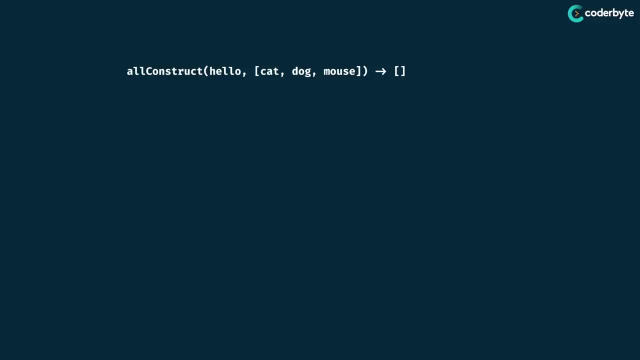 ways to create Hello. that means that our collection is empty, right? This has a length of zero, meaning there are zero ways to create Hello. Now let's say we had another base scenario, Let's say we had to generate the empty string using the same array of word bank, And that 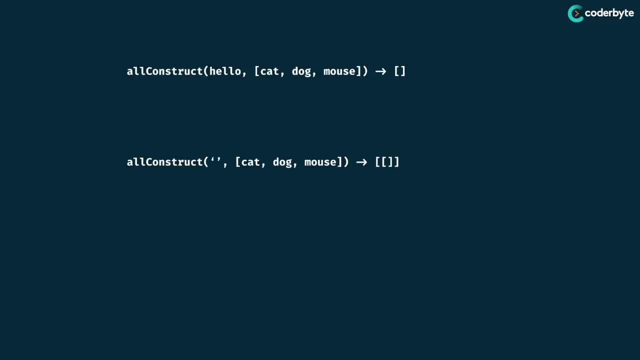 scenario, I think it's reasonable to return an array containing an empty array. And again, the reason is: if it is possible to create the target string, then we need to return a 2d array, right where the outer array represents the collection, And if there's one sub array, 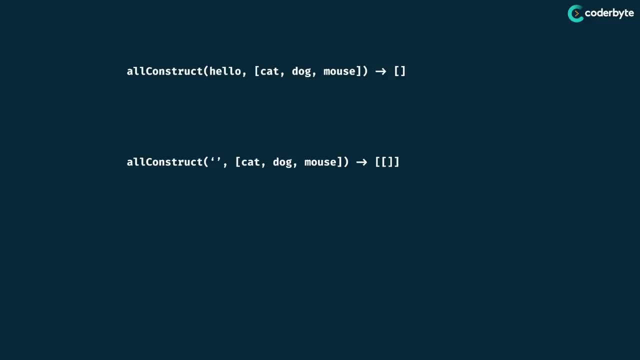 inside of that outer array. that means there's one way to create the empty string. And what is that one way? Well, it's to take no elements from the word bank. So I think this is going to be consistent logic. this is going to be a really important way to think about this. 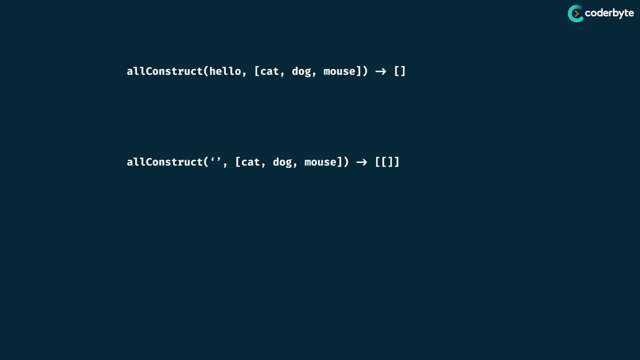 problem, That is, when we're given a target that cannot be constructed using the word bank. we should return an empty array right, a one dimensional empty array, because there are zero ways to create it. On the flip side, if I've ever given the 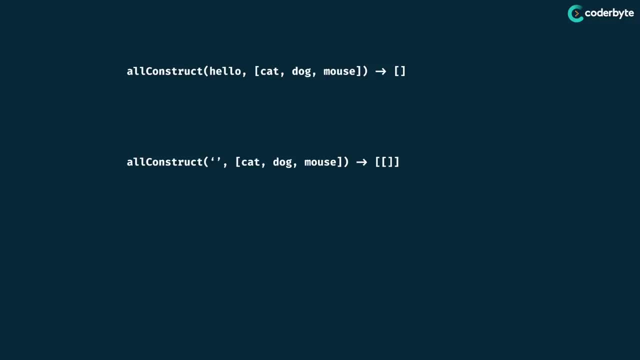 empty string. we know that it's always possible, And so we should return like a two dimensional empty array. Cool, So with that, let's look at some tree examples now. So let's say I had this large example from before. we know that the overall tree, like we've always know, 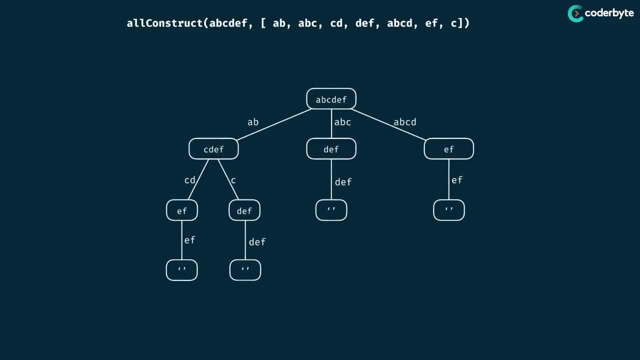 created would look something like this: Obviously, now we're just reframing this problem in the return values that we do for our base cases. So you notice that there are four base cases here that kind of reached the empty string And I know that those represent the four ways to create ABCD F. Now I have to adjust the 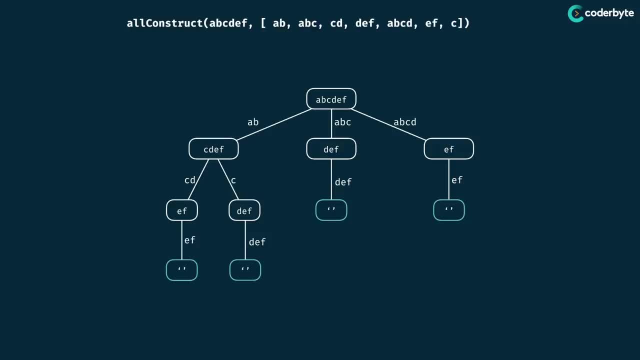 return values here. So I'm already saying that if I have the empty string, then that should return an empty 2d array. So it looks something like this, right, And how will I actually reconstruct the entire solution from these very small sub solutions? So let's just 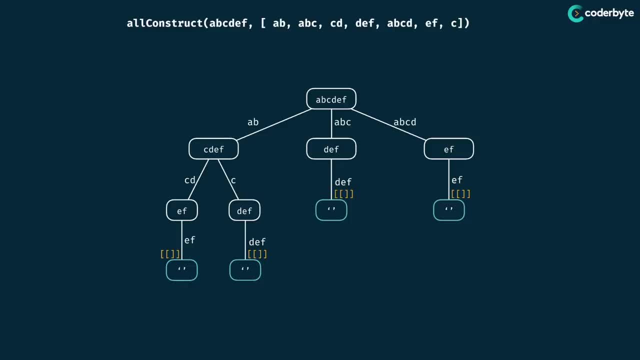 stay focused on the left sub tree right now. I know that these arrays are going to return back to their parents, And when I do that, I also need to make sure that I include the edge that I actually use to transition to the child, In other words, 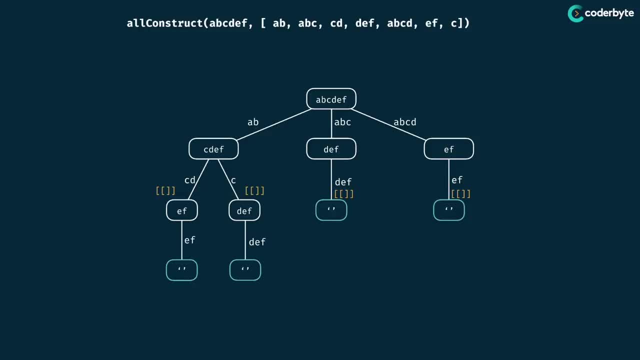 I'm going to be sure to push the label for the edge into each of those sub arrays. So the key insight is this: right, I'm just pushing those edges into their sub arrays And from here I continue the pattern up a little further, right? So I know that these arrays return. 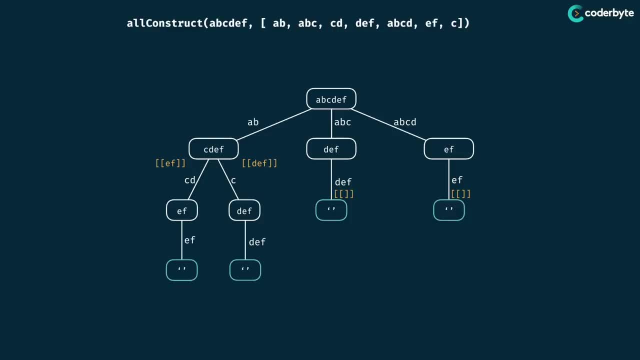 their parent over here And I still, you know, push the edges that I took to get them back. I took to get to those children. So, on the left, I'm going to put CD in the front, on the right, I'm going to put C in the front, resulting in this: And then, at this point, 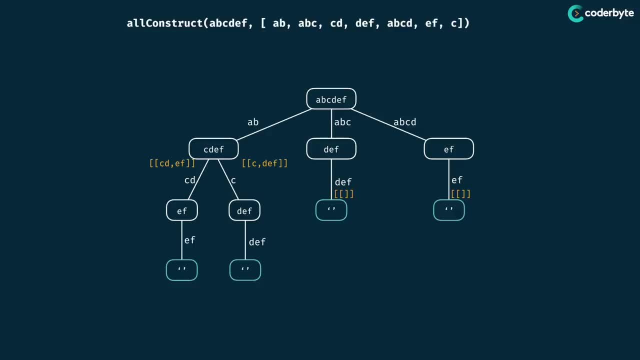 notice that this node rooted at C, D, E, f. that is actually going to receive both of these collections, right? And what should this node do? Well, it really needs to just combine a both of these arrays. recall that, you know, we technically receive a two dimensional. 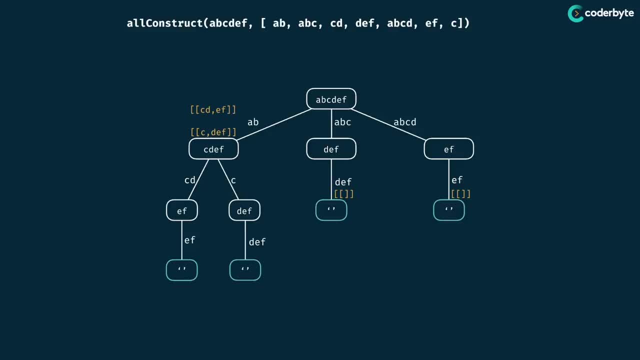 arrays, which means that a sub array represents one of these sub arrays. So you see that the sub array will actually perform a job through the random table. So, if I repeat what I said, the sub array here will actually run a single array. So I'm going to go ahead and just use this. 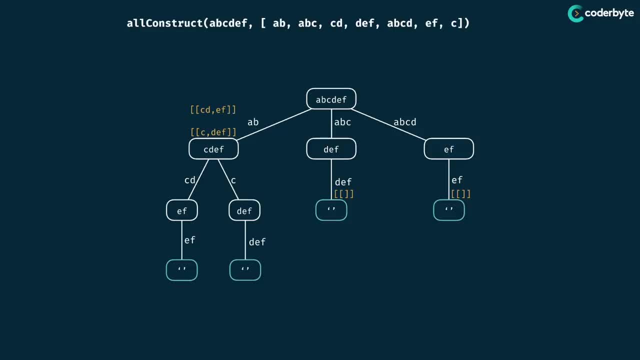 of the ways to create the actual target. So if I just concatenate these two two dimensional arrays, that yields this construct, And if I do a quick spot check, I'll see if this is compatible with what the question is asking. right, This is a two dimensional array And I know there are actually 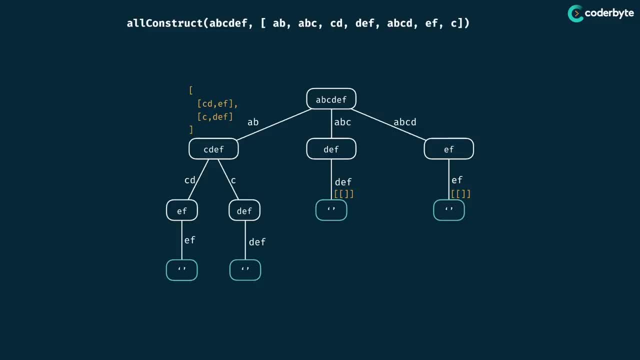 two ways that we can create CDF. If I look at what this is saying, the first way is to do CD plus EF, and the other way is to do C plus D, F, And so this cell problem is correct in itself. So I'm going to. 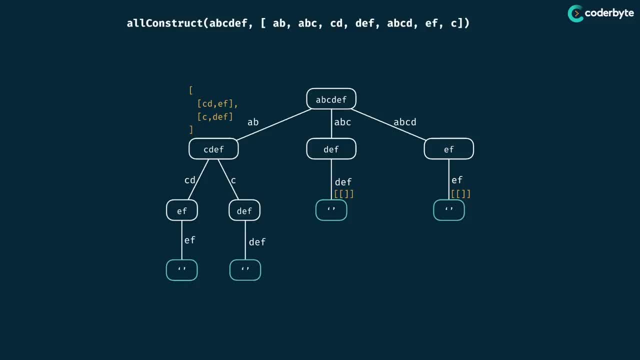 use the same exact logic to trace through the right hand side. I know that these cases return to their parent. then the parent is responsible for adding the edge to each of those sub arrays like this. Now I'm just going to reorganize everything at the top, just to give us some more. 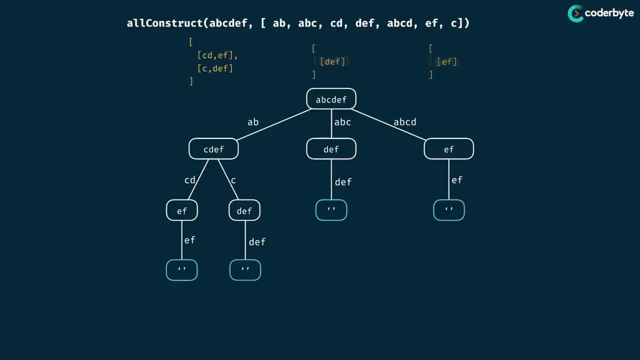 room And maybe I'll even spread out these brackets to make it look more symmetric. But I'm not done here. I still need to consume each of the edges at the very top of the tree. So if I look at my left hand set of arrays, I know that those need to receive a B. 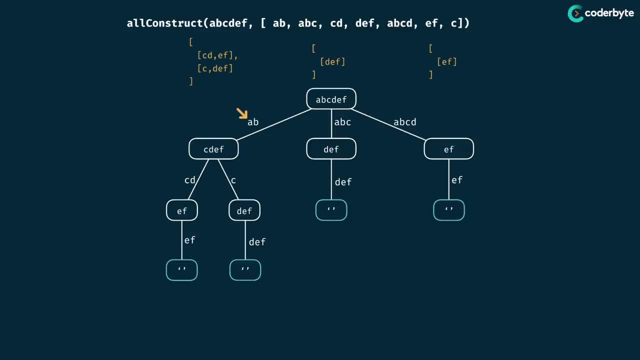 in other words, they need to have a B place at the front of each of those. So I'll just do that right. In the same way, all of the arrays in the middle, which is really just a one sub array, need to add ABC to. 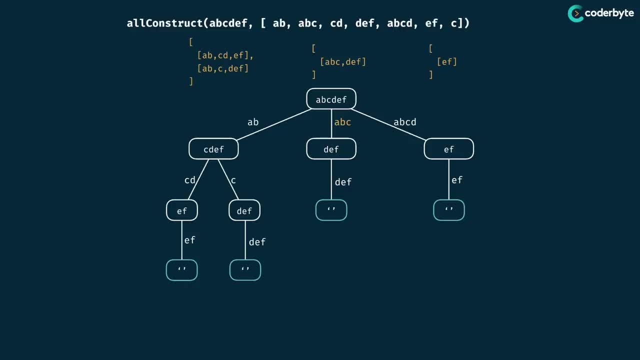 the front of them like this. And finally, same thing on the right hand side with ABCD. Cool. And if I look at what I have, these represent the four ways that we can actually create our original target string. But at this point, 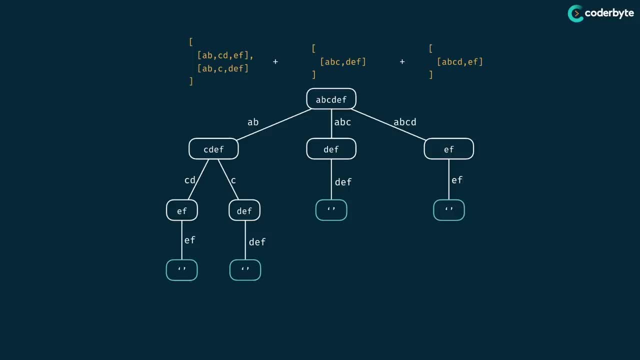 the root node just needs to concatenate each of these two dimensional arrays together, So it really just combines them into a single 2d array like this. And if I do a quick sanity check, I know that each of these sub arrays represents one of the paths that I can take to a base case. 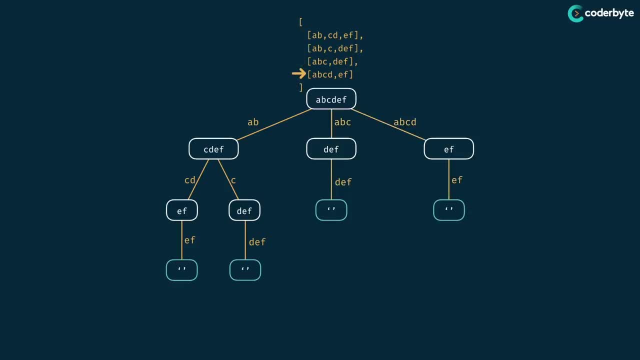 down my tree, which is exactly what we intended at the start. So this type of recursion is definitely more complex than the previous examples, But hopefully you can recognize what's similar to our last examples. right, Let's do one more together, though. Let's go back to this purple example. 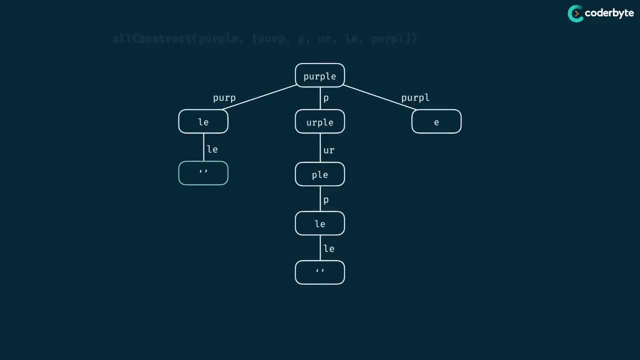 the full tree would look like this And we'll trace through this. So on the left hand side, we're going to start with a 2d empty array right, Because that's the base case for the empty string, meaning that, hey, it is possible to create the empty string in one way, And that is to 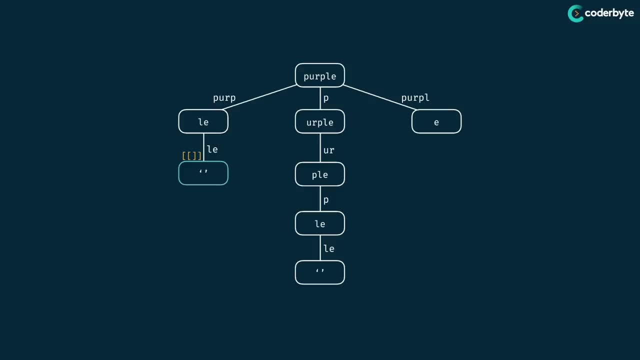 just take nothing. So I do the same logic as our last example, meaning I returned to my parent, but I'm being sure to also include the value of the edge right, And so the key insight here is: I'm being sure to add the edge label and not the actual node label here, the node and the edge. 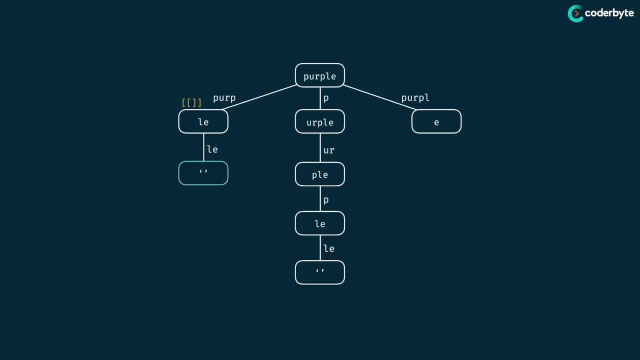 have the same thing, le, But I'm really looking forward to adding the edge right, So I add le over here, And likewise this returns to its parent even further, And so we'll add that last edge of perp. Cool, Now I need to do everything for this middle path, And so what I'll do is 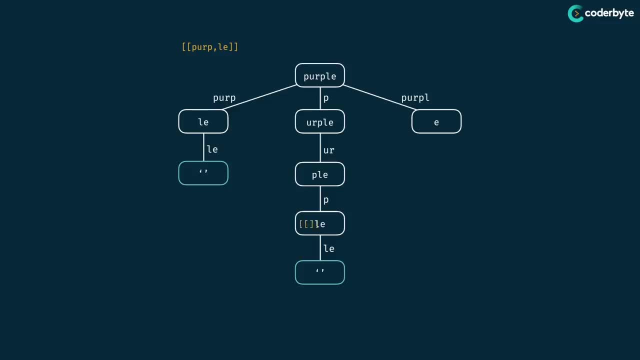 return the empty 2d right at the very bottom And this really bubbles up all the way to the top And we just accumulate every edge label as we go right. So it sort of looks like this: And what's really interesting about this right hand path, this is actually a base case that 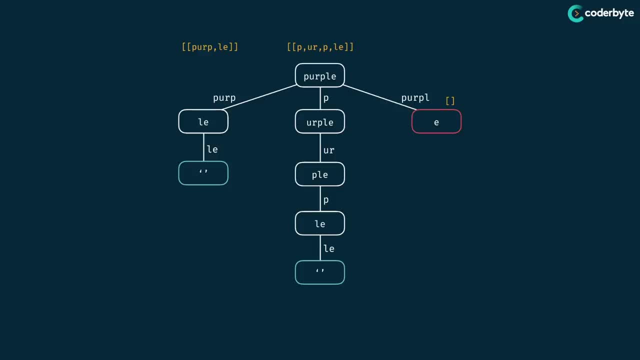 doesn't work out, meaning we kind of hit a dead end at E, And what we said in our initial examples was: whenever we have a target string that cannot be created at all by using words of the word bank, then we're going to return a one dimensional empty array, And that actually works out in our favor. 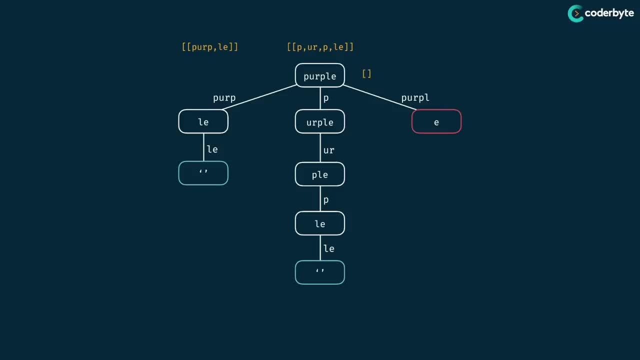 because if we return this empty array to our parents, our parent is going to try to add the image into every element of this empty array, But if there are no elements in this array, then it's going to add nothing. In other words, this one dimensional empty array. 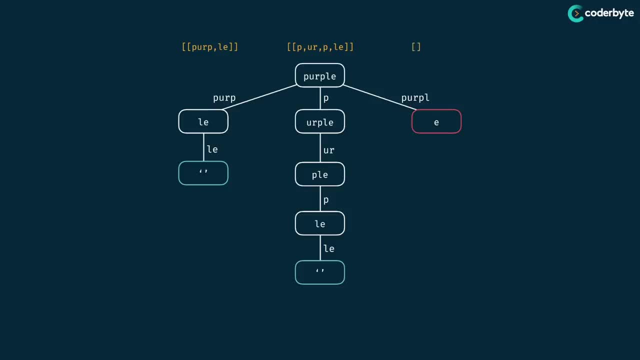 really just bubbles to the very top And, like always, if I just concatenate all three of these arrays together, I actually end up with my final answer. notice that when I concatenate an empty array to the rest of these, I will actually contribute nothing to my final answer, which. 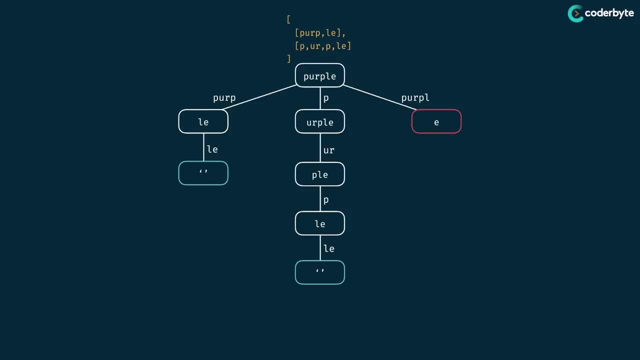 makes sense, because there are no paths that work out on that right hand side. So our final answer is just this: Like we know, both of those sub arrays represent the two different ways that we can create purple. All right, I'm feeling pretty good about this process. Now let's go ahead and 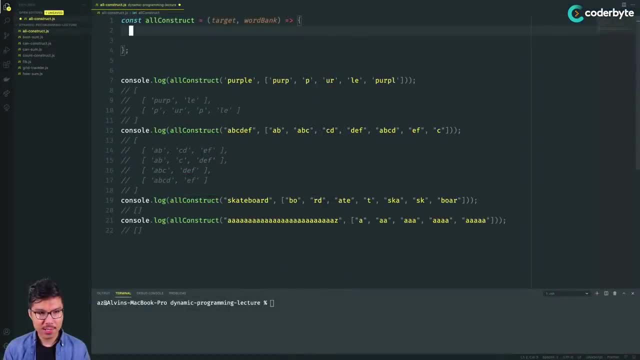 code it up. All right, programmers back in the code editor. another problem, another solution. So let's start by laying out the base case over here. Now, like we said, we'll say, if the target is the empty string, then we want to return a two dimensional empty array. right, The single. 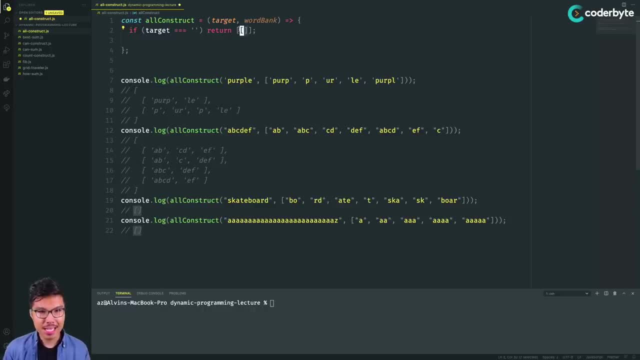 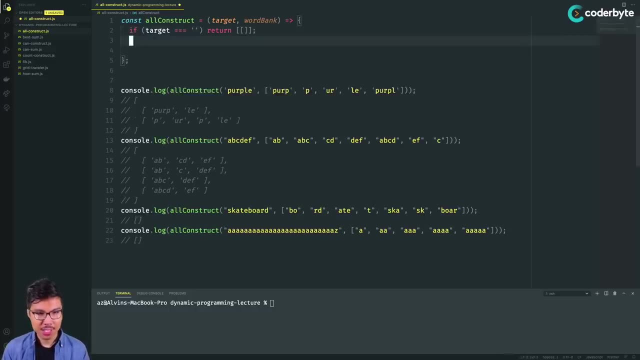 sub array here represents the one way you can create the empty string: by taking Nothing right, by taking no words of the word bank Nice, And then, besides that, we need to make our recursive logic. So that's going to be very similar to what we've always done for this. 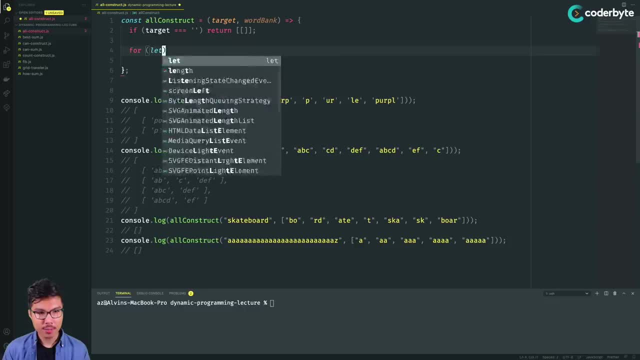 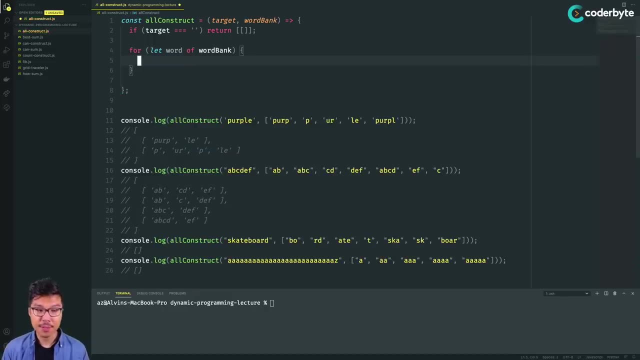 style of problem. So I'm going to iterate through every word of the word bank. So I'll say: let word of word bank, word bank, And I need to still check if there's a prefix, right, if this word is a prefix. So if target dot index of word, if that index is zero, then I know that it must be a. 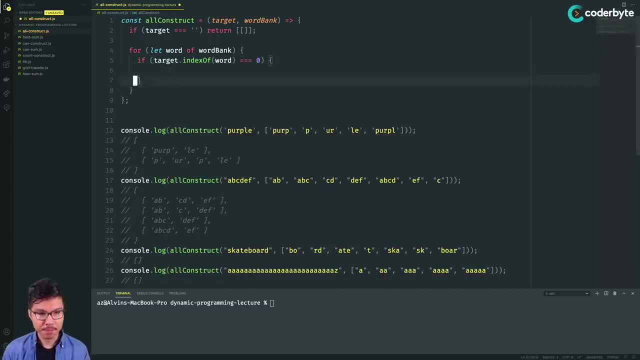 prefix So I can continue Some code inside Nice. And so what I'll do is I'll go ahead and create an extra variable just to store the target after I remove the word, which would give me like the suffix. So I'll say const. 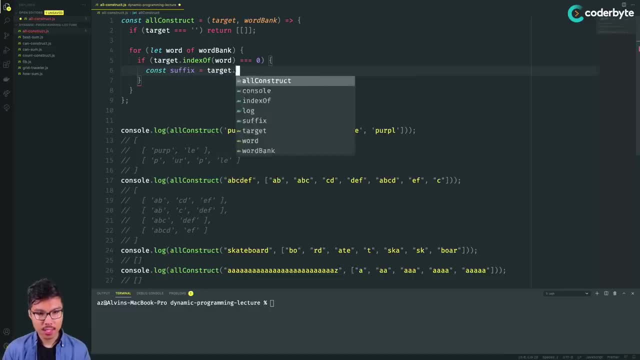 suffix equals and I'll say target dot slice of word dot length. So we've seen this pattern before. but just to refresh, this just gives us everything after the word. So basically, once you move the word, what is the remainder of the string all the way to the end? Now that I have 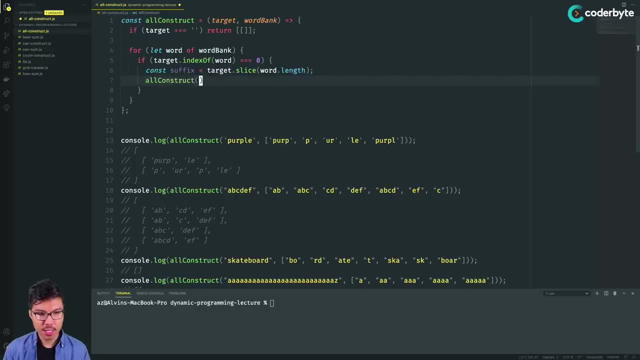 this function. I actually want to call my function recursively on that remainder Right, Just like this. I'll pass along the same word, bank, Cool, And now here's where things gets a little intense, right. So we've been doing a lot of problems. you're using this recursive structure and 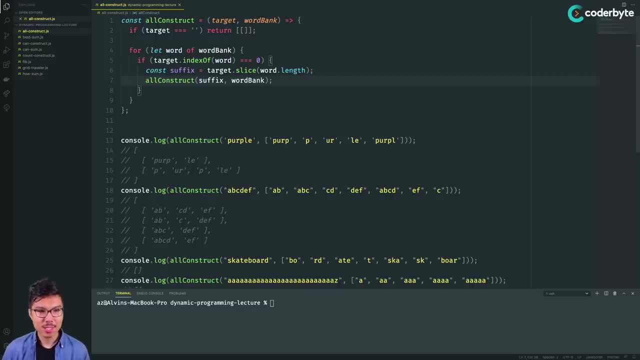 then we memorize it in the long run. I think the most important thing to do is, when you make your recursive call, you really just assume that your function works right. So I think about what type I should get back from all construct. So I know that, all construct. I'm just going to. expect my backend to actually do the same thing. So I'm going to go back to my function So we'll see if I can get a regular call. So I need to go ahead and right click on if this is a recursive call. So right. so I think about what type I should get back from all construct. So I know that all construct. 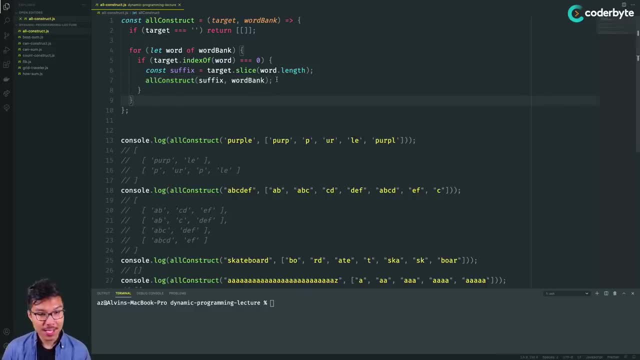 So I know that all construction give me back an array right. it's gonna give me back an array containing all of the ways to make the suffix. If there are no ways to make the suffix, then it's going to give me like an empty array right, And so I'm going to assume that here, So I'll create. 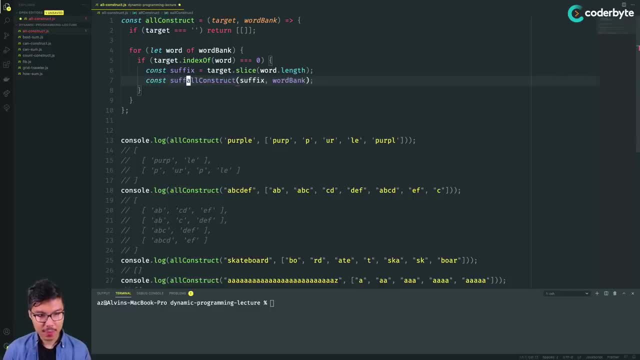 a variable, And I'll call it, let's say, the suffix ways, And the reason I'm naming it like this is I really want us to, in our head, think about the return value from this as an array of all the ways to build the suffix. Cool, So that's going to be a two dimensional array, right? 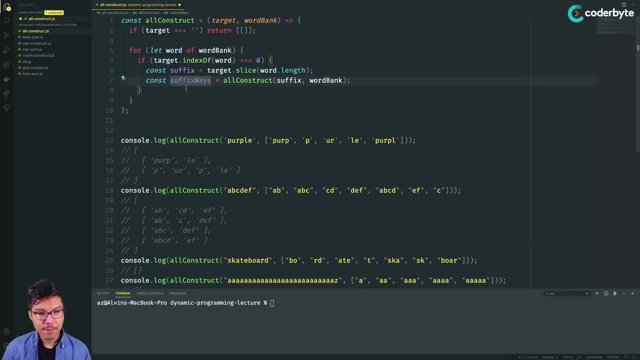 if there are many ways to do it, Nice. So if this gives me all the ways to make the suffix, how can I get all the ways to make the original target, like in this current stack frame? Well, what I need to do is really just take each of those suffix ways and add my word to the front. 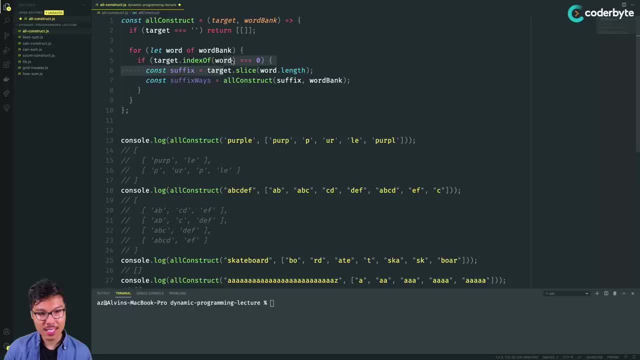 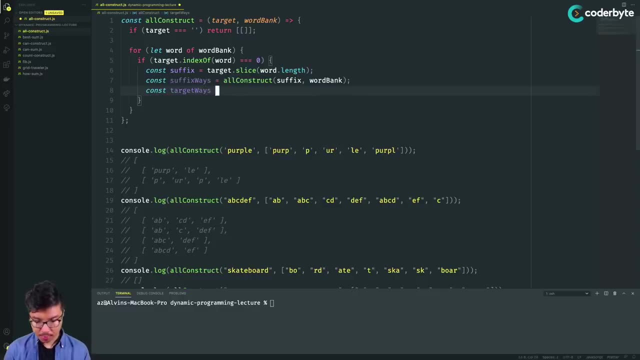 of it right. I used this word to even create the suffix in the first place. So what I can do is I'm going to say my target ways. So now I want to relate how the suffix ways can be used to build my original target right. All I need to do is really iterate over every sub array over here. 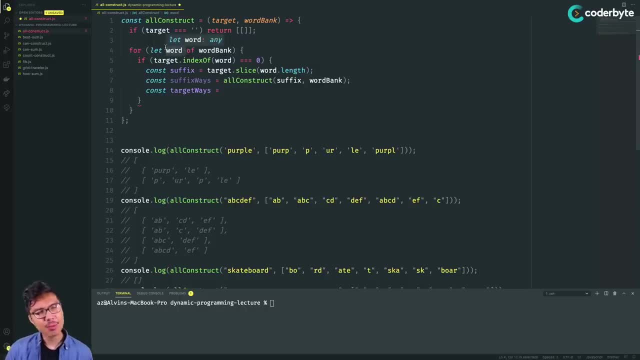 and add my word to the front of it. Right? That's exactly the process we took in the tree diagram, right? So I can use some nice JavaScript methods here. If I just want to basically manipulate every element of the array, I can do a map here. So 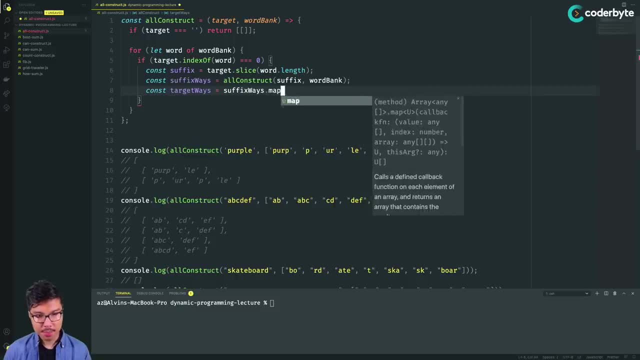 I'll say suffix ways, dot, map, And I know that a single element there is going to be one way. I'll say singular, And then what I want to do is just take that same way, copy it over meaning. I just spread out elements, But I'm also going to put the word that I took in the front. We've seen this syntax. 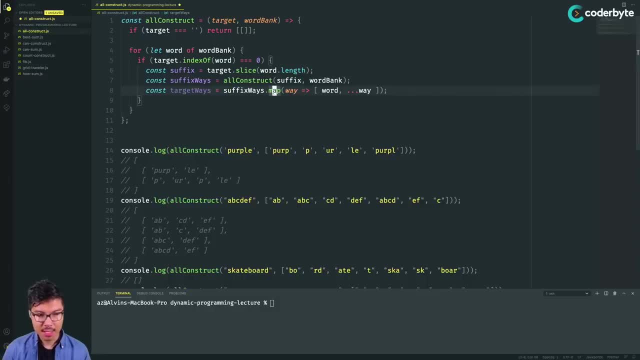 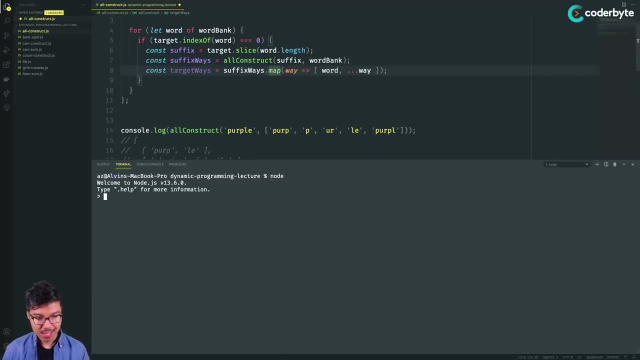 before. although maybe this like map method is maybe new for you, Maybe you're not super familiar with JavaScript. I think that's fair game. So let's hop into the node REPL Just to demo this. let's say I had some array. I'll just make this array 1234.. So there's my array, what I can. 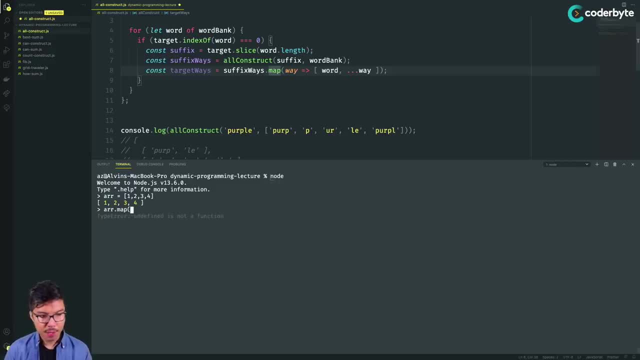 do in general is use array dot map, And map is a function you should pass in a callback. So that means another function, And what I'll do is this callback is going to take in every element And it's going to be an arrow function. what's going to return is really just how I want to modify. 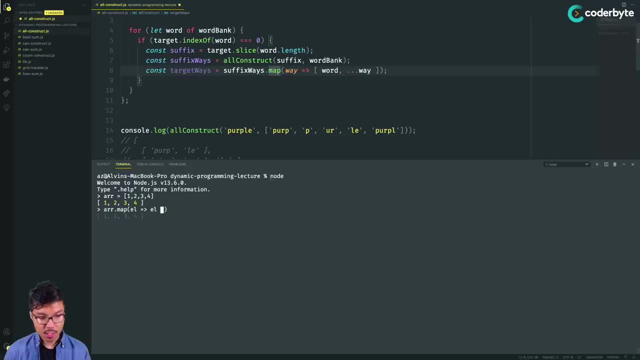 the elements. Let's say I wanted to multiply every element by two, right the return value you have. this callback function is going to become a new element of the new array. So notice, I get back to 468,. my original array was 1234.. And I get back a new array using map And so 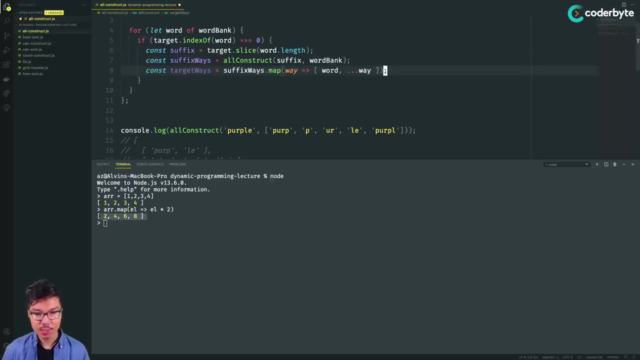 essentially what I'm doing in this example on line eight, my actual code- I'm just taking every sub array and just inserting my word at the front of every sub array. So an example that speaks closer to our exact code would make it look something like this: like suffix ways it's going. 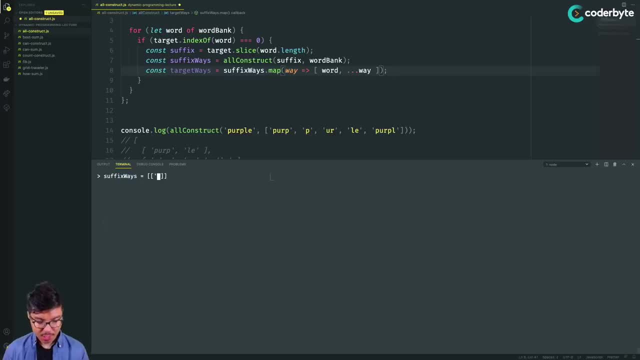 to be a 2d array. So I'll make a sub array, maybe just an array of some strings, kind of arbitrary right now. So I'll say x, y and then z, And then the second sub array will be maybe, I don't know. 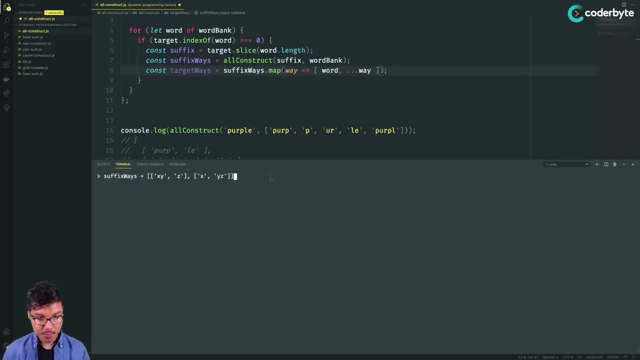 like a x and then a y, z, Right. So that's my original array, And what I want to do is, if I say suffix ways, dot map, now let's say for every way. that is every sub array I just want to copy over. 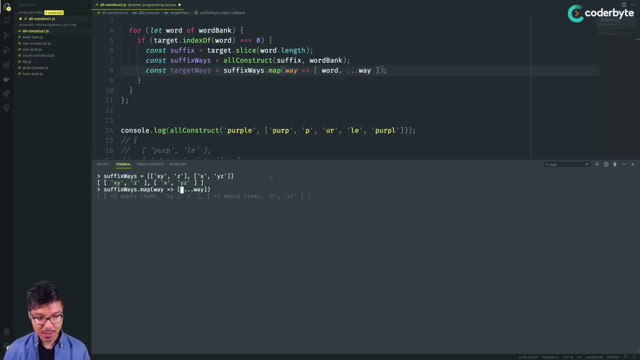 that way by spreading out, And then I'll just copy over that way by spreading out, And then I'll just go ahead and put I don't know like an A at the front, just like this. So notice what I get back. 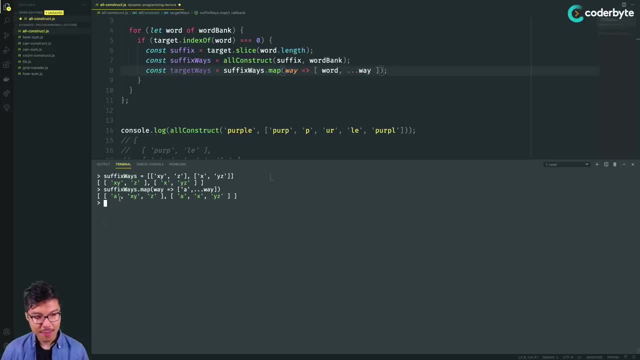 I basically have every sub array from before, except now I have a as the first element of both of those goals. That's all I'm doing in this particular chunk of code. Awesome, So we'll leave the node repl back to our running solution. And now that I have the target ways, that's good, It's. 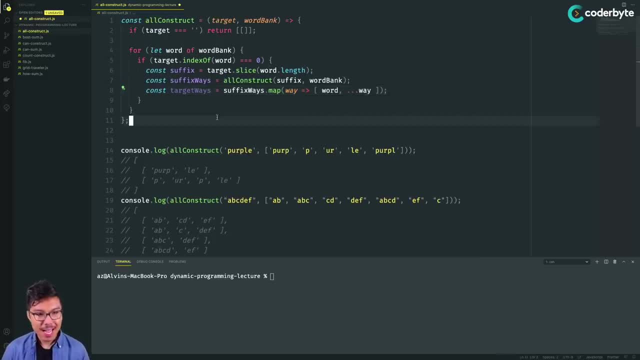 basically just like a piece of the answer I need. However, now this is really only going to give me all of the ways to make a target that use this word that I'm currently like on in my iteration. However, I know that this for loop gives me multiple branches. right, it's going to use all of the words that are. 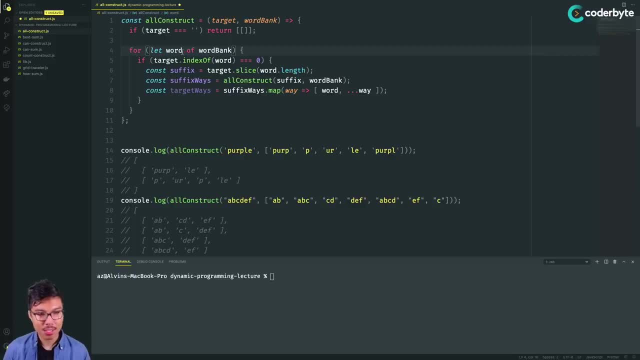 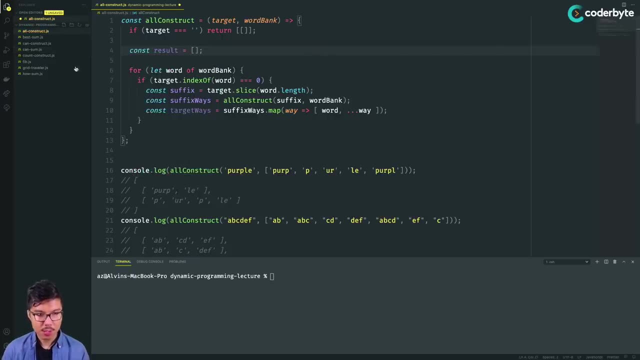 possible to create the target. So I need to kind of gather them all together. So I'll create a variable on the outside. I'll call it result. now store everything right. So across all of these iterations I just want to add the target ways into the results. I'm going to do: result dot push. 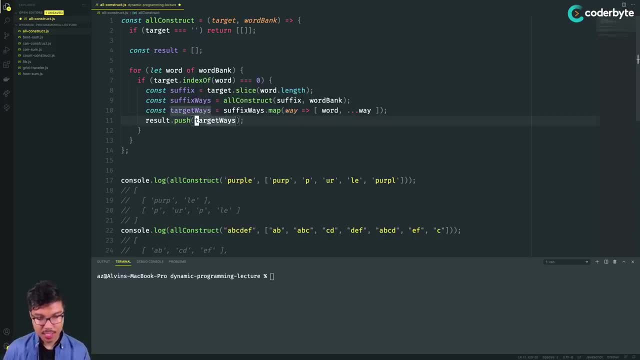 target ways and I need to actually spread this out. That way I don't nest things too deeply, right? Remember that this is a one dimensional array. Right now, target ways would be two dimensional. I don't want to just push target ways into result, Otherwise I get like a three. 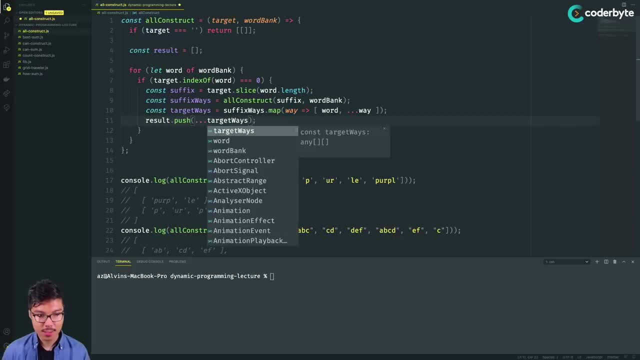 dimensional array. So I'm going to be sure to spread out target ways, right? So with that, let's actually go ahead and give this around. I think all I need to do now is after my for loop, right after I'm done getting all the ways. 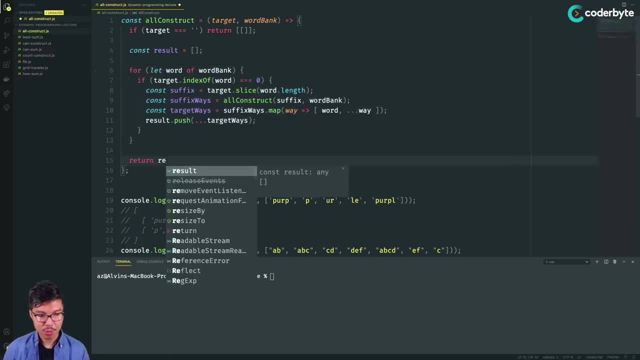 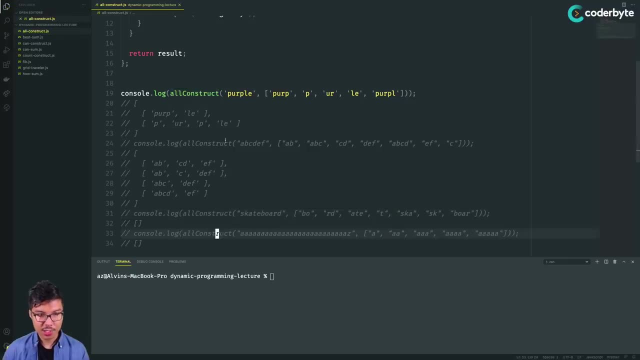 then I can just return the results And this should just work recursively. So let's just try maybe the first example for now and see how we do So. I should get you know a two dimensional array where I have two ways to make purple right. Let's give that a go, I'll. 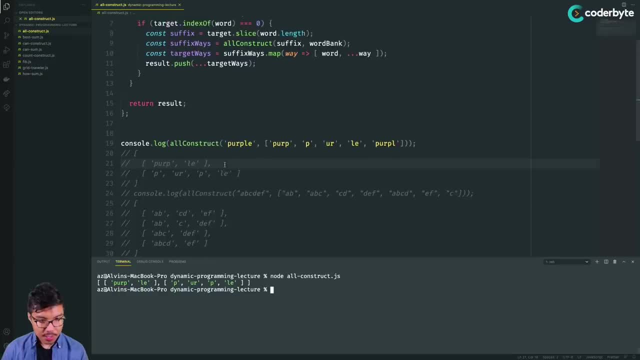 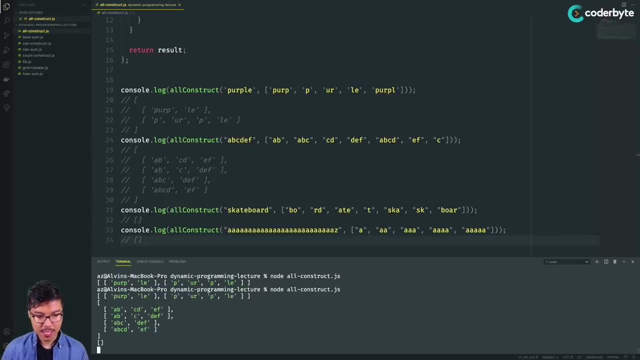 construct Nice And that's looking pretty good. That is a correct answer. Let's try these other ones now while we're here. So we should get a nice large array for that second example: Nice, Here it is, And then the 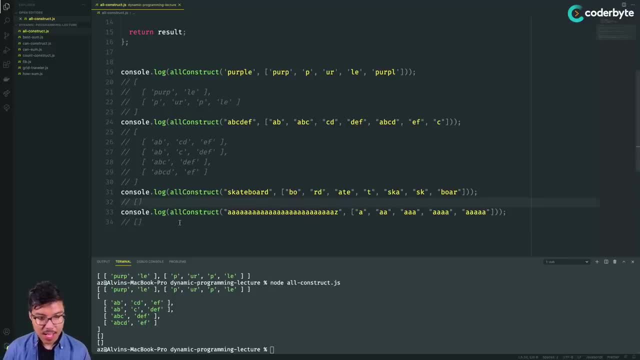 third example: skateboard should return just an empty array because it's not possible And it looks like that last example is also not possible. So we do get an empty array And, if you kind of notice, to get that last answer like we did in our other examples, it does noticeably take. 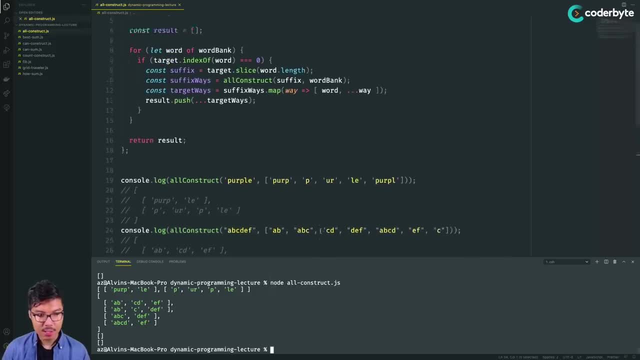 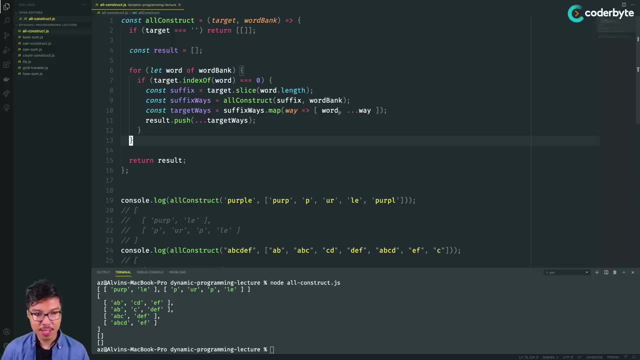 some amounts of time. But before we get to that, let's take a look at this code and make sure we really understand it. So the biggest logical leap we made here was really, you know, assuming that we get back valid data from line nine, right. And then it's all about how we can. 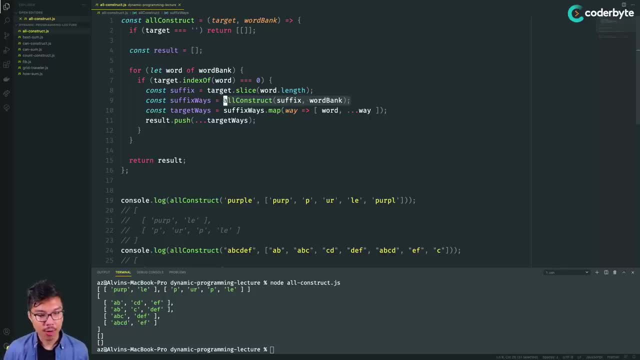 you know, adjust that sub result to get our full answer right. So if I get all the ways to make the suffix, then for each of those ways I can just add my word in front of them, And that would give me all the ways to make my target right. And then I need to continue that process for every choice. 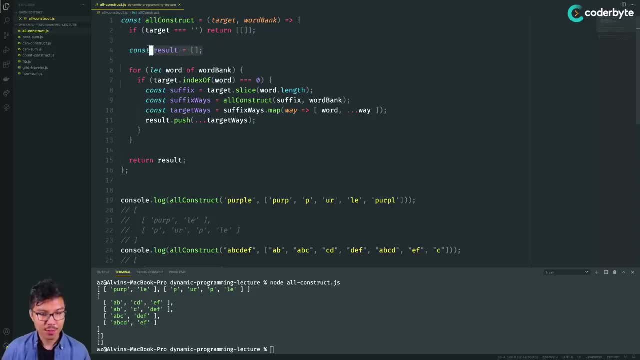 of word, which is why I'm maintaining this like a massive results variable outside of the for loop, just pushing all the ways into this result over time, maybe just to be super clear. you're not familiar with, like this push method, especially when you're using this push method. 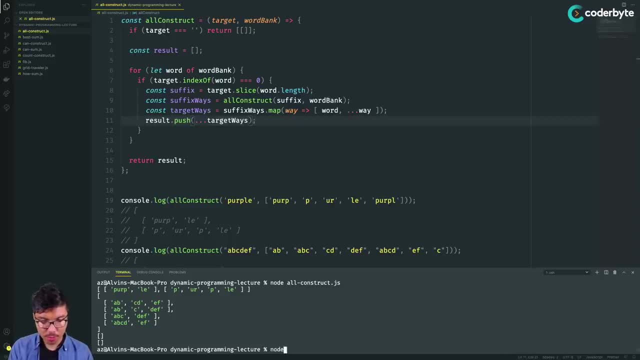 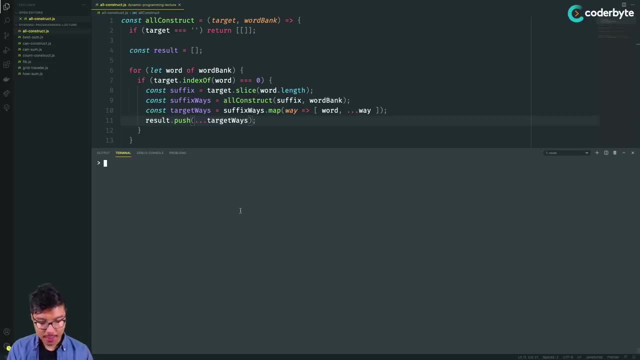 especially when you use the spread operator with it as well, can really easily step through that. So in isolation- right, this is just using push and spread in general, if I had some, let's say, array, And let's say it was just an array of just some elements- 1234.. 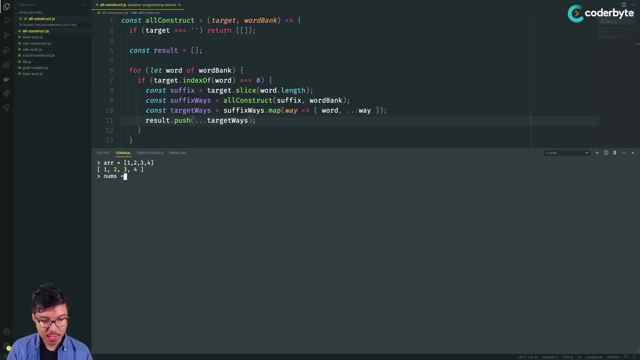 Then I had another array. I'll call it just nums. Let's say, in nums I had elements of seven and eight. So here's my original array And here's my nums. And if I did array dot, push nums, you're actually going to force some nesting in this array. So 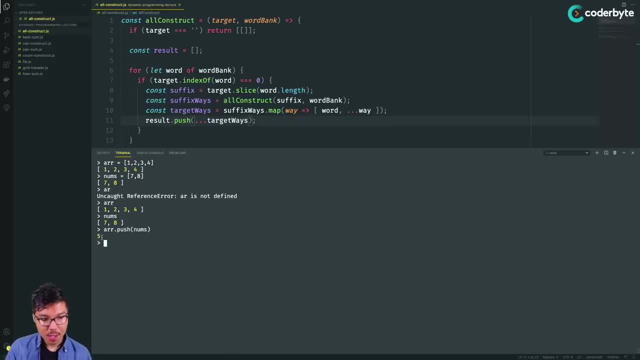 array dot push returns of a new length, But it also actually manipulates or mutates the argument you call it on. So if I look at the array now, notice that it actually has another array nested inside. That's because I literally just push the entire nums. If you wanted to do something a. 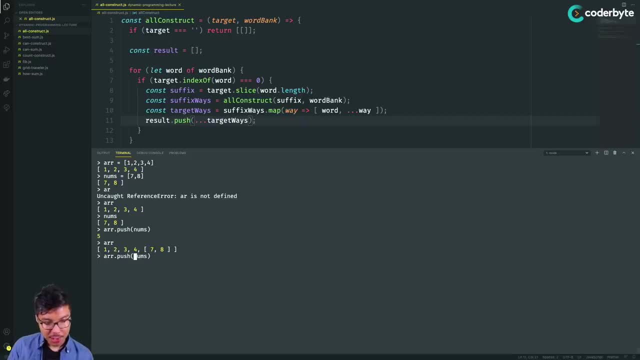 little different. what you can say is array, dot, push and you spread out nums. what's going to do is comma separate of the seven and eight, basically removing the outer brackets from it. So if you look at this now, like at the array, notice that with that second push now I just 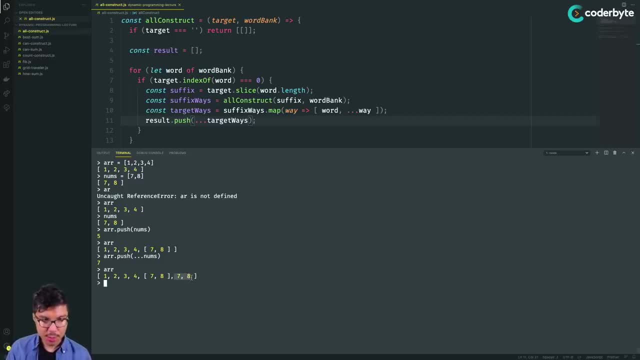 added a seven and eight without those additional brackets. So that's all I'm doing over here. Like I said, I don't want to add another level of nesting to the result array. right, it should just always remain, at most, a two dimensional array. Cool, But overall it looks like we have solved. this one And let's kind of talk about if there is even a way to do this. let's say, let's say, let's call this an array of nesting. Now let's say: nesting is this one, So I've got to do another Mask, So this: 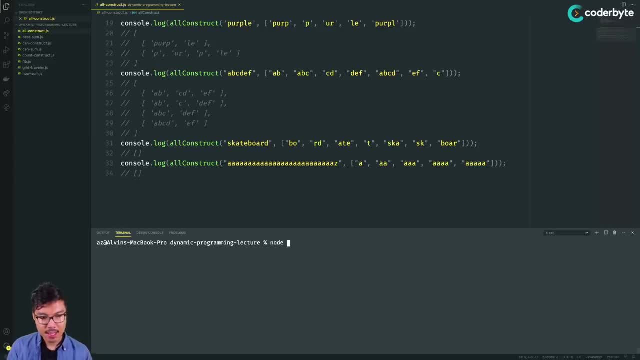 will be the Nesting method. So the Nesting method is going to do an array of nesting right. So I'll use the Nesting method and kind of talk about if there is even a way to make this faster. this is kind of an interesting 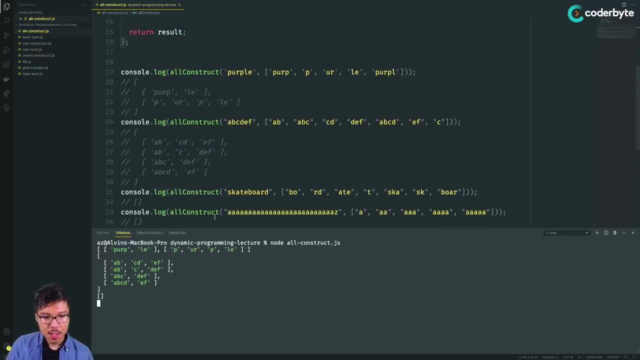 problem, So this is looking pretty good. So earlier, when we were on the drawing board, we said that, alright, because of what they're asking in this problem, it is basically going to require a full exploration, right? If I want you to return every possible way to make. 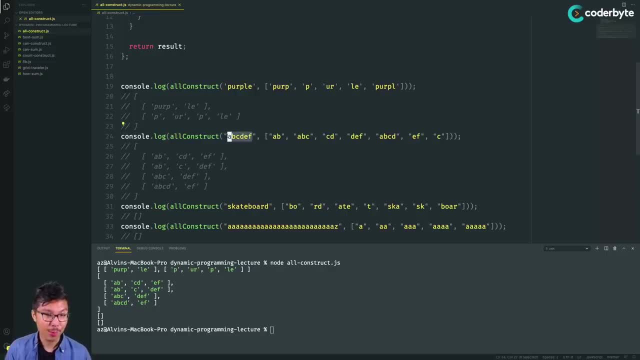 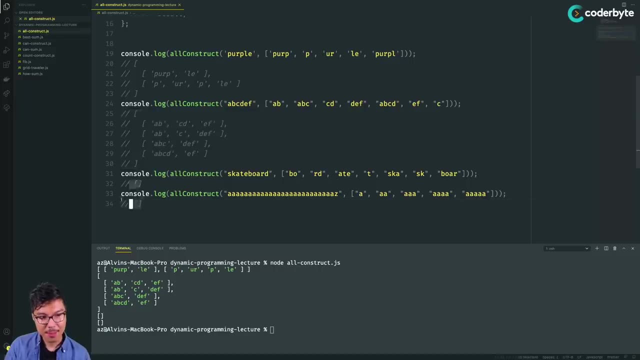 the target string, you'll just have to kind of do all the work of creating all of those sub arrays, right. So we can't really avoid that stuff over here. If you think about this example on like 3334,, this is actually not the worst, worst case anymore, Right here. 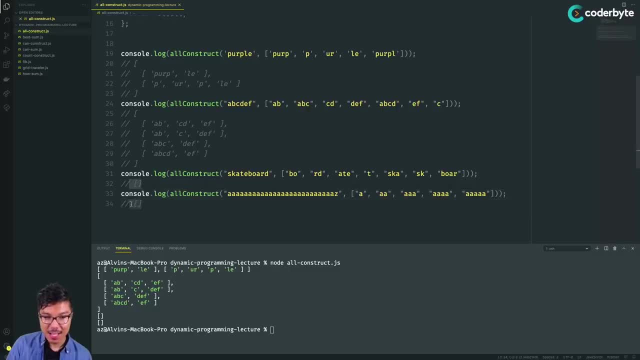 we know that eventually we're going to return just an empty array, because we can never generate the final z in this example, However, if I remove the Z, then the result will be a very, very massive 2d array, because there are bunch of ways to actually make this target. 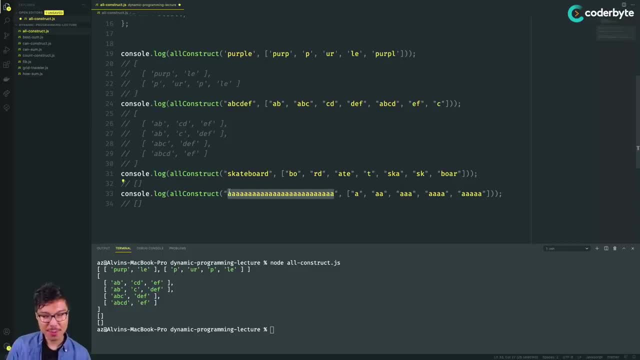 string Right. So we've kind of changed the direction of what it means to be like worst. on this example, let's say we brought this to use the Z. If you really cared about optimizing, like this particular scenario, you would find some benefit to like memoizing it, although. 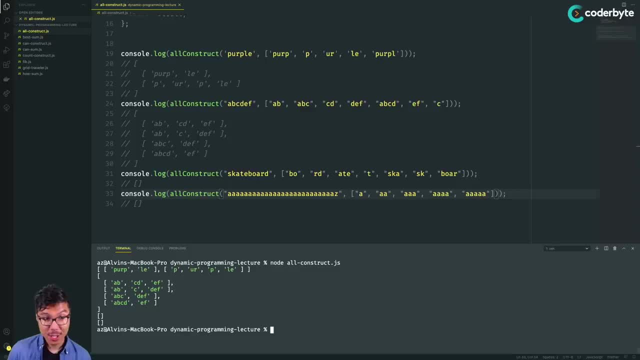 it wouldn't really affect the worst case, because the worst case is actually where you return a two dimensional array and not just an empty array. So maybe just because it's good practice will memoize this, But when we go to the drawing board we'll see that. 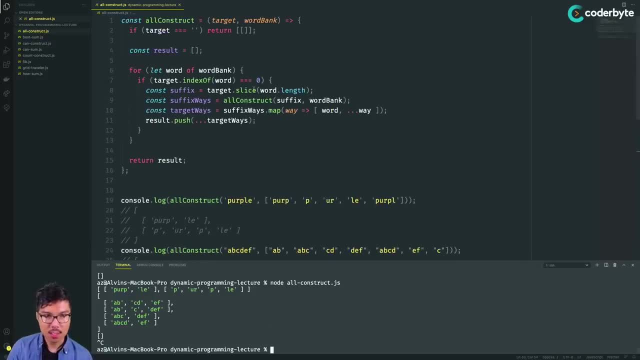 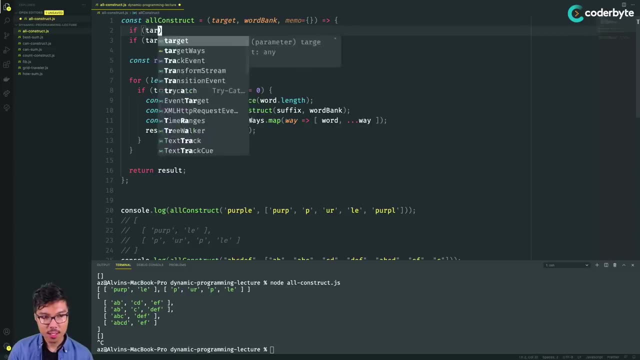 this actually doesn't really matter. We're going to go to the drawing board and we'll see that this actually doesn't affect the true, a bigger, worst case. But if you just want to optimize it slightly, let's say we baked in our memo over here. then we check, you know if our target is in the memo. 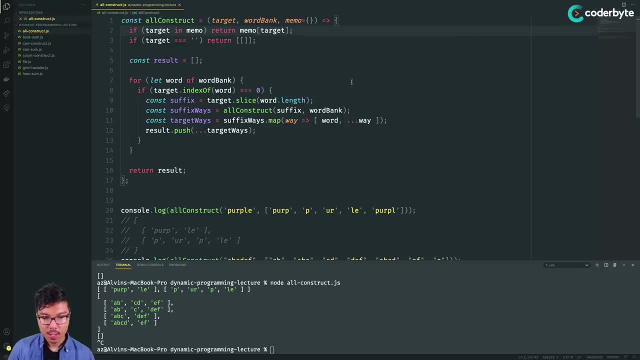 and if it is, then we return the memo at the target. we'll be sure to pass along that memo to our recursive calls, And then we just need to make sure that for our return value on line 16, we actually store that inside of our memo, using the target as a key, and then 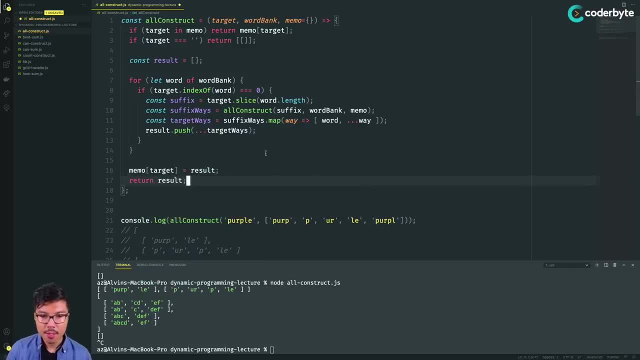 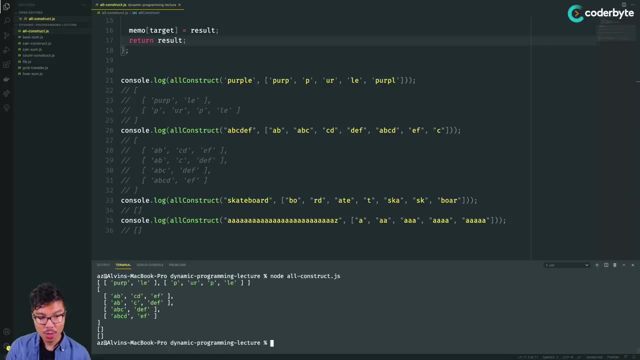 we still complete the return by returning result, like we once did. Cool, So let's run this now, And I would agree that the last example now runs faster, but it is not the worst case- is a really important thing to understand here. right? The worst case is when you actually have to create a massive 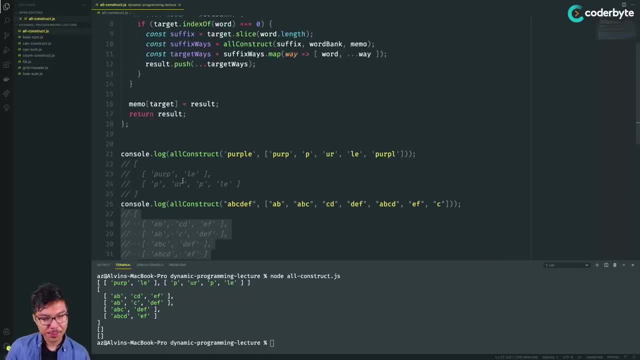 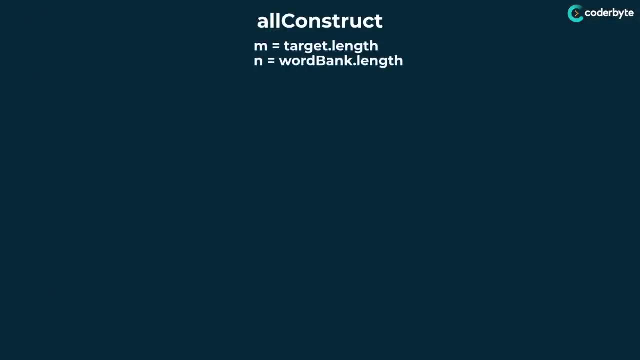 sub array right, And so let's head to the drawing board and see our final conclusion about the complexity here. Like we usually do, we'll define m to be the length of the target string, And then we'll see the number of words in the word bank. we know that this problem asks. 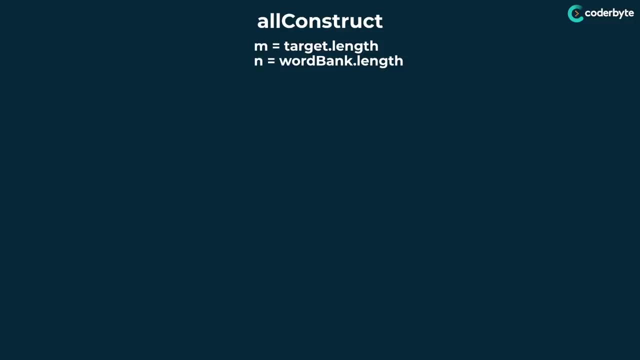 us to return an array containing every combination that generates the target string And to come up with that answer, we have to visualize it like a tree, sort of like this: In our previous drawing we saw how each leaf of this tree represents one way we could create the target. 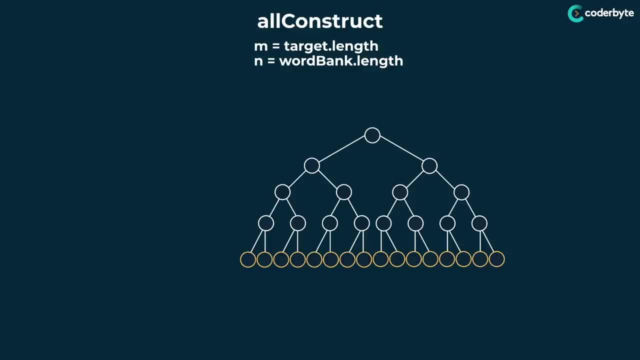 string. In other words, if we can figure out the total number of leaves in a tree like this, then we would basically have the number that represents how many different ways or how many sub arrays we have to generate In this problem. we already know that, based on our process. we described that there are 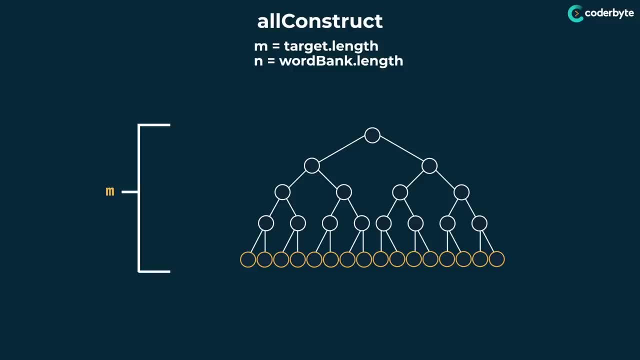 dimensions to this tree. we know that the height of this tree is going to be m And we know that from one level to the next, we really just multiply the number of nodes by n, And that means at the base of this tree, we would have n to the m number of nodes. 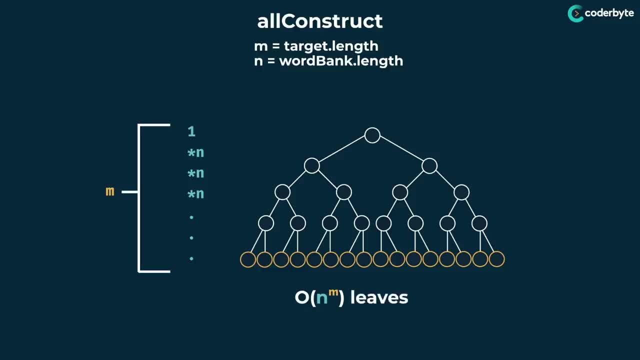 right. So we have n to the m leaves, which means that we have n to the m different combinations that generate the target string. And if we have to represent each of these n to the m, n to the m combinations, then we definitely need n to the m sub arrays in our output. And 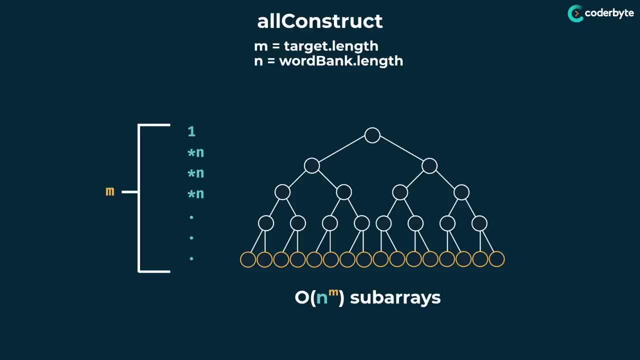 so what we're saying here is: no matter what clever implementation we create, we really have to return a result that is exponential in size, And that's really going to drive the complexity of this one. you can't do any better than exponential over here, And so 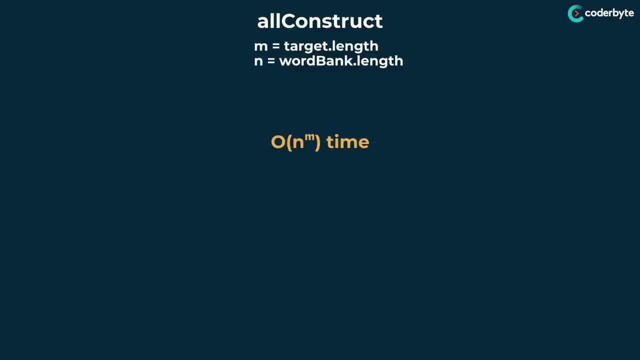 overall, we'll say that the time complexity of this is n to the m or just exponential. If you wanted to split hairs here, you can really multiply by some additional factors of m And that alone really gives us the overall complexity right. Because once something 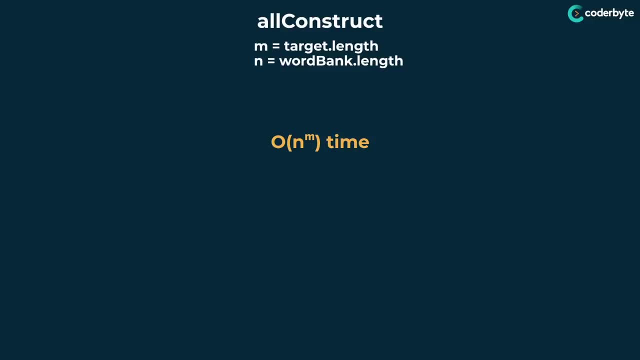 is exponential. there's really no coming back from that. And in a different vein, we can say that this space, complexity for this is O of M, like we usually say. it's really just the height of the recursion tree. In an example like this, where output is very large, we 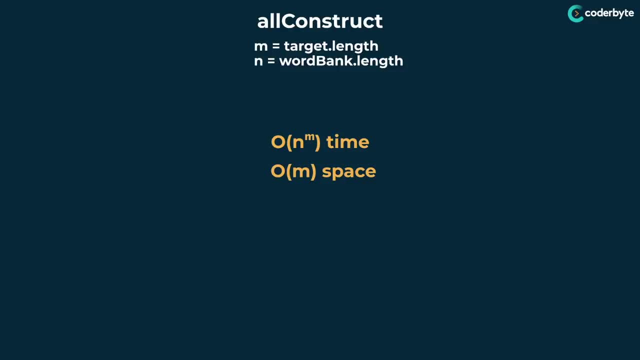 usually don't include the size of the output or the size of the result into our space complexity, which case obviously would also be exponential in space because the result is exponential right? So we'll just refer to the additional space we use for the call stack, which would be: 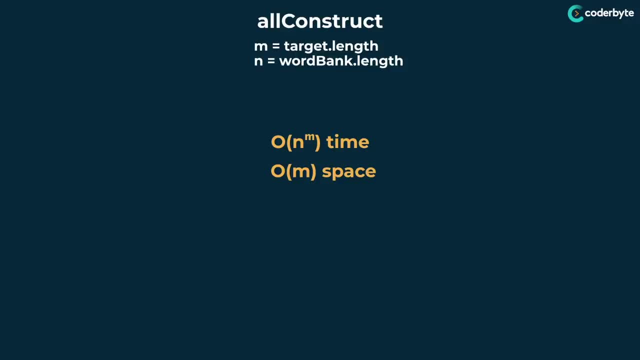 O of M right, any solution you come up with for this problem would be just about this: fast, All right, and there we have our all construct problem. So at this point we've gone over many dynamic programming problems And we use that memo ization strategy to work. 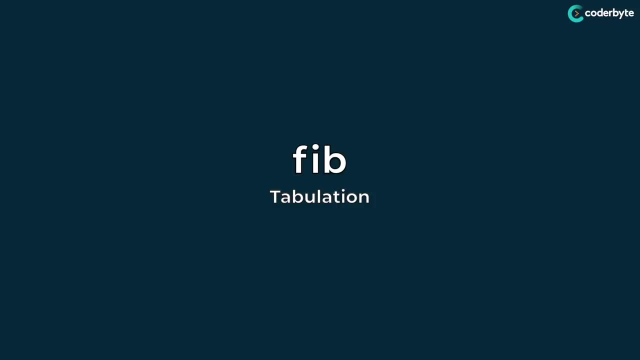 out a solution for all of them. However, memo ization is only one of the ways we can actually implement a dynamic programming solution. Right now, I want to revisit all of those problems, but this time use a different lens of understanding. As always, I want us to. 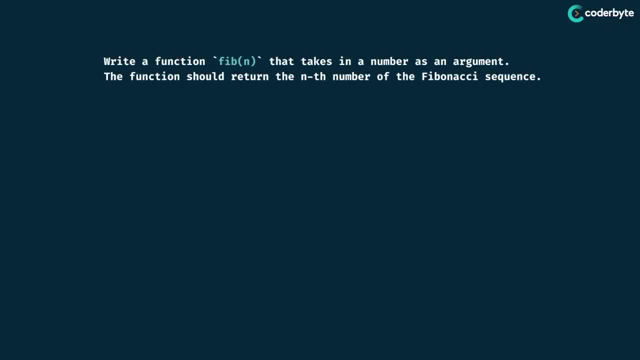 ease into things, So we'll warm up with this fib function. This is the same problem as last time. In other words, I want us to return the nth number of the Fibonacci sequence. Here I'll say that the zeroth number of the sequence is zero and the first number of 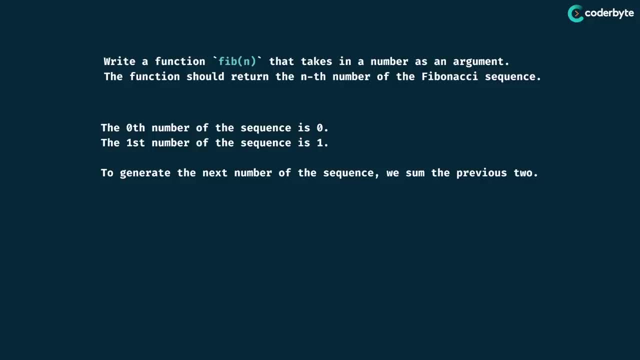 the sequence is one. you might notice that this time around I'm saying that the zeroth number is zero and the first number is one, Whereas in the first time we did this, we said the first number is one and the second number is one. However, no matter how you, 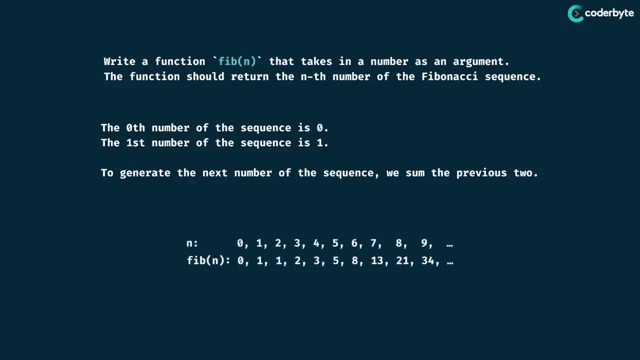 start the sequence, they will both actually give you the same series of numbers, So we're going to go ahead and do that. In other words, down below here I have some examples for n, as well as what the output for our fib function should be. In other words, if I asked you, 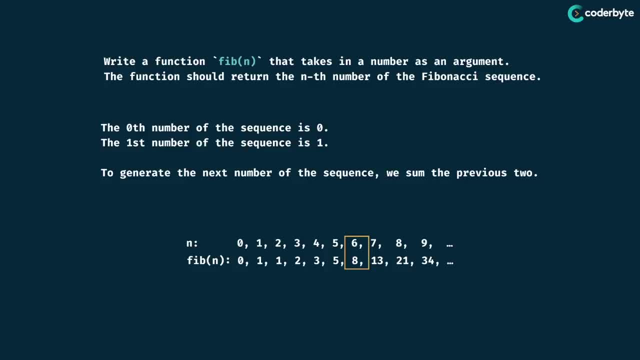 for the six Fibonacci number, the answer there is eight, like we always expect. Alright, let's get into the heart of this strategy, right? What does tabulation even mean? Well, it's all about building a table. So what we'll do now is step through a tabulated strategy. 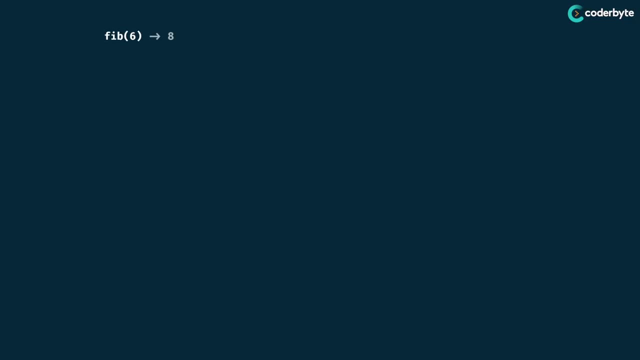 for calculating fib of six. I know that in the long run I have to return the final answer of eight right, So I hope that I get the answer of eight by the end of this little trace With tabulation. we're choosing to do is really think about this dynamic programming problem. 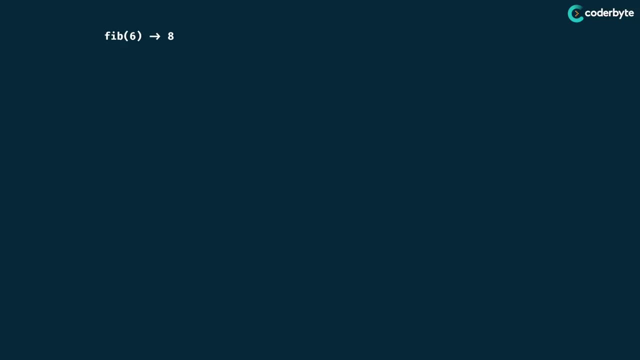 still in terms of sub problems. But instead of doing it recursively, we do it iteratively by building a table, really just an array, And I'm going to begin it with roughly the size of the input. In other words, if my input here is the number six, then I basically want: 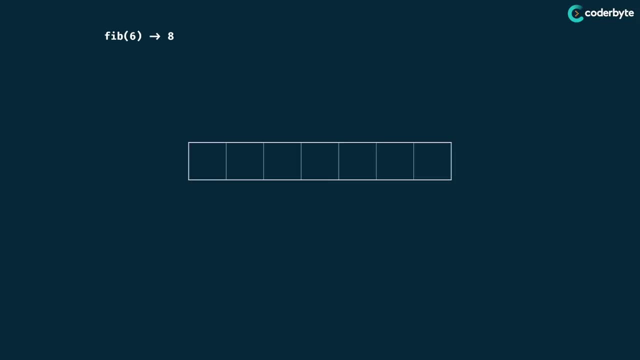 an array of length six. Notice that if I want the indices of this array to kind of line up perfectly with the original input number, I'm going to have to actually add an extra position. And this array spans indices zero through six, which kind of means that there actually 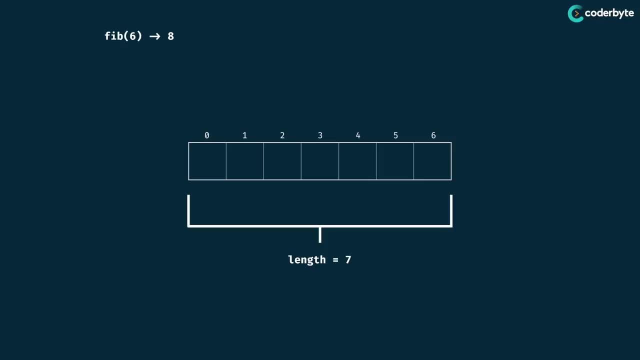 are seven different elements here. right, the length of this array is seven. So something very common that I see when students tried to implement a tabulated strategies, they kind of overlook this off by one nature, right? So technically I'm creating an array that. 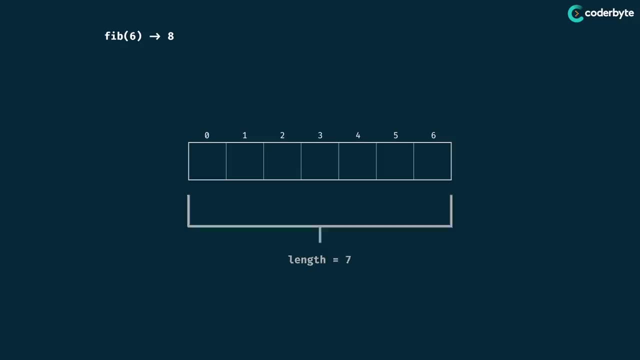 has one greater length than my number input. But any case, if this is my array, what do I want it to represent? Well, in the long run, I want to actually fill out this array in a way where each array is equal to one, In other words, each array belongs to a object. 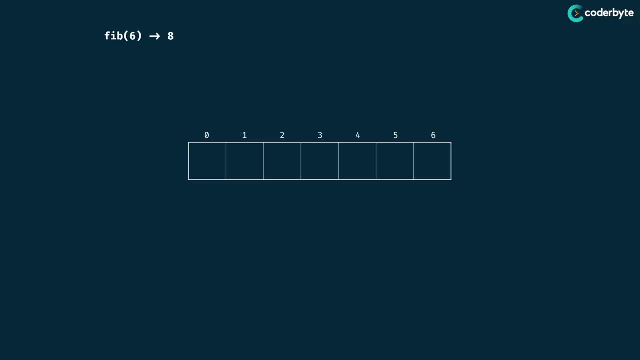 sub problem corresponds to an element of this array. So here's I'm going to begin this table. the move here is to actually initialize every position of this table with zero, And the reason for me initializing zero everywhere in this array is the fact that I know Fibonacci requires me to. 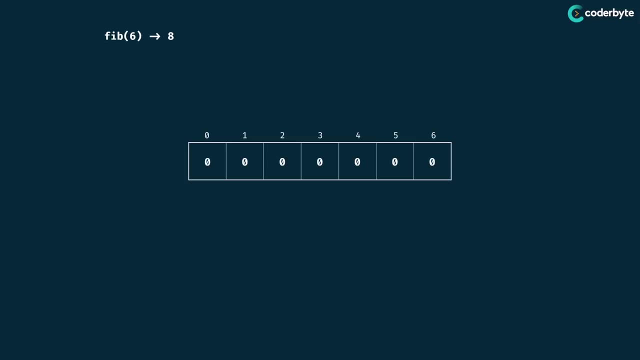 take a sum right, and zero is a really great starting value when I need to calculate a running sum right. But along with that, I need to be sure to seed the starting values within this table. In other words, if I look at the zero position of this table, it already has a zero, which makes 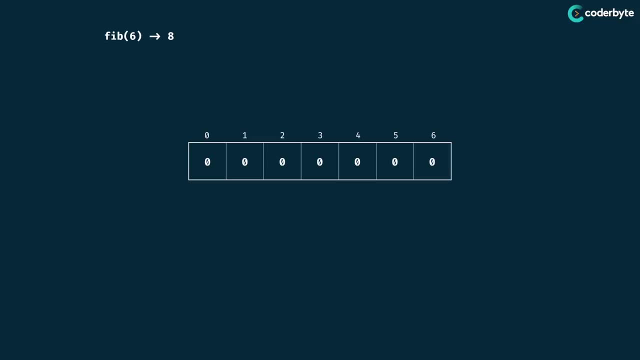 sense, because the zero number of the Fibonacci sequence is zero. But what I should also do is make index one contain a value of one, And that kind of entails that, hey, the first Fibonacci number is indeed one. And now, at this point, once I've seeded those initial values, now I can 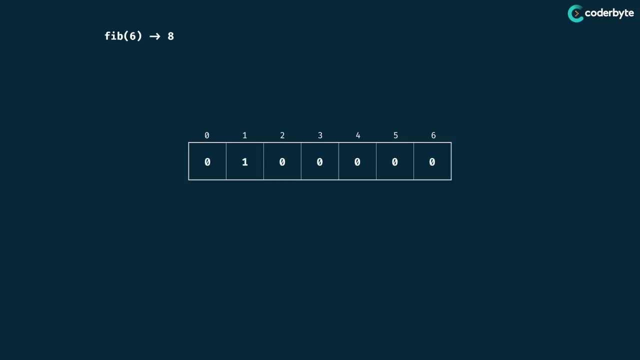 actually run the general algorithm to fill out this table. So now it's just a matter of iterating through this table. So I'm going to start, you know, at the very first position of the table, probably just with a regular for loop, And what I need to do is 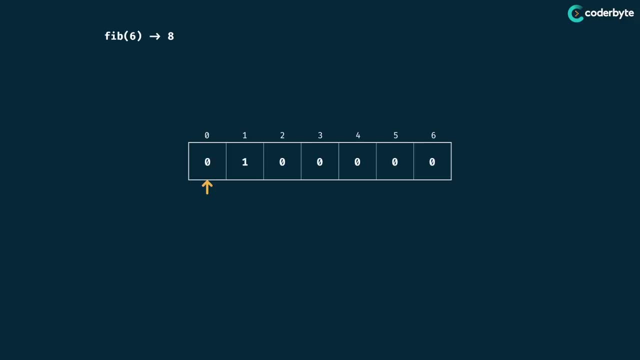 really remember the definition of Fibonacci right. So if I have this number currently in the array zero, that's a zero Fibonacci number. what I can do is just add this current number that I have kind of pointed to in yellow to the next two positions And the reasoning: there is a Fibonacci. 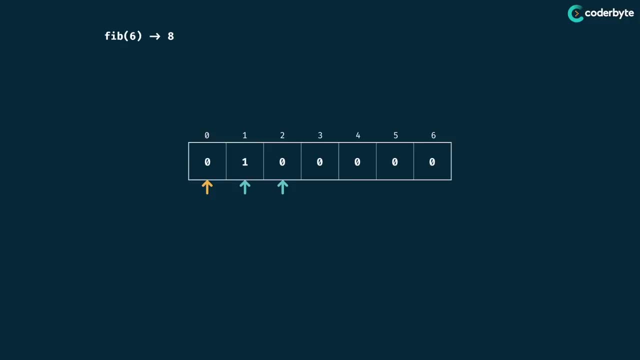 number is used to contribute to the sum of for the next two Fibonacci numbers. So I'm going to do is take the zero and add it to the next two positions. Obviously, since it's zero, I actually don't change the values of those next two positions, So nothing really is going to change. 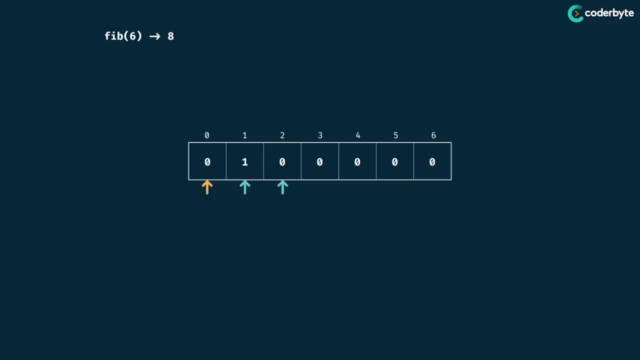 It's just calculated on that first iteration, But any case, I can continue on to the next iteration. So my current position is always in yellow And the next two positions are pointed to in blue. At this point, my current position says one, so what I should do is take one. 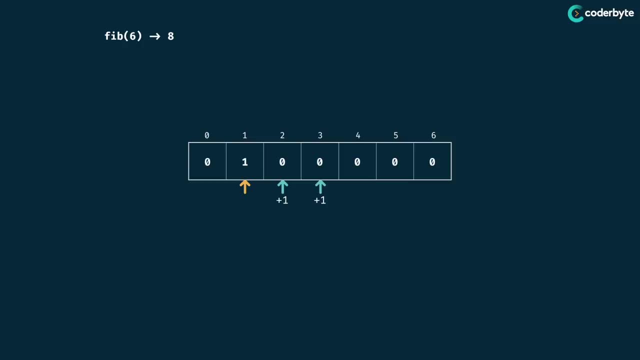 and add it to both of my next positions. So that means two and three, or indices two and three contain both a one and a one, which so far makes some sense because, at least for the two, the second number of the Fibonacci sequence is indeed one. I can do the 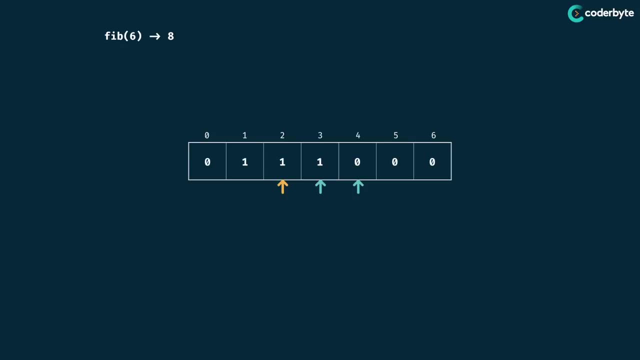 same thing. right, My current position contains a one, So I'll add that one into my next two positions. Keep doing this. I add two to my next two positions, add three to my next two positions, And at this point I sort of reach the end of my array. So I know that I probably shouldn't. 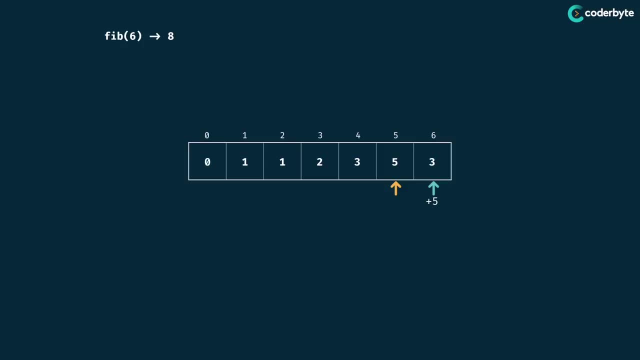 step out of bounds. So really just want to look one position ahead over here, And at this point I just add five into my next position, which actually works out to an eight being stored in index six of this array which is sort of a common use case, And at this point we just want: 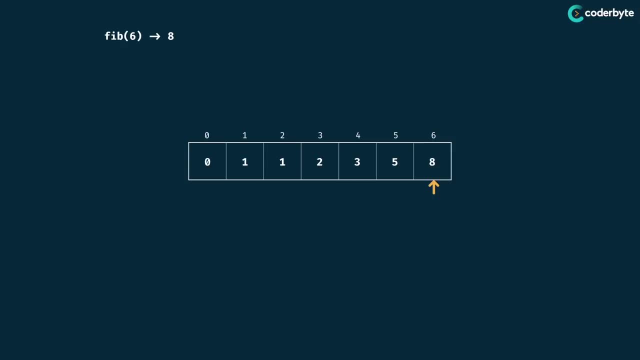 makes sense because, logically, the sixth number of the Fibonacci sequence is a. just like we intended. That's all. there is a tabulating Fibonacci. the most apparent difference from our previous like recursive strategy was: this is not recursive right? This, really. 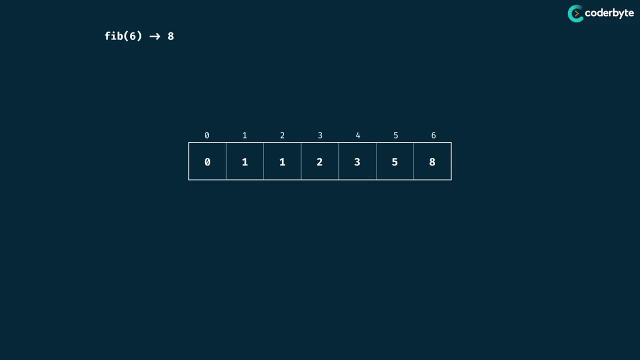 just requires us to iterate through an array. So it's a fully iterative process And at this point the actual complexity of this is really straightforward to kind of foresee. we know that we're just going to iterate through an array of size n. that must mean that our 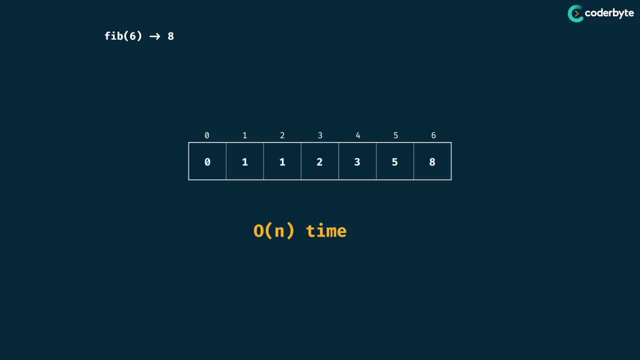 time, complexity is just n. In the same way, the only space we use is really just the space of the array, which I know is still going to be size n as well. So overall, we're looking at a linear solution for fib. So before we hop into the code for this one, I just want 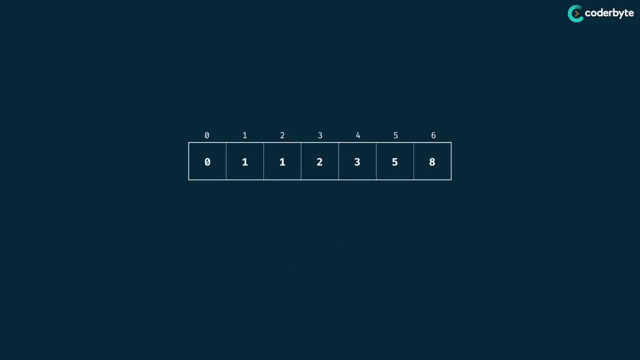 to draw a really important connection. So although at face value this iterative strategy looks very different from the recursive solution, a lot of the logic really carries over. I'm still using my overlapping sub problems to solve this one. So, for example, I know that 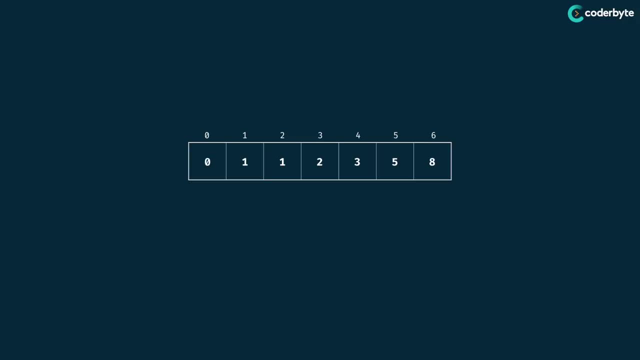 every index of this array really corresponds to some number. input for fib of n, right? so I can kind of visualize it like this, right? like we said, the six Fibonacci number is eight, So I'm just going to choose a position of this table. let's say I looked at fib of 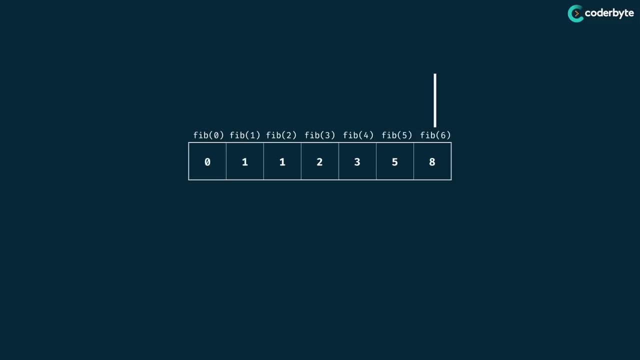 six. So I know that to calculate fib of six what I did was really add the previous two numbers into this position, right? And if you kind of see that the shape of this, if I kind of drop the table and even just ignore the rest of the 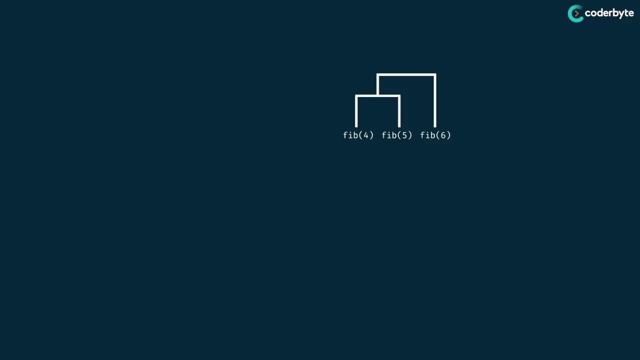 sub problems. this is basically just a tree, right? I can kind of shift things around And it really looks like this. So overall, you're looking at really the same relationship of for calculating Fibonacci. it's just encoded in a table instead of the recursive tree. 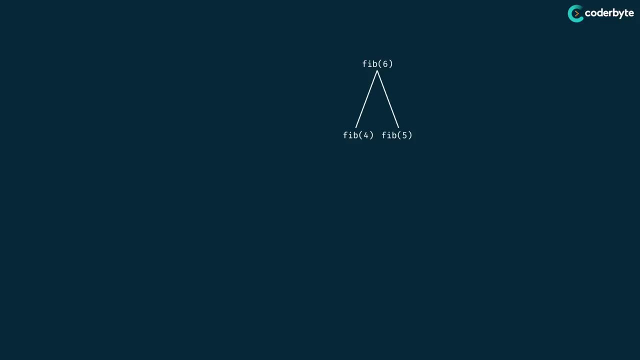 But overall, if you understand, you know the recursive solution, you should still find, you know, some comfort inside of this iterative solution. But I think at this point let's hop into the code for this one. Alright, programmers, let's go ahead and translate that strategy. 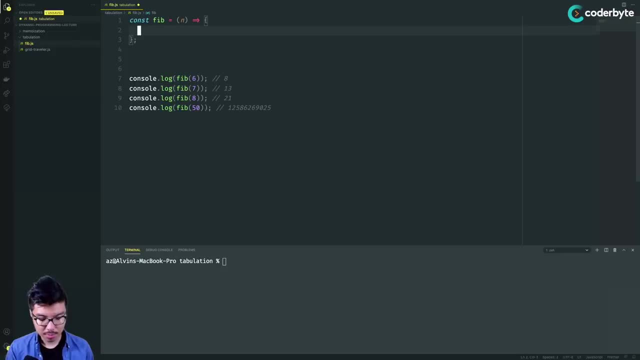 into some code. All right, let's go ahead and translate that strategy into some code. All right, programmers, let's go ahead and translate that strategy into some code. All right, code. So I'll start by creating a table, which really just means creating an array. So I'll 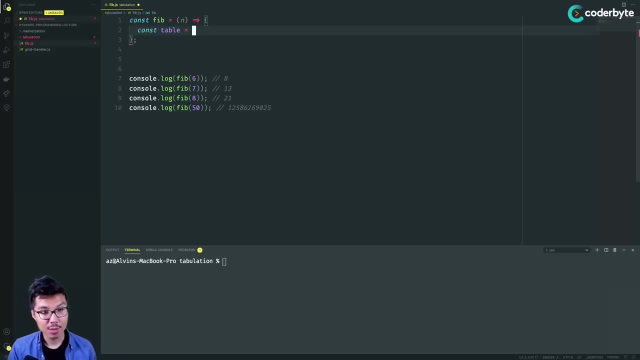 call this table And I need this array to have certain dimensions that are roughly the size of n. So to do that in JavaScript I can say array and call a static method and pass in my desired size. So here I want to say n plus one, But for the reason we did, 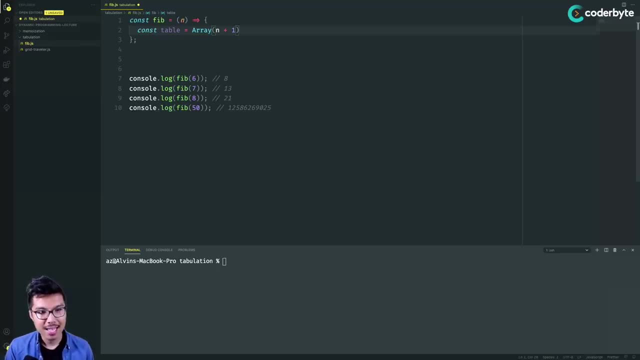 in the sketch, right, I need to make sure that the last index of this array is exactly n. I have to do the plus one here, because of course indices start at zero. Cool, that should give me an array of that n plus one size, And then, at this point, what I want. 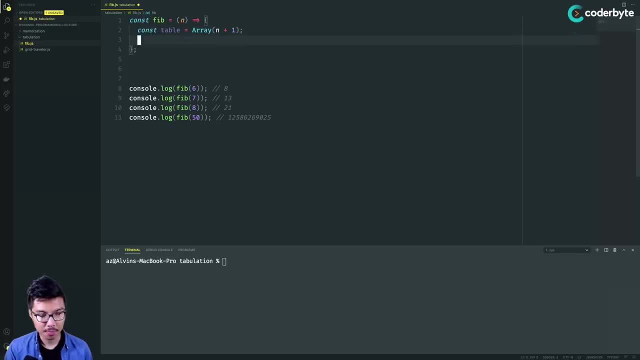 to do is assign particular values into this table. So let's just say I console dot log what this table looks like And I'll just run this first example of fib of six. So I'll give this a go. So notice that the array that prints out is this: it says like seven empty. 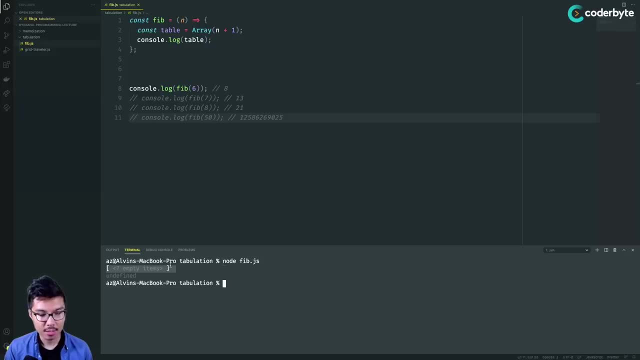 items, which means that the elements are undefined right now. According to our strategy, what we should do is assign these all to zero. So what I can do is, after I initialize the array over here, I can fill it up with all zeros using the dot fill method. right, it's an array instance method, So with 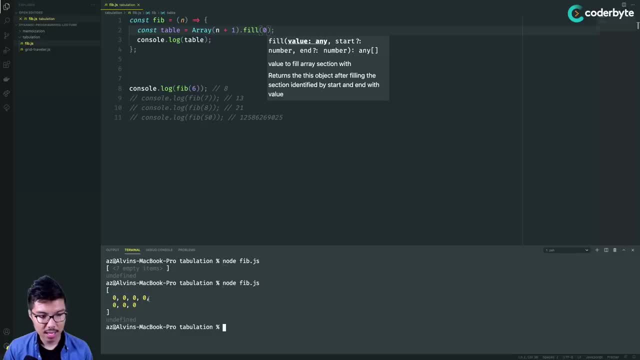 that change. now I should have a seven zeros inside of this array- Cool, So that's looking pretty good. At this point I also need to fill up a particular value inside of the table. I really need to make sure that the index one contains a value of one right, so I can say: table at index one equals one. 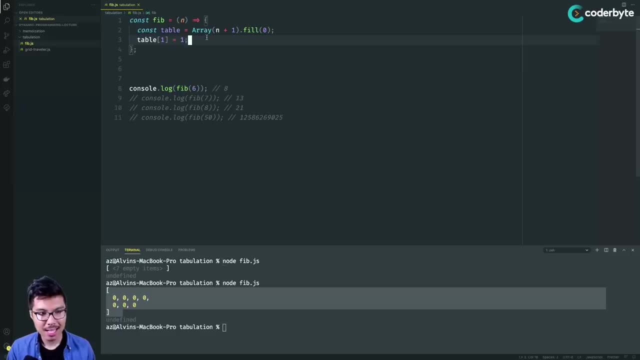 So we're seeding index one with a value of one to symbolize that the first Fibonacci number is one. remember that we kind of have like two base scenarios in Fibonacci. Let's just console dot log with this table looks like now to make sure it's in the correct. 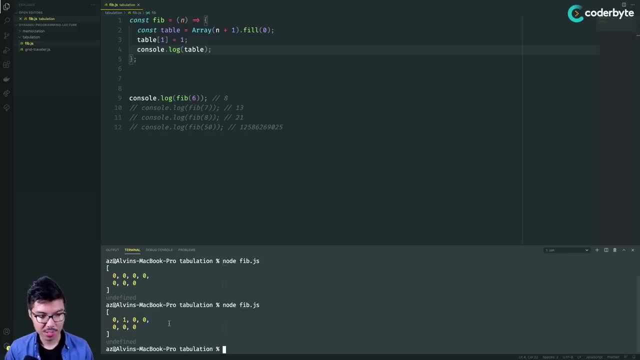 state before we actually iterate through it. Cool, So this is a good starting point for our table. So at this point what I want to do is iterate through the table. So use a regular for loop. for that I'm gonna need access to the indices. So I'll say: let i equals zero And I'll go up to and. 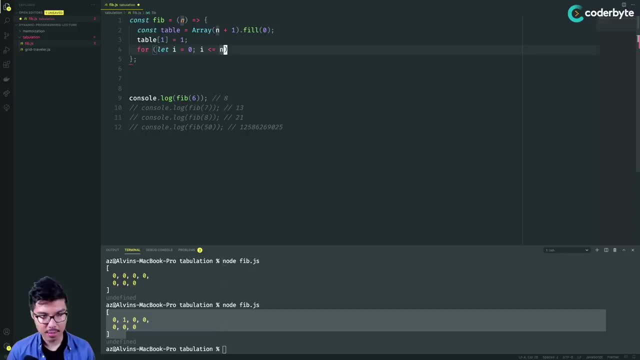 including n, which basically give me iterations through the entire table. And I'll do. i plus plus, I'm going to hit every position. Cool, According to what we did in our strategy, what I should do is look at the next two positions after I right. So I'll say: is I'm going to? 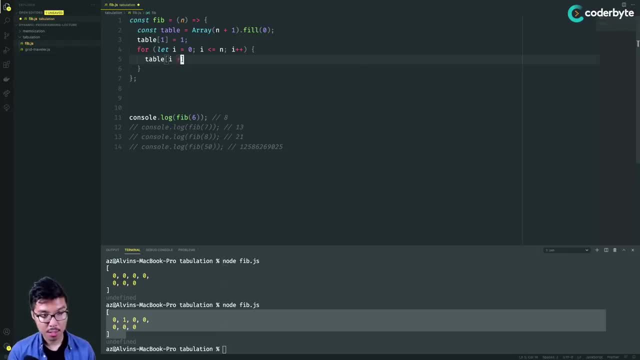 look ahead in the table And I'll look at positions I plus one and also I plus two, Right Of course. right now I'm currently situated at position i And what I did was I added into those two neighboring positions. I added my current value in the table, So 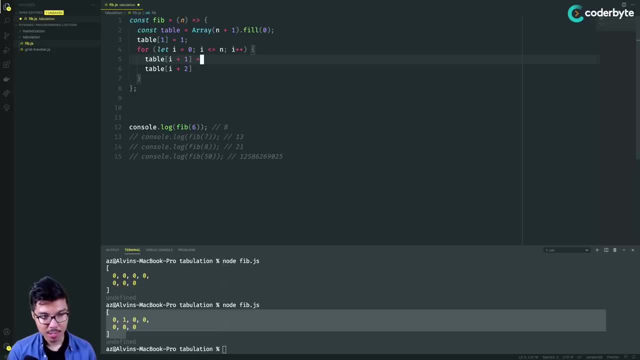 what I'll say is: in my next position, I plus one. I'm going to increment it by exactly what table I says: right? so I'm incrementing my next position by the value in my current position. the same will hold true for the next position two spaces away. All right, 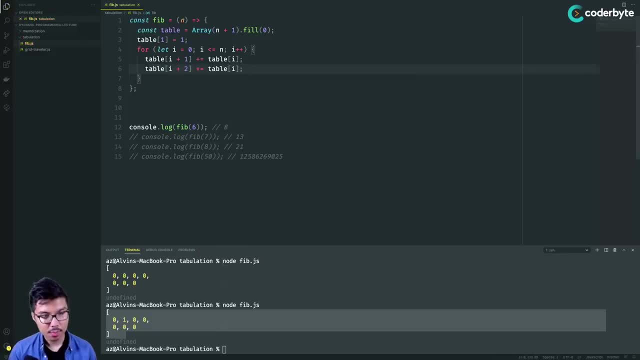 they both get plus equals table I- Nice, So this is looking pretty good. After we're done doing this process for the entire table, right? we're just going left to right filling in our next two neighboring positions. what we'll do is just return our answer, which should: 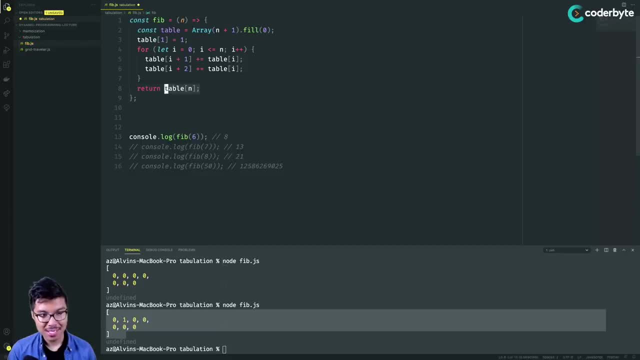 be table at position n right. To finish this off, I just want to return the table at index n, because the elements of this array correspond to the Fibonacci number right And the index is sort of the input to my function. So let's try these examples. We'll give them all a. 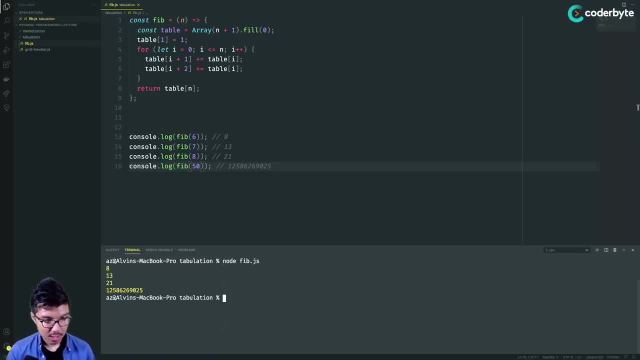 go Cool. So I get 813, 21 in this very large number, And this actually looks correct, Nice. So this is a fair implementation of Fibonacci. Notice that because we're already using an iterative strategy, we already satisfy a decent complexity for even this, this last example. 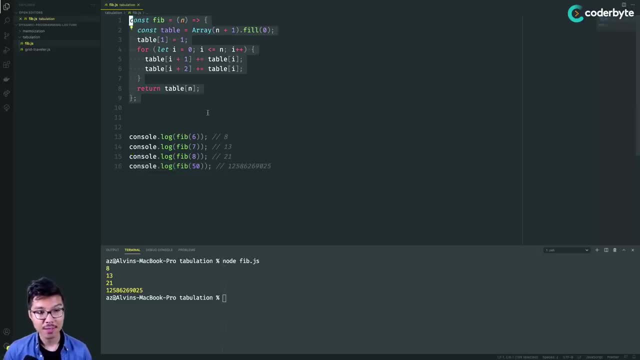 over here. we already mentioned the time and space complexity of this strategy. right, It gives us a linear time and space. However, you may already have in your head that we could actually optimize a little more here and just use a constant amount of space. However, 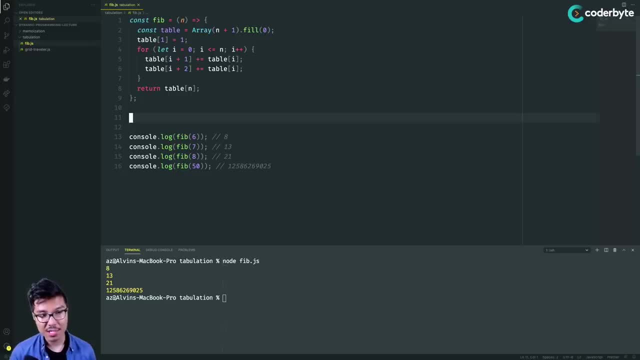 if you want to kind of subscribe to just a generic tabulation strategy that I know is going to be useful in most problems, I will kind of stick to this overarching pattern right of initializing our table upfront. that is roughly the size of the input and then 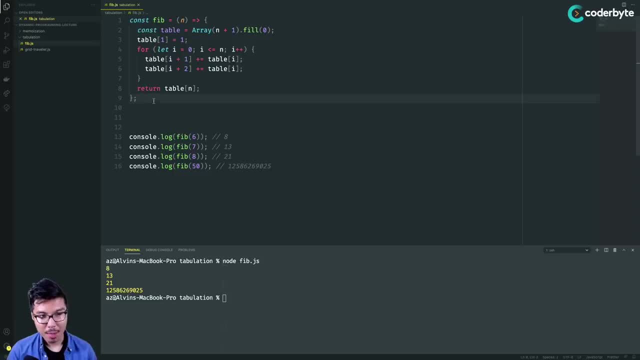 iterating through that table. Of course, you can probably finesse this fib function to only track two variables: represent your last Fibonacci number as well as your last last Fibonacci number. But I'll leave that to you because it's not really a classic tabulation which. 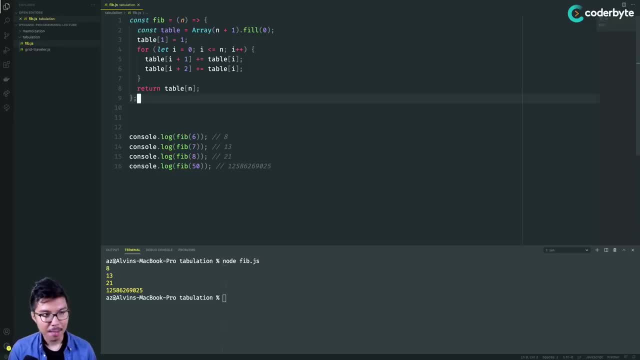 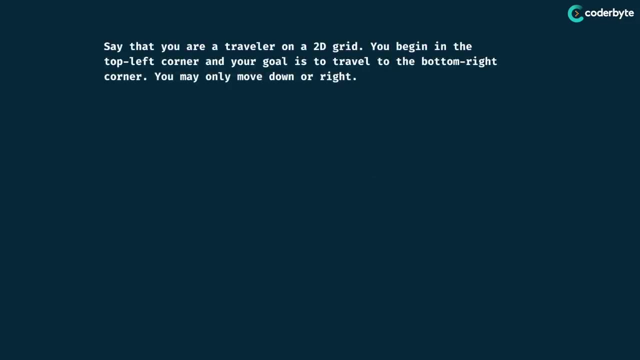 is a topic I want to drill into our heads right now. Let's head back to the drawing board and do another problem. All right now. let's revisit that grid traveler problem using tabulation. So, like before, we're going to have a 2d grid and we start in the top left. 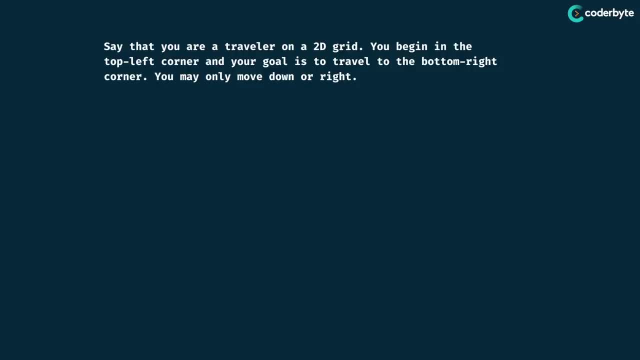 corner And our goal is to go to the bottom right corner. we only have two possible moves at any point in time, that is, to move down or to the right. And how many ways can we actually travel to the goal if we had a grid of dimensions? 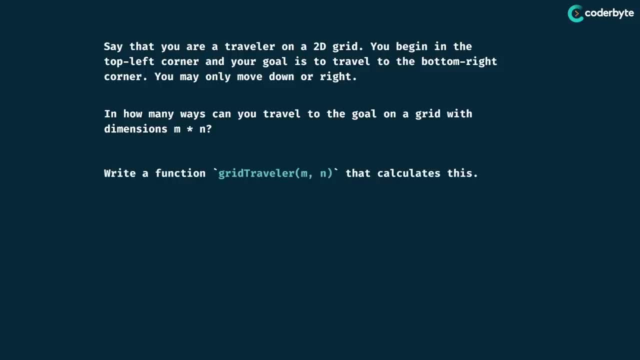 m by n And we want to write our function to actually calculate this. So let's trace through how we can build a table for this one. Let's say we're going through grid traveler of a three by three grid. that means that our output should be six in the long run. 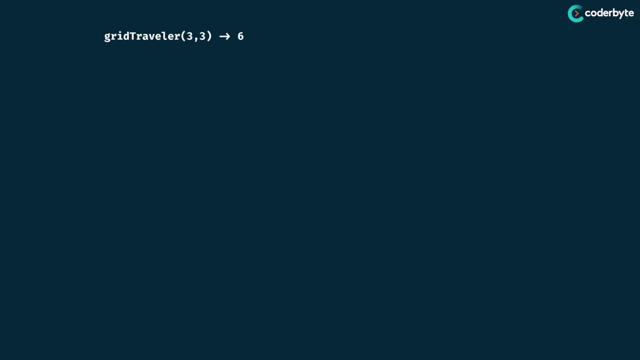 So, like before, our first step in this tabulation recipe is to create a table that is roughly the size of the input, And so here I have two inputs, and they really represent the number of rows and number of columns, So I can create a 2d array to correspond to that. 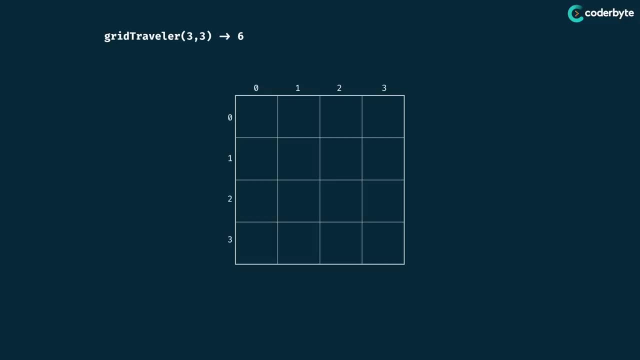 Like before, if I want the indices to match up here, I'm going to have to make sure that this two dimensional array has dimensions four by four right. If I give it a four by four array, that means that the bottom right index is really three comma three, which works. 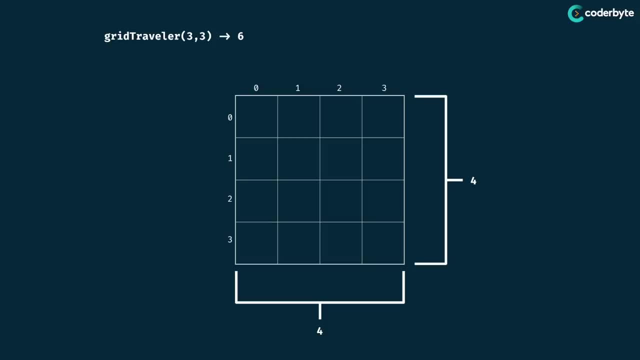 out nicely, very similar to what we did in that last fib problem. Cool, So I established the dimensions of for my table. Now I have to figure out what should I actually begin my table with Right? What are the good seed values to use here? Well, I know this is a 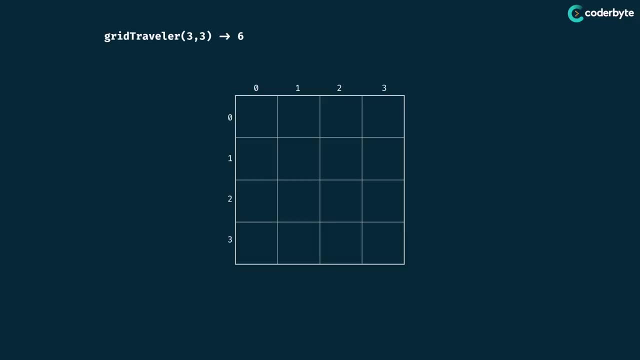 counting problem right, Because they're asking me to count the number of ways to travel through this grid. For these counting problems, a good initial value to choose is usually zero, So I'm going to put zero everywhere in this grid, But at that point I may need to seed. 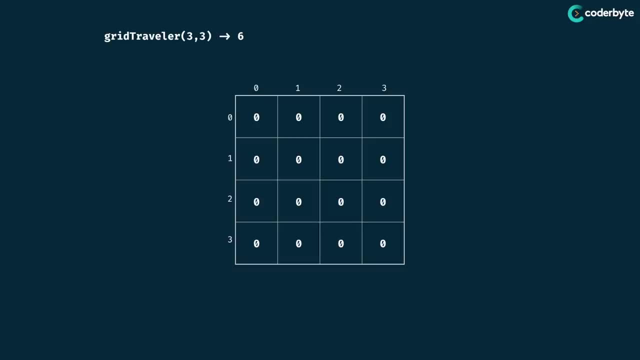 another value, another position in this table. If you recall our previous discussion about this grid traveler problem, we said that it's a really important case that all right grid traveler of a one by one should return one right. there is one way to travel through a one by one grid, And so I'll go ahead and 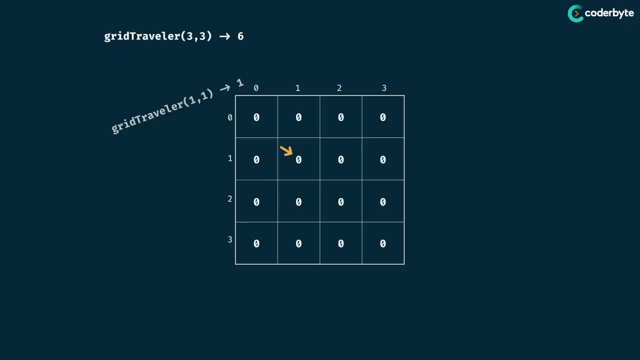 actually take that information and encode it into my table. So I'll make index one- one, actually contain the element of one, And that should give me a nice starting point for this algorithm. So at this point what we want to do is iterate through this table and come. 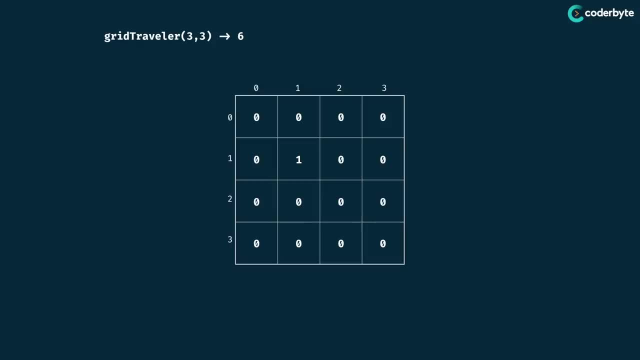 up with some logic that combines the values in this table right, basically combining different sub problems to solve my larger problem at hand. So let's just begin in the top left corner of this grid. In the long run, we can really implement this kind of iterative pattern through a grid using just some nested for loops right. 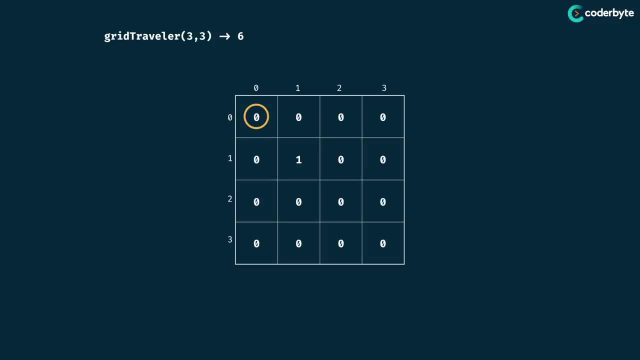 And the key insight is: I know if I'm at this position if I see a zero at indices. zero, comma zero, that means in a zero by zero grid, there are zero ways to move through it, which makes sense, right, Because if any of your dimensions contain a zero, then that must. 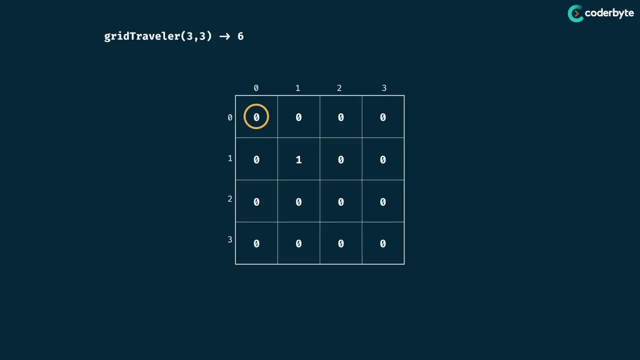 mean that your grid is empty, right. So the game isn't even valid. But if we want to have, if we want to have some consistent logic, the move is to use your current position, highlighted in yellow, right now and add it to your neighbors, right. According to the game, I can only move. 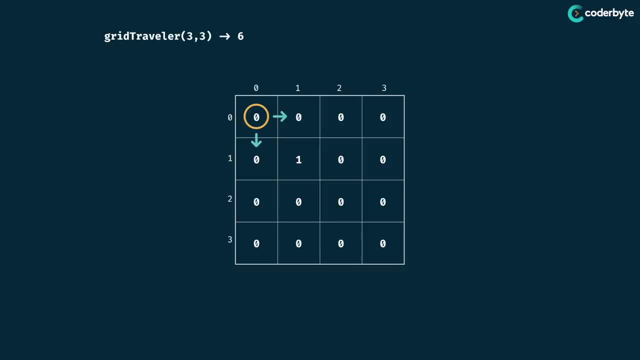 to the right or downward. So technically, what I'm doing right now is I'm taking my current positions element and adding it to my down neighbor and my right neighbor. Obviously, if I just have a zero in my current position, then really no arithmetic takes place. But 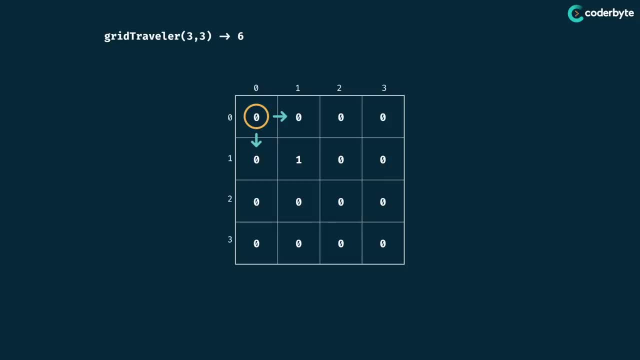 let's go ahead and do these iterations, just to make sure we have consistent logic, right? So if I keep adding these zeros to their right and down neighbors, nothing changes for now, until I get to the next row, right? This first iteration, next row: still just add zero to its down and right. But once I'm 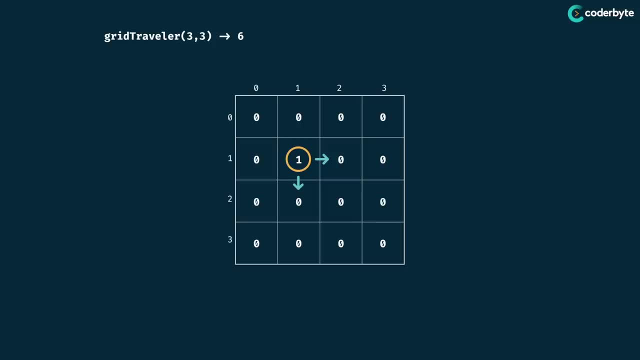 at this point I'm going to take this one, I'm going to add it to my right and down neighbor, So that means they both turn into a one. I keep following this pattern. right, Both of my neighbors turn into a one And obviously whenever I kind of reach, like, the bounds of 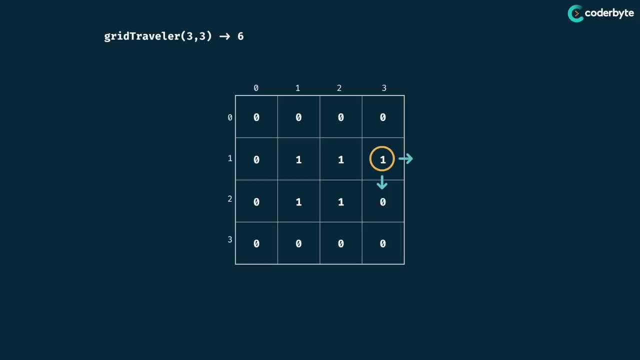 my grid. I need to probably make sure that I don't do any illegal array operations, But that's really an implementation detail for the code. So on to our next row. we contribute zero to both of our neighbors. Here we contribute one to both of our neighbors. Now we contribute. 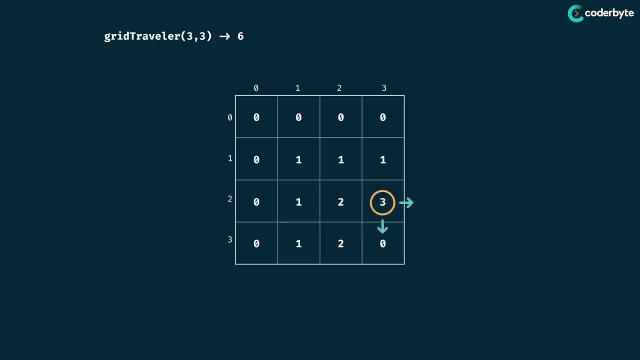 two to both of our neighbors. And here we contribute three to both of our neighbors. And finally things get interesting. in the very, very last row, I contribute zero to my neighbors, I contribute one to my neighbor, I contribute three to my neighbor, And at 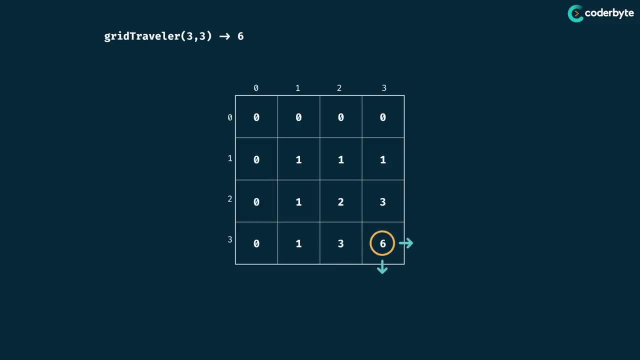 this point, we've kind of finished iterating through the entire grid. Now, if you look at this position, it contains a six symbolizing that, hey, how can you actually travel through a three by three grid? Well, there are actually six different ways. 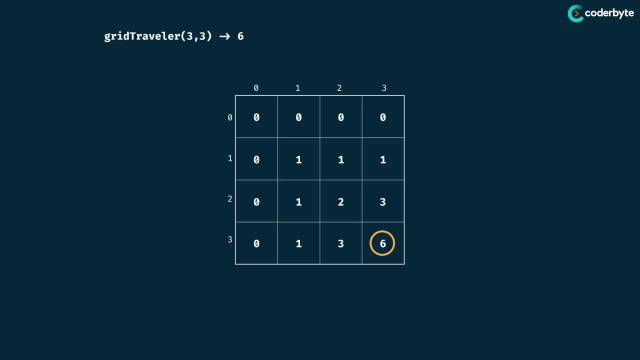 you could do that. So before we jump into the code for this one, you can probably already foresee the complexity of this. So we know that the complexity is really driven by the dimensions of this table. I know that this table is going to have m rows and n columns. 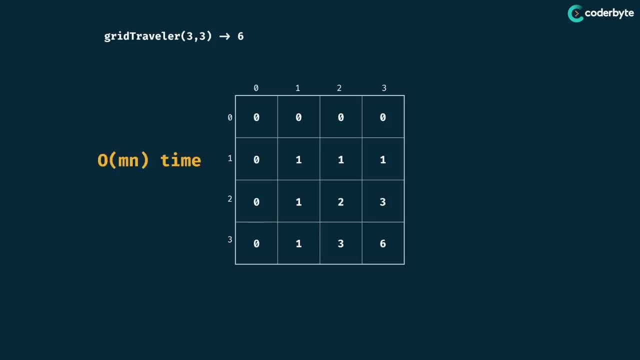 So if I need to iterate through this table, it's just going to take m times n time. And along with that, what is the space That we need? Well, it's really just a space for this 2d array, which is, of course, still. 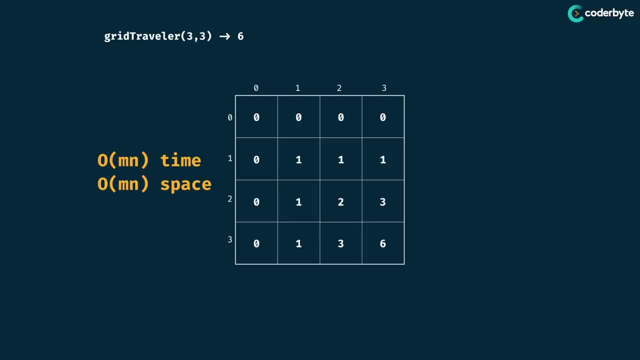 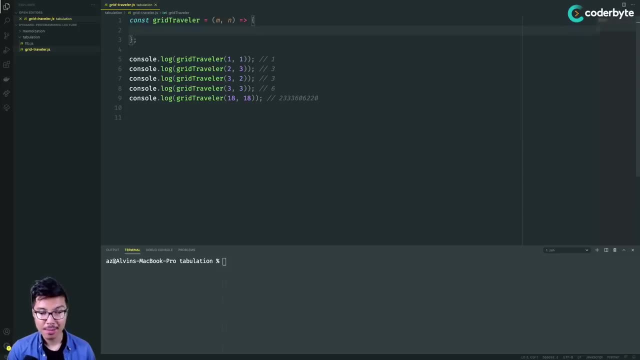 m by n, So overall I have m times, n time and space. Let's jump into the code for this one now. All right back in the code editor. let's work on implementing this grid traveler tabulation strategy. So we'll start by initializing our table, which is gonna be a little more complex. 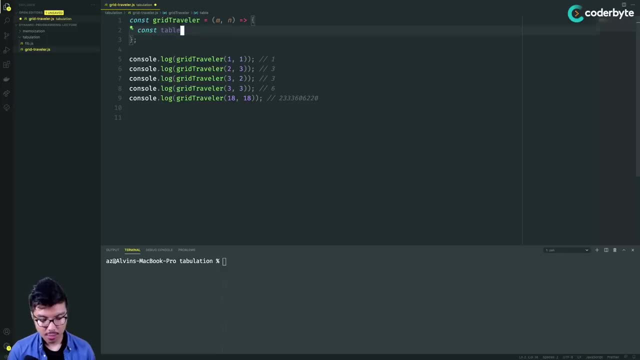 here compared to our last food function, because it needs to be a 2d array. So what I'll do is I'll start by creating, let's say, the correct number of rows, So that will be as simple as calling array. And I want really dimensions m plus one again, I have to adjust for that. 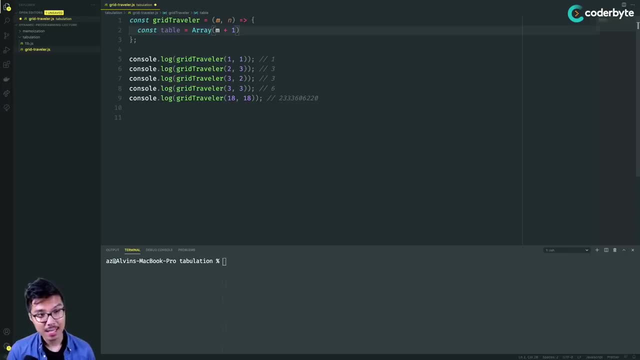 off by one error, because I want the max index in this table to actually be exactly m right and I know indices start at zero, So I'm going to up it by one over here, Cool. So I'll give me the correct number of rows And I want to make sure that the elements inside of this 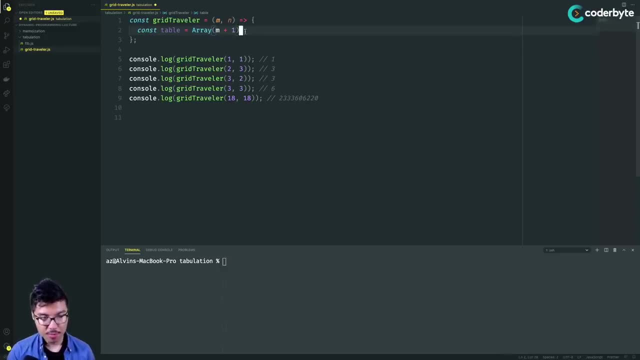 array are also other sub arrays. So a trick I can do for that is we're going to fill this up. It's kind of just a very particular JavaScript pattern. I'm going to call fill on this array I just created, And afterwards I'm able to map over it. Cool, So maybe I'll spread this. 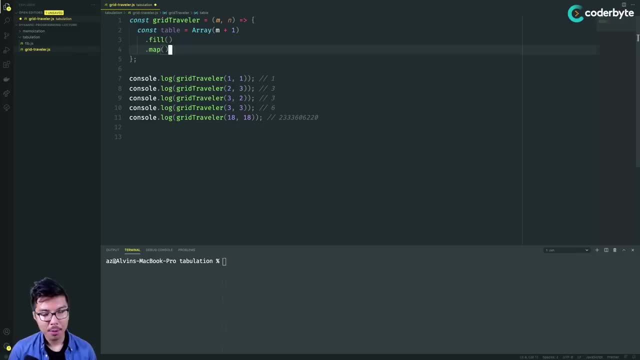 out like this, And when I map over this array, what I want to do is make sure that every element of the array is going to be a new array like this, this time of dimensions n plus one, though. So I have roughly m rows and n columns, So let's go ahead and just see what the shape. 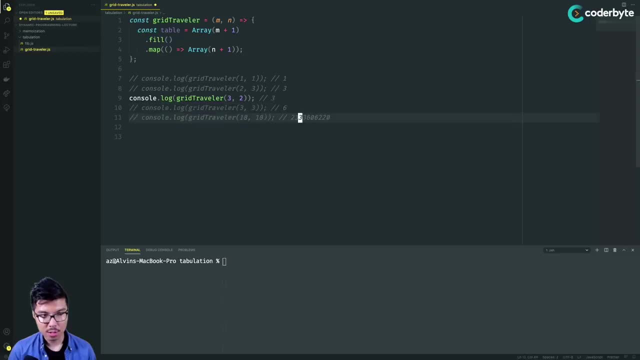 type of this is when I print out, let's say, the three by two example. So we'll go ahead and run this code. So notice that if I look at the arrays I printed out here, it looks like I have a four by three array, which makes sense because again I increase my initial. 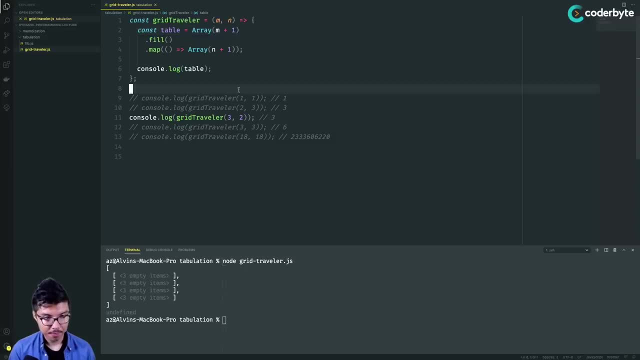 dimensions by one. that looks good to go. However, what we'll want to do is really understand how, what this map is useful for. So a very common mistake that you might be tempted to do is: can't I just, you know, skip this map part and then do the fill with the array? 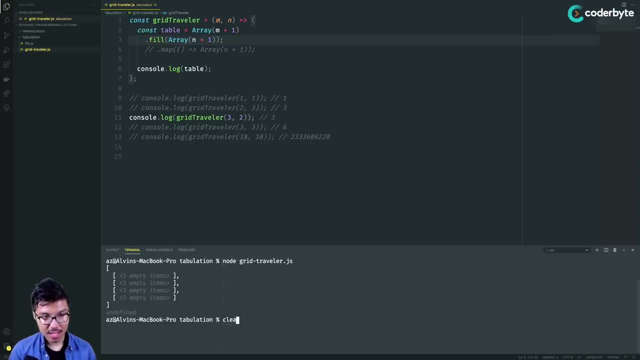 of n plus one, So that will look like it gives you the same thing. So I'll run that code. But if you read it this way, what you're doing is you're filling the entire outer array with a single array instance multiple times, right? So the shortcoming of this code is: let's. 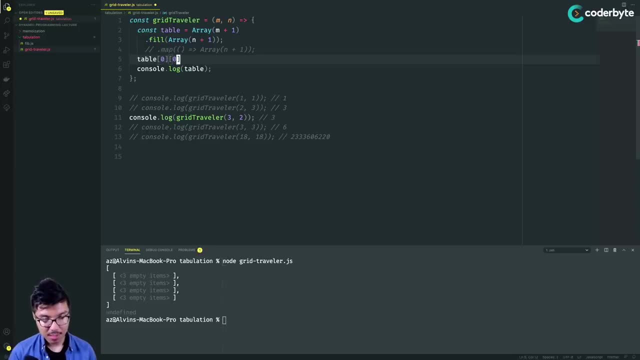 say I kind of change only one position of the table. let's say I just made an x kind of arbitrarily, that would have actually look like it changed many positions of the grid right. And that's because this is technically just one array that's inserted multiple times into the outer array, whereas 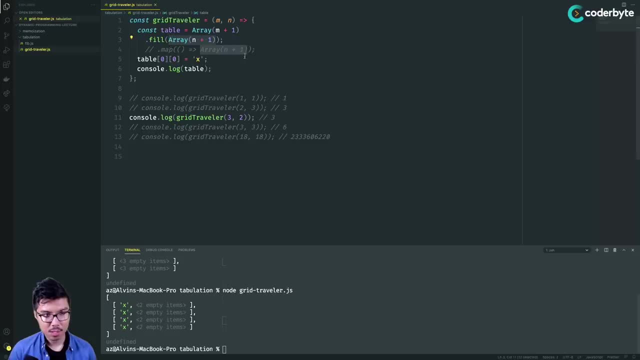 I need a really unique array references, So that's how we need the map pattern here. I know every time we evaluate the callback function to map, it's actually going to execute this entire function, which means it's going to give us a new inner array instance, right? 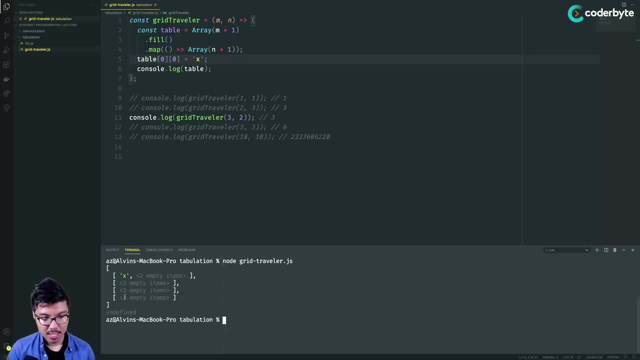 So if I use this map pattern, I run again. this is really the intended behavior, right? I have a unique array as a sub arrays here, So let's take out this expert. But, that being said, now that I have the correct shape of 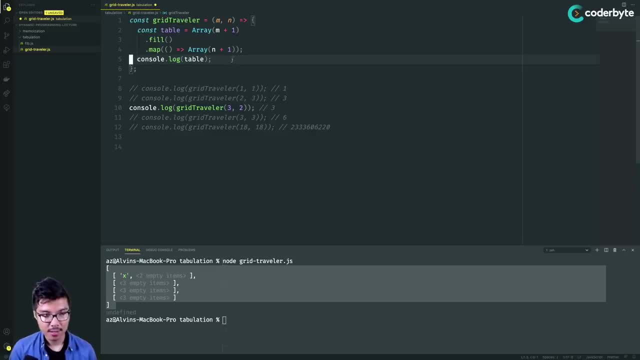 my table. I need to insert some good starting values, right? So what are the seed values here? Well, recall, in our strategy we said that basically the entire table could contain mostly zeros, So maybe I'll bake that right into this line. So after I make a new subarray, 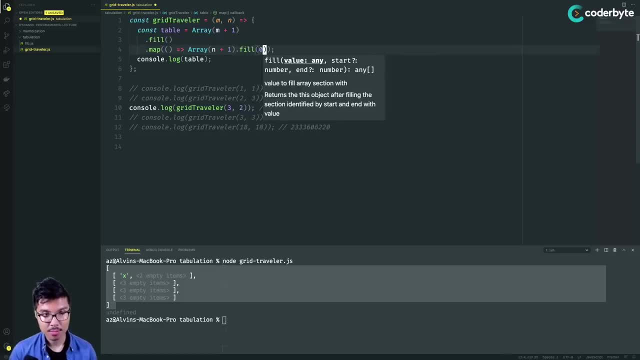 I'll be sure to fill it with some zeros. So if I run that now, I should have a nice table. Cool, So it's looking pretty good At this point. I also need to see it. another value: right, We talked about it in that we should see table at position one, one with 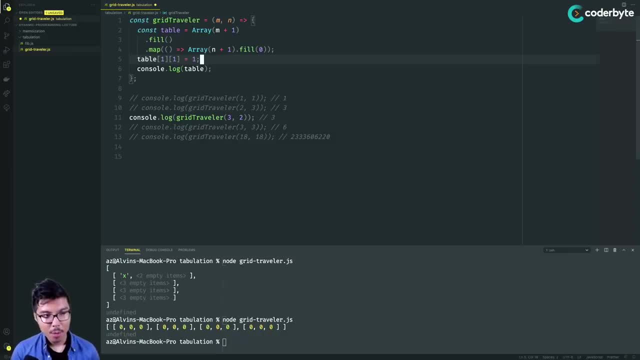 exactly one, because it's sort of like our base case: when we have a one by one grid, there's definitely only one way to travel through it. So now we have the elements of one in position one one Nice. So at this point now I need to iterate through my table and fill in the position. 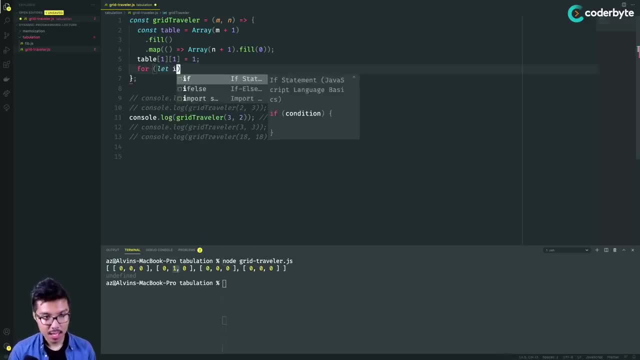 So I'm going to use just nested loops for this. So I'll say, let's i equal zero, And I want to make sure that I goes up to n, including m, right, basically the dimensions of the table, and I'll do I plus, plus and very similar for my inner loop, being sure this time to 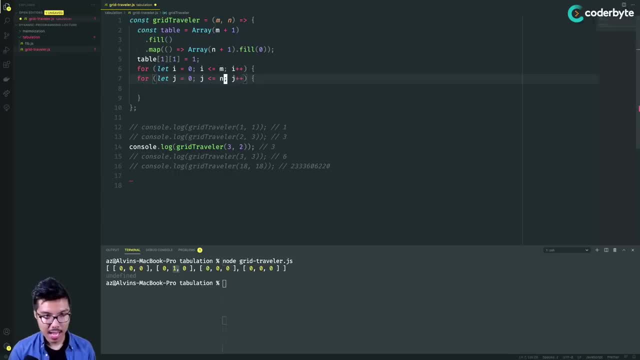 reference J, and J is going to go up to n this time. Also, just have classic nested loops just iterating through this two dimensional array, right? So, as I'm iterating through the table, what was the logic we traced through in our drawing? Well, what I needed to do, 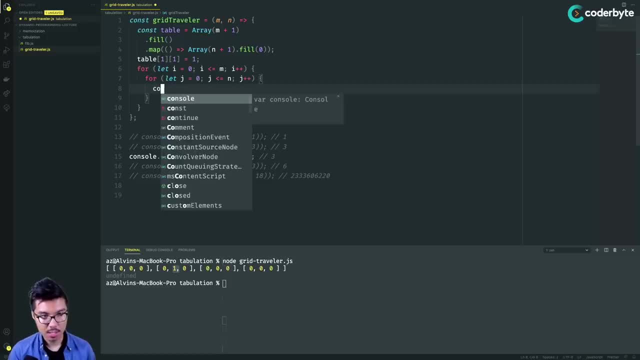 was take my current element that I'm at, so maybe I'll call it, let's say, my current. So my current element would be at table ij. So I need to take this current element and I need to add it into my right neighbor and my down neighbor right. So if my row is a 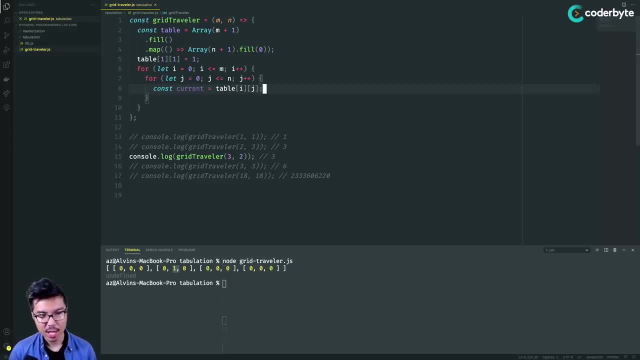 i and my columns j. it just means I do some arithmetic on i and j right. So if I want to increment my, let's say, right neighbor, what I can say is: look at table, at position i j plus one that would be directly to my right, and I'm going to increase it by whatever. 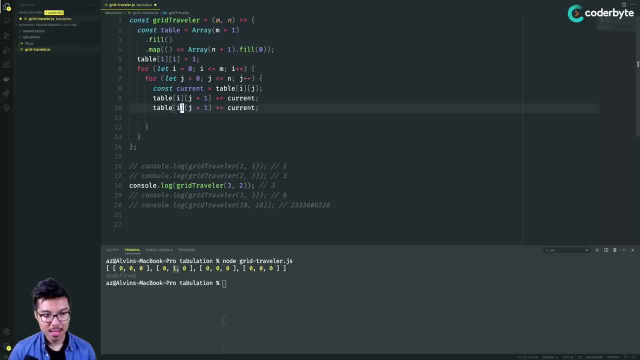 this current is. If I want to look at my down neighbor, then that'd be i plus one, but I keep j the same, Cool, So this will add to my two neighbors that are to the right of me and below me, And at this point, what we have to be aware of is, like, what happens at our edges of this. 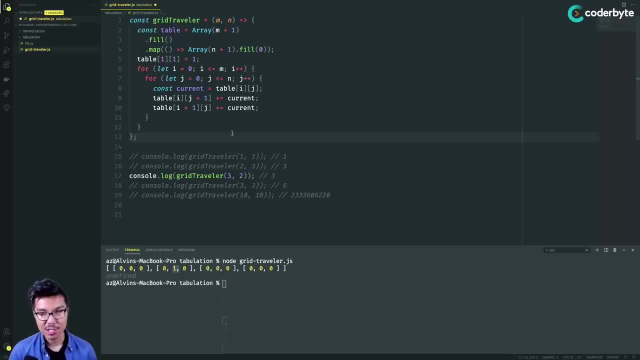 table. we know that if we're already at like, the last position of a row, if I do j plus one, I'm going to go out of bounds. And so to make sure I don't step out of bounds on these increment expressions, I'll need some conditional logic. So I'll say: if the right. 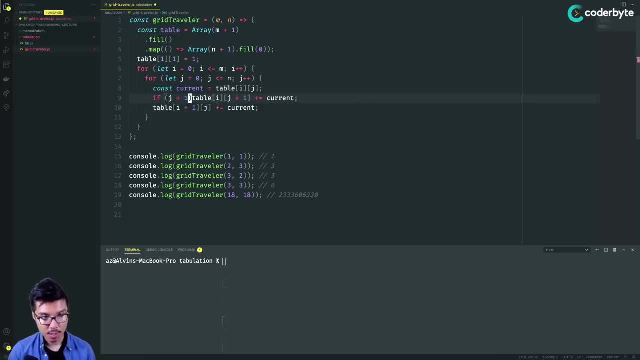 position is inbound. so if j plus one is less than or equal to n, then I'll go ahead and increment it, and should be okay. And likewise, if I plus one is less than or equal to m, then I'll also increment, right, Notice. 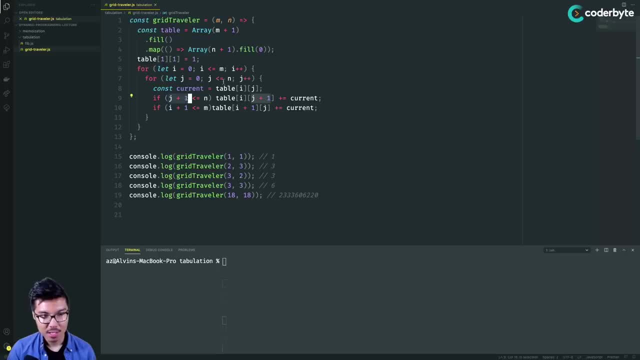 that when I check my like j value, that should be using n right, because that's the number of columns and then I is a number of rows, so it should use m Cool. So what I have so far is alright. I'm iterating through every position of my table And I'm going to take 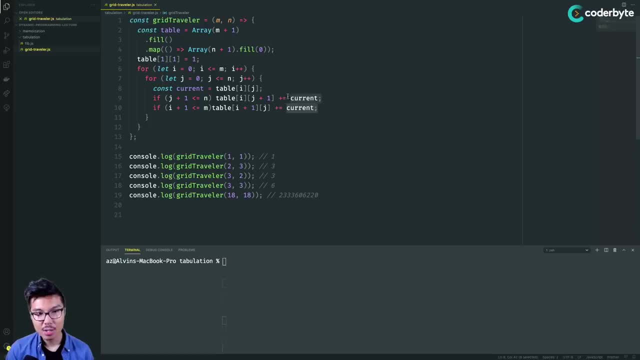 the element at my current position and I'm going to add it into my right neighbor as well as my down neighbor, But only if they actually exist, Cool, So once I'm done filling up the table, then my final answer should just be at position M and right, just a very a bottom right corner. 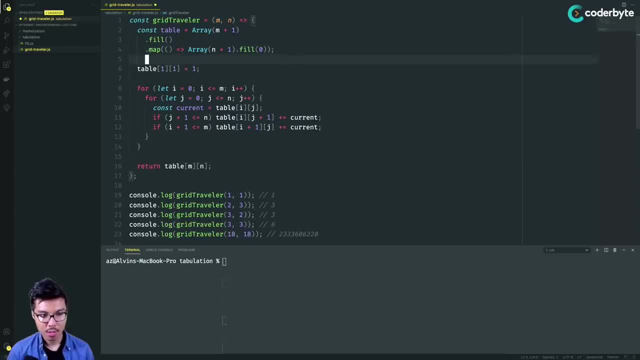 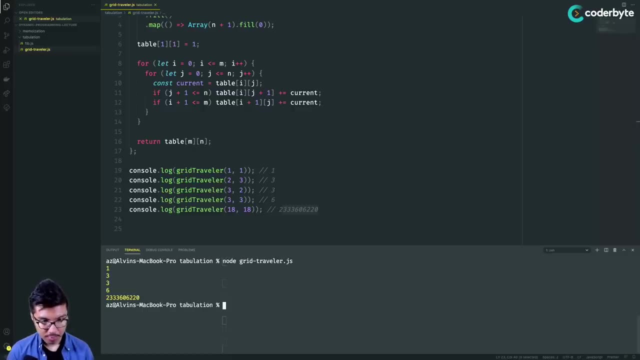 here. So let's give this code a run. So I should get 1336.. And then there's a very large number of run grid traveler, Nice, and looks like this solution is totally working And we are already satisfying the last example here. I don't know if you were able to see that on the screen. Let's give. 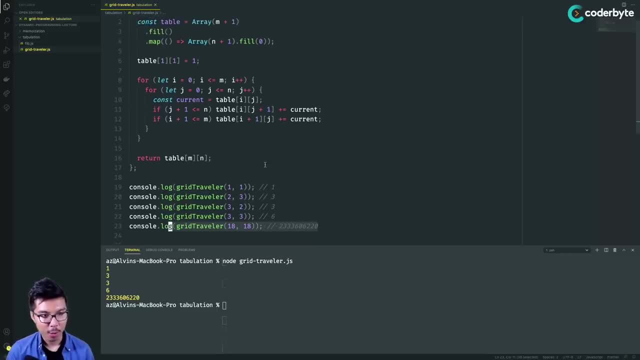 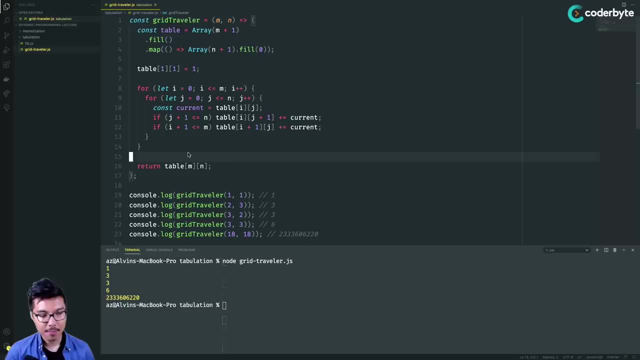 right. if you tabulate off the bat, you will have a pretty quick solution, And we already traced through the complexity for this. So take a moment to you know. look at this code, let it sink in, or really try to understand how we took that whiteboard strategy and implemented. 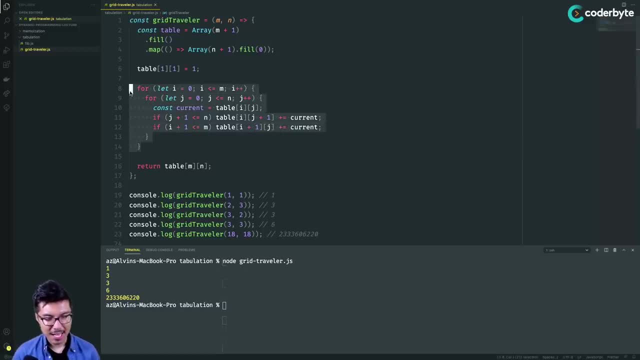 it in some code. right, we do have to do some like kind of fine implementation details, especially with the bounds checking here. But I think the most important logic is about how our current position of the table contributes to our immediate neighbors, to the right right. 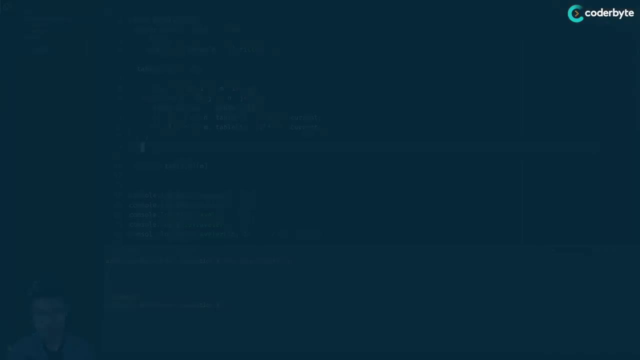 and downward. With that, I think let's head back into the drawing board. Alright, now that we've seen tabulation in two different problems, hopefully you're noticing some patterns, right? Let's give ourselves some rules we can follow to tackle any dynamic programming. 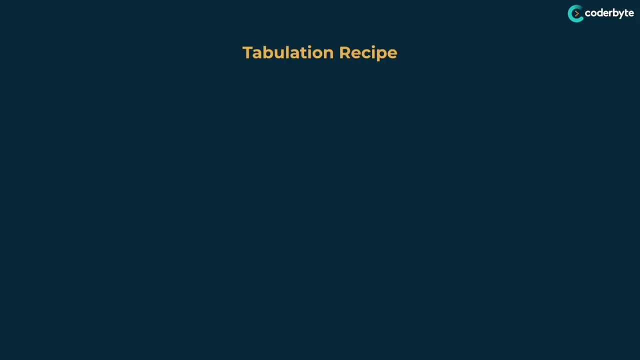 problem using a general tabulation strategy. With this tabulation recipe it's going to be pretty different compared to our memo ization recipe in that there aren't like two main steps. When I talked about memo ization I said: make sure you implement the brute force. 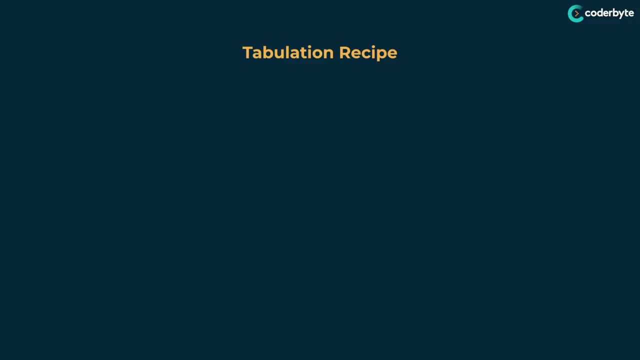 first And then add the memo ization afterwards, Whereas if you just try to tabulate a problem, you're really going to have the most efficient version of your solution all in one swoop. And so what is our first step for tabulation? Well, of course, you have to visualize it. 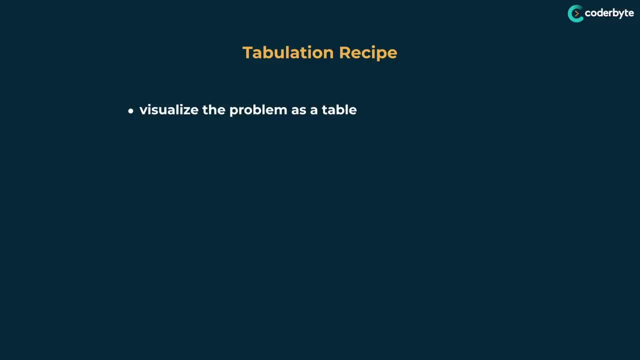 as a table And that really begins with a conversation of what should like the size or dimensions of the table B. that should definitely be correlated, based on the size of the input. So in the case of Fibonacci of n, we made our table roughly. you know n elements long sometimes. you definitely have to watch. 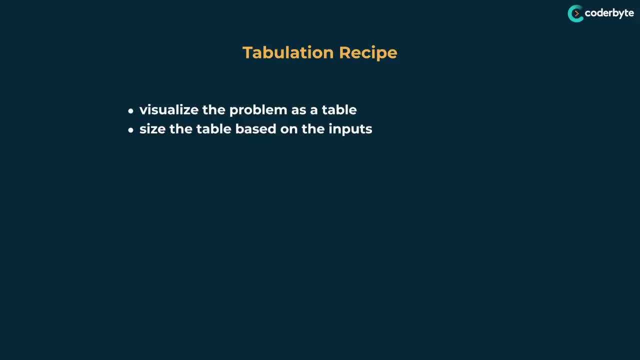 out for like an off by one scenario which we've been seeing lately And the case of our grid traveler problem. we saw that because our- you know, problem represents a grid, we had to create a two dimensional table at that, So figure out the size of your table. 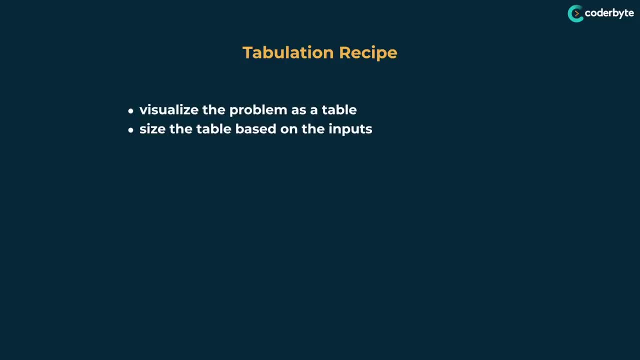 based on the inputs to the problem- Cool. Once we do that, we need to initialize some values within the table. To me, this is always about choosing compatible types. In other words, if your problem asks you to return a number, then it'd be wise to initialize. 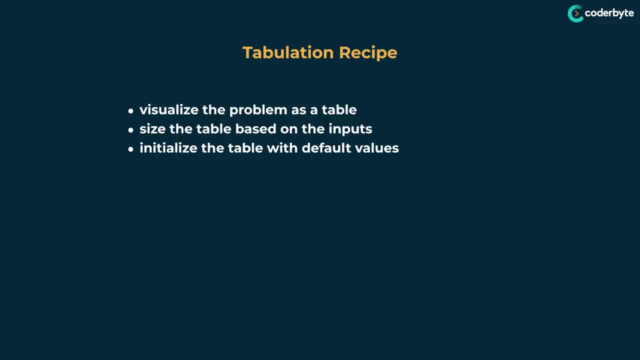 the values of your table with numbers right. On the flip side of that, if I was asked to return a Boolean in a problem, they'll consider initializing true or false within the table. Cool, And once I have all of the kind of generic values filled up in the table, then I choose. 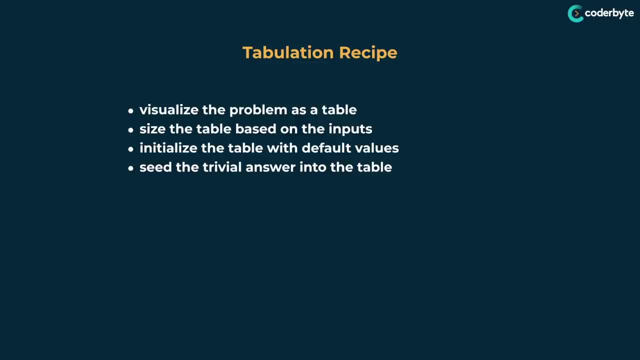 my very important seed value right. I know that this seed value should capture the scenario where I have a trivially small instance of the input where I automatically know the answer right. So in the case of our classic Fibonacci, that means I just seed the n one. 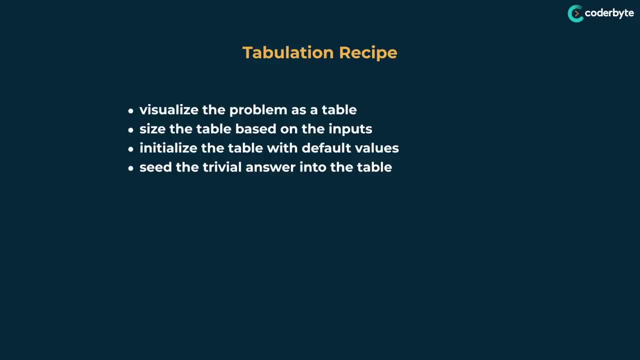 and the n two values of my table, with one and one respectively. And in the case of our grid traveler, we were sure to you know, capture the scenario where we had a one by one grid. So you're gonna need to see seed those values because that's the basis upon which we fill the rest of the table. 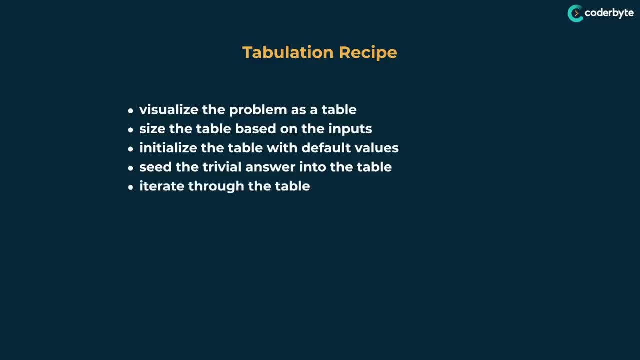 And then we have the hard part, which is really iterating through the table, And you have to come up with some logic right As you iterate through the table. you have to design some logic that fills further positions of the table based on the current position And 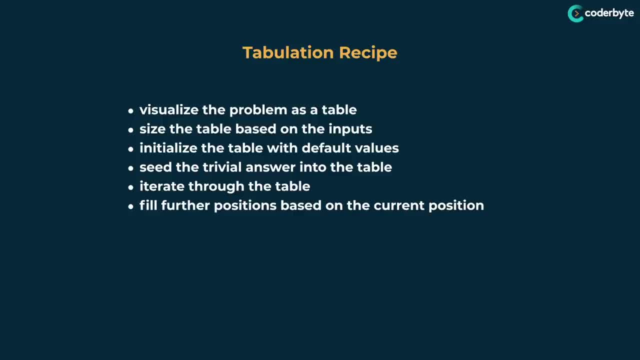 you really have to. you know, look to the problem to figure out what the logic is. In the case of Fibonacci, it's as simple as if I'm at some position of the table. I look one space ahead and two spaces ahead. 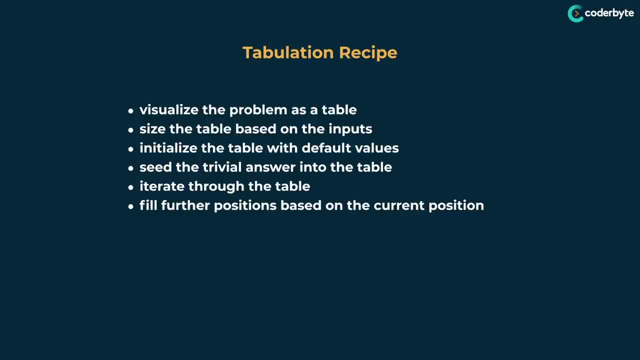 Now you can see this is a very reminiscent of the pattern Fibonacci. in the case of our grid, traveler problem was about looking the unit to the right or the unit downward, effectively shrinking the size of our grid. So it's really you know, up to you to figure out the logic. 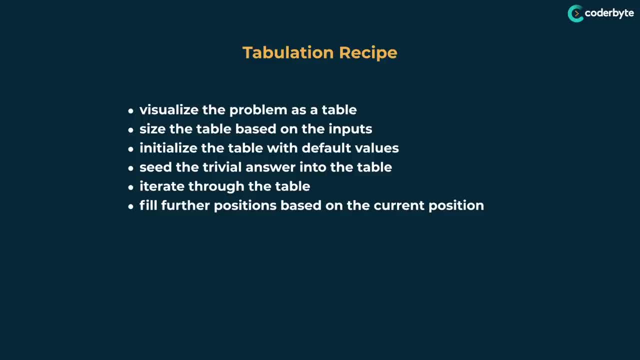 look for language in the problem. What I always do is focus on what options I have at any point in the problem. right, My options are: do I go rightward Or do I go downward in that grid traveler problem? So we'll stick to these rules as we tackle our attack. Let's 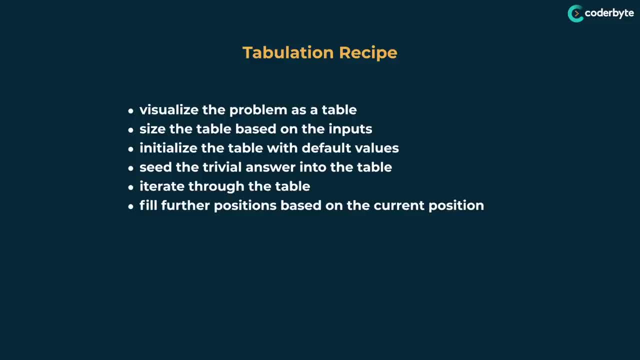 get started. So what we're going to be doing is we're going to be looking at the problems of the grid, and I'll share a few examples of the problem. So let's first look at our grid traveler problem, tabulation problems, and we'll utilize them right now. Okay, so let's work on tabulating. 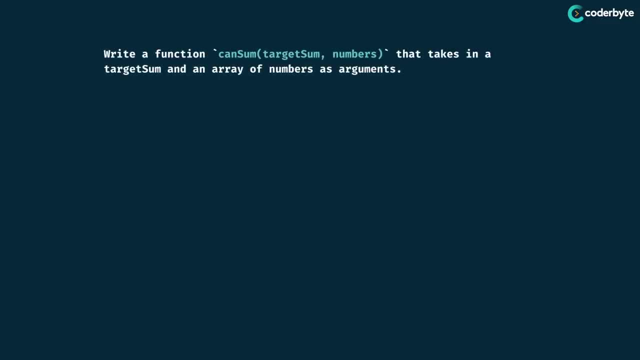 our can sum problem now. So recall that in this problem we want to do is take in a target sum as an argument as well as an array of numbers, And we want to return a Boolean indicating whether or not we could generate the target sum by adding numbers in the array we can. 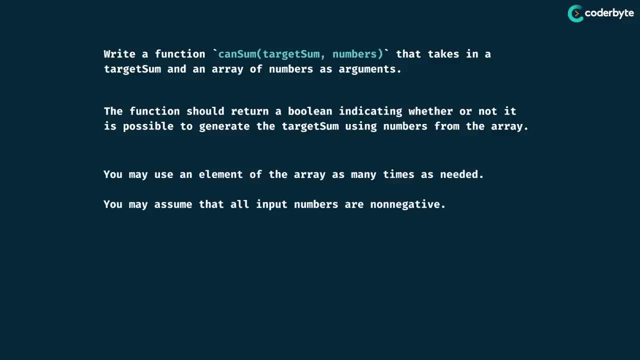 reuse an element of the array as many times as we want. We can also assume that all the input numbers over here are non negative. So we've solved this problem before right recursively using memo ization. But now we'll want to use a tabulation point of view. So 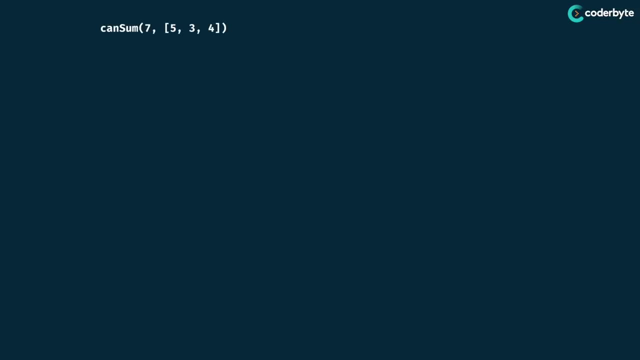 let's come up with the strategy here. So let's say I gave you this input of seven and an array of 534.. In the long run, the answer is true, because it is possible to generate seven. right, You can either do a three plus four or a four plus three, and that would 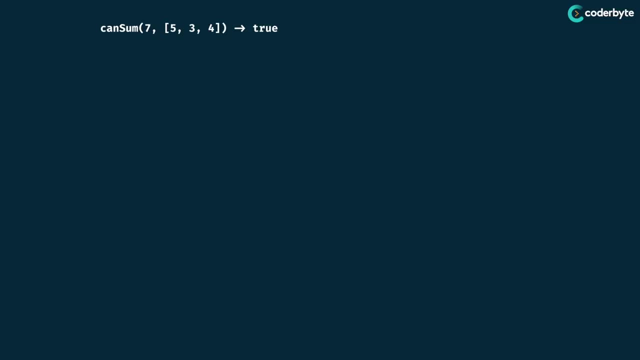 give you your original target. So you know that in the first step for tabulation, what we need to do is create a table. But I guess the question here is: how do we generate a target? And the answer is: what size table do I create? I have two inputs. I have the. 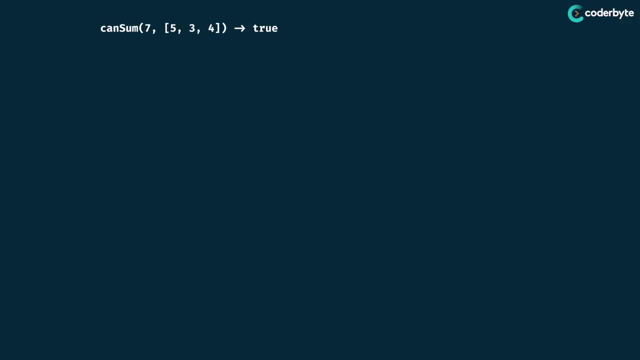 target, as well as the array of numbers, which of those actually contribute to my initial table, And so the key insight is to think about, you know, what's going to change throughout the problem, In other words, if we can reuse the numbers of the array as many times as. 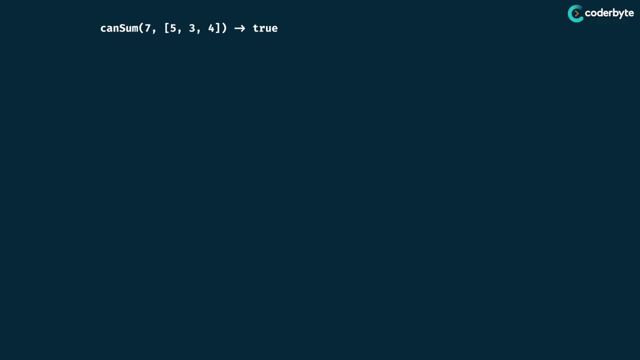 we need, then it's not like we're shrinking the size of that array. However, if we think about the target number or the target sum that we're given, we do have a goal of actually reaching that target, So then we're going to increase to it. 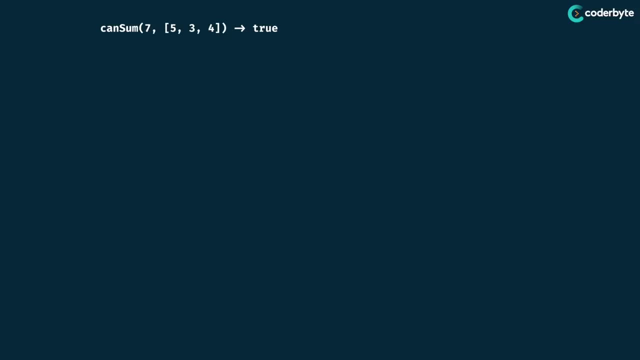 Over time, and so I'm going to use that as a basis for my table. that is, I want to create an array that is roughly the size of my target sum. So because the target sum is seven, I want to make sure that the indices line up perfectly. So I'll actually have to create 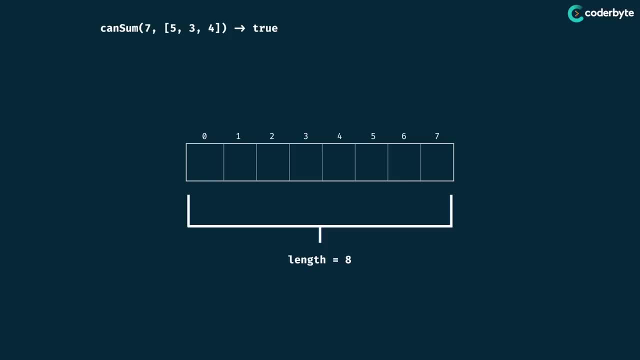 an array with length eight And in general, I just be creating an array of length target sum plus one, because we have that classic off by one error over here. All right, now that we have the correct size of table, what do I actually want to store inside? That is? 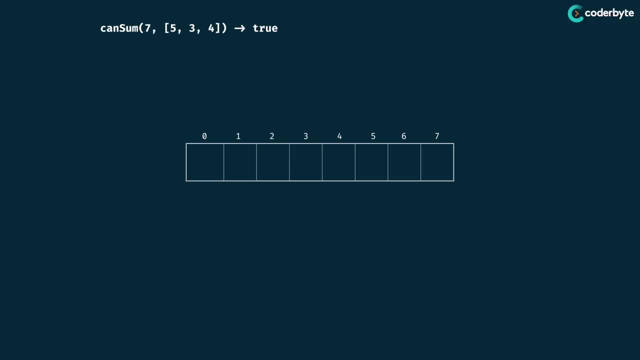 what should the eventual elements of this array be? So a really nice rule of thumb you can use for that is to just recognize what type of your answer should be in the long run, right. So here they're asking for a Boolean answer. So that really tells me that. 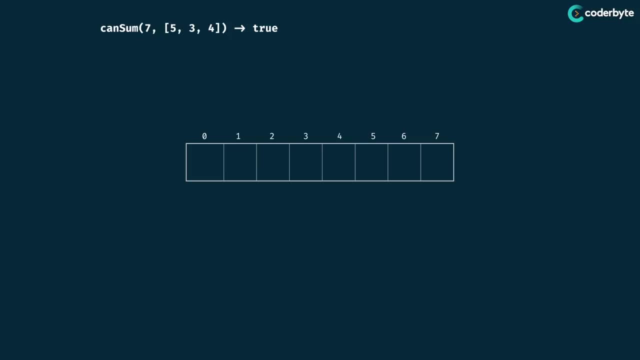 I should probably put some Boolean data as the elements of this array. So I'm going to start by initializing every element of this array with a false value. And the reasoning is right now we're kind of assuming, before we check anything, that none of these target. 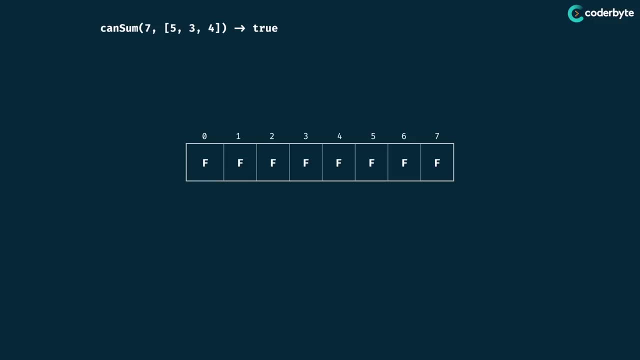 sums are actually possible to be generated- Cool, But now I have to think about any particular seed values. I need something inherent to this. can some problem is we treat the target sum of zero very special, right sort of the base that we use. In other words, someone gave me a target of zero, I know that that. 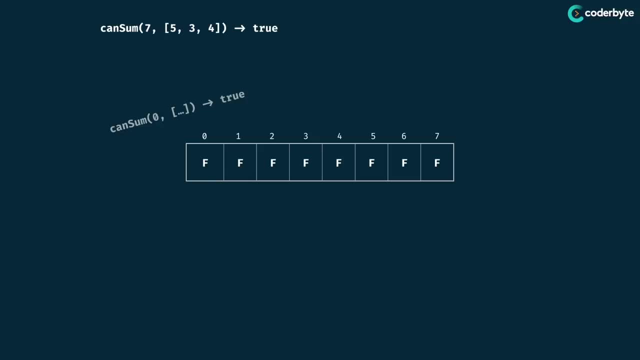 is always possible, no matter what elements I have in the array, because to generate zero I can just take no elements of the array. So that's going to be a really important seed value here. So I'm going to populate index zero with the element true. Cool. So now I'm 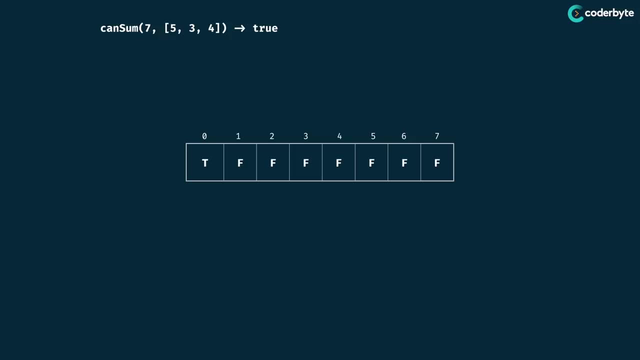 going to have some good seed value. Now we want to think about how we can flush out the other elements of this array, sort of in a linear fashion, right? So I know I'm gonna have to iterate through this table, So let's just start at the very first index. So right, 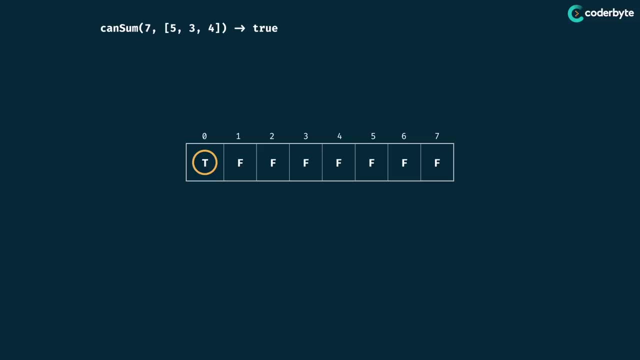 now I'm looking at index zero And if I'm situated in any position of this array, then the value I'm currently looking at should basically say: you know, is it possible to generate that index amount? In other words, since I have a true at index zero, then I 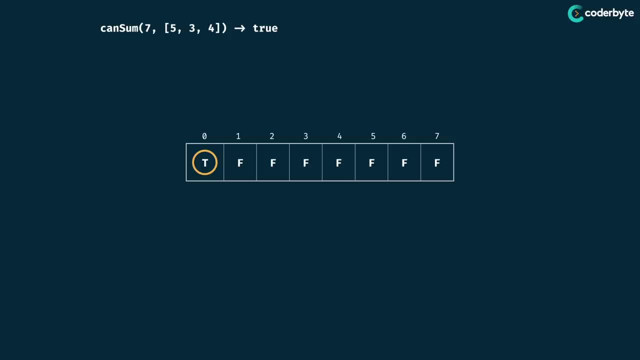 know that it is a positive. All right, let's check it out. All right, let's do this. All possible to generate zero using the coins of the array. But now that I'm at this position, how can I actually transition into the further positions of this table? And so what I want? 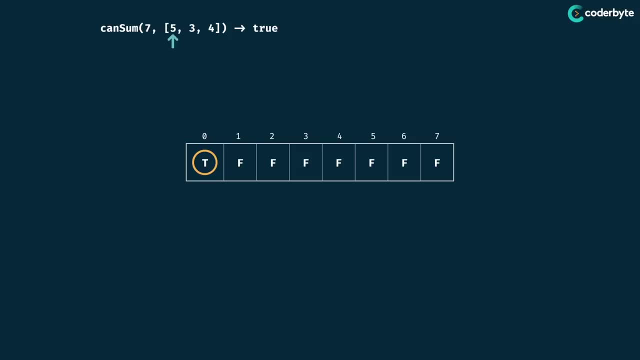 to do now is consider the possible numbers that I can take into my son. So I'm going to start by looking at this first element of five. I know that if it's possible to generate zero, then if I also have a five in the array, then it's also possible to generate five in. 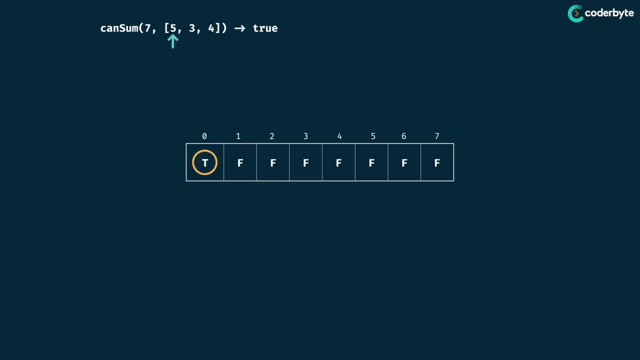 the context of my array, that means I should look about five spaces ahead from my current position. So I look at this spot right, exactly five indices ahead, And right now I should actually replace this false value that's stored at index five with a true And again the. 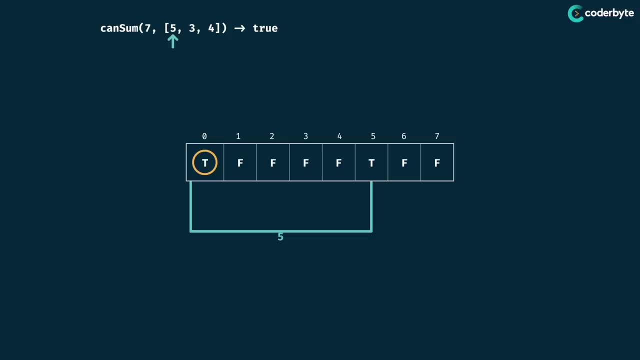 reasoning is: if it's possible to generate my current amount- right, right, and I have a true in the zero, it's possible to generate my current amount and I could take a five- then it means that the position five steps later should also be true. 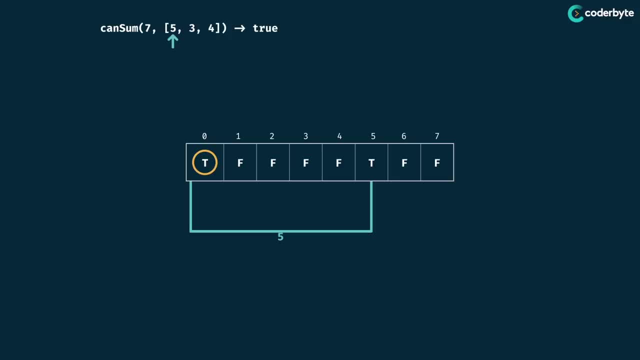 Right, And I want to actually continue this process for the other values in my numbers array, So I'm just going to look at the next element of three. That's basically telling me that, hey, the next spot three places away should also become a true, So I'll just go. 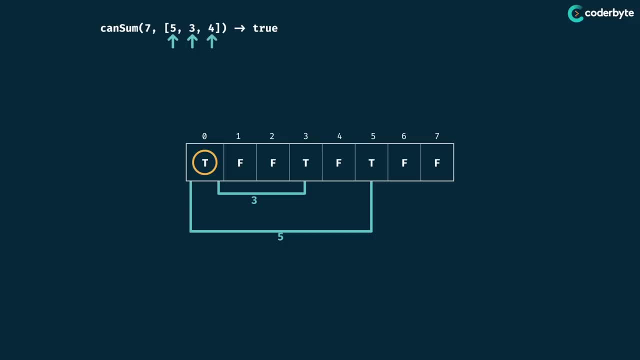 ahead and make that a true. And finally, likewise for the last element of four right, the element four spaces ahead should also be turned to true. Cool, And at this point I think I finished, like my very very first iteration, that is, when my current is at index zero. 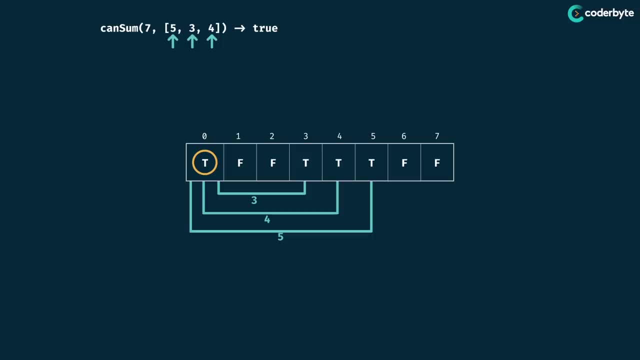 And at this point I just want to keep iterating through the array, So I'm just going to shift my point of view or one space to the right. So now I'm looking at my current as index. one notice that over here my current element is actually false. So what that means is: 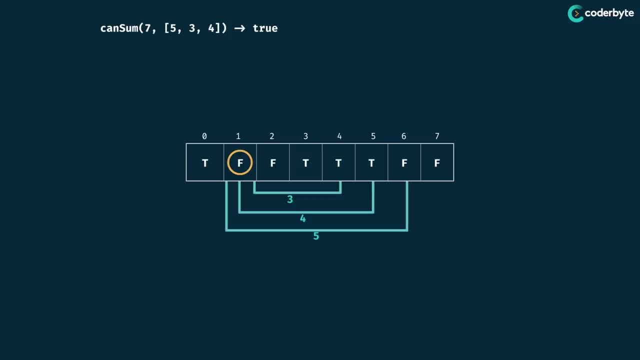 it is not possible to generate a one using the numbers of the array, which logically makes sense, where I only have five, three and four. So there's no way you can ever give me back a one, right? So if I have a false value at my current position, then I should. 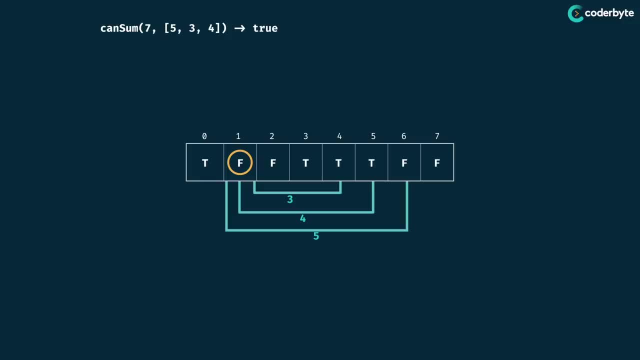 not modify, like my further values, by looking ahead. So notice that if I look at my edge for five, if I look five spaces ahead, I am not going to make that a true because my current position is not true, right, So I'm going to keep iterating. Same thing happens when 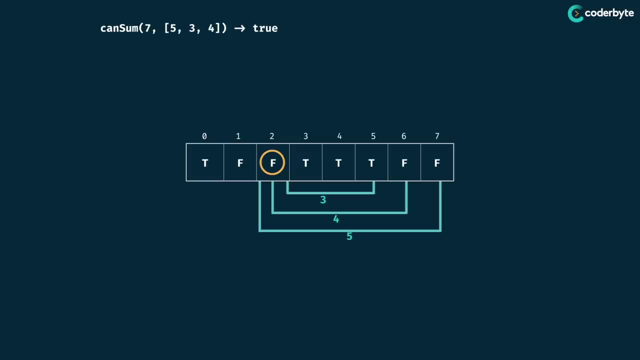 I'm at index two because the current value is false. there's nothing to be done here. Things get really more interesting on this iteration right. I'm at index three as my current, then I see a true at this position, So that means I need to look ahead to my future. 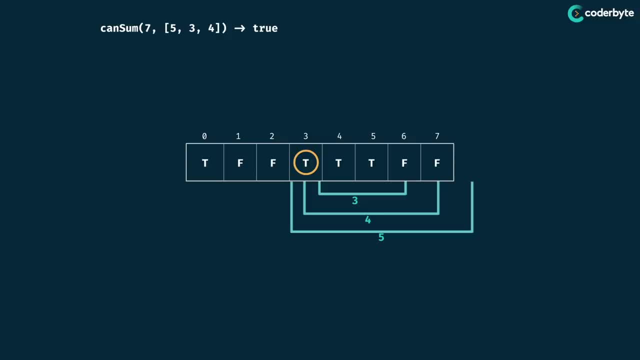 positions. I need to find them to be true. Obviously you'll notice over here, if I look five positions ahead when I'm currently at index three, then that would actually be out of bounds. So I don't need to look that far ahead. So we'll kind of drop that connection. But at 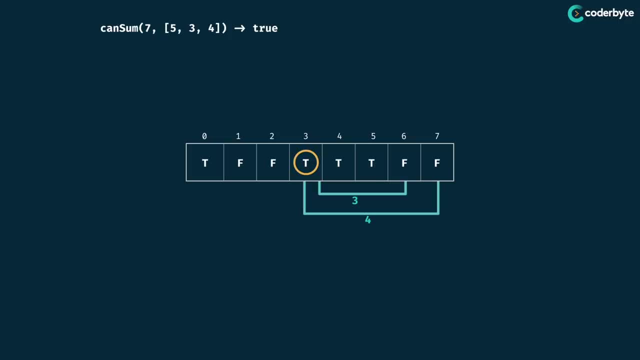 this point, I should make the space three positions ahead true, as well as a space four positions ahead. So that means that indices six and seven are set to true, right? I keep doing this process all the way through the entire table. Notice that as I keep iterating, 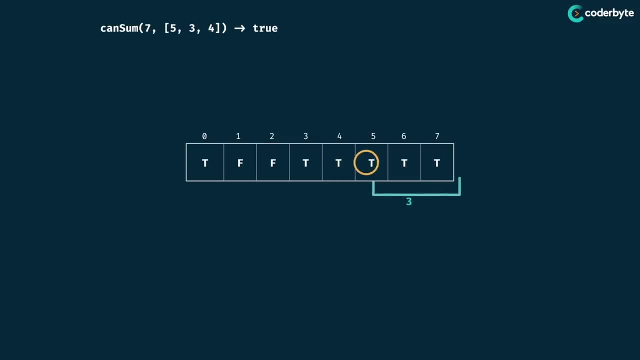 toward the right, these forward looking references kind of stop being useful because it goes out of bounds. But the point is, by the end of all of these iterations I do have a true stored at index seven, which means that it is possible not to generate a quantity of seven. And if I 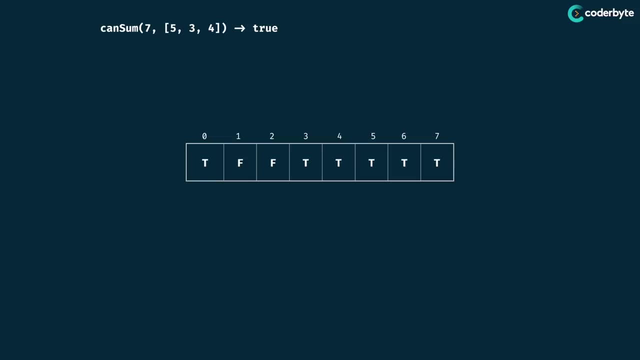 do a quick spot check and I look at just my entire table right now. it has very consistent data. In other words, if I notice where all of the true values are right there at 0,, 3,, 4,, 5,, 6, and 7,, that means that all of those quantities for target are actually possible. 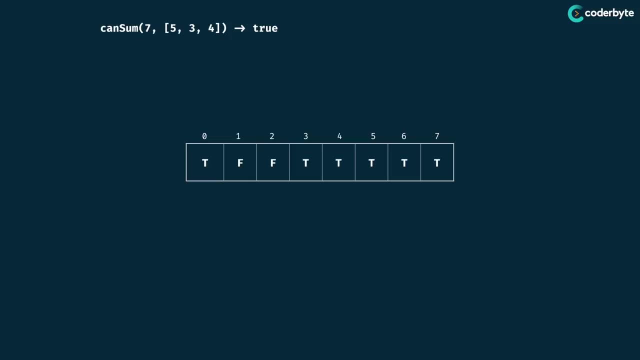 Right On the flip side. if I look at the only elements and indices that are false, like one and two, that makes sense because those are the only quantities that are not possible, where you can't possibly generate a one and two using a five, three and four as your. 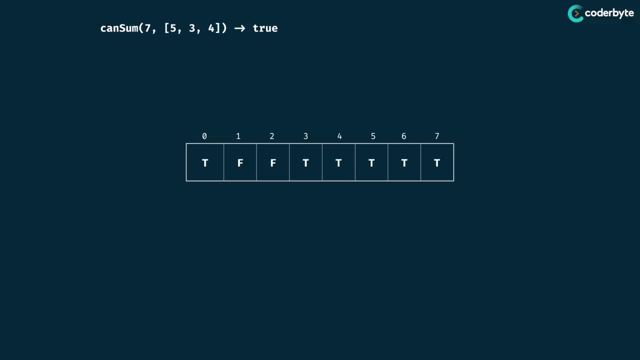 options are adding up right. So we know, by the end of this algorithm, the element that is stored at the last position of our table would be the final answer, right? So if it's true, then it's possible. if it's false, it is definitely not possible. Alright, so let's. 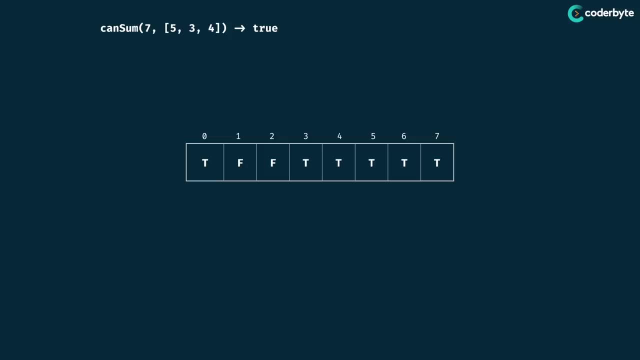 wrap up this sketch by actually talking outside of the table. So here's how this whole idea sketch, by actually talking about the complexity of this. as always, we'll define our terms. So we'll say that n is going to be the target sum, which is just a number, And the flip. 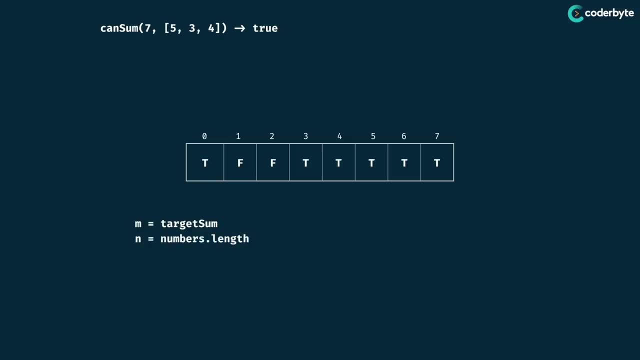 side of that, we'll say that n is going to be the length of the numbers array And we already have the vibe that. hey, both of these terms definitely affect our complexity, right? If you give me a larger target sum, that's probably a harder thing to calculate In the 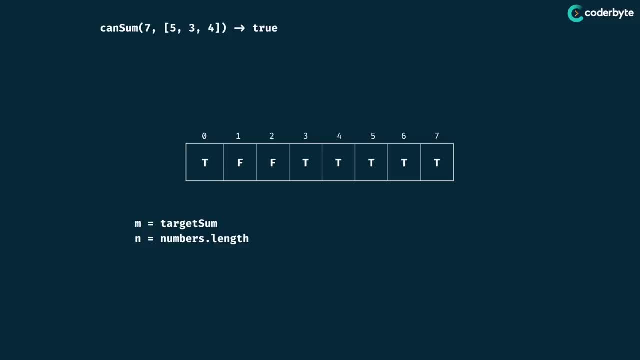 same way, if you give me more numbers to choose from, it's even harder to calculate, right, And we can recognize that. the algorithm just has us flush out this table, And I know that the table is of size m, so we're going to have at least m. However, as I iterate through 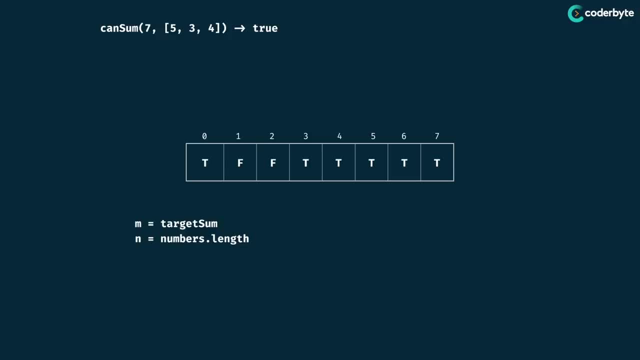 every position of the table. what I had to do was actually look ahead in the table for every single element of the numbers array. So I know that that's going to be accomplished basically using some nested loops, or I'm going to have a loop to iterate through just. 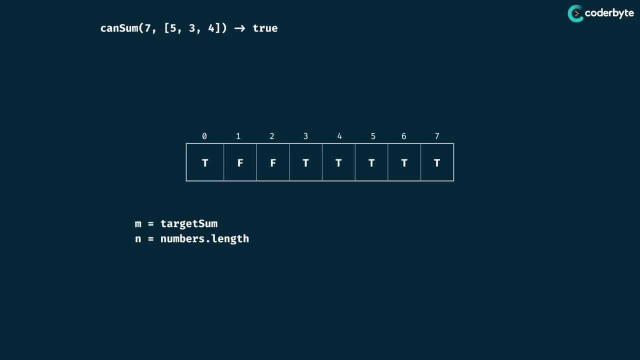 the table and then a nested loop to iterate through every number of the numbers array. So, overall, I'm looking at an m times n time complexity And along with that, what is the space here? Well, the space is really just the exact size of this table which is based. 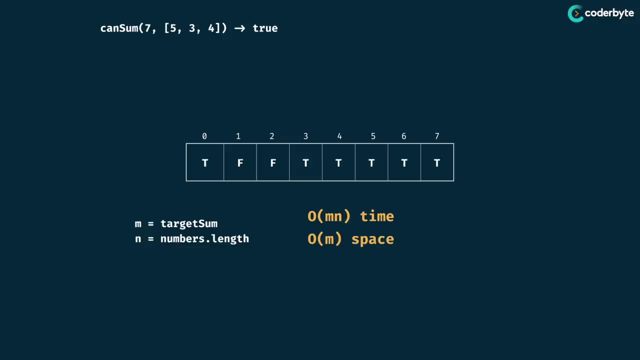 solely on m. So I have just m space overall. Nice. So this is already looking like inefficient implementation, especially because we're not dabbling with any exponential complexity over here. I think let's work on the code now. So here we are, back in the code editor. Let's 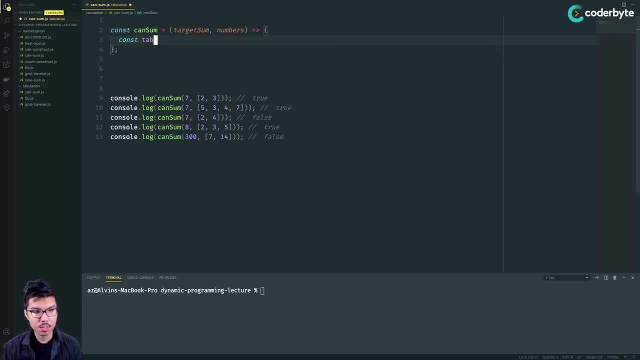 start, like we usually do, by creating our table. So I'll store this table And, like we discussed in our drawing, we need to make it roughly the size of our target sum. So I'll create an array. I need to make sure that the indices lineup directly right. 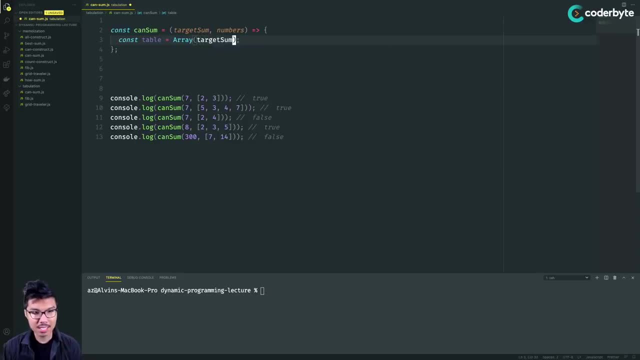 I want index that is exactly the target sum, So I'm gonna initialize it to target some plus one, right? So that means, if I pass in, target sum is seven, I'm going to create an array of length eight, which means that it's very last index is seven, which is perfect. 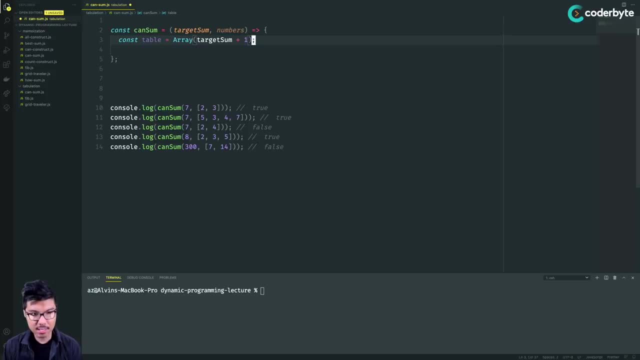 Cool, And while we're here, we'll go ahead and actually initialize this array with all false values, So I'll type in the same. All right, I'm just going to leave this one as is. We'll call it a target sum. And now that we have our target sum, let's call it on this. 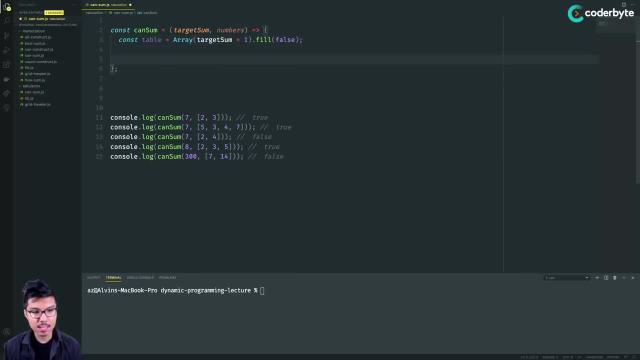 I'm going to call it an array of various kinds of numbers. We're going to call it a target sum. So I'll do that. I need to make sure that I seed index zero with a true symbolizing that the target sum of zero it's always possible to be made even before I look at you know. 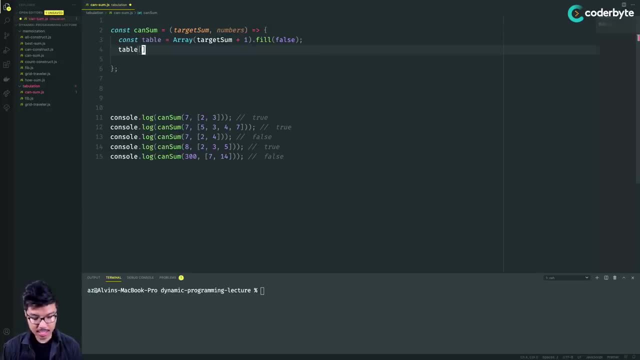 what's in the numbers array. So I'll just go ahead and say table at index zero is equal to true. So let's just console dot log what this table looks like so far And I'll just run, let's say, the second example here. So I should see my array of length beats up need. 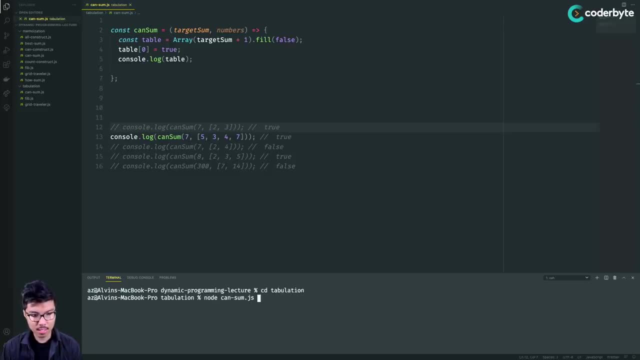 to go into this tabulation folder. Now we're going to run this guy, Cool. So that looks like a good table right. Eight elements, and I do have a true at index zero, Nice. So at this point. now I want to actually lay out the core algorithm by iterating through. 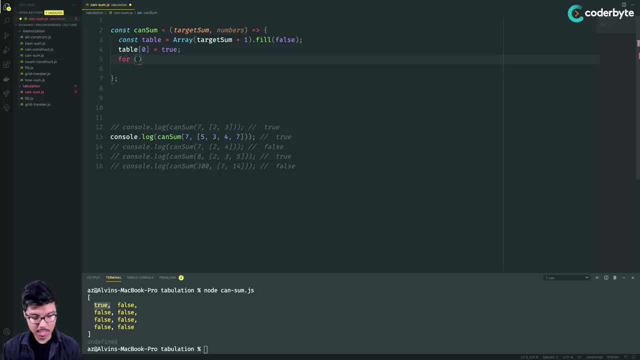 the table. So I'm gonna use a regular for loop here. Let's say: let's I equals zero, go up to. I can even include, if I wanted to, up to and including the table dot length. Yes, you could also say a target sum here, some thing based on target sum. 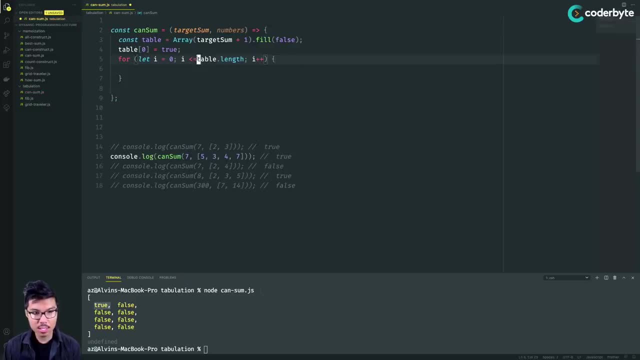 I'll do. I plus, plus. And here I'm going to choose to iterate using, you know, the manual index, because I know I have to do some arithmetic to look ahead in the array. But as I iterate through every element of the array, I want to actually check. 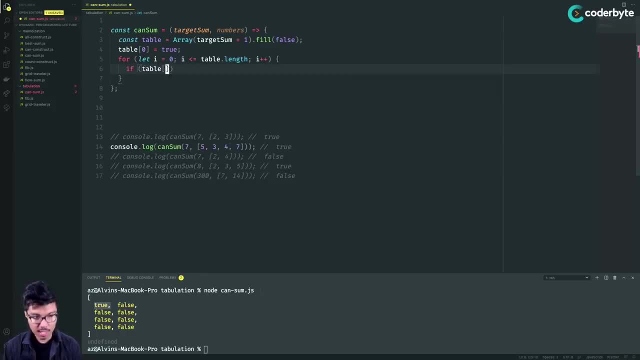 you know if this position is true, So I'll check. if table at index i is true, Cool, Because I know inside of this if statement I need to basically jump ahead or look ahead based on what's in my numbers array. But I only need to do that if my current position is. 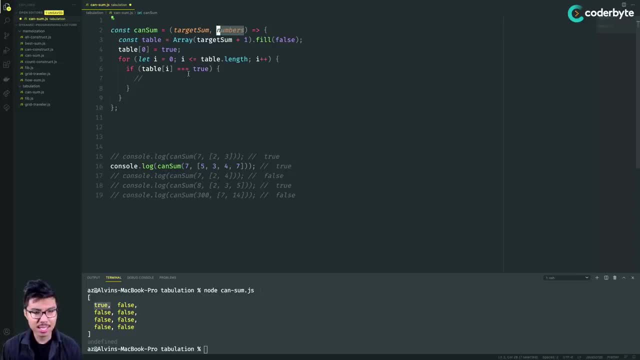 true, right, I only get to look ahead. if it's even possible to get to this current amount, right, the current amount I'm sort of tracing through it would be at index i. So, at this point inside of my if statement, what I want. 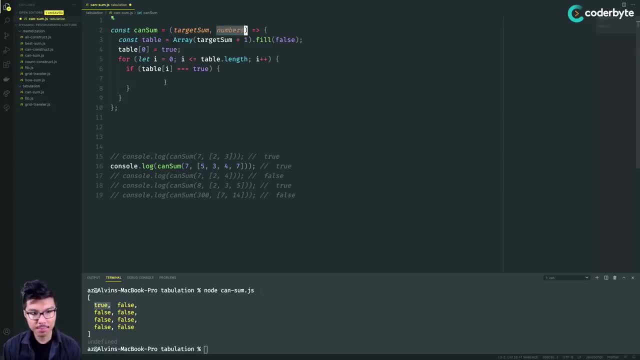 to do is now look ahead for each number of this array. So I'll nest a loop here And I just want to look at the elements of this array. So I'll say for let's say let num of numbers. So I'm grabbing each element this time, And now for this number element I want. 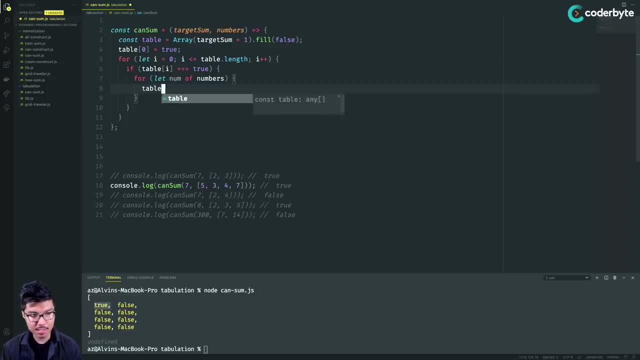 to look that many spaces ahead. So I want to look at basically table, at index i plus the number, Cool. So imagine that I'm on like the first iteration of this. I know I is going to be zero, So that's the very, very first index of my table And if my num is five then I'm 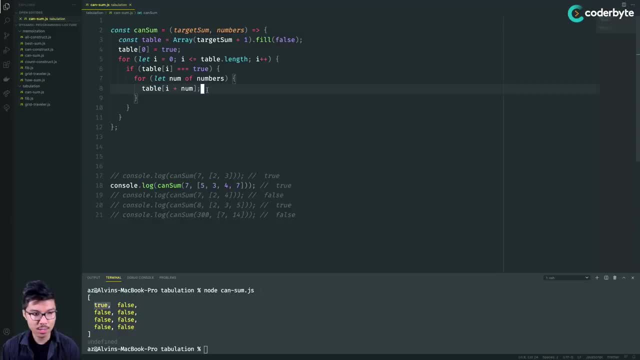 going to do zero plus five, looking five spaces ahead, right, just like we did in our trace. And for this position, that is like five spaces ahead, I want to assign it to be true, basically saying that, hey, if my current position is reachable and I can take a step of exactly, 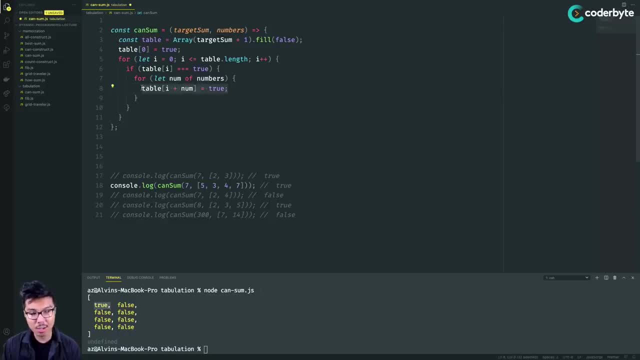 num, then that must mean position i plus num is also reachable right, And that entire for loop goes inside of this if statement. So I'm going to look at this first iteration of this array. So I want to look at this first iteration of this array And I'm going to 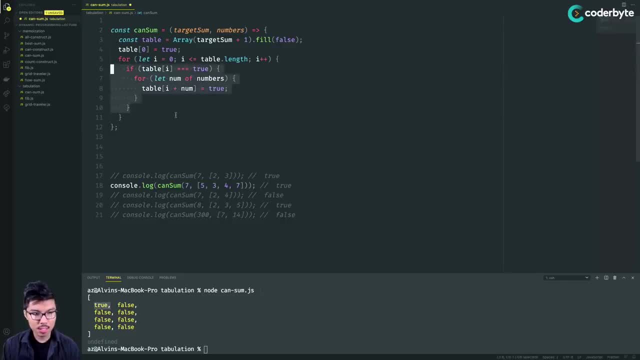 include my Curry statement right. So this code is looking pretty good So far. I think the last thing we need is just to return our final answer Afterward on entering through the table. So here I'll just return table at index targets. 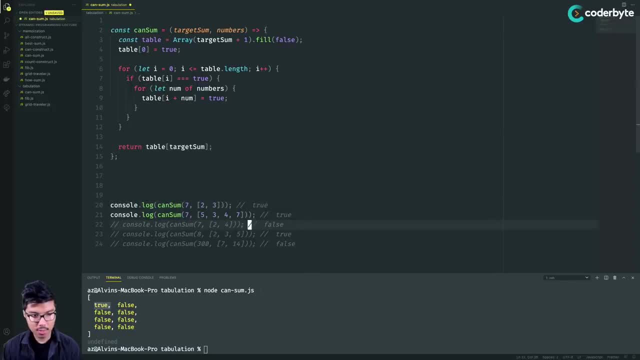 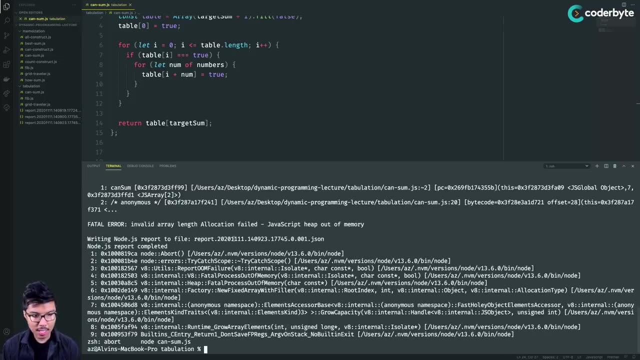 Cool, So let's- let's go ahead and run these examples. Maybe we'll have to debug some stuff. Looks like I have a- probably an infinite loop. Yeah, my program crashed with some massive, so let's debug this one together. There's something that I'm not considering in my code. 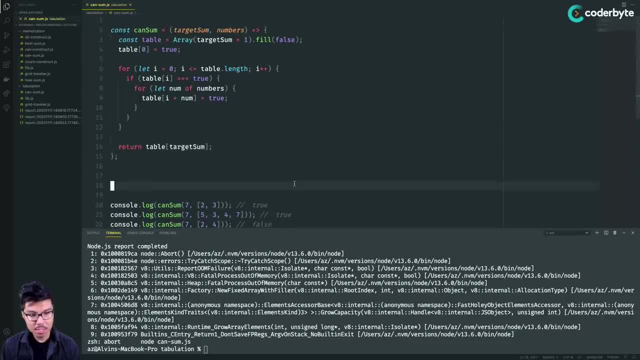 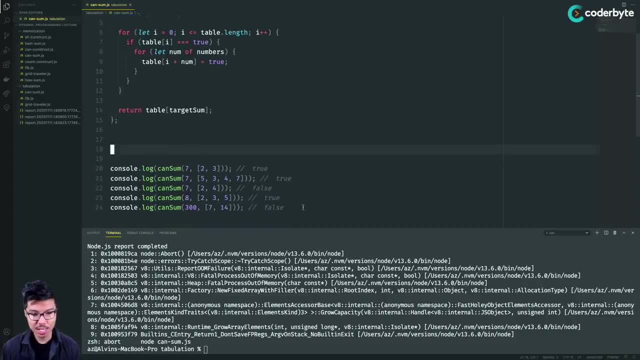 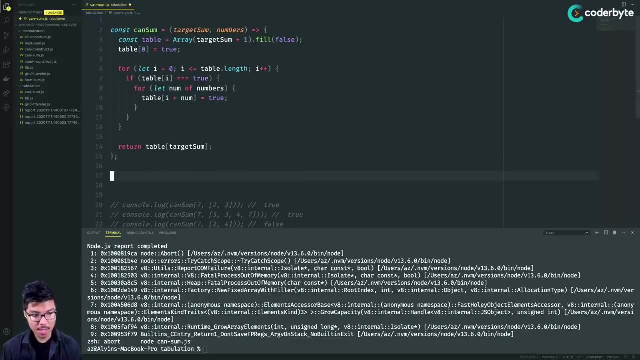 but we did consider when we drew it out. So something that is probably breaking right now is having to do with, like the balance checking. Something that's kind of unfortunate in JavaScript is this characteristic. this may have different behavior depending on the programming language that you're following along in, But I know in JavaScript, if I had 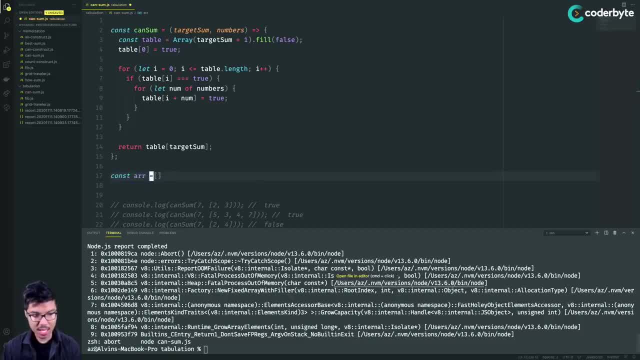 some array. let's say array and I set it equal to just a handful of elements. let's say A, B and C. If you actually do like array at some out of bounds index, like index- I don't know, 10, and I assign it like x. that will actually change like the effective. 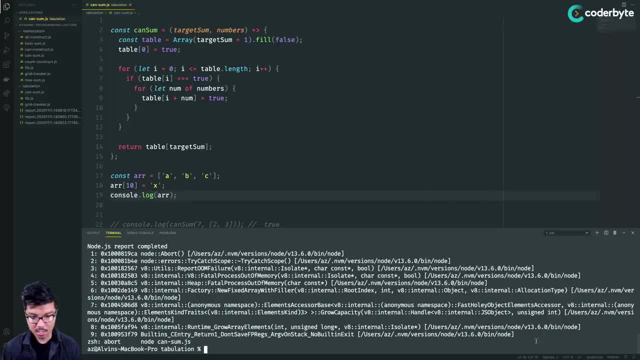 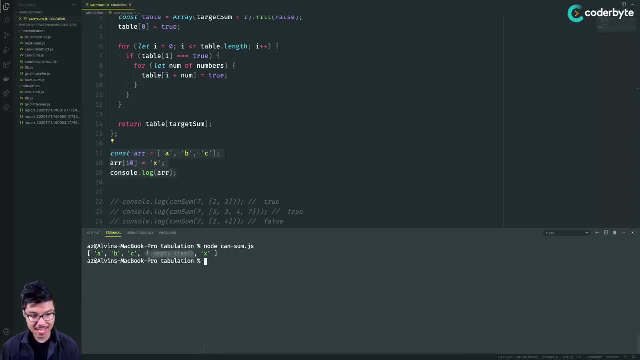 length of this array. So if I take a look at what happens here, so just running this kind of offhand example, when we run this notice that we have about seven empty items before we have the x. Basically when you do this type of weird assignment in JavaScript, 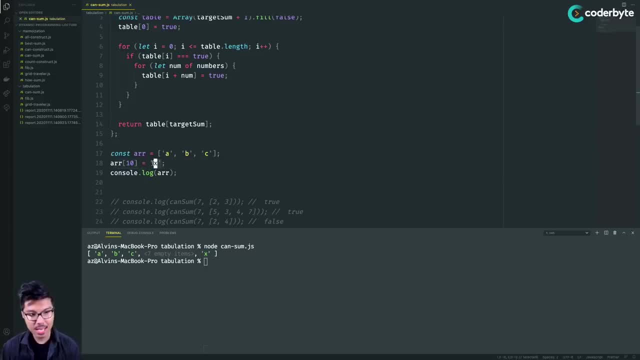 it's going to like lengthen your array that way and make sure that this Hey new element of x is placed at exactly index 10.. And so why is that relevant? Well, in my code here I don't really check if I'm out of bounds right, And I just assign to something that's potentially outside of. 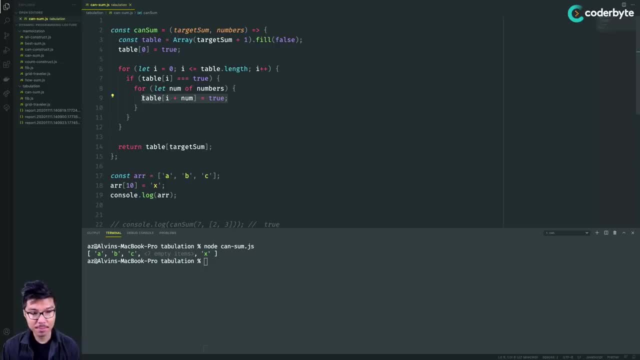 the current length of my array, of my table, rather. And if I do that, then this condition is a little suspicious, right? Because if I do this assignment on line nine to an out of bounds position, then the length will get longer And that's sort of like a circular. 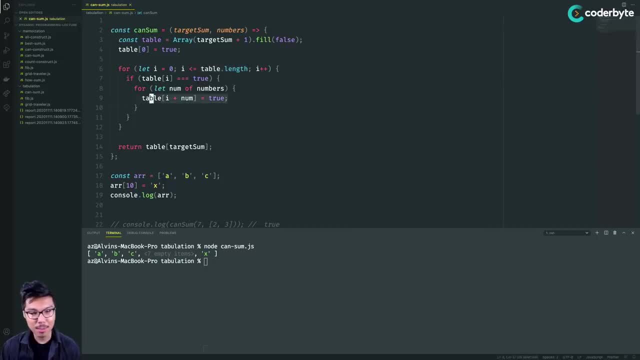 argument right, I keep iterating, only to make more stuff out of bounds, only to lengthen the table even more. So that's why I ended up with like an infinite loop over here. One way I can fix that is to just maybe limit this, So I won't make a table that length. 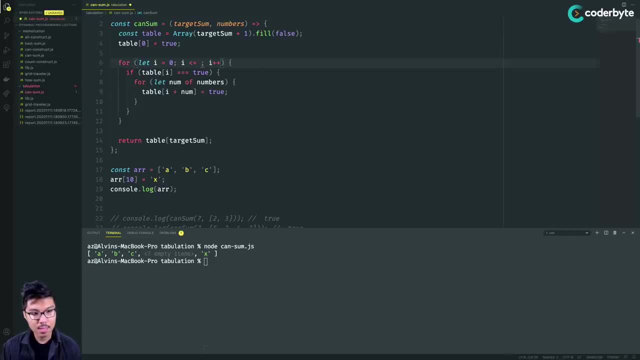 that's a little too dynamic. I know I can basically stop once I reach the target sum, So that might actually be the better move over here. Pretty, pretty fair bug, though. With that, let's go ahead and run this code again. Okay, so now we have a table that's out of bounds And we're going to go ahead and run this code again. Okay, so now we have a table that's out of bounds And we're going to go ahead and run this code again. So now we have double attributes of eight lists. Let's. make that into the class. So we're going to go ahead and run that up And then we're going to kind of pull out our properties of angels- g is g sets- And we're actually going to be able to create the third problem In here we have, let's say, a scheme, right? 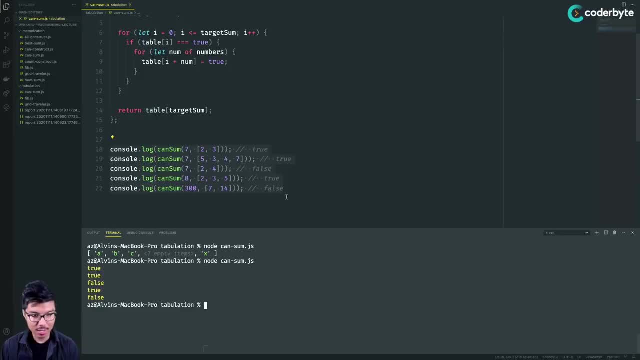 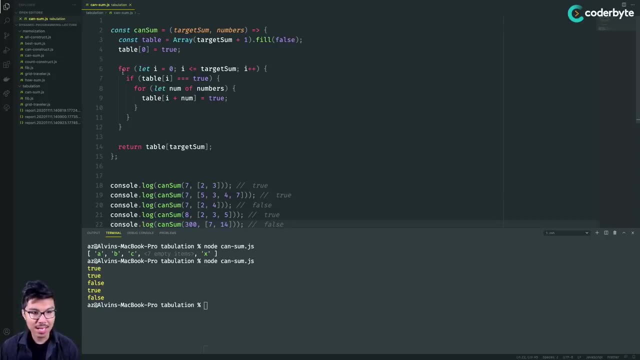 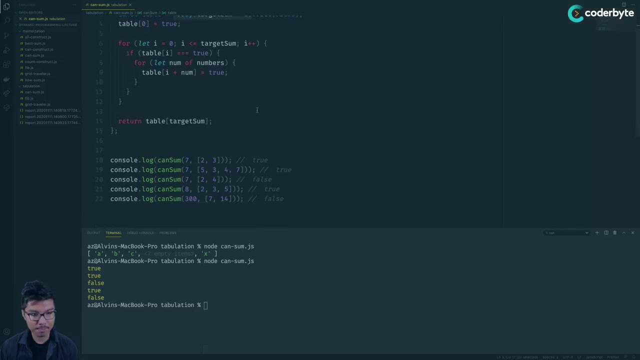 You can go ahead and create structure that decodes dual made issues with our dot deductions g sets. Now you can. how to do that is if we run available Specifications pad. But was that string is also running the shooting Azure and our means type didn't? 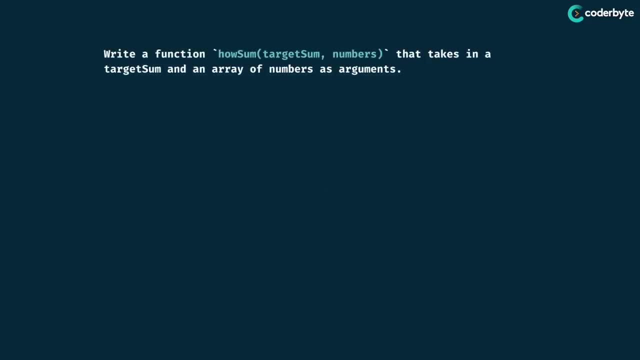 Alright, now let's work on the how, some variation of this problem. So, like before, I'm going to take in the target sum as well as an array of numbers, But this time around, what I want to do is return an array containing a combination of elements that actually adds up to the target. 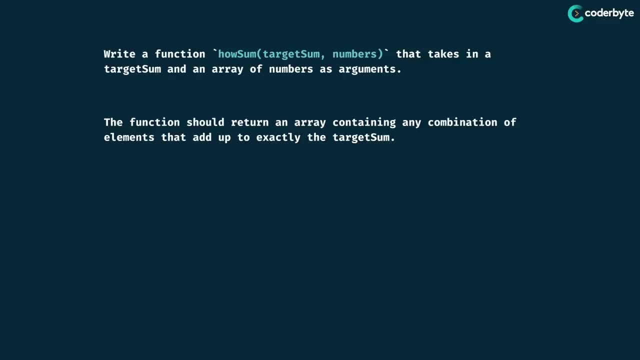 sum right. So here I want to return exactly one way, if it's possible. Along with that, let's say that it's actually not possible to return the target sum, then I should just return the null value, And if it's the case that there are actual multiple combinations, 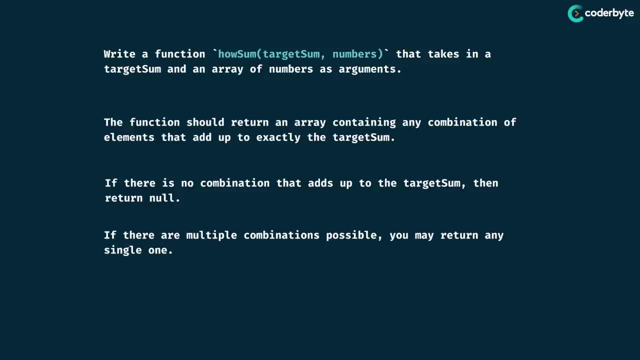 that can generate the target sum. I can return any one of those, So we expect the strategy for this one to be very similar to our last problem. However, we will need some nuance logic to return the array now, right, Because I don't want just Boolean data wants to return. 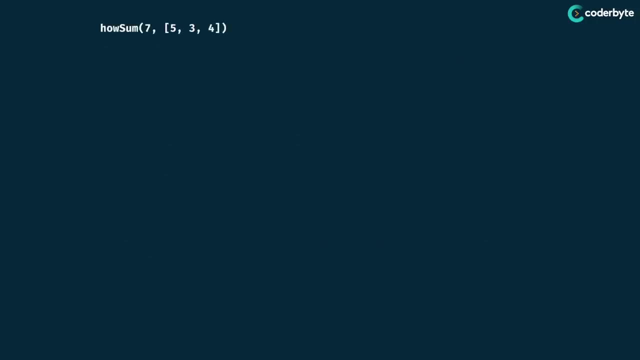 an array. So let's sketch this one out. Let's say I'm stepping through this example where my target is seven and my array is 534.. For this input, a reasonable answer to return would be an array of three comma four. right, Because I can add three plus four to get seven. 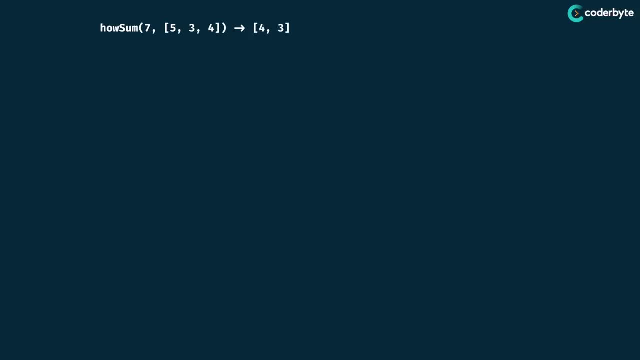 you can also, I guess, switch around the order of these elements. So if you also returned four comma three, I think that would also be a valid answer. Point being: I just want to return at least one way that can generate the target. So we: 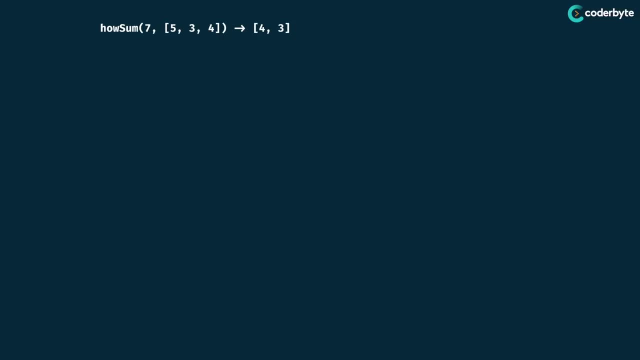 know we want to solve this one with tabulation, And so we'll just follow our recipe right? I need to construct and initialize some table, And we already know that the size of this table is going to be based on the target sum, So roughly seven elements. But we of course 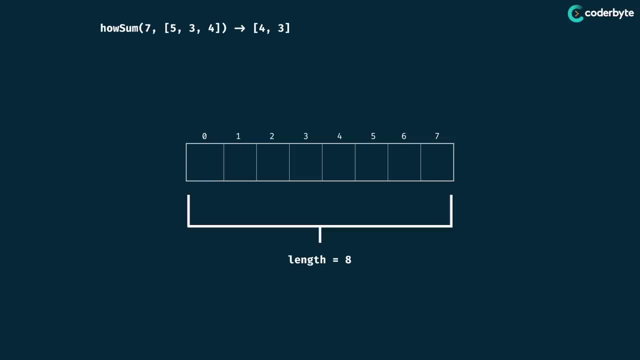 had that classic off by one nature, right, Because I want the last index of this table to align with the actual number argument. So I'm going to initialize this array with a length that is target sum plus one. Cool. So now that I have the correct shape of table, what do I actually have to initialize as elements? 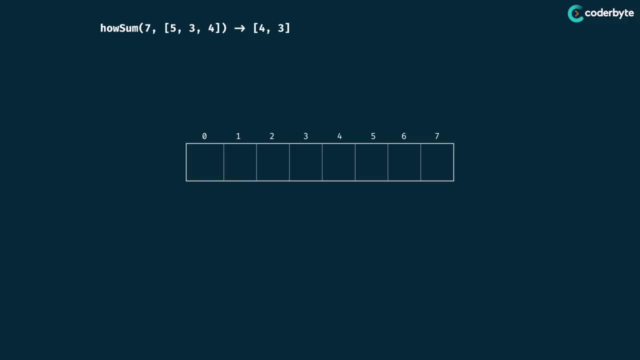 inside of this table. Previously, in like the Boolean version of this problem, we initialized everything as false, right And the reasoning there was. before we actually try all the possibilities, we're going to just assume that it's not possible to generate every quantity. 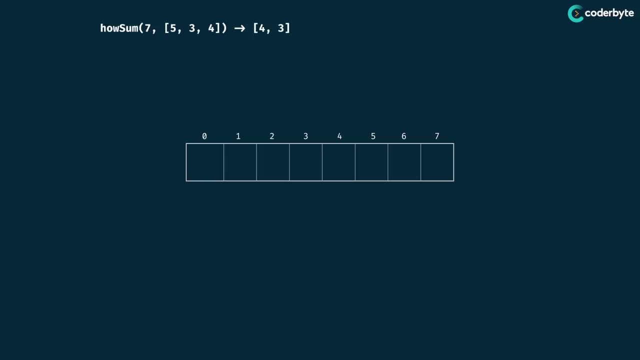 we just want to adapt that for this new type of problem. They tell us that if it's not possible to generate every quantity, we're going to have to initialize everything as well. So now that we have the correct shape of table, let's say we want to generate an. 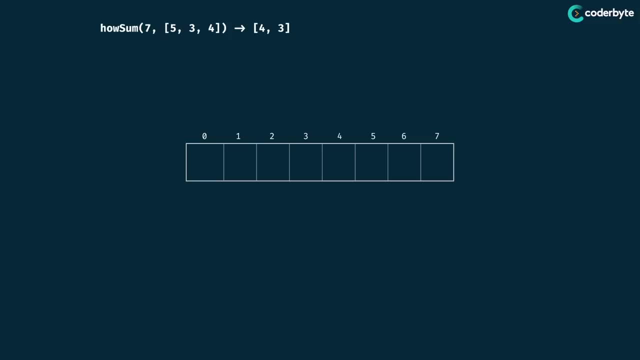 amount, then we should just return null. So I think null is actually a great initial value to just put everywhere in your table. So at the start we're going to assume that none of the values or none of the amounts are actually possible to be generated. No, 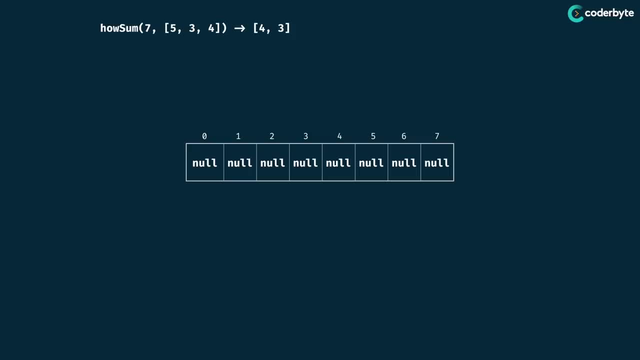 is sort of the analog for false in this rendition. Cool. So now that I have a most of the values added to the table, now I need to figure out what's the appropriate seed value is. I need some actual data to begin and get the ball rolling on this one. So, like we expect it's. 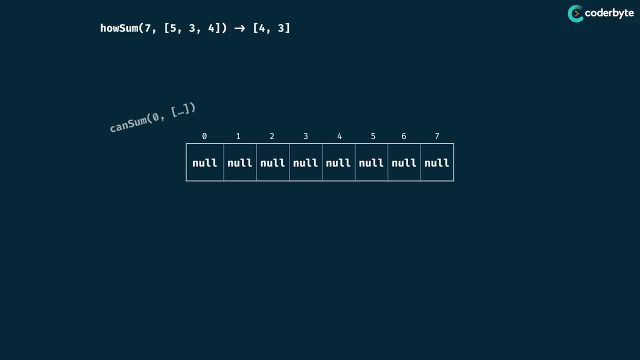 really so easy to figure out. So here's our argument for point D. you actually have to number the numbers And if you look at the bounds and you can see if you changes the value of the数 here it means that you're going to have an array that you're going to 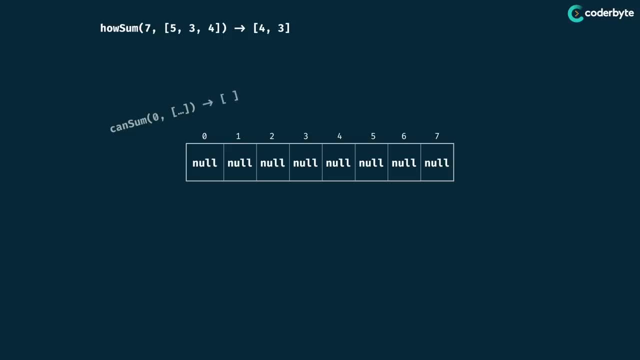 have only one of the values added or not. So we have the number one, zero, And then you have the number two, one, two, two and three, And so you have the number one one, two and three, And the number one one, two, two and three, And then your first. 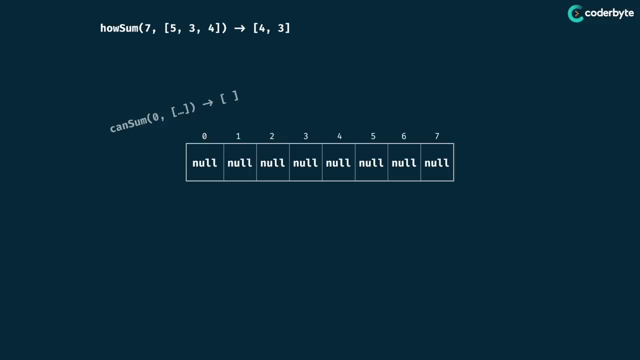 variable is going to have to be original And since the number one, one, one, two and three are the nice numbers, because these numbers are the number one, one, two, two, three and four. So basically, as a result, we want to interpret all the numbers in that. 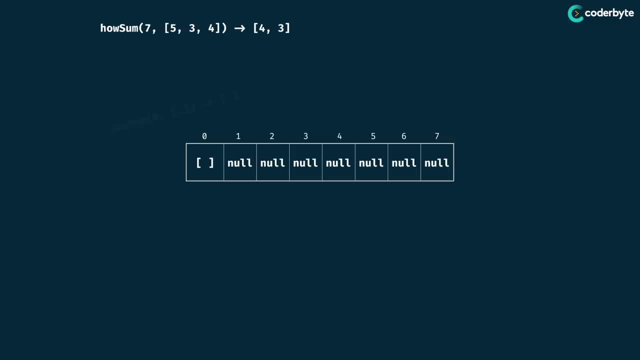 an empty array, And at this point what we want to do is, of course, iterate through our table and come up with some logic we can use to fill out further positions of the table based on our current position. So let's say, we begin at index zero. So here I am and 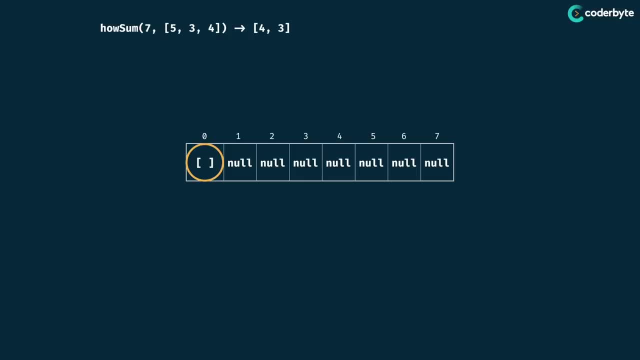 I have to figure out which further positions of the table should I be looking at. We've seen this pattern before. I should just base that off of what I have as options in my numbers array. So look at my first number of five. that means I could look exactly five spaces. 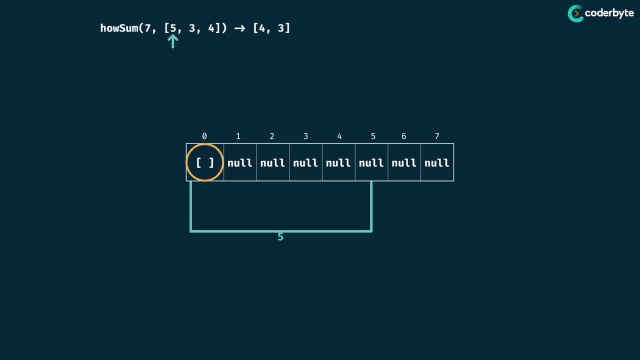 ahead in the table at this position, And so if I know that my current position is possible, I see that I have an array in my current position that I know it's possible. If this current position is possible, then a position exactly five steps later would also be possible, right. 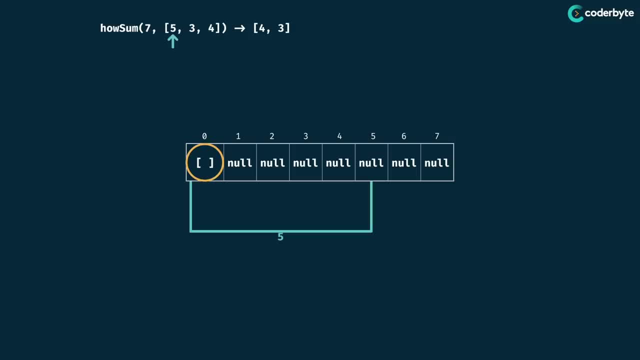 And so what I'll do is I'm just going to copy my current value into my further value. In other words, I'm going to put an empty array at position five, right. However, I also have to include the number that I'm using right now. right, I took a five to actually get to this position. 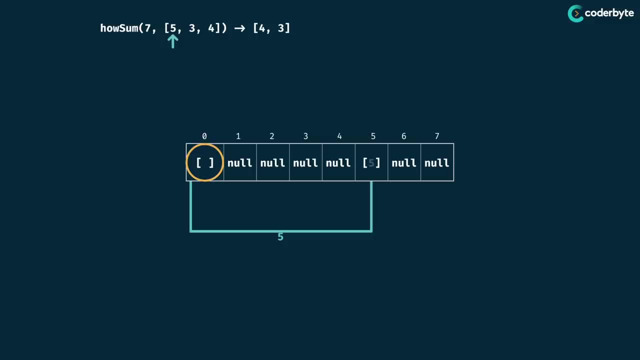 in the first place. So I'm also going to add a five into that array. Cool, If I do a quick spot check, this is a reasonable thing to do, Because if I look at the state of that index five, it contains an array of five, meaning that, hey, you can return a sum of. 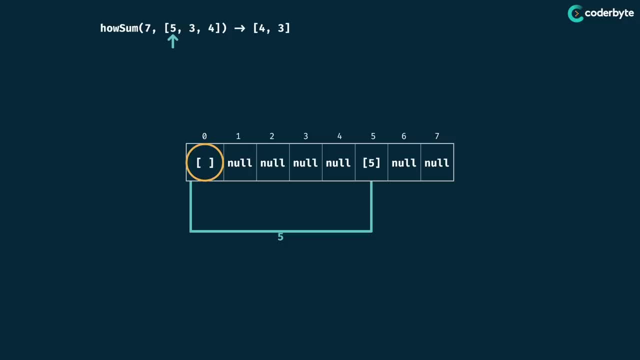 five by just taking a single five, And with this I want to do the same logic for the other numbers of the numbers array, right? So if I have the three, I'll look three positions ahead of my current place And I'll also start by copying over the array at my current position. So I copy. 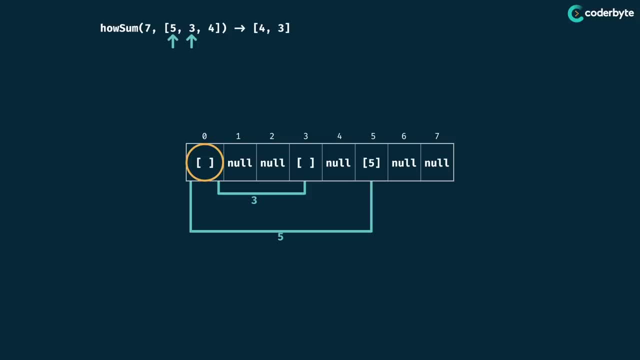 over the empty array And after I copy that array I actually want to populate it with the number that I took to get to the spot in the first place. So I just go ahead and put a three in that array And the same thing happens for the four. So if you go to the 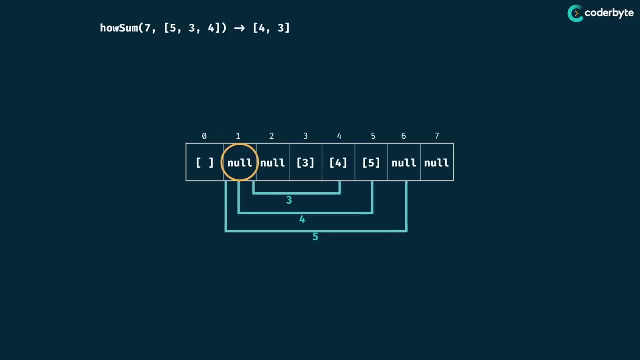 next iteration, we see that our current element is null. That means that the amount right, in other words our index amount, is actually not possible. It's not possible to get to the spot. It's not reachable, meaning we can't get an amount of one by adding up any. 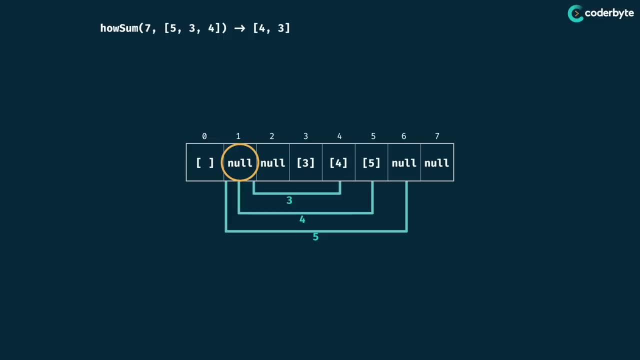 numbers of the given array. So what I should not do is actually manipulate any further values from this position. So I just continue these base iterations. Same thing happens when I'm at index two, But things get more interesting when I'm at index three. right, 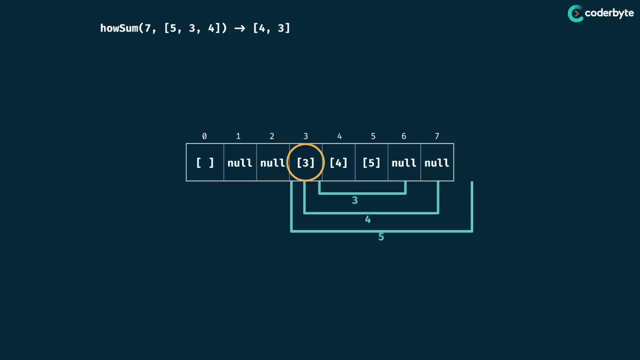 I see that the element here is not no, So it is possible to generate three, And so what I want to do is go ahead and look at my, my forward values and sort of copy my current number, And then I'm going to copy that number And then I'm going to go ahead and put it. 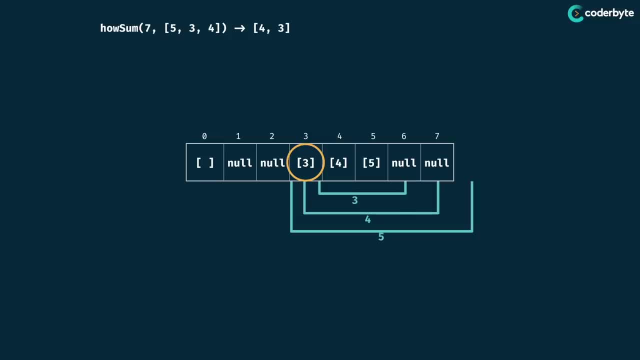 into my current position. And then I'm going to go ahead and put it into my current position, my current array over. So I know I don't need to look five spaces ahead because that would be out of bounds. So I'm going to look at the position exactly three spaces ahead in. 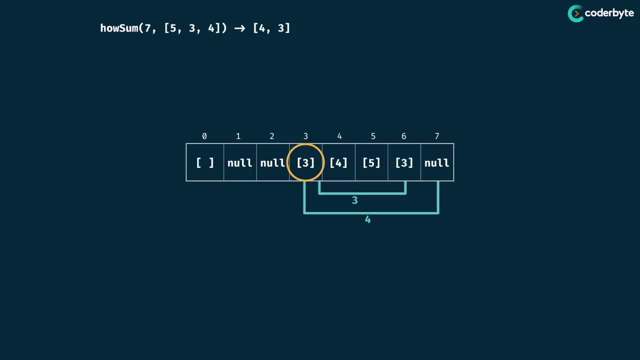 the table and copy over my current array like this. What I also need to do is make sure that I include the number that I'm using right now, which is three right, because I'm looking three spaces ahead. So I end up with three comma three at index six of my table, which 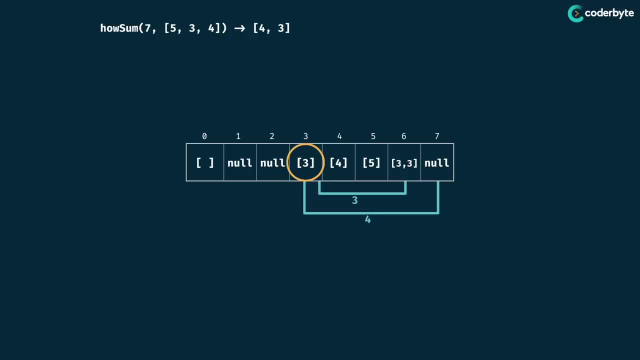 is reasonable, right? I also want to do something very similar for the position four spaces ahead. So I'm going to copy over my current array but then also include the four that I'm using up right now. So now I have three, four over here. Cool, At this point you can. 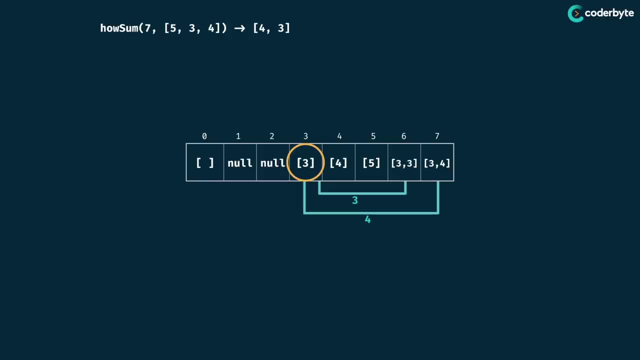 kind of see where this is heading right. I've actually already populated index seven of my table, And three comma four is exactly a one way we could create the seven. So we could stop here. However, let's say that you continued the algorithm, So in the next iteration, 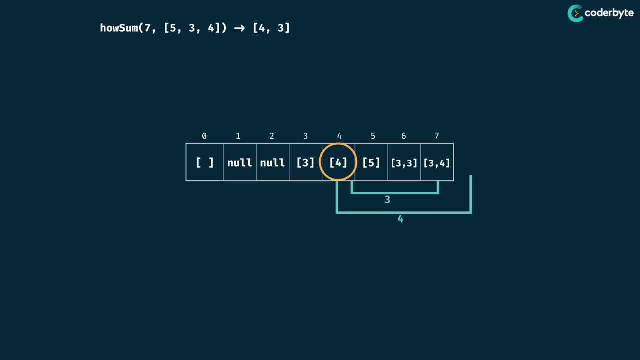 I know that this space for indices ahead would be out of bounds, So I don't need to look there, But according to our general logic, I would actually manipulate the spot of the table. three moves ahead, right, And so what I'll do is if I, you know, follow the same exact. 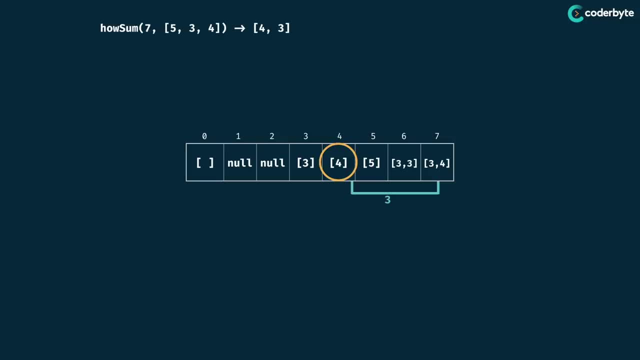 logic or I'm being consistent. I'm not really changing any of the rules here. I would copy over my current array into that position. So I basically overwrite index seven with just an array of four. But then at this point I would also be sure to include the number. 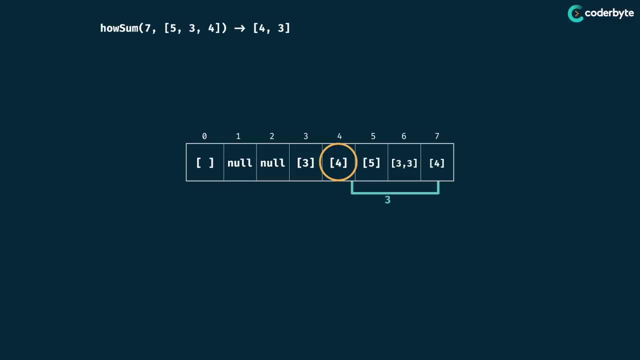 that I'm using right now, which is three, right, because I'm looking three spaces ahead. So I end up with four comma three, Three, which happens to be like another way I can generate these seven. So it doesn't matter if you actually continued this algorithm, Right? So if I continued, I would basically 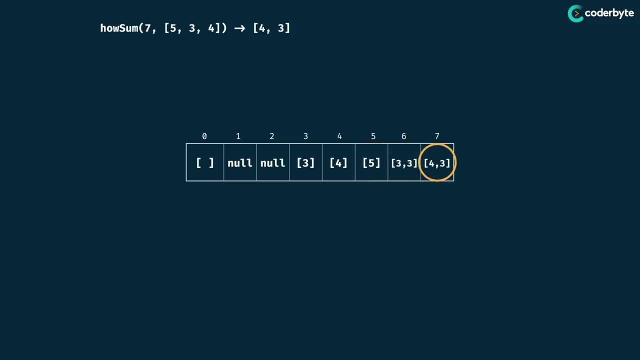 just keep iterating until I hit the very end. And what do I know? the element at index seven is exactly an array of 43. Cool. So the point is you actually don't have to like exit early As you iterate through the table. you'll be okay to just finish all of your iterations. 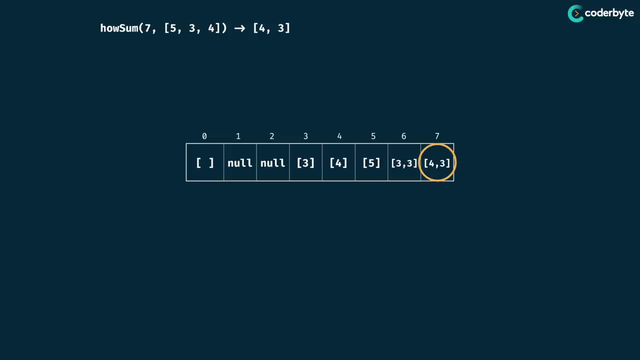 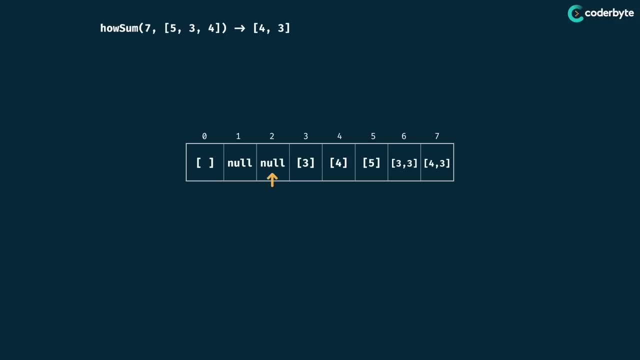 now I just go back here And if I look at my table, I don't see this. this is the number of numbers I have, And so if I look at my table, I don't see that number, which is zero. I look at index two: there's a null, meaning that it's not possible to make a two by using 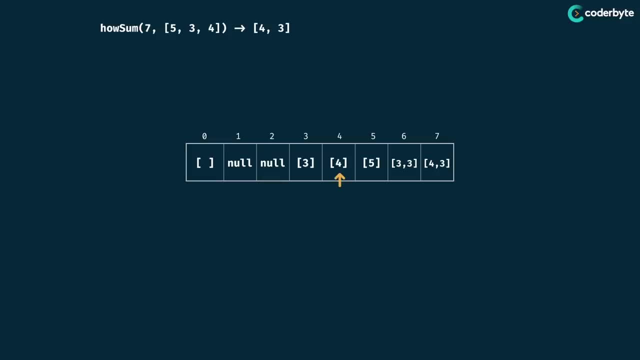 elements of the array. In a similar way, if I look at index four, there's a sub array of four, meaning you can just take one for to make a sum of four. Similarly, you can take two, threes to make a sum of six And, of course, you can make a seven by doing four. 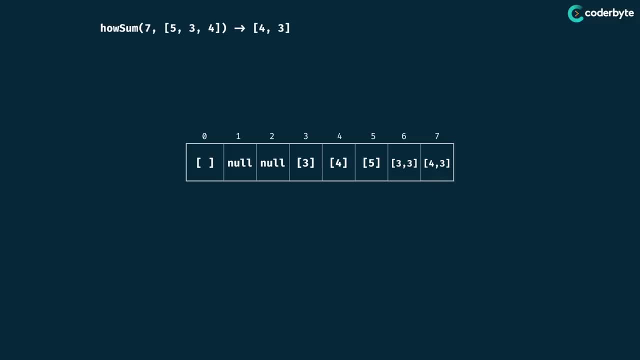 and three. So now that we have a plan of attack, let's look at the complexity for this. So of course, the M will represent the target sum and our n will represent the length of the numbers array. So if we begin with just the time complexity, we know that we're going. 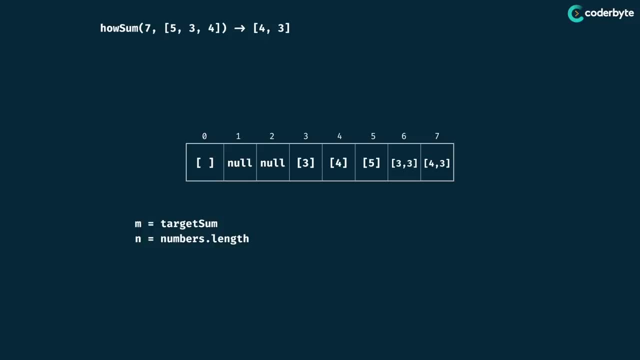 to at least iterate through the table and the tables of size m right, So I have at least an M in my time complexity. But for every space in the table or in every iteration of that loop, I need to also iterate through all of the numbers in my number input array. 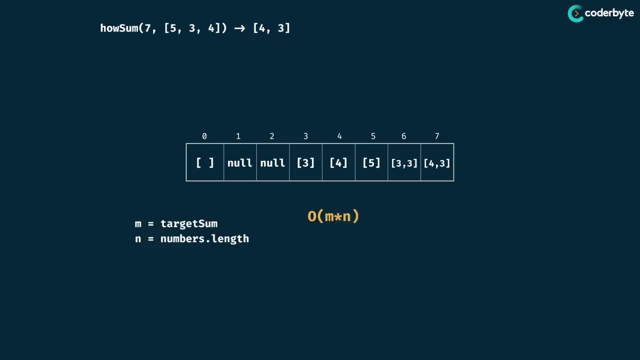 And so I can multiply by n over here, Nice, But at this point now let's say that I actually need to take a valid step here. Then what I also did was copy over the array at my current position into that forward looking position, And I know that a sub array will be at most of length. m right, Remember that. 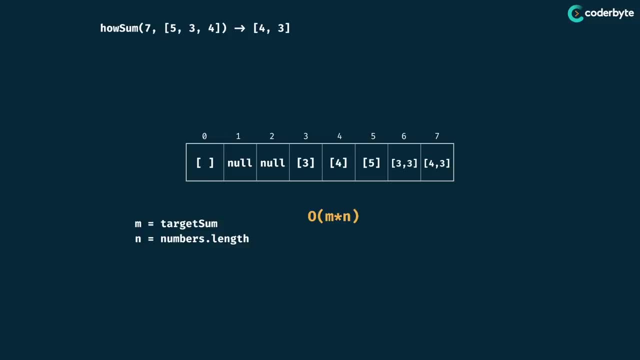 m is our target amount. the worst possible or largest way we can generate the target sum would be to have an array of exactly m ones right, And so we'll say that in the worst case we have to copy over an array of an additional length m. So that means our 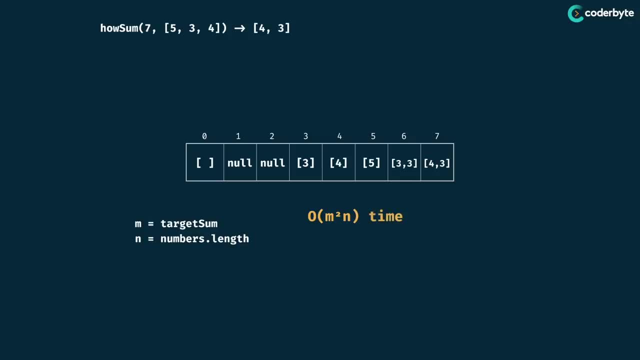 time is really m squared times n. Now let's come up with the sum of the numbers array. So thank you, guys for supporting me today And we'll see you in the next video. And if you enjoyed this video, feel free to leave a comment down below And, of course, make. 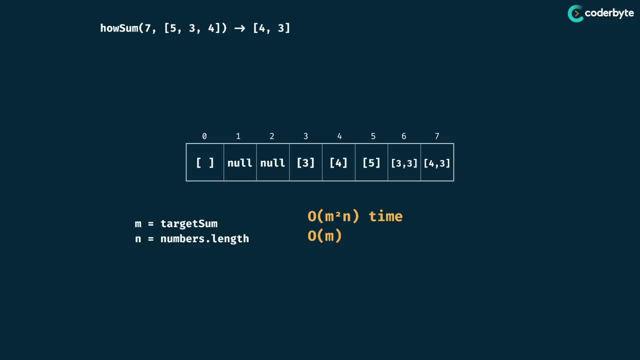 sure to subscribe to the channel so that you can never miss out on anything new. Thanks again for watching. If you have any questions, please do not hesitate to ask them in the comments, And then I'll see you in the next one. Bye. 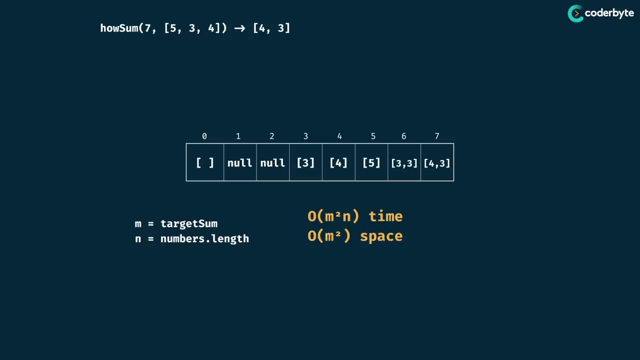 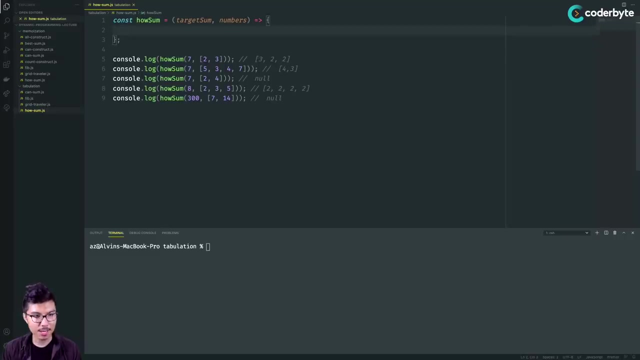 Bye in a reasonable amount of time. All right, I think we're ready to hop into the code for this one. All right, programmers, back in my trusty editor. let's go ahead and tabulate this one out. So we'll need to create the table to begin right. So I'll create my table. 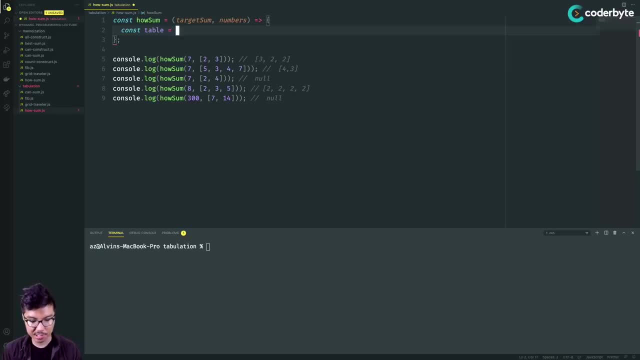 and it should have roughly target some positions in it. really, I need to increase it by one. So I'll say array and I'll pass in target some plus one. that way the final index aligns. I'm going to go ahead and fill this table up with all of those nulls, right, exactly? 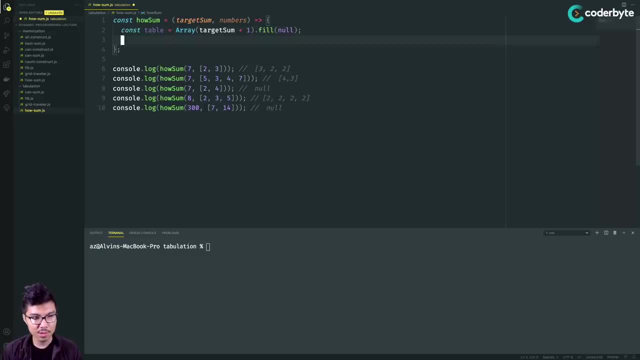 what we did in our drawing. What I also need to be sure to do is make sure we populate index zero of our table, with an empty array serves as sort of like a base case, in that we know that the target sum of zero can always be generated. right, You can generate the. 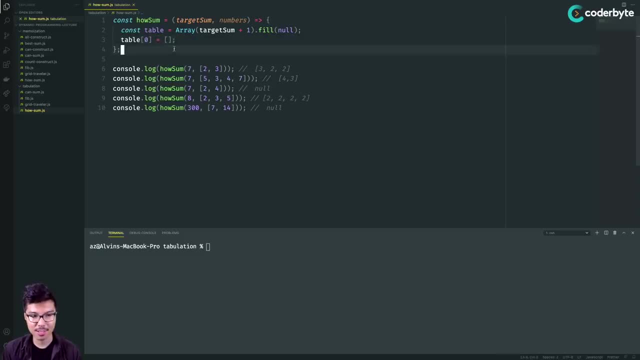 target sum of zero by taking no elements from the numbers array. right, If you took the sum of this array, it would be zero. Nice, This point we need to iterate through our table. So we've seen this code before. Equals zero. 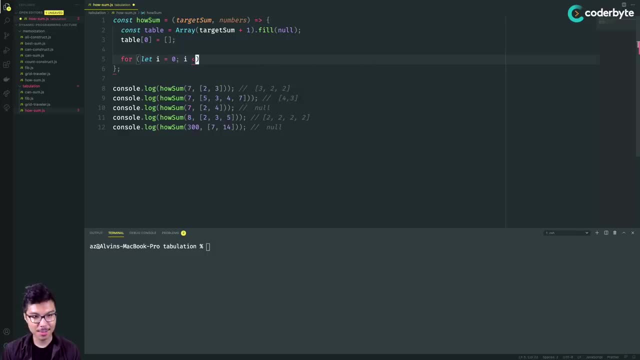 Go up to- and I won't mess this up This time- I'll go up to and including target some I'll do I plus plus. So so far very similar in shape to our last problem. Now that I'm iterating through every element of the table, I need to add some conditional logic, If you remember. 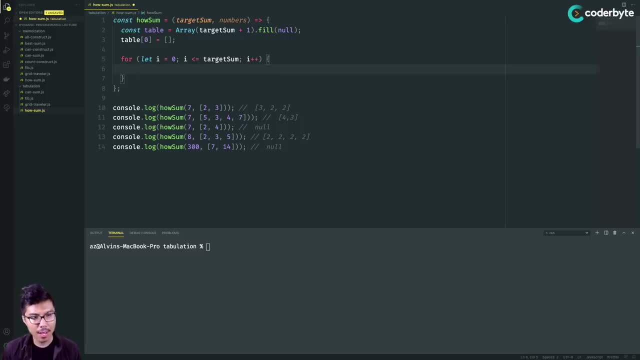 from my drawing. we only did, like the heavy logic, when our current position was not null, right, Because if it is null and you can't even reach this current position in the first place, So I'm going to check, hey, if my current amount is attainable. 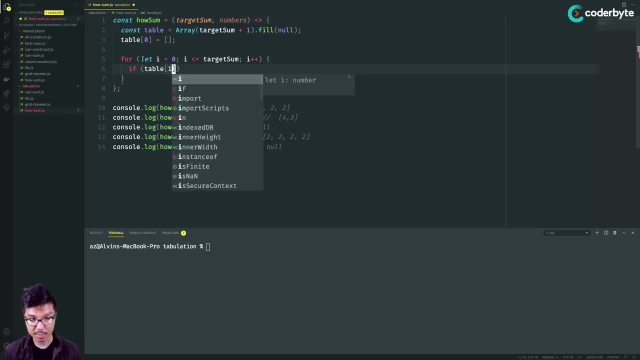 In other words, if table at index i, which is my current amount, if that is not no, if it's not no, then I can generate amount i Cool. So if I can generate amounts I, then I know some other things could also be generated. That is, I want to look forward in my table. 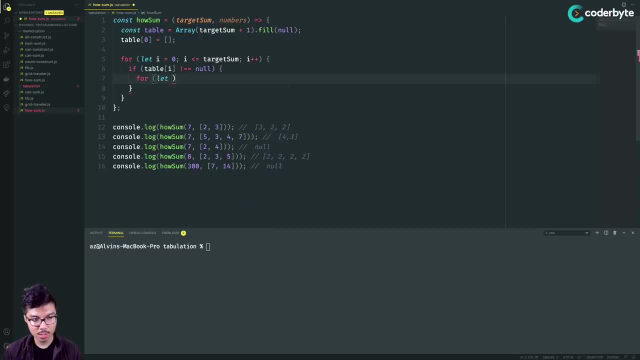 for every number in the numbers array. So I'll say let num of numbers. So I'm getting the elements of the numbers array And I need to look at that Number of positions ahead, right? So if I'm at i right now, that means that a forward. 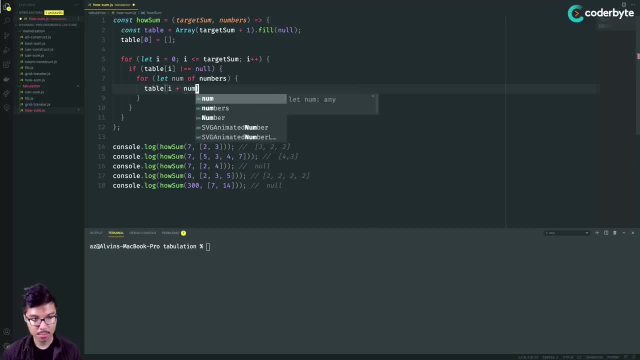 looking position would be at table i plus num. Cool, And I need to assign something over here. So I'm going to do is start by copying over the sub array at position i at my current position. right, I know that if table i is not no, then the only possibility 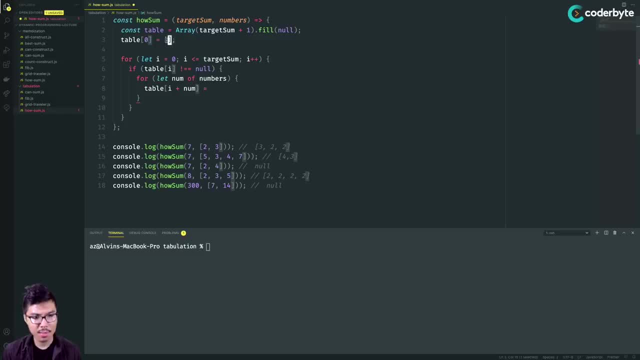 that it could be is an array, right? It could be array of zero elements, or it can be an array of many elements. No matter what that array looks like, I'm just going to copy over that array. So I'm going to spread out all of the elements of table i And so far, like this logic is looking, 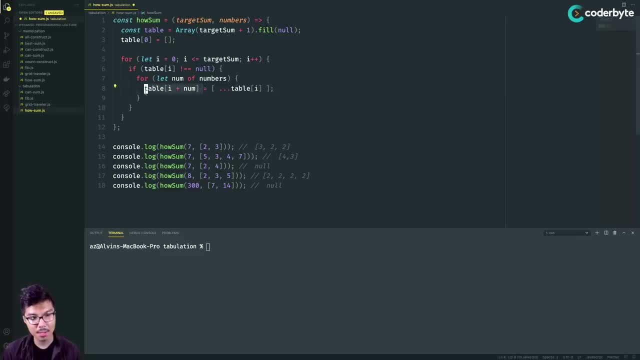 pretty good, because I'm basing my assignment on table i plus num off of table i. right, But in addition to that, I also need to include this choice of num, So I'm just going to add that into this new array as well, using some syntax that we've seen previously in the course. 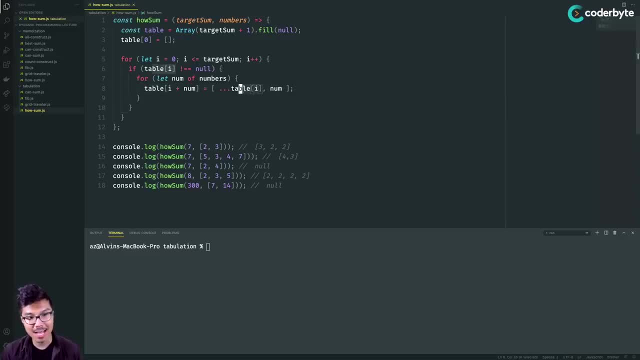 right. So I'm just copying over all of the elements of the sub array at table i And adding on, in addition to that, my current number Nice. So this code is looking pretty good. I think at this point all we need to do is let all these iterations finish and 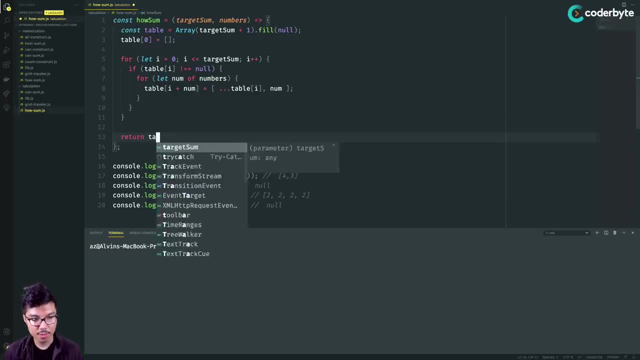 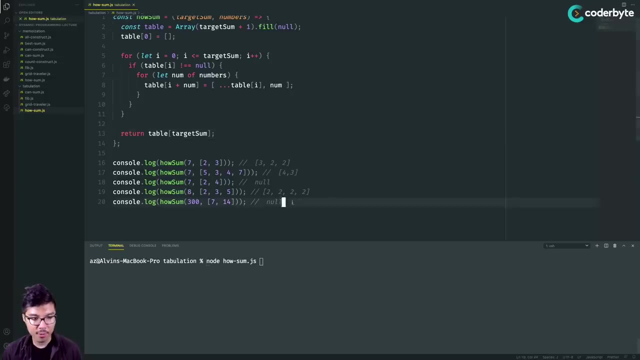 then wrap up by returning the last entry of the table, or really the table at index target. some cool, so not that much different from our last piece of code. Let's give this a shot. So I'll run how some, and here I have a few diverse examples, written Notice, that's. 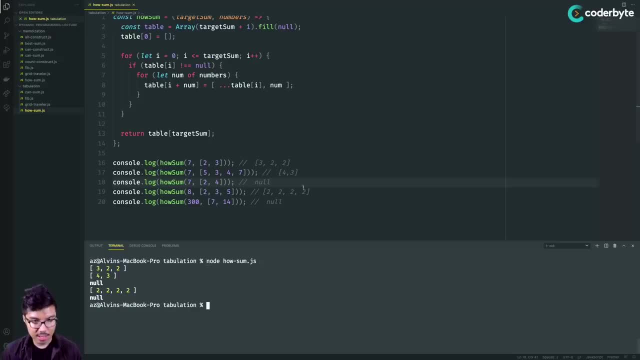 some of them should return. no, because they're not possible. If we check these- 3243, no bunch of twos and another no nice- it looks like this code is totally working. Notice that we already have a very efficient algorithm, kind of off the bat, kind of comes free with. 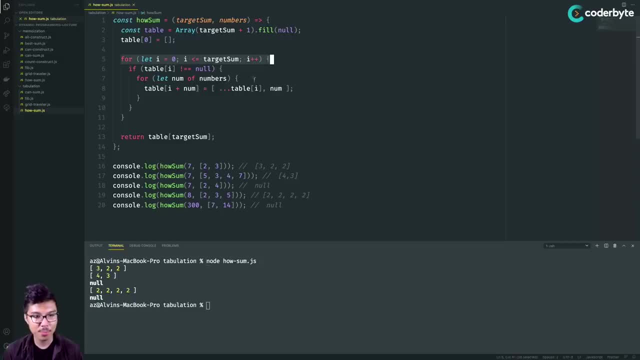 tabulation. we definitely have m iterations in this for loop. we have n iterations on the inner loop. But then we also have to consider this copying over logic right. copying over an array will be at most m, So it's m times n times m, which means that we're going to 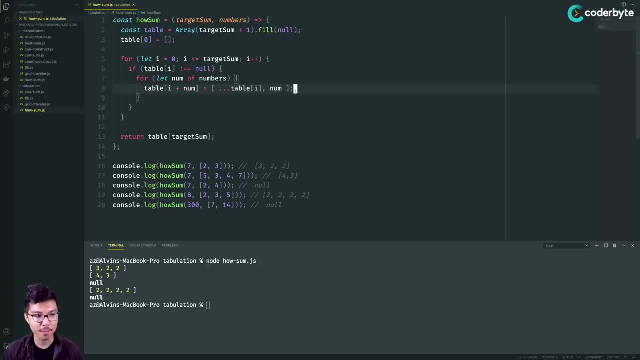 have m times n times m, which is just m squared n, exactly how we spoke about it before. Something I really want to emphasize is: you know, in isolation, if someone just asked you to solve like this how some problem, I don't think it's an easy problem. However, it probably 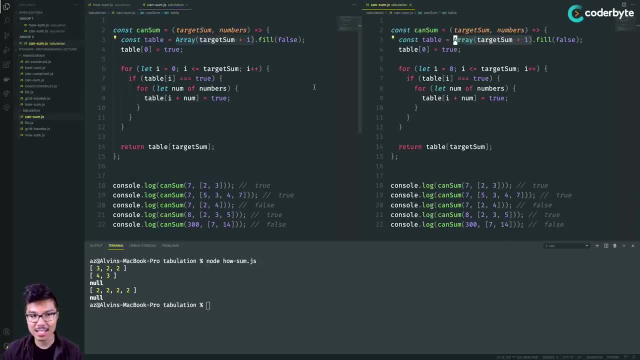 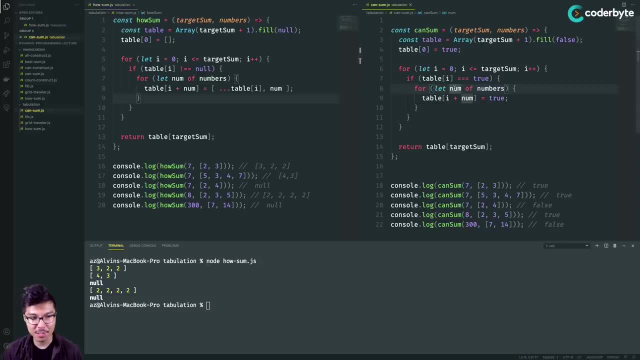 feels almost trivial, especially since we just did a cancer right. there's a really really straightforward progression to these problems. If you compare the how some and can some functions, they're very, very similar, right, really just changing the type that. 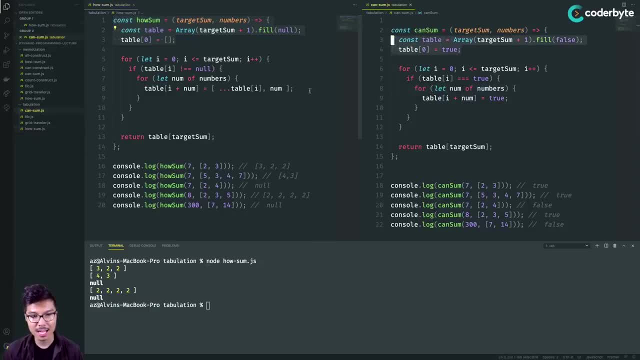 we store inside of our table, as well as The assignment that we do when we transition into our further elements of that table, really just adjusting that logic for the data type that they're asking us for, right, I had like some array answers here And here I have some Boolean answers. Alright, so we're smashing. 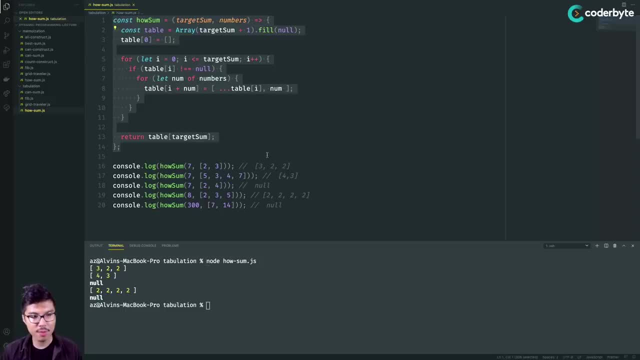 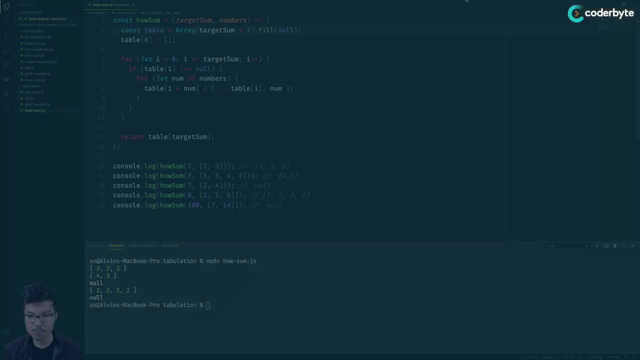 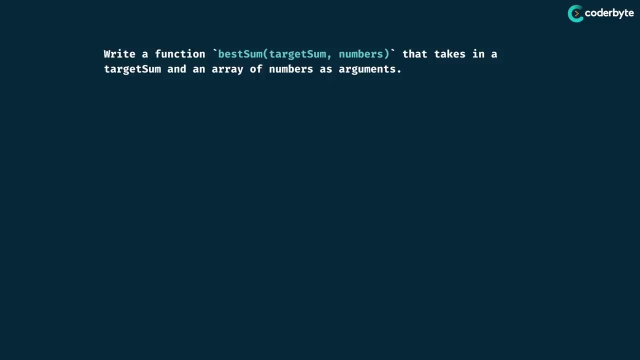 through all of these tabulation exercises. Let's do one more variation of this target some problem. That way we'll have a little bit of an increase in the difficulty. It's time to read. Let's revisit the best some problem. So we're going to take in again the target some as. 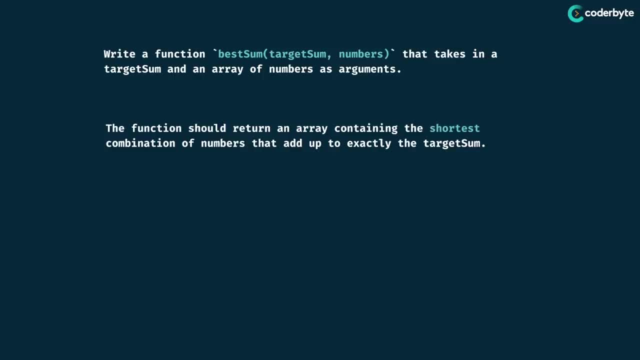 well as an array of numbers. This time, what we want to do is return an array containing the shortest combination that adds up to the target some, And if we have any ties for the shortest combination, we can return any one of those shortest. So you take a look at an. 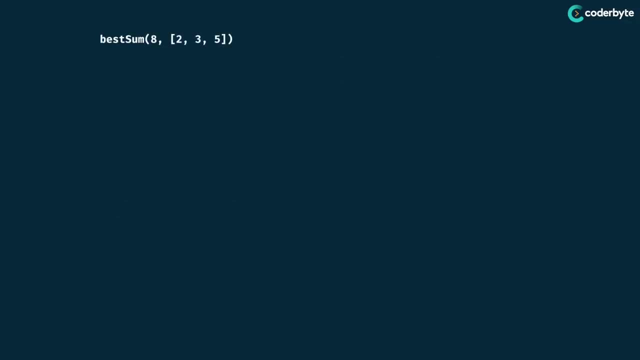 example, what kind of like we did before. if we have eight and an array of 235, there are a few different combinations that can yield eight. right, I can do two plus two plus two plus two, or I can do two plus three plus three, or I can do three plus five, And then 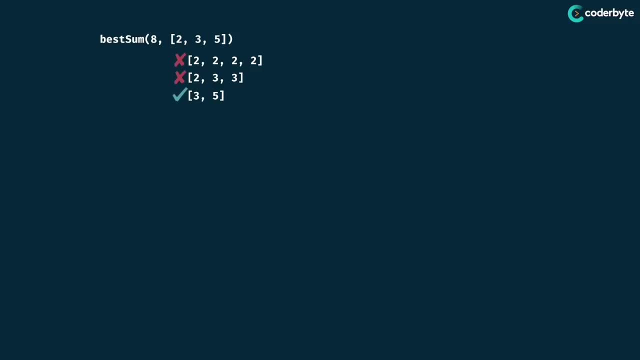 I can do three plus five, And among these options, the shortest one is obviously the three plus five, So that should be the return value over here. Obviously, if you returned five comma three, that would also be a valid answer. Nice, So let's start tackling this. 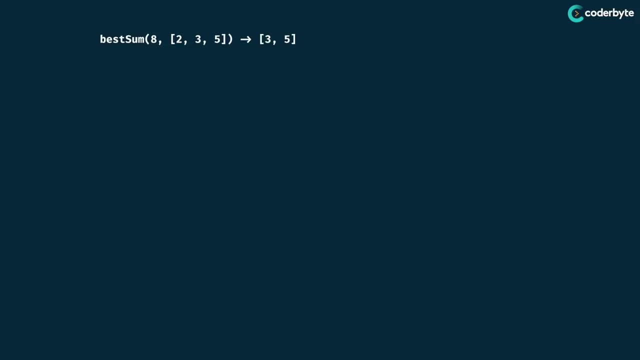 with our classic tabulation recipe. So we need to decide on the size of our table. Like we usually say, it's going to be based on the target sum and not so much the length of the numbers array And, like we've been saying recently, it would be nice if the last index 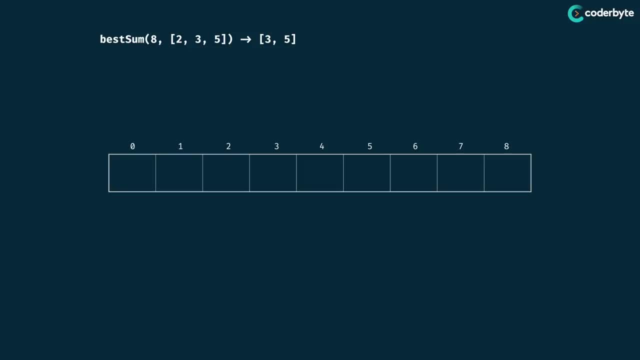 of the table aligns with the original target. So although the last index of this table is eight, that does mean that its length would be nine. right, Let's start by seeding the proper values here. I always want to begin my my value seed with the type that's kind of relevant to this problem, In other words, 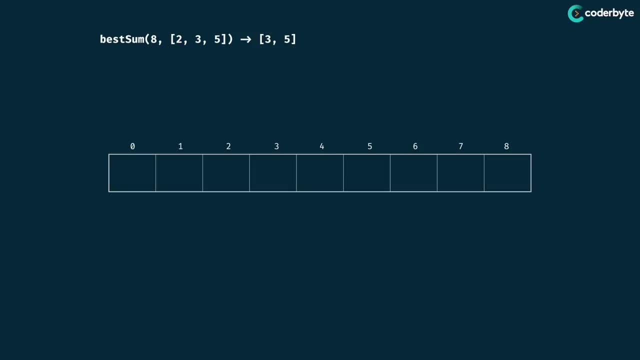 they want us to always return an array if there is at least one valid way to generate the sum, And I know that trivially. if I wanted to calculate the best sum for zero, no matter what array of numbers I'm given the answer: there is always an empty array. So I'm going. 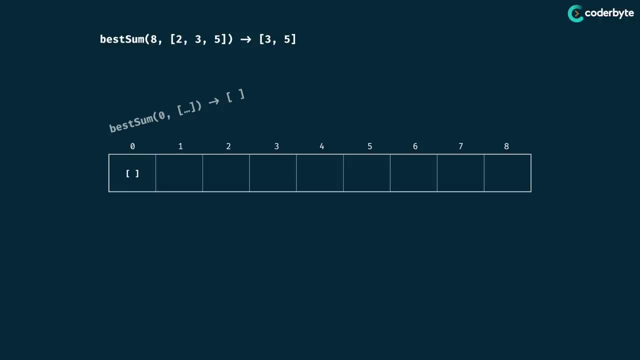 to store that value at index zero of my table. And now for the rest of the values in the array. I can't be sure if I can generate them yet, So I'm going to initialize them as null, just like our last problem. At this point we can begin our general algorithm by iterating. 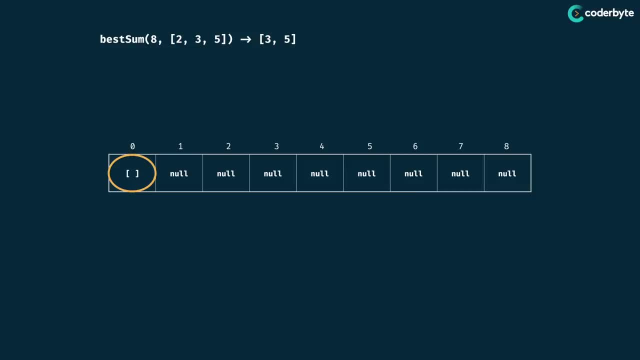 through the table. So what I'll do now is look ahead from my current position based on the numbers of the numbers array. So I'm going to look two spaces ahead. Right now I see that there's a null inside of that position, which means I haven't quite found a way to. 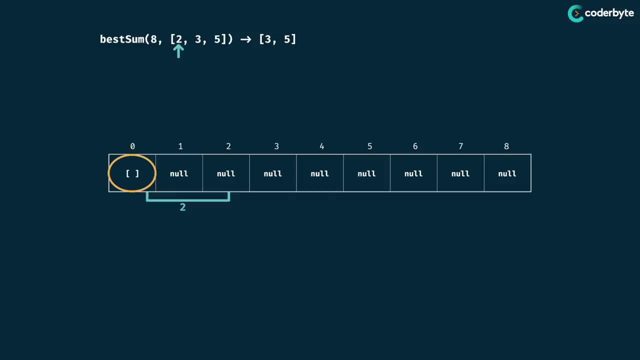 create two. So I'm actually finding a way right now. right, I can copy over the array from my current position, But I also need to populate it with how far I'm looking ahead by. so just a two inside And do this for the other numbers of the numbers array, So something similar. 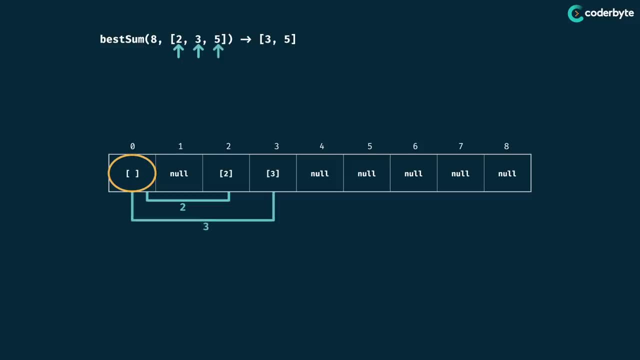 happens for three as well as for the five. Notice that since I just began the algorithm, this is a really the first time I'm finding any solution for these further values, And so let's keep these iterations going. I'm going to shift my frame of reference by one. 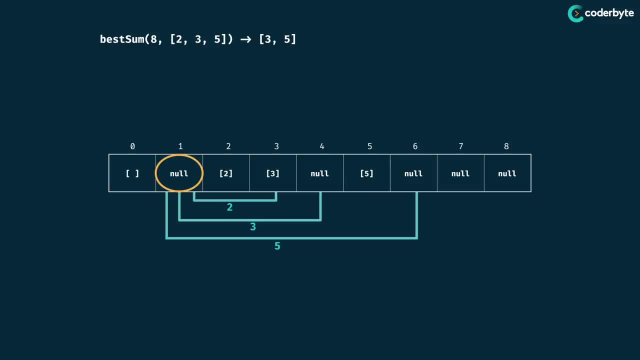 So this is the same model that kind of entails that one is unreachable. right, I have no way to generate a sum of one, so I actually don't do any logic from this current position. So we move ahead to two. Since I do have a non null value, I have an array over here. 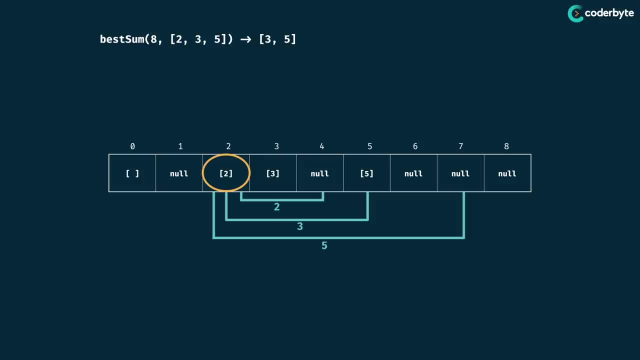 That means I should look ahead to my future values. So I start by looking two spaces ahead. I see that at index four there's a null, which means that I actually need to replace that. now, right, I'm going to copy over my current array, But then I also add the value. 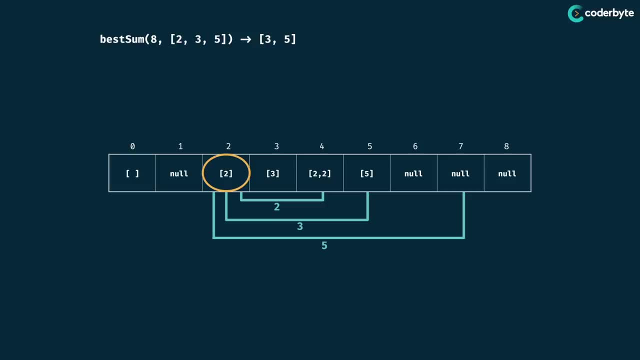 for how far I'm looking ahead by. So now I have two comma two inside of that index of four. So now I look ahead three spaces, which means I'm analyzing index five. I'll notice that index five already has an array there And if I actually continue my sort of standard, 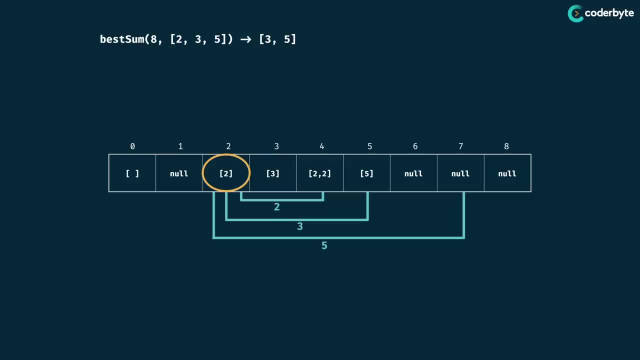 process. I would consider this array, I would copy over my current terrain, yellow, which is an array of two. then I would also add the element I'm looking ahead by, which is three, And technically, two comma three is one of the ways I can generate five, but it's. 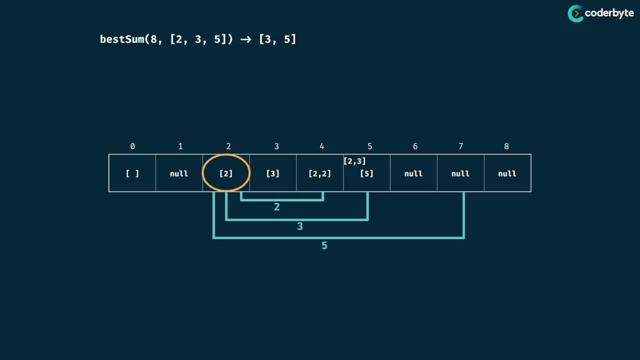 definitely not the shortest way, right? I can basically compare the length of these arrays And notice that the original array of just five is definitely shorter, So that one should get to stay in this spot. Cool, I'll do something similar for five spaces. 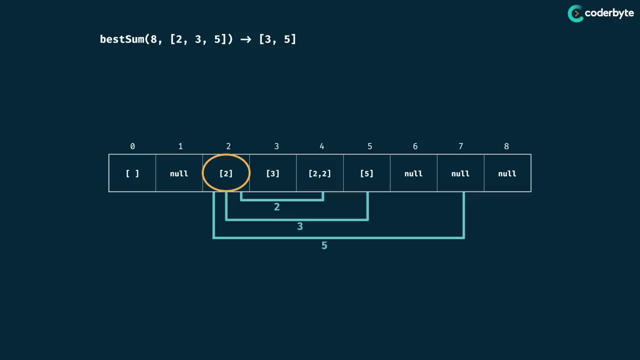 ahead. I see five spaces ahead. for my current position- yellow- there's a null right at index seven, which means that I can just go ahead and put this new array inside. So I copy over the array of two, then I add the five right, because that's how far I'm looking ahead. 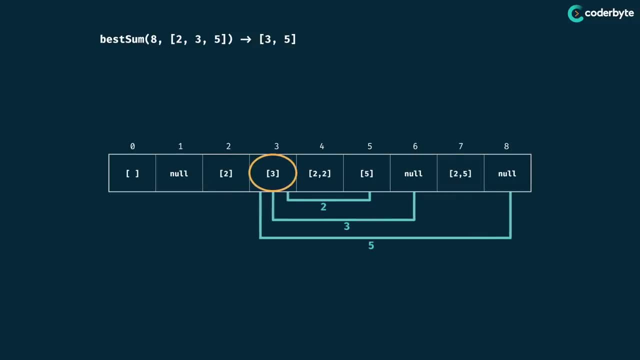 I keep this process rolling, I'm going to modify two spaces ahead. Notice that this sub array I'm considering would still be longer than what's already stored at index five. So I actually don't use the three comma two. right, the five gets to stay. Now I look three spaces ahead And this would 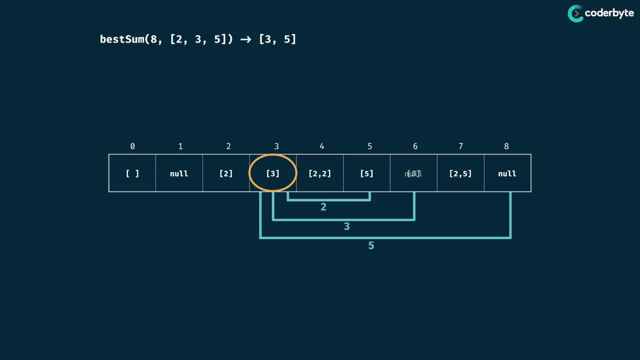 actually be the first time. I found at least a way to generate six. So I copy over my current array and also add my look ahead value And now, if I look five spaces ahead, there's a null currently in that index eight, which means that I'm actually 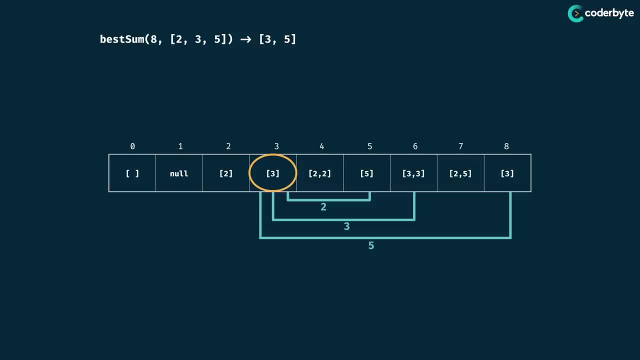 finding the first way to generate eight. So I copy over my array of three And then I add my five for my look ahead. Cool, And at this point we've actually already found a way to generate eight, And you can probably foresee that this would be the shortest way. 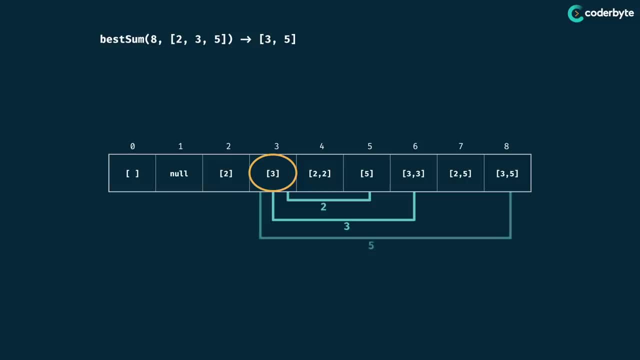 in the long run, However, if we kind of continued this algorithm, there would actually be nothing wrong with continuing it, right? it's not like we're ever going to put something longer in that spot. So if we continue our algorithm as normal, if I look two spaces ahead from 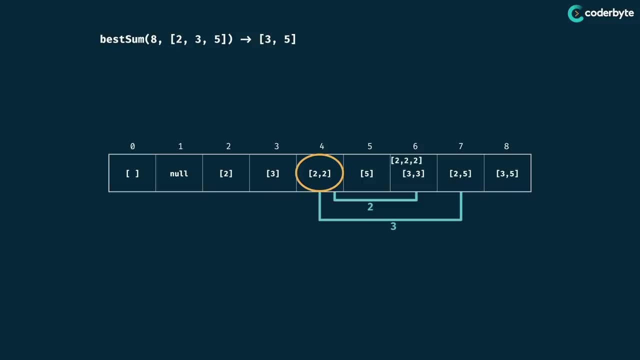 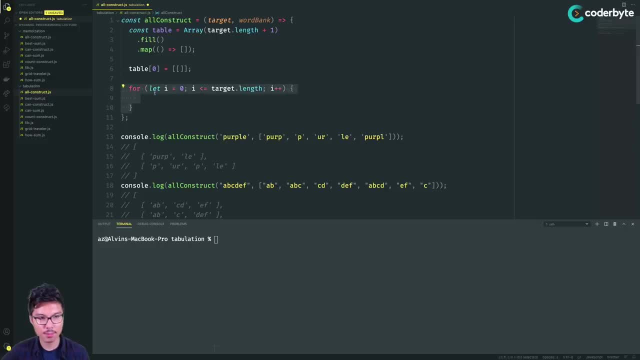 times before. So I'm iterating through my table And what I'll also do is look at all of the words right? So on every iteration I'm going to consider some words of the word bank. So I'll say: let word of word bank And, like before, I still need to check that right. 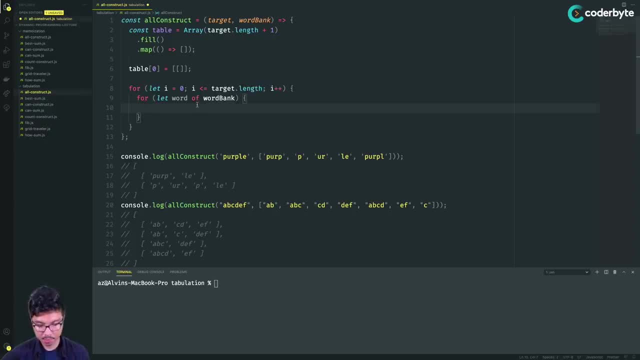 these words better have matching characters, based on my current position. So I'll use that classic logic- right seen it many times by now- And I'll slice a segment out of my target string. I'll say target dot slice, starting index i and grabbing the next word. 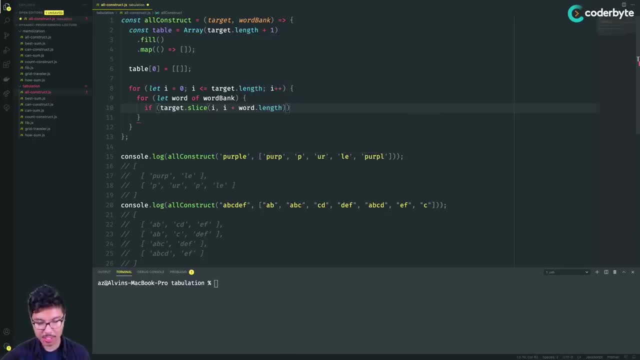 dot. length: number of characters: Cool, I'm going to compare that chunk to the current word that I'm iterating through Nice. So using this if statement, I'm sort of filtering down all the words and only going to do some logic on the words that match based on my 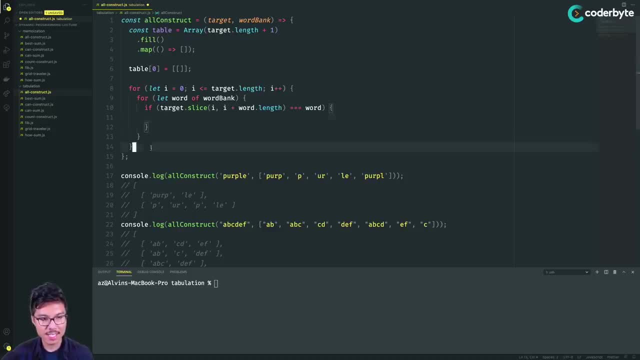 current position, Nice, And so we've seen, you know this- nested for loop and if statement before right we're now, we're adding our new logic within this if statement goal. all I need to do is really understand what types. 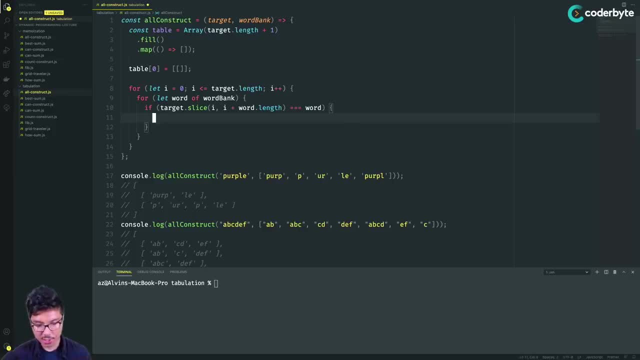 of data I'm dealing with here. Alright, so let's say I just wrote this expression table at index i. what that's going to do is just reference my current spot in the table And if I think about what data it's going to be, it's definitely going to be an array, right? 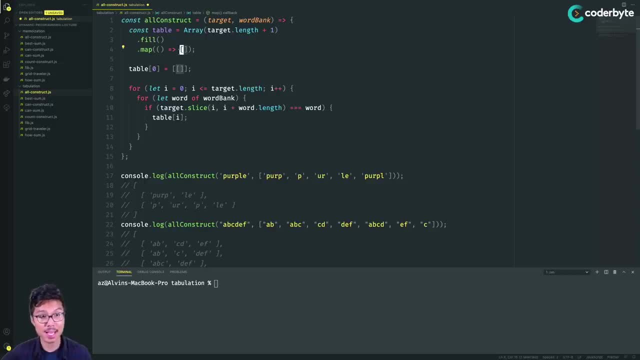 It's either going to be like an empty array, meaning there are no ways to make this current target, Or it could be a multi dimensional array where every sub array represents one way I can make the current target. So if this is all of the combinations that generate my current, then what I'll do is 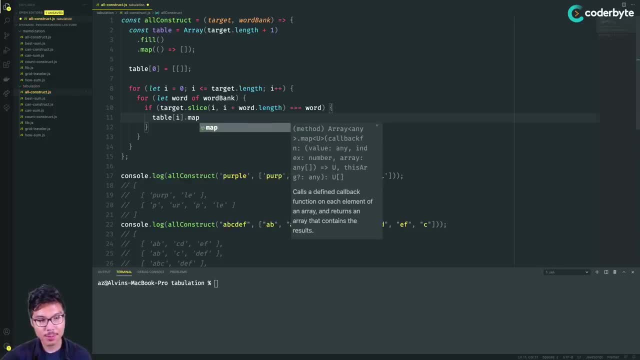 I'm going to map over them. Remember, in our drawing what we did was kind of copy over all of our current combinations, But then make sure we also add our word that we're using right now to the end of each of those combinations. So that's what I'm doing, right? 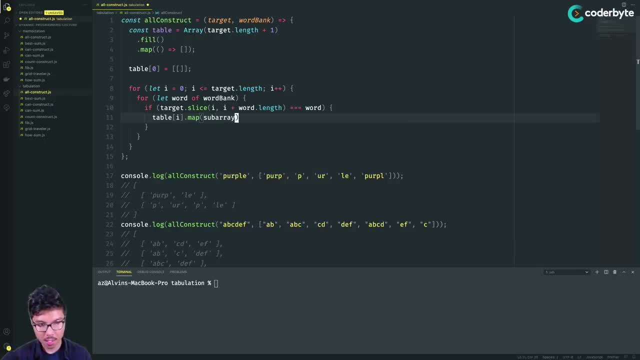 here I'm going to map over every sub array, And what I'll do is I'll just copy over the elements of that sub array using that spread syntax that we've seen before, And then I'm going to add in my word, And then I'll also be sure to add on at the end my word: Nice. 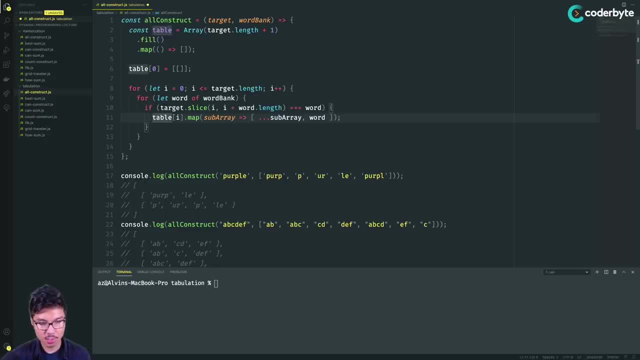 And then that will give me, let's say, our new combinations. So I'll just say that to a variable maybe. So new combinations is going to be a 2d array right where every sub array represents some combination, And I want to take these combinations and add them into that further. 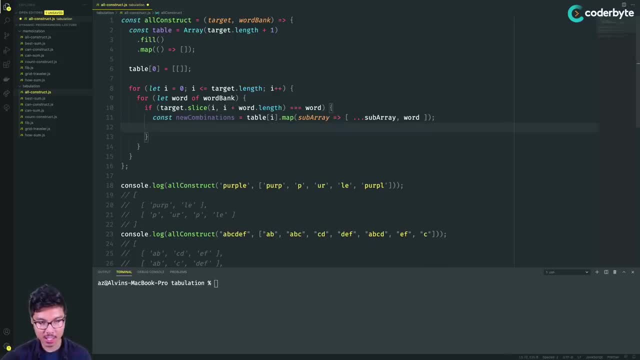 spot inside of my table. So I know I need to kind of look ahead in my table So I can look at table at index I. So I know I need to kind of look ahead in my table So I can look at table at index I. 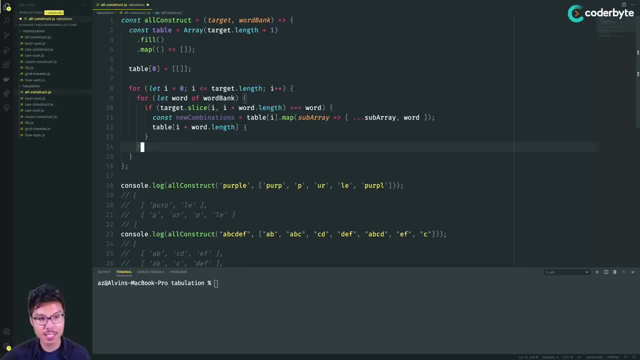 plus word length. And I know that all positions of the table are going to be arrays, right? So this is going to be an array. there's going to be some data that might already exist at this position, right? So what I don't want to do is just assign new combinations, because then that would overwrite. 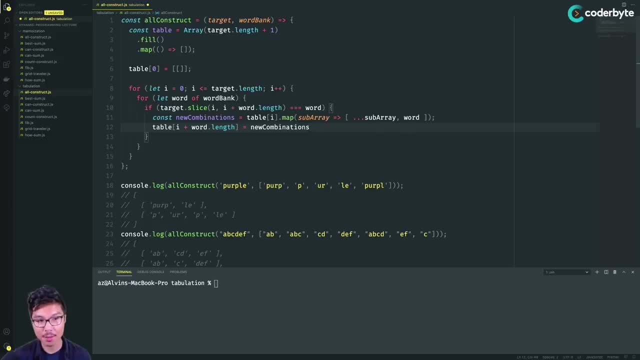 any previous existing combinations that I already found for this position. Instead, I need to make sure that I just add these new combinations to that list, right? So what I'll do here is: I'll push to that array, I'll push all of the elements of my new combinations right. So here I can. 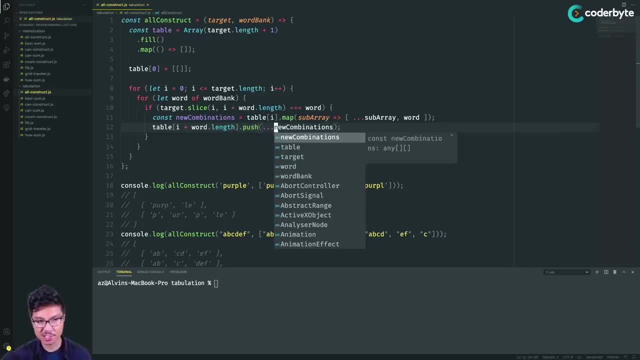 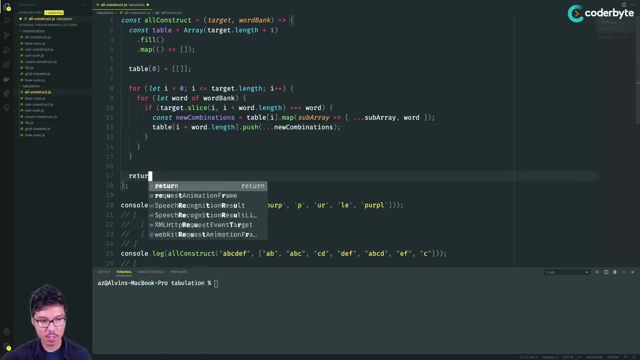 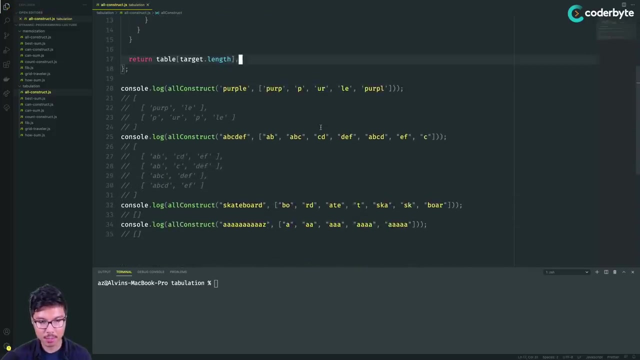 spread this out. when I spread it out that way, I don't add any additional nesting over here, right? So this is looking pretty good. I think let's go ahead and return the table at target dot length Here. I have some examples down below. Let's give this a shot. 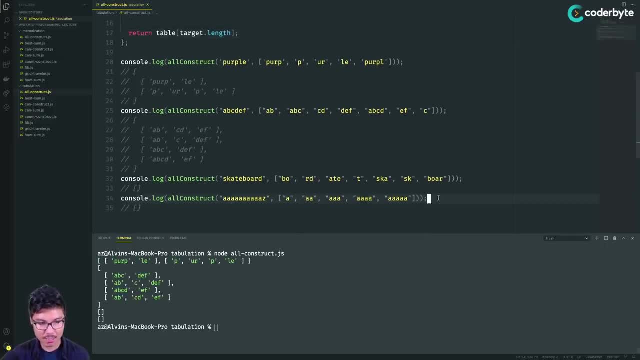 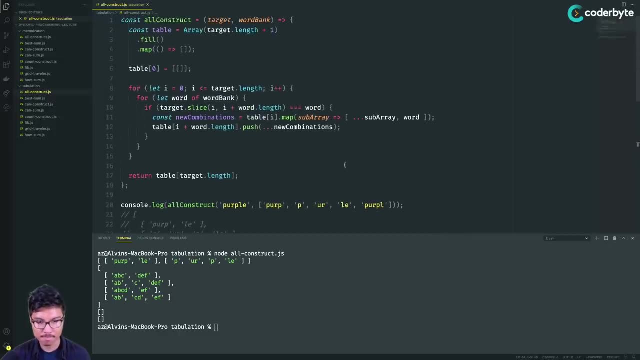 Nice, And these answers look correct, right? Notice that these last two examples should return empty arrays because they are impossible to generate. Cool, So let's hover over this code for a moment. Probably the most tedious logic here would be these two lines, right? Really, try to understand how, like these two lines translate. 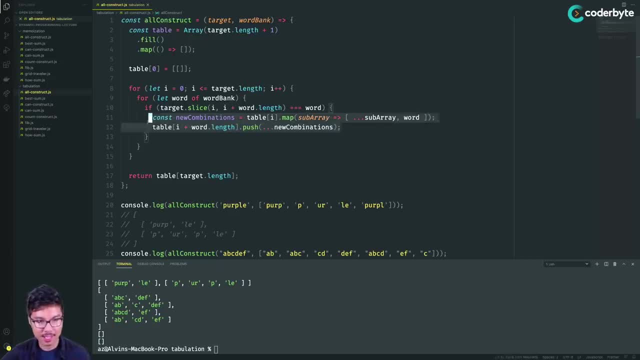 into the logic we did in our drawing. So let's break down these lines again, right, Line 11 is going to take all of the combinations in my current position in my drawing that was like my yellow box, And it's going to add: 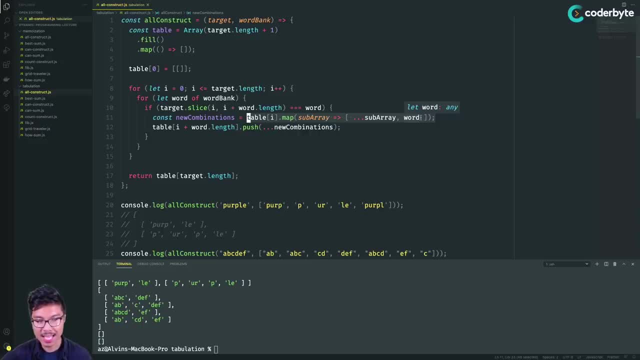 Add our current word to each of those combinations, and then we're going to take each of those new arrays and add them to the list at our further position, right being sure not to overwrite. We already spoke about the complexity of this one. it's definitely going to be. 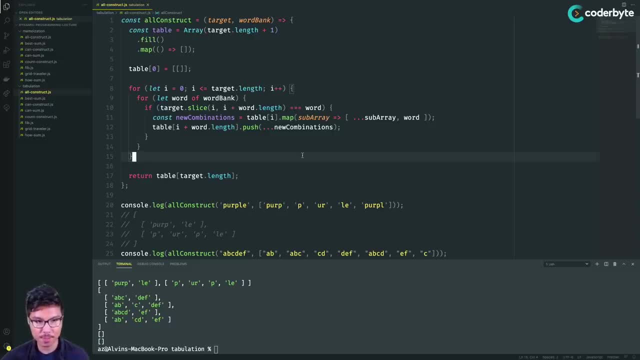 exponential, probably a little more than exponential, Right? If you imagine all the work we have to do using these maps and, like spreading, we have to actually construct our results array, which is going to contain an exponential number in this result array. So we're going to grab some. like this fundamental again because we have some. Well, we just ran into a session where we're going to get ourselves taken over and set some math rules. let's try to create some felicidades to the other kind of like complex way. So this is going to take some good examples and let's see what we can do. first, 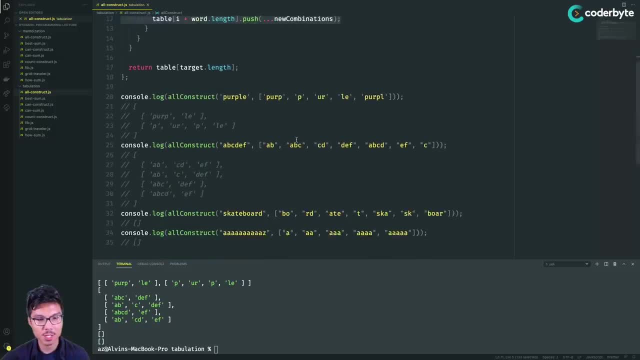 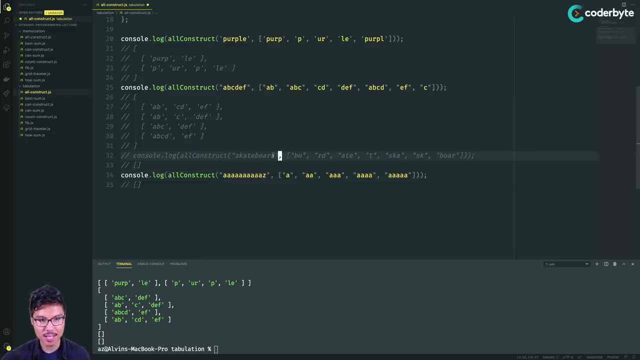 an exponential number of things, Right? So even if I look at this last example, let's say that I made it a little longer, right? So let's say, actually blew up the size of that input. It's going to be very, very slow, might even crash, but let's just do it So. 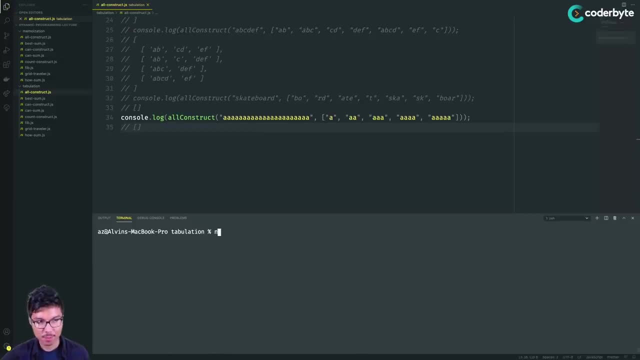 let's say I had a bunch of A's here just for fun. So if we try this example, Yeah, looks like our program still crashes, right? This is going to return a really, really a massive array- probably can't even fit into memory over here, right? So we'll get like: 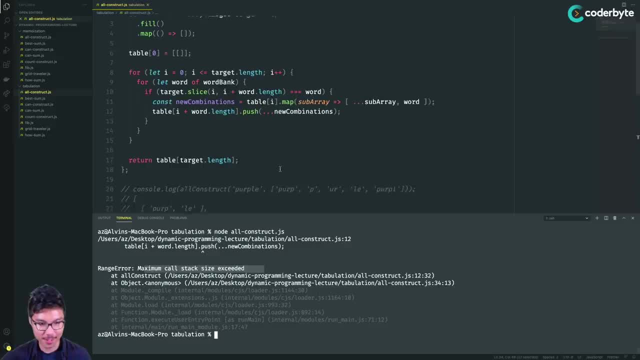 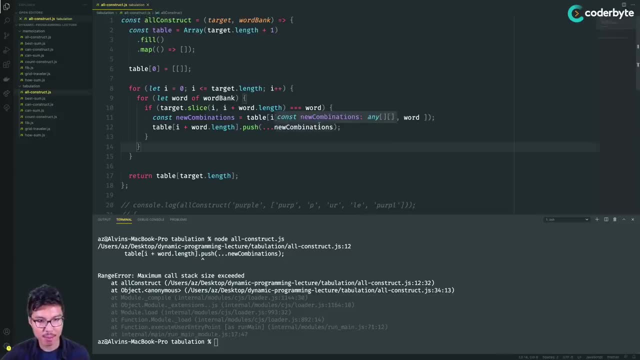 a stack size exceeded, even though this isn't even recursive right. Just calling functions a way too much over here. So, no matter what we do, we really expect this problem to sort of demand an exponential solution. With that. let's head back into the drawing board, where 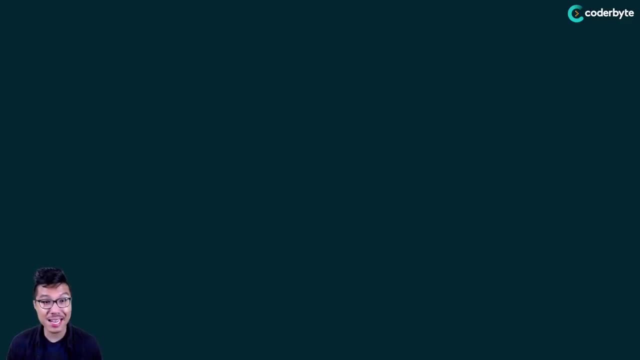 we can wrap up this course. Alright, programmers, by now we've solved many different dynamic programming problems together, And I want to leave us with some final advice. So whenever you're starting to attack any dynamic programming problem, start by really taking a moment and noticing any overlapping. 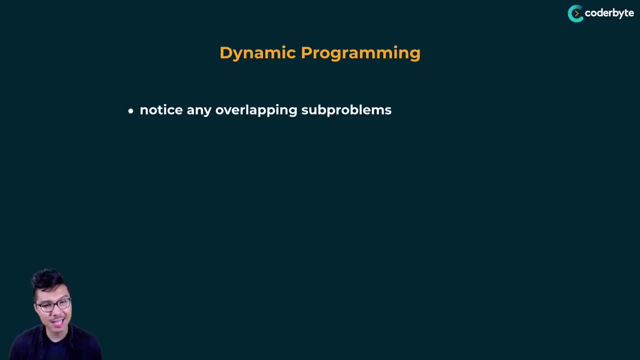 sub problems And then from there really focus on, like the input to the problem, in particular its type, And from there you should be able to recognize what is the trivial, smallest input. So in our string problems usually that means the empty string. in our array problems 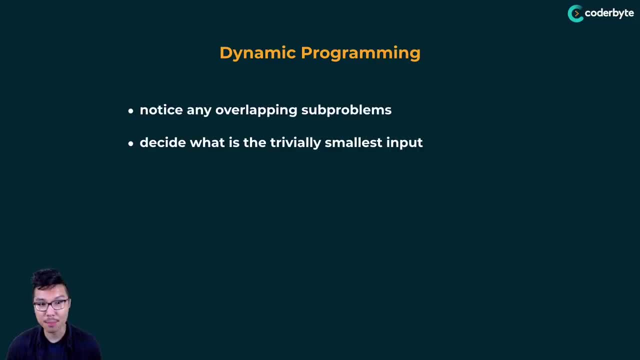 it's the empty array or in our number problems, it's usually a number like zero or one right. Is there some input? Is there an input? So, for example, in this case we're going to be using the step number five If the number